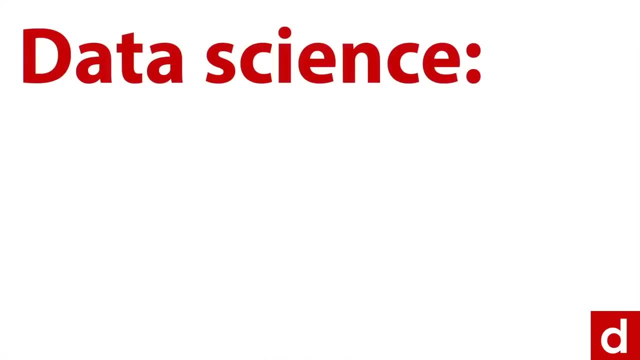 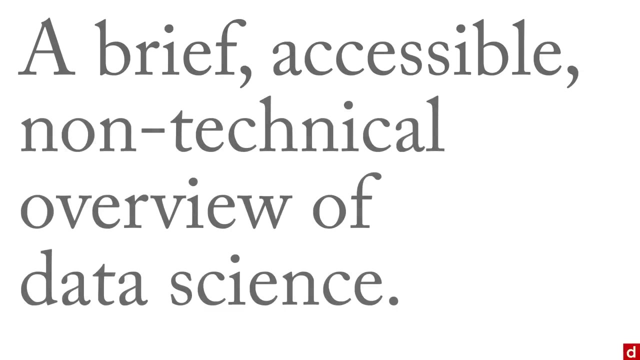 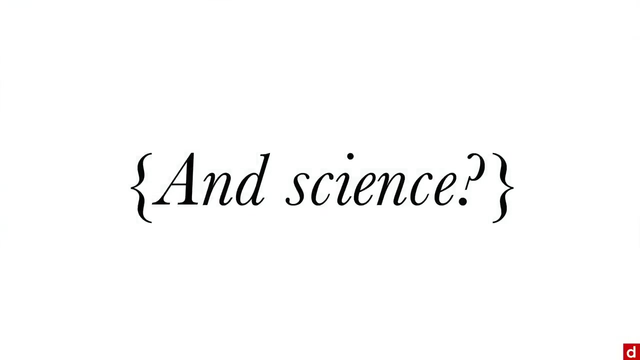 Welcome to Data Science. An Introduction. I'm Barton Poulsen, and what we're going to do in this course is we're going to have a brief, accessible and non-technical overview of the field of data science. Now, some people, when they hear data science, they start thinking things like data and think about piles of equations and numbers, and then to throw on top of that science and think about people working in their lab and they start to say: that's not for me. I'm not really a technical person and that just seems much too techie. 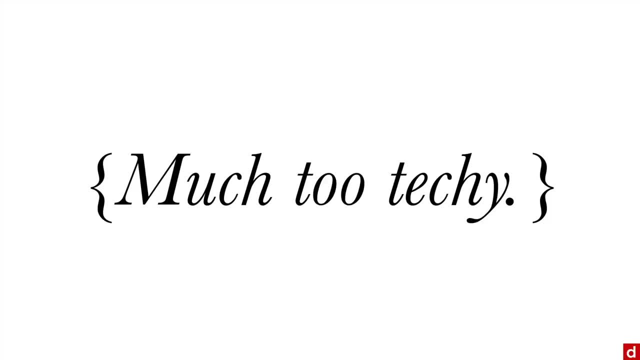 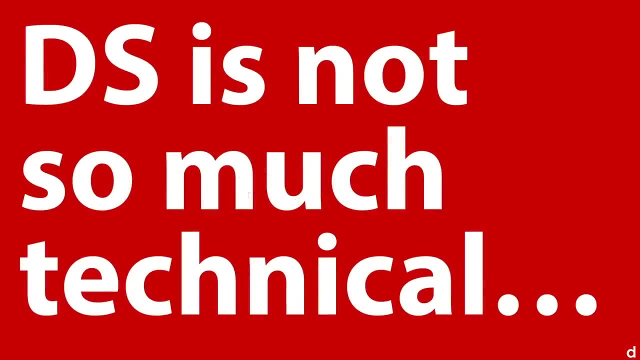 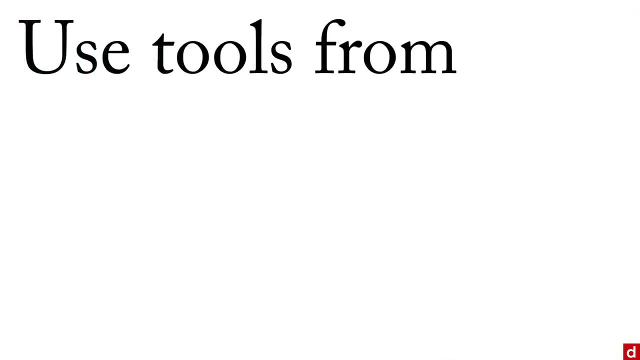 Well, here's the important thing to know. While a lot of people get really fired up about the technical aspects of data science, the important thing is that data science is not so much a technical discipline but creative, And really that's true. The reason I say that is because in data science, you use tools that come from coding and statistics and from math, but you use those to work creatively with data. 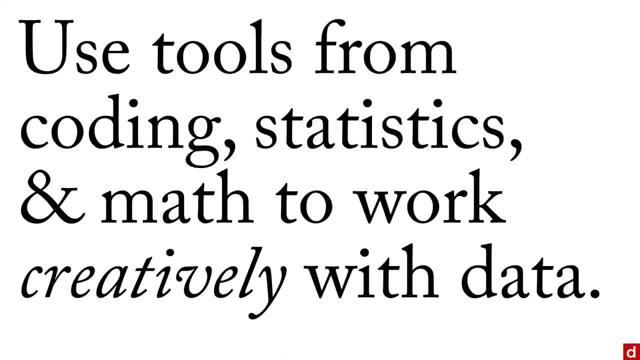 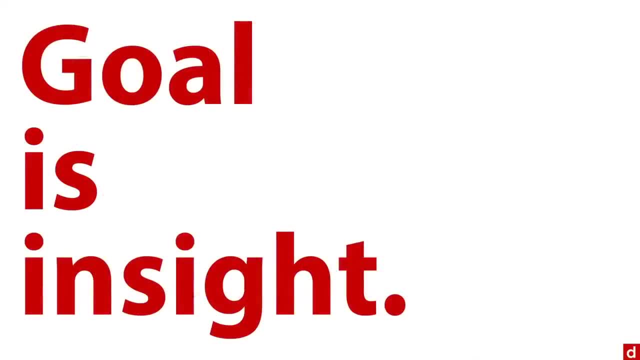 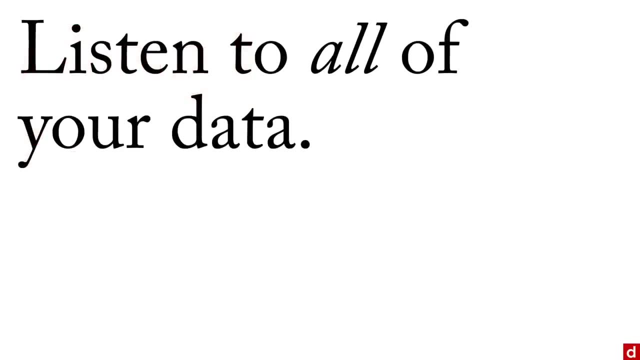 The idea is that there's always more than one way to solve a problem or answer a question and, most importantly, to get insight, because the goal, no matter how you go about it, is to get insight from your data, And what makes data science unique compared to so many other things is that you try to listen to all of your data, even when it doesn't fit in easily with your standard approaches and paradigms. 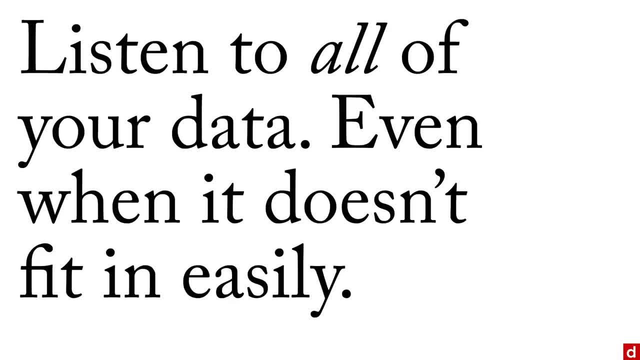 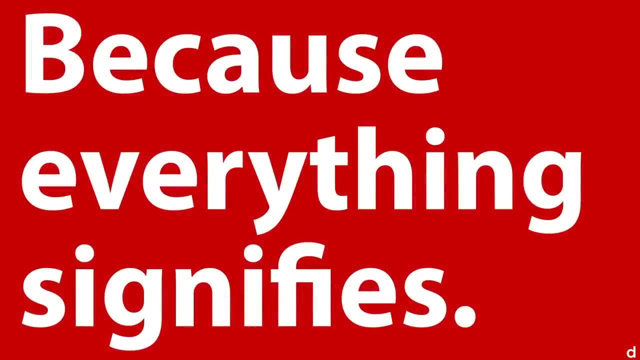 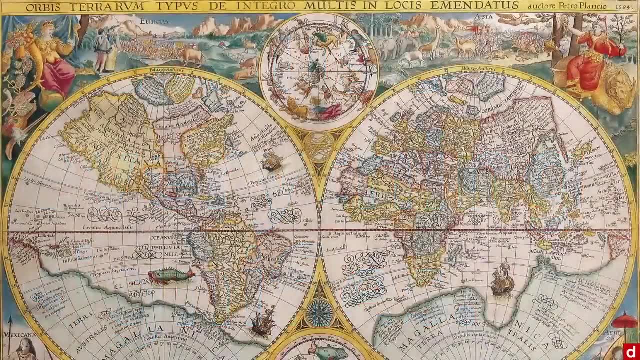 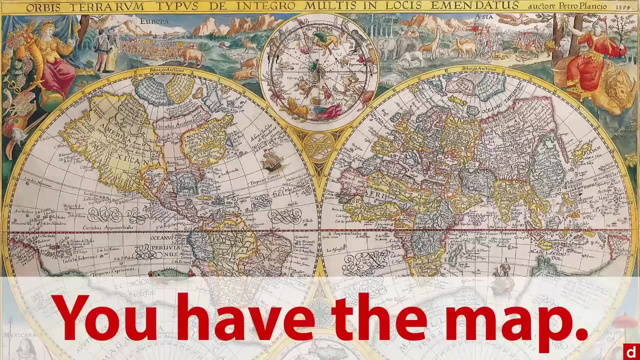 You're trying to be much more inclusive in your analysis, and the reason you want to do that is because everything signifies, everything carries meaning and everything can give you additional understanding and insight. And so in this course, what we're trying to do is give you a map to the field of data science and how you can use it, And so now you have the map in your hands and you can get ready to get going with data science. 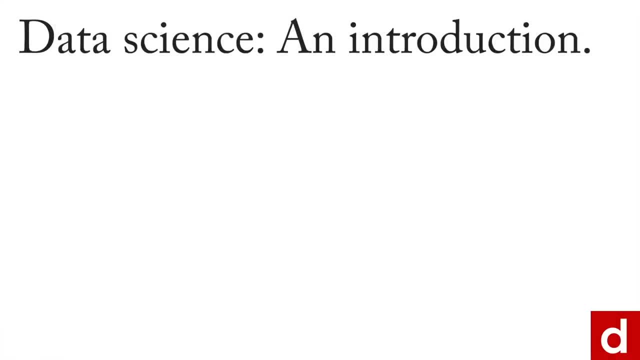 Welcome back to Data Science in Introduction, and we're going to begin this course by defining data science. That makes sense, But we're going to do it in kind of a funny way. The first thing I'm going to talk about is the demand for data science. 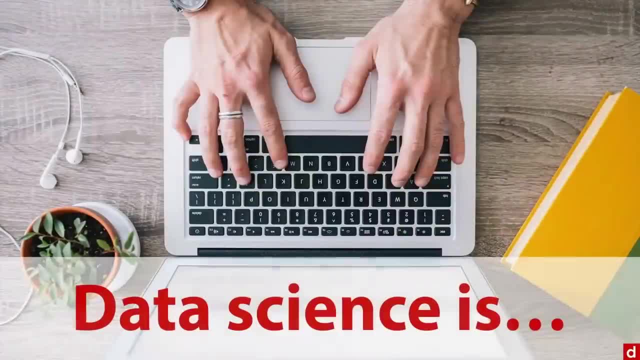 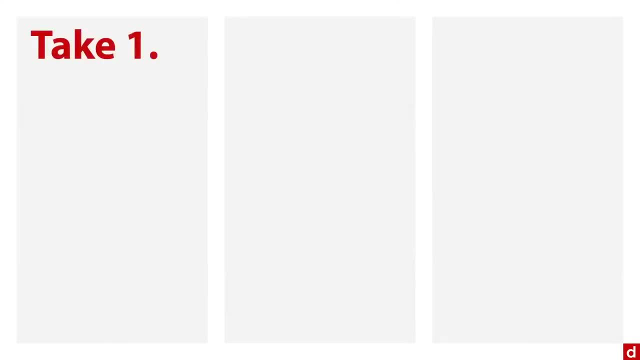 So let's take a quick look Now. data science can be defined in a few ways. I'm going to give you some short definitions. Take one on. my definition is that data science is coding math and statistics in applied settings. That's a reasonable, working definition. 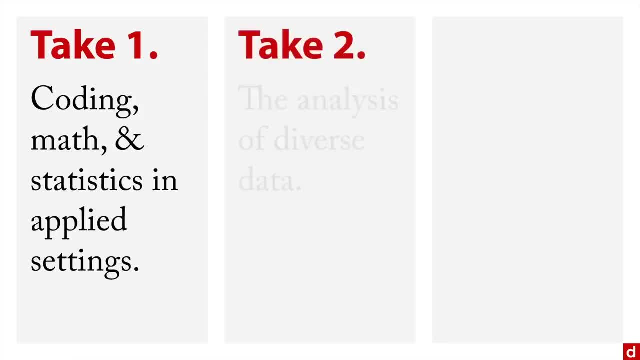 But if you want to be a little more concise, I've got- take two on a definition- that data science is the analysis of diverse data or data that you didn't think would fit into standard analytic approaches. A third way to think about it is that data science is inclusive analysis. It includes all of the data, all of the information that you have in order to get the most insightful and compelling answer to your research questions. 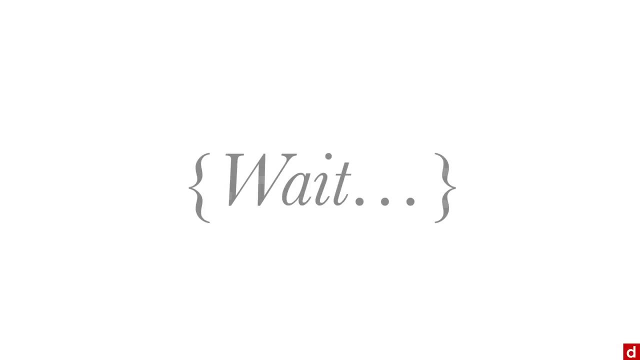 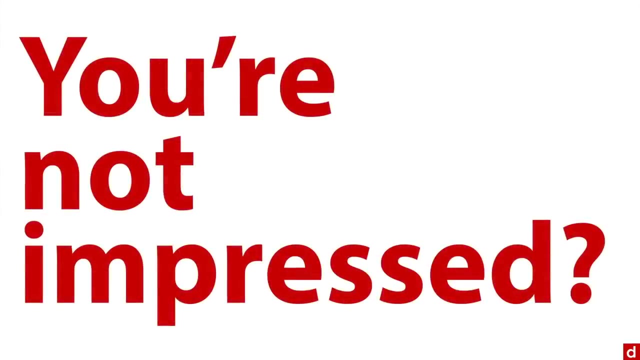 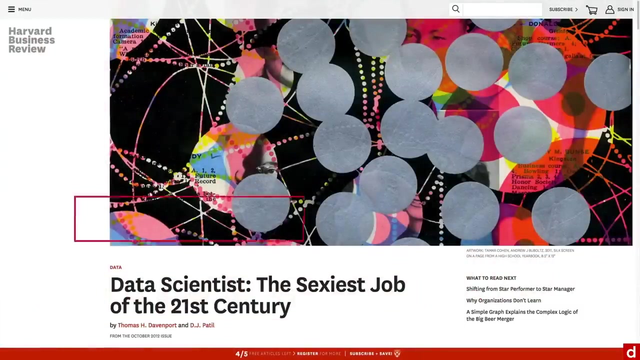 Now you may say to yourself: wait, that's it. Well, if you're not impressed, let me show you a few things. First off, let's take a look at this article. scientists, the sexiest job of the 21st century, and please note that this is. 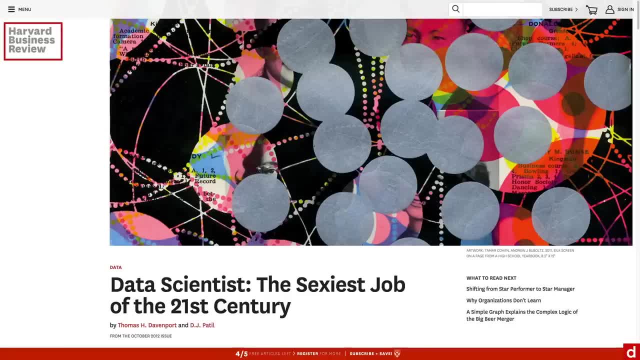 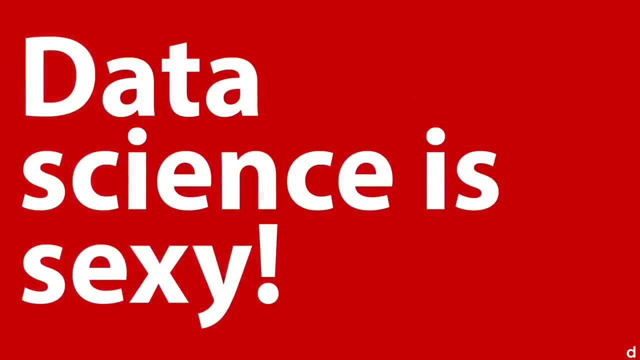 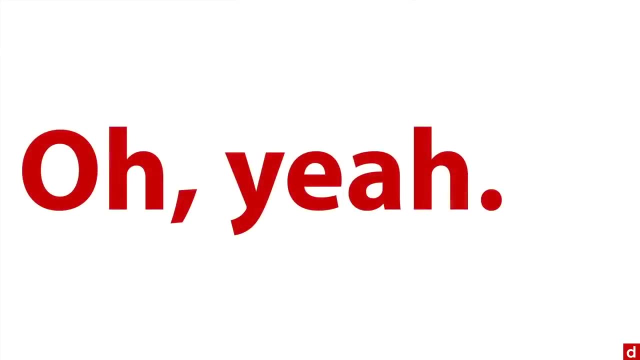 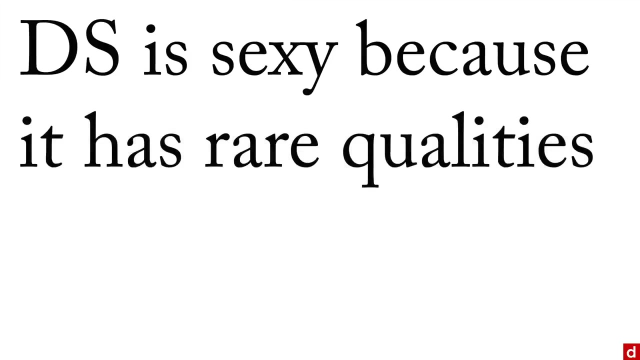 coming from Harvard Business Review. so this is an authoritative source and it's the official source of this, saying that data science is sexy. yeah, again, you may be saying to yourself: sexy? I hardly think so. oh, oh, yeah, it's sexy. and the reason data science is sexy is because, first, it has rare qualities and, second, 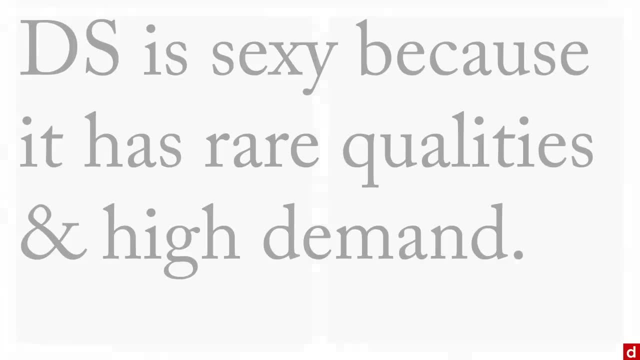 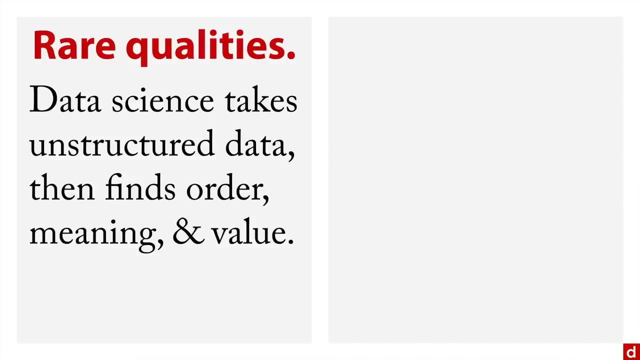 it has high demand. let me say a little more about those. the rare qualities are that data science takes unstructured data, then finds order, meaning and value in the data. those are important but they're not easy to come across. second, high demand. well, the reason it's in high demand is because data science provides 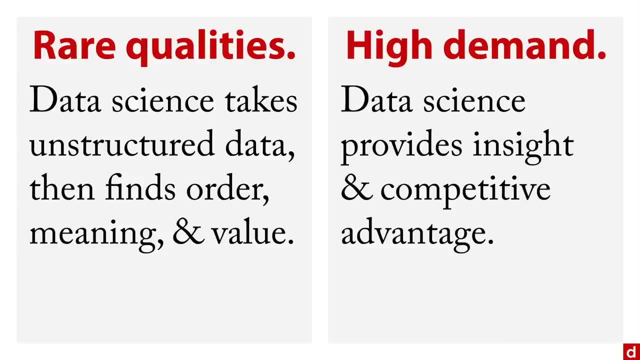 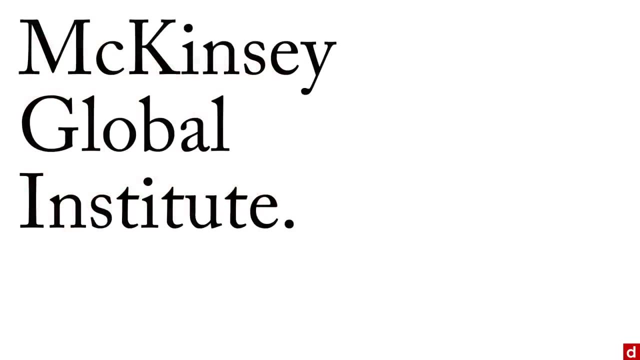 insight into what's going on around you and, critically, it provides competitive advantage, which is a huge thing in business settings. now let me go back and say a little more about demand. let's take a look at a few other sources. so, for instance, the McKinsey Global Institute published a 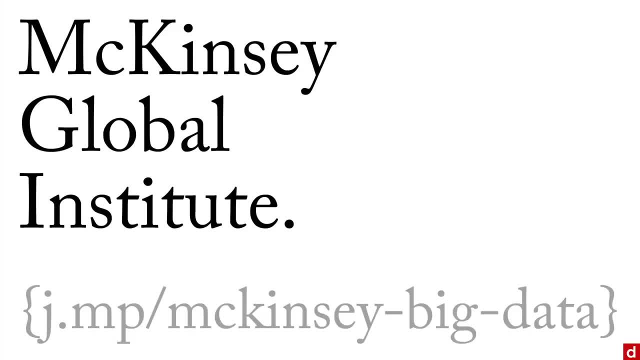 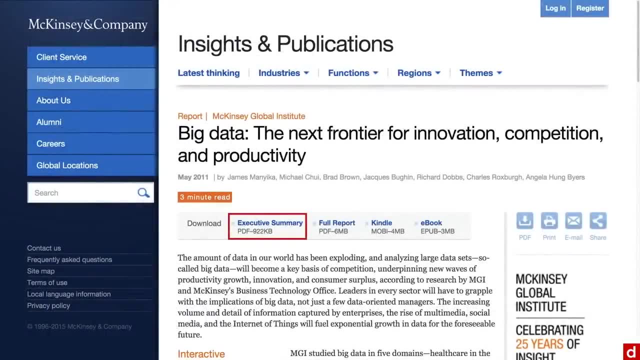 very well-known paper and you can get at it with this URL and if you go to that web page, this is what's going to come up, and we're going to take a quick look at this one: the executive summary. it's a PDF that you can download and, if you, 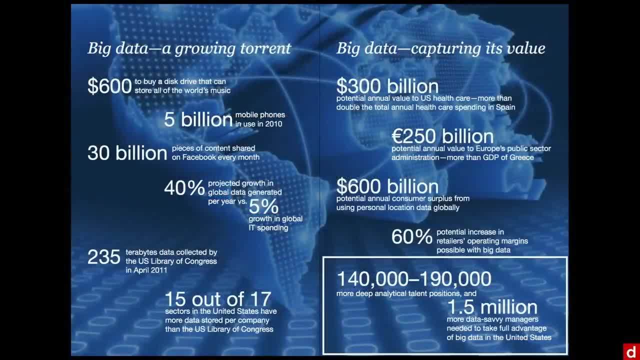 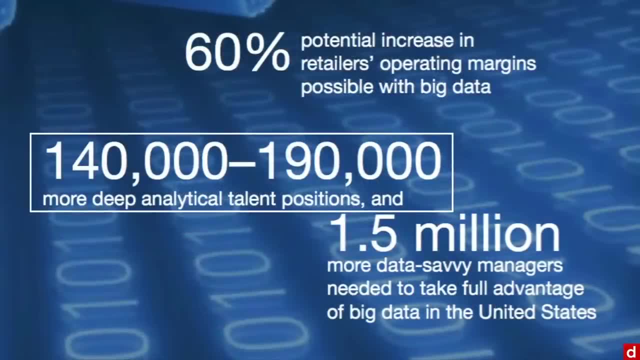 open that up, you'll find this page and let's take a look at the bottom right corner. two numbers here. I'm going to zoom in on those. the first one is they are projecting a need in the next few years for somewhere between 140 and 190 thousand deep analytical talent. 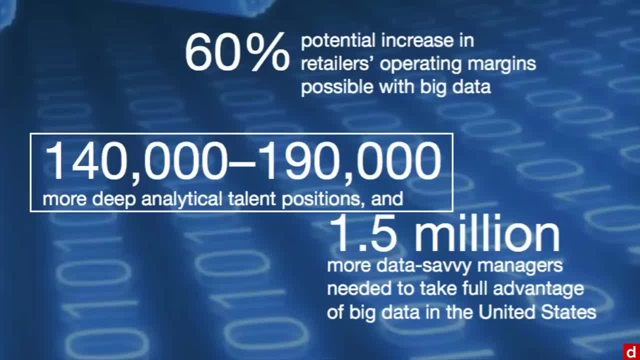 positions. so this means actual practicing data scientists. that's a huge number, but almost ten times as high is 1.5 million more data savvy managers will be needed to take full advantage of big data in the United States now. the second one is the data science, that's people who aren't necessarily doing the 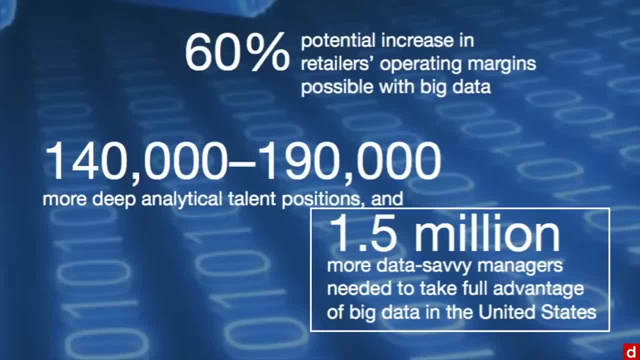 analysis, but have to understand it. you have to speak data, and that's one of the main purposes of this particular course is to help people who may or may not be the practicing data scientists learn to understand what they can get out of data and some of the methods used to get there. let's take a look at another. 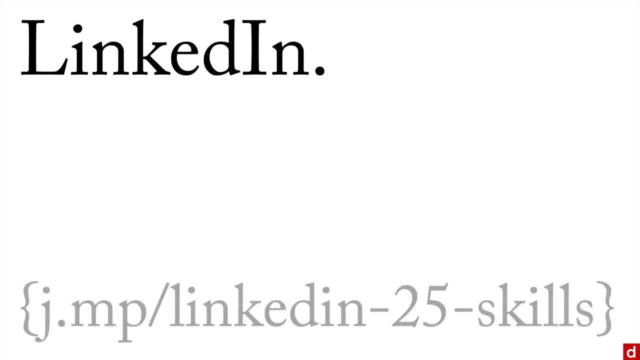 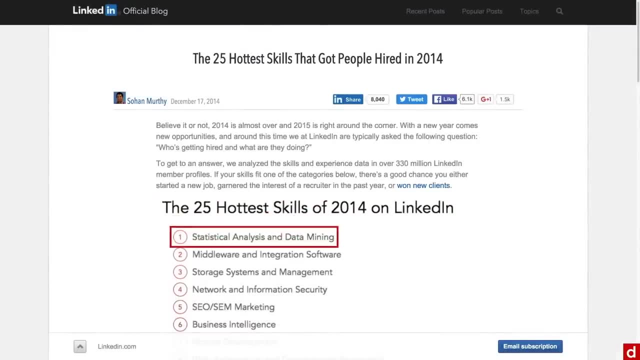 article from LinkedIn. here's a shortcut URL for it and that will bring you to this webpage: the 25 hottest job skills that got people hired in 2014. and take a look at number one here: statistical analysis and data mining very closely related to data science and, just to be clear, this was number one in Australia. 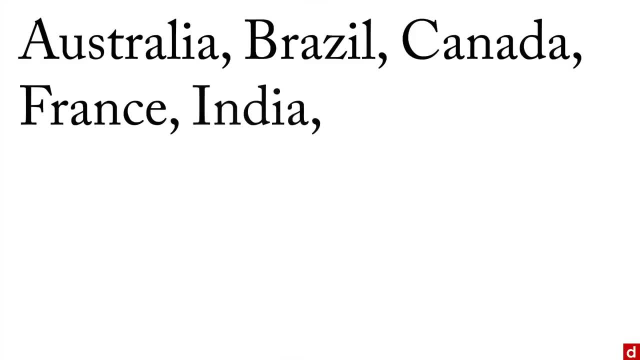 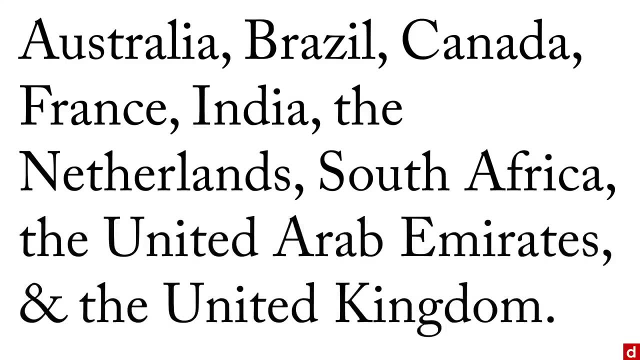 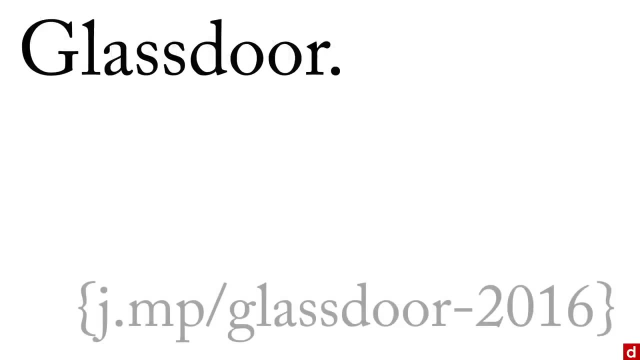 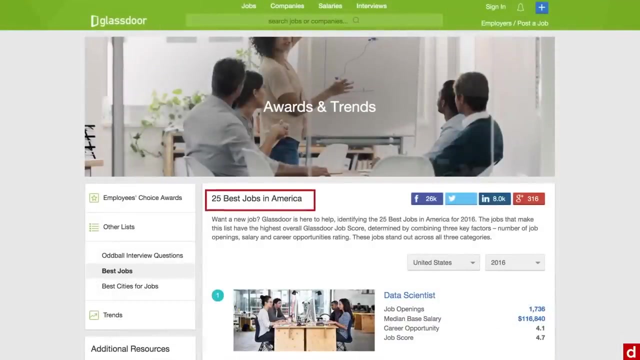 and Brazil and Canada and France and India, in the Netherlands, in South Africa and the United Arab Emirates, in the United Kingdom, everywhere. and if you need a little more, let's take a look at Glassdoor, which published an article this year, 2016, And it's about the 25 best jobs in America. And look at number one right here: It's data. 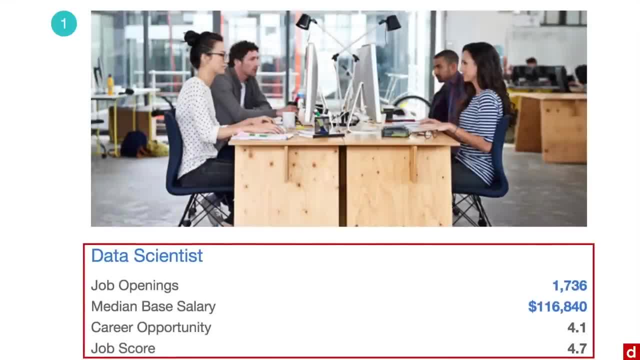 scientists And we can zoom in on this information. It says there's going to be 1700 job openings, with a median base salary of over 116,000 and fabulous career opportunities and job scores. So if you want to take all of this together, the conclusion you can reach is that data science pays, And I 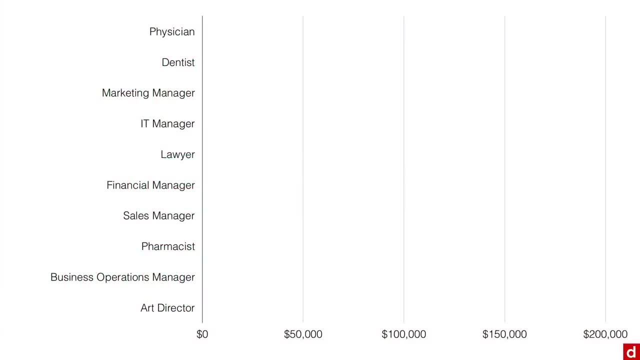 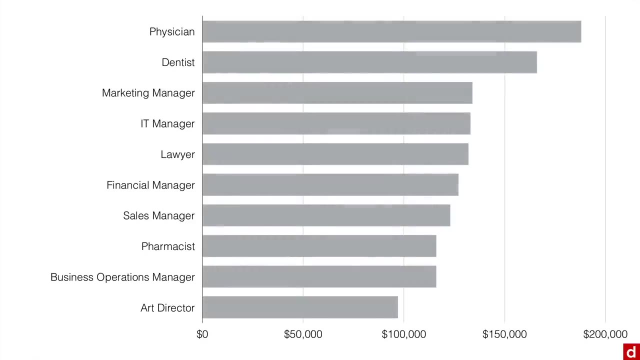 can show you a little more about that. So, for instance, here's a list of the top 10 highest paying salaries that I got from US News. We have physicians or doctors, dentists and lawyers and so on. Now, if we add data scientists to this list, using data from O'Reillycom, we have to push. things around the site. And it goes in third with an average total salary, not the base that we had in the other one, but the total compensation of about $144,000 a year. That's extraordinary. So, in sum, what do we get from all of this? First off, we learned that there. 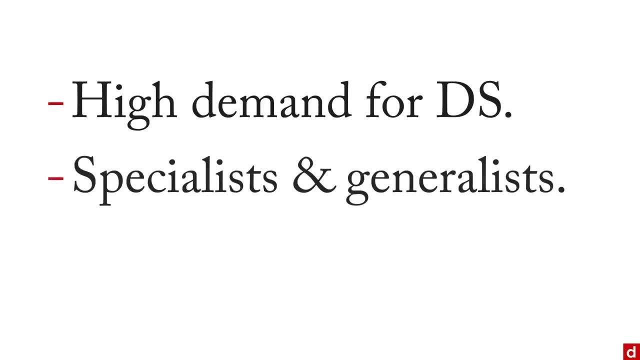 is a very high demand for data science. Second, we learned that there's a critical need for both specialists- those are the sort of practicing data scientists- and for generalists- people who speak the language and know what can be done. And, of course, there's excellent pay And all together. 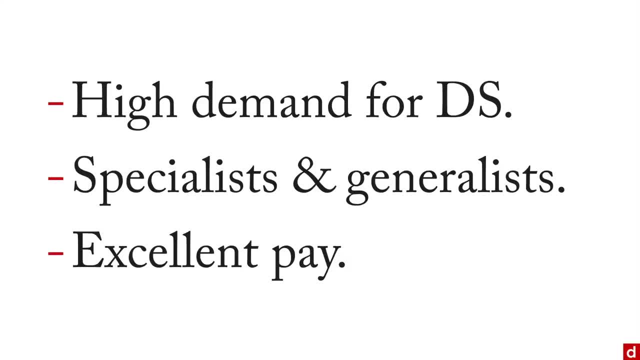 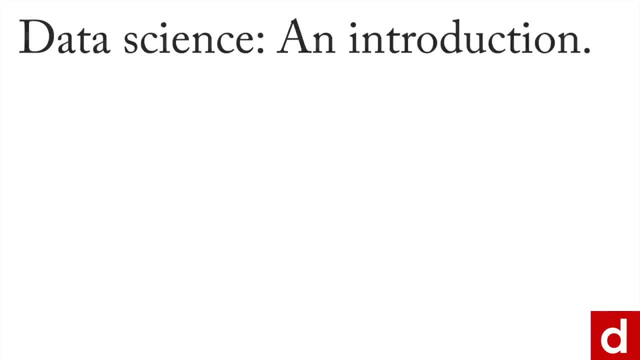 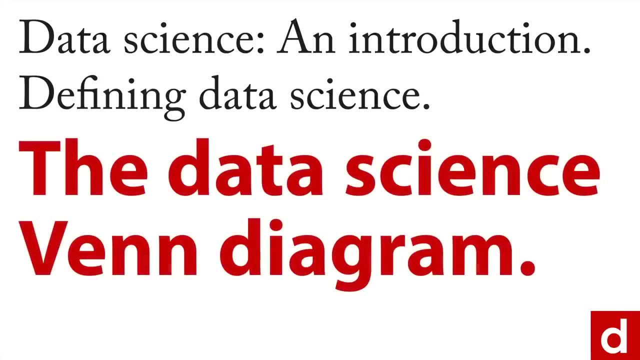 this makes data science a compelling career alternative and a way of making you better at whatever you're doing. Back here in data science, we're going to continue our attempt to define data science by looking at something that's really well known in the field: the data science Venn diagram. Now, if you want to, you can think of. 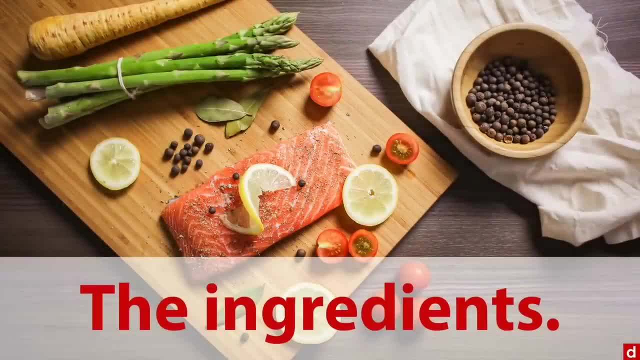 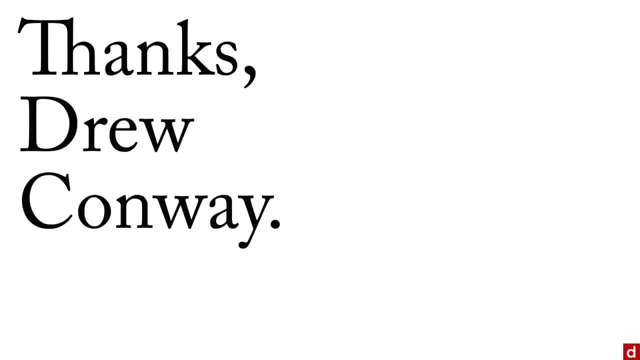 this in terms of what are the ingredients of data science. Well, we're going to first say thanks to Drew Conway, the guy who came up with this, And if you want to see the original article, you can go to this address. But what Drew said is that data science is made of three things And we can put them as overlapping circles, because it's the 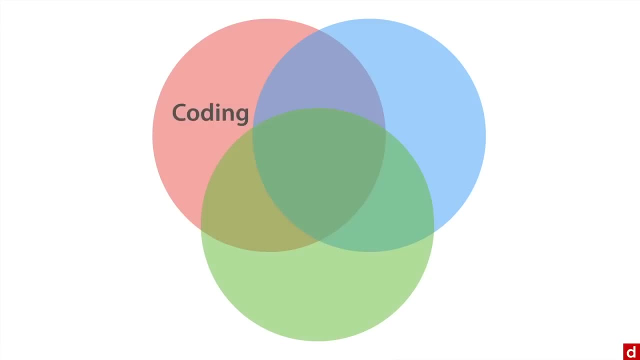 intersection that's important Here. on the top left is coding or computer programming, or, as he calls it, hacking, On the top right is stats or stats and mathematics or quantitative abilities in general, And on the bottom is domain expertise or intimate familiarity with a particular field of practice: business or health or education or something like that. 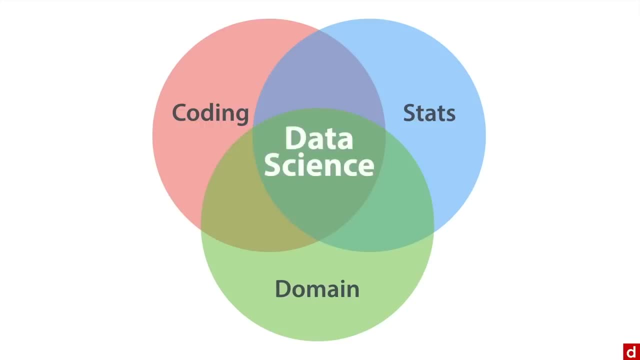 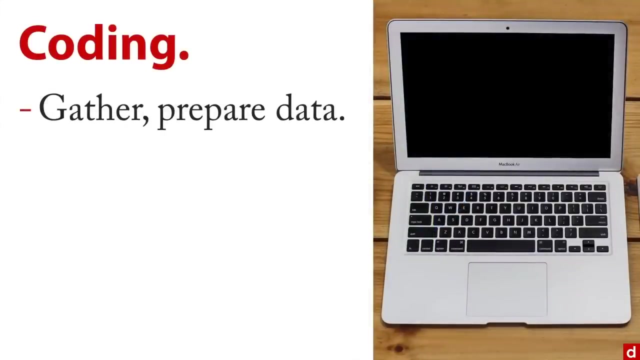 And the intersection here in the middle, that is data science. So it's the combination of coding and statistics and math and domain knowledge. Now let's say a little more about coding. The reason coding is important is because it helps you gather and prepare the data. 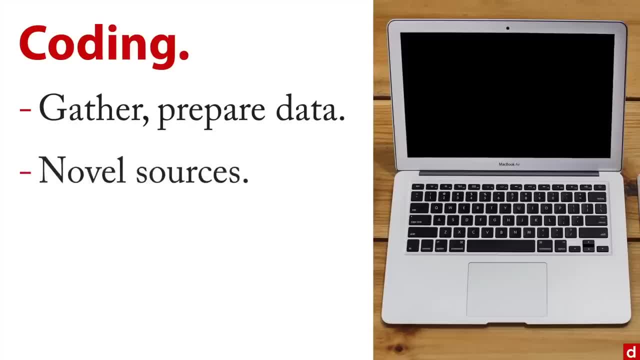 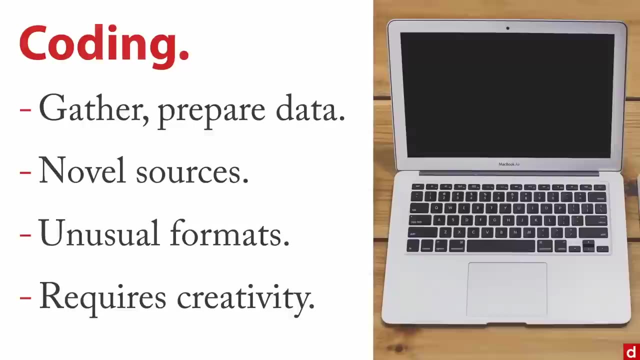 Because a lot of the data comes from novel sources and it's not necessarily ready for you to gather, And it can be in very unusual formats, And so coding is important because it can require some real creativity to get the data from these sources to put it into your analysis. 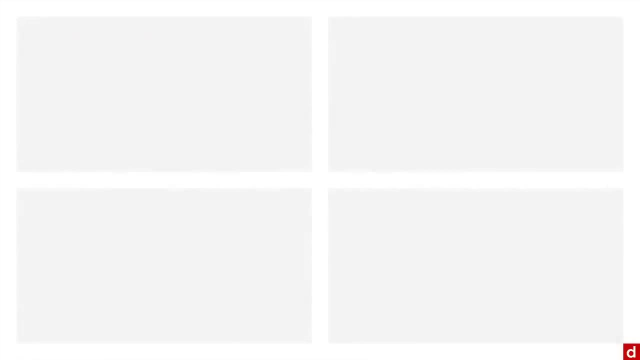 Now a few kinds of coding that are important. For instance, there's statistical coding. A couple of major languages in this are R and Python, two open source free programming languages. R specifically for data, Python's general purpose, but well adapted to data. 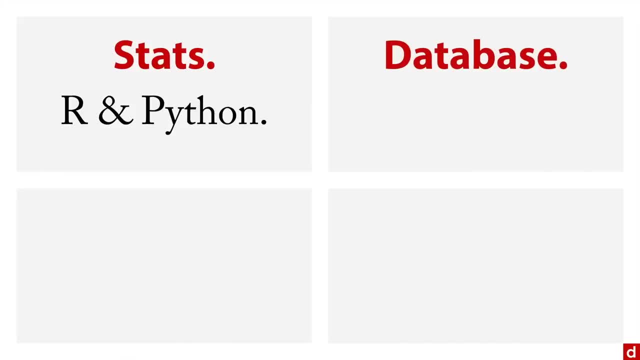 The ability to work with databases. This is important too. The most common language there is SQL, usually pronounced sequel, which stands for structured query language, because that's where the data is. Also, there's the command line interface or, if you're on a Mac, people just call it the. 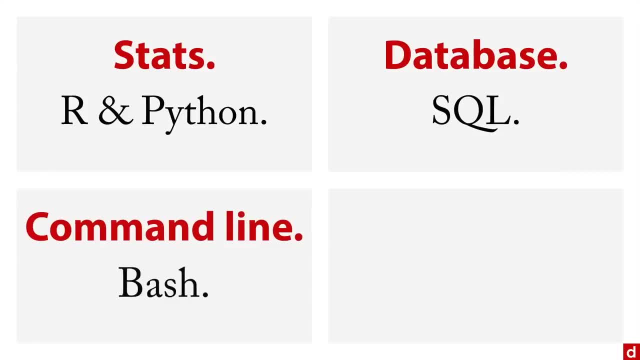 terminal. The most common language there is bash, which actually stands for born again shell, And then searching is important, and regex, or regular expressions. while there's not a huge amount to learn, But what you learn there it's a small little field. 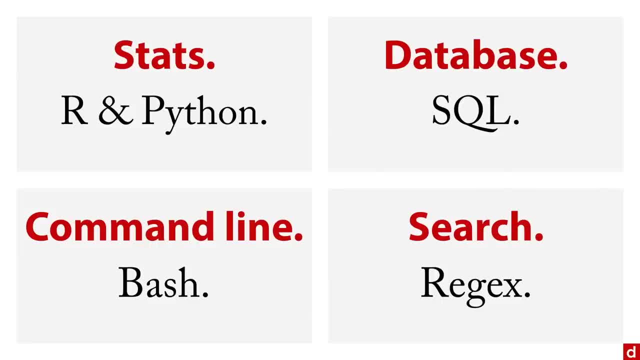 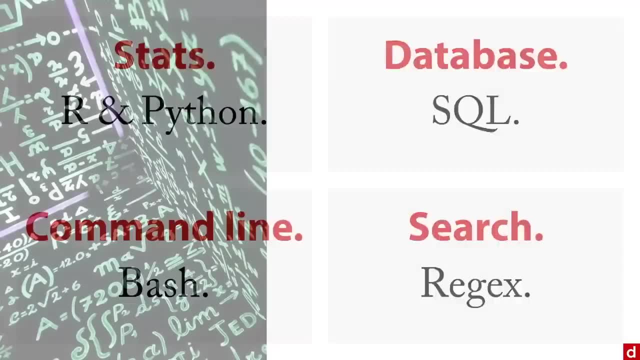 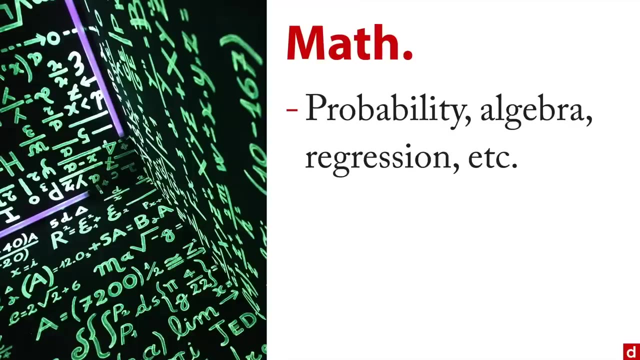 It's sort of like super powered wildcard searching that makes it possible for you to both find the data and reformat it in ways that are going to be helpful for your analysis. Now let's say a few things about the math. You're going to need things like a little bit of probability, some algebra, of course. 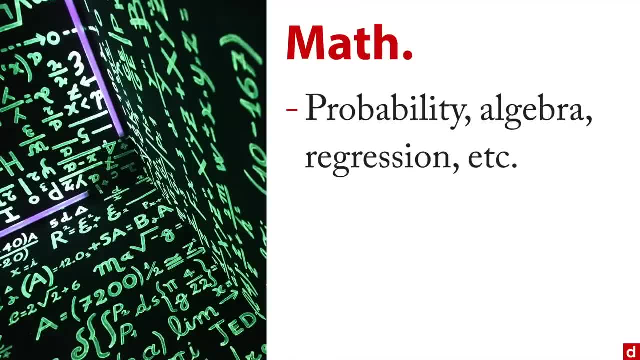 regression, very common statistical procedure. Those things are important And the reason you need the math is because that's going to help you choose the appropriate procedures To answer the question with the data that you have and probably even more importantly, it's going to help you diagnose problems when things don't go as expected. 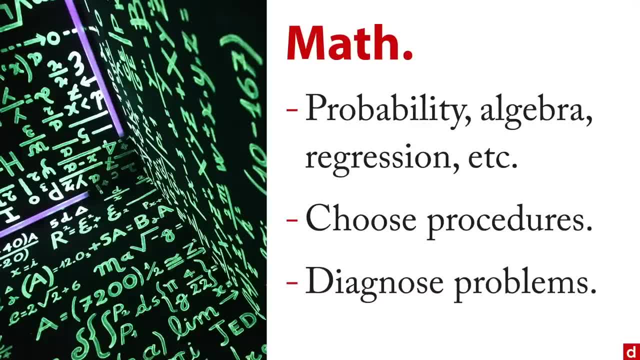 And, given that you're trying to do new things with new data in new ways, you're probably going to come across problems, And so the ability to understand the mechanics of what's going on is going to give you a big advantage. And the third element of the data science Venn diagram is some sort of domain expertise. 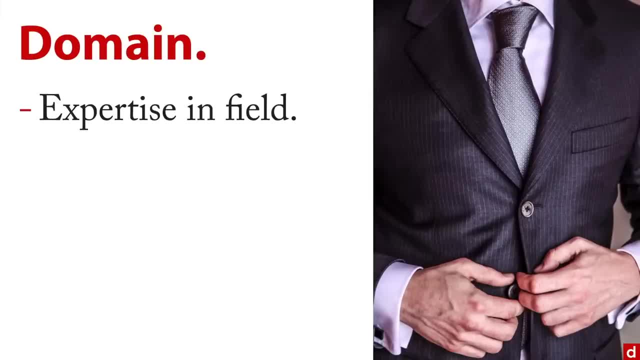 Think of it as expertise in the field that you're in. Business settings are common. You need to know about the goals of that field, the methods that are used, the constraints that people come across, And it's important because, whatever your results are, you need to be able to implement them. 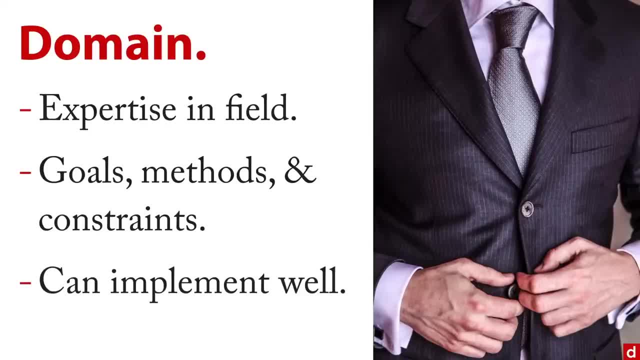 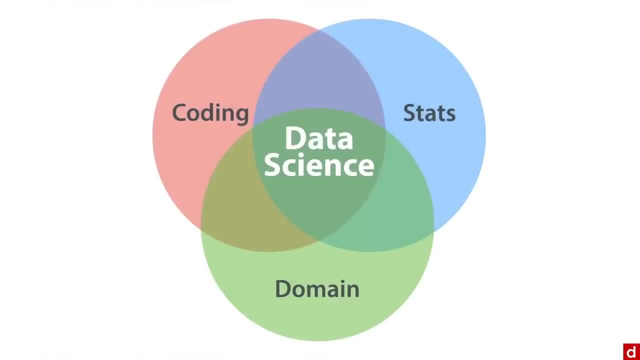 well, Data science is very practical and it's designed to accomplish something, And your familiarity with a particular field of practice is going to make it that much easier and more impactful when you implement the results of your analysis. Now let's go back to our Venn diagram here just for a moment. 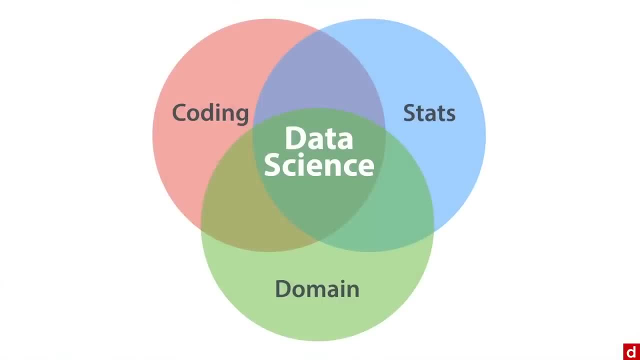 Okay, So this is a Venn. We also have these intersections of two circles at a time: At the top is machine learning, At the bottom right is traditional research and on the bottom left is what Drew Conway called the danger zone. Let me talk about each of these. 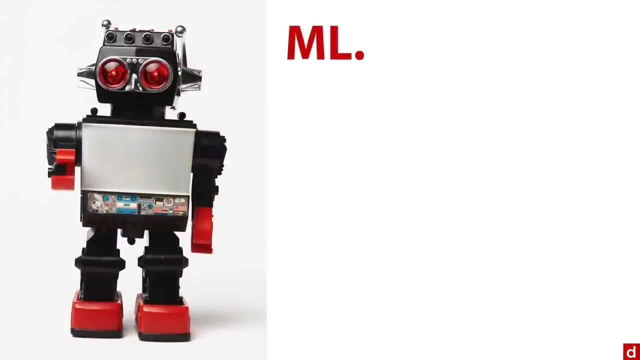 First off, machine learning or ML. Now you think about machine learning and the idea here is that it represents coding or statistical programming and mathematics without any real domain expertise. Sometimes these are referred to as black box models. They kind of throw data in and you don't even necessarily have to know what it means. 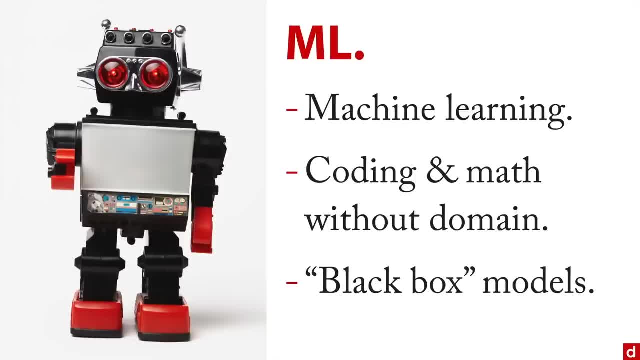 or what language it's in and it'll just kind of crunch through it all and it'll give you some regularities. That can be very helpful. but machine learning is considered slightly different from data science because it doesn't involve the particular applications in a specific domain. 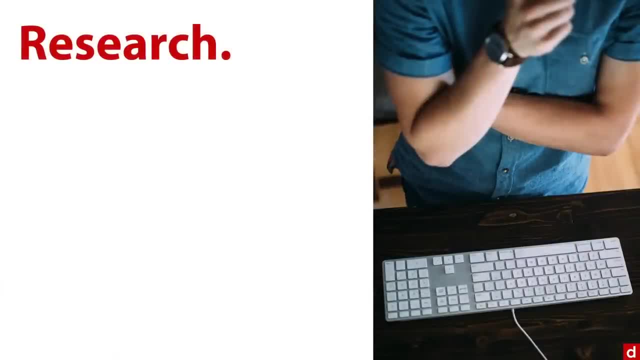 Also there's traditional research. This is where you have math or statistics and you have domain knowledge, often very intensive domain knowledge, But without the coding or programming. Now you can get away with that because the data that you use in traditional research 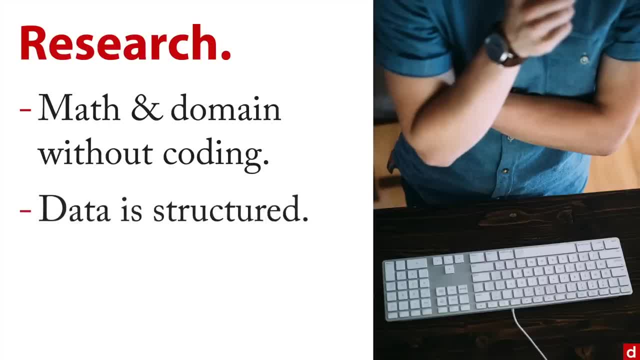 is highly structured, It comes in rows and columns, it's typically complete and it's typically ready for analysis. It doesn't mean your life is easy, because now you have to expend an enormous amount of effort in the method, in designing the project and in the interpretation of the data. 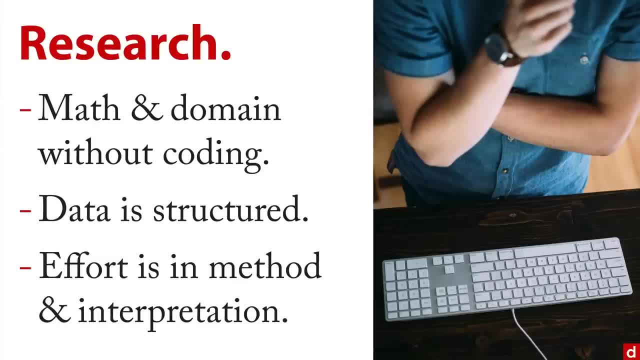 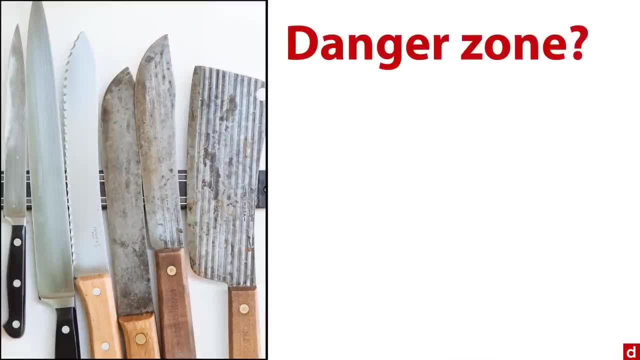 So still very heavy intellectual, cognitive work, but it comes in a different place. Finally, there's what Conway called the danger zone, And that's the intersection of coding and domain knowledge, but without math or statistics. Now he says it's unlikely to happen, and that's probably true. 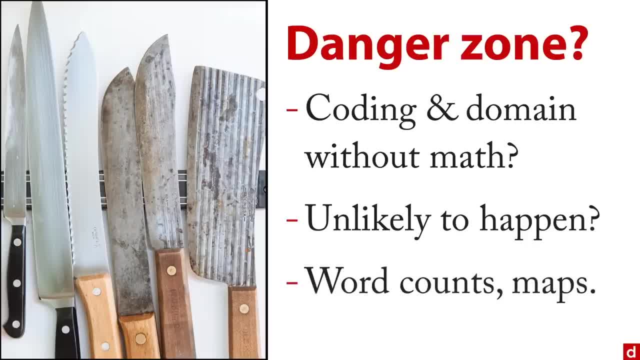 On the other hand, I can think of some common examples, what are called word counts, where you take a large document or a series of documents and you count how often each word appears in there. That can actually tell you some important things, And also drawing maps and showing how things change across place and maybe across time. 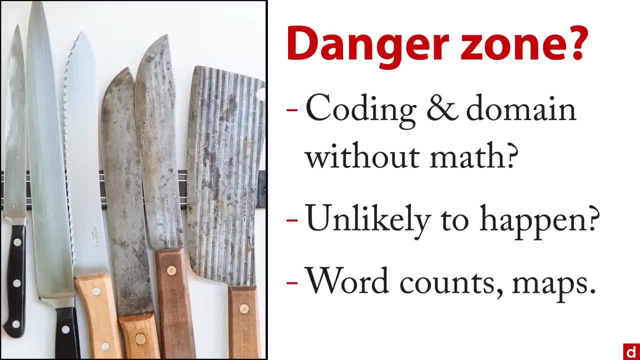 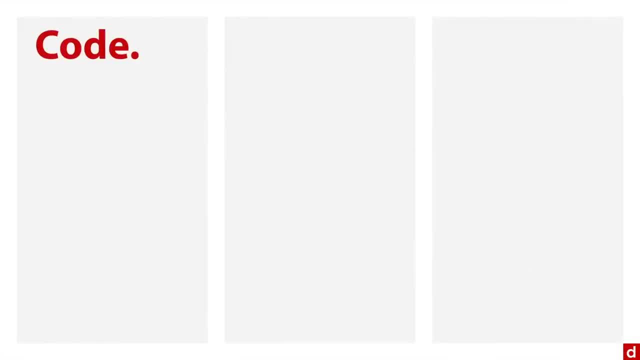 You don't necessarily have to have the math- You can do that- But it can be very insightful and helpful. So let's think about a couple of backgrounds where people come from here. First is coding. You can have people who are coders, who can do math, stats and business. 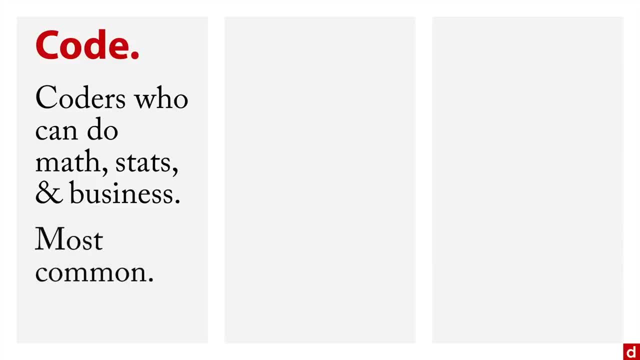 So you get the three things, and this is probably the most common. Most of the people come from a programming background. On the other hand, there's also stats or statistics, And you can get statisticians who can code and who also can do business. 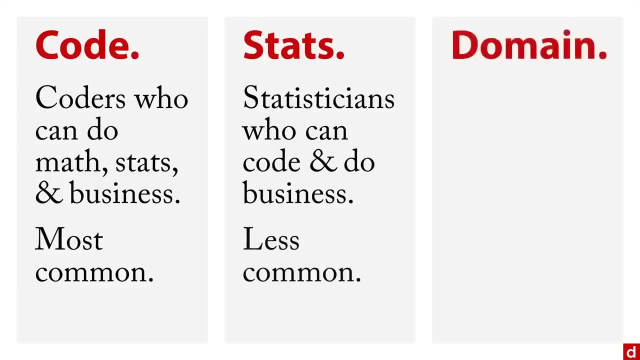 That's less common, But it does happen. And finally, there's people who come into data science from a particular domain. These are, for instance, business people who can code and do numbers, And they're the least common, But all of these are important to data science. 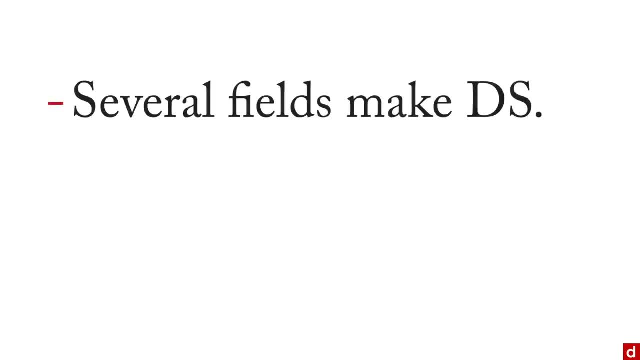 And so, in sum, here's what we can take away. First, several fields make up data science. Second, diverse skills and backgrounds are important and they're needed in data science. And third, there are many roles involved, Because there's a lot of different things that need to happen. 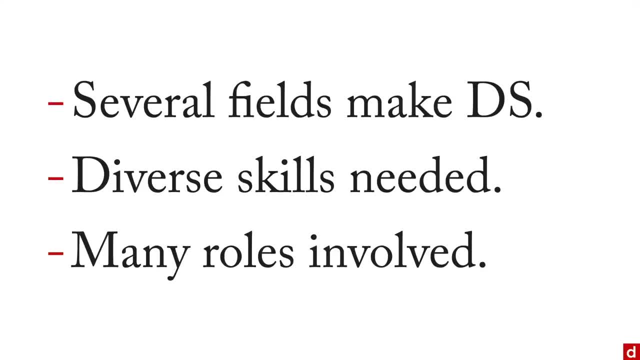 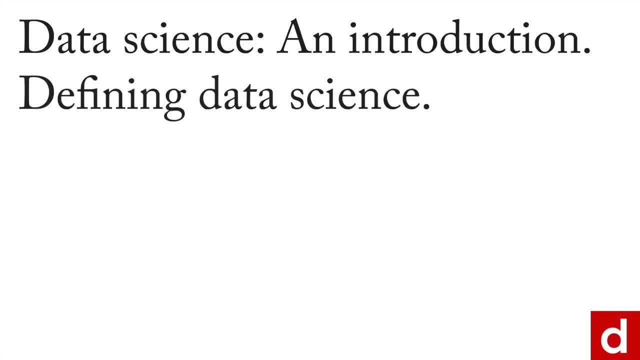 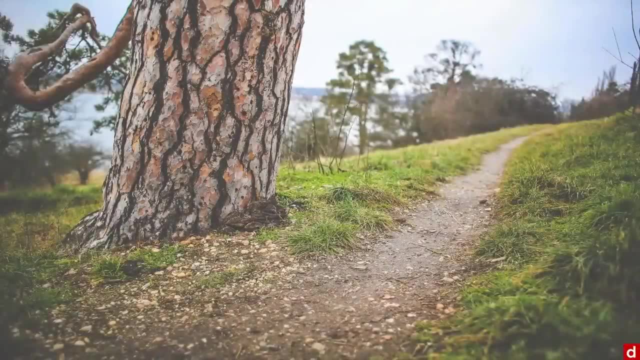 We'll say more about that in our next movie. The next step in our data science introduction and our definition of data science is to talk about the data science pathway. So I like to think of this as when you're working on a major project you got to do. 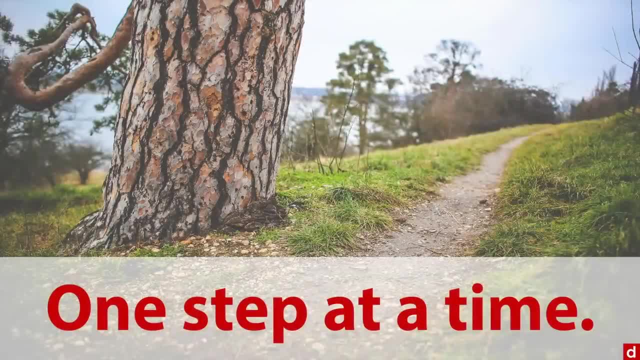 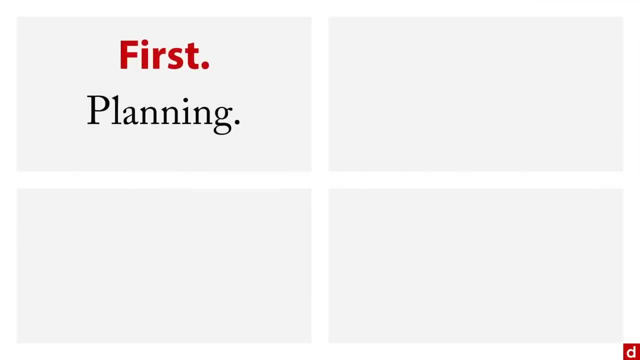 one step at a time to get from here to there. In data science you can take the various steps. you can put them into a couple of general categories. First, there are the steps that involve planning. second, there's the data prep. third, there's 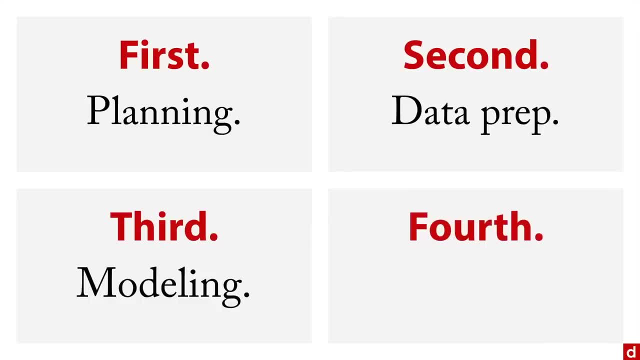 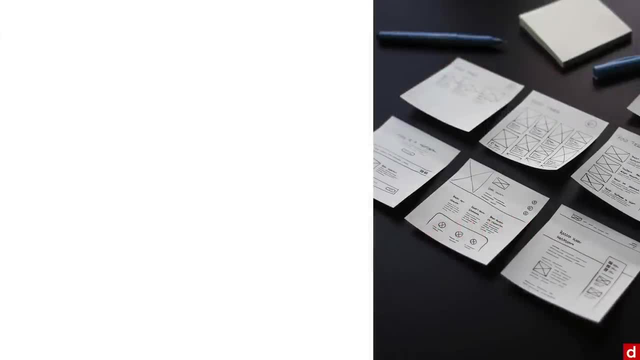 the actual modeling of the data. and fourth, there's the follow up, And there are several steps within each of these. I'll explain each of them briefly. First, let's talk about planning. The first thing you need to do is you need to define the goals of your project, so you 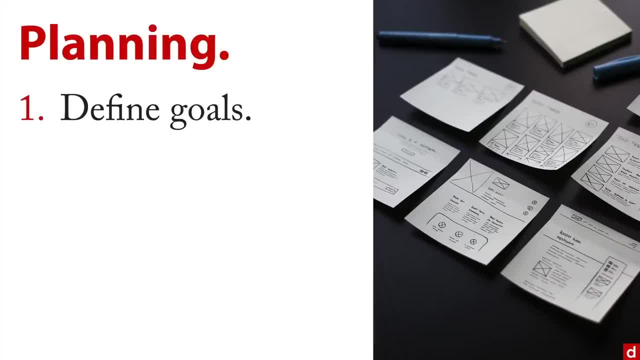 know how to use your resources well and also so you know when you're done. Second, you need to organize your resources So you might have data from several different sources. You might have different software packages, You might have different people, which gets us to the third one. 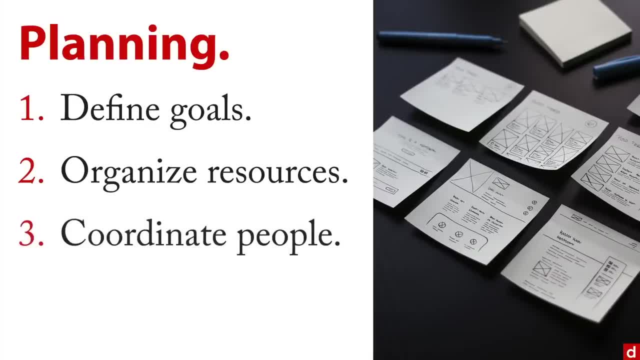 You need to coordinate the people so they can work together productively. If you're doing a handoff, it needs to be clear who's going to do what and how their work is going to go together. And then, really to state the obvious, you need to schedule the project so things can. 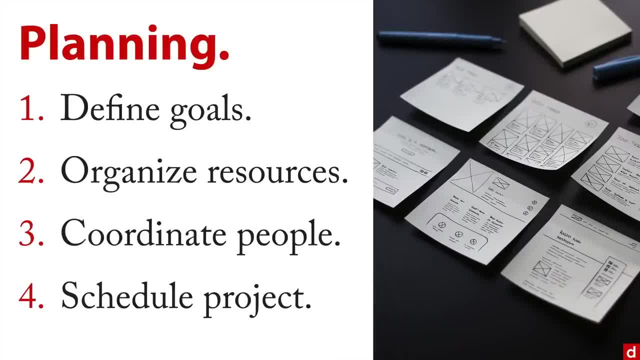 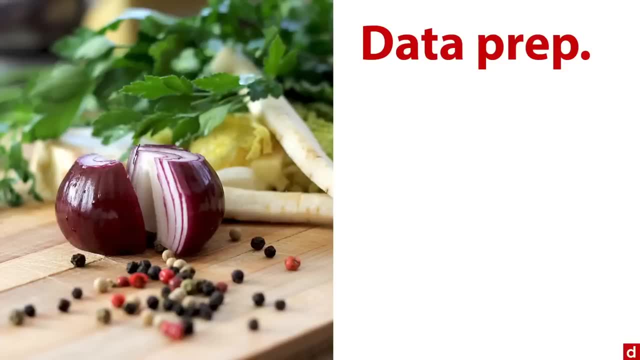 move along smoothly and you can finish in a reasonable amount of time. Next is the data prep You're taking, like food prep and getting the raw ingredients ready. First, of course, is you need to get the data, and it can come from many different sources. 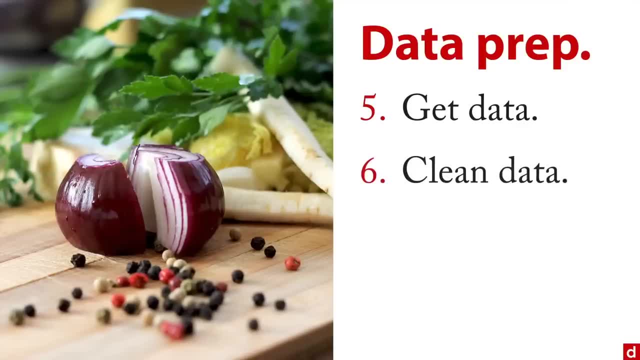 and be in many different formats. You need to clean the data And the sad thing is this tends to be a very large part of any data science project, And that's because you're bringing in unusual data from a lot of different places. You also want to explore the data, that is, really see what it looks like, how many people 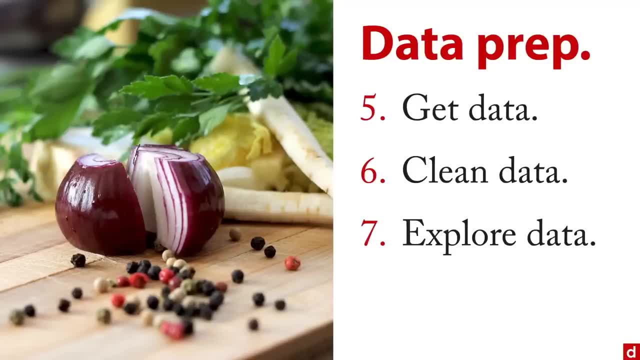 are in each group, what the shape of the distributions are like, what's associated with what, And you may need to refine the data, and that means choosing variables to include, choosing cases to include or exclude, making any transformations to the data you need to do. 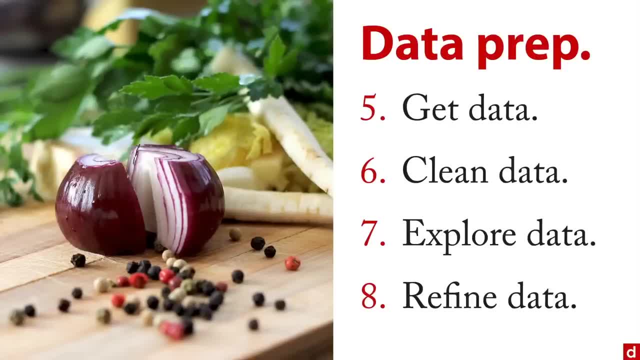 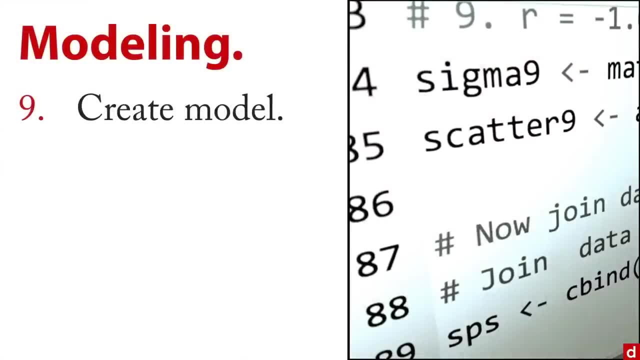 And of course these steps kind of can bounce back and forth from one to the other. The third group is modeling, or statistical modeling. This is where you actually want to create the statistical model. So, for instance, you might do a regression analysis. 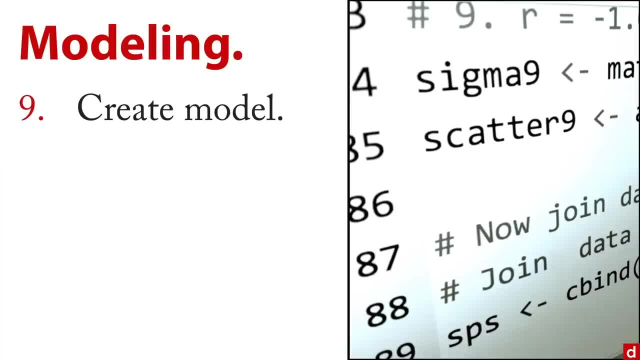 Or you might do a neural network. But whatever you do, once you create your model, you have to validate the model. You might do that with holdout validation. You might do it really with a very small replication, if you can. You also need to evaluate the model. 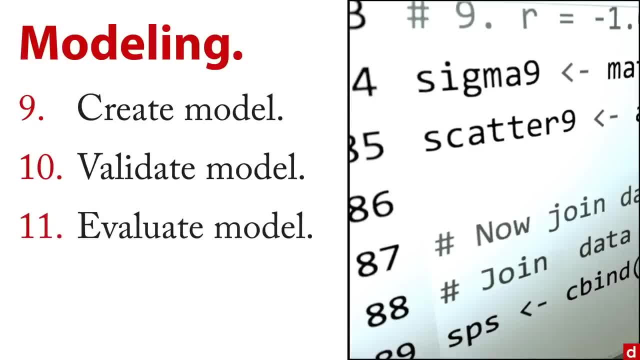 So, once you know that the model is accurate, what does it actually mean and how much does it tell you? And then, finally, you need to refine the model. So, for instance, there may be variables You want to throw out, there may be additional ones you want to include. 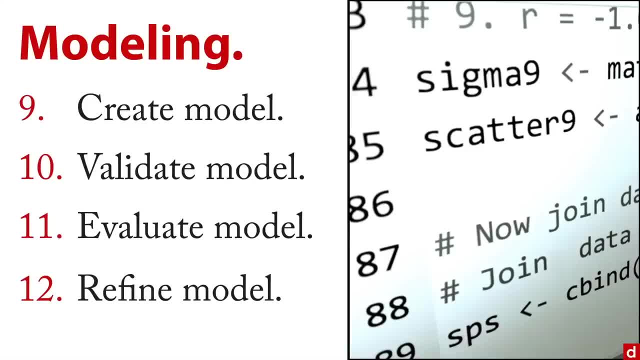 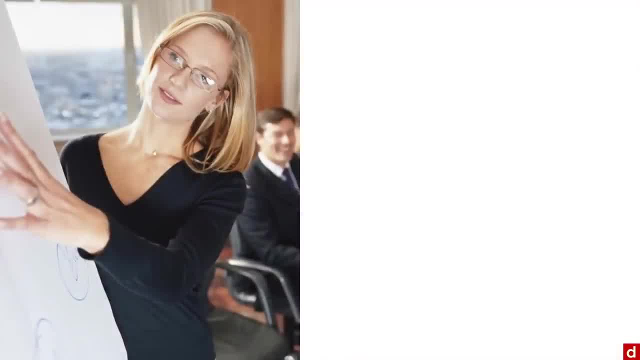 You may want to again transform some of the data. You may want to get it so it's easier to interpret and apply. And that gets us to the last part of the data science pathway And that's follow up. And once you've created your model, you need to present the model, because it's usually 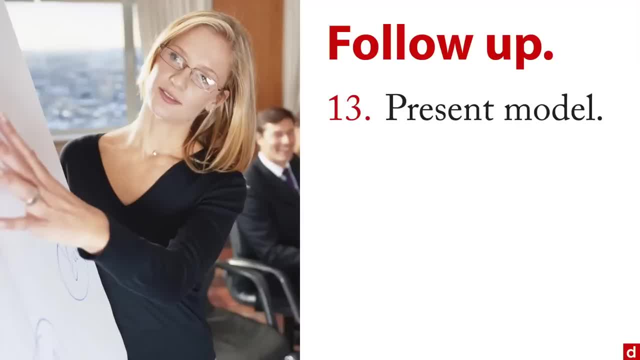 work that's being done for a client Could be in-house, could be a third party, but you need to take the insights that you got and share them in a meaningful way With other people. You also need to deploy the model It's usually being done in order to accomplish something. 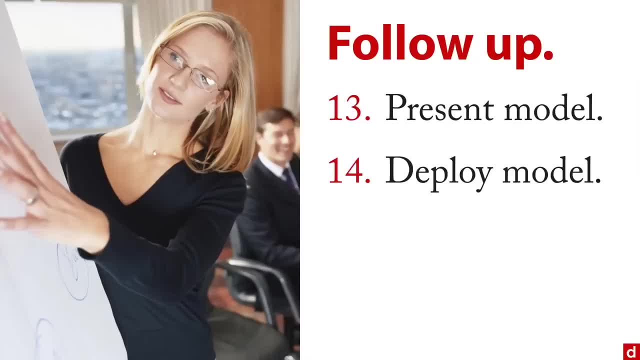 So, for instance, if you're working with an e-commerce site, you may be developing a recommendation engine that says people who bought this and this might buy this. You need to actually stick it on the website and see if it works the way you expected it. 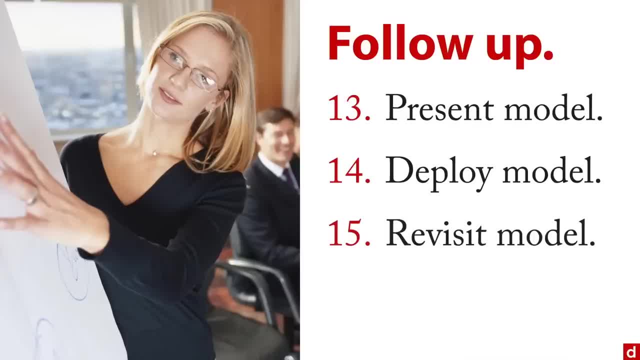 to. Then you need to revisit the model, because a lot of times, the data that you worked on is not necessarily all of the data And things can change. Okay, You get out in the real world, or things just change over time, And so you have to see how well your model is working. 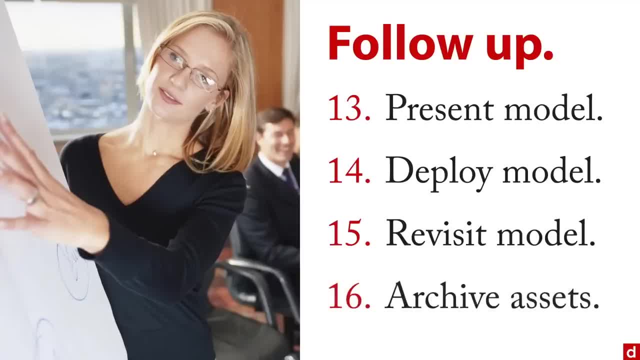 And then, just to be thorough, you need to archive the assets, document what you have, and make it possible for you or for others to repeat the analysis or develop off of it in the future. So those are the general steps of what I consider the data science pathway. 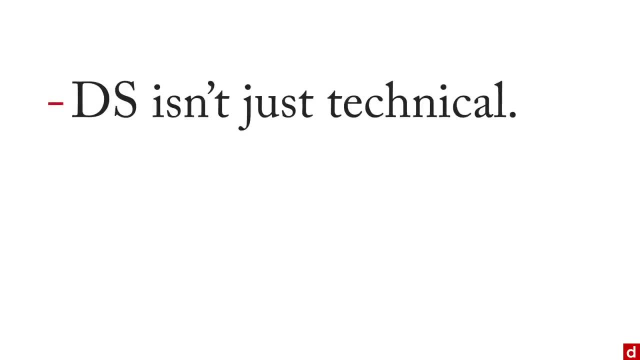 And, in sum, what we get from this is three things. First, data science isn't just a technical field. It's not just coding. Things like planning and presenting and implementing are just as important. Also, contextual skills: knowing how it works in a particular field, knowing how it will. 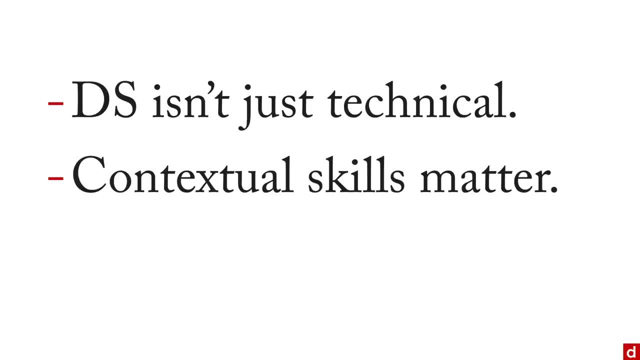 be implemented. those skills matter as well. And then, as you got from this whole thing, there's a lot of things to do, And if you go one step at a time, there'll be less backtracking and you'll ultimately be more productive in your data science projects. 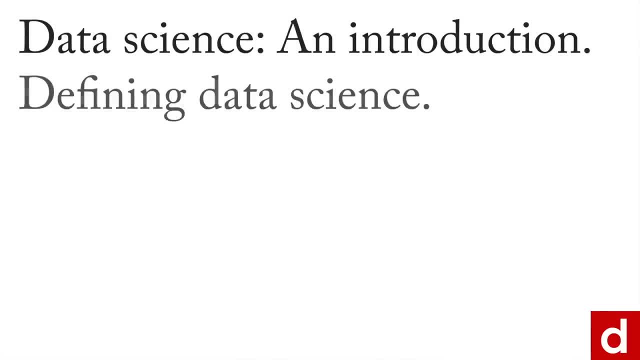 We'll continue. We'll continue our definition of data science by looking at the roles that are involved in data science, the way that different people can contribute to it. That's because it tends to be a collaborative thing and it's nice to be able to say that. 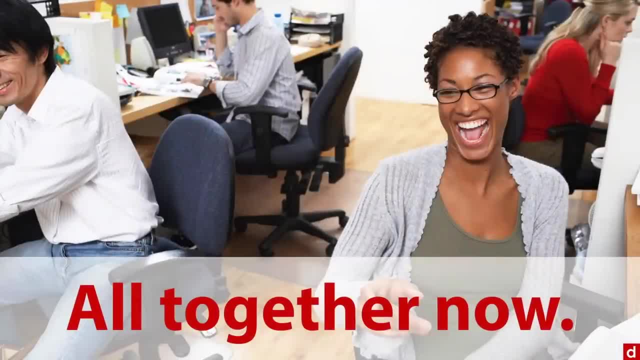 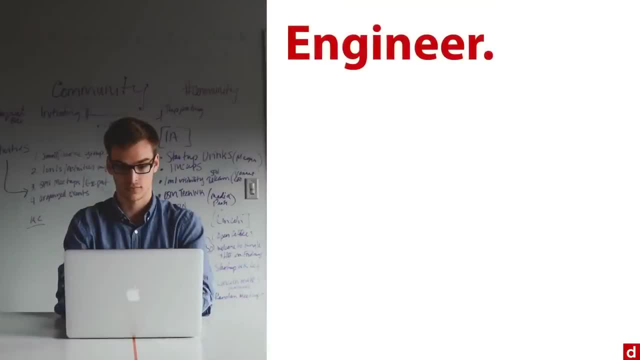 we're all together, working together towards a single goal. So let's talk about some of the roles involved in data science and how they contribute to the projects. First off, let's take a look at engineers. These are people who focus on the backend hardware, for instance, the servers and the 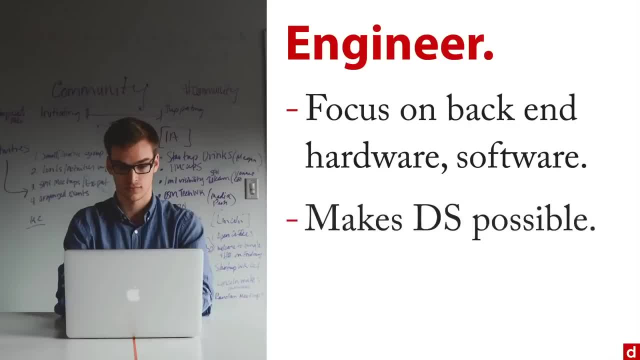 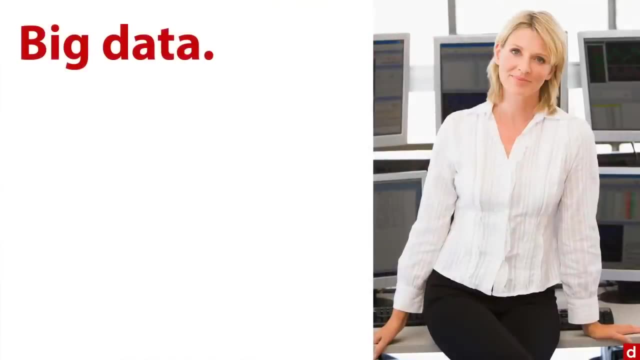 software that runs them. This is what makes data science possible, And it includes people like developers, software developers or database administrators, and they provide the foundation for the rest of the work. Next, you can also have people who are big data specialists. 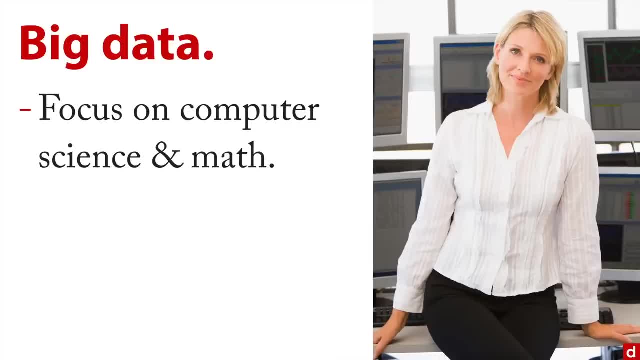 These are people who focus on computer science and mathematics, and they may do machine learning algorithms as a way of processing very large amounts of data, and they often create what are called data products, So a thing that tells you what restaurant to go to or that says you might know these. 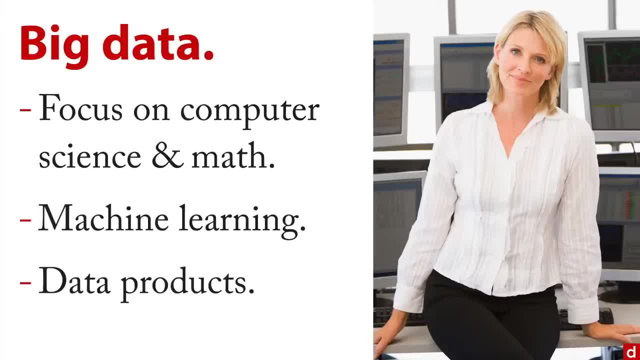 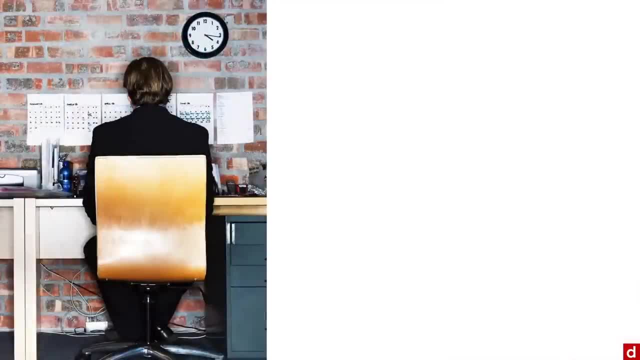 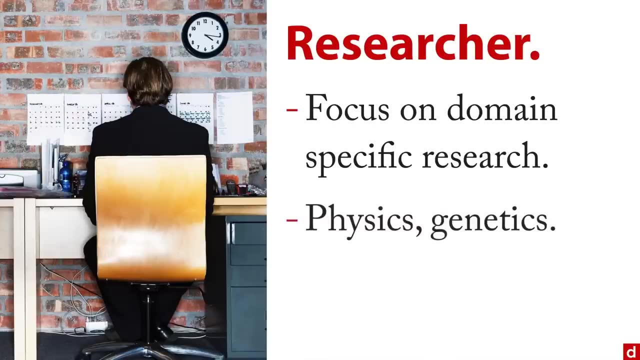 friends or provides ways of linking up photos. Those are data products and those often involve a huge amount of very technical work. behind them There are also researchers. These are people who focus on domain specific research, So, for instance, physics or genetics or whatever, and these people tend to have very strong 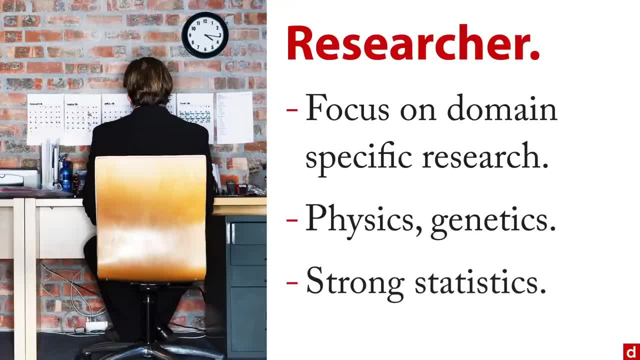 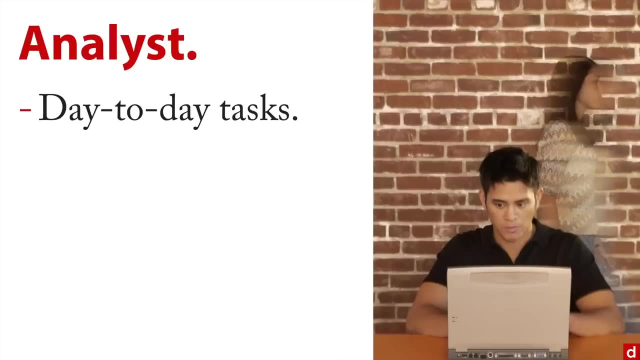 statistics And they can use some of the procedures and some of the data that comes from the other people, like the big data researchers, but they focus on these specific questions. Also, in the data science realm you'll find analysts. These are people who focus on the day to day tasks of running a business. 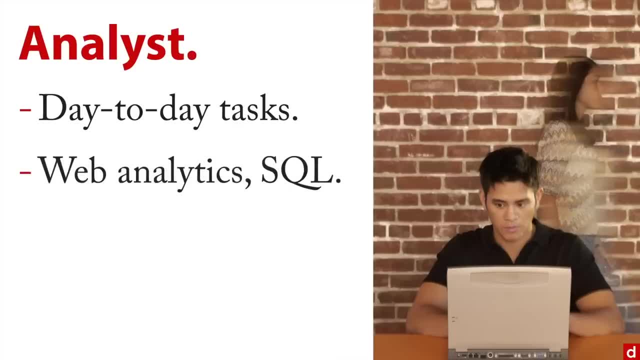 So, for instance, they might do web analytics like Google Analytics, or they might pull data from a SQL database, And this information is very important and good for business. And so analysts are key to the day to day functioning of business. But you know, they may not exactly be data science proper, because most of the data they're 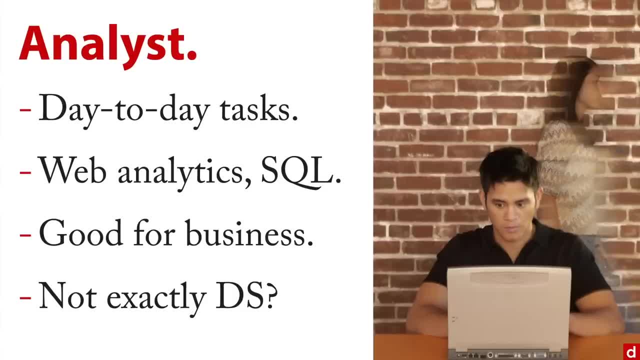 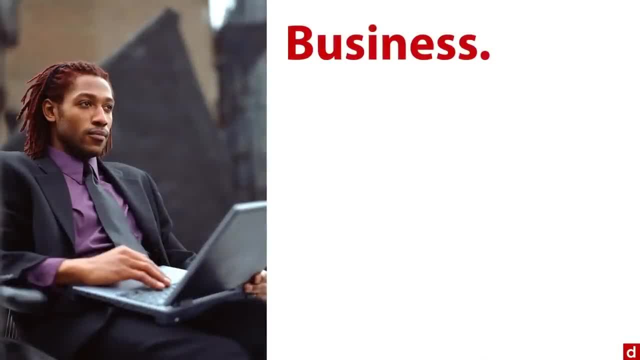 they're working with is going to be pretty structured. Nevertheless, they play a critical role in business in general. And then, speaking of business, you have the actual business people, the men and women who organize and run businesses. These people need to be able to frame business relevant questions that can be answered with 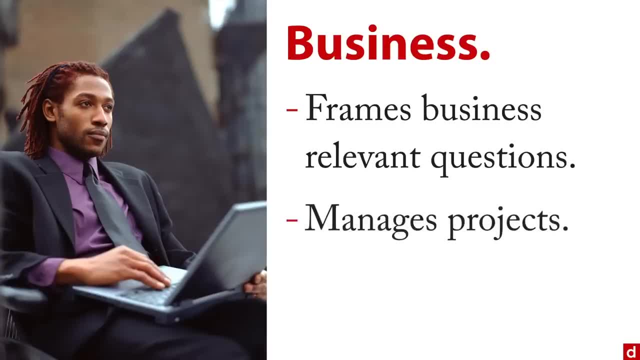 the data. Also, the business person manages the project and the efforts and the resources of others And, while they may not actually be doing the coding, they must speak data. they must know how the data works, what it can answer and how to implement it. 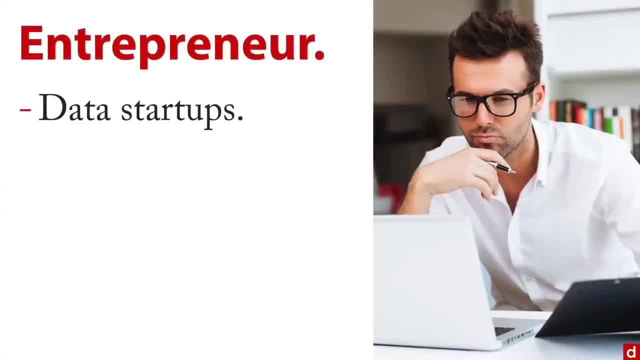 You can also have entrepreneurs, So you might have, for instance, a data startup. they're starting their own little social network or their own little web search platform. An entrepreneur That needs data and business skills And, truthfully, they have to be creative at every step along the way, usually because 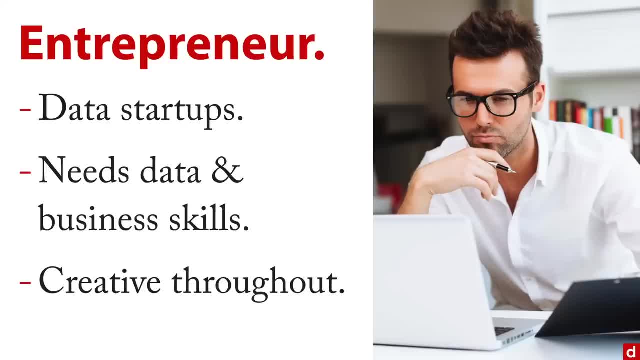 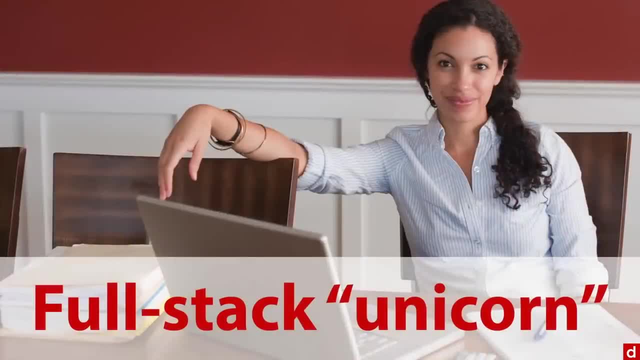 they're doing it all themselves at a smaller scale. Then we have, in data science, something known as the full stack unicorn, And this is a person who can do everything at an expert level, And they're called a unicorn because, truthfully, they may not actually exist. 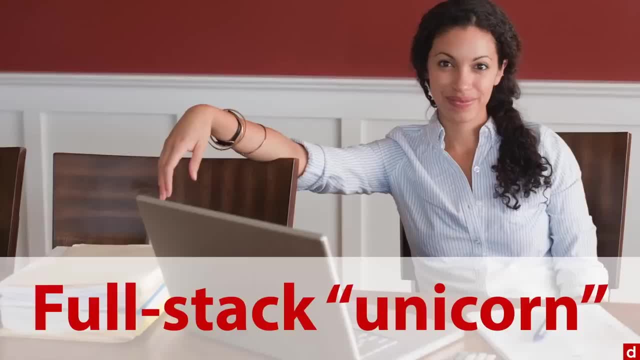 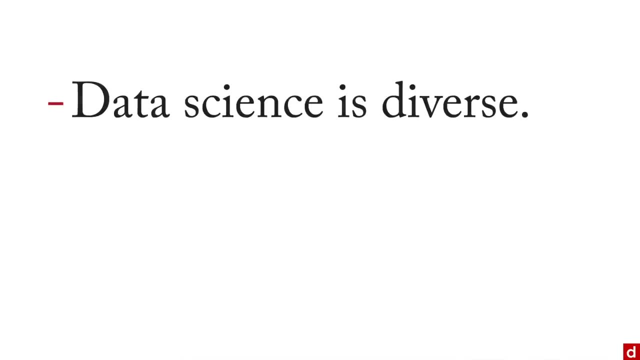 I'll have more to say about that later, But for right now we can sum up what we got out of this video By three things. Number one: data science is diverse. There's a lot of different people who go into it. 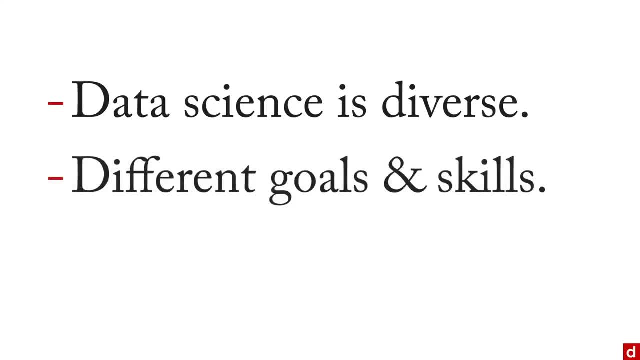 And they have different goals for their work And they bring in different skills and different experiences and different approaches. Also, they tend to work in very different contexts: An entrepreneur works in a very different place from a business manager works in a very different place from an academic researcher. 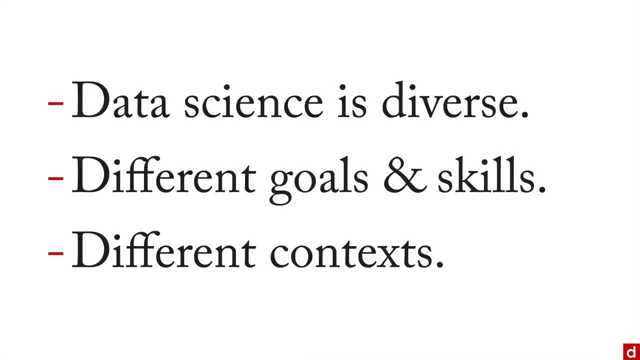 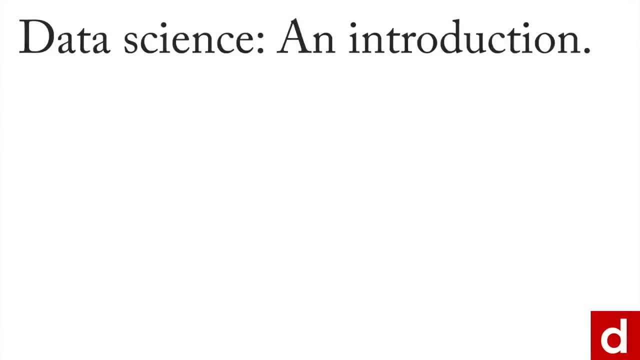 But all of them are connected in some way to data science and make it a richer field. The last thing I want to say in data science and introduction, where I'm trying to define data science, is to talk about teams in data science. The idea here is that data science has many different tools and different people are going 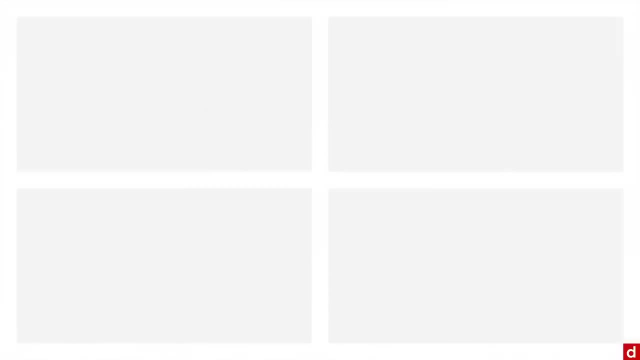 to be experts in each one of them. Now you have, for instance, coding, and you have statistics. Also, you have fields like design or business and management that are involved, And the question, of course, is: okay, Who can do all of it? 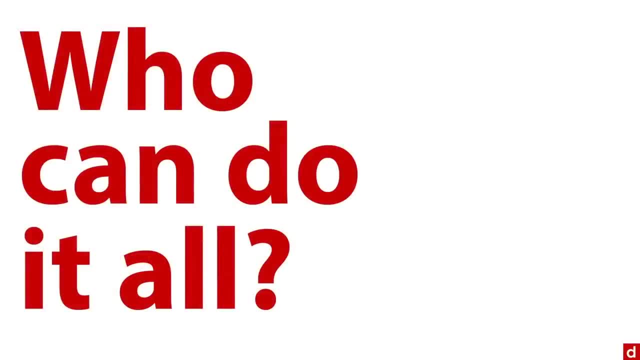 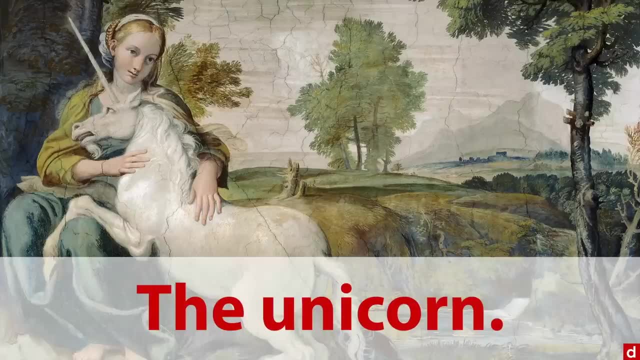 Who's able to do all of these things at the level that we need? Well, that's where we get this saying- I've mentioned it before: It's the unicorn, And, just like in ancient history, the unicorn is a mythical creature with magical abilities. 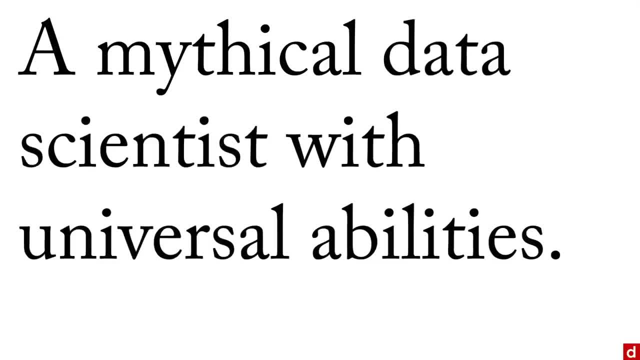 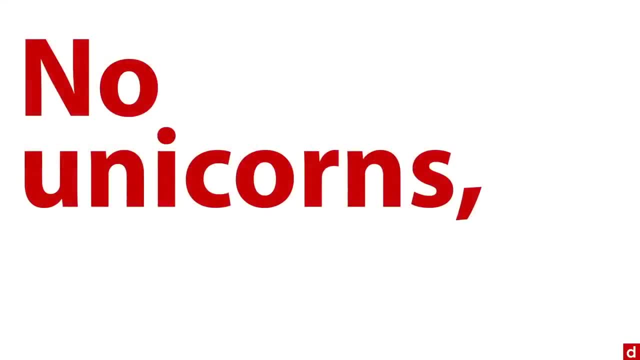 In data science it works a little differently. It is a mythical data scientist with universal abilities. The trouble is, as we know from the real world, there's really no unicorns- animals- And there's no unicorns, And there's really not many unicorns in data science. 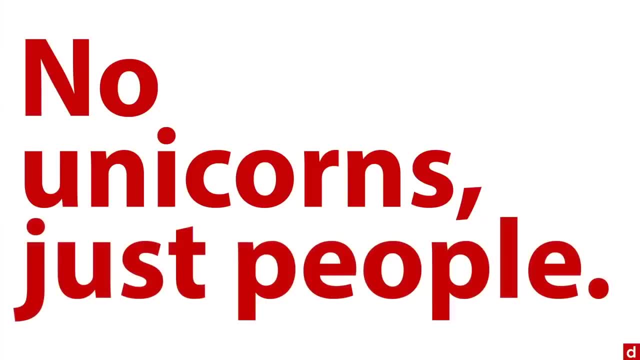 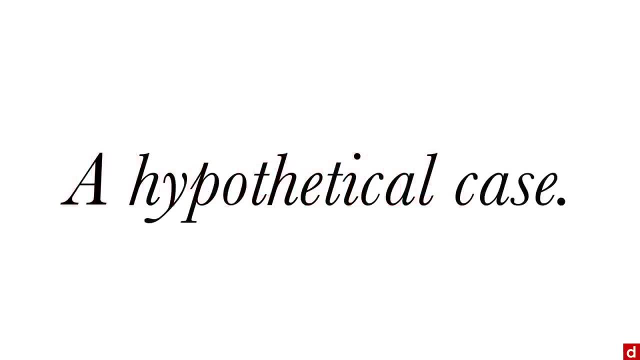 Really, there's just people, And so we have to find out how we can do the projects even though we don't have this one person who can do everything for everybody. So let's take a hypothetical case just for a moment. I'm going to give you some fictional people. 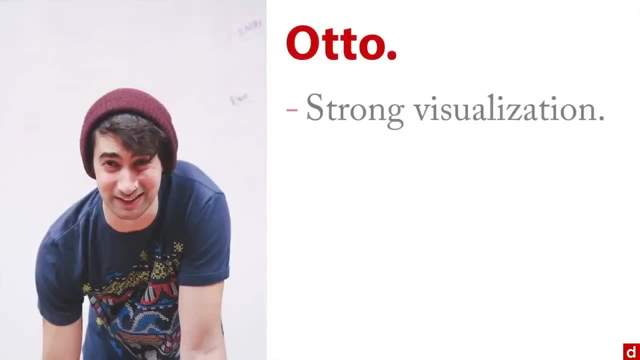 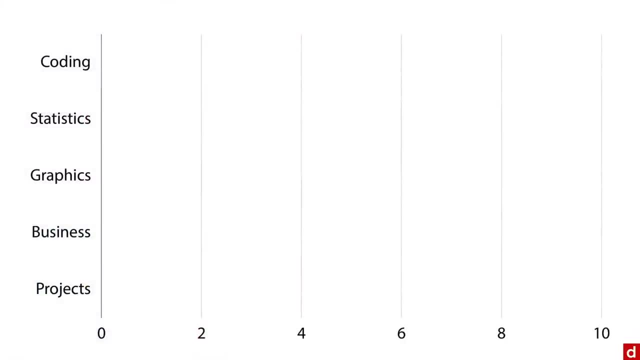 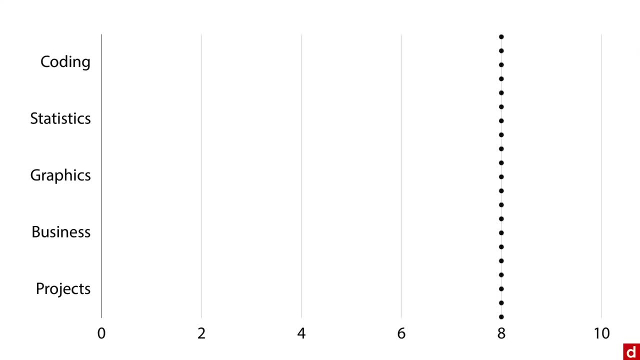 There's something about his abilities. So here we got five things that we need to have happen, And for the project to work, they all have to happen at at least a level of 8 on the 0 to 10.. If we take his coding ability, he's almost there. 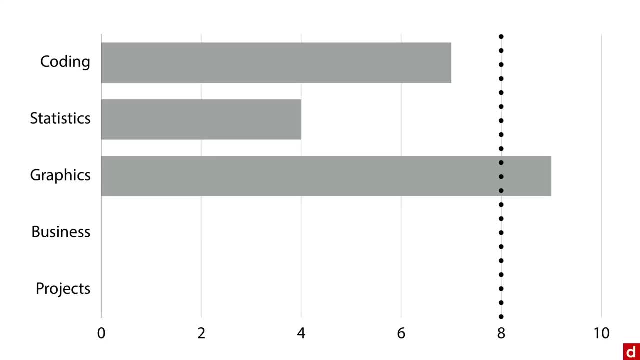 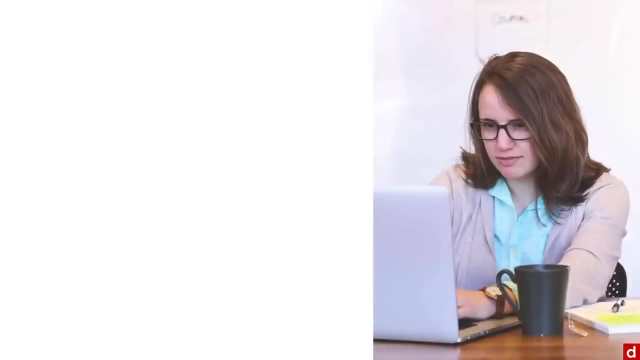 Statistics, not quite halfway Graphics. yes, He can do that, And then business All right And project Pretty good. So what you can see here is: in only one of these five areas is Otto sufficient on his own. On the other hand, let's pair them up with somebody else. Let's take a look at Lucy. 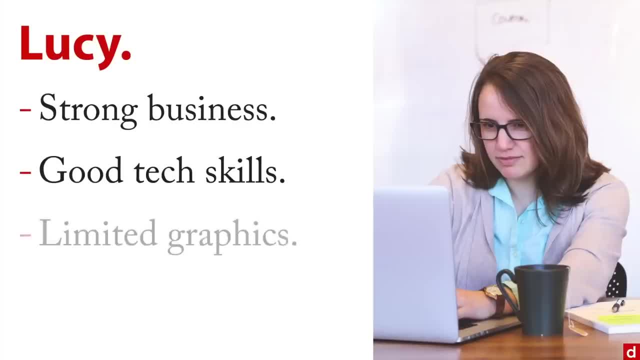 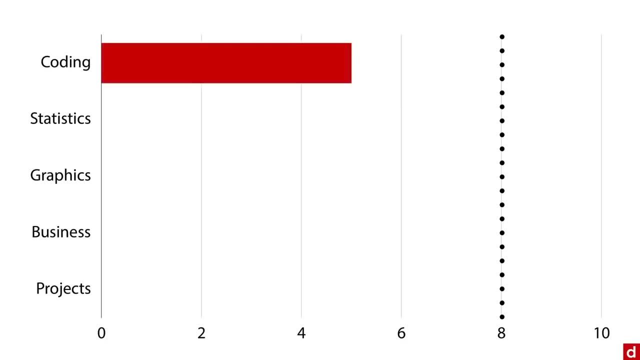 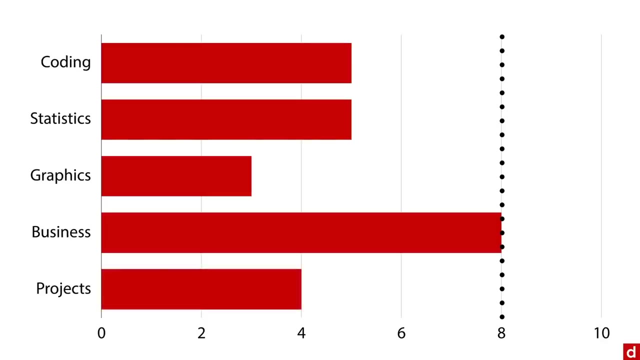 And Lucy has strong business training, has good tech skills, but has limited graphics, And so if we get her profile on the same thing that we saw, there's coding, pretty good statistics, pretty good graphics, not so much business. good and projects okay. Now the important thing here is: 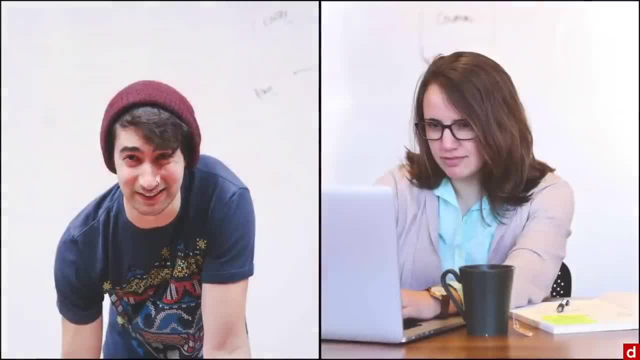 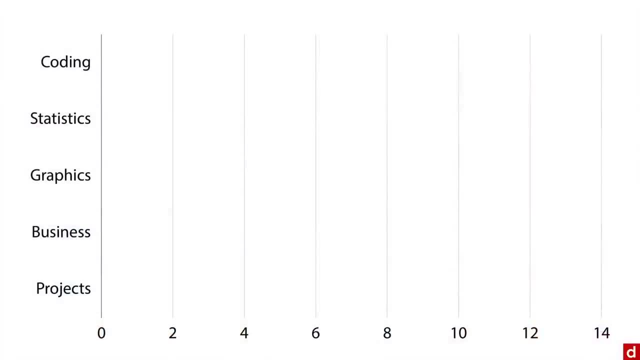 that we can make a team. So let's take our two fictional people, Otto and Lucy, and we can put together their abilities. Now actually have to change the scale here a little bit to accommodate the both of them, But our criterion still is at eight. we need a level of eight in order to do. 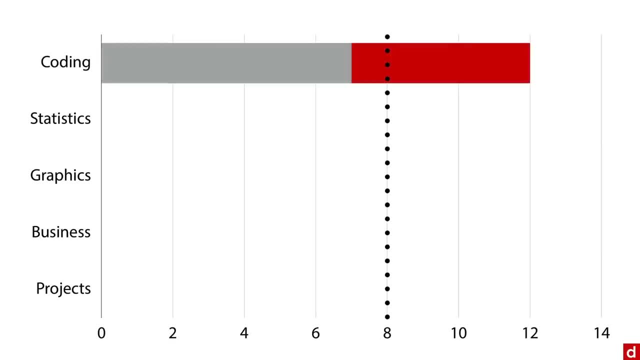 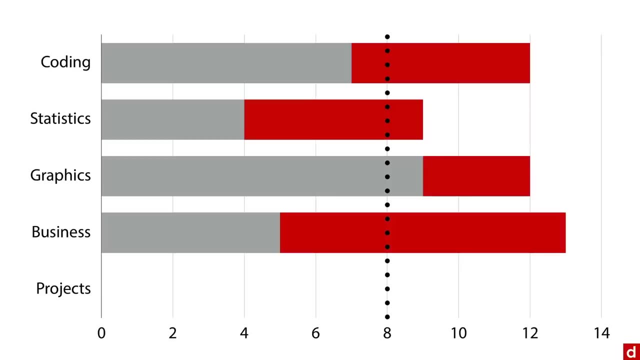 the project competently And we combine them. Oh look, coding is now past eight, Statistics is past eight, graphics is way past, business way past, And then the projects there too, And so when we combine their skills, we are able to get the level that we need for. 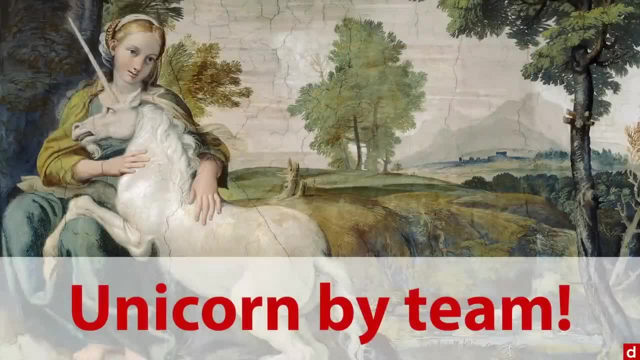 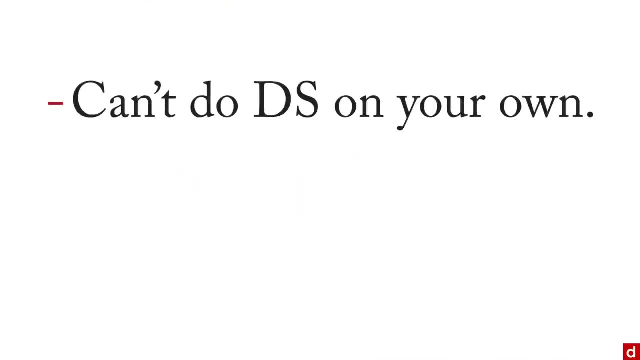 everything. Or to put it another way, we have now created a unicorn by team And that makes it possible to do the data science project. So in some you usually can't do data science on your own. That's a very rare individual. Or, more specifically, people need people And in data, 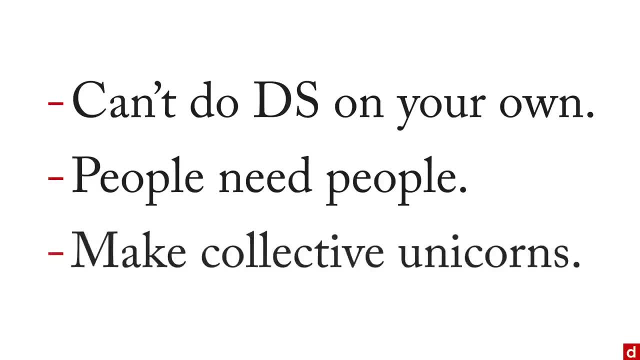 science, you have the opportunity to take several people and do the project, And so when we combine data science on your own, that's a very rare individual Or, more specifically, people need people and make collective unicorns, So you can get the insight that you need in your project. 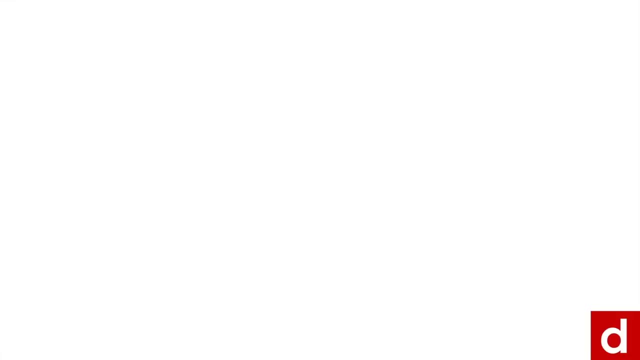 and you can get the things done that you want. In order to get a better understanding of data science, it can be helpful to look at contrasts between data science and other fields. Probably the most informative is with big data, Because these two terms are actually often confused. It. 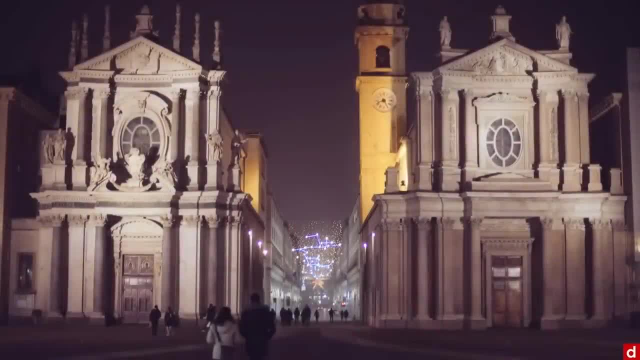 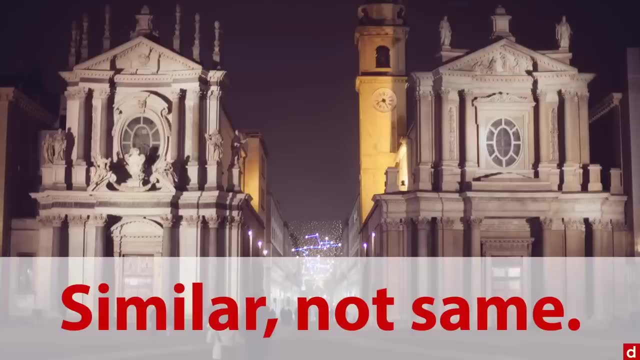 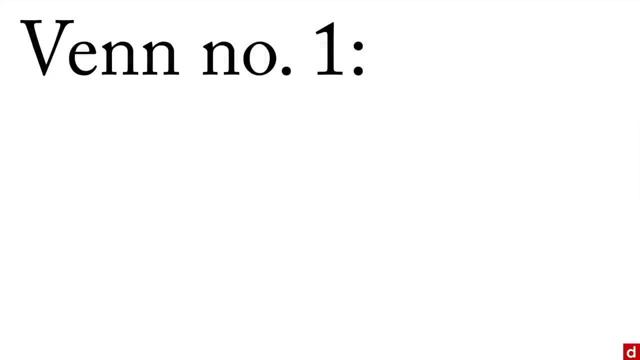 makes me think of situations where you have two things that are very similar but not the same, like we have here in the Piazza. Part of the problem stems from the fact that data science and big data both have Venn diagrams associated with them. So, for instance, Venn number one for data science is something we've seen. 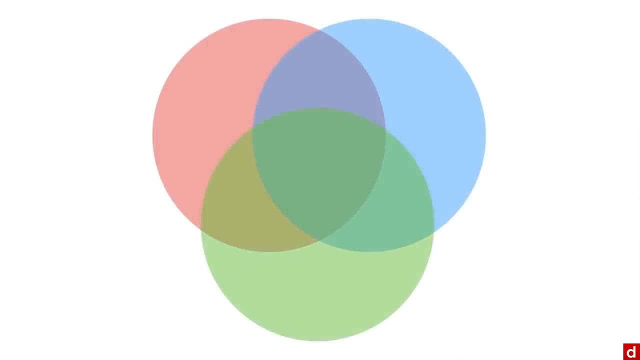 already. we have three circles And we have coding and we have math and we have some domain expertise that put together get data science. On the other hand, Venn diagram number two is for big data. It also has a Venn diagram for data science. So we have three circles And we have coding and we have 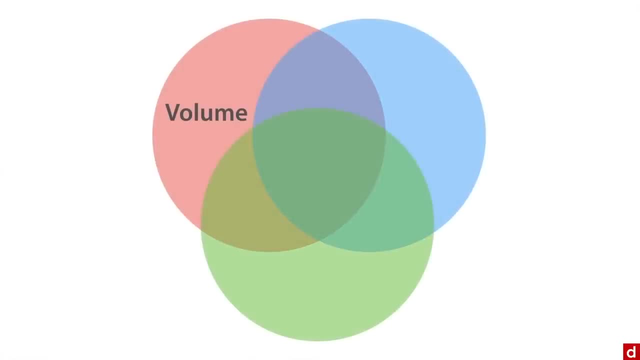 math and we also have three circles And we have the high volume of data, the rapid velocity of data and the extreme variety of data. Take those three V's together, you get big data. Now we can also combine these two, if we want, in a third Venn diagram. we call big data and data. 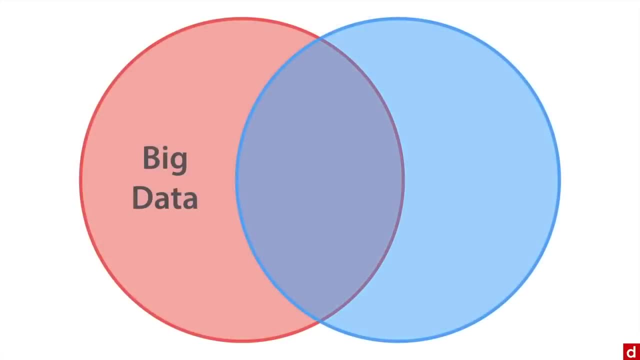 science. This time is just two circles, with big data on the left and data science on the right, And the intersection there in the middle is big data science, which actually is a real term, And the intersection there in the middle is also a real term And if you want to do a compare and 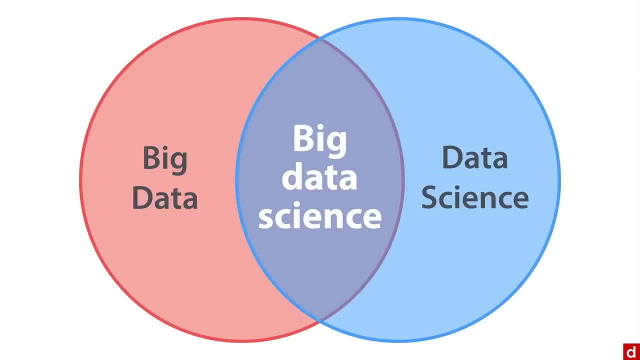 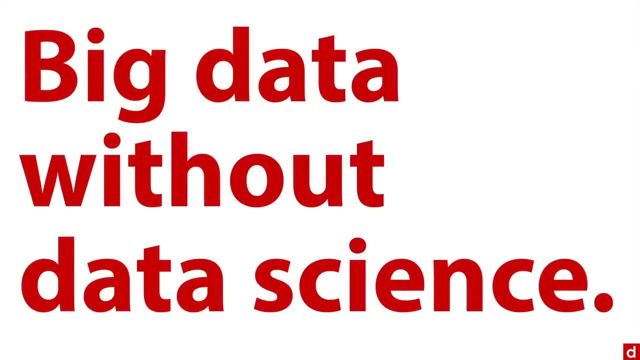 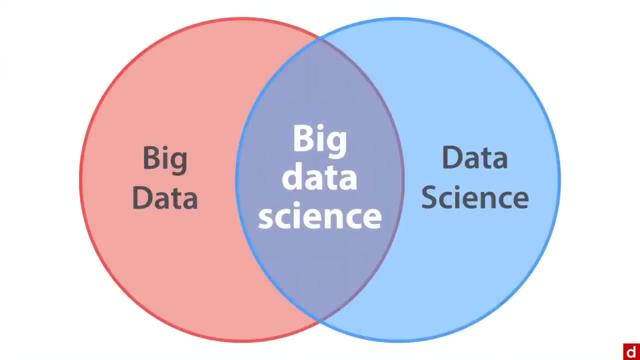 contrast. it kind of helps to look at how you can have one without the other. So let's start by looking at big data without data science. So these are situations where you may have the volume or velocity variety data but don't need all the tools of data science, So we're just looking at. 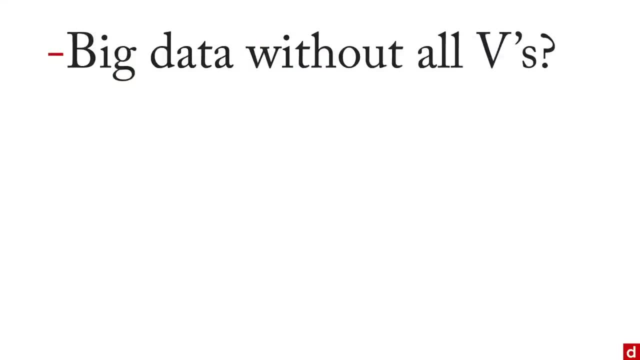 the left side of the equation right now. Now, truthfully, this only works if you have big data without all three V's. Some say you have to have the volume of data without all three V's, And some say you have to have the volume, velocity and variety for to count as big data. I basically 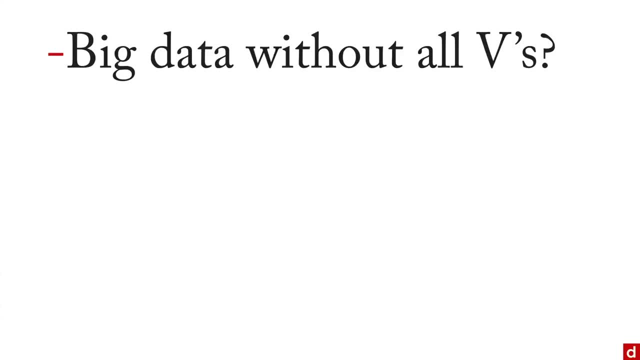 say, anything that doesn't fit into a standard machine is probably big data. I can think of a couple of examples here of things that might count as big data but maybe don't count as data science. Machine learning, where you can have very large data sets and probably very complex, doesn't. 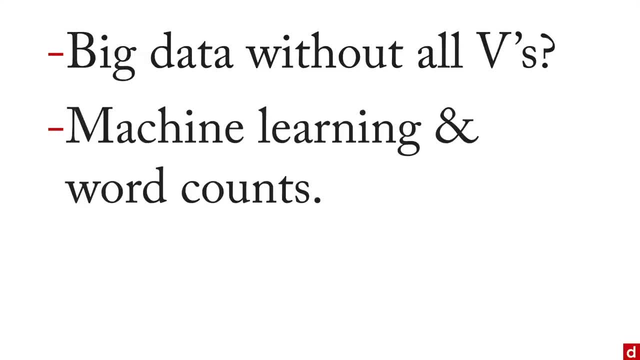 require much domain expertise. So that may not be data science word counts, where you have an enormous amount of data science, but it doesn't require much domain expertise. So that may not be data science word counts, where you have an enormous amount of data science, but it doesn't. 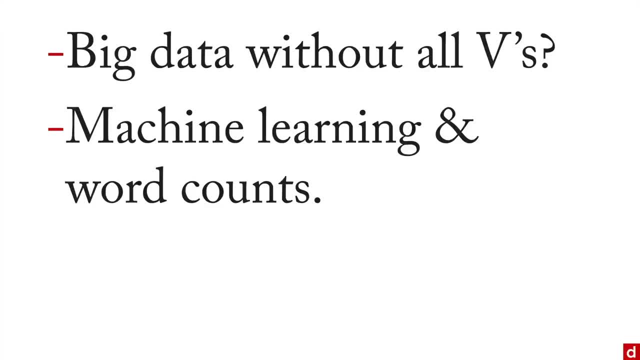 require much domain in terms of quantitative skills or even domain expertise, And it's actually a pretty simple analysis again- doesn't require much sophistication in terms of quantitative skills or even domain expertise. So, maybe, maybe not. data science, On the other hand, 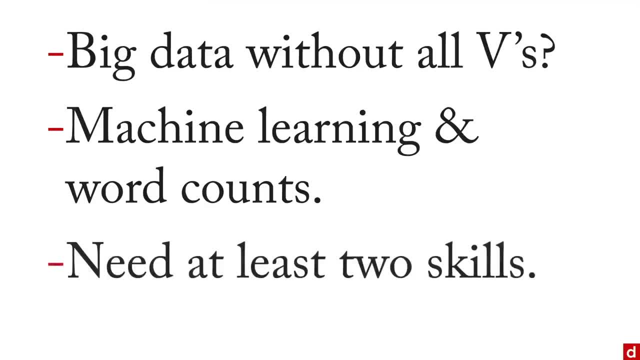 to do any of these, you're going to need to have at least two skills. you're going to need to have the coding, and you will probably have to have some sort of quantitative skills as well. So how about data science without big data? 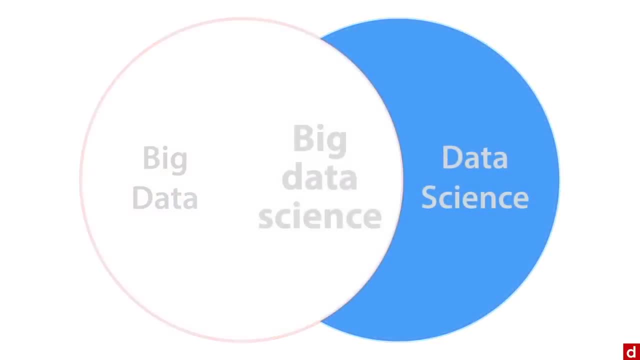 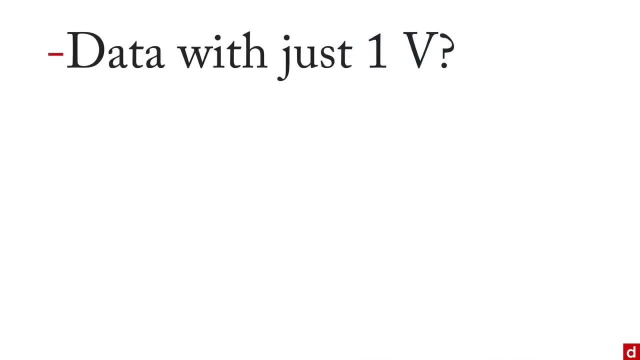 data. That's the right side of this diagram. Well, to make that happen, you're probably talking about data with just one of the three V's from big data, So either volume or velocity or variety, but singly, So, for instance, genetics data. you have a huge amount of data And 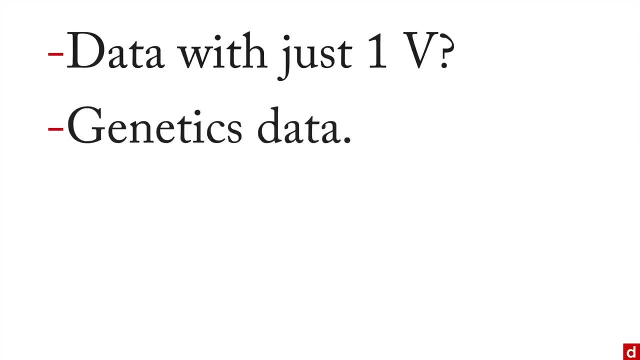 it comes in a very set structure and it tends to come in at once, So you got a lot of volume And it's a very challenging thing to work with. you have to use data science, but it may or may not count as big data. Similarly, streaming sensor data, where you have data. 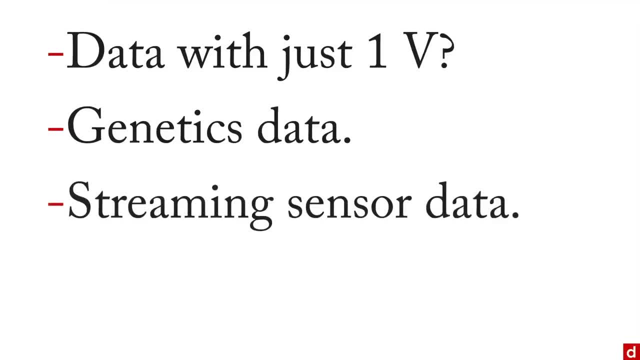 coming in very quickly, but you're not necessarily saving it. you're just looking at these windows in it. That's a lot of velocity And it's difficult to deal with. it takes data science, the full skill set, but it may not require big data per se Or facial recognition, where 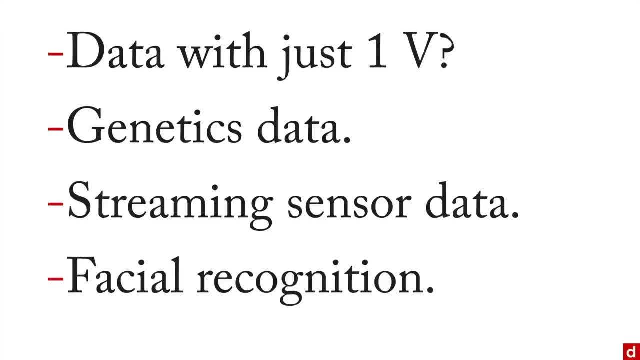 you have enormous variety in the data because you're getting full data, Photos or videos that are coming in Again. very difficult to deal with, requires a lot of ingenuity and creativity. may or may not count as big data, depending on how much of 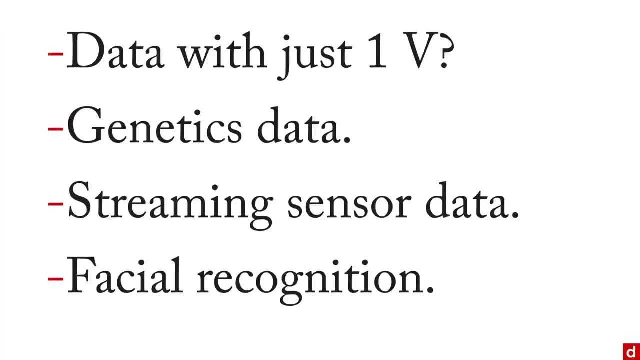 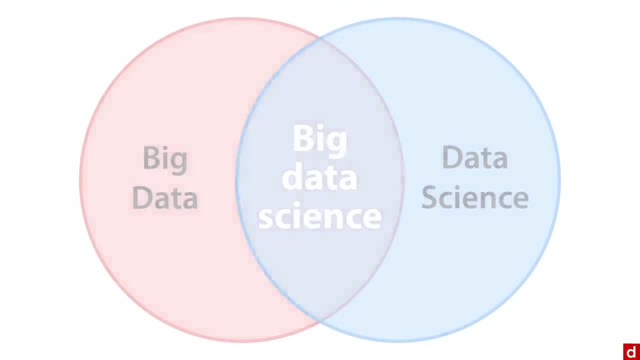 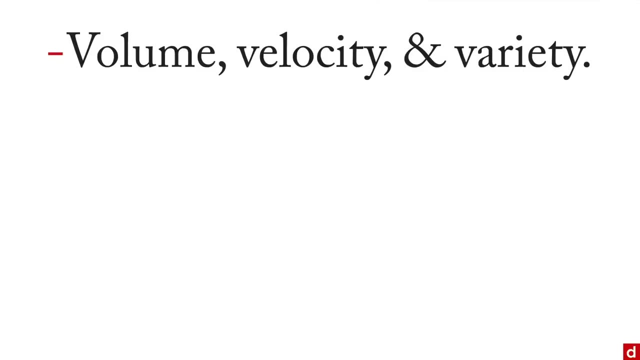 a stickler. you are about definitions. Now, if you want to combine the two, we can talk about big data science, And in that case we're looking right here at the middle. this is a situation where you have volume and velocity and variety in your data And, truthfully, 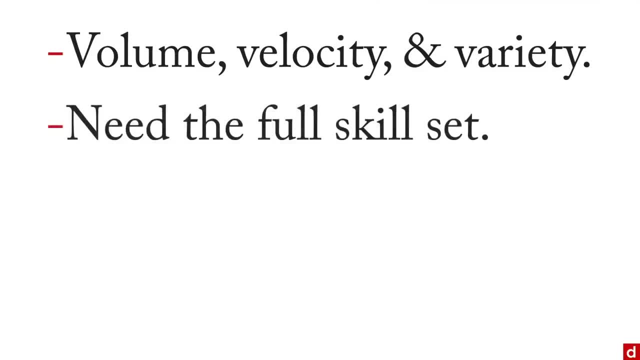 if you have the three of those, you are going to need the full data science skill set, you're going to need coding and statistics and math, and you're going to have to have domain expertise, primarily because of the variety you're dealing with. But taken all together, you do have to have all of it. So, in sum, here's what we get. 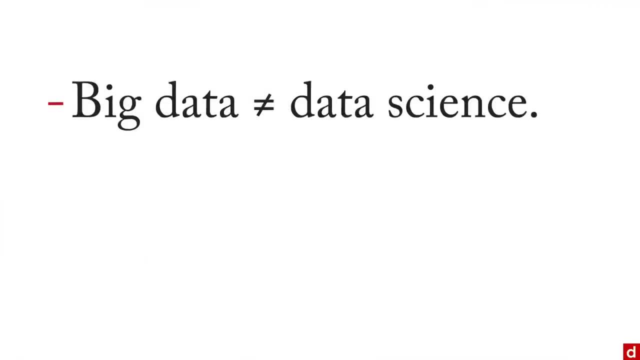 Big data is not equal to, is not identical to, data science. Now, there's common ground And a lot of people who are good at big data are good at data science, and vice versa, But they are conceptually distinct. On the other hand, there is the shared middle ground of big data science that unifies the 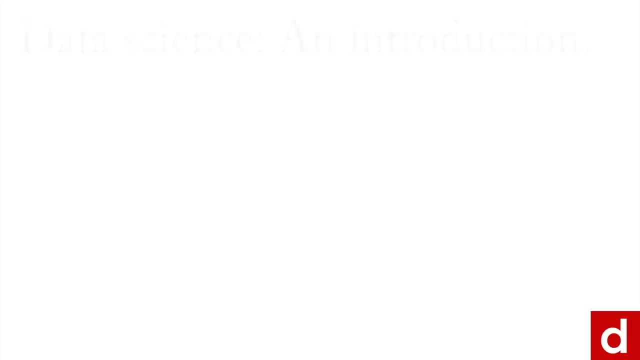 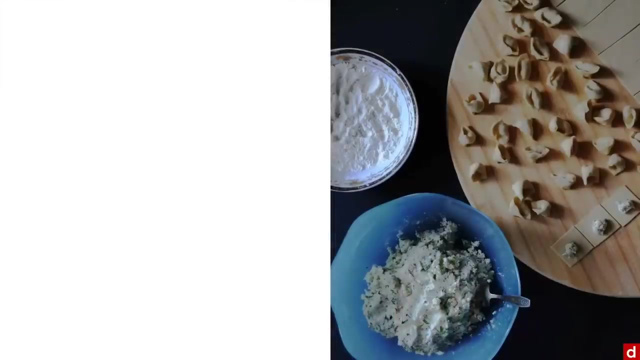 two separate fields. Another important contrast you can make in trying to understand data science is to compare it with coding or computer programming. Now, this is where you're trying to work with a machine and you're trying to talk to that machine to get it to do things In one. 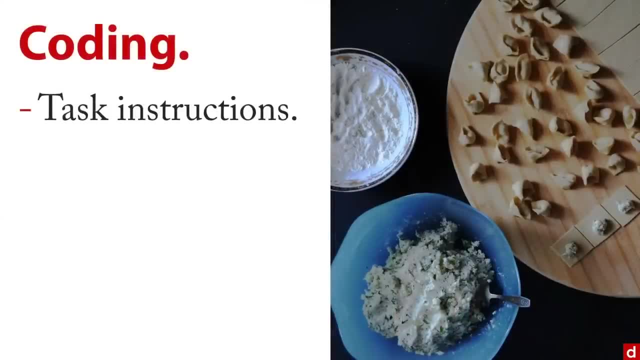 sense you can think of coding as just giving task instructions how to do something, and it's a lot like a record. But in another sense you can think of coding as just giving task instructions how to do something, and it's a lot like a record. But in another sense you can think of coding as just giving 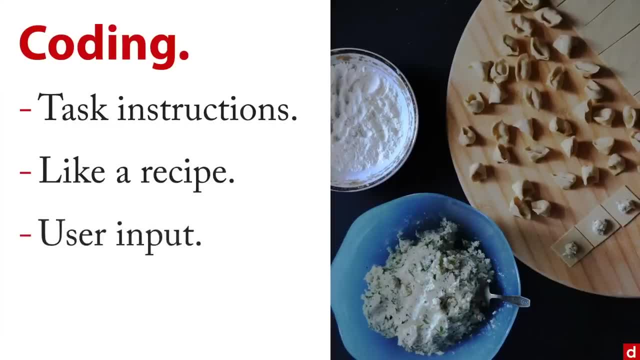 task instructions how to do something and it's a lot like a record. But in another sense you can think of coding as just giving task instructions how to do something, and it's a lot like a record. When you're cooking, you get some sort of user input or other input And then maybe you have if 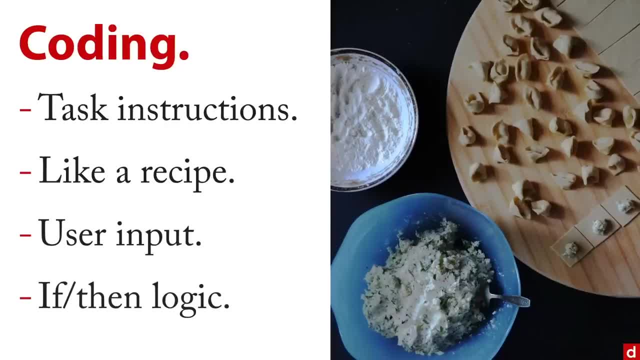 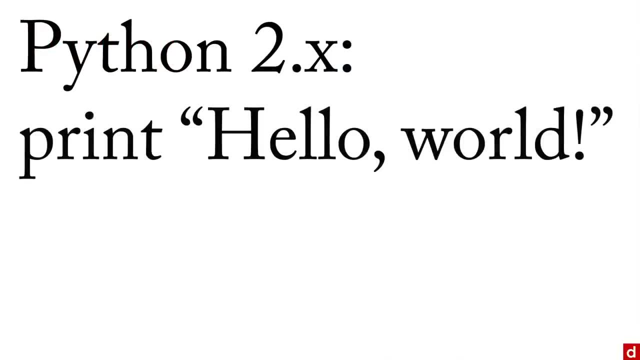 then logic and you get output from it. To take an extremely simple example, if you're programming in Python version two, you write print and then in quotes, Hello world, and that will put the words Hello world on the screen. So you gave it some instructions and it gave you some output. Very 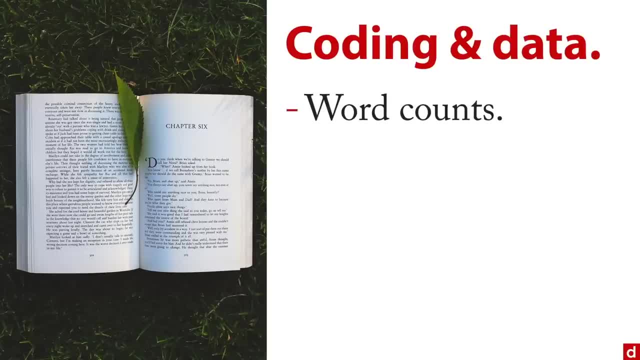 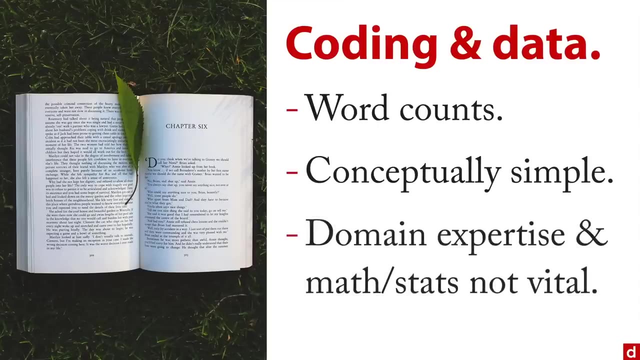 it's a little more complicated. So, for instance, there's word counts, where you take a book or a whole collection of books, You take the words and you count how many there are in there. Now this is. this is a conceptually simple task And domain expertise in really math and statistics are not vital. But to 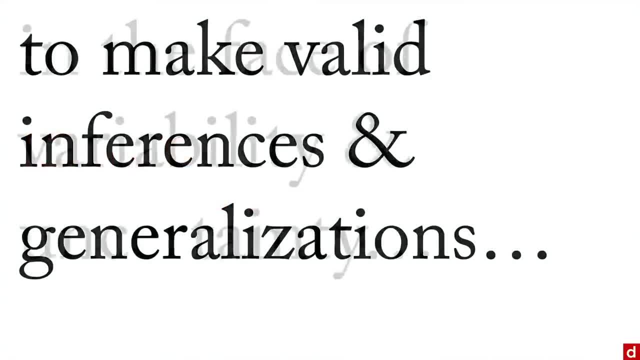 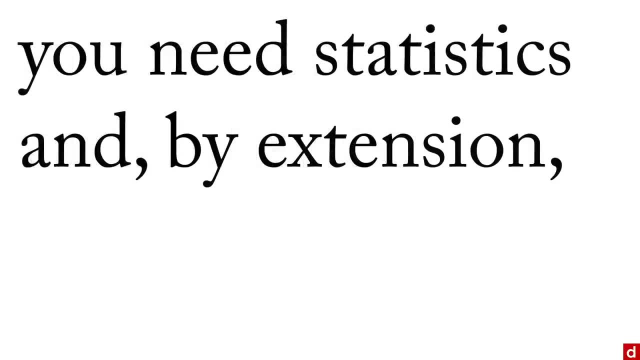 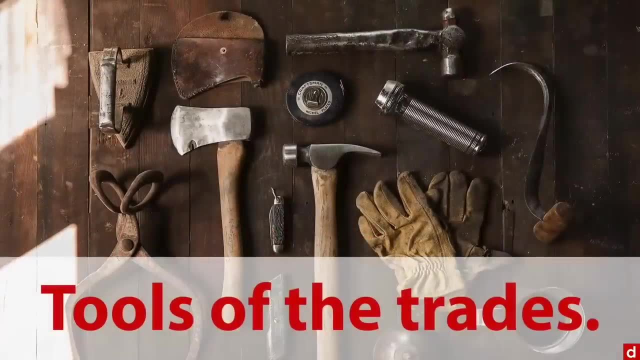 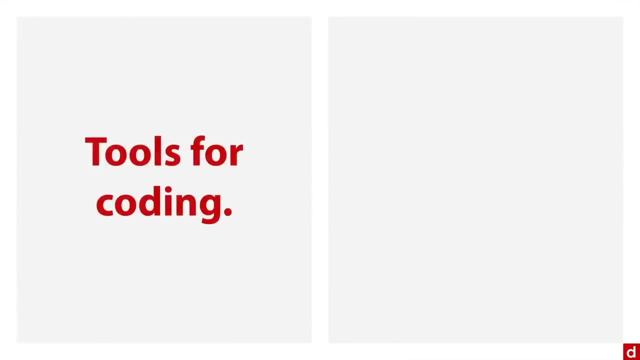 make valid inferences and generalizations In the face of variability and uncertainty in the data. you need statistics And, by extension, you need data science. It might help to compare the two by looking at the tools of the respective trades. So, for instance, there are tools for coding or generic computer programming, And 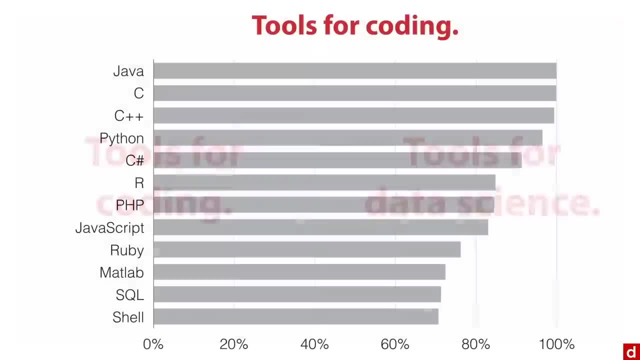 there are tools that are specific to data science. So what I have right here is a list from the I triple E of the top 10 programming languages in 2015.. And it starts at Java and C and goes down to the shell, And some of these are also used for data science. So, for instance, Python and R and SQL are used for data. 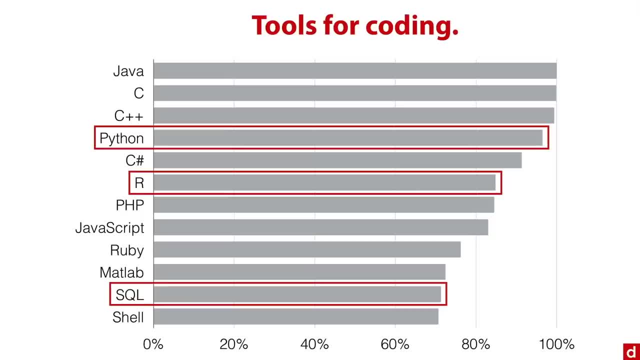 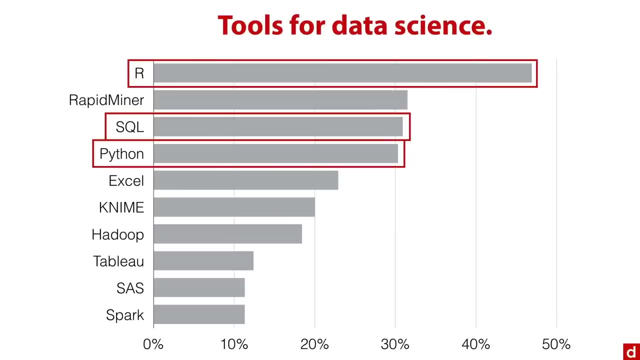 science, But the other ones aren't major ones in data science. So let's in fact take a look at a different list of most popular tools for data science, And you see that things move around a little bit. Now ours at the top, sequels there, pythons there- But for me, what's the most interesting thing on this list is that Excel is number. 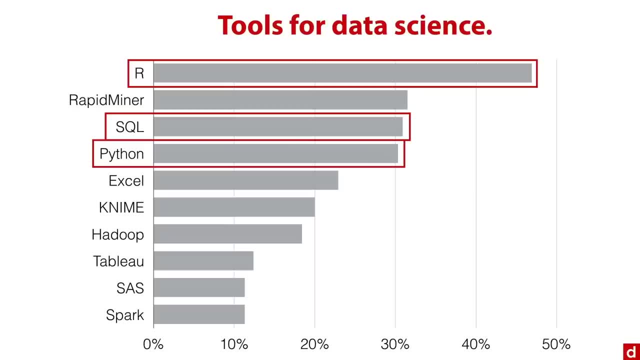 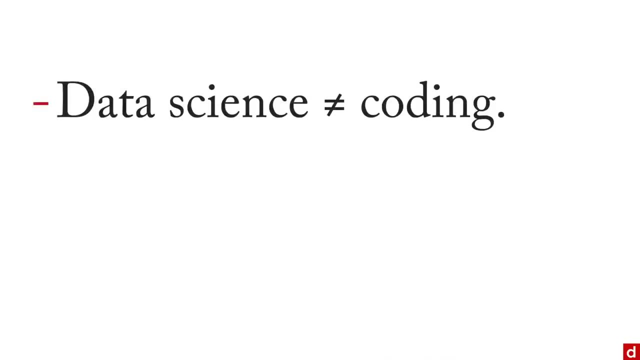 five, which would never be considered programming per se, but is in fact a very important tool for data science, And that's one of the ways that we can compare and contrast computer programming with data science. In sum, we can say this: data science is not equal to coding. 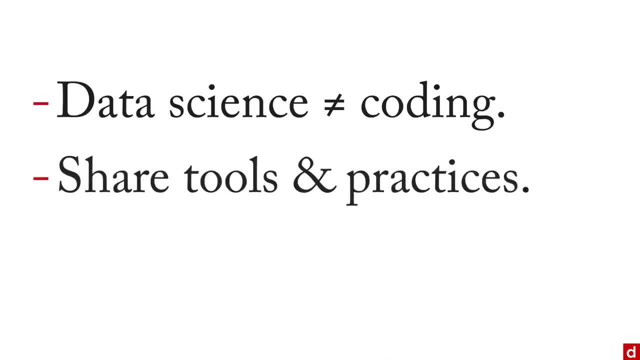 they're different things. On the other hand, they share some of the tools and they share some practices, specifically when coding for data. On the other hand, there is one very big difference in that statistics, Statistical ability, is one of the major separators between 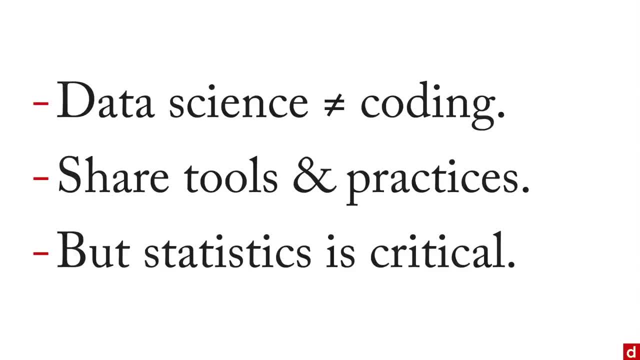 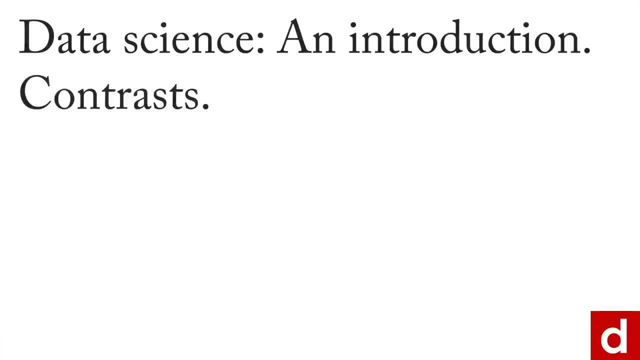 general purpose programming and data science programming. When we talk about data science and we're contrasting it with some fields, another field that a lot of people get confused and think they're the same thing is data science and statistics. Now I'll tell you there's a lot in common, But we can talk a little bit about the 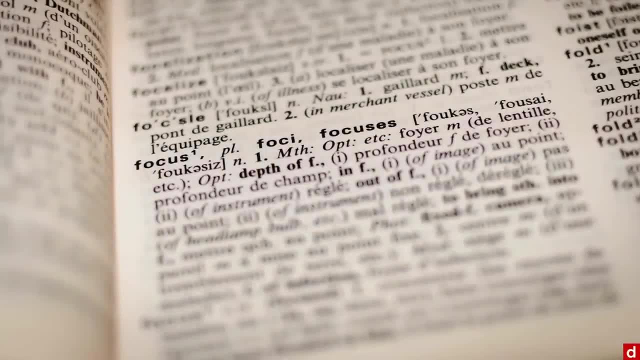 different focuses of each And we can talk a little bit about the different focuses of each. And we can talk a little bit about the different focuses of each, And we also get into the issue of sort of definitionalism that data science is different. 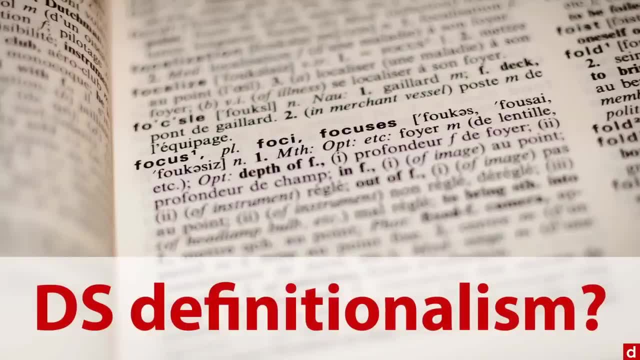 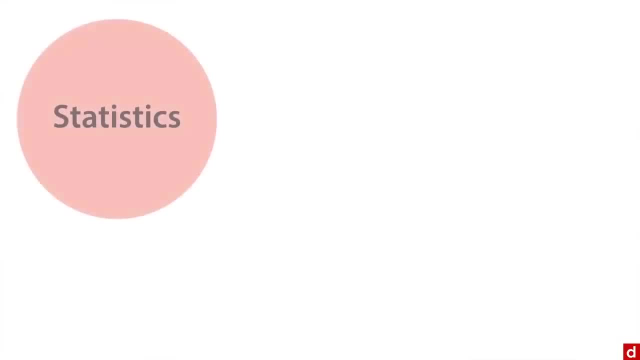 because we define it differently, even when there's an awful lot in common between the two. It helps to take a look at some of the things that go on in each field. So let's start here about statistics. put a little circle here and we'll put data science. And, to borrow a term from 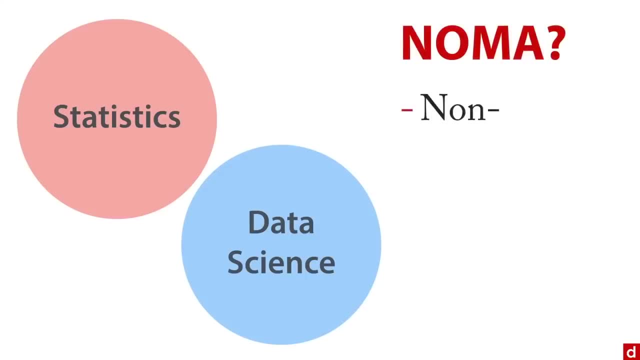 Stephen Jay Gould. we can call these non overlapping magisteria or NOMA. So you think of them as separate fields and then you can call them non overlapping magisteria or NOMA, And then you can call them non overlapping magy, TC, Fan Space and all together, pointing out which fields are. 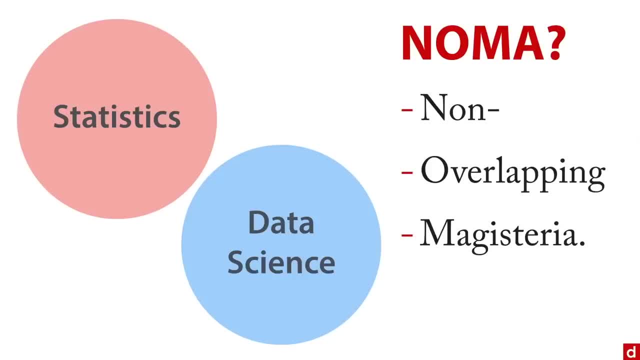 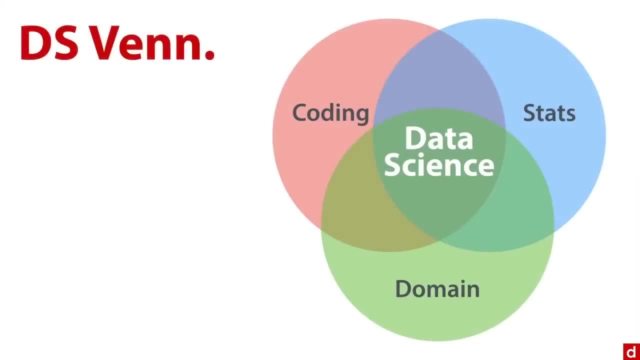 tieแต for data science. So basically there's two fields that are sovereign unto themselves, with nothing to do with each other. But you know that doesn't seem right, And part of that. if we go back to the data science Venn diagram, you know statistics is one part of it. there it is in the 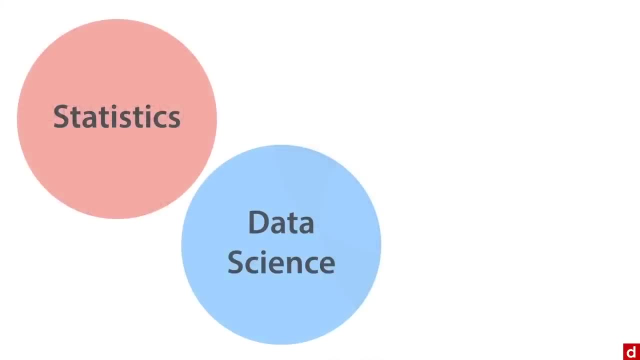 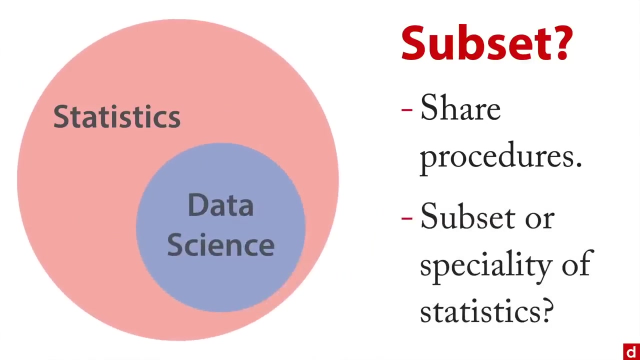 top corner. So now, what do we do? What's the relationship? So it doesn't make sense to say these are totally separate areas. maybe data science and statistics- because they share- is a subset or a specialty of statistics, more like this. But if data science were just a subset or 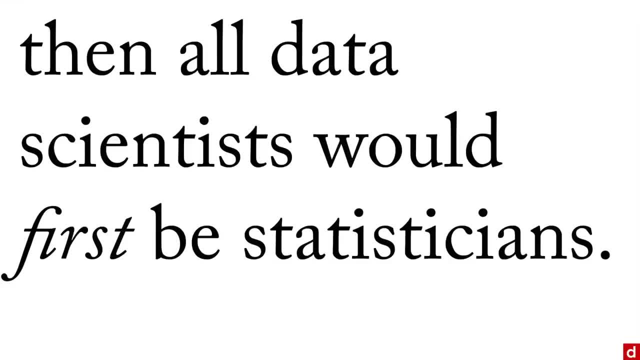 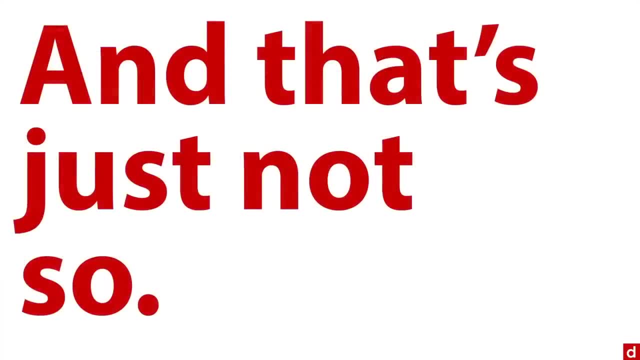 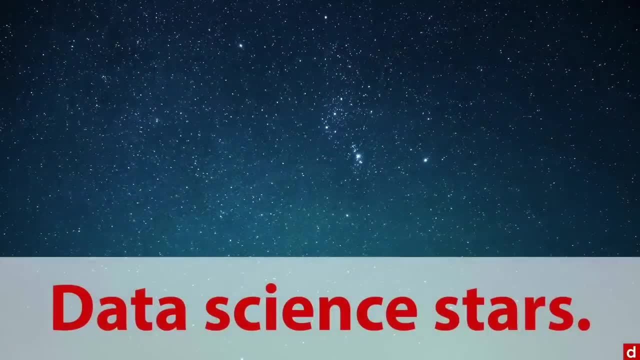 specialty within statistics, then it would follow that all data scientists would first be statisticians, And interestingly, that's just not so. Say, for instance, we take a look at the data science stars, the superstars in the field, we go to a rather intimidating article. it's called the. 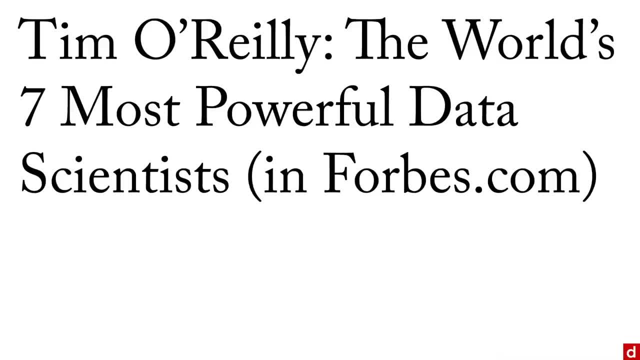 world's seven most powerful data scientists from forbescom, And you can see the article if you go to this URL. There's actually more than seven people on the list because sometimes he brings them up in pairs. But let's check their degree, see what their academic training is in. If we 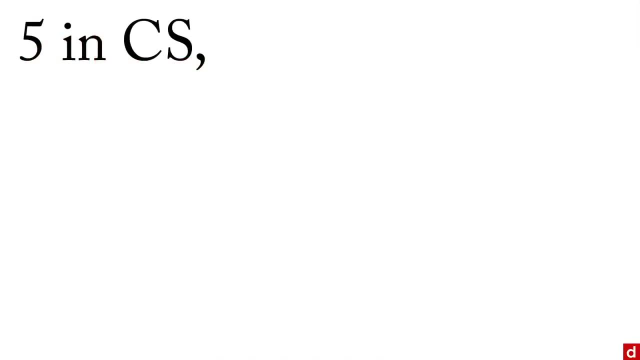 take all the people on this list, we have five degrees in computer science, three in math, two in math and three in math. So if we take all the people on this list, we have five degrees in computer science, three in math, two in math and three in math. So if we take all the people on this, 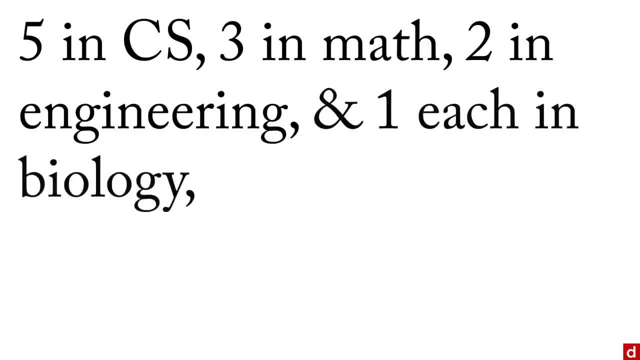 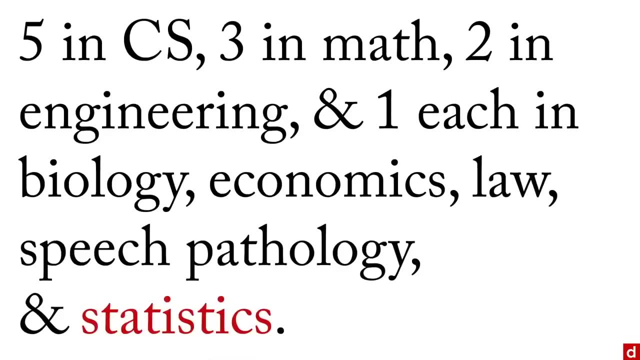 list, we have five degrees in computer science, three in math, two in engineering and one each in biology, economics, law, speech pathology and one in statistics, And so that tells us, of course, that these major people in data science are not trained as statisticians. only one of them has. 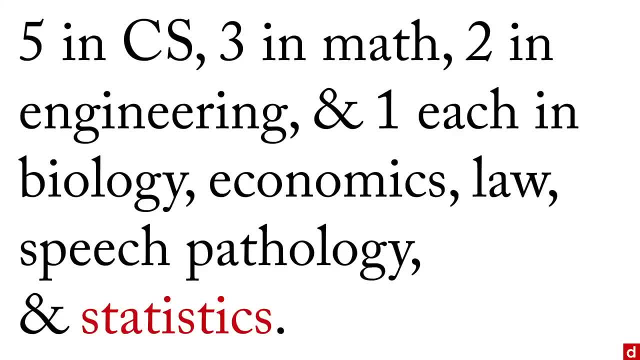 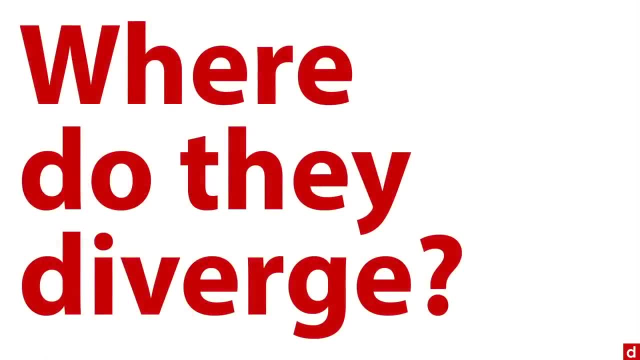 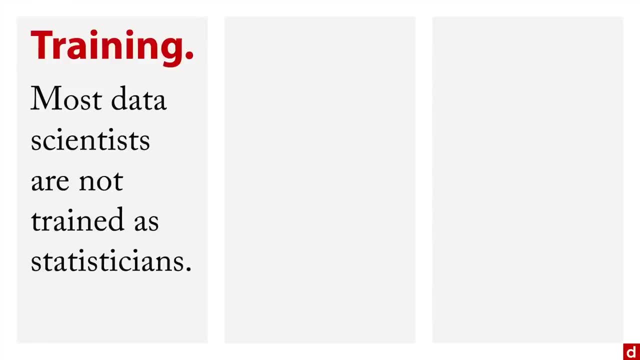 formal training in that. So that gets us to the next question: where do these two fields, statistics and data science, diverge? Because they seem like they should have a lot in common but they don't have a lot in training. And specifically, we can look at the training. Most data scientists are not. 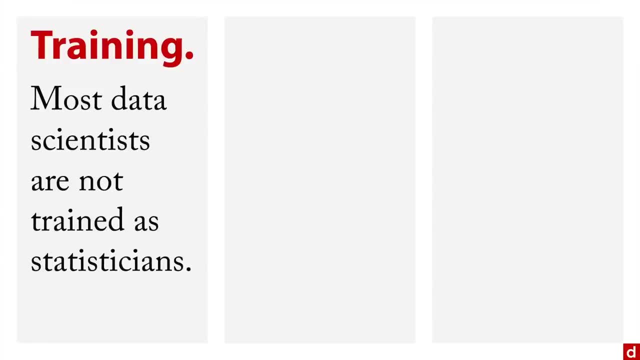 trained formally as statisticians. Also, in practice, things like machine learning and big data, which are central to data science, are not shared generally with most of statistics, And so they have separate domains there. And then there's the really important issue of context: Data scientists. 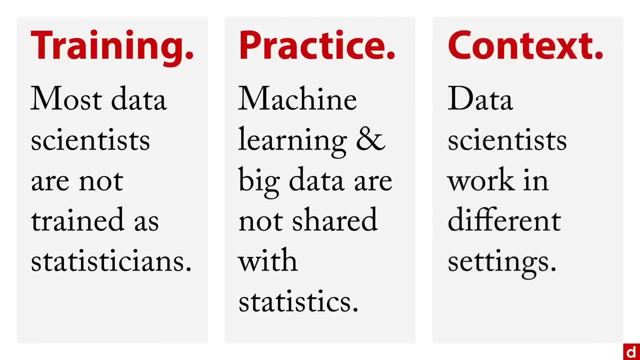 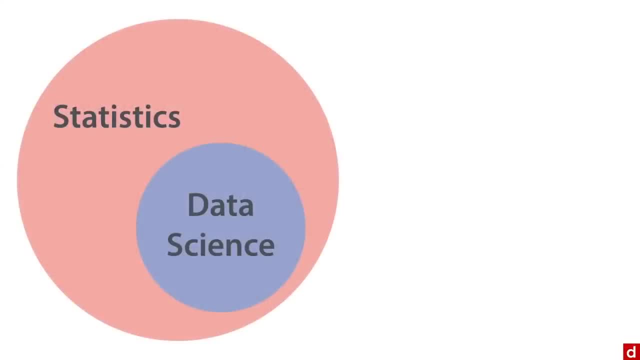 tend to work in different settings than statisticians. Specifically, data scientists very often work in commercial settings, where they're trying to get recommendation engines or ways of developing a product that will make them money. So maybe instead of having data science as a subset of statistics, we can think of it more, as these two fields have different niches. They 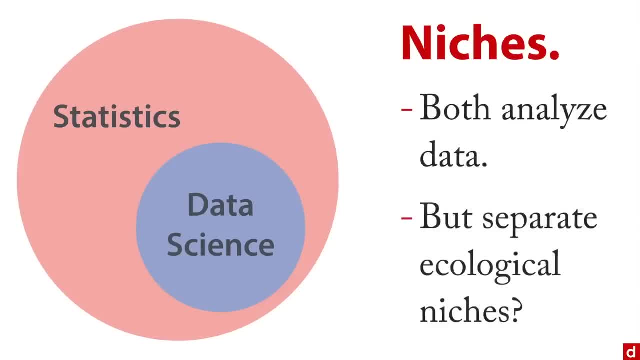 both analyze data, but they do different things in different ways. So maybe we can think of data science as a subset of statistics. Maybe it's fair to say they share, they overlap, they both have analysis in common of data, but otherwise they are ecologically distinct. So, in sum, what we can. 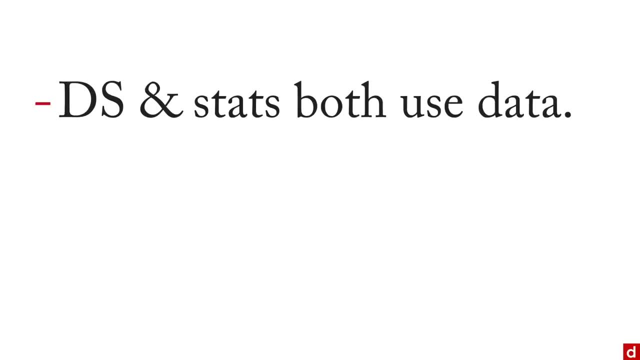 say here is that data science and statistics both use data and they analyze it, But the people in each tend to come from different backgrounds And they tend to function with different goals and contexts And in that way render them to be conceptualized. 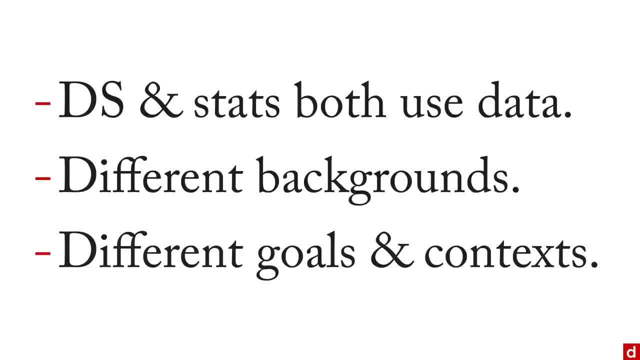 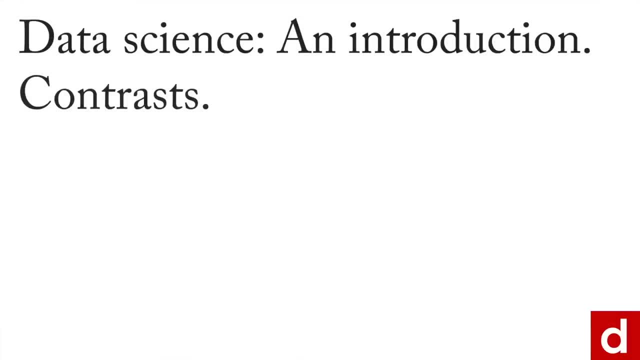 Actually distinct fields, despite the apparent overlap As we work to get a grasp on data science. there's one more contrast I want to make explicitly, And that's between data science and business intelligence or BI. The idea here is that business intelligence is data in real life. 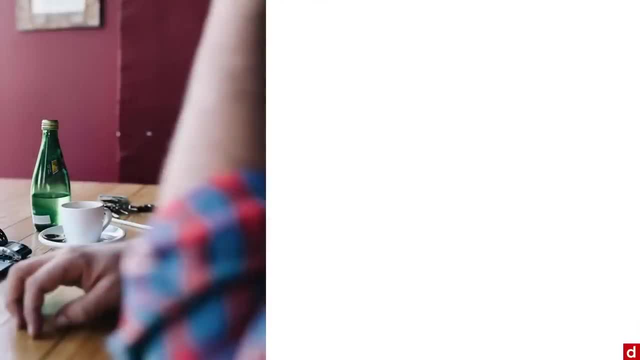 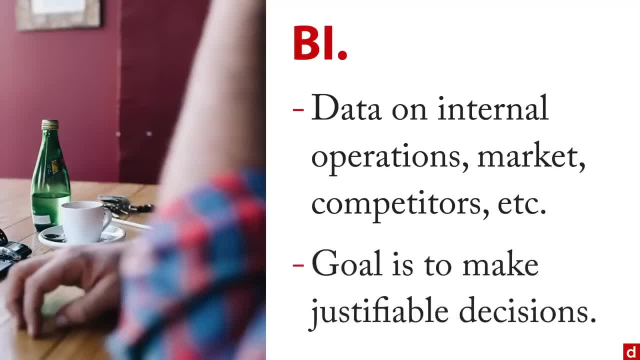 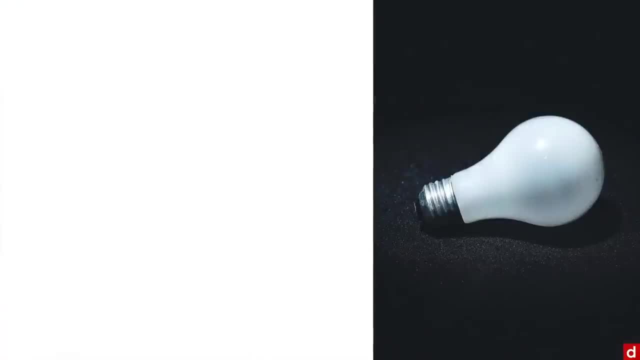 sitting in the bar and doing whenever comes to your mind. Now, data science is involved with this, except you know, really there's no coding in bi, There's using apps that already exists, And the statistics in business intelligence tend to be very simple. They tend to be counts. 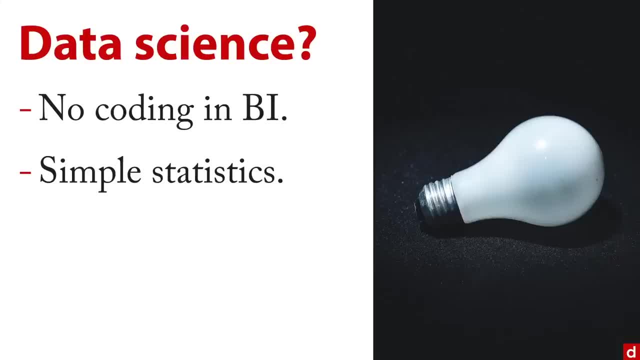 and percentages and ratios, And so it's simple. the light bulb is simple, it just does its one job. there's nothing super sophisticated there. Instead, the focus in business intelligence is on domain expertise and on really useful direct utility. It's simple, it's effective and it provides insight. Now, one of the main 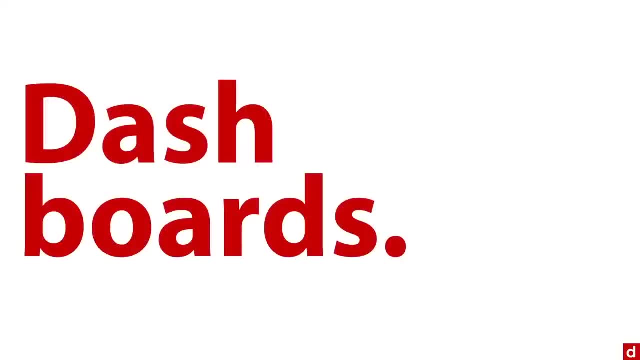 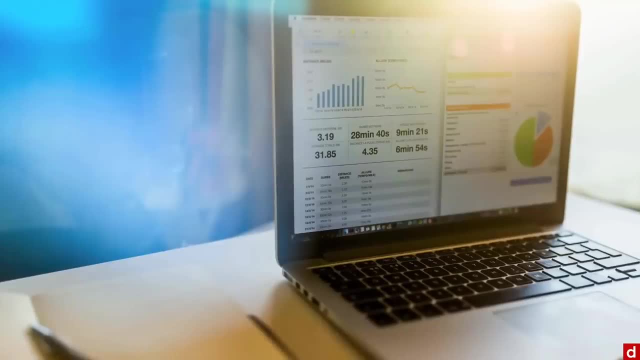 associations with business intelligence is what are called dashboards or data dashboards. They look like this: it's a collection of charts and tables that go together to give you a very quick overview of what's going on your business. And well, a lot of data scientists may, let's say, 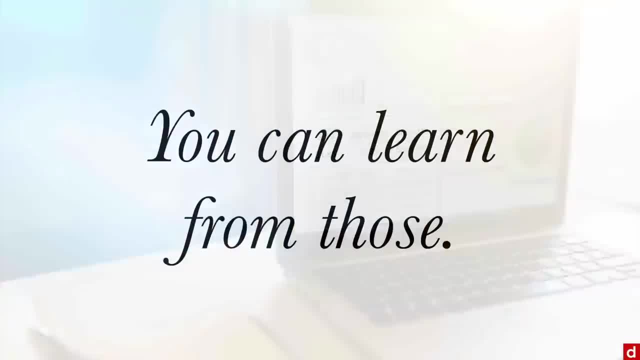 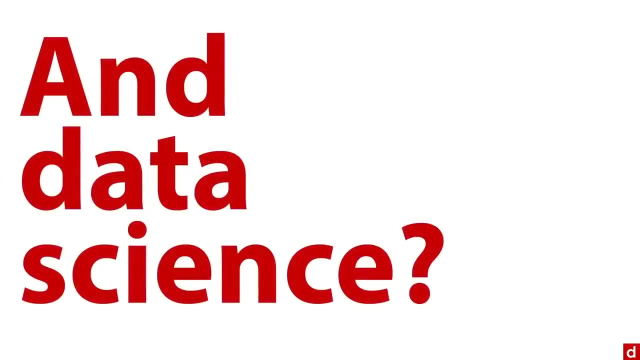 look down their nose upon dashboards, I'll say this: most of them are very well designed and you can learn a huge amount about user interaction and the accessibility of information from dashboards. So, really, where does data science come into this? What's the connection? 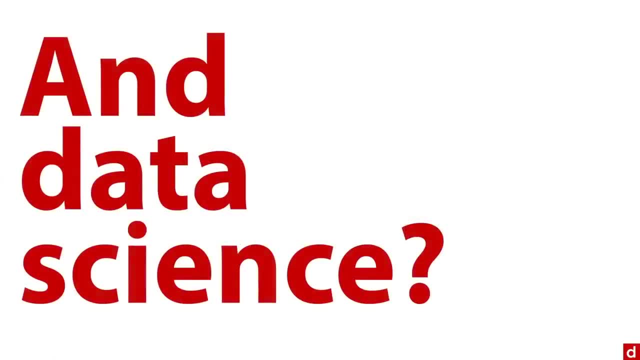 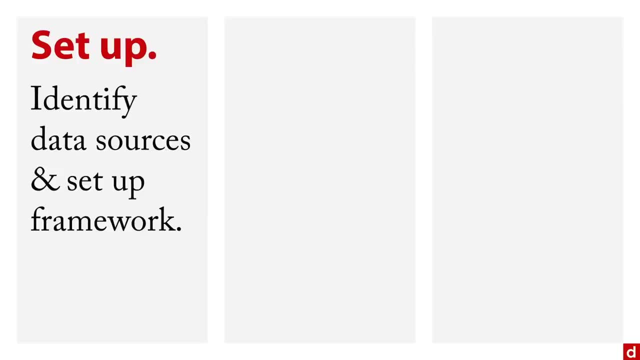 between data science and Google Analytics. technically, we have systems, a community and business intelligence. Well, data science can be useful to BI in terms of setting it up, identifying data sources and creating or setting up the framework for something like a dashboard or a business intelligence system. Also, data science can be used to extend it. Data science: 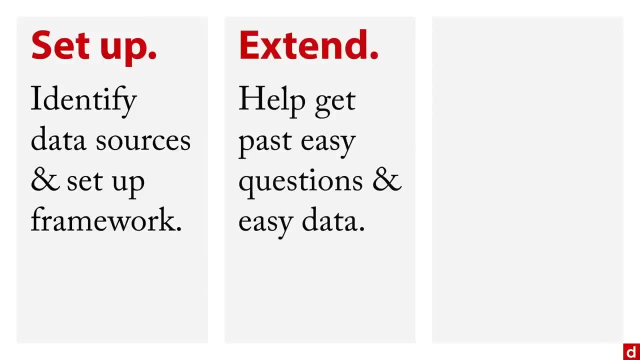 can help get past the easy questions and the easy data to get the questions that are actually most useful to you, even if they require really sometimes data that's hard to wrangle and work with, And also there's an interesting interaction here that goes the other way. 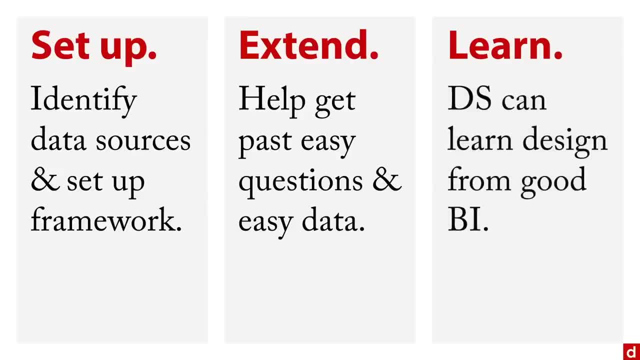 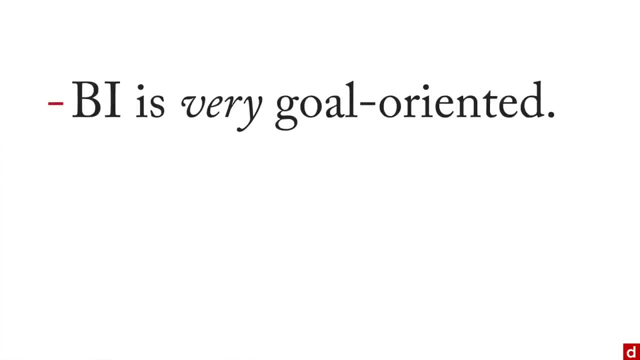 Data science practitioners can learn a lot about design from good business intelligence applications, So I strongly encourage anybody in data science to look at them carefully and see what they can learn. In some, business intelligence, or BI, is very goal oriented. Data science perhaps prepares the data and sets up the form for business intelligence, But also data science 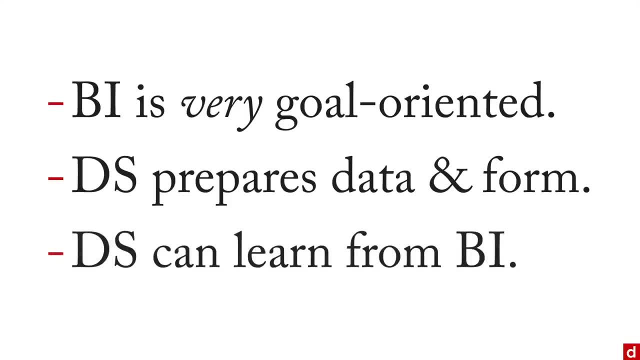 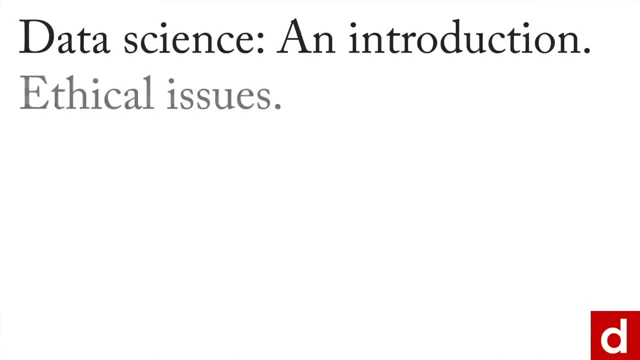 can learn a lot about usability and accessibility from business intelligence, And so it's always worth taking a close look. Data science has a lot of really wonderful things about it, But it is important to consider some ethical issues, And I'll specifically call this: do no harm in your data. 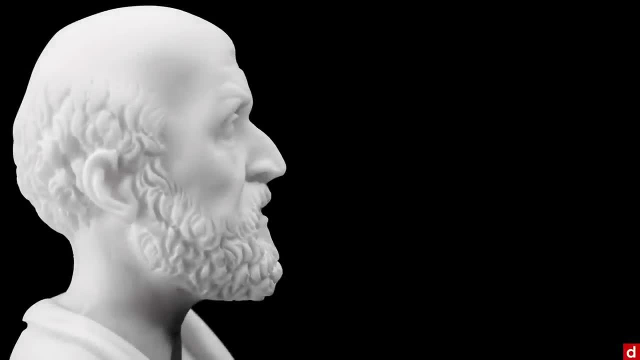 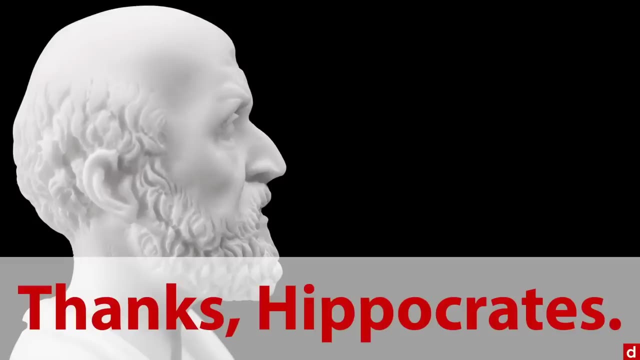 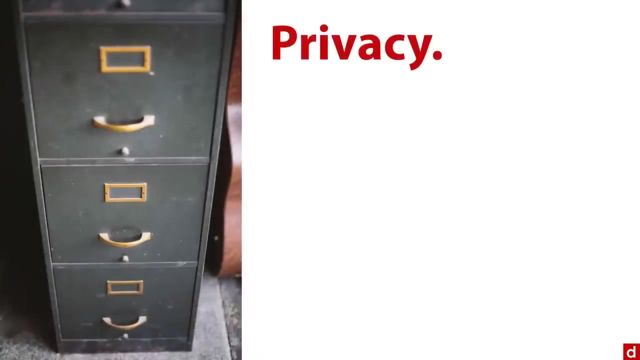 science Projects, And for that we can say thanks to Hippocrates, the guy who gave us the Hippocratic oath of do no harm. Let's specifically talk about some of the important ethical issues very briefly that come up in data science. Number one is privacy. that data tells you a lot about people. 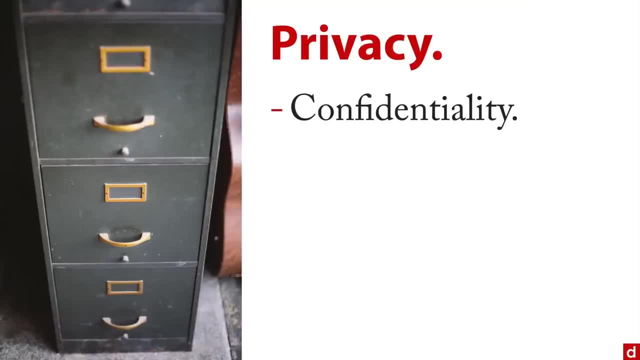 and you need to be concerned about the confidentiality. If you have private information about people- their names, their social security numbers, their addresses, their credit scores, their social security numbers, their addresses, their credit scores, their health- that's private, that's confidential And you shouldn't share that information unless they 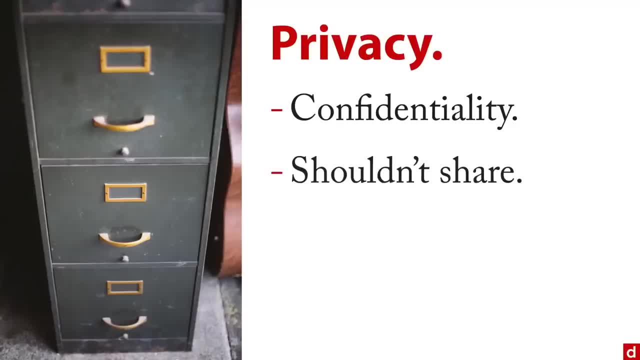 specifically gave you permission. Now, one of the reasons this presents a special challenge in data science because we'll see later, a lot of the sources that are used in data science were not intended for sharing. If you scrape data from a website or from PDFs, you need to make sure that. 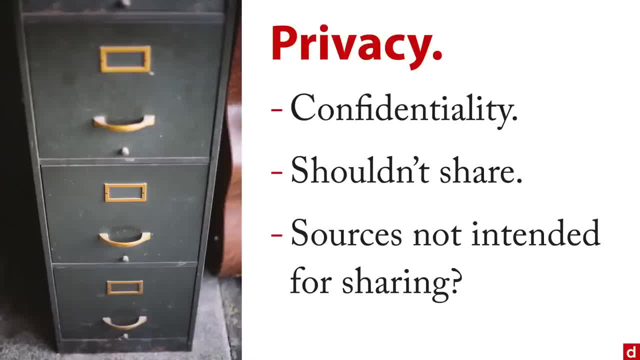 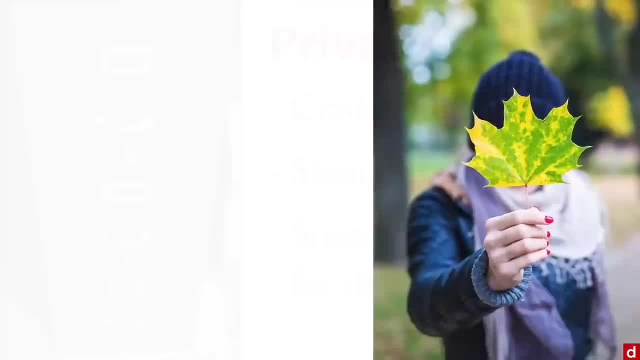 it's okay to do that, But it was originally created without the intention of sharing, So privacy is something that really falls upon the analyst to make sure they're doing it properly. Next is anonymity. One of the interesting things we find is that it's really not hard to identify. 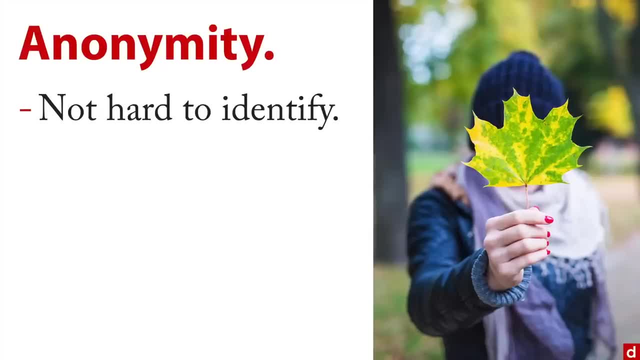 people in data. If you have a little bit of GPS data and you know where a person was at four different points in time, you have about a 95% chance of knowing exactly who they are. You look at things like HIPAA, that's the Health Insurance Portability and Accountability Act. 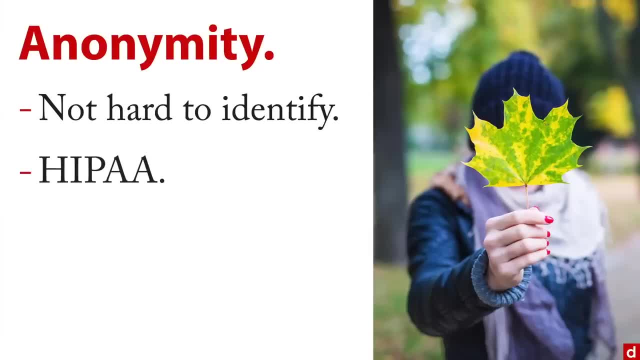 Before HIPAA, it was really easy to identify people for medical records. Since then, it has become much more difficult to identify people uniquely. That's an important thing for really people's well being. And then also proprietary data. If you're working for a client, a company, and they give you their own data, that data may. 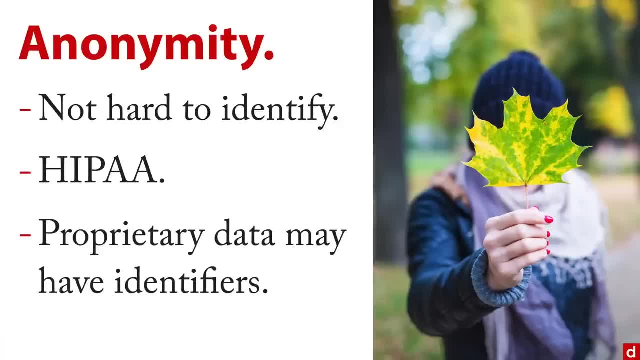 have identifiers, you may know who the people are and they're not anonymous anymore. So anonymity may or may not be their major efforts to make data anonymous, But really the primary thing is that even if you do know who the data is, you will be able to identify people. So anonymity is a very 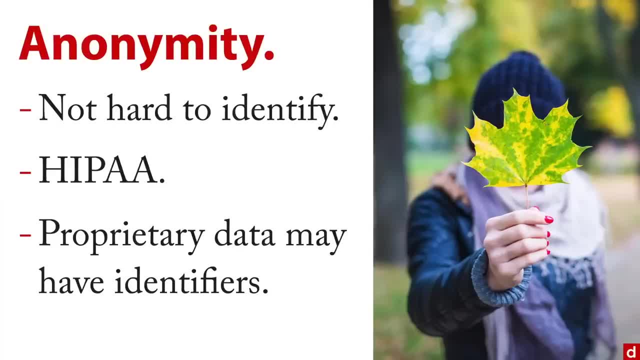 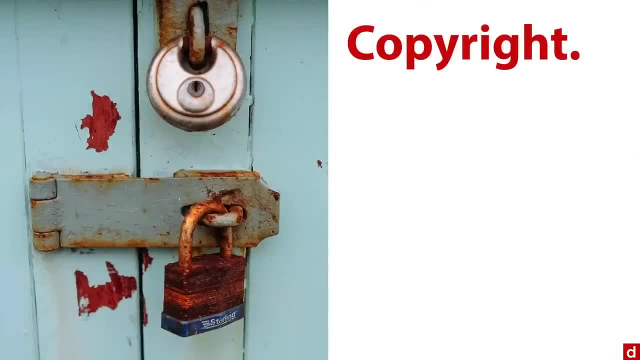 know who they are, that you still maintain the privacy and confidentiality of the data. Next, there's the issue about copyright, where people try to lock down information. Now, just because something is on the web doesn't mean that you're allowed to use it. 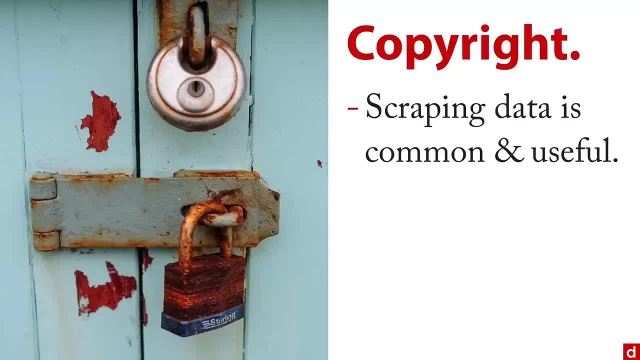 Scraping data from websites is a very common and a useful way of getting data for projects. You can get data from web pages, from PDFs, from images, from audio, from really a huge number of things. But again, the assumption that because it's on the web, it's okay to use it is not true. 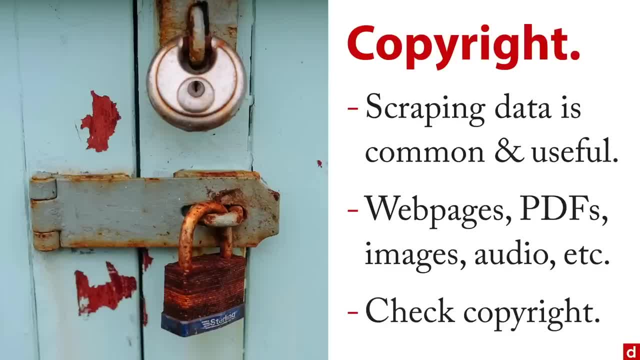 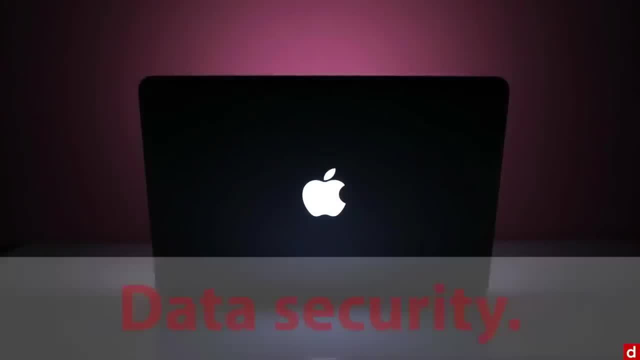 You always need to check copyright and make sure that it's acceptable for you to access that particular data. Next in our very ominous picture is data security, And the idea here is that when you go through all the effort to get data from websites, you're going to get data from websites. 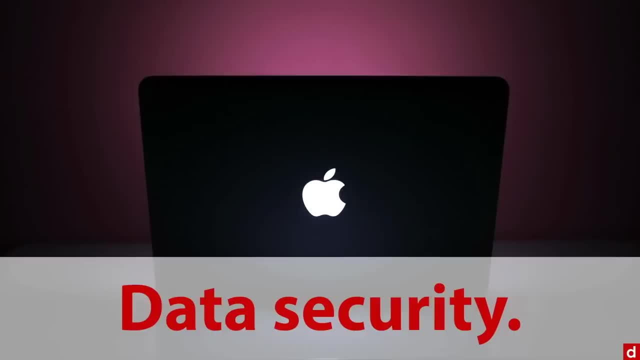 Gather data to clean it up and prepare for an analysis. You've created something that's very valuable to a lot of people And you have to be concerned about hackers trying to come in and steal the data, especially if the data is not anonymous and it has identifiers in it. 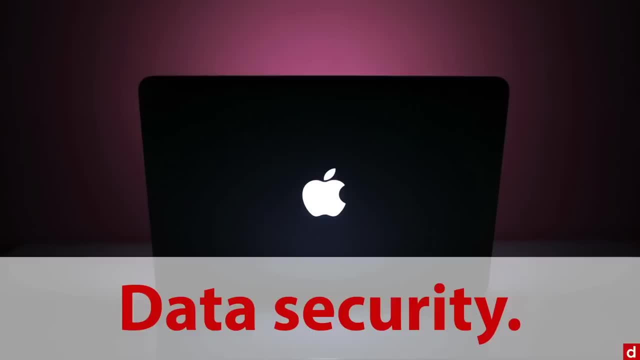 And so there is an additional burden placed on the analyst to ensure, to the best of their ability, that the data is safe and cannot be broken into and stolen, And that can include very simple things like a person who is on the project but is no longer, but took the data on a flash drive. 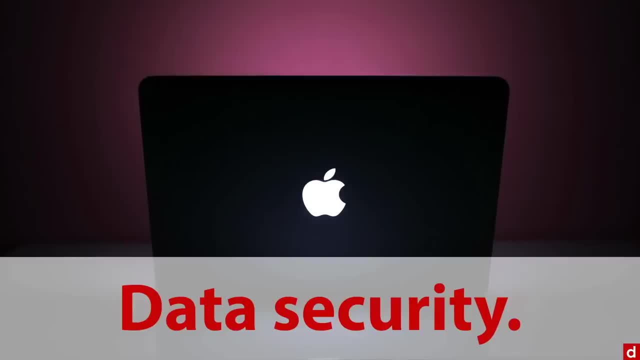 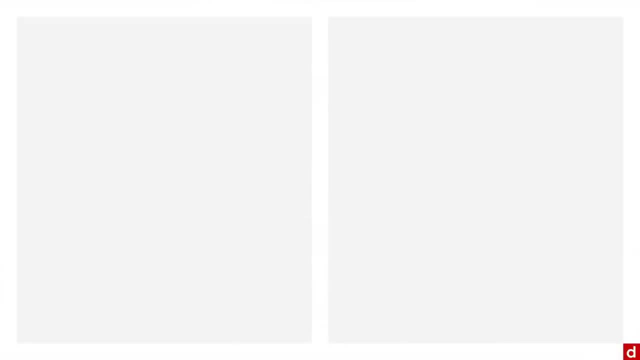 You have to find ways to make sure that that can't happen as well. There's a lot of possibilities. It's tricky, but it's something that you have to consider thoroughly. Now two other things that come up in terms of ethics but don't usually get addressed in these. 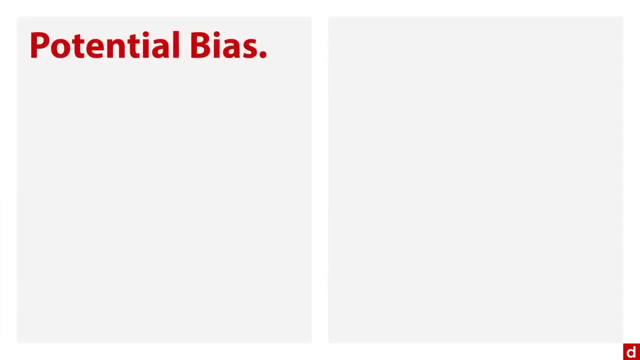 conversations. Number one is potential bias. The idea here is that the algorithms or the formulas that are used in data science are only as neutral and bias free as the rules and the data that they get, And so that's one of the things that we need to be careful about. And the other thing 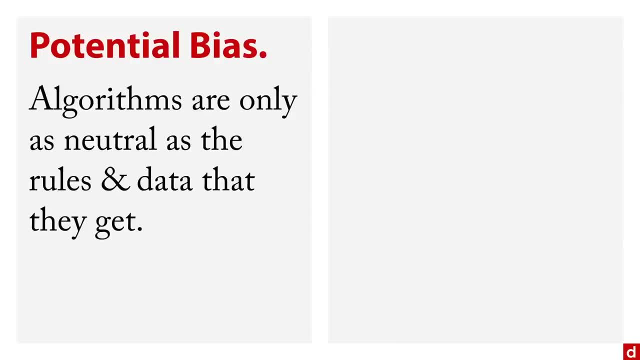 here is that if you have rules that address something that is associated with, for instance, gender or age or race or economic standing, you might unintentionally be building in those factors which say, for instance, for Title IX, you're not supposed to. you might be building those into the 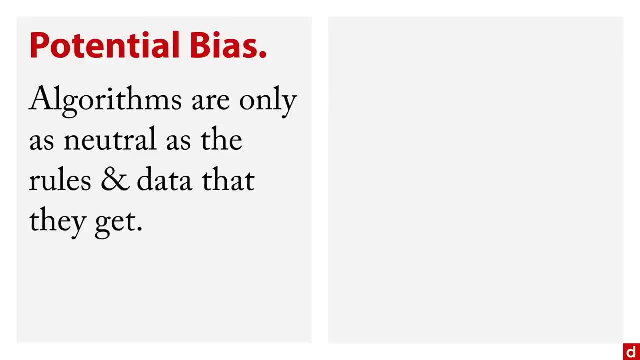 system without being aware of it, And an algorithm has this sheen of objectivity And people can say they can place confidence in it, but they can't. And so the idea here is that if you have rules that address something, you might unintentionally be building in those factors which say, for instance, 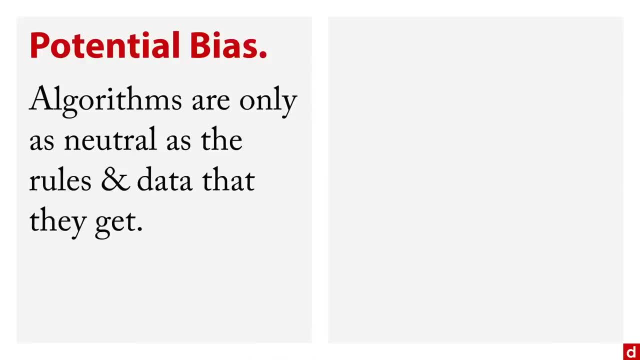 gender or age or age or economic standing. you might unintentionally be building in those factors without realizing that it's replicating some of the prejudices that may happen in real life. Another issue is overconfidence, And the idea here is that analyses are limited simplifications. 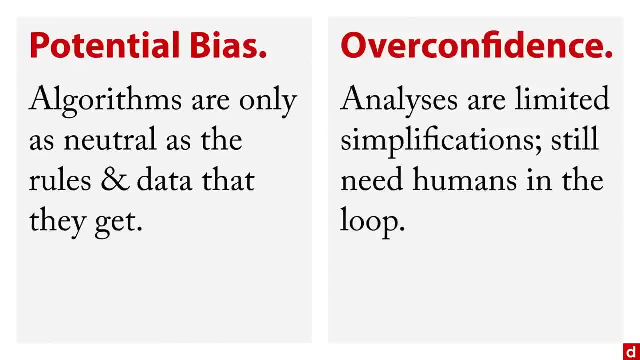 they have to be, that. that's just what they are, And because of this, you still need humans in the loop to help interpret and apply this. The problem is when people run an algorithm, they get out a number, say to 10 decimal places, and they say: this must be true. And they say this must be true. 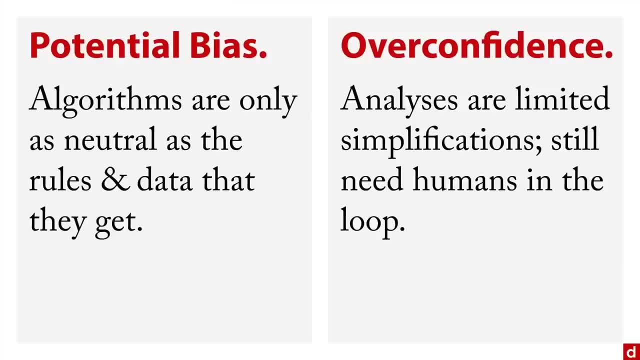 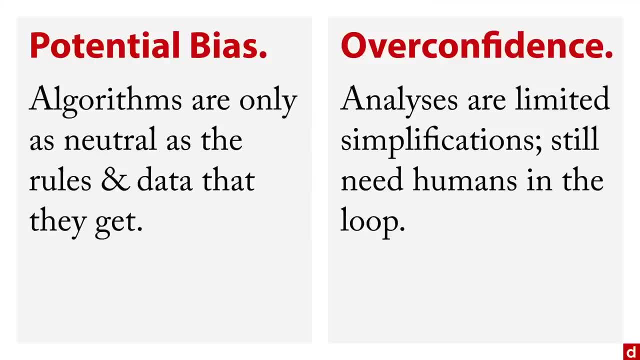 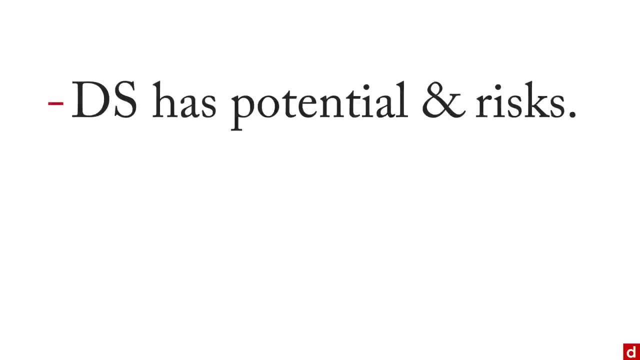 have enormous problems and go down the wrong path with too much confidence in your own analyses. So, once again, humility is in order when doing data science work. In sum, data science has enormous potential, but it also has significant risks involved in the projects. Part of the. 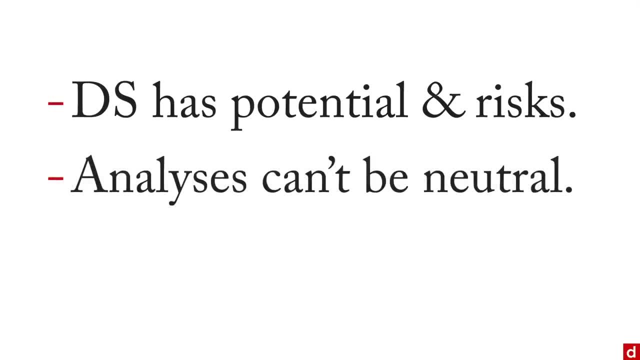 problem is that analyses can't be neutral, that you have to look at how the algorithms are associated with the preferences, prejudices and biases of the people who made them, And what that means is that, no matter what, good judgment is always vital to the quality and success of a data. 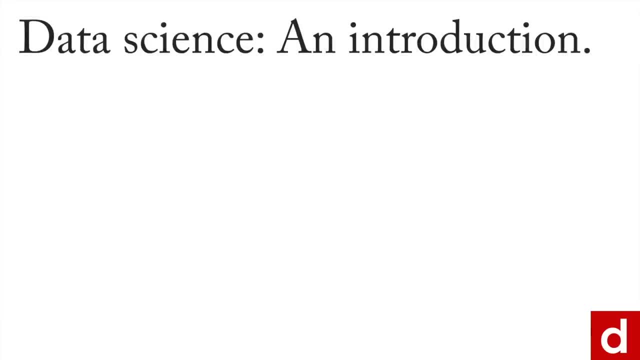 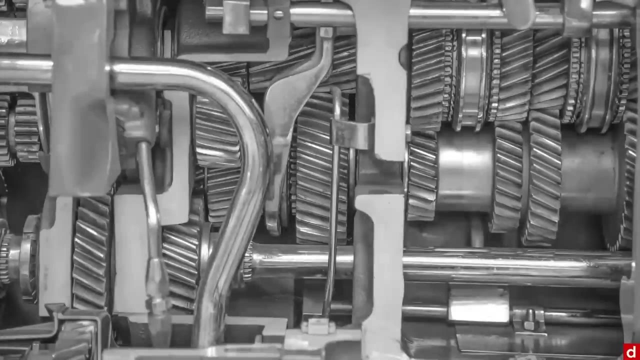 science project. Data science is a field that is strongly associated with its methods or procedures. In this section of videos, we're going to provide a brief overview of the methods that are used in data science. Now, just as a quick warning: in this section things can get kind of technical and that can cause some. 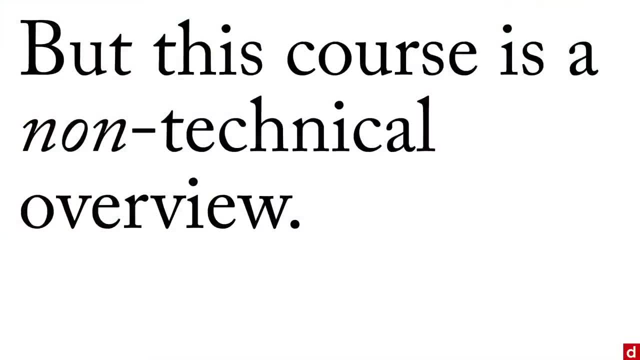 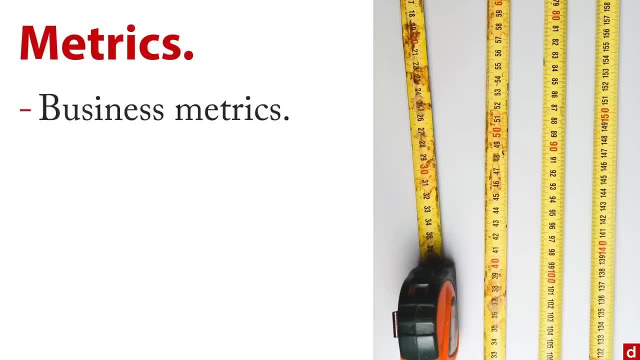 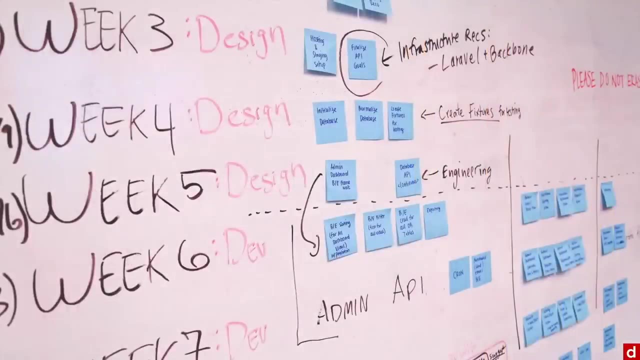 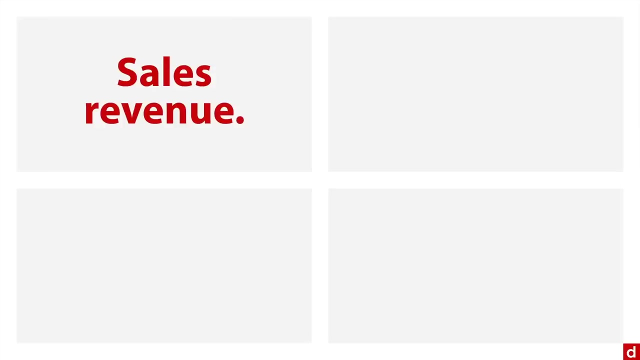 stuff is in the other course, But this course is a non technical overview. The technical hands on stuff is in the other course, But this course is a non technical overview. The technical hands on moving the merchandise: Are you getting sales? Also, there's the issue of leads generated, new 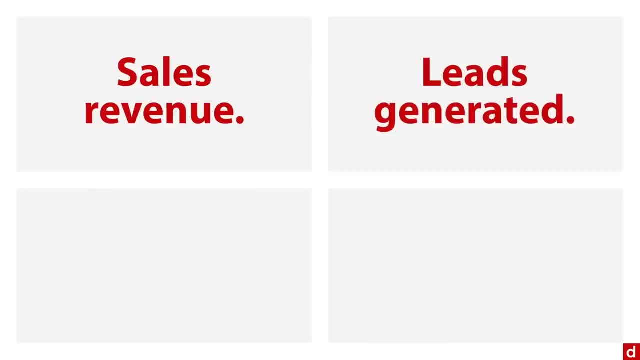 customers or new potential customers, because that then in turn is associated with future sales. There's also the issue of customer value, or lifetime customer value. So you may have a small number of customers, but they all have a lot of revenue And you can use that to really 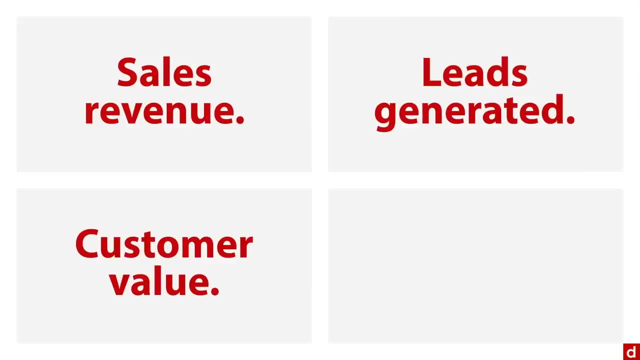 predict the overall profitability of your current system. And then there's churn rate, which has to do with, you know, losing and gaining new customers and having a lot of turnover. So any of these are potential ways of defining success and measuring it. These are potential metrics. there are others. 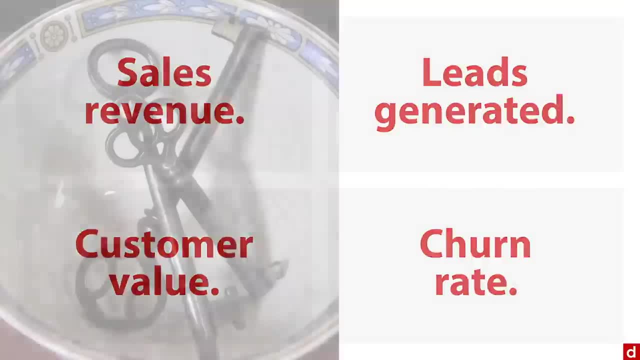 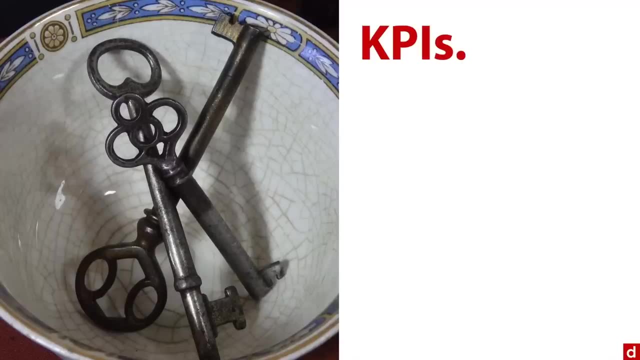 but these are some really common ones. Now, I mentioned earlier something called a key performance indicator or KPI. KPIs come from David Parmenter and he's got a few ways of describing them. He says a key performance indicator for business number one should be: 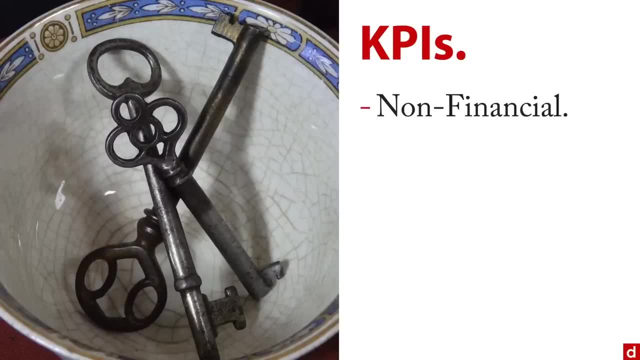 non financial, So not just the bottom line, But something else that might be associated with it or that measures the overall productivity of the association. They should be timely, for instance weekly, daily or even constantly gathered information. They should have a CEO focus. So the senior management team are the 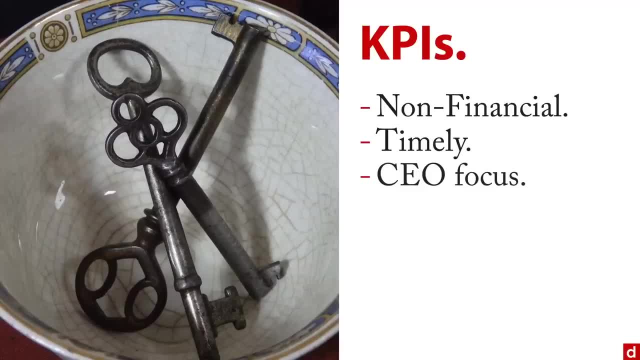 ones who generally make the decisions that affect how the organization acts on the KPIs. They should be simple, So everybody in the organization, everybody knows what they are and knows what to do about them. They should be simple, So everybody in the organization, everybody knows. 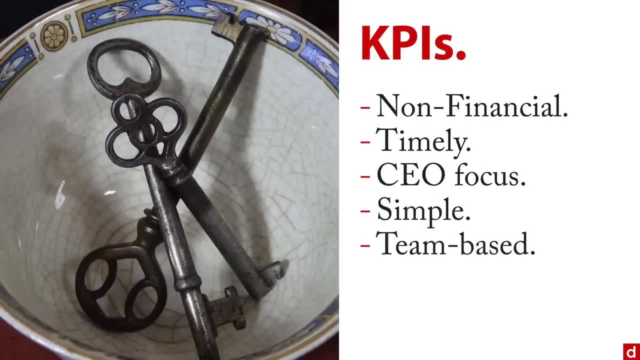 what to do about them. They should be team based So teams can take joint responsibility for meeting each one of the KPIs. They should have significant impact. What that really means is they should affect more than one important outcome, So you can do profitability. 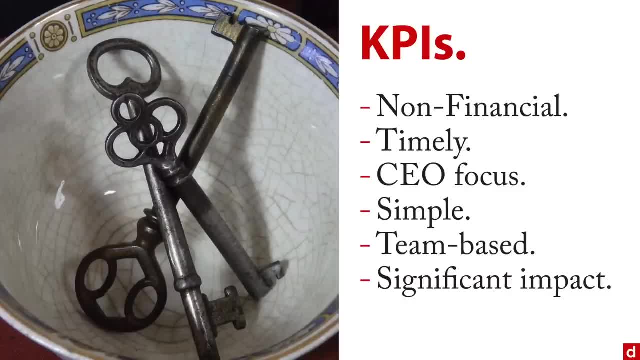 and market reach, or improved manufacturing time and fewer defects. And finally, an ideal KPI has a limited dark side. That means there's fewer possibilities for reinforcing the wrong behaviors and rewarding people for sort of exploiting the system. Next there are SMART. 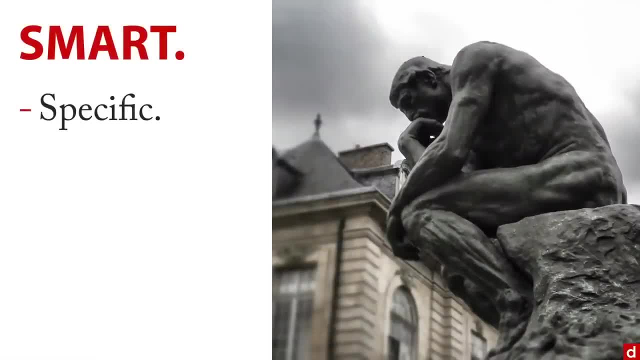 goals where SMART stands for specific, measurable, assignable to a particular person. realistic, meaning you can actually do it with the resources you have at hand and time bound, so you know when it can get done. So whenever you form a goal, you should try to. 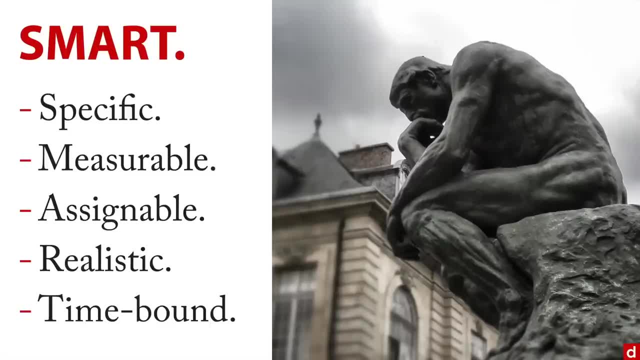 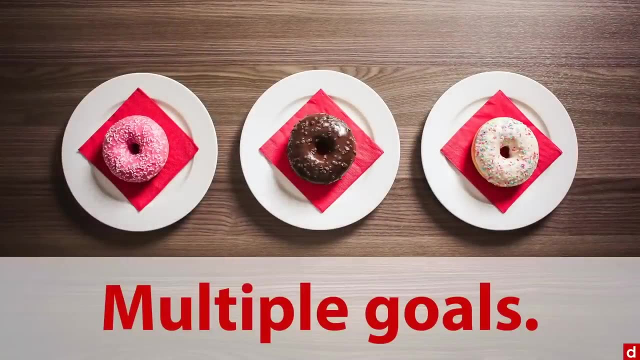 assess it on each of these criteria, And that's a way of saying that this is a good goal to be used as a metric for the success of our organization. Now, the trick, however, is when you have multiple goals, multiple possible endpoints, And the reason that's difficult is: 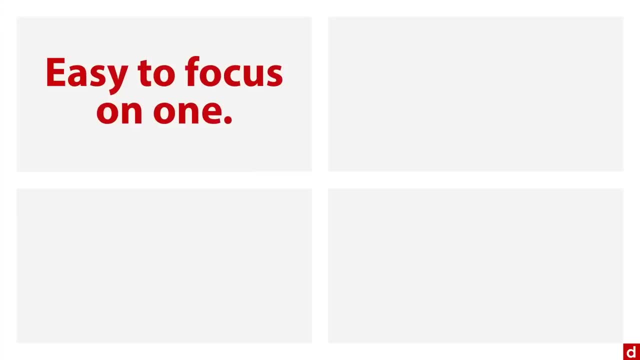 because, well, it's easy to focus on one goal. if you're just trying to maximize revenue, or if you're just trying to maximize- you know- graduation rate, there's a lot of things you can do. It becomes more difficult when you have to focus on many things simultaneously, especially because 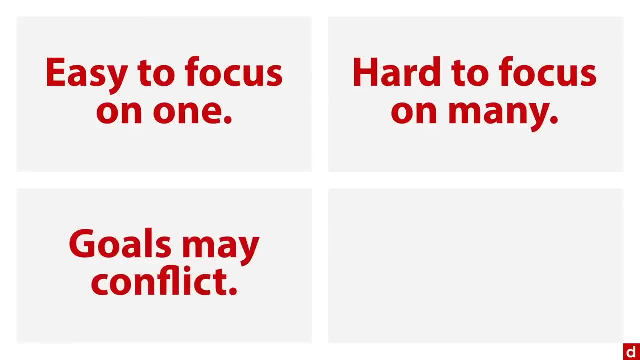 some of these goals may conflict. So if you have a goal, you have to focus on one goal, and if you click the things that you do to maximize, one may impair the other, And so when that happens, you actually need to start engaging in a deliberate process of optimization. you need to 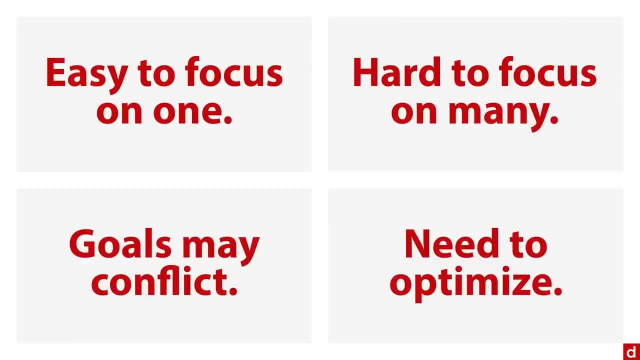 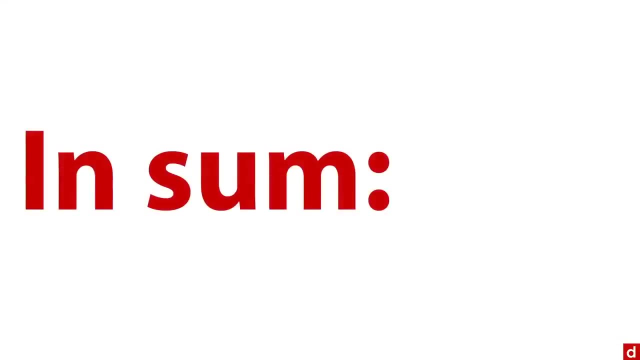 optimize, And there are ways that you can do this. If you have enough data, you can do a mathematical optimization to find the ideal balance of efforts to pursue one goal and the other goal at the same time. Now this is a very general summary And let me finish with this: in some metrics, 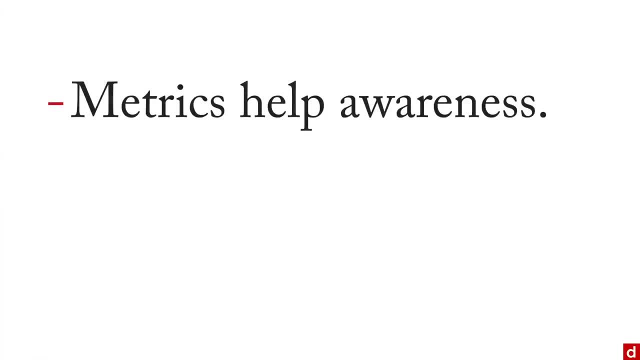 or methods for measuring, can help awareness of how well your organization is functioning and how well you're reaching your goals. There are many different methods available for defining success and measuring progress towards those things. The trick, however, comes when you have to balance efforts to reach multiple goals simultaneously, which can bring in the need for things like 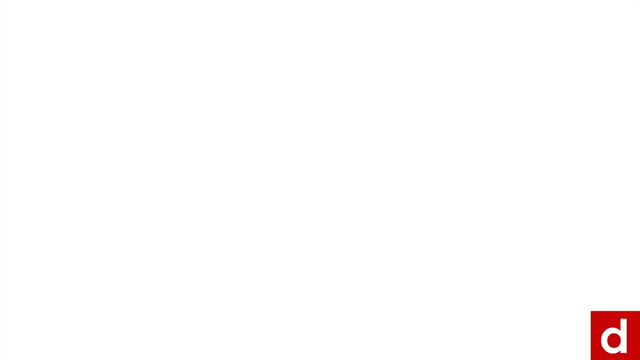 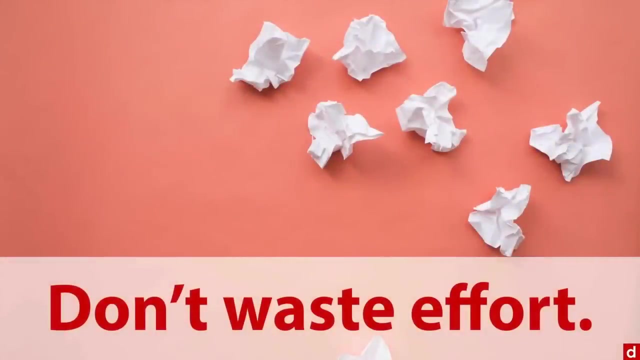 optimization. When talking about data sourcing and measurement, one very important issue has to do with the accuracy of your measurements. The idea here is that you don't want to have to throw away all your ideas. you don't want to waste effort. One way of doing this in a very 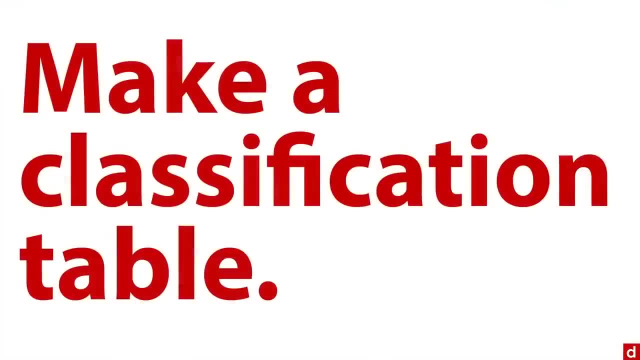 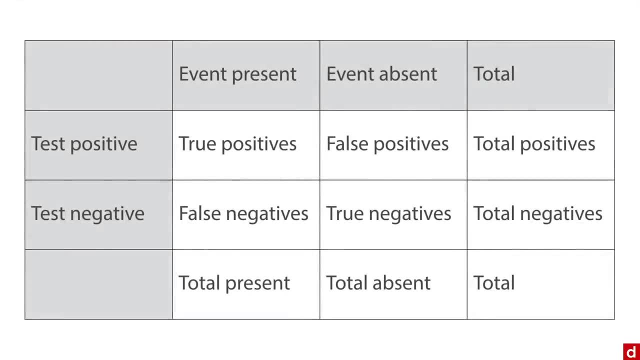 quantitative fashion is to make a classification table. So what that looks like is this. you talk about, for instance, positive results, negative results, And in fact, let's start by looking at the top here, the middle. two columns here talk about whether an event is present, whether your. 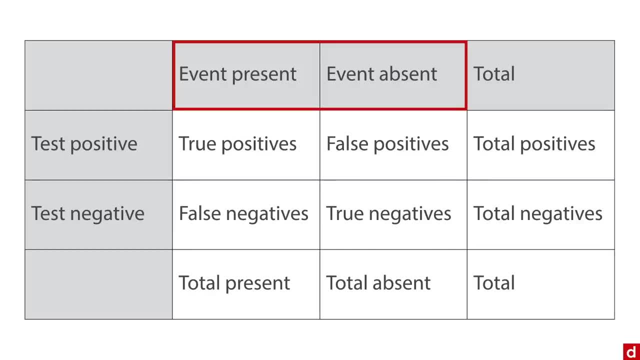 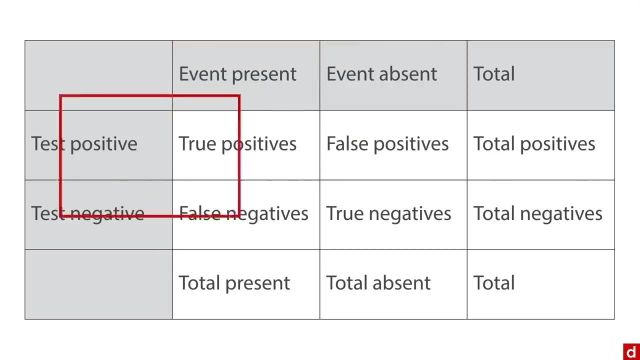 thing is actually happening or not. On the left here is whether the test or the indicator suggests that a thing is or is not happening, And then you have these combinations of true positives, where the test says it's happening and it really is, and false positive where the test says it's. 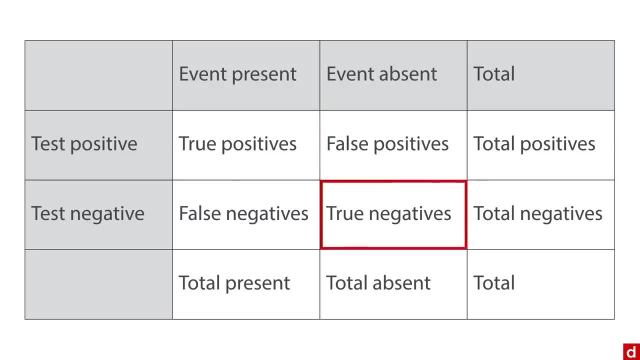 happening but it's not. And then, below that, true negatives, where the test says it isn't happening and that's correct, And then false negatives, where the test says there's nothing going on, but there is in fact the event occurring. And then you start to get the column totals. 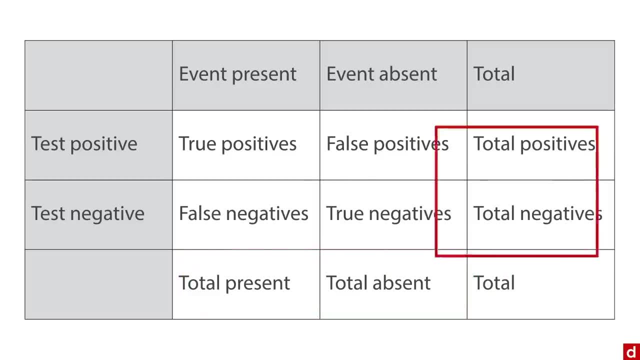 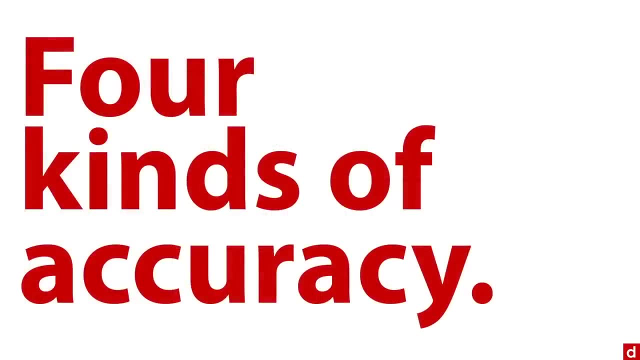 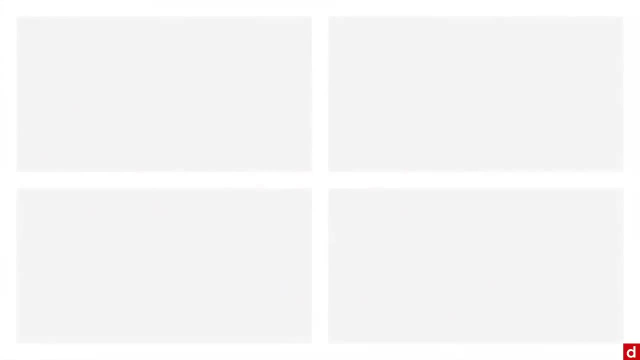 the total number of events present or absent and the row totals that talk about the test results. Now, from this table, what you get is four kinds of accuracy, or really four different ways of quantifying accuracy using different standards, And they go by these names: sensitivity, specificity. 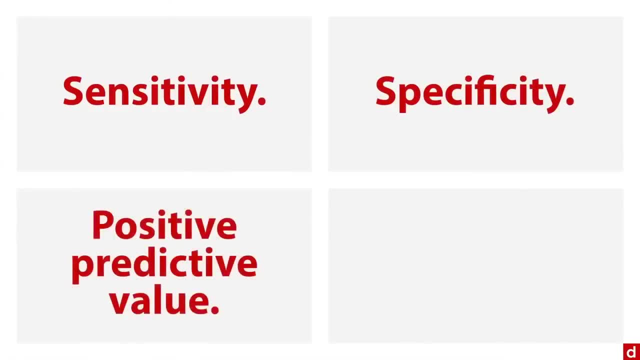 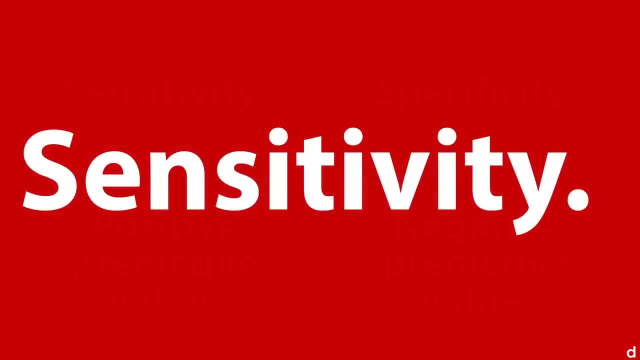 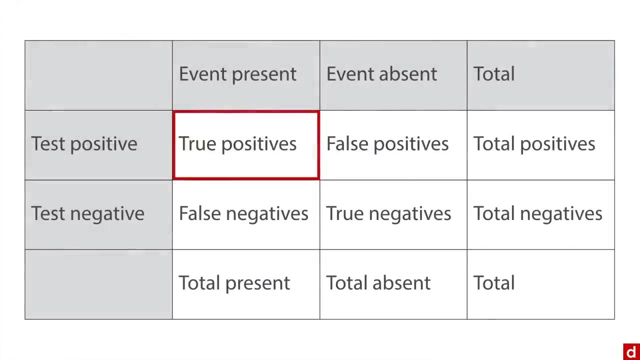 positive predictive value and negative predictive value. I'll show you very briefly how each of them works. Sensitivity can be expressed this way: If there's a fire, does the alarm ring? you want that to happen, And so that's a matter of looking at the true positives. 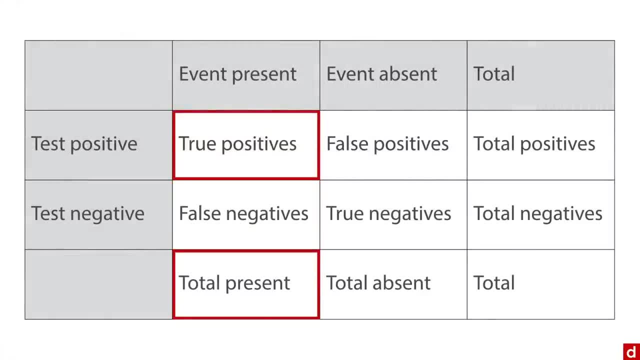 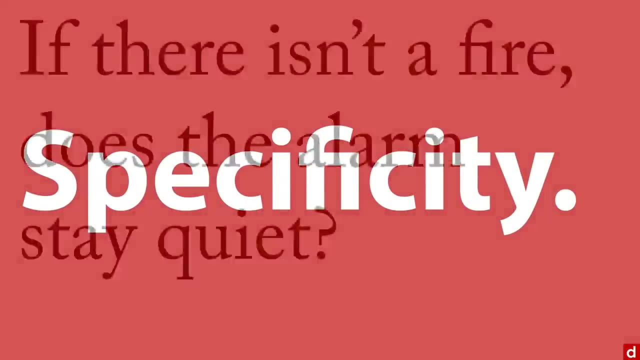 and dividing that by the total number of alarms. So the test positive means there's an alarm and the event present means there's a fire. you want to always to have an alarm when they're there's a fire. Specificity, on the other hand, is sort of the flip side of this. If there isn't a 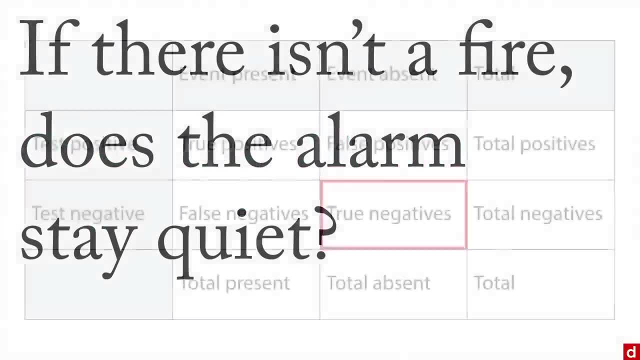 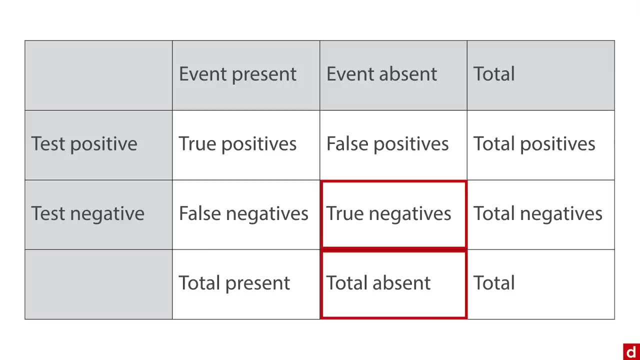 fire. does the alarm stay quiet? This is where you're looking at the ratio of true negatives to total absent events, where there's no fire and the alarms aren't ringing, And that's what you want. Now, those are looking at columns. you can also go sideways across rows. So the first one: 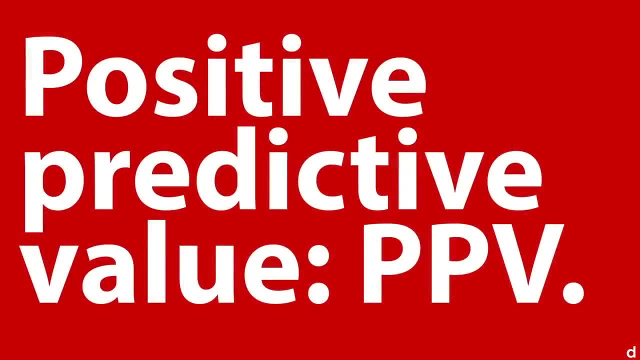 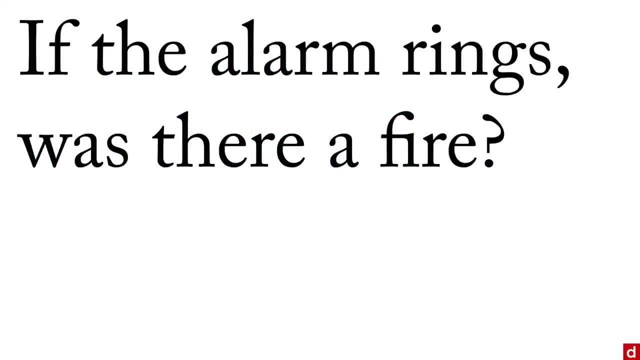 there is positive predictive value, often just abbreviated as PPV, And we flip around the order a little bit. this one says: if the alarm rings was there a fire. So now you're looking at the true positives and dividing it by the total number. 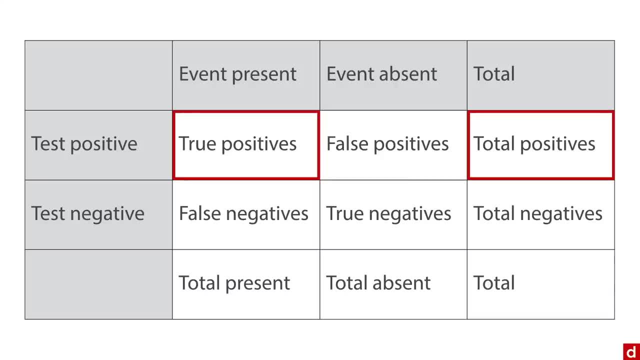 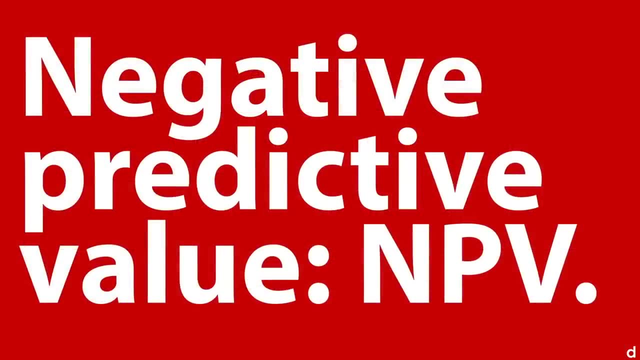 of positives. total number of positives is: anytime the alarm rings. true positives is because there was a fire, and negative predictive value, or Npv, says: if the alarm doesn't ring, does that in fact mean that there is no fire. Well, here you list. 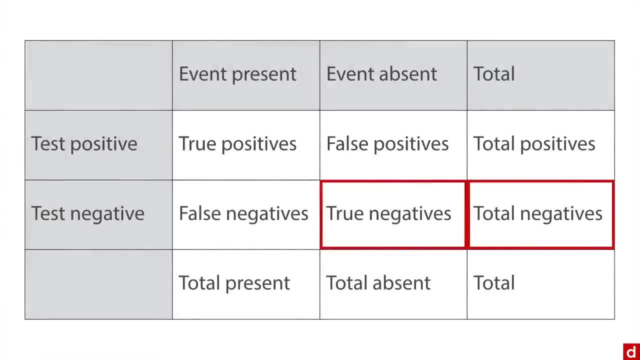 at true negatives and dividing it by total negatives, the time that it doesn't ring. And again, you want to maximize that. so the true negatives account for all of the negatives. the same way, you want the true positives to account for all of the positives, and so on. Now you can. 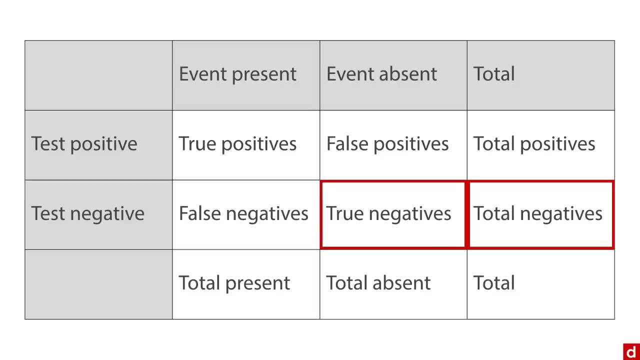 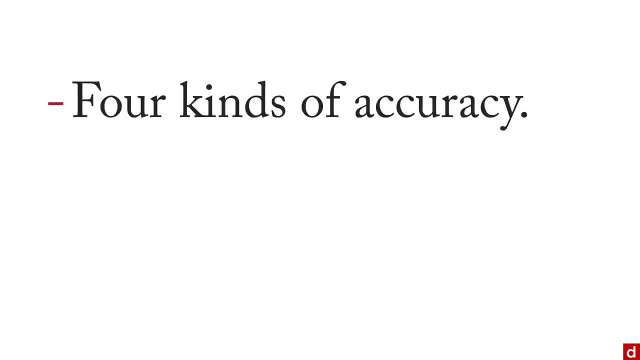 put numbers on all of these, going from 0% to 100%, And the idea is to maximize each one as much as you can. So, in sum, from these tables we get four kinds of accuracy and there's a different focus for each one, But the same overall goal. you want to identify the true positives and true negatives. 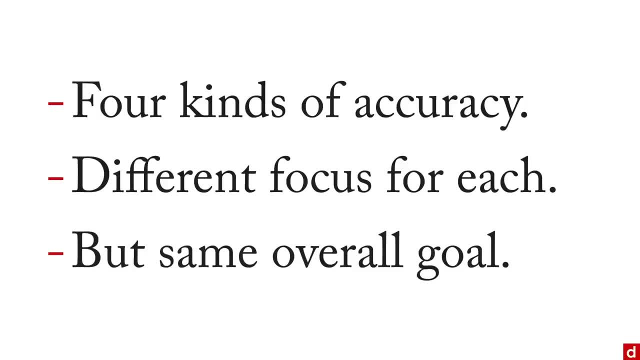 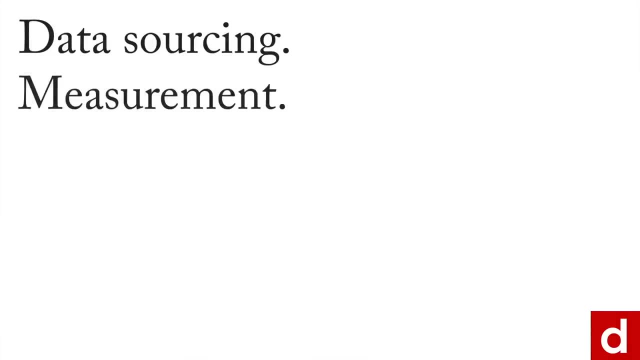 and avoid the false positives and false negatives, And this is one way of putting numbers on an index, really on the accuracy of your measurement. Now, data sourcing may seem like a very quantitative topic, especially when we're talking about measurement, But I want to measure one important thing here, And that is the social 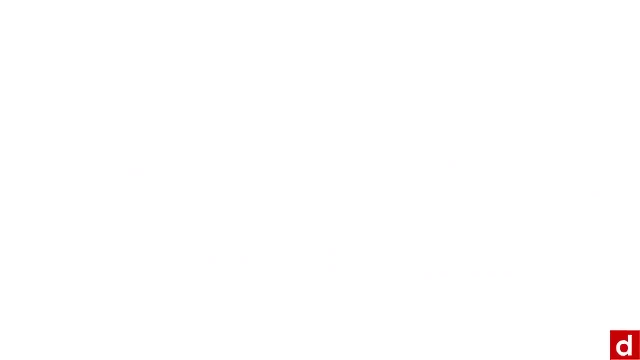 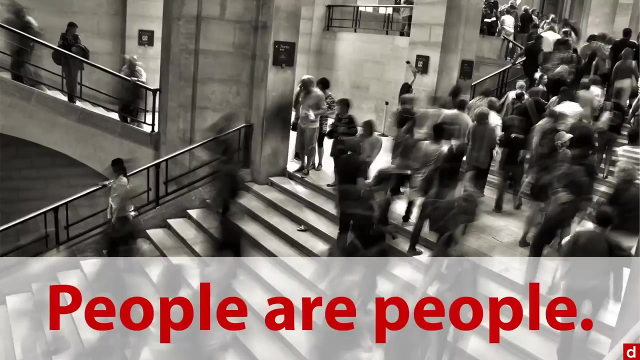 context of measurement. The idea here really is that people are people and they all have their own goals and they're going their own ways, And we all have our own thoughts and feelings that don't always coincide with each other, And this can affect measurement. And so, for instance, 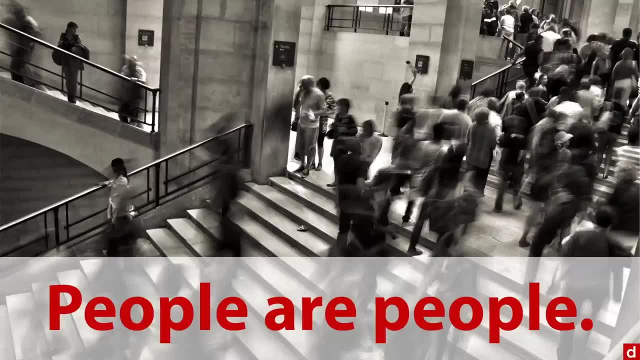 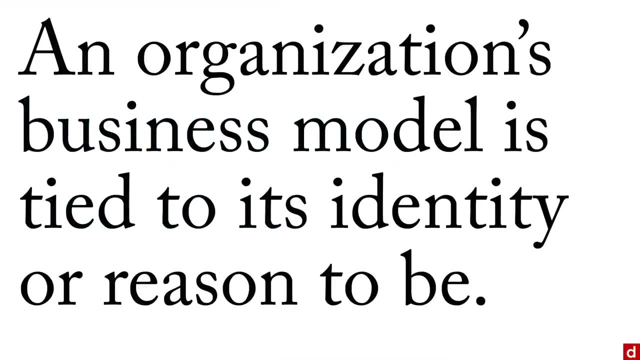 when you're trying to define your goals and you're trying to maximize them, you want to look at things like, for instance, the business model. an organization's business model- the way they conduct their business, the way they make their money- is tied to its identity. 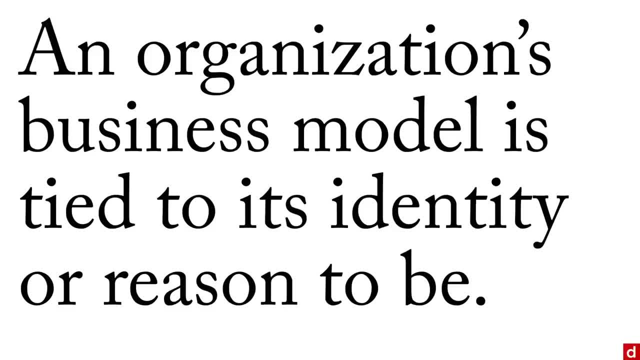 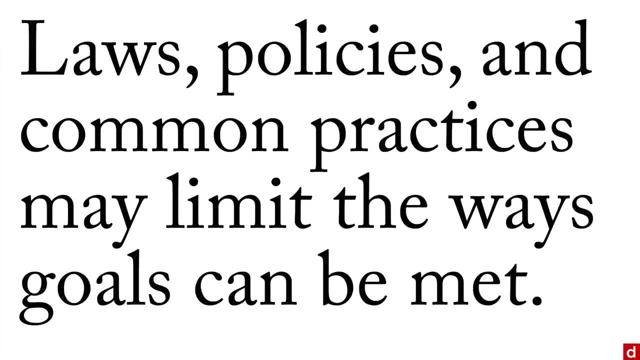 And it's reason to be. And if you make a recommendation that's contrary to their business model, that can actually be perceived as a threat to their core identity And people tend to get freaked out in that situation. Also, restrictions: So, for instance, there may be laws, policies and common practices, both organizationally. 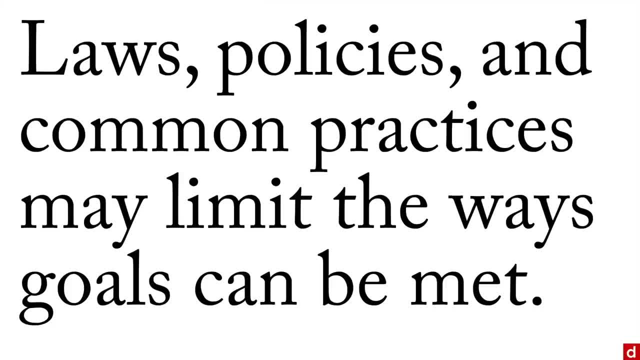 and culturally. that may limit the ways that goals can be met. Now, most of these make a lot of sense. So the idea is: you can't just do anything you want. You need to have these constraints, And when you make your recommendations, maybe you'll work creatively in them, as long as 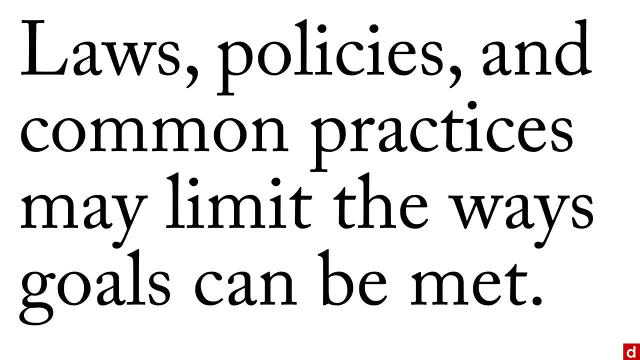 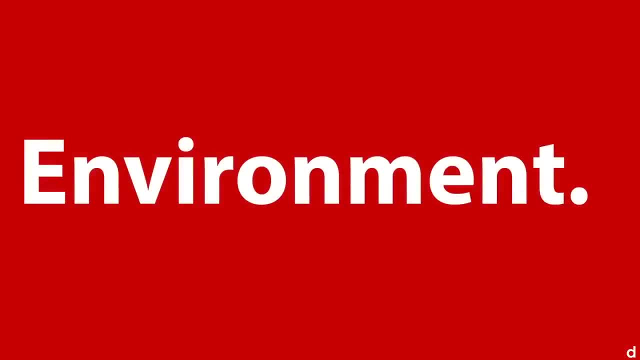 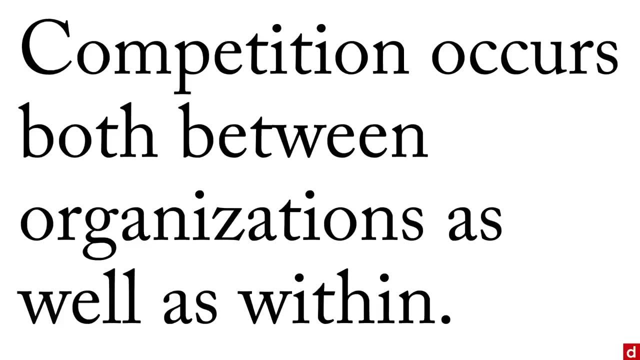 you're still behaving legally and ethically, But you do need to be aware of these constraints. Next is the environment, And the idea here is that competition occurs both between organizations. that company here is trying to reach a goal, but they're competing with company B over there. 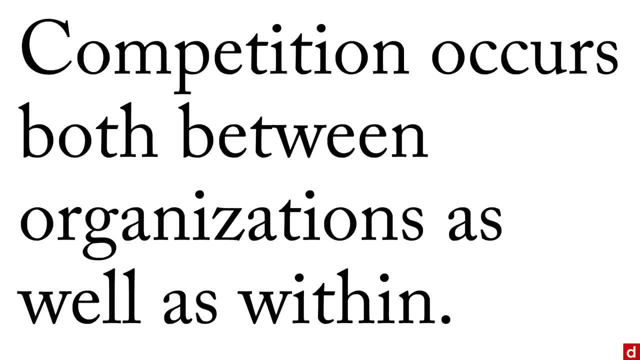 But probably even more significantly, there is competition within the organization. This is really a recognition of- Okay, I'm going to do this. This is really a recognition of office politics and that when you, as a consultant, make a recommendation based on your analysis, you need to understand you're kind of dropping a little football. 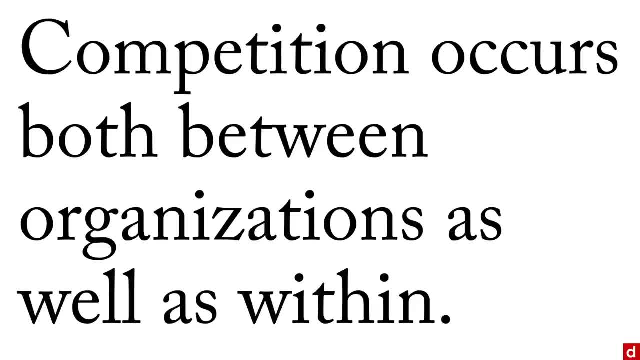 into the office and things are going to further- one person's career maybe to the detriment of another, And in order for your recommendations to have the maximum effectiveness, they need to play out well in the office. That's something that you need to be aware of as you're making your recommendations. 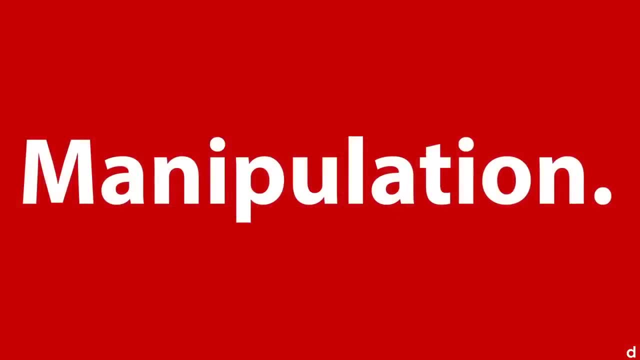 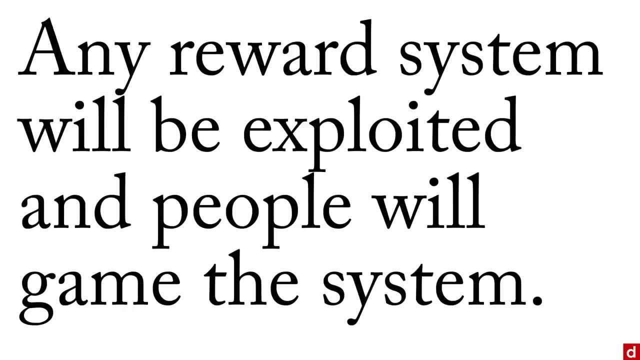 Finally, there's the issue of manipulation, And a sad truism about people is that any reward system, any reward system at all, will be exploited and people will generally game the system. This happens especially when you have a strong cutoff. you need to get at least 80% or you. 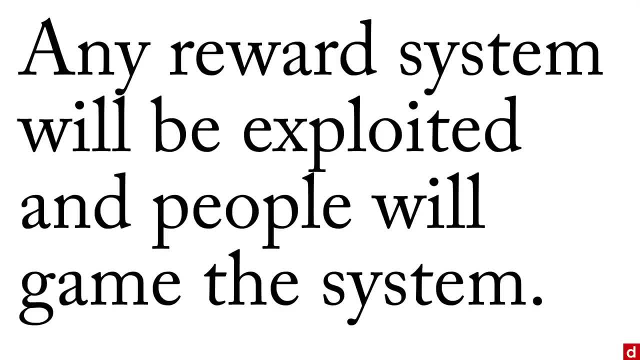 get fired And people will do anything to make their numbers appear to be 80%. This happens an awful lot when you look at executive compensation systems. it looks a lot when you have very high stakes school testing. It happens. It happens in an enormous number of situations. 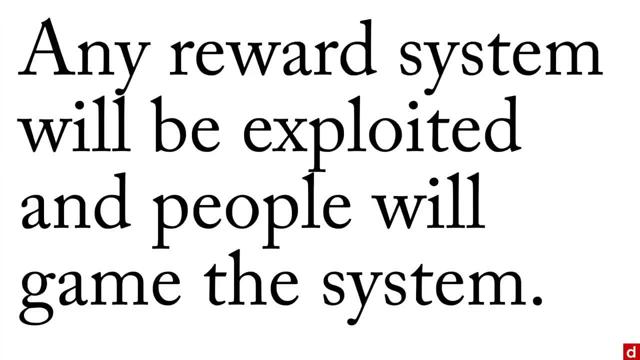 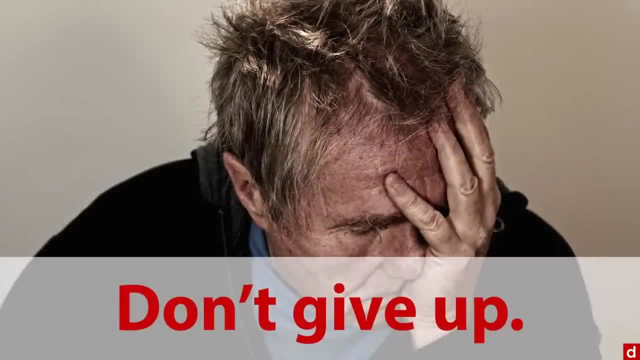 And so you need to be aware of the risk of exploitation and gaming. Now don't think, then, that all is lost. Don't give up. You can still do really wonderful assessment. you can get good metrics. just be aware of these particular issues and be sensitive to them as you both conduct your research and 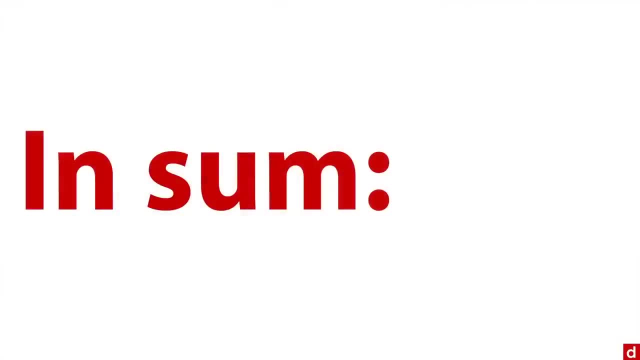 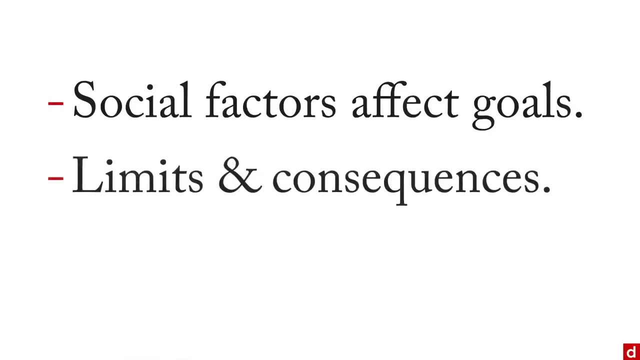 as you make your recommendations. So, in sum, social factors affect goals and they affect the way that you meet those goals. There are limits and consequences both on how you reach the goals and how really what the goal should be, And that, when you're making advice on how to reach those goals, please be sensitive. 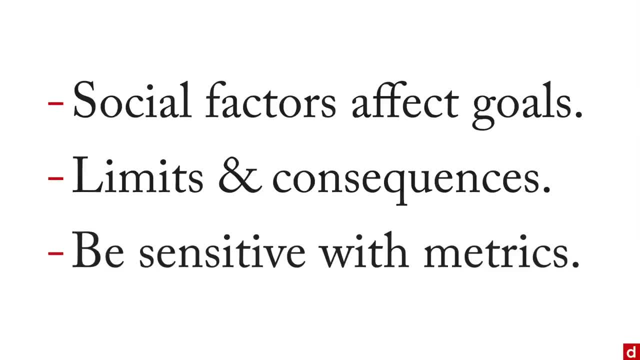 to how things play out with metrics and how people will adapt their behavior to meet the goals. That way you can make something that's more likely to be implemented the way you meant and more likely to predict accurately what can happen with your goals. 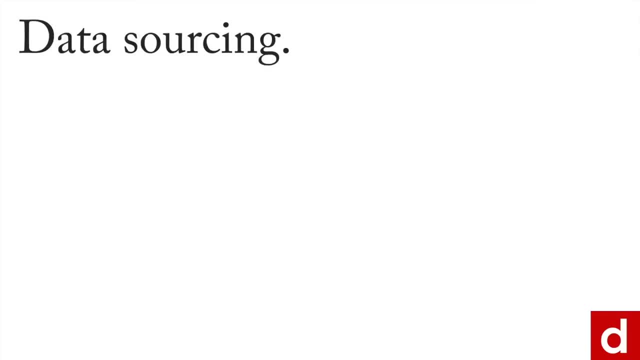 When it comes to data, When it comes to data sourcing, obviously, the most important thing is to get data, But the easiest way to do that, at least in theory, is to use existing data. Think of it as going to the bookshelf and getting the data that you have right there. 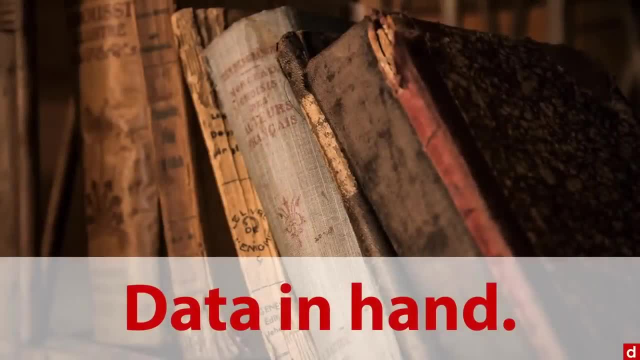 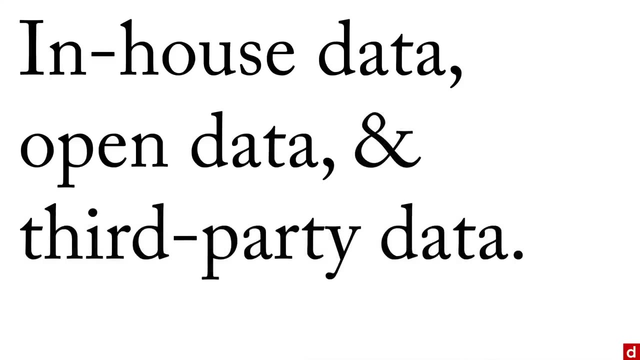 at hand. Now, there's a few different ways to do this. You can get in-house data, you can get open data and you can get third party data. Another nice way to think of that is proprietary public and purchased data. 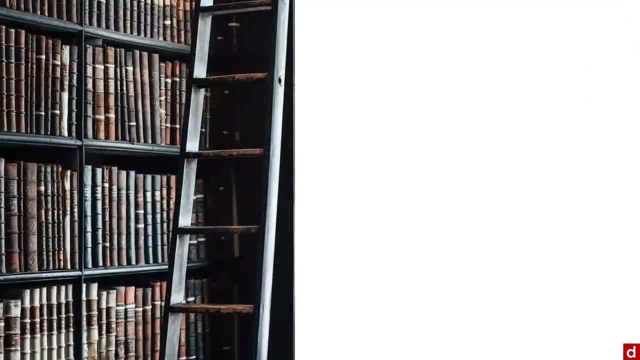 The three P's I've heard it called. Let's talk about each of these a little bit more. So, in-house data: that's stuff that's already in your organization. What's nice about that is it can be really fast and easy. 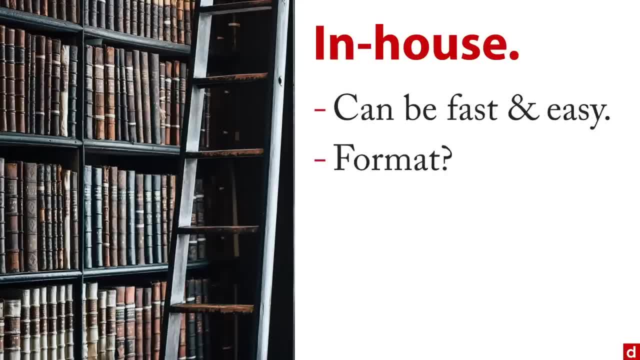 It's right there And the format may be appropriate for the kind of software and the computer that you're using. If you're fortunate, there's good documentation, although sometimes, when it's in-house, people just kind of throw it together. So you have to watch out for that. 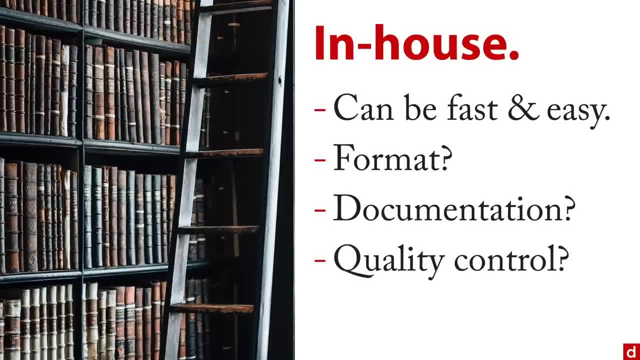 And there's the issue of quality control. Now You can get in-house data, but you need to pay attention with in-house because you don't know the circumstances necessarily under which people gathered the data and how much attention they were paying to something. 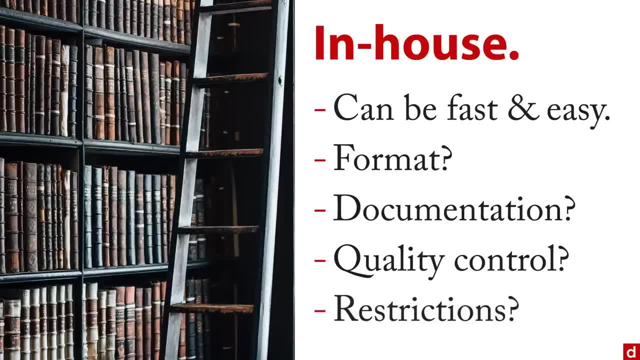 There's also an issue of restrictions. There may be some data that, while it's in-house, you may not be allowed to use, or you may not be able to publish the results or share the results with other people. So these are things that you need to think about when you're going to use in-house data. 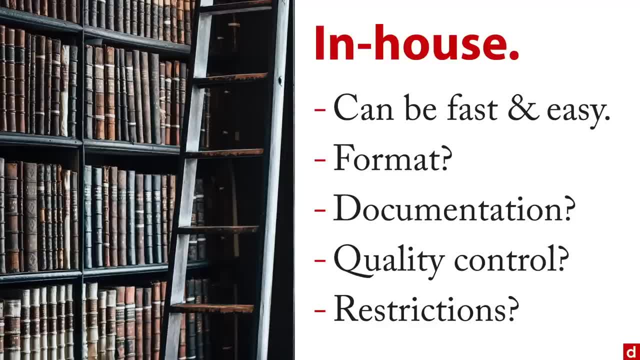 in terms of how can you use it to facilitate your data science work. So that's a great question. Thank you. I'm sure there's a lot of work to be done to be able to use in-house data in a more efficient way. 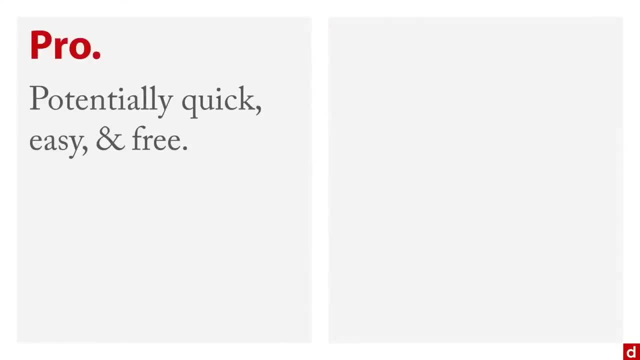 And that's why we're going to talk a little bit more about that in a second. Let's get into this. What are the pros and cons of in-house data in the data science project? So what are the pros and cons? So in-house data- potentially quick, easy, free- hopefully- is standardized. 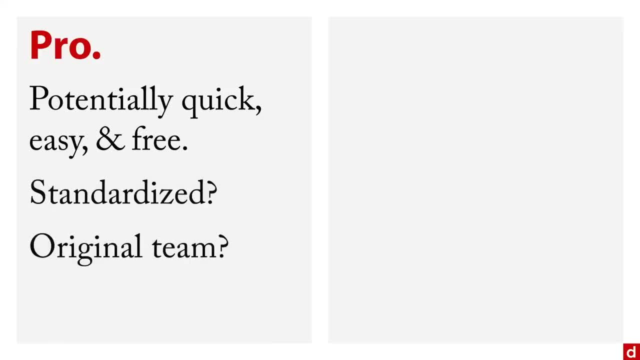 Maybe even the original team that conducted this study is still there. You might have identifiers in the data which make it easier for you to do an individual level analysis. On the cons side, however, the in-house data simply may not exist. Maybe it's just not there. 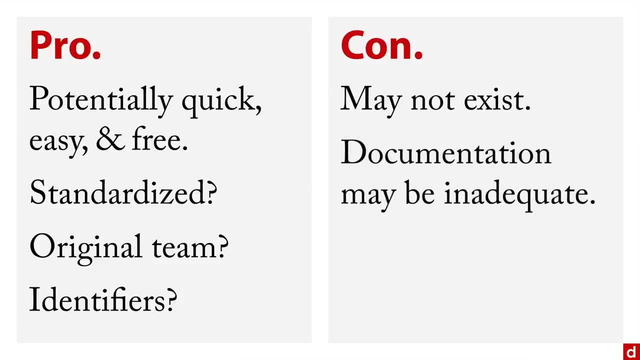 Or the documentation may be inadequate And, of course, the quality may be uncertain- always true, but maybe something you have to pay more attention to when you're using in house data. Now, another choice is open data, like going to the library and 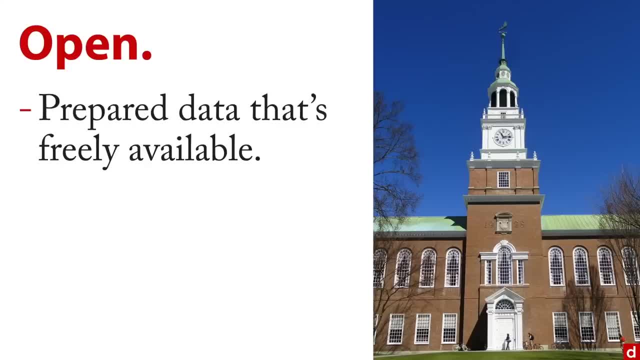 getting something. This is prepared data that's freely available consists of things like government data and corporate data and scientific data from a number of sources. Let me show you some of my favorite open data sources, just so you know where they are and that they exist- Probably the best. 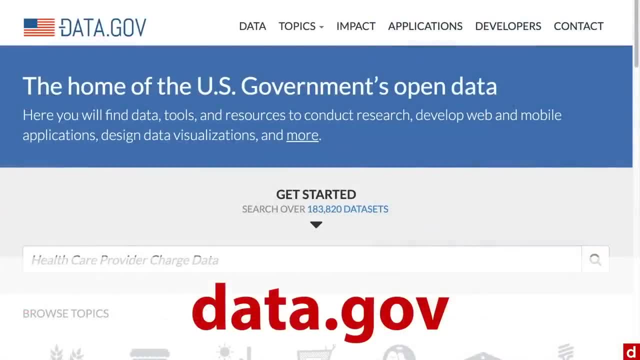 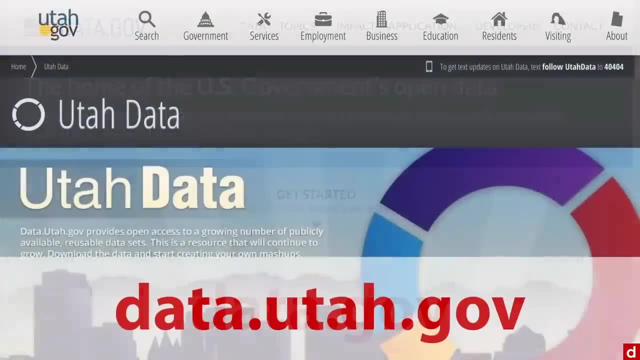 one is datagov here in the US- That is the it says right here- the home of the US government's open data. Or you may have a state level one. For instance, I'm in Utah and we have datautahgov. 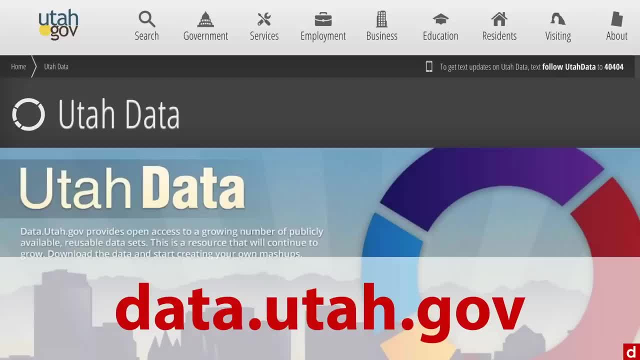 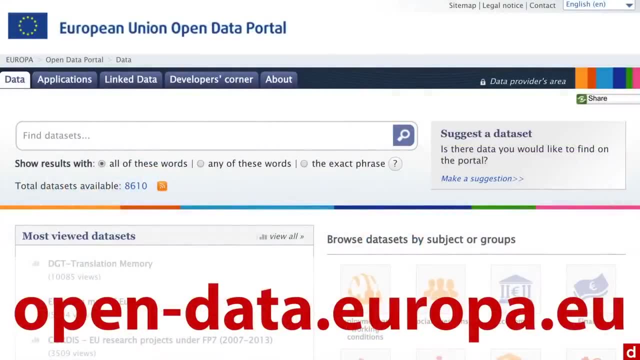 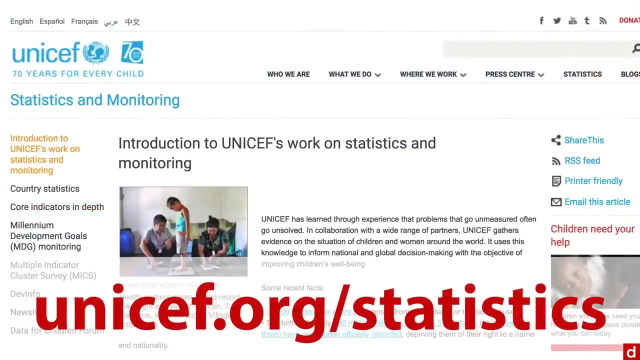 also a great source of more regional information. If you're in Europe, you have open-dataeuropaeu, the European Union Open Data, And then there are major nonprofit organizations. So the UN has uniceforg slash statistics for their statistical and monitoring data. The World Health Organization- 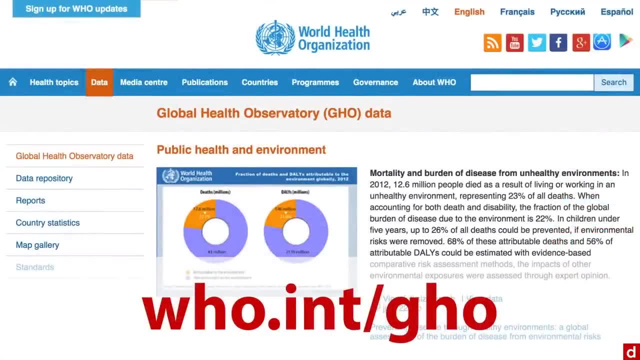 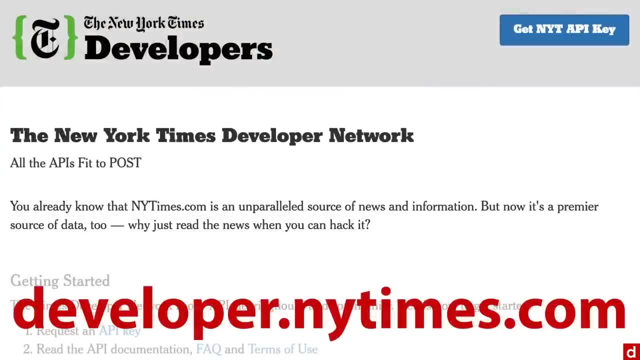 has the Global Health Observatory at whoint slash gho. And then there are private organizations that work in the public interest, such as the Pew Research Center, which shares a lot of its datasets, and the New York Times, Which makes it possible to use APIs to access a huge amount of the data of things they've published. 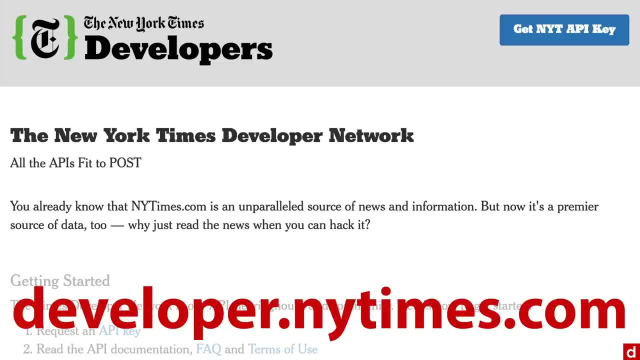 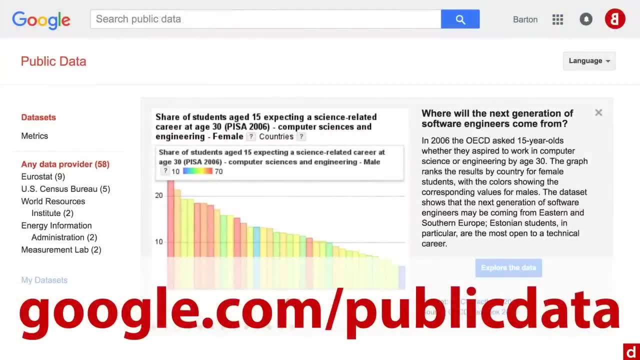 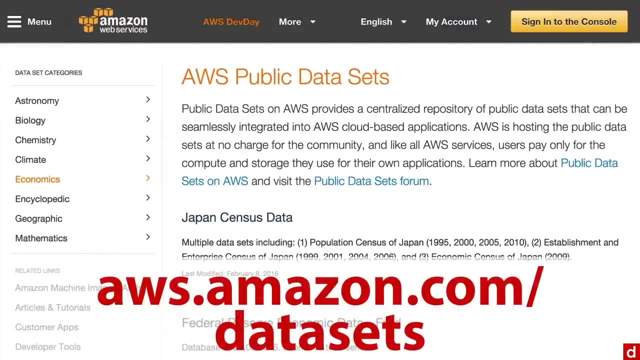 over a huge time span, And then two of the mother loads. there's Google, which, at googlecom, has public data, which is a wonderful thing, And then Amazon, at awsamazoncom datasets, has gargantuan datasets. So if you needed a dataset that was like five terabytes in size, this is the place. 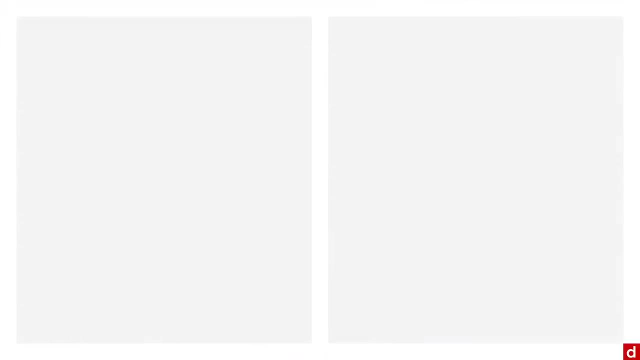 you would go to get it. There are some pros and cons to using this kind of open data. First is that you can get very valuable datasets that maybe cost millions of dollars to gather and to process, And you can get a very wide range of topics and times and groups of people and so on, And often 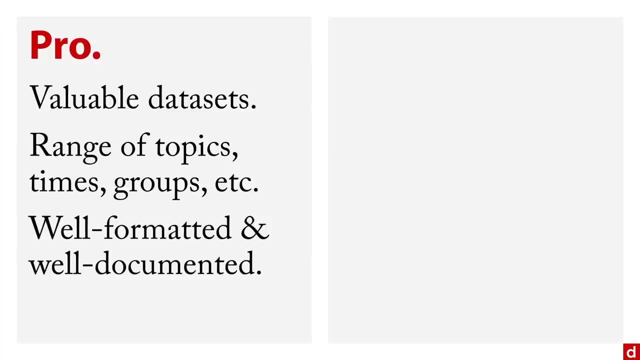 the data is very well formatted and well documented. There are, however, a few cons. Sometimes there's. by a sample, say, for instance, you only get people who have internet access and that can mean, you know, not everybody. Sometimes the meaning of the data is not clear or it may not mean exactly what you. 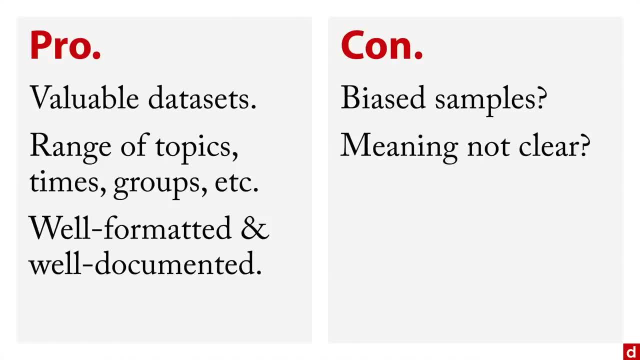 want it to. A potential problem is that sometimes you may need to share your analyses, And if you're doing proprietary research, well, it's gonna have to be open research instead, And so that can create a cramp with some of your clients. And then, finally, there are issues. 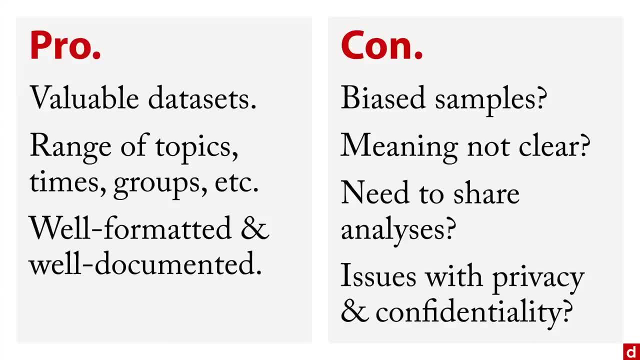 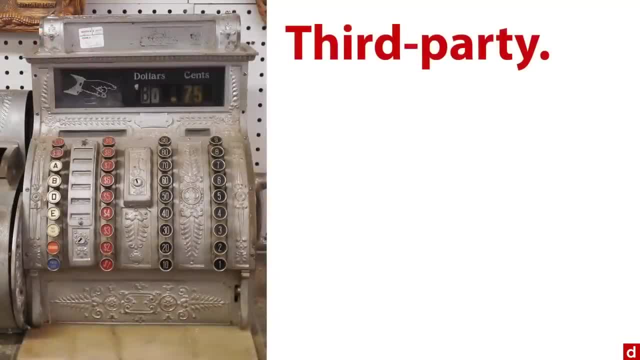 with privacy and confidentiality, And in public data that usually means that the identifiers are not there And you're gonna have to work at a larger aggregate level of measurement. Another option is to use data from a third party. These go by the name data as a service. 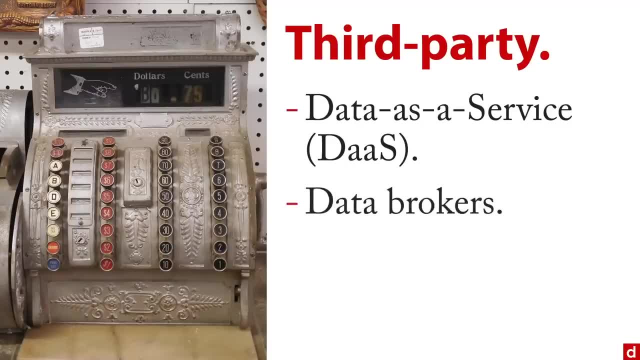 or DAS. You can also call them data brokers, And the thing about data brokers is they can give you an enormous amount of data on many different topics. Plus, they can save you some time and effort by actually doing some of the processing for you, And that can include 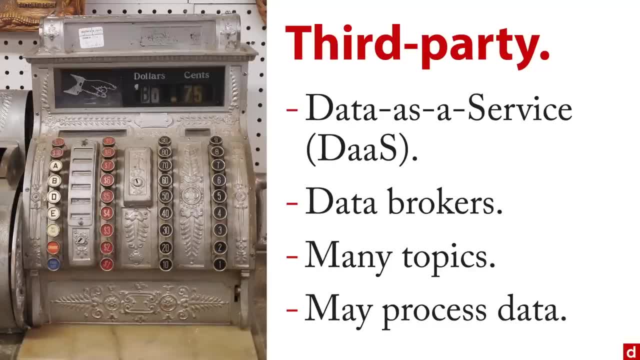 things like consumer behaviors and preferences. they can get contact information. they can do marketing, identity and finances. there's a lot of things. There's a number of data brokers around. Here's a few of them. Axiom is probably the biggest one. 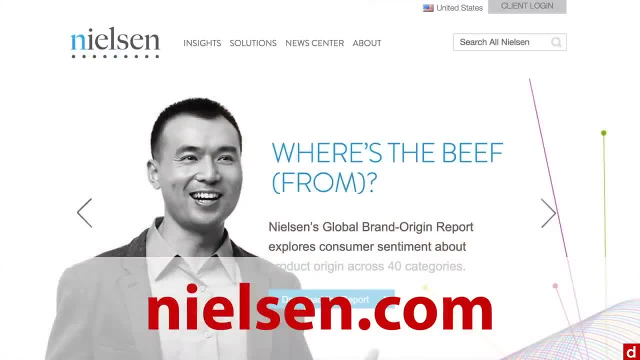 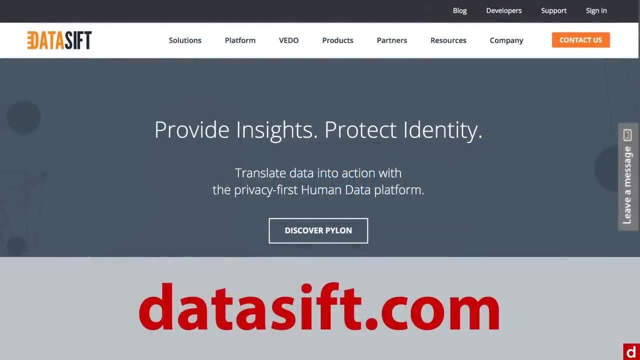 in terms of marketing data. There's also Nielsen, which provides data primarily for media consumption, And there's another organization, data sift. That's a smaller, newer one, And there's a pretty wide range of choices, But these are some of the big ones. Now the thing about 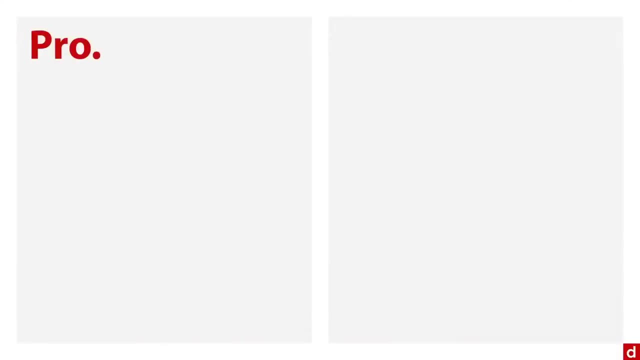 using data brokers. there's some pros and there's some cons. The pros are, first, that it can save you a lot of time and effort. And then, finally, there are some pros and there are some cons. The pros are, first, that it can save you a lot of time and effort. 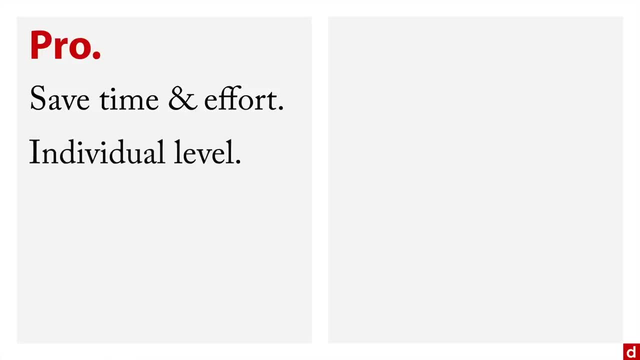 It can also give you individual level data which can be hard to get from open data. Open data is usually at the community level. They can give you information about specific consumers. They can even give you summaries and inferences about things like credit scores and marital 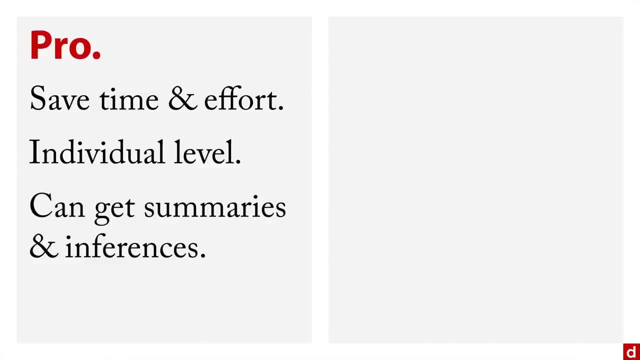 status, possibly even whether a person gambles or smokes. Now, the con is this Number one: it can be really expensive. I mean, this is a huge service, it provides a lot of benefit and it's priced accordingly. Also, you still need to validate it. You still need to double check that it means what. 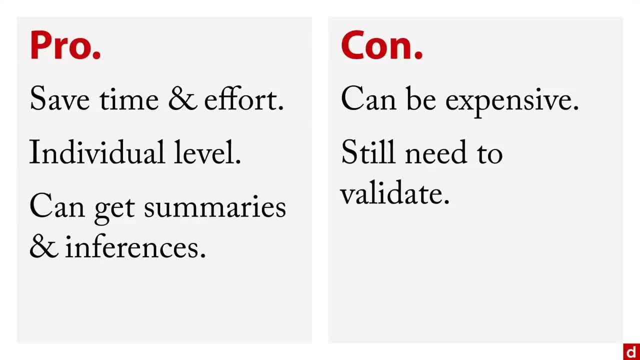 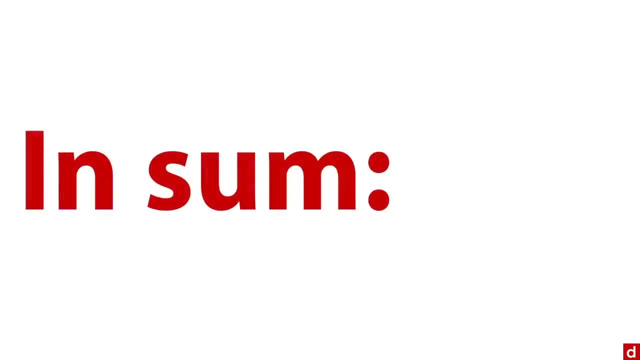 you think it means and that it works in with what you want. And probably a real sticking point here is the use of third party data is distasteful to many people, And so you have to be aware of that as you're making your choices. So, in sum, as far as data sourcing, 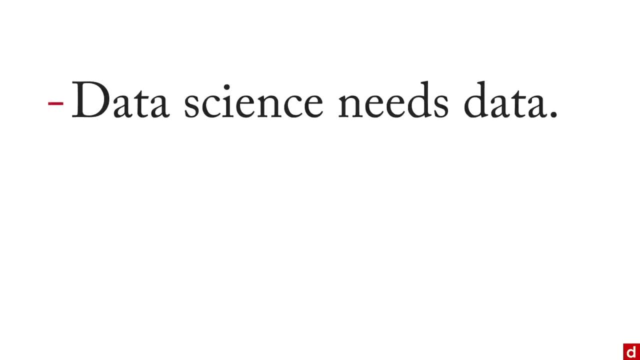 existing data goes. obviously, data science needs data And there's the three Ps of data sources. There's proprietary and public and purchase. But no matter what source you use, you need to pay attention to quality, into the meaning and the usability of the data to help you. 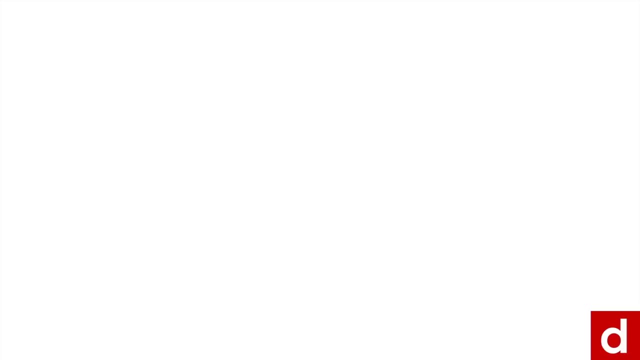 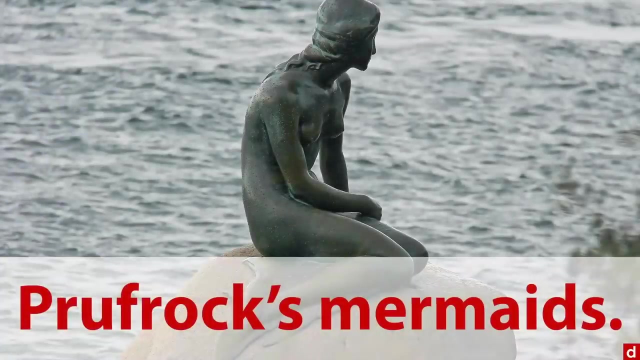 along in your own projects. When it comes to data sourcing, a really good way of getting data is to use what are called API's. Now, I like to think of these as the digital version of proof rocks mermaids. If you're familiar with the love song of J alpha, proof rock by 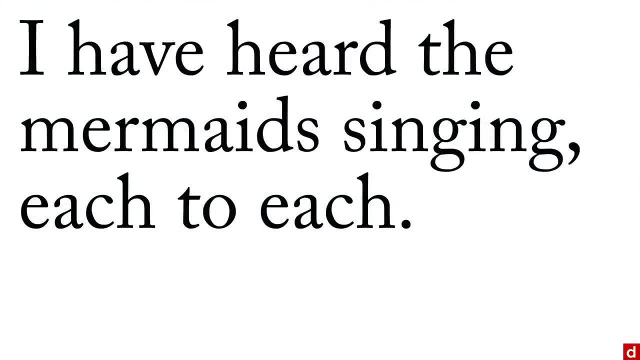 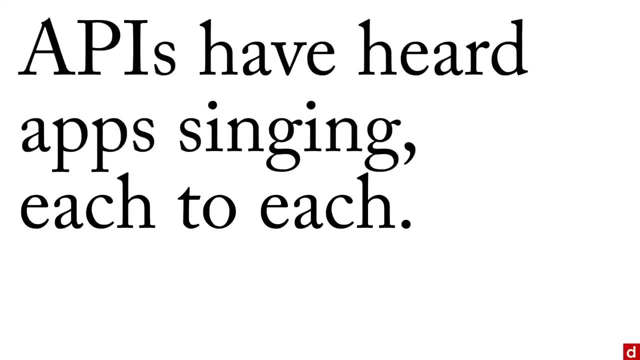 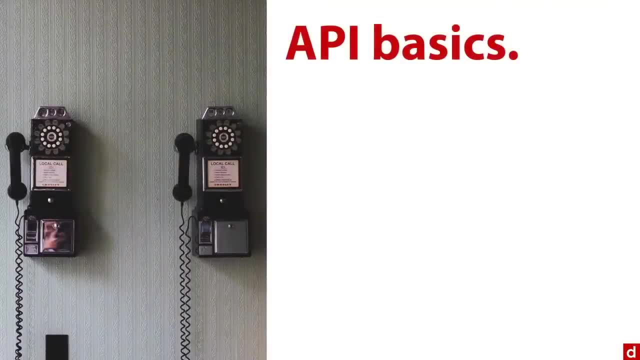 Elliott. He says: I have heard the mermaids singing each to each. that's TS Eliot, And I like to adapt that to say: API's- have heard apps singing each to each, And that's by me. Now, more specifically, when we talk about an API, what we're talking about is something 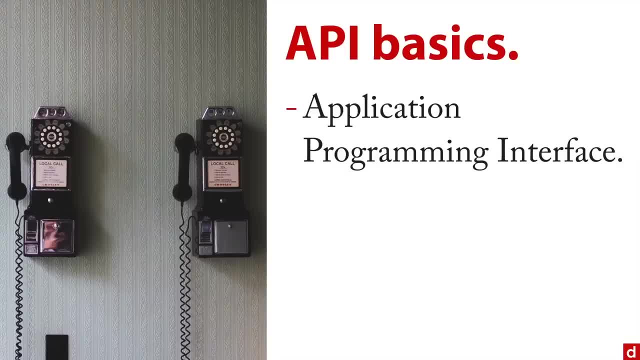 called an application programming interface, And this is something that allows programs to talk to each other. It's most important use in terms of data science is it allows you to get web data. It allows you to get, So in data science, you need to have a huge database, The only. 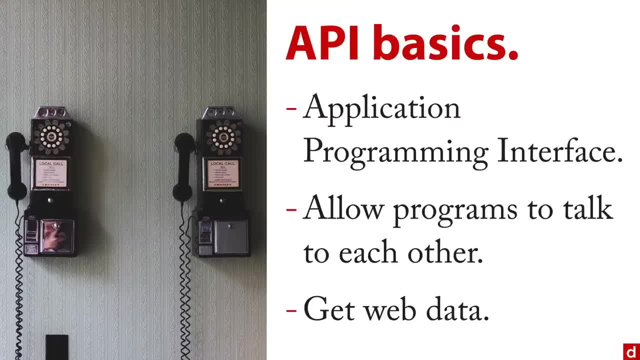 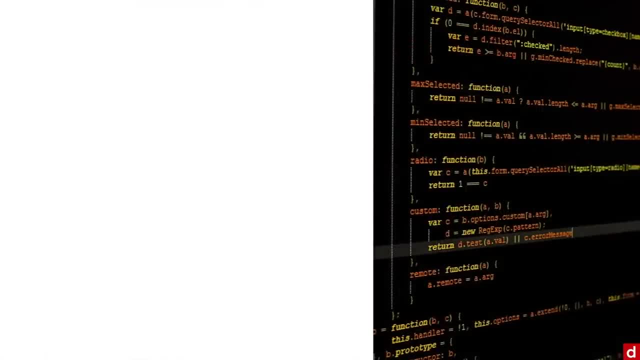 program to directly go to the web on its own, grab the data, bring it back in almost as though it were local data, And that's a really wonderful thing. Now, the most common version of APIs for data science are called REST APIs. That stands for representational state transfer. That's the 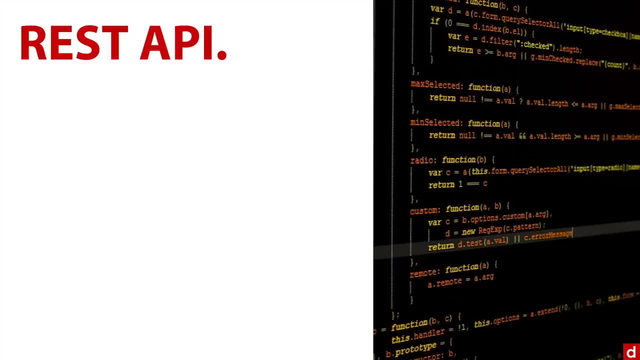 software architectural style of the World Wide Web, And it allows you to access data on web pages via HTTP. That's the hypertext transfer protocol that you know runs the web as we know it, And when you download the data, you usually get it in JSON format that stands for JavaScript object. 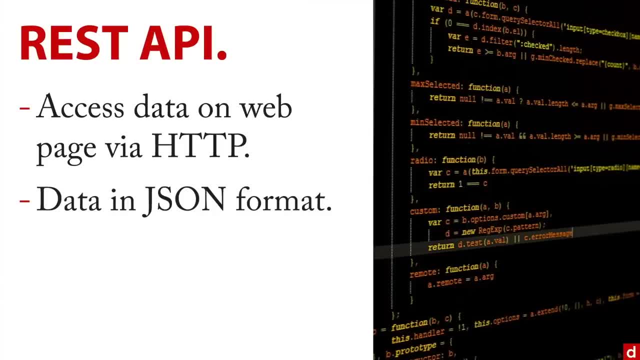 notation. The nice thing about that is that's human readable, but it's even better for machines. Then you can take that information and you can send it directly to other programs. And the nice thing about REST APIs is that they're what's called language agnostic, meaning any program. 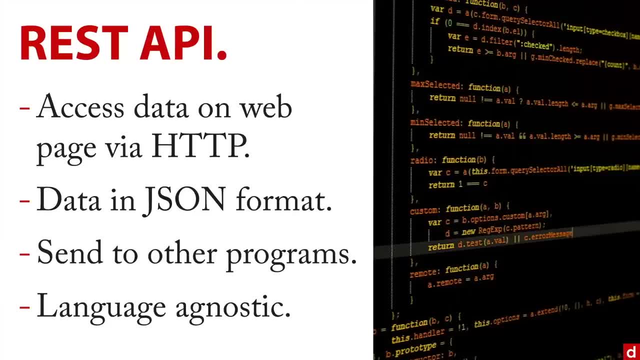 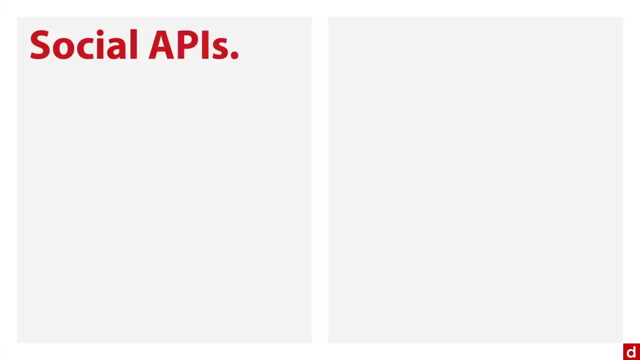 programming language can call a REST API, can get data from the web and can do whatever it needs to with it. Now there are a few kinds of API's that are really common. The first is what are called social API's. These are ways of interfacing with social networks. So, for instance, the most common 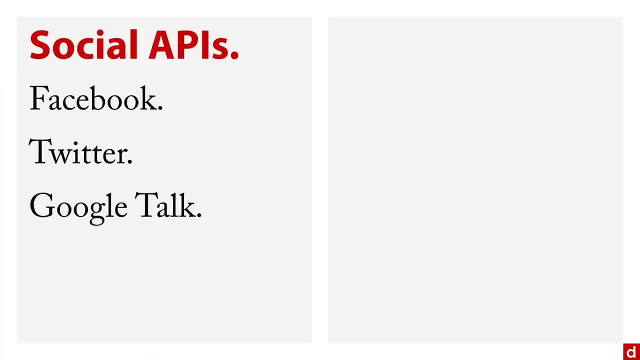 is Facebook. there's also Twitter, Google Talk has been a big one, and Foursquare as well, And then SoundCloud. these are on lists of the most popular ones. And then there are also what are called visual API's, which are for getting data, And then there are also the most popular ones, which are: 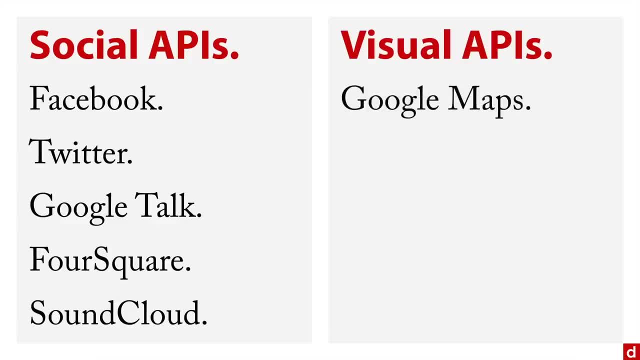 visual data. So, for instance, Google Maps is the most common, But YouTube- something that accesses YouTube on a particular website- or AccuWeather, which is for getting weather information, Pinterest for photos and Flickr for photos as well. So these are some really common API's. 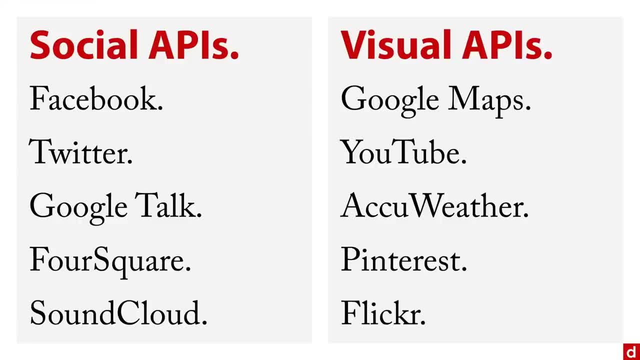 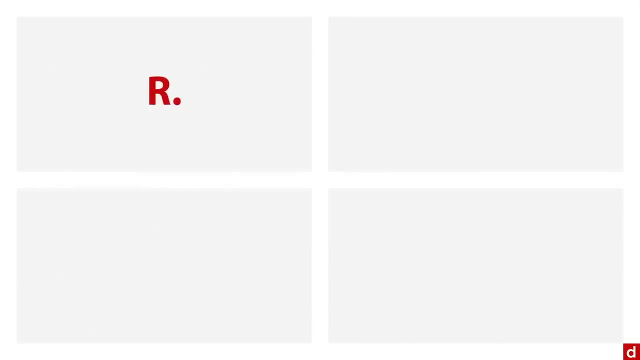 and you can program your computer to pull in data from any of these services and sites and integrate it into your own website or, here, into your own data analysis. Now, there's a few different ways you can do this. You can program it in our the statistical 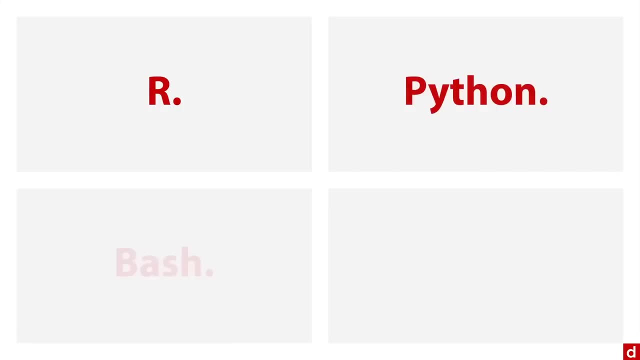 programming language. you can do it in Python. Also, you can even do it in the very basic bash command line interface, And there's a ton of other applications. basically, anything can access an API one way or another. Now I'd like to show you how this works in our, so I'm going to open up a script. 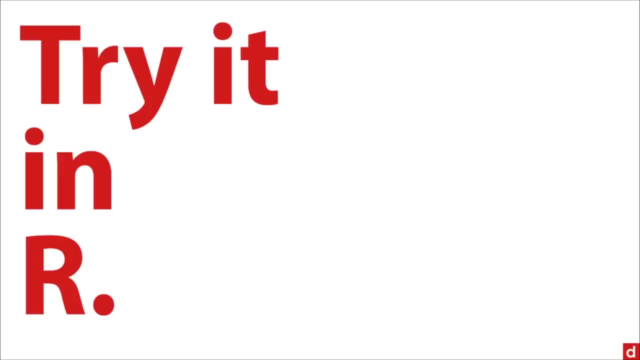 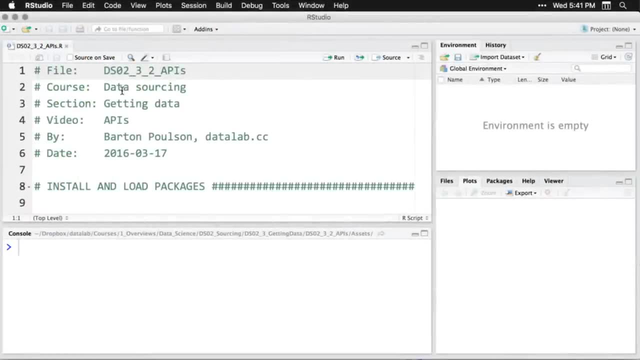 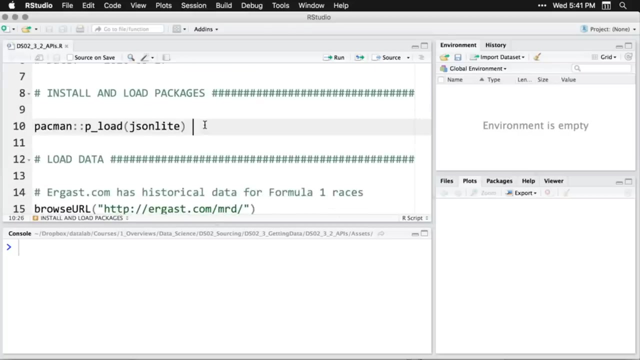 in our studio And then I'm going to use it to get some very basic information from a web page. Let me show you how this works. I've opened up a script in our studio that allows me to do some data sourcing here. Now I'm just going to use a package called JSON light. I'm going to load. 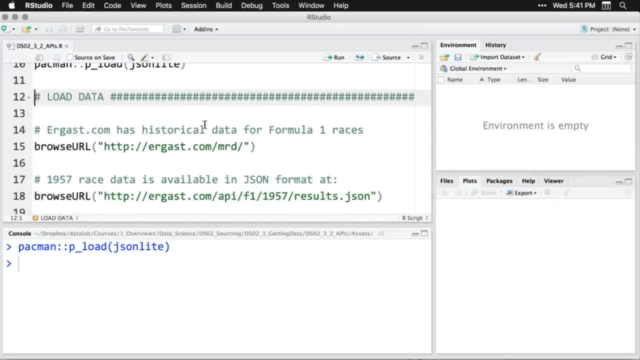 that one up, And then I'm going to go to a couple of websites. I'm going to be getting historical data from Formula One car races And I'm going to be getting it from airgascom. Now, if we go to this page right here, I can just go straight to my browser right now And 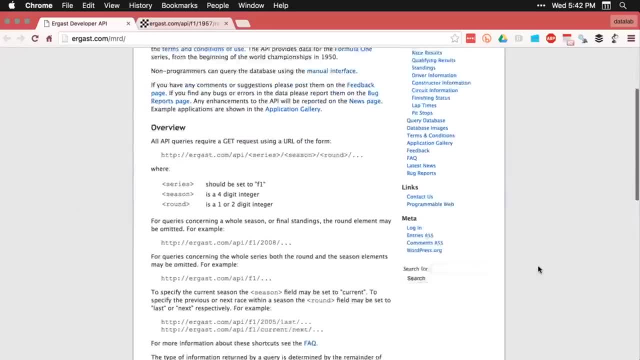 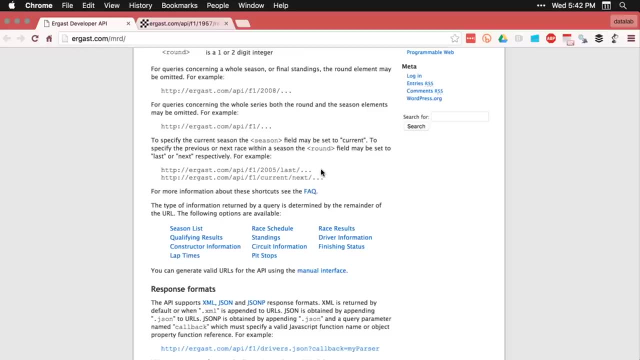 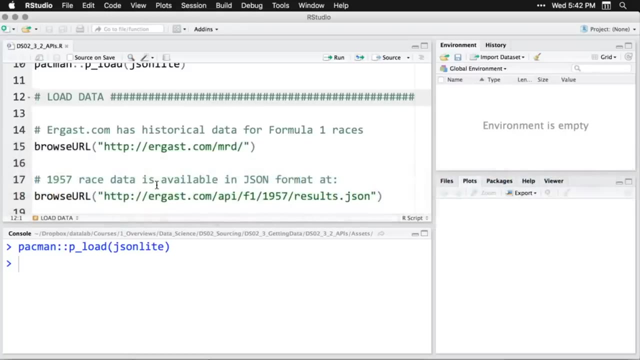 this is what it looks like. it gives you the API documentation. So what you're doing for an API is you're just entering a web address And in that web address it includes the information that you want. I'll go back to our here for a second, And if I want to get information about 1957 races in 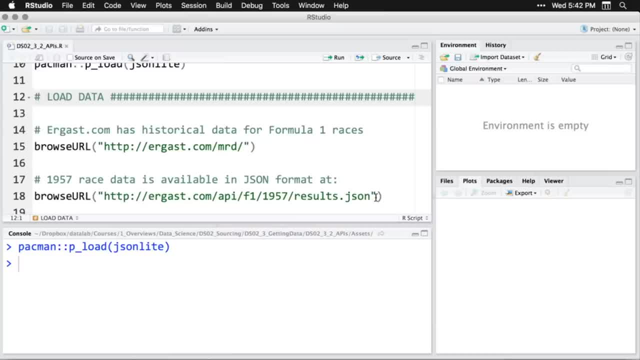 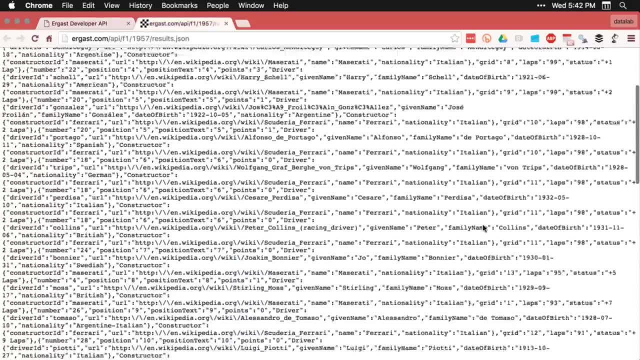 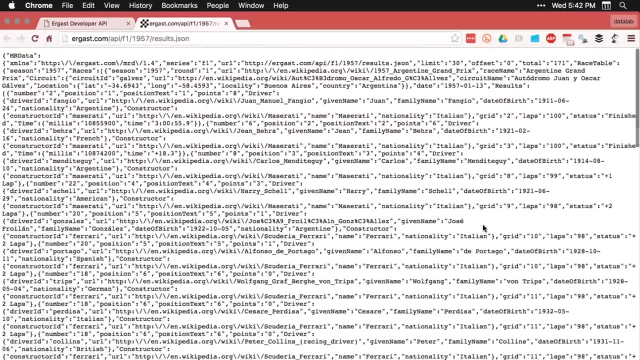 JSON format. I go to this address- I can skip over to that for a second- And what you see is it's kind of a mess here, But it is all labeled and it's clear to the computer what's going on here. I'll 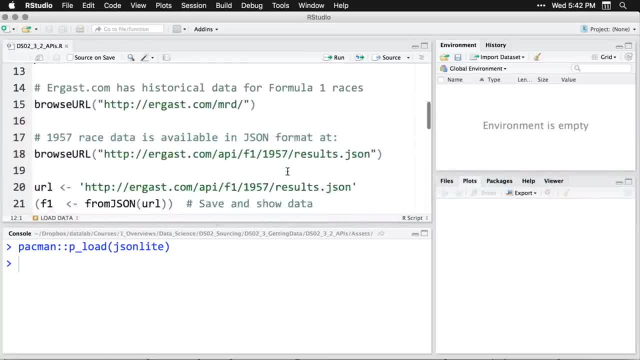 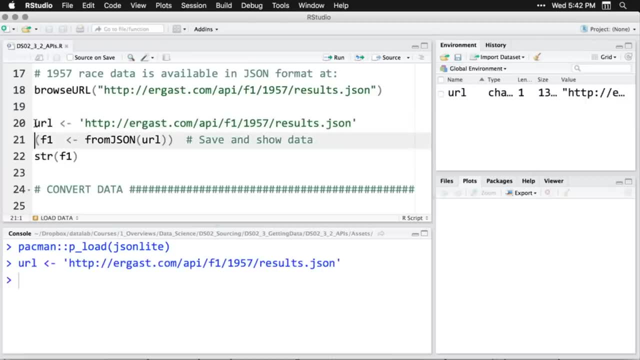 go back to our, And so what I'm going to do is I'm going to save that URL into an object here in R And then I'm going to use the command from JSON to read that URL and save it into our, and which it. 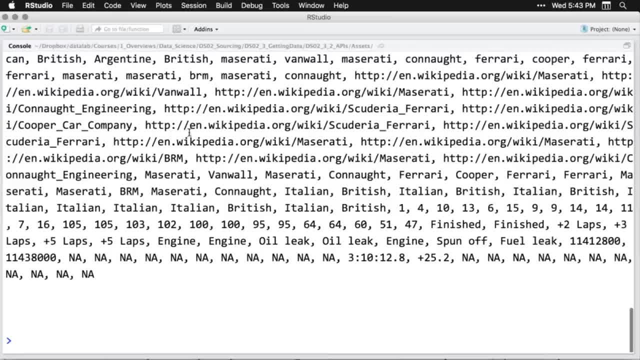 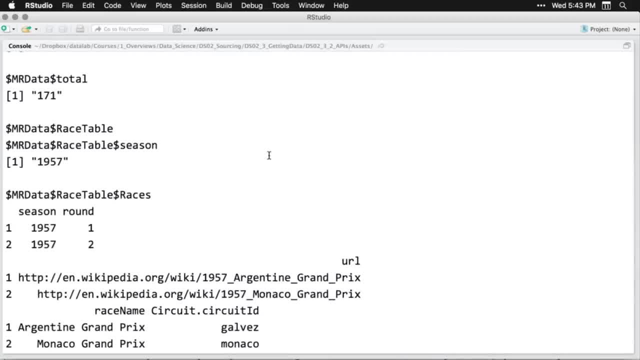 is now done And I'm going to zoom in on that So you can see what's happened. I've got this sort of mess of text, Actually a list object in R, And then I'm going to get just the structure of that object. So I'm 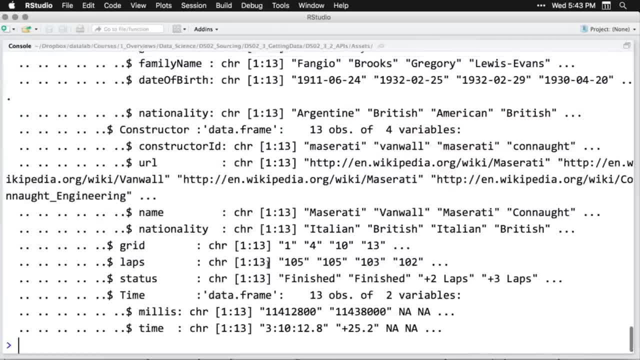 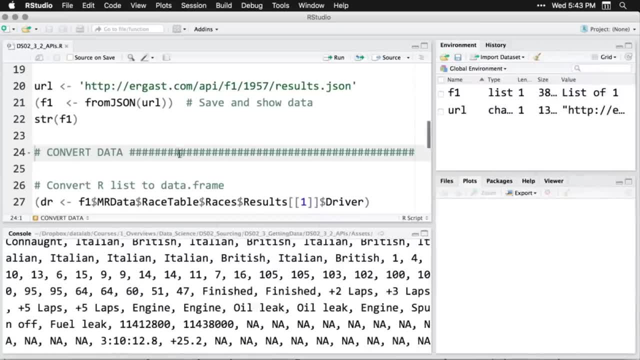 going to do this one right here And you can see that it's a list and it gives you the names of all the variables within each one of the lists, And what I'm going to do is I'm going to convert that list to a data frame by. I went through the list and found exactly where the information I wanted. 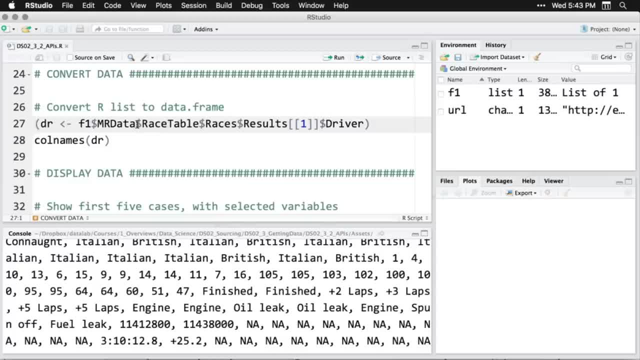 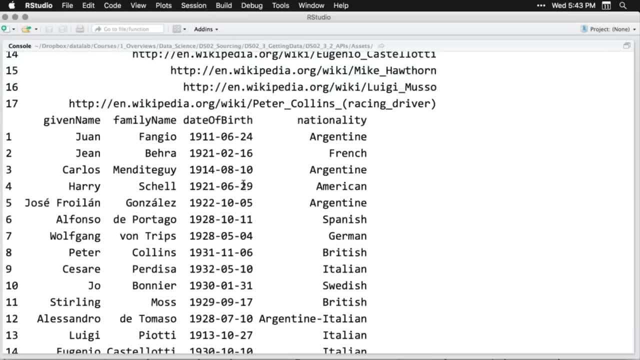 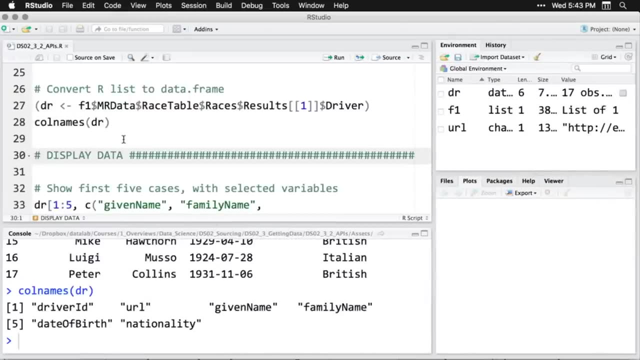 was located. you have to use this big long statement here. That'll give me the names of the drivers. Let me zoom in on that again. There they are, And then I'm going to get just the column names for that bit of the data frame. And so what I have here is six different variables And then 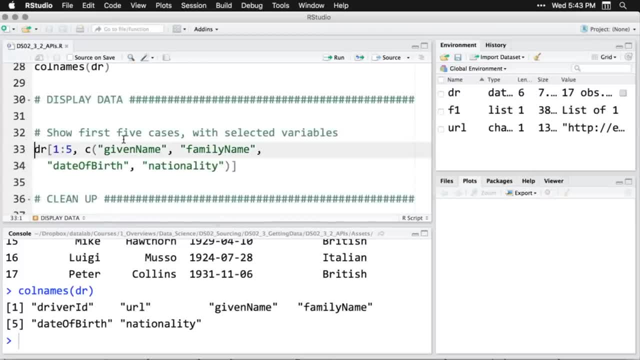 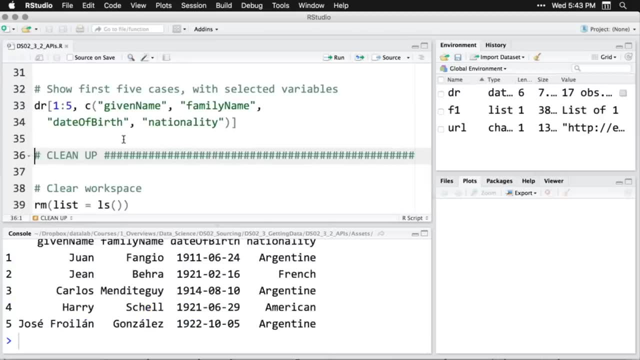 what I'm going to do is I'm going to pick just the first five cases and I'm going to select some variables and put them in a different order, And when I do that, this is what I get. I'll zoom in on that again, And the first five people listed in the list are the ones that are listed in the list. 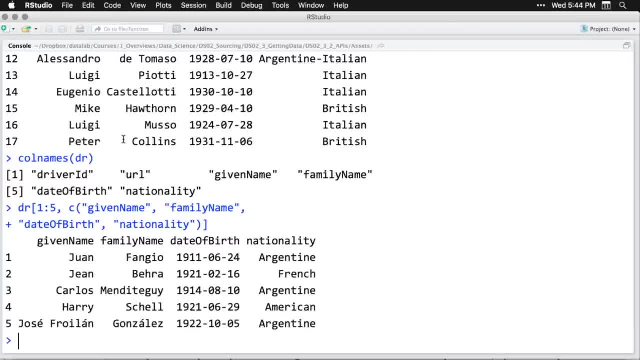 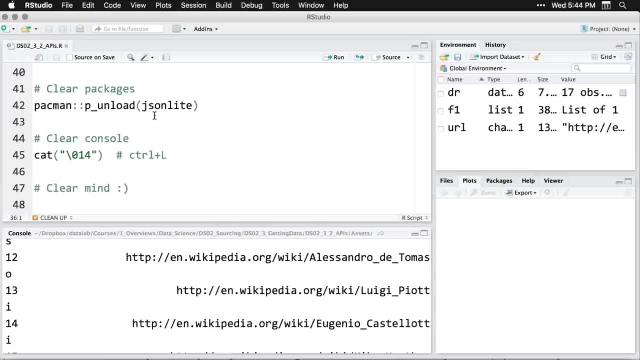 This data set that I pulled in from 1957. Our one, Fangio, makes sense, one of the greatest drivers ever- and other people who competed in that year, And so what I've done is, by using this API call in ours- very simple thing to do- I was able to pull data off that web page in a structured format and 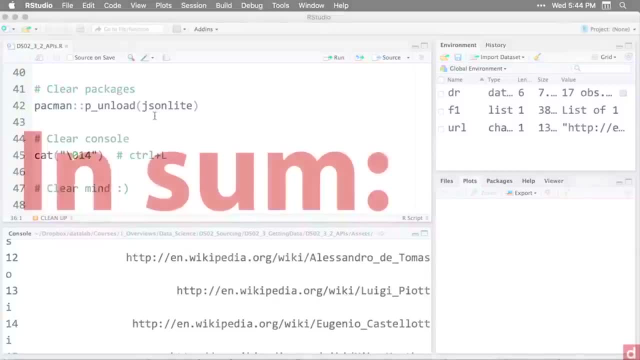 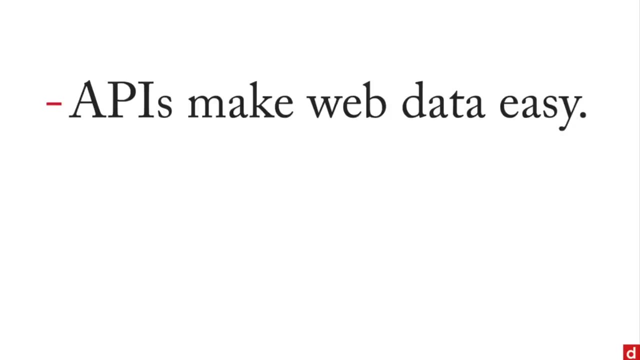 do a very simple analysis with it And let's sum up what we've learned from all this. First off, API's make it really easy to work with web data. They structure it, they call it for you And then they feed it straight into the programs for you. 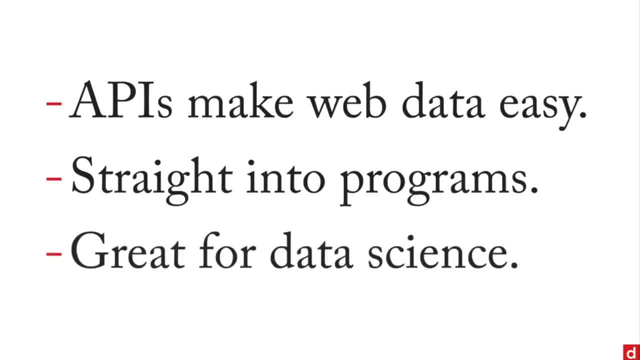 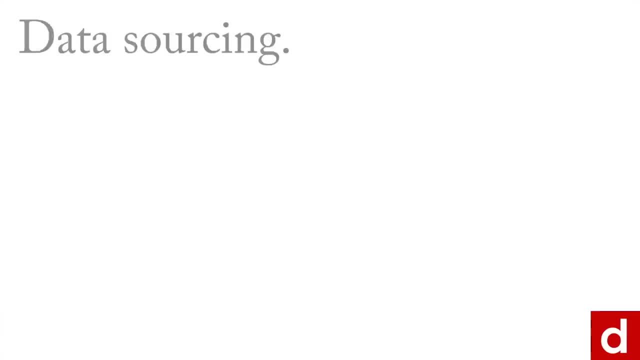 to analyze, And they're one of the best ways of getting data and getting started in data science When you're looking for data. another great way of getting data is through scraping, And what that means is pulling information from web pages. I like to think of it as when data is hiding in. 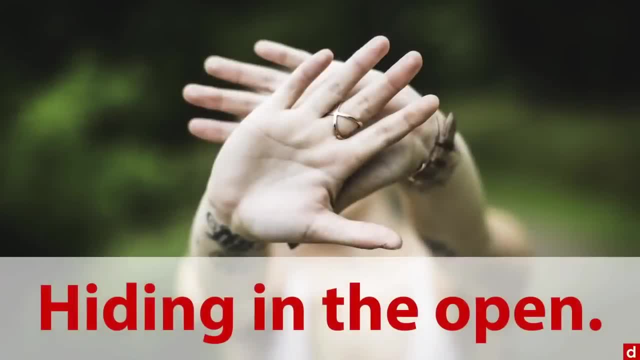 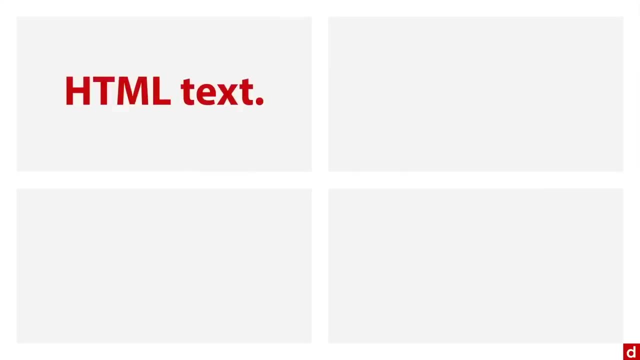 the open. It's there, you can see it, But there's not an easy, immediate way to get that data Now, when you're dealing with scraping. you can get data in several different formats. You can get HTML text from web pages. you can get HTML tables- the rows and columns that appear on web pages. 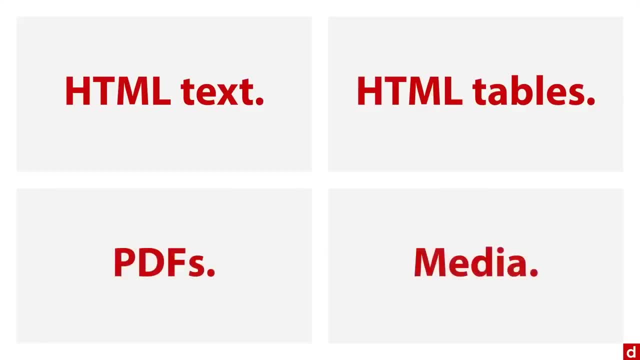 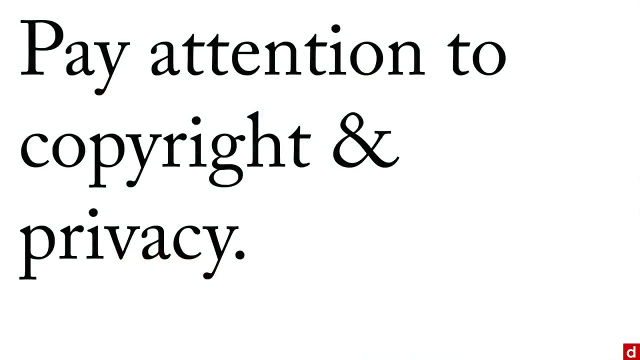 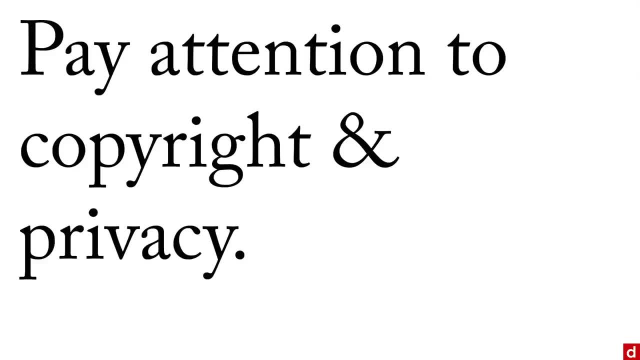 to pull it out. information gets copyrighted, And so when I use examples here, I make sure that this is stuff that's publicly available, And you should do the same when you're doing your own analyses. Now, if you want to scrape data, there's a couple of ways to do it. Number one is to use apps that. 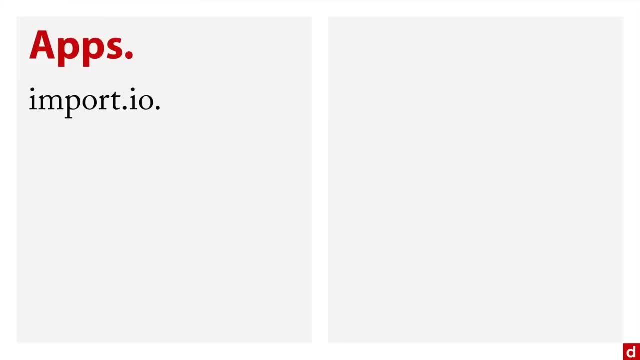 are developed for this. So, for instance, importio is one of my favorites. It's both a web page- that's its address- and it's a downloadable app. There's also a scraper wiki. there's an application called tabula, And you can even do scraping in Google Sheets, which I'll demonstrate. 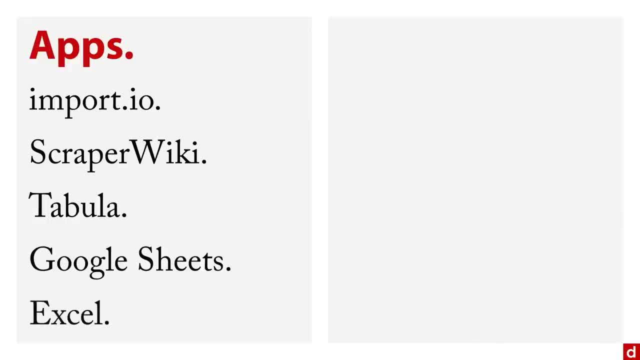 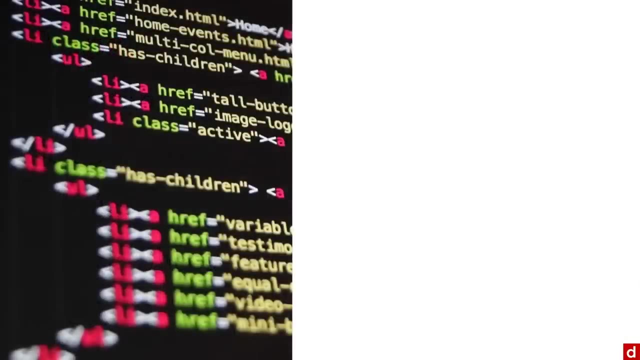 in a second and Excel. Or if you don't want to use an app, or if you want to do something that apps don't really let you do, you can code your scraper. you can do it directly in R or Python or bash or even Java or PHP. Now what you're going to do is you're going to be looking for 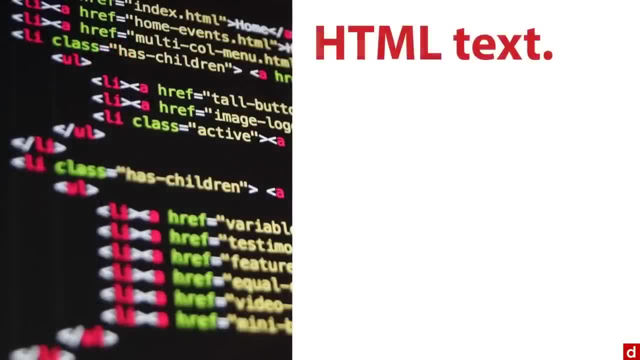 information on the web page. If you're looking for HTML text, what you're going to do is you're going to pull that out and you're going to pull that out, And then you're going to pull that out- structured text from web pages, similar to how a reader view works in a browser. It uses HTML tags. 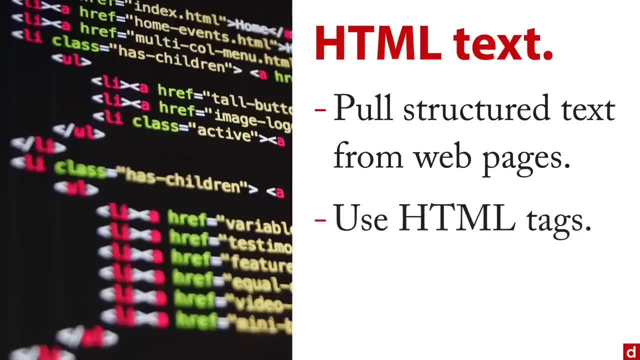 on the web page to identify what's the important information. So that's things like body and h1 for header one and P for paragraph in the angle brackets. You can also get information from HTML tables, although this is a physical table of rows and columns. I'm showing you This also. 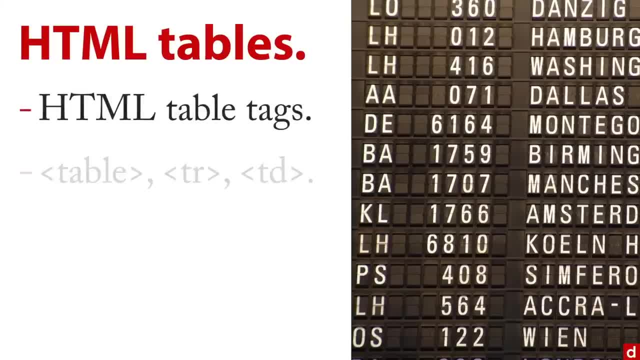 uses HTML table tags. that's like table, and TR for table row and TD for row, And you can also get information for table data. that's a cell. The trick is, when you're doing this, you need the table number, And sometimes you just have to find that through trial and error. Let me give you an. 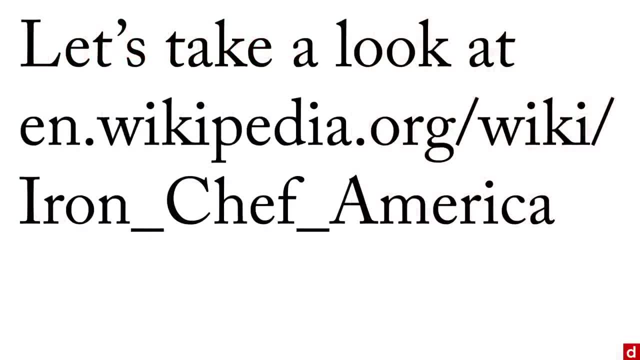 example of how this works. Let's take a look at this Wikipedia page on the Iron Chef America competition. I'm going to go to the web right now and show you that one. So here we are in Wikipedia- Iron Chef America- And if you scroll down a little bit you see we got a whole bunch. 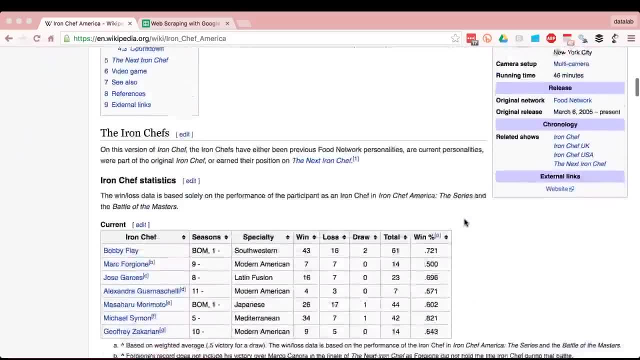 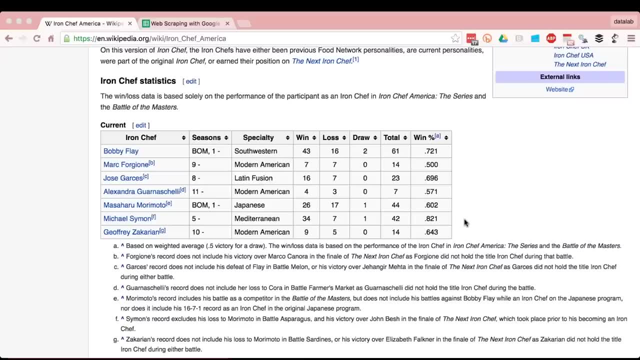 of text here and we've got our table of contents, And then we come down here. we have a table that lists the winners, the statistics for the winners, And let's say, we want to pull that from this web page into another program for us to analyze. Well, there's an extremely easy way. 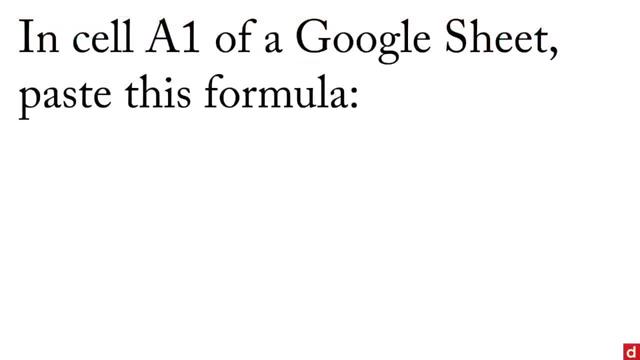 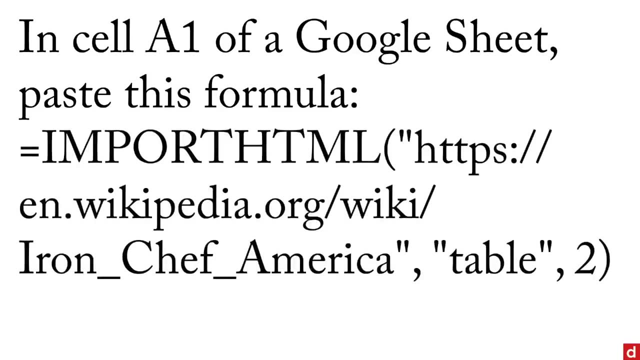 to do this with Google Sheets. All we need to do is open up a Google Sheet And in cell a one of that Google Sheet, we paste in this formula: it's import HTML. then you give the web page. then you say that you're importing a table. you have to put that stuff in quotes and the index. 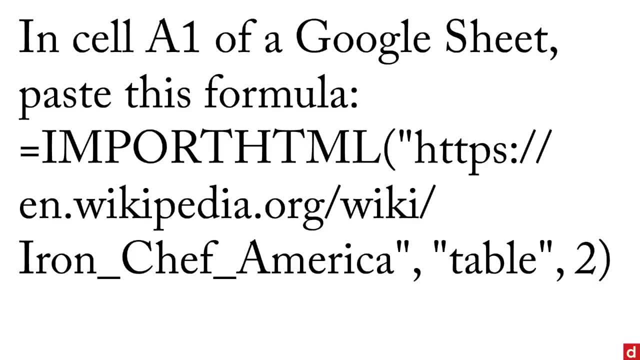 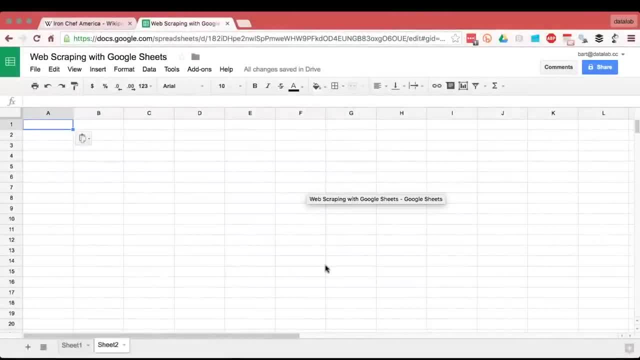 number for the table. I had to poke around a little bit to figure out that this one was table number two. So let me go to Google Sheets and show you how this works. Here I have a Google Sheet And right now it's got nothing in it. But watch this. if I come here to this cell and I simply paste, 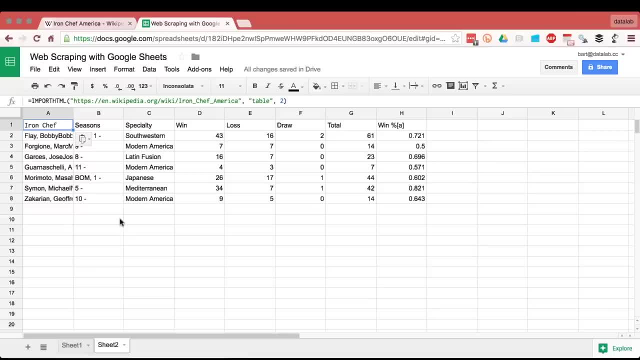 in that information. all this stuff to sort of magically propagates into the sheet makes it extremely easy to deal with, And now I can, for instance, save this as a CSV file, put it in another program, lots of options, And so this is a very simple way to do this, And so this is a 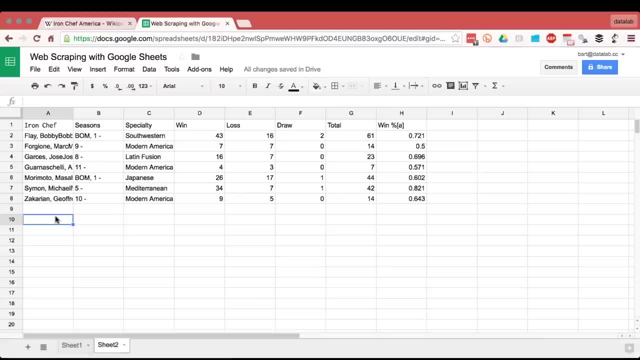 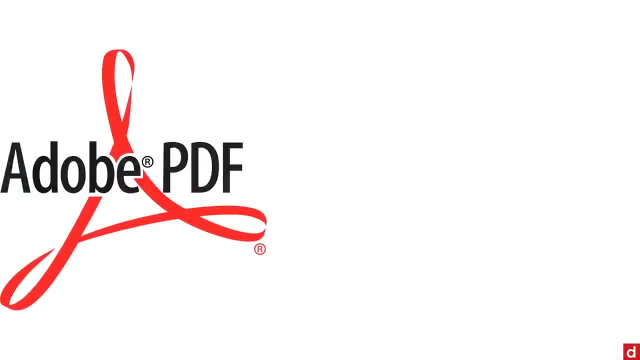 one way that I'm scraping the data from a web page, because I didn't use an API, But I just use a very simple one line command in Google Sheets to get the information. Now, that was an HTML table. you can also scrape data from PDFs. you have to be aware of whether it's a native PDF. I call that a. 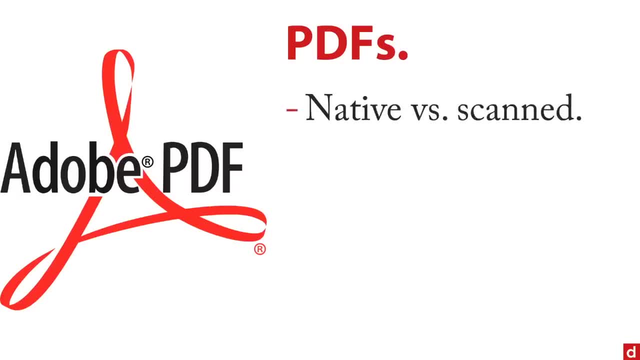 text PDF or a scanned or image PDF, And what it does with native PDFs is it looks for text elements. Again, those are like code that indicates this is text, And you can deal with raster images, that's pixel images or vector, which draws the lines, And that's what makes them infinitely. 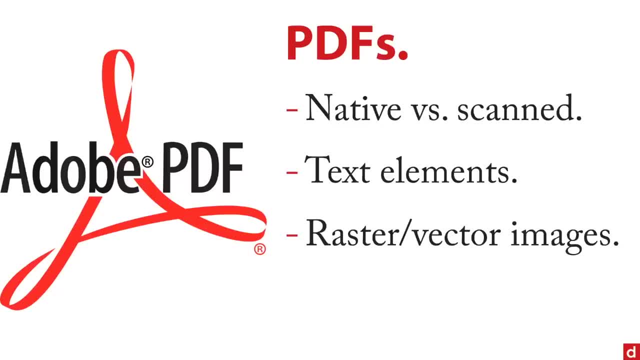 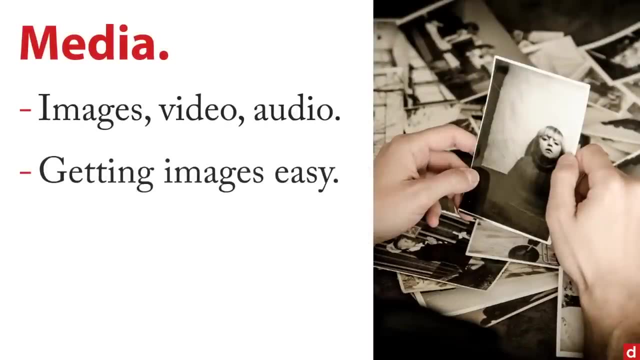 scalable in many situations. And then in PDFs you can deal with tabular data, but you probably have to use a specialized program like scraper, wiki or tabula in order to get that. And then, finally, media like images and video and audio. getting images is easy. you can download them in. 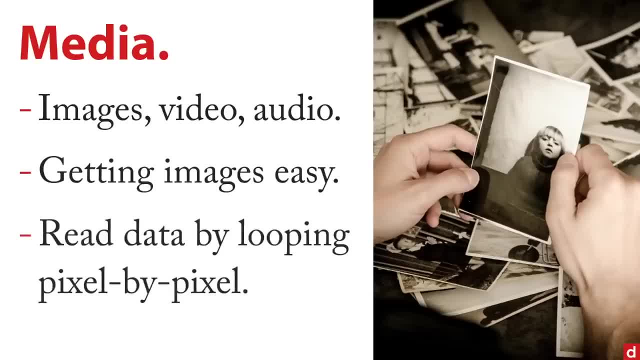 a lot of different ways And then if you want to read data from them- say, for instance, you have a heat map of a country- you can go through it, but you'll probably have to download a lot of them. You might have to write a program that loops through the image pixel by pixel to read the. 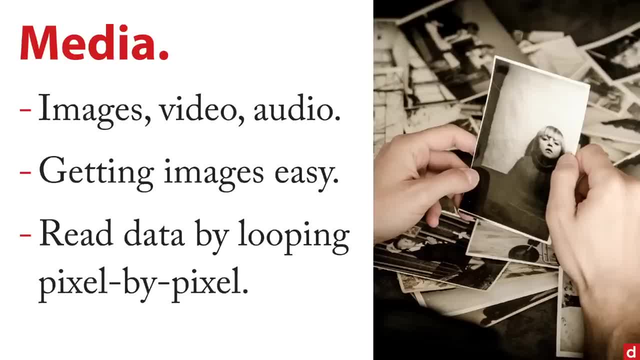 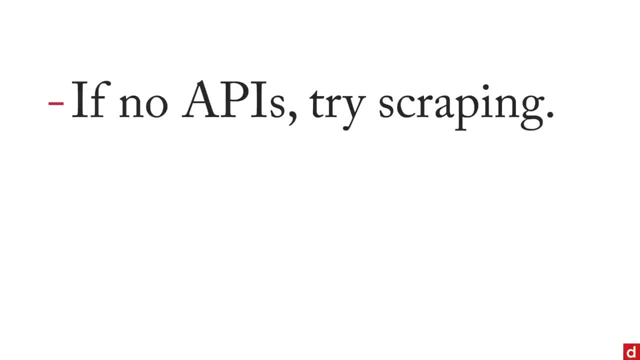 data and then encode it numerically into your statistical program. Now that's my very brief summary, And let's summarize that. First off, if the data you're trying to get at doesn't have an existing API, you can try scraping And you can use specialized apps for scraping, or you can write. 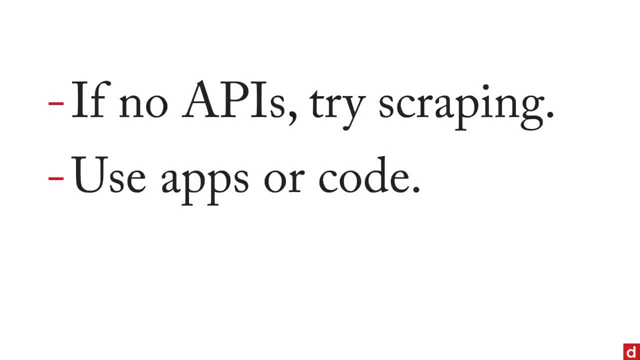 code in a language like our, Python. But no matter what you do be sensitive to issues of copyright and privacy, So you don't get yourself in hot water, But instead you make an analysis that can be of great use to you or to your client. 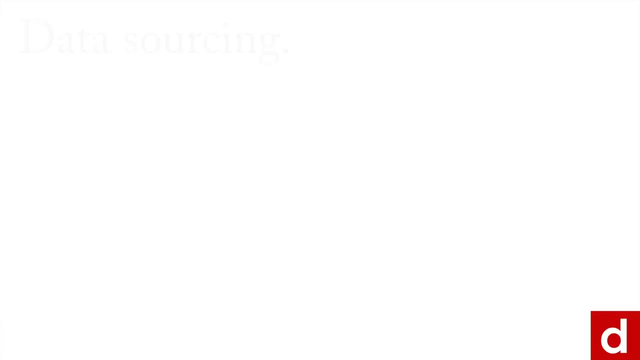 The next step in data sourcing is making data, And specifically, we're talking about getting new data. I like to think of this, as you're getting your hands on and you're getting data de novo- new data. So can't find the data that you need for your analysis? Well, one simple solution is. 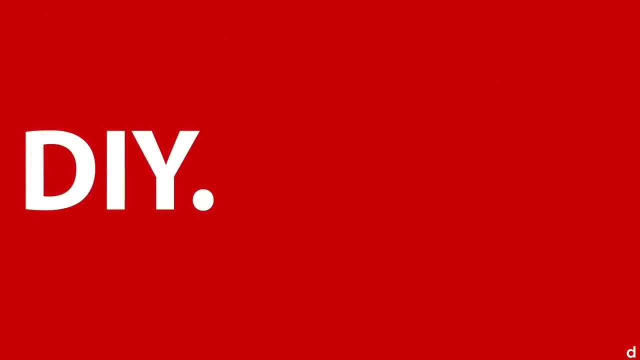 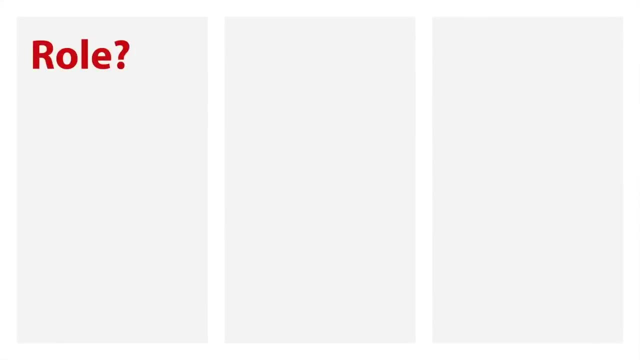 do it yourself, And we're going to talk about a few general strategies used for doing that. Now, these strategies vary in a few dimensions. First off is the role. Are you passive and simply observing stuff that's happening already, Or are you active, where you play a role in creating the 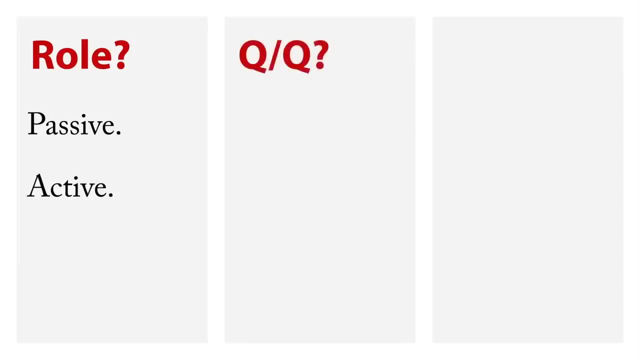 situation to get the data. And then there's the QQ question, And that is: are you going to get quantitative or numerical data, Or are you going to get qualitative data, which usually means text, paragraph sentences, as well as things like photos and videos and audio? And also, how are you going? 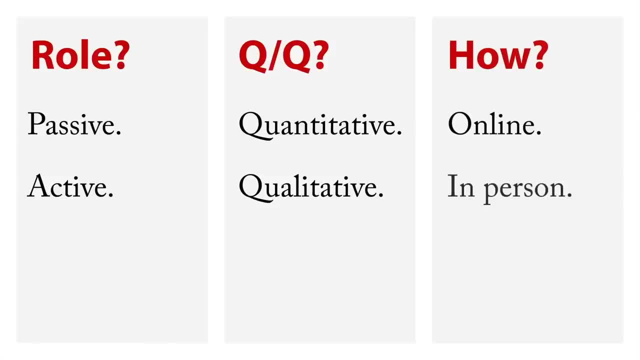 to get the data? Do you want to get it online Or do you want to get it in person? Now, there's other choices in these, but these are some of the big delineators of the different methods. When you look at those, you get a few possible options. Number one is interviews, And I'll say more about 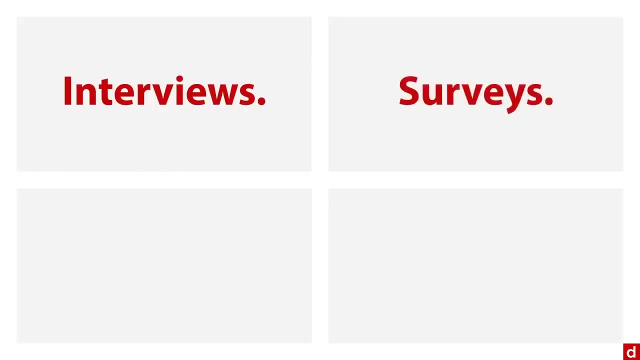 those. Another one is surveys, A third one is card sorting And the fourth one is an experiments, although I actually want to split experiments into two kinds of categories. The first one is laboratory experiments, And that's in person projects, And the third one is in person projects. 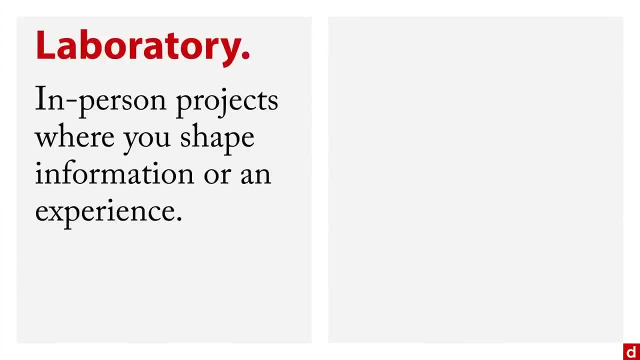 Where you shape the information or an experience for the participants as a way of seeing how that involvement changes their reactions. doesn't necessarily mean that you're a participant, but you create the situation. And then there's also a B testing. This is automated online testing. 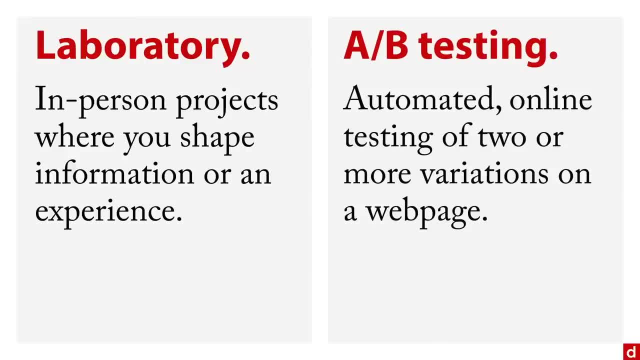 of two or more variations on a web page. It's a very, very simple kind of experimentation. there's actually very useful for optimizing websites. So, in sum, from this very short introduction, make sure you can get exactly what you need. 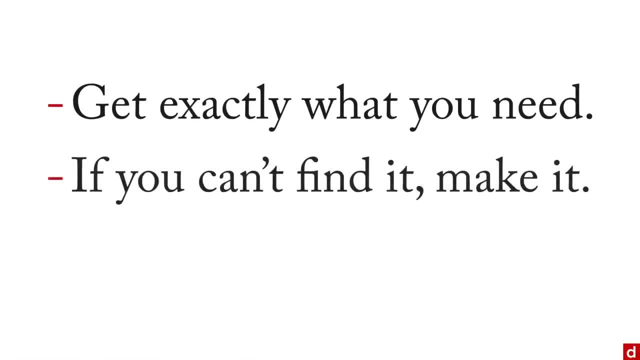 get the data you need to answer your question, And if you can't find it somewhere, then make it. And, as always, you have many possible methods, each of which have their own strengths and their own compromises, And we'll talk about each of those in the following sections. The first method of data. 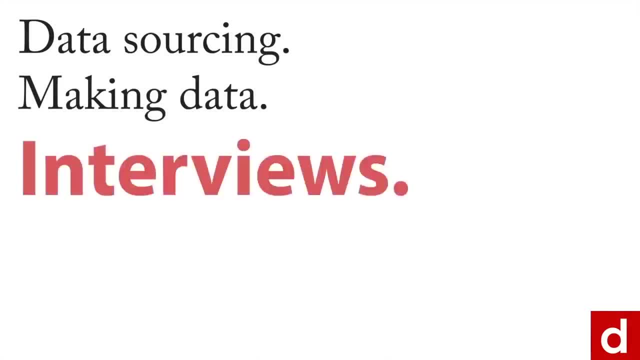 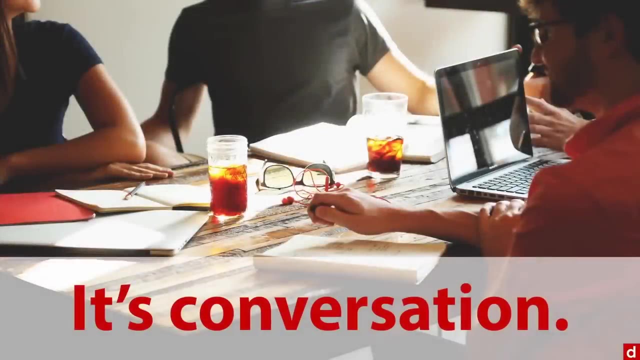 sourcing, where you're making new data. that I want to talk about is interviews, And that's not because the most common, but because it's the one you would do for the most basic problem. Now, basically, an interview is nothing more than a conversation with another person or a group of people, And the 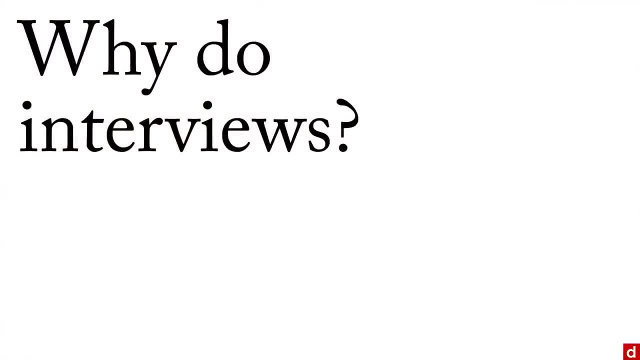 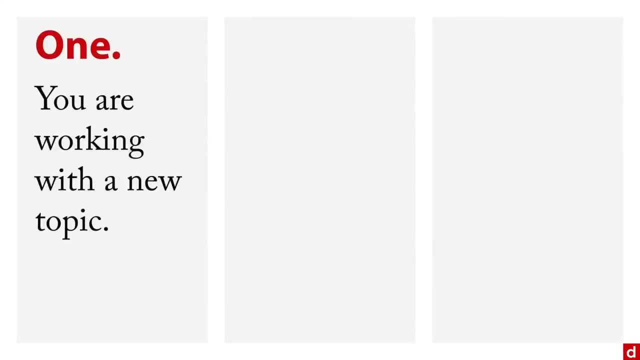 fundamental question is: why do interviews as opposed to doing a survey or something else? Well, there's a few good reasons to do that. Number one: you're working with a new topic and you don't know what people's responses will be, how they'll react, And so you need something very open ended. 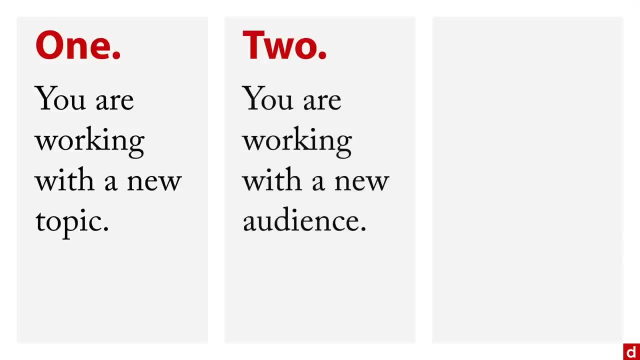 Number two: you're working with a new audience. you don't know how they will react, in particular, to what it is you're trying to do. And number three: something's going on with the current situation. it's not working anymore And you need to find out what's going on And you need to find ways. 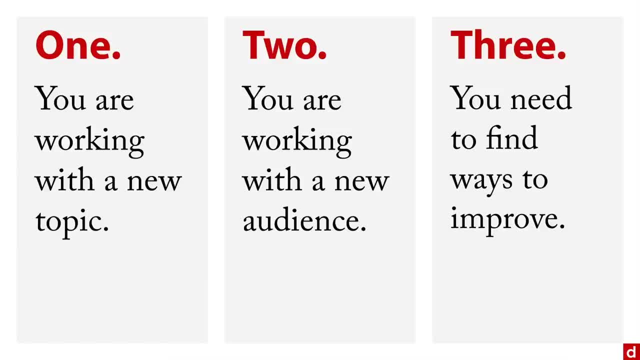 to improve the open ended information where you get past your existing categories and boundaries, can be one of the most useful methods for getting that data. If you want to put it another way, you want to do interviews when you don't want to constrain response. 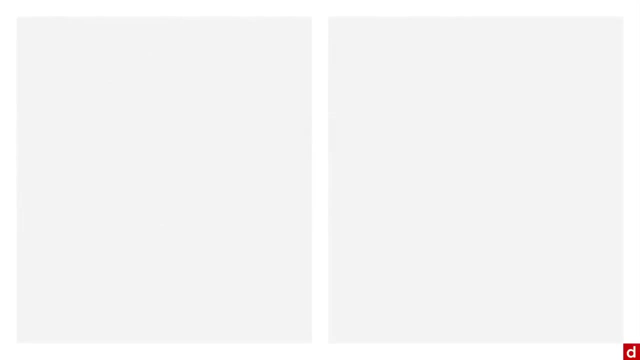 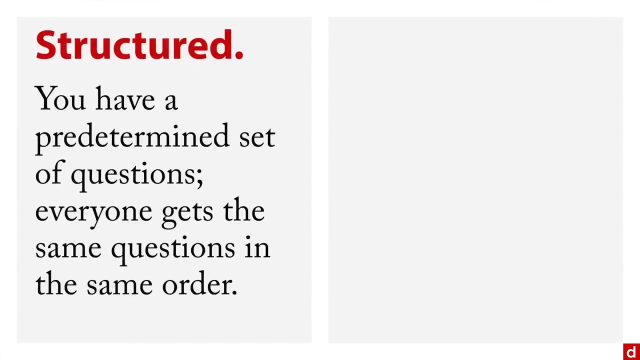 Now, when it comes to interviews, you have one very basic choice, And that's whether you do a structured interview And with a structured interview, you have a predetermined set of questions And everyone gets the same questions in the same order. It gives a lot of consistency. 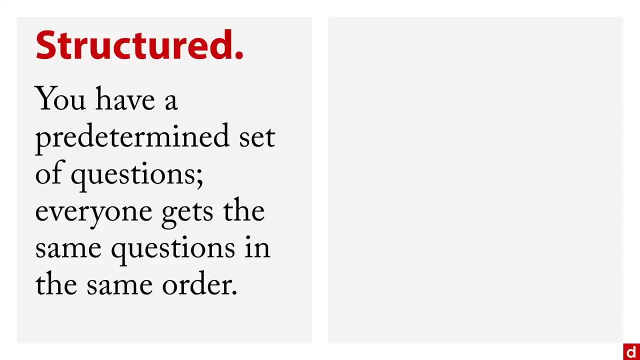 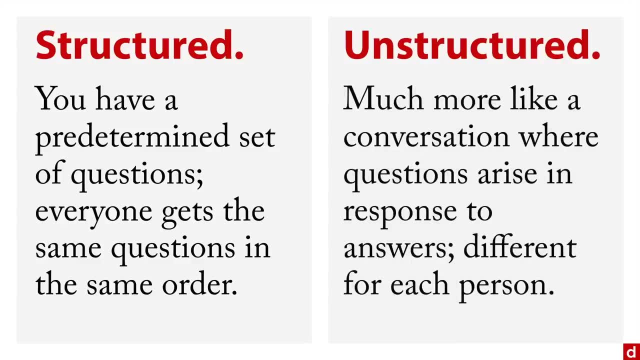 even though the responses are open ended. And then you can also have what's called an unstructured interview, And this is a whole lot more like a conversation where you as the interviewer and the person you're talking to- your questions- arise in response to their answers. Consequently, an unstructured interview can be. 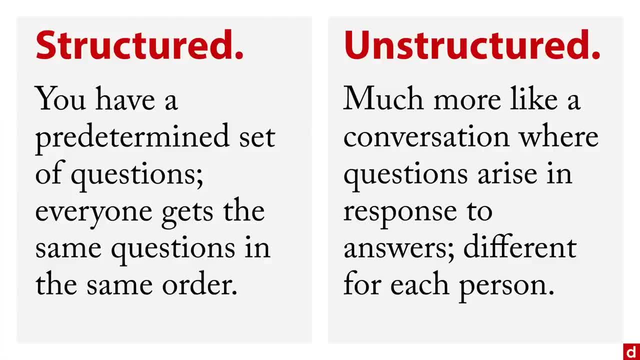 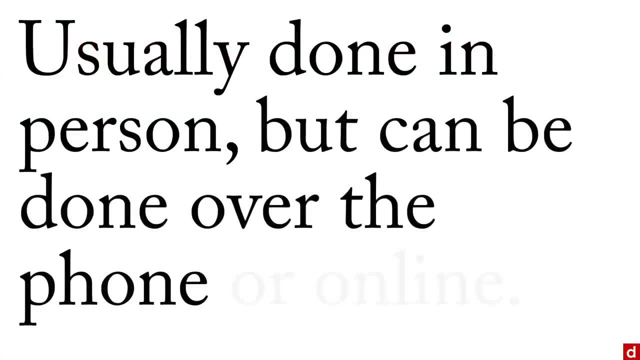 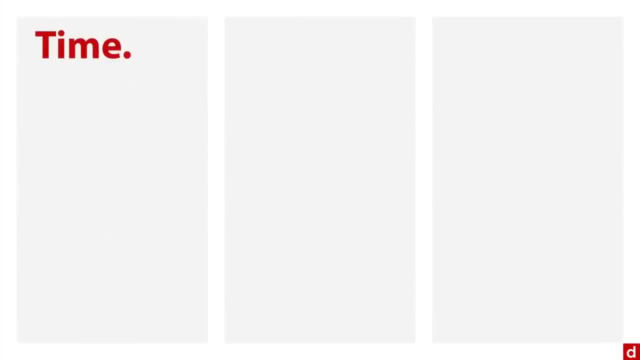 different for each person that you talk to. Also, interviews are usually done in person, But, not surprisingly, they can be done over the phone or often online. Now a couple of things to keep in mind about interviews. Number one is time. interviews can range from just a few minutes to. 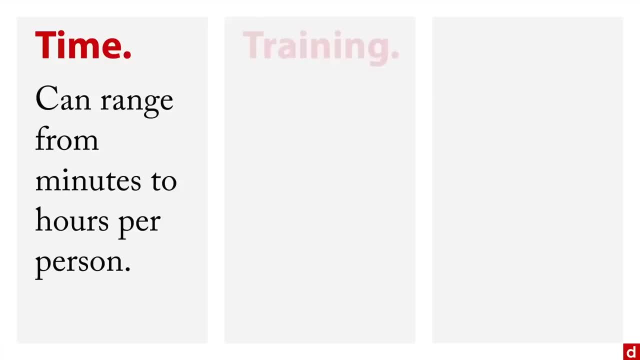 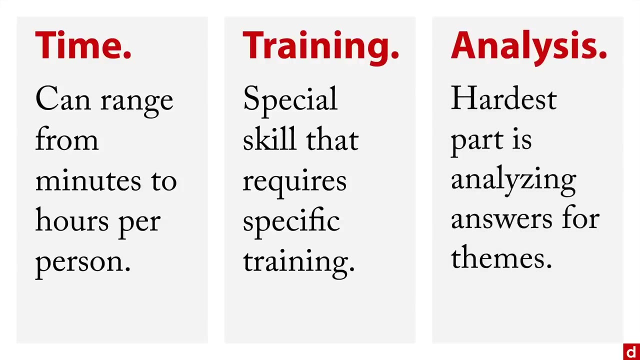 several hours per person. Second is training. Interviewing is a special skill that usually requires specific training. Now, asking the questions is not necessarily the hard part. The really tricky part is the analysis. The hardest part of interviews by far is analyzing the answers for themes and way of extracting the 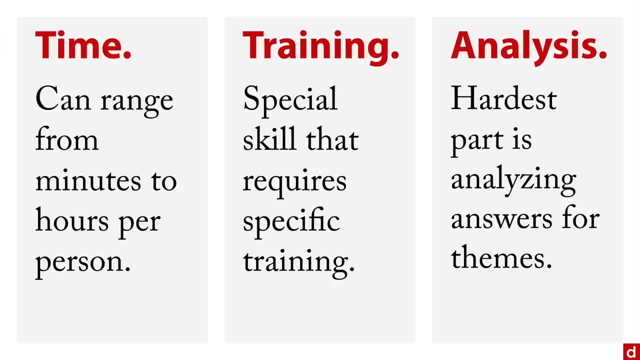 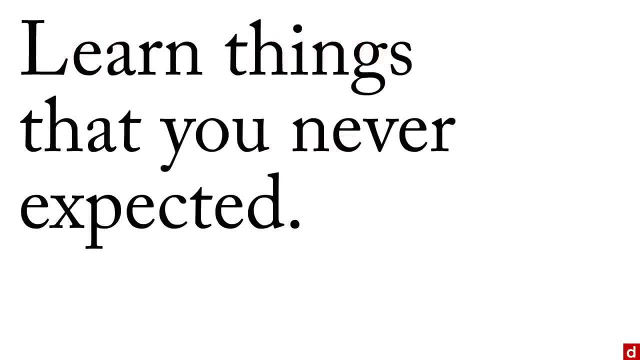 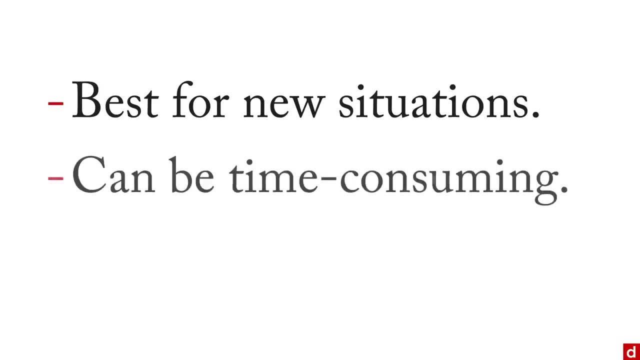 new categories and the dimensions that you need for your further research. The beautiful thing about interviews is they allow you to learn things that you never expected. So, in sum, interviews are best for new situations or new audiences. On the other hand, they can be time. 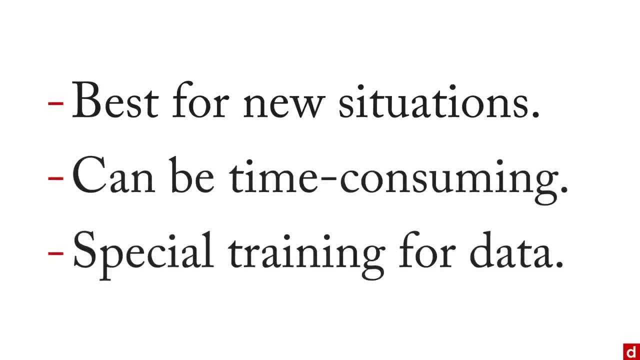 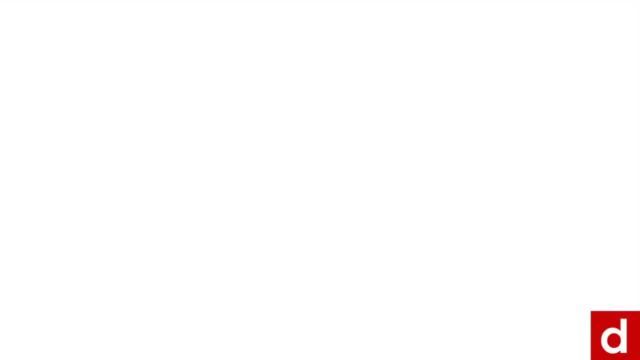 consuming, And they also require special training both to conduct the interview but, even more, to analyze the highly qualitative data that you get from them. An interesting topic in data sourcing, when you're making data, is card sorting. Now, this isn't something that comes up very often. 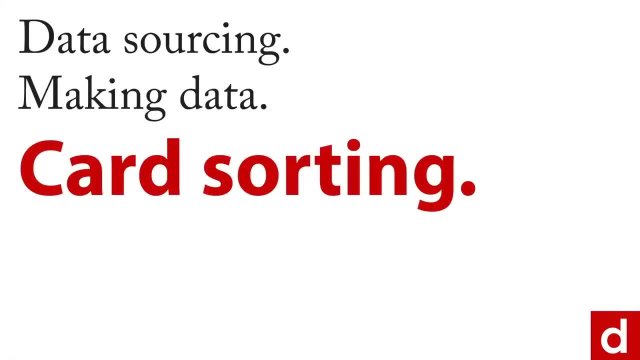 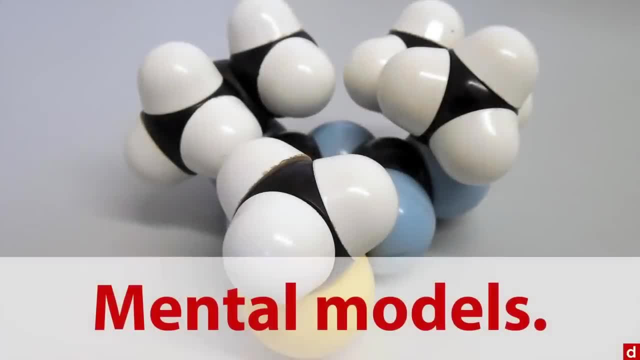 research. Think of it as what you're trying to do in your research. Think of it as what you're trying to do. it's like building a model of a molecule. here You're trying to build a mental model or a model of people's. 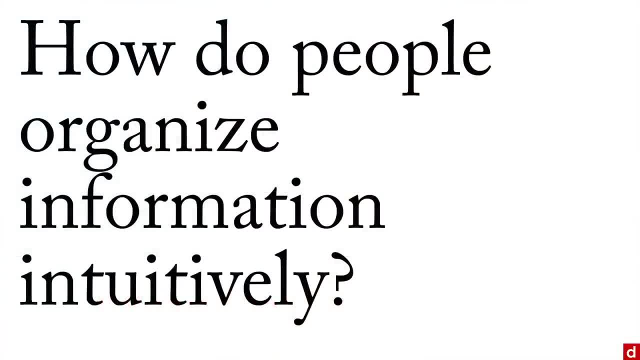 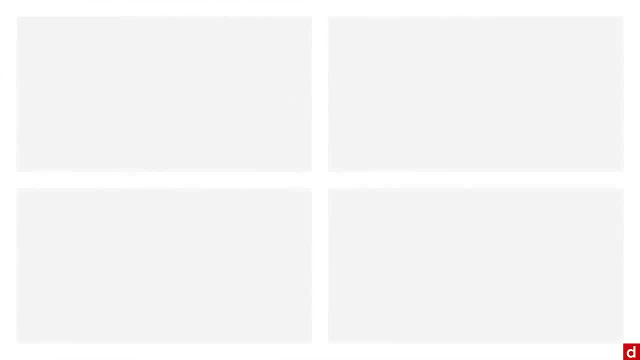 mental structures. But, more specifically, how do people organize information intuitively? And also, how does that relate to the things that you're doing online? Now, the basic procedure goes like this: You take a bunch of little topics and you write each one on a separate card And you can do. 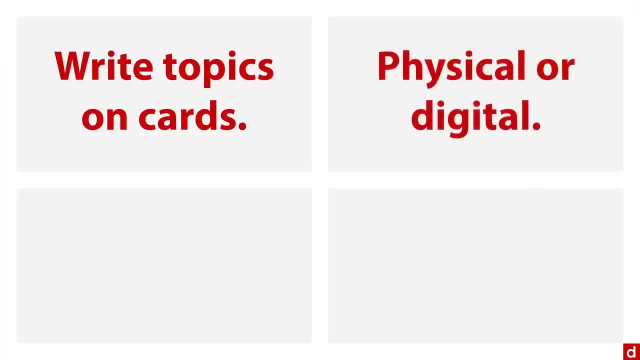 this physically with like three by five cards, or there's a lot of programs that allow you to do a digital version of it. Then what you do is you give this information to a group of respondents and the people sort those cards So they put similar topics with each other, different topics over here, and so on. 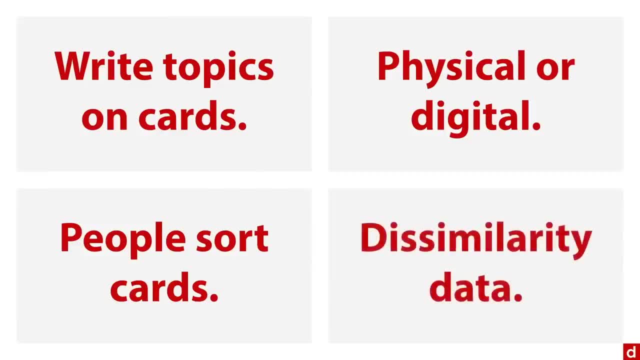 And then you take that information And from that you're able to calculate what's called dissimilarity data. Think of it as like the distance or the difference between various topics, And that gives you the raw data to analyze how things are structured. Now 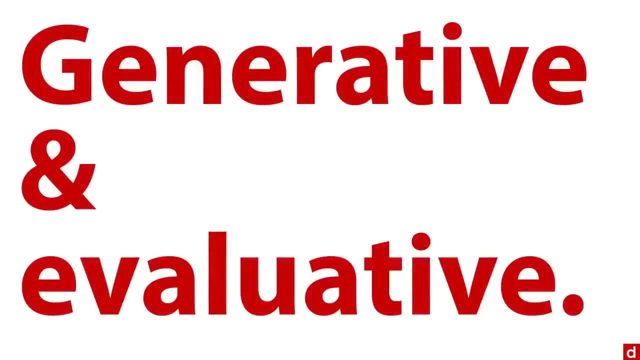 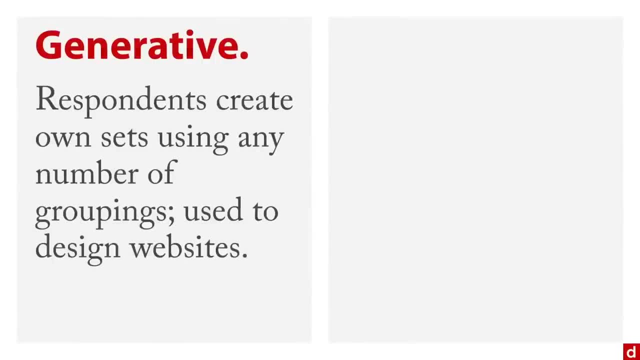 there are two very general kinds of card sorting tasks. They're generative and there's evaluative. A generative card sorting task is one in which respondents create their own sets, their own piles of cards, using any number of groupings they like, And this might be used, for instance, 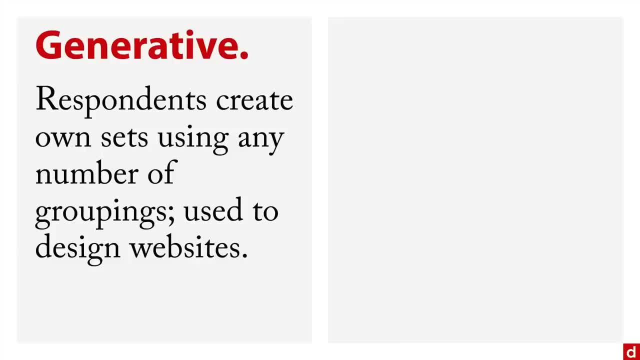 to design a website. If people are going to be looking for one kind of information next to another one, then you want to put that together on the website so they know where to expect it. On the other hand, if you've already created a website, then you can do an evaluative card. 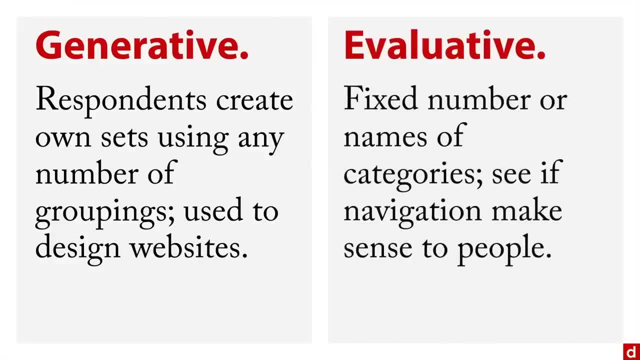 sorting. This is where you have a fixed number or fixed names of categories, like, for instance, the way you've set up your menus already, And then what you do is you see if people naturally put the cards into these various categories that you've created. That's a way of verifying that. 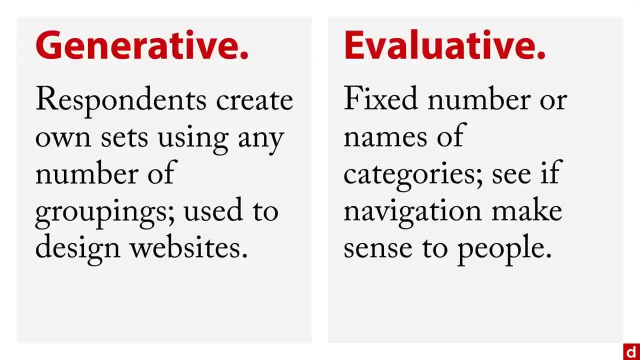 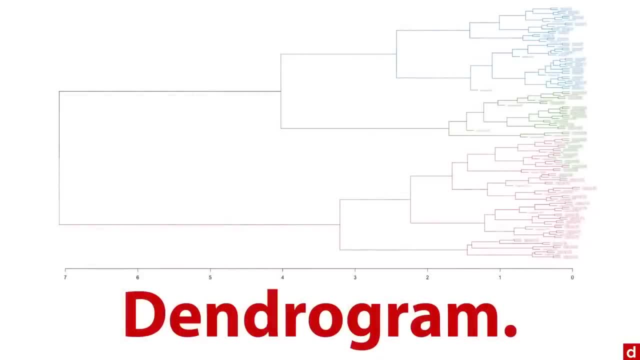 your hierarchical structure makes sense to people. Now, whichever method you do, generative or evaluative, what you end up with when you do a card structure is an interesting kind of visualization. It's called a dendrogram. That actually means branches And what we have here 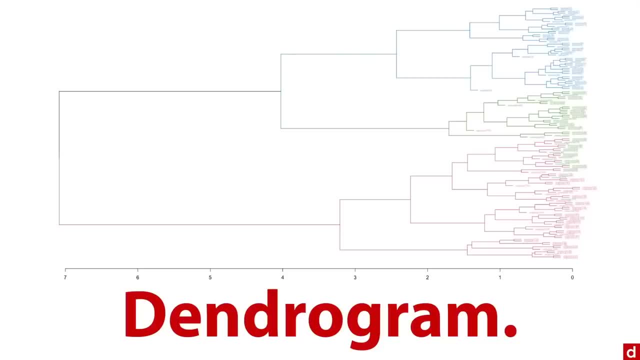 is actually 150 data points, If you're familiar with Fisher's iris data. that's what's going on here, And it groups it from one giant group on the left and then splits it in pieces and pieces and pieces until you end up with lots of different observations. Well, actually, individual level. 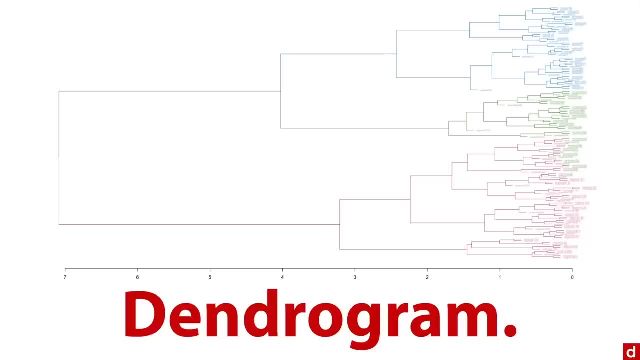 observations at the end, But you can cut things off into two Or three groups or wherever it's most useful for you here as a way of visualizing the entire collection of similarity or dissimilarity between the individual pieces of information that you had. 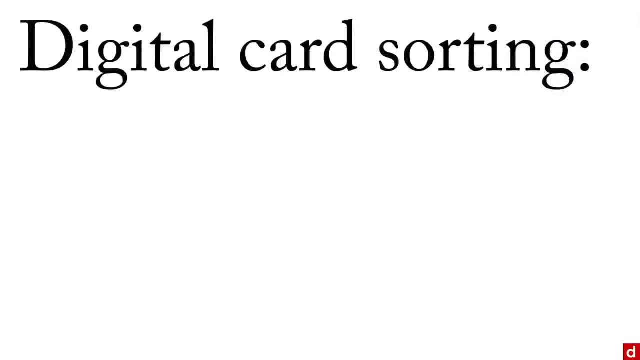 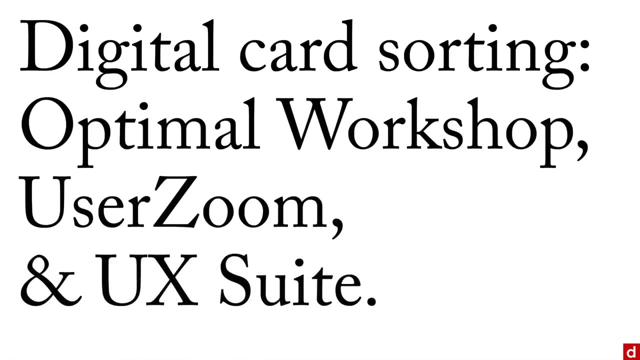 people sort. Now I'll just mention very quickly: if you want to do digital card sorting, which makes your life infinitely easier because keeping track of physical cards is really hard- You can use something like optimal workshop or user zoom or UX suite. These are some of the most common. 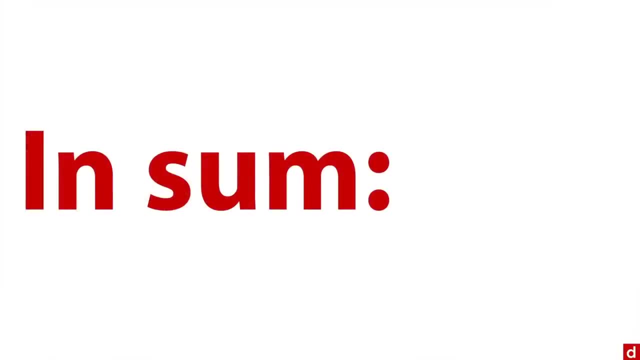 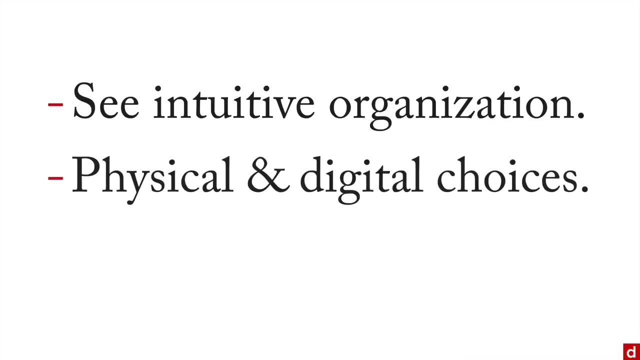 choices. Now let's just sum up what we've learned about card sorting in this extremely brief overview. Number one, card sorting, allows you to see intuitive organization of information in a hierarchical format. You can do it with physical cards or you also have digital choices for doing. 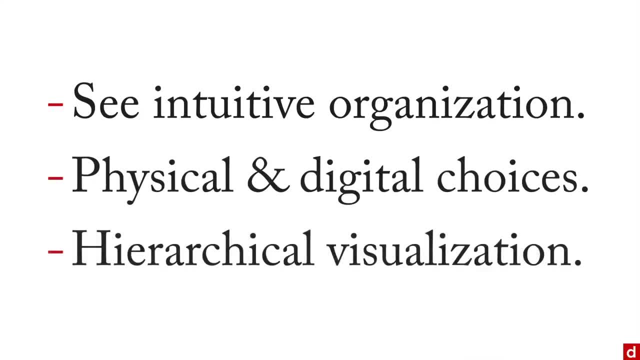 the same thing And when you're done, you actually get this hierarchical or branched visualization of how the information is structured and related to each other. When you're doing your data sorting, you're making data. sometimes you can't get what you want through the easy ways And you got to take 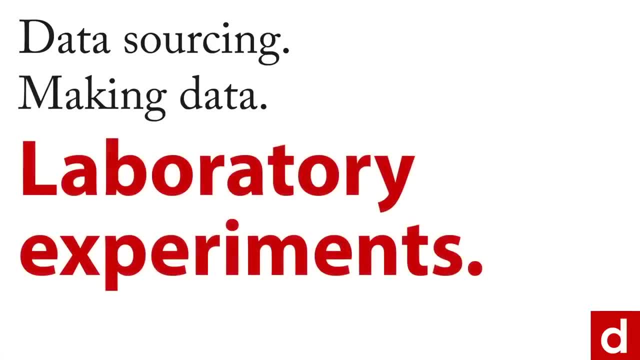 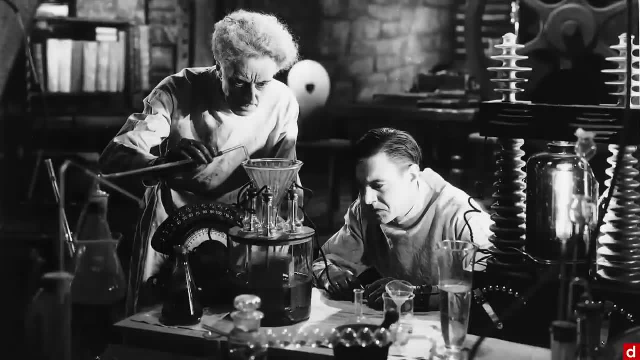 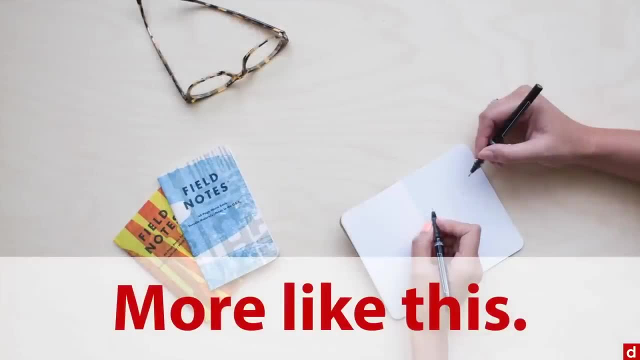 the hard way And you can do what I'm calling laboratory experiments. Now, of course, when I mentioned laboratory experiments, people start to think of stuff like, you know, Dr Frankenstein in his lab. but lab experiments are less like this And in fact, they're a little more like this. 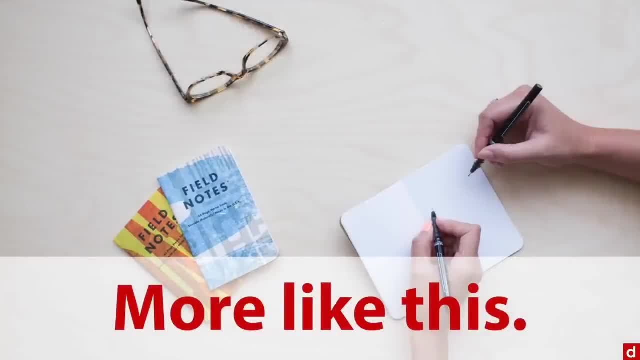 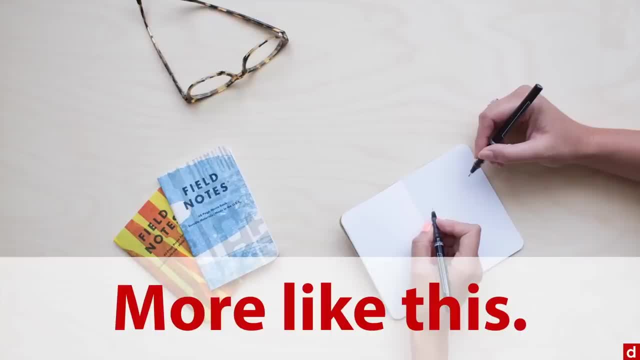 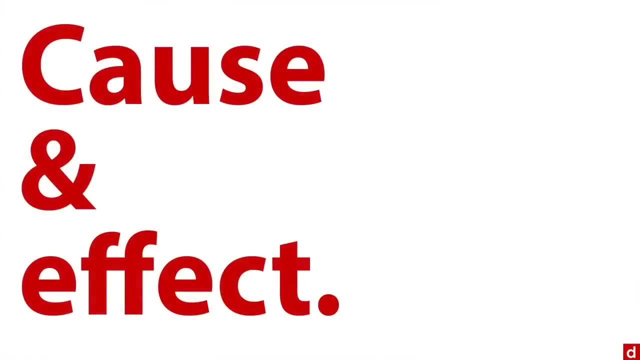 lot of work And it's not been the threatening kind. Now, the reason you do a lab experiment is because you want to determine cause and effect, And this is the single, most theoretically viable way of getting that information. Now, what makes an experiment an experiment is the fact that 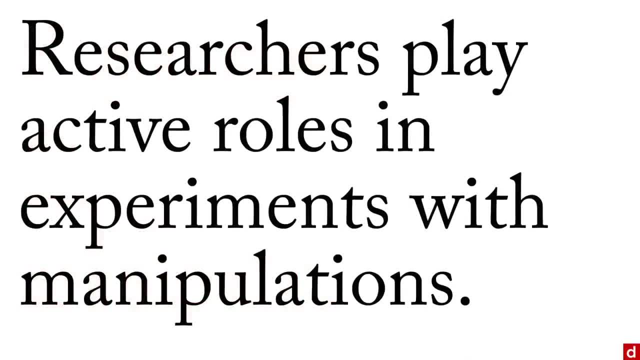 researchers play active roles in experiments with manipulations. Now people get a little freaked out when they hear manipulations, things that you're coercing people and messing with their mind. All that means is you are manipulating the information that you're getting And you're 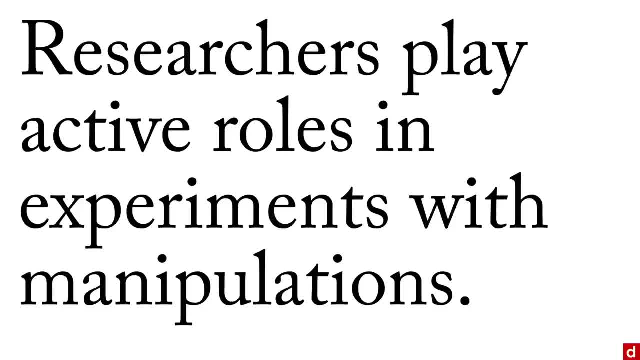 in the situation. you're causing something to be different for one group of people or one situation than another. It's a benign thing, But it allows you to see how people react to those different variations. Now you're going to want to do an experiment. you're going to want to have focused 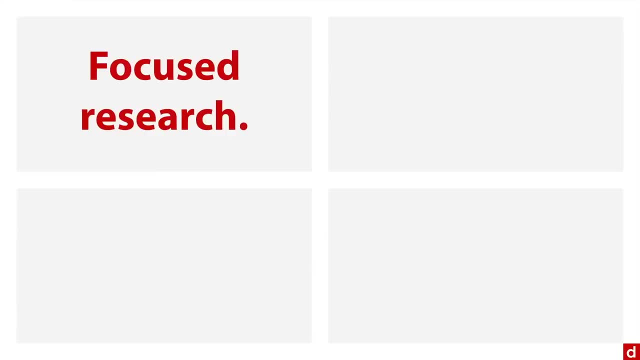 research. it's usually done to test one thing or one variation at a time, And it's usually hypothesis driven. Usually you don't do an experiment until you've done enough background research to say: I expect people to react This way to the situation and this way to the other. A key component of all of this is that 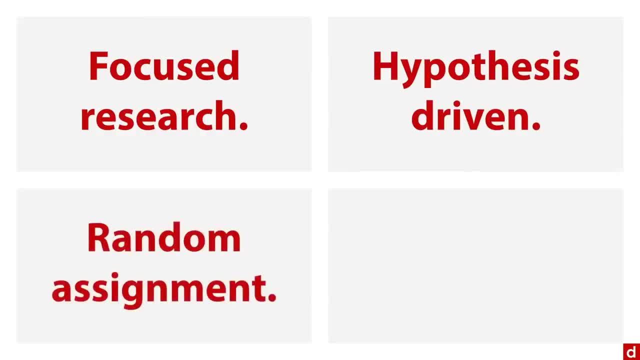 experiments almost always have random assignments, So, regardless of how you got your sample, when they're in your study, you randomly assign them to one condition or another, And what that does is it balances out the pre existing differences between groups, And that's a great way of taking care of confounds and artifacts- the things that are unintentionally. 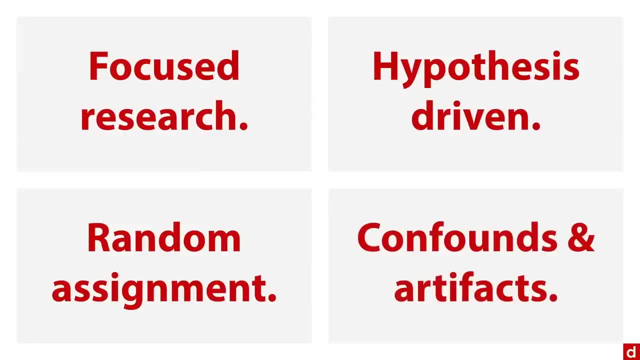 associated with differences between groups that provide alternate explanations For your data. if you've done good random assignment and you have a large enough people, then those confounds and artifacts are basically minimized. Now, some places where you're likely to see a laboratory experiments in this version are, for instance, eye tracking and web design. 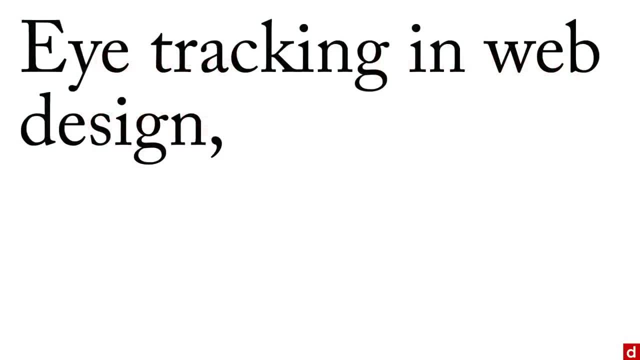 That's where you have to bring people in front of a computer and you stick a thing there that sees where they're looking. That's how we know, for instance, that people don't really look at ads on the side of web pages. Another very common place is research in medicine and education. 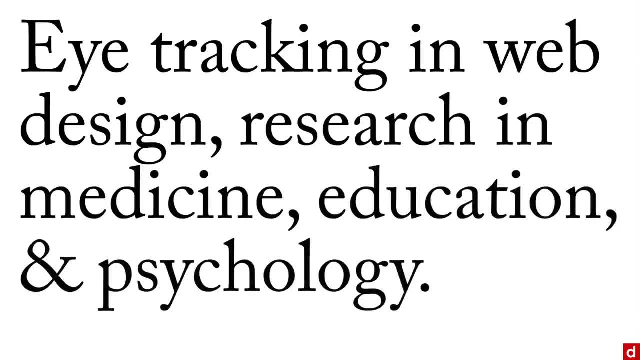 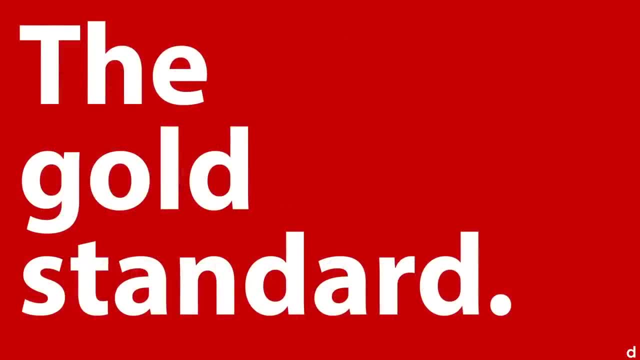 And in my field, psychology. And in all of these, what you find is that experimental research is considered the gold standard for reliable, valid information about cause and effect. On the other hand, while it's a wonderful thing to have, it does come at a cost. Here's how that. 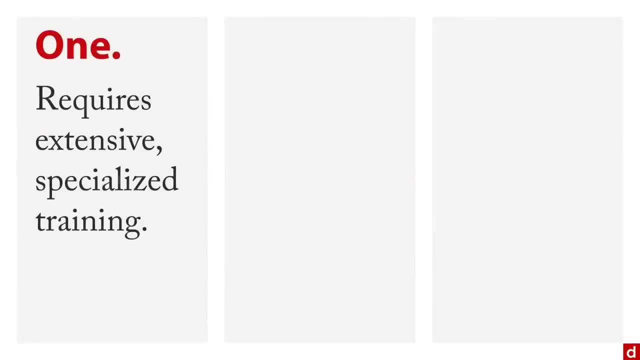 works. Number one experimentation requires extensive specialized training. It's not a simple thing to pick up. Two experiments are often very time consuming and labor intensive. I've known some that take hours per person. And number three experiments can be very expensive. 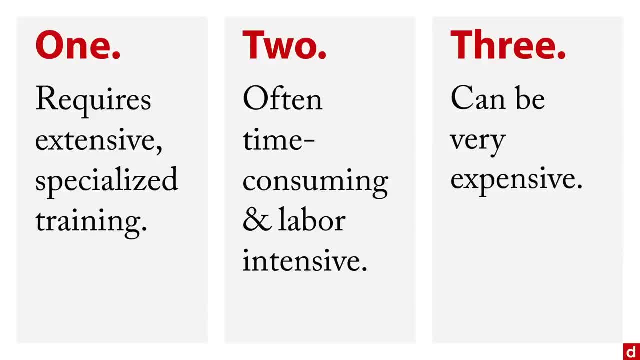 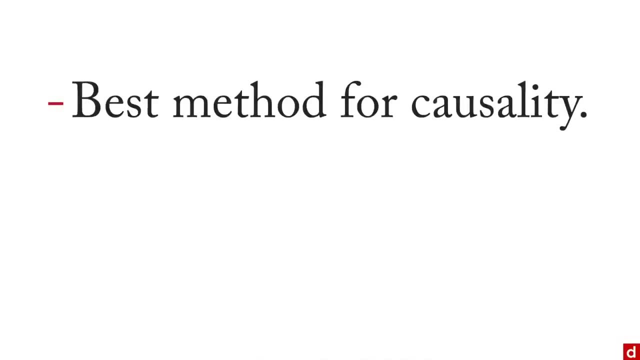 So what that all means is you want to make sure that you've done enough background research and you need to have a situation where it's sufficiently important to get really reliable cause and effect information to justify these costs for experimentation. In sum, laboratory experimentation is generally considered the best method for causality or assessing causality. 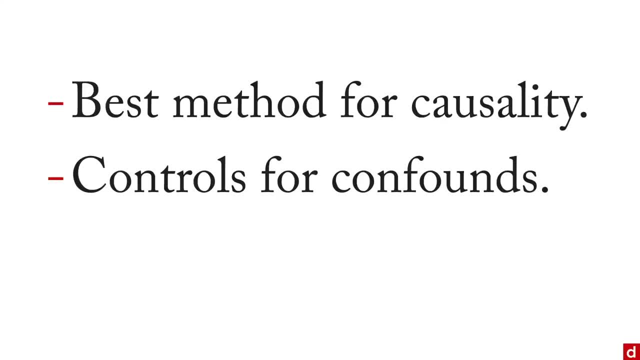 That's because it allows you to control for confounds through randomization. On the other hand, it can be difficult to do So. be careful and thoughtful when considering whether you need to do an experiment and how to actually go about doing it. There's one final procedure I want to. 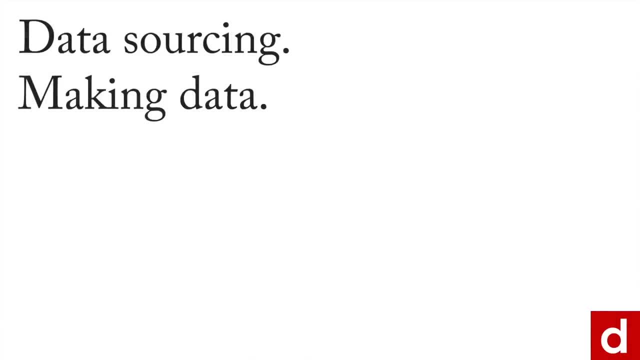 talk about in terms of data sourcing and making new data. It's a form of experimentation, It's simply called A-B testing, And it's extremely common in the web world. So, for instance, I just barely grabbed a screenshot of amazoncom's homepage And I just grabbed a screenshot of 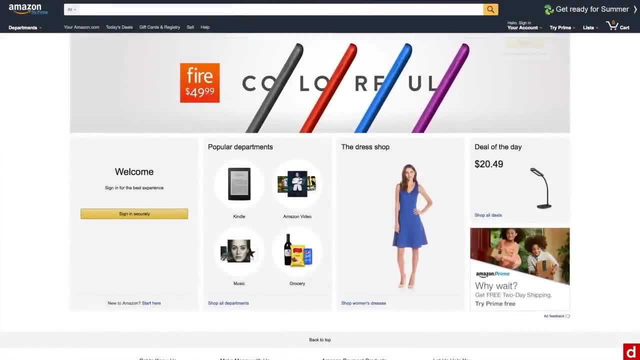 amazoncom's homepage And you've got these various elements on the homepage. And I just noticed, by the way, when I did this, that this woman is actually a animated gif, So she moves around. That was kind of weird. Never seen that before. But the thing about this is this entire. 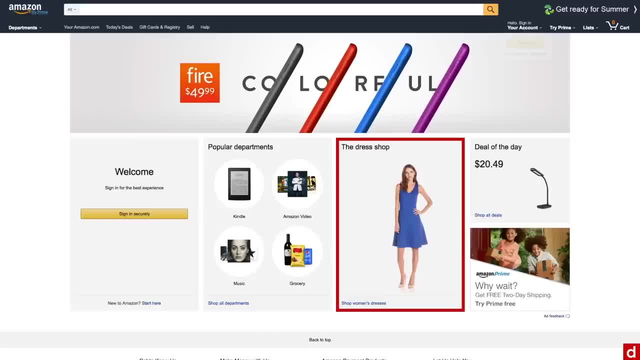 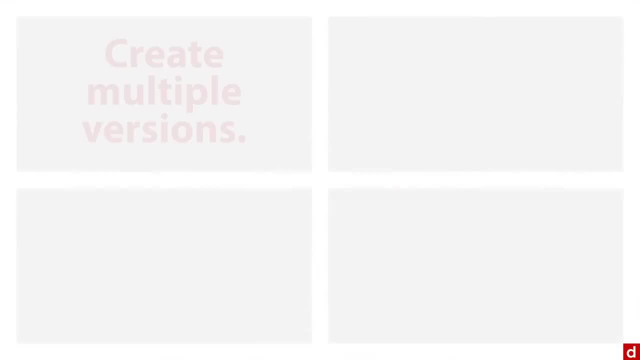 layout, how things are organized and how they're on there, will have been determined by variations on A-B testing by Amazon. Here's how it works For your webpage: you pick one element like what's the headline or what are the colors or what's the organization. 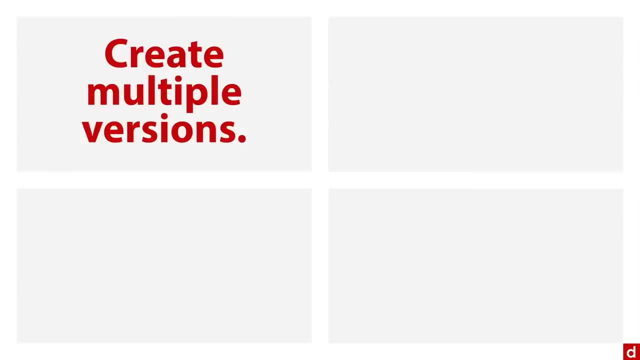 or how do you word something And you create multiple versions, maybe just two, version A and version B, which is why he called A-B testing- And then when people visit your webpage, you randomly assign those visitors to one version or another. You have software that does that for you. 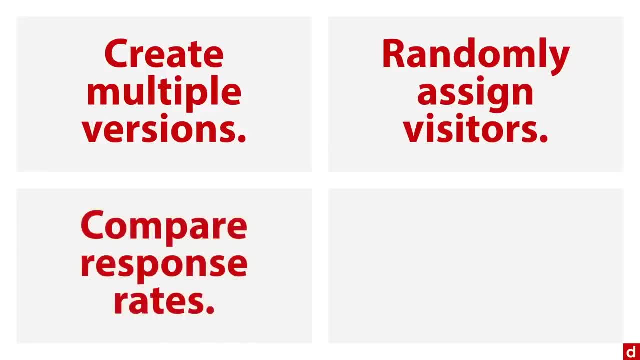 automatically, And then you compare the response rates on some response- I'll show you those in a second- And then, once you have enough data, you implement the best version. you sort of set that one solid and then you go on to something else Now in terms of response rates. 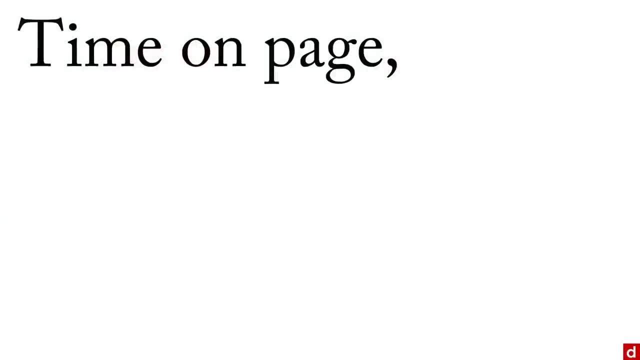 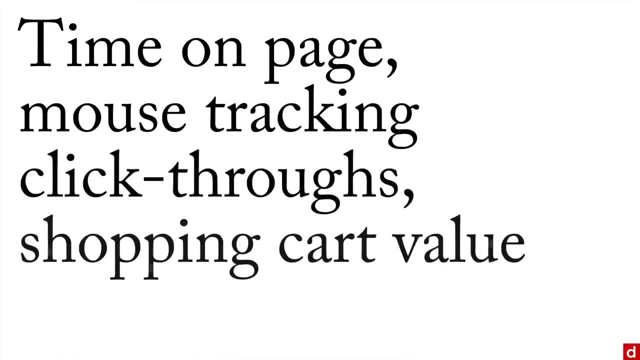 there's a lot of different outcomes you can look at. You can look at how long a person's on a page. you can actually do mouse tracking if you want to. You can look at click throughs. You can also look at shopping cart value or abandonment- a lot of possible outcomes. All of these contribute through. 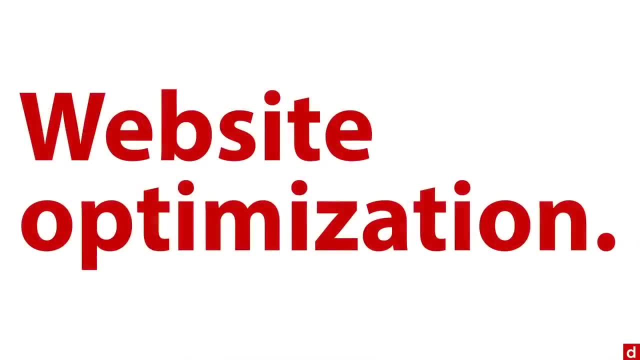 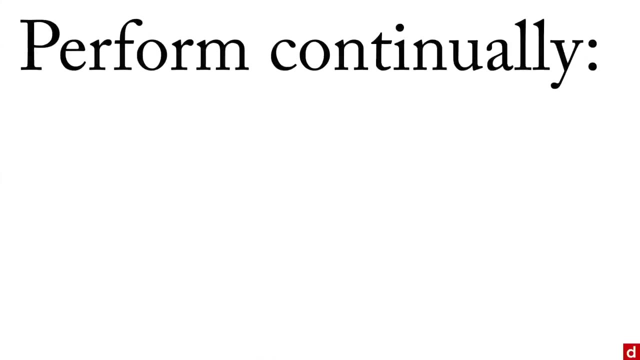 A-B testing to the general concept of website optimization to make your website as effective as it can possibly be. Now, the idea also is that this is something you're going to do a lot. You can perform A-B tests continually. In fact, I've seen one person say that. what A-B testing? 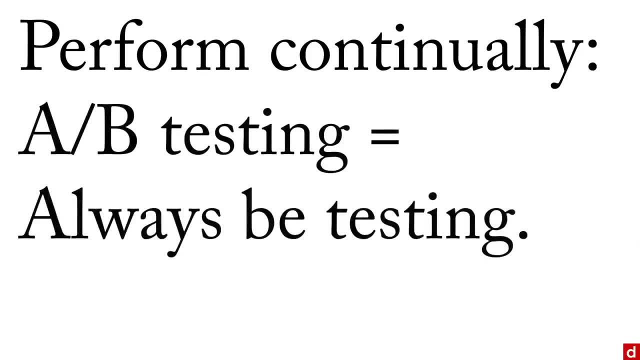 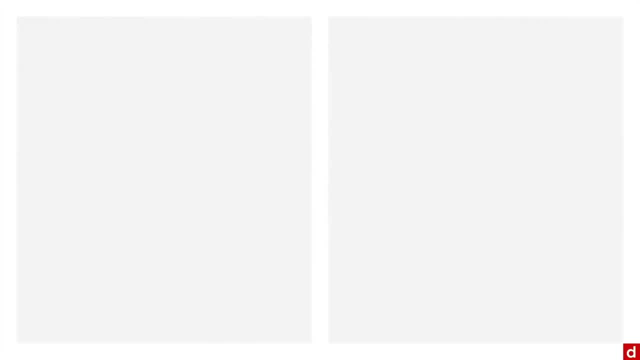 really stands for is always B testing. Kind of cute, but it does give you the idea that improvement is a constant process. Now, if you want some software to do A-B testing, two of the most common choices are Optimizely and VWO, which stands for Visual Web Optimizer- Now many others. 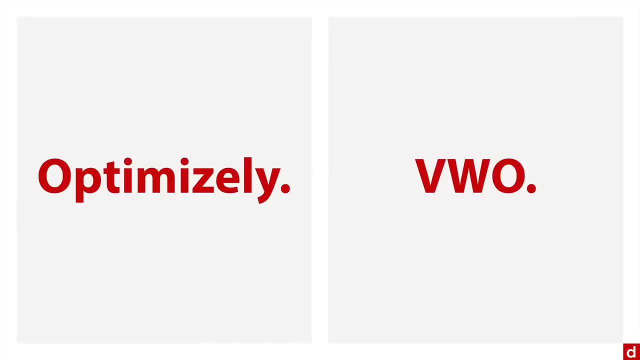 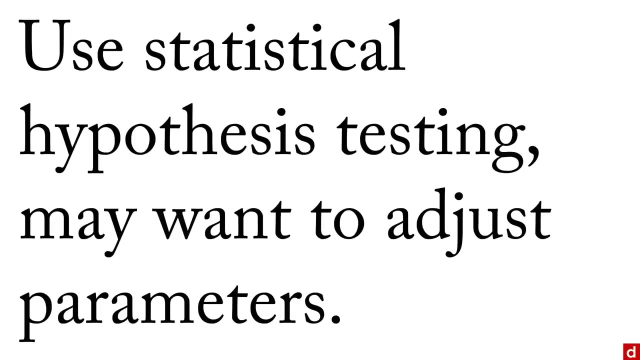 are available, but these are especially common And when you get the data you're going to use statistical hypothesis testing to compare the differences. or really the software does it for you automatically. But you may want to adjust the parameters because most software packages cut off testing a little too soon and the information is not quite as 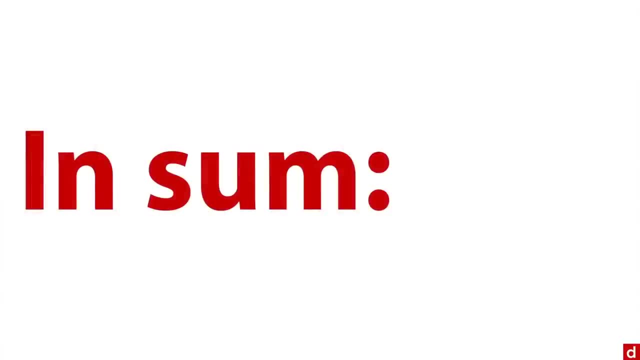 reliable, as it should be. But in sum, here's what we can say about A-B testing. It's a version of website experimentation. It's done online, which makes it really easy to get a lot of data very quickly. It allows you to optimize the design of your website for whatever outcome. 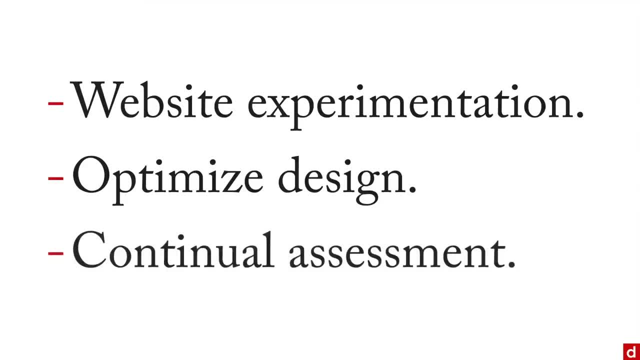 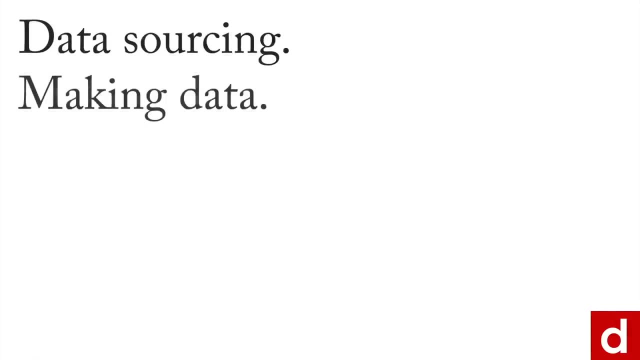 as important to you, And it can be done as a series of continual assessments, testing and development to make sure that you're accomplishing what you want to as effectively as possible for as many people as possible. The next logical step in data: sourcing and making data. 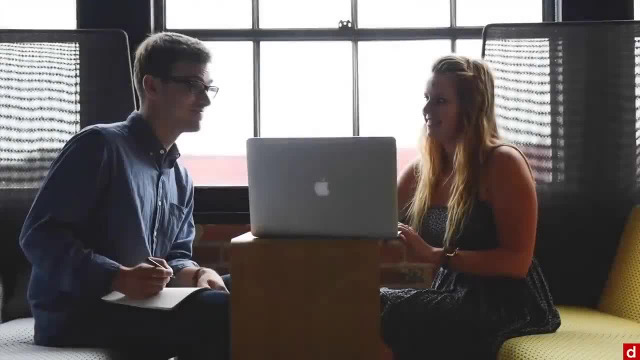 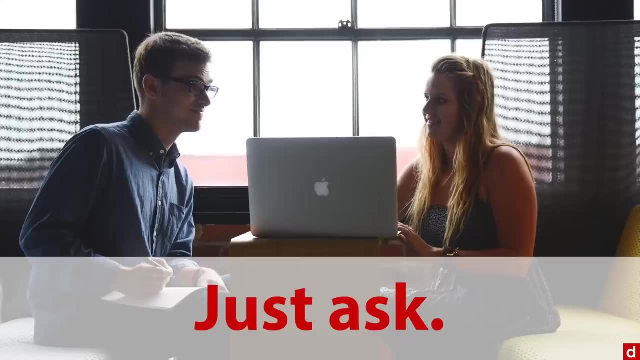 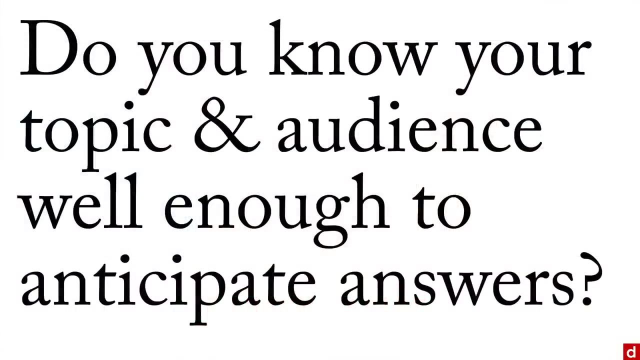 is surveys. Now think of this: if you want to know something, just ask. That's the easy way. And if you want to do a survey, under certain situations. the real question is: Do you know your topic and your audience well enough to anticipate their answers, to know what? 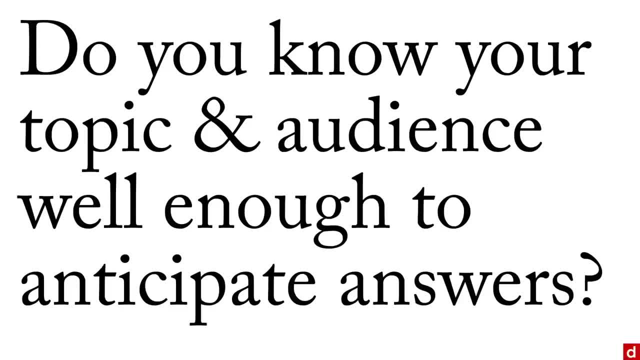 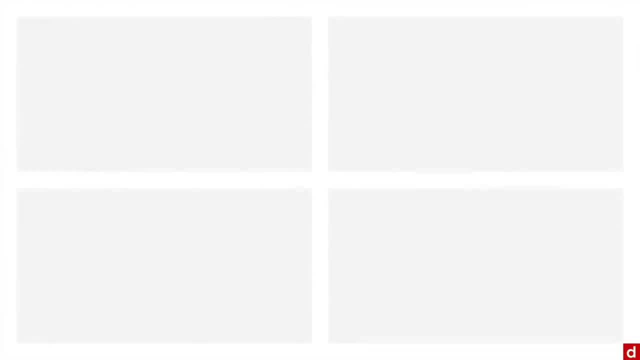 the range of their answers and the dimensions and the categories that are going to be important. If you do, then a survey might be a good approach. Now, just as there were a few dimensions for interviews, there's a few dimensions for surveys. you can do what's called a closed ended survey. 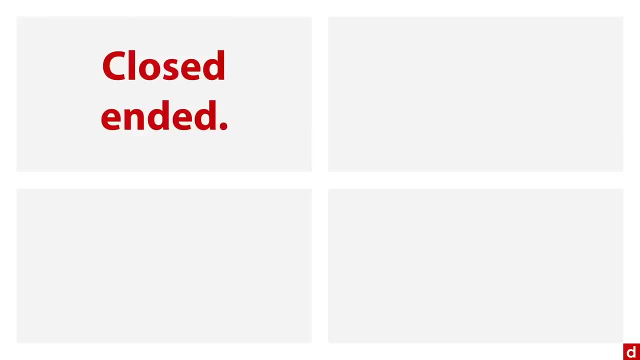 That's also called a forced choice is where you give people just particular options, like a multiple choice. You can have an open ended survey where you have the same questions for everybody but you allow them to write in a free form response. You can do surveys in person And 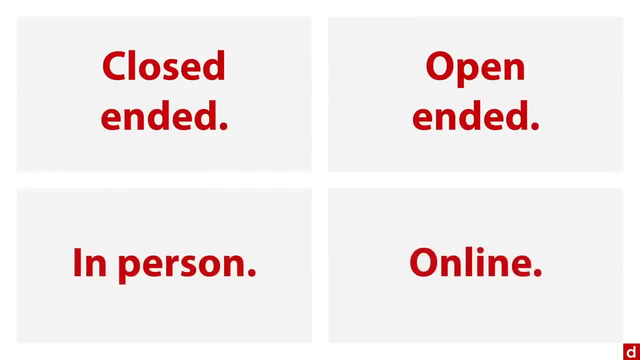 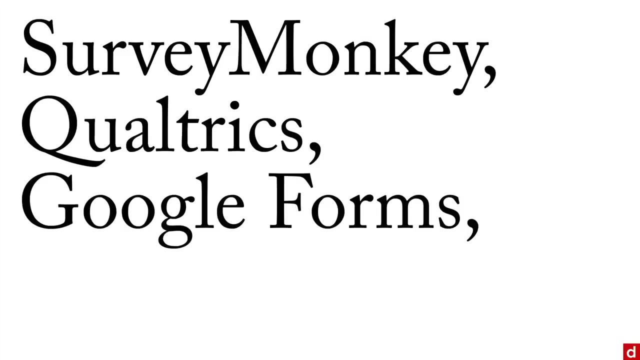 you can also do them online or over the mail or phone, or, however, And now it's very common to use software when doing surveys. Some really common applications for online surveys are SurveyMonkey and Qualtrics, or, at the very simple end, there's Google Forms. And at the simple and pretty end, 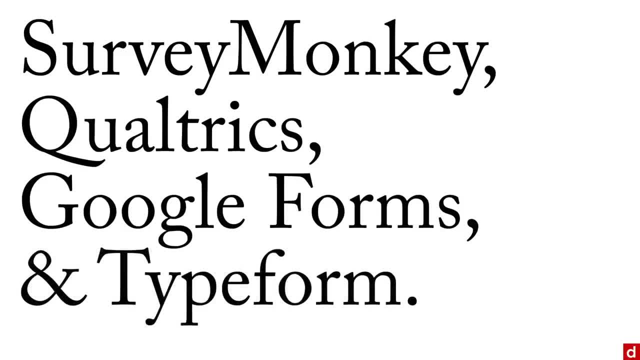 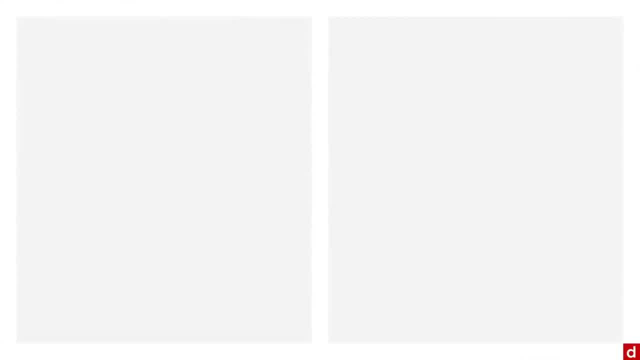 there's Typeform. There's a lot more choices, But these are some of the major players and how you can get data from online participants in survey format. Now, the nice thing about surveys is, you know, they're really easy to do, They're very easy to set up And they're really easy to send out to. 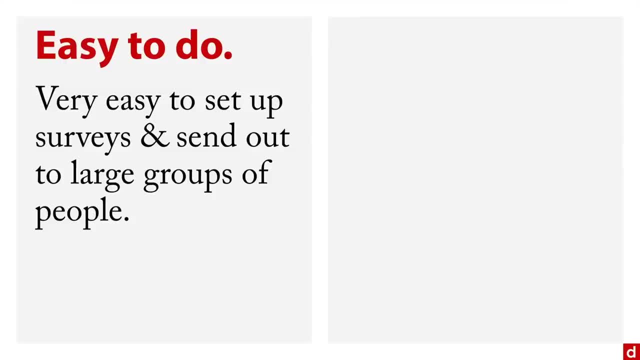 large groups of people, you can get tons of data really fast. On the other hand, the same way that they're easy to do, they're also really easy to do badly. The problem is that the questions you ask, they can be ambiguous, they can be double bearable. 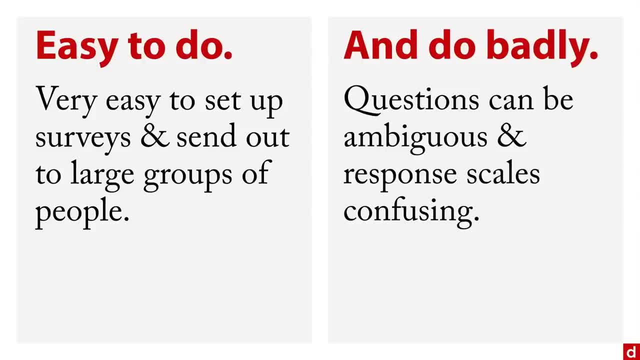 They can be loaded And the response scales can be confusing. So if you say I never think this particular way in a person puts strongly disagree, they may not know exactly what you're trying to get at. So you have to take special effort to make sure that the meaning is clear, unambiguous and 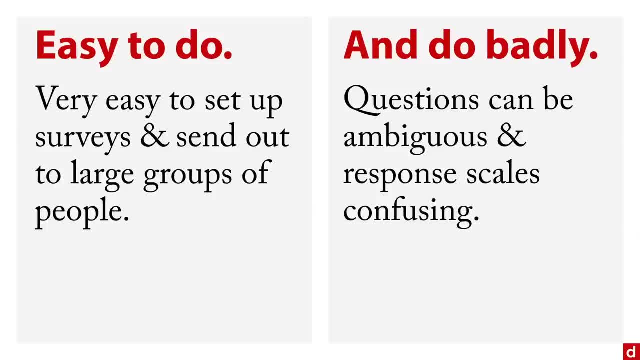 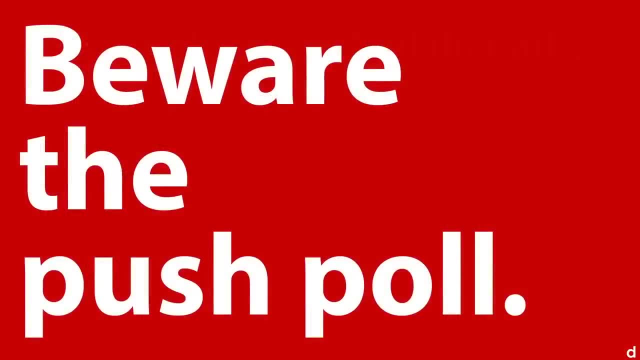 that the rating scale, the way that people respond, is very clear and they know where their answer falls, which gets us into one of the things about people behaving badly, And that is: beware the push pull. During election time, like we're in right now, a push pull is something that sounds like a survey. 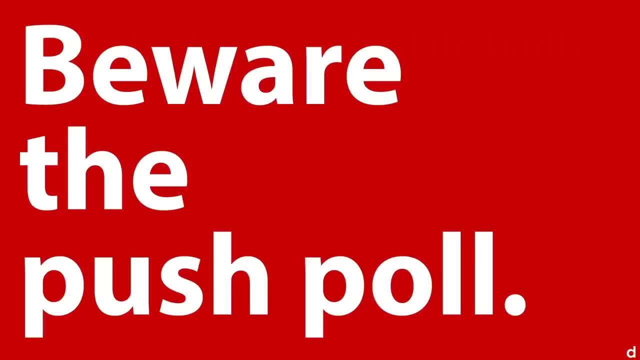 But really what it is is a very biased attempt to get data just fodder for social media campaigns, or I'm going to make a chart that says that 98% of people agree with me. A push pull is one that's so biased there's really only one way to answer to the questions. This is considered extremely. 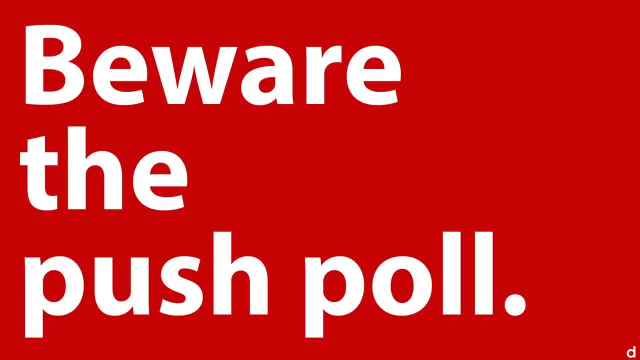 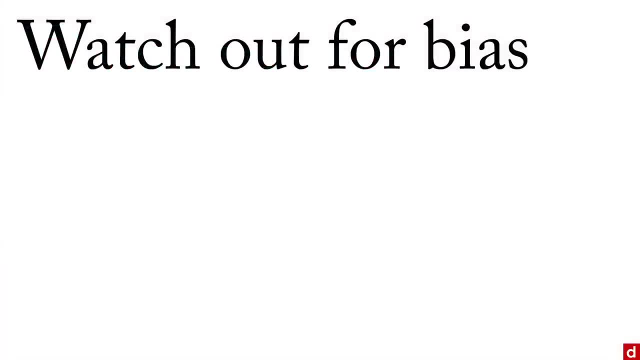 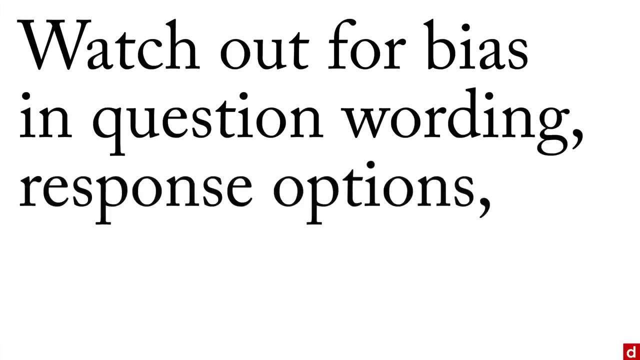 irresponsible and unethical from a research point of view. Just hang up on them Now, aside from that violation of research ethics, you do need to do other things like watch out for bias in the question wording, in the response options and also in the sample selection, because any one of those can push. 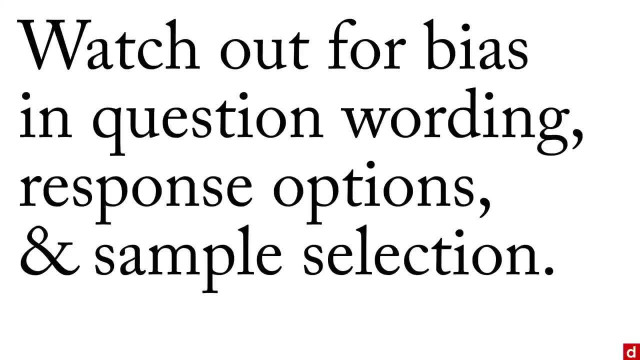 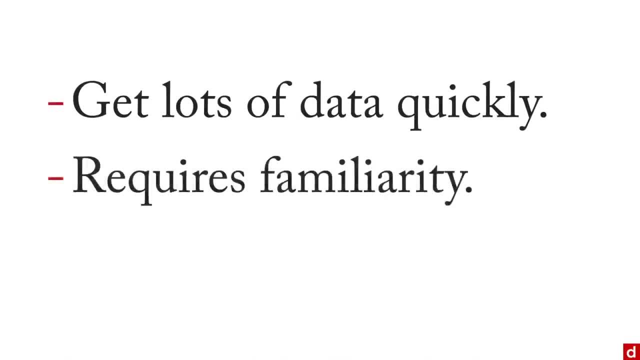 your responses off one way or another without you really being aware that it's happening. So in some- let's say this- about surveys, you can get lots of data quickly. On the other hand, it requires familiarity with the possible answers in your audience, So you know sort of what to expect. 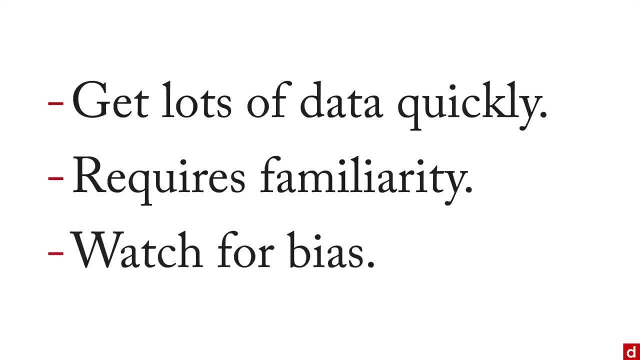 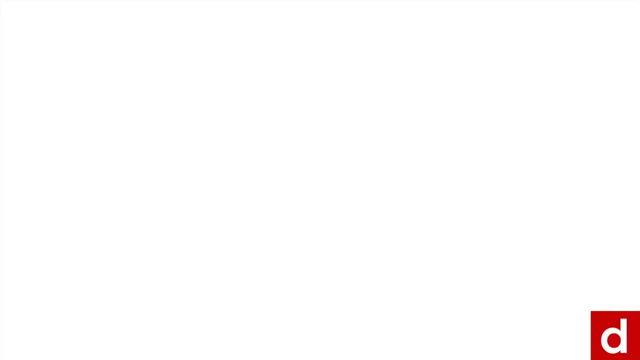 and no matter what you do, you need to watch for bias to make sure that your answers are going to be representative of the group that you're really concerned about understanding. The very last thing I want to talk about in terms of data sourcing is to talk about the next steps And probably the 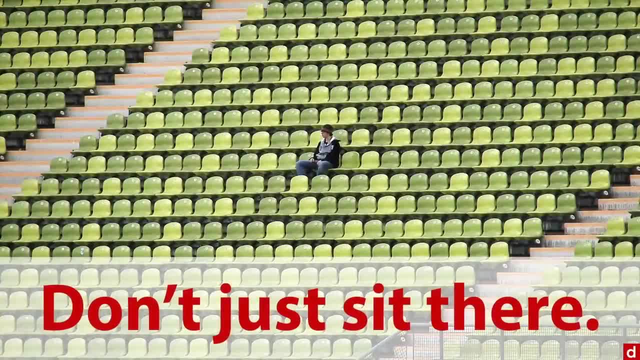 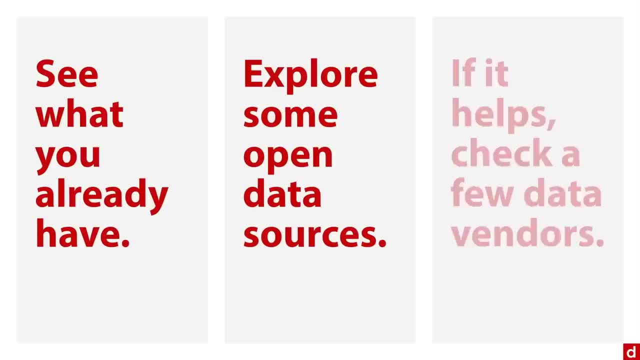 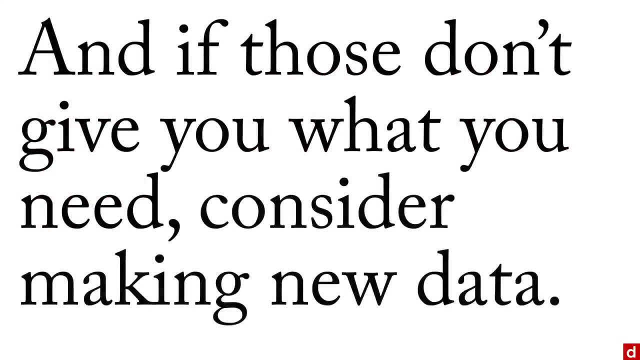 most important thing is you know, don't just sit there. I want you to go and see what you already have. try to explore some open data sources And, if it helps, check with a few data vendors, And if those don't give you what you need to do your project, then consider making new data. 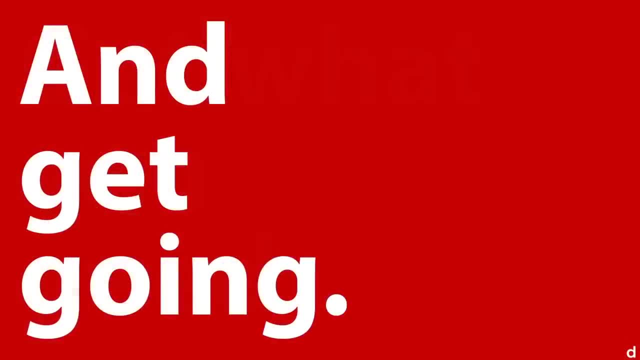 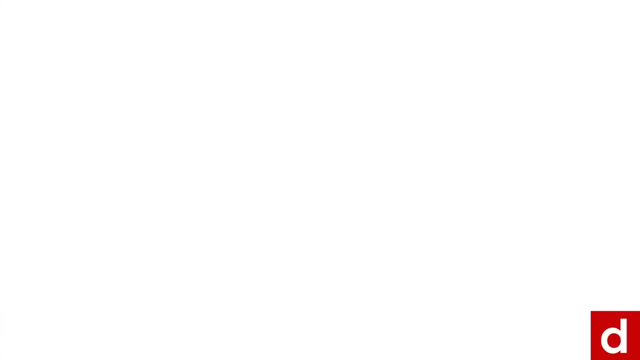 Again, the idea here is: get what you need And get going. Thanks for joining me And good luck on your own projects. Welcome to coding in data science. I'm Bart Poulsen, And what we're going to do in this series of videos is we're going to take a little look at the tools of data science. So 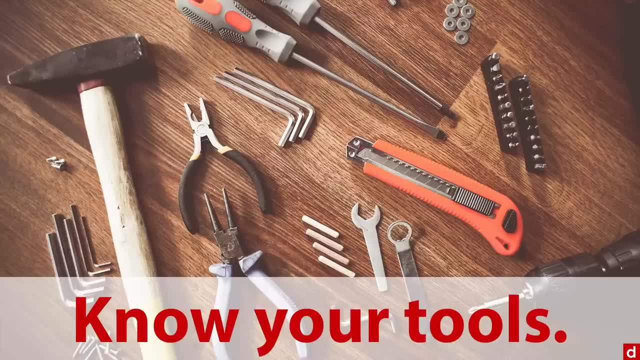 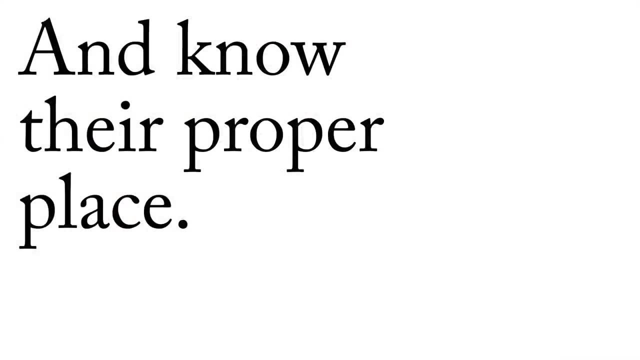 I'm inviting you to know your tools, but probably even more important than that is to know their proper place. Now, I mentioned that because a lot of the times when people talk about data tools, they talk about it as though that were the same. 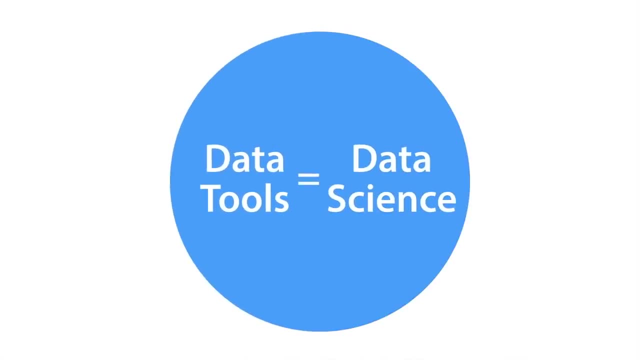 thing as data science, as though they were the same set, But I think, if you look at it for just a second, that's not really the case. Data tools are simply one element of data science, because data science is made up of a lot more than the tools that you use. It includes things like business. 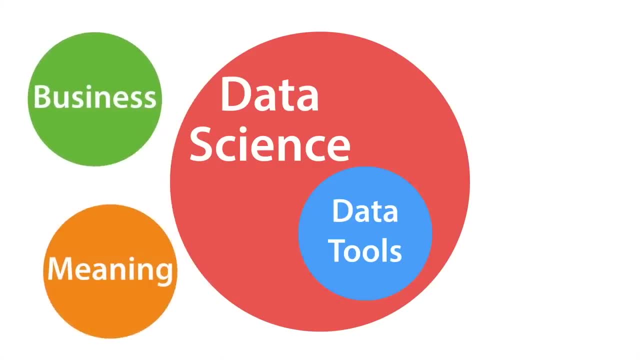 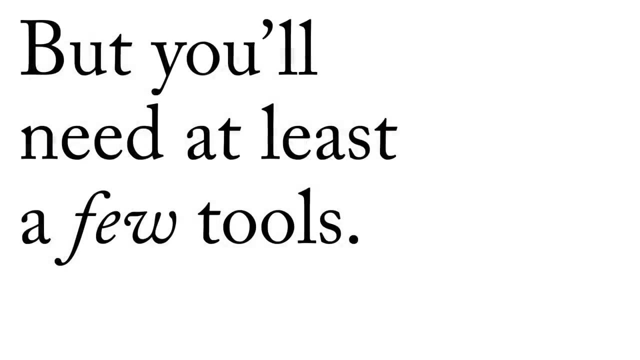 knowledge. it includes the meaning making an interpretation, includes social factors, And so there's much more than just the tools involved. That being said, you will need at least a few tools, And so we're going to talk about some of the things that you can use in data science, if it works well for you. 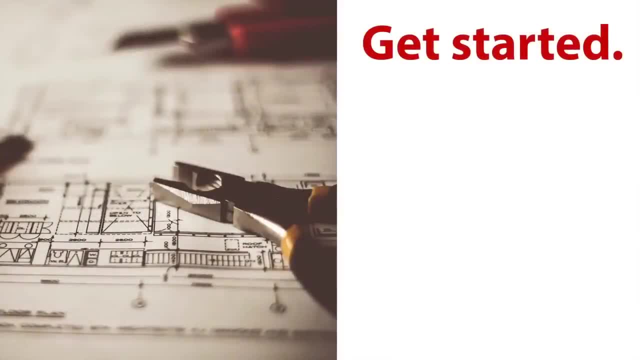 In terms of getting started, the basic things. Number one is spreadsheets. It's the universal data tool And I'll talk about how they play an important role in data science. Number two is a visualization tool. Number two is a visualization tool. Number two is a visualization tool. Number two: 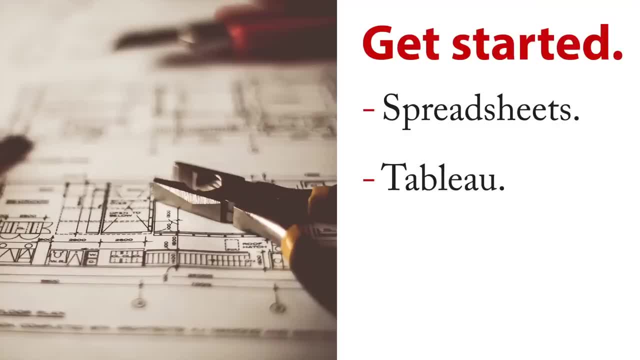 is a visualization program called Tableau. There's Tableau public, which is free, And there's Tableau desktop And there's also something called Tableau server. But Tableau is a fabulous program for data visualization And I'm convinced, for most people, provides the great majority of what they. 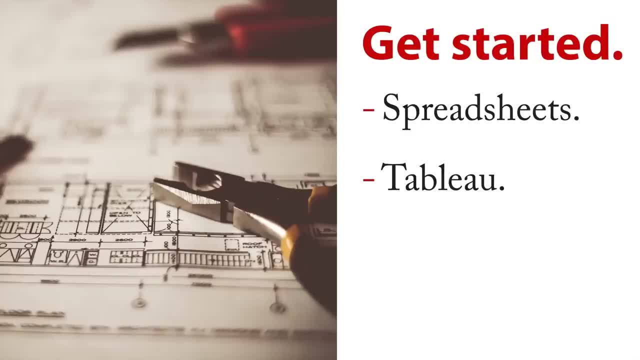 need And, though while it's not a tool, I do need to talk about the formats used in web data, because you have to be able to navigate that when doing a lot of data science work. Then we can talk about some of the essential tools for data science. Those 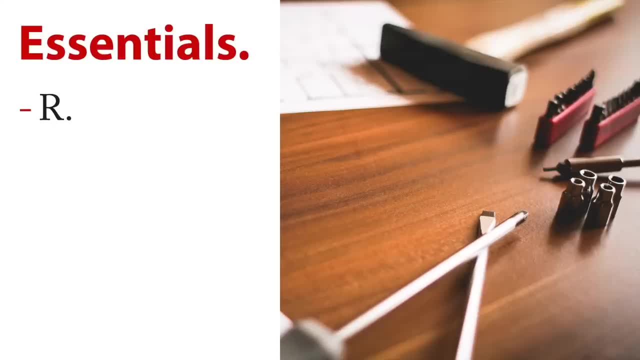 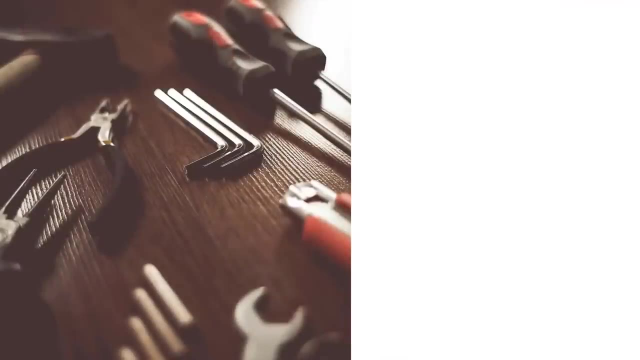 include the programming language R, which is specifically for data. There's the general purpose programming language, Python, which has been well adapted to data, And there's the database language, SQL, or SQL for a structured query language. Then, if you want to go beyond that, 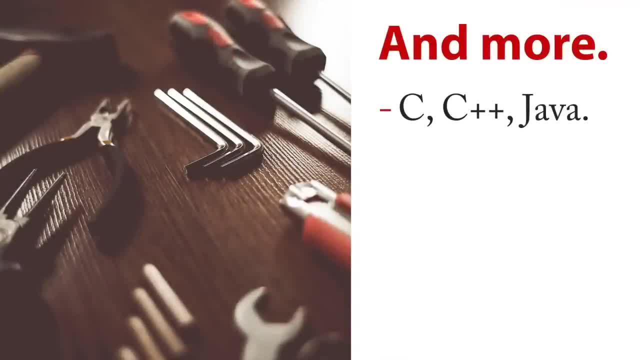 there are some other things that you can do. They're the general purpose programming languages C, C++ and Java, which are very frequently used to form the foundation of data science and sort of the whole area of data science. So there's a lot of different types of programming languages that 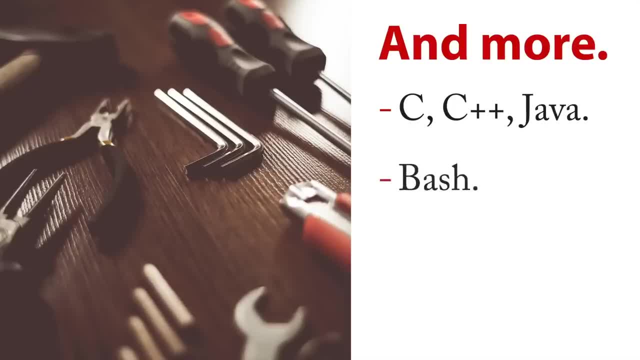 are available. There's the high level. production code is going to rely on those as well. There's the command line interface language, Bash, which is very common as a very quick tool for manipulating data. And then there's the sort of wildcard supercharged regular expressions or regex We'll. 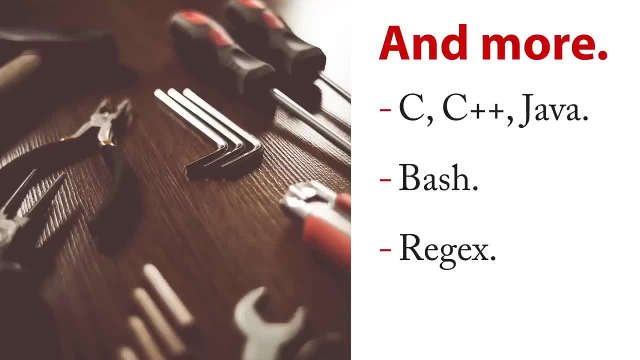 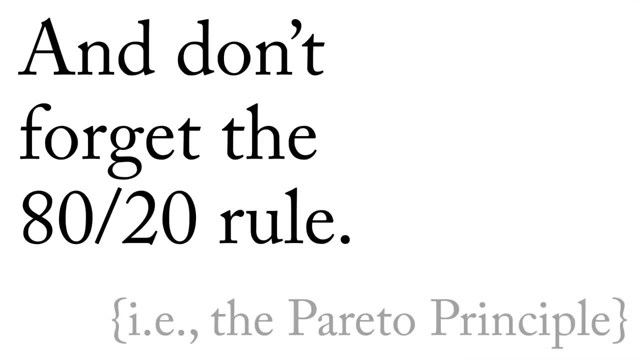 talk about all of these in separate courses, But as you consider all the tools that you can use, the 8020 rule, also known as the Pareto principle, And the idea here is that you're going to get a lot of bang for your buck out of a small number of things, And I'm going to show you a little sample. 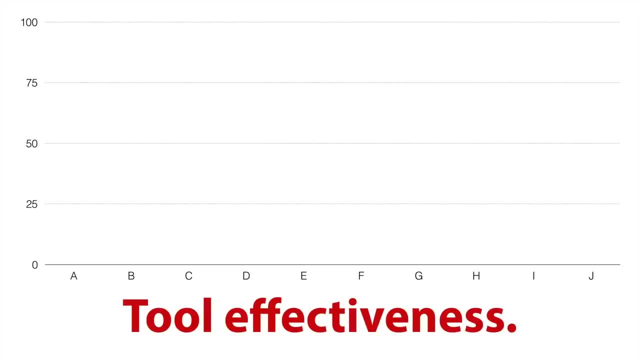 graph here. Imagine that you have 10 different tools and we'll call them A through B. A does a lot for you, B does a little bit less and it kind of tapers down to. you've got a bunch of tools that do just a little bit of stuff that you need Now, instead of looking at the individual. 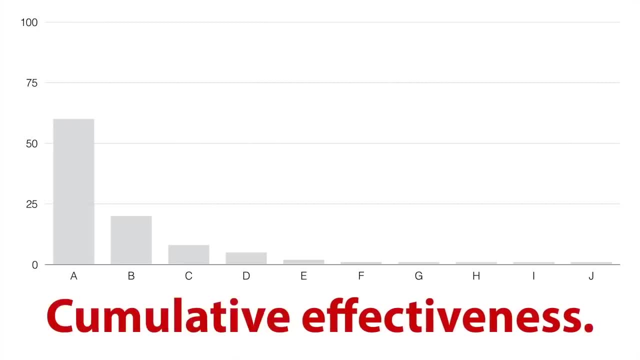 effectiveness. look at the cumulative effectiveness. how much are you able to accomplish with a combination of tools? Well, the first one's right here, at 60%, where the tool started. then you add on the 20% from B and it goes up. and then you add on C and D and you add up little. 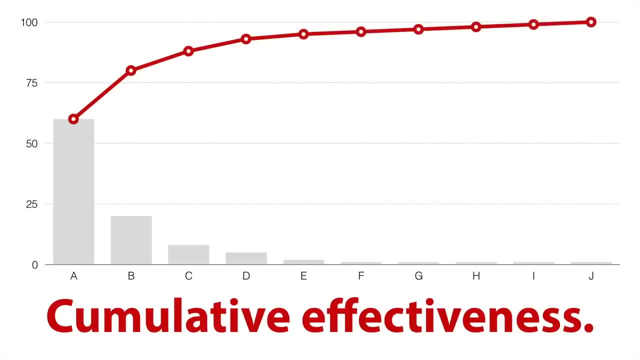 smaller, smaller pieces, And by the time you get to the end, you've got 100% of effectiveness from your 10 tools combined. The important thing about this is you only have to go to the second tool. that's two out of 10.. So that's B, that's. 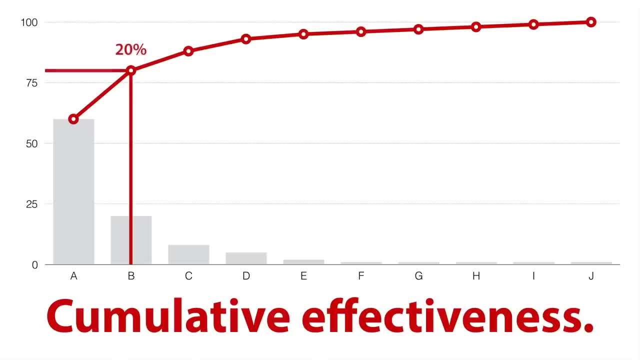 20%, 20% of your tools And in this made up example you've got 80% of your output. So 80% of the output from 20% of the tools. That's a that's a fictional example of the Pareto principle. But 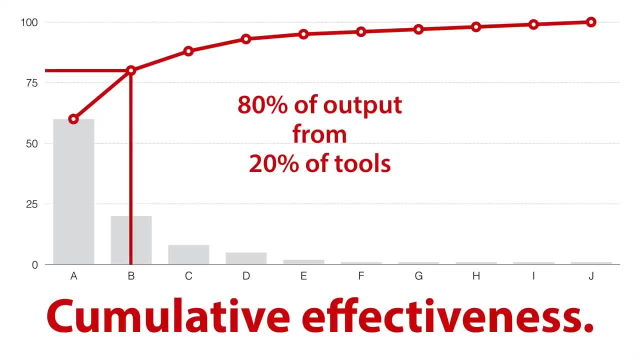 I find in real life, it tends to work something approximately like that, And so you don't necessarily have to learn everything, And you don't have to learn how to do everything in everything. Instead, you want to focus on the tools that will be most productive, and specifically, 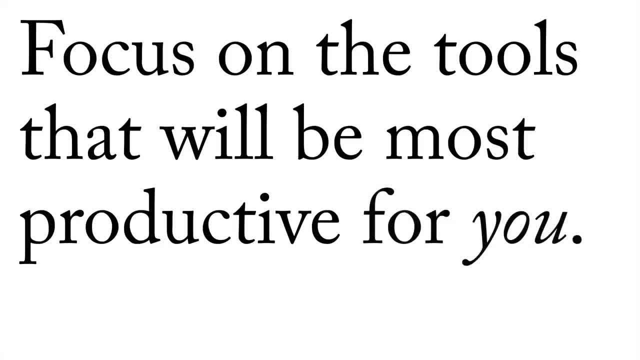 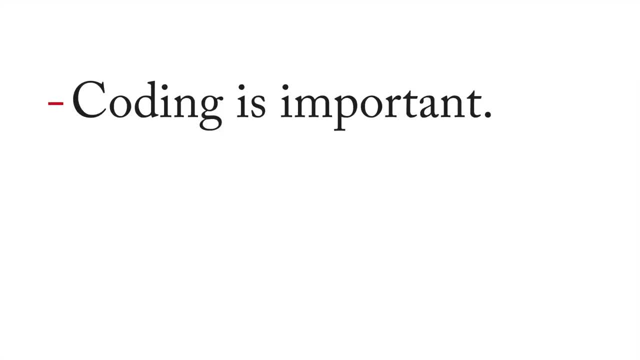 most productive for you. So, in sum, let's say these three things. Number one: coding, or simply the ability to manipulate data with programs and computers. Coding is important, But data science is much greater than the collection of tools that's used in it. And then, finally, as you're, 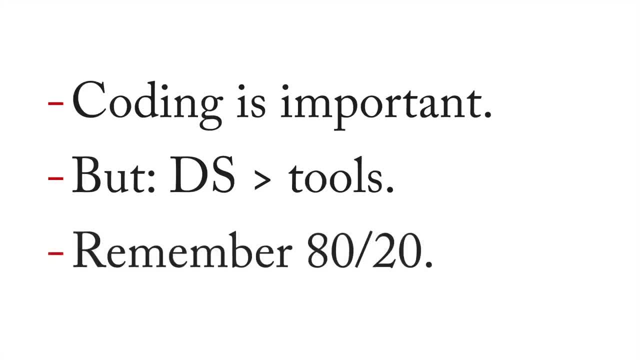 trying to decide what tools to use and what you need to learn and how to work. Remember the 8020 rule: you're going to get a lot of bang from a small set of tools, So focus on the tools that are going to be most useful for you and conducting your own data science projects As we begin our 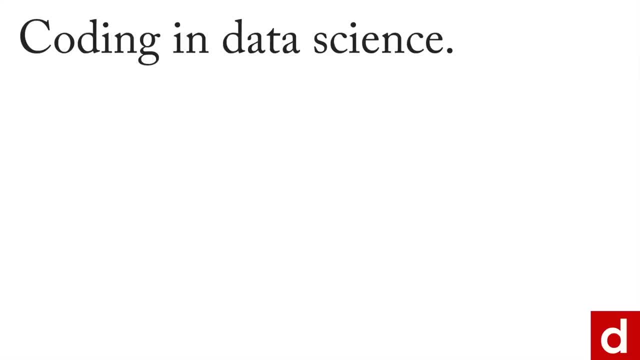 discussion of coding and data science. I actually want to begin with something that's not coding. I want to talk about applications or programs that are already created that allow you to manipulate data, And we're going to begin with the most basic of these spreadsheets. We're going to 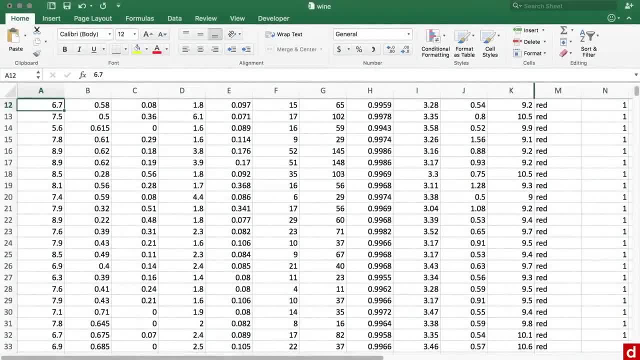 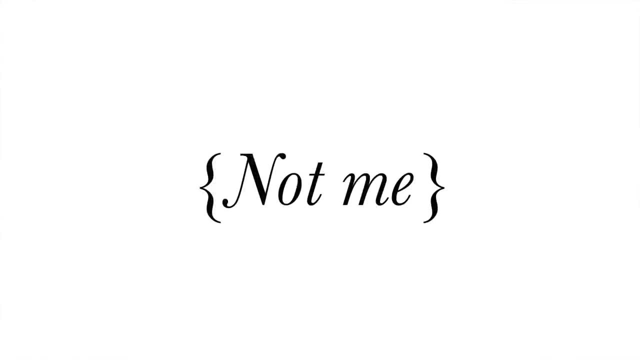 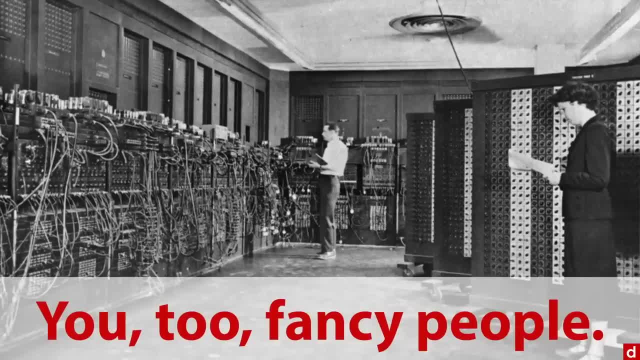 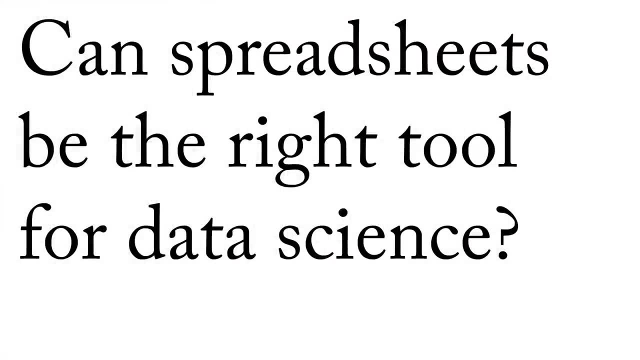 things going on, But you know what. you too fancy people. you need spreadsheets as well. There's a few reasons for this. Most importantly, spreadsheets can be the right tool for data science in a lot of circumstances. There are a few reasons for that. Number one: spreadsheets. 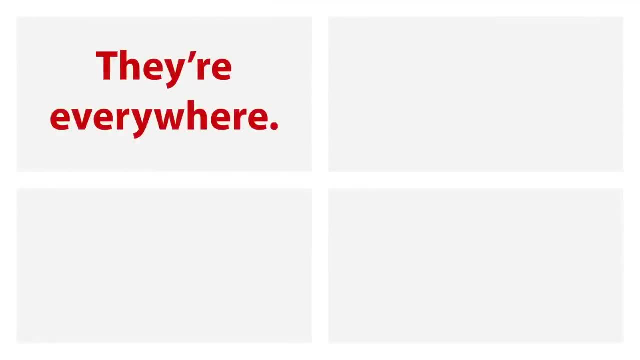 they're everywhere, they're ubiquitous, they're installed on a billion machines around the world And everybody uses them. they probably have more data sets in spreadsheets than anything else, And so it's a very common format. Importantly, it's probably your clients format. 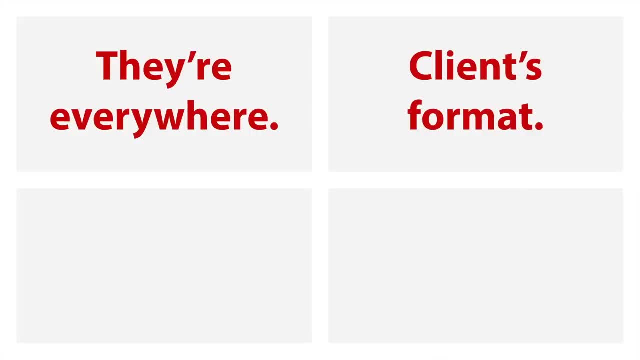 A lot of your clients are going to be using spreadsheets for their own data. I've worked with billion dollar companies that keep all of their data in spreadsheets, And so when you're working with them, you need to know how to manipulate that and how to work with it Also. 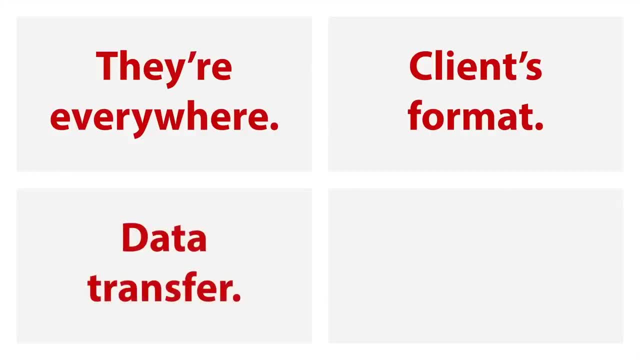 regardless of what you're doing. spreadsheets, specifically CSV, comma separated value files, are sort of the lingua franca, the universal interchange format for data transfer, to allow you to take it from one program to another And then, truthfully, in a lot of situations they're really easy to use And, if you want, 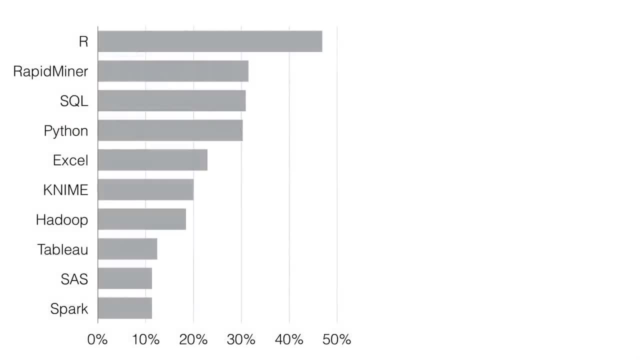 a second opinion on this. let's take a look at this ranking. There's a survey of data mining experts- it's the KD nuggets data mining poll, And these are the tools they most use in their own work. And look at this lowly: Excel is fifth on the list. And in fact, what's interesting about it? 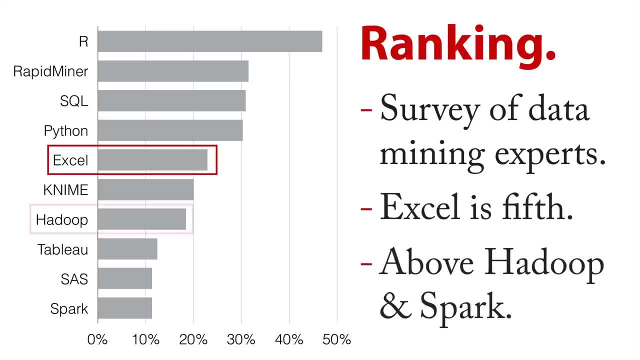 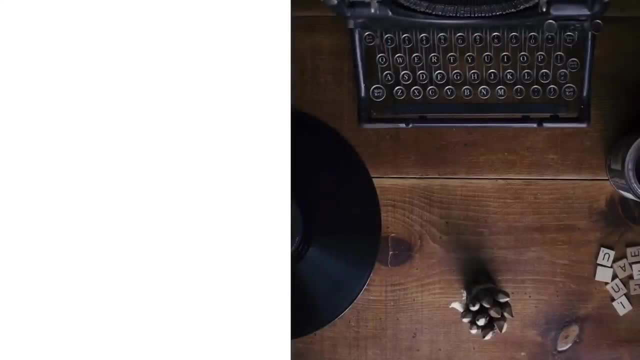 it's above Hadoop and spark, two of the major big data fancy tools, And so Excel really does have place of pride in a toolkit for a data analyst. Now, since we're going to going to sort of the low tech end of things, let's talk about some of the things that you can do with a spreadsheet. 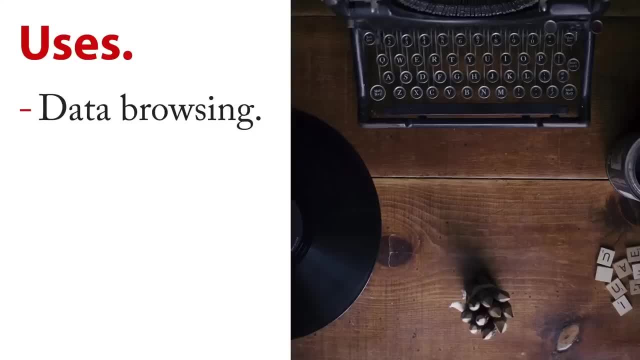 Number one. they're really good for data browsing. you actually get to see all the data and the data that's in front of you, which isn't true if you're doing something like our Python. they're really good for sorting data. sort by this column than this column than this. 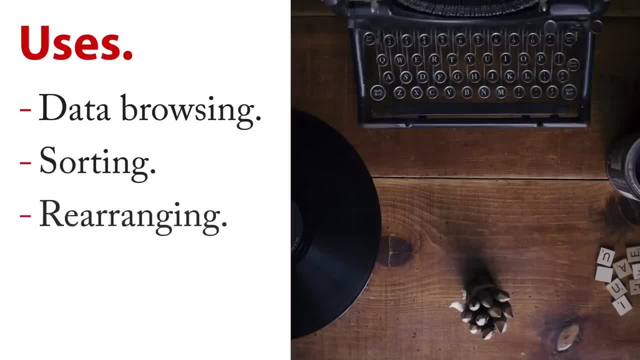 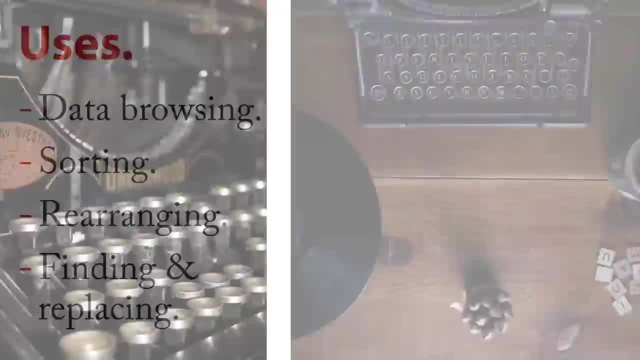 column. They're really good for rearranging columns and cells and moving things around. They're good for finding and replacing and seeing what happens. So you know that it worked right. Some more uses: They're really good for formatting, especially conditional formatting. 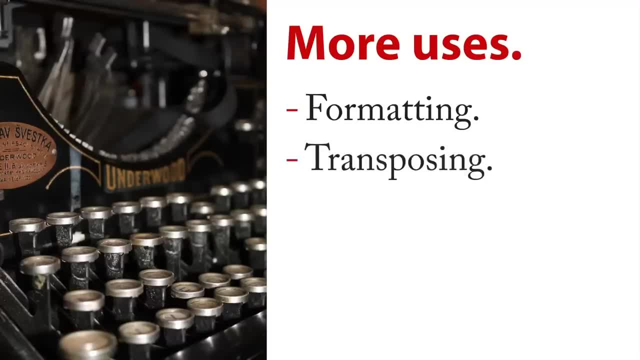 They're good for transposing data, switching the rows and the columns- they make that really easy. Now, it's true, if you're a big, fancy data scientist, you're probably using GitHub, But for everybody else in the world, spreadsheets and the tracking changes is a wonderful way to do it. You. 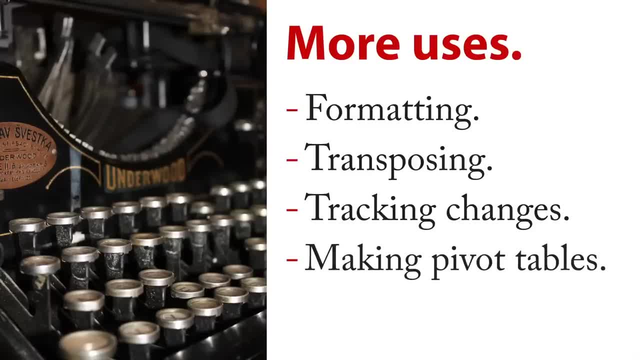 can make pivot tables. that allows you to explore the data in a very hands on way, in a very intuitive way, And they're also really good for arranging the output for consumption. Now, when you're working with spreadsheets, however, there's one thing you need to be aware of. they're really 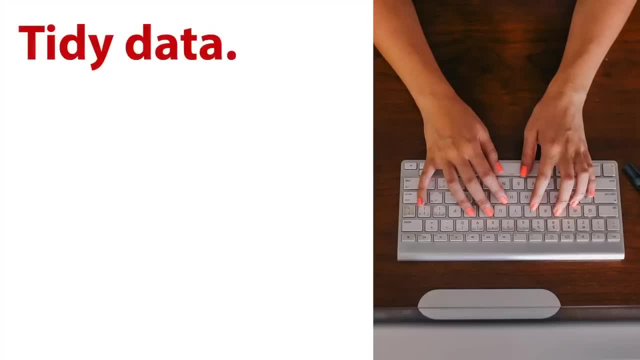 flexible, But that flexibility can be a problem And that when you're working in data science, you specifically want to be concerned about something called tidy data. That's a term I borrowed from Hadley Wickham, very well known developer in the R world. Tidy data is for: 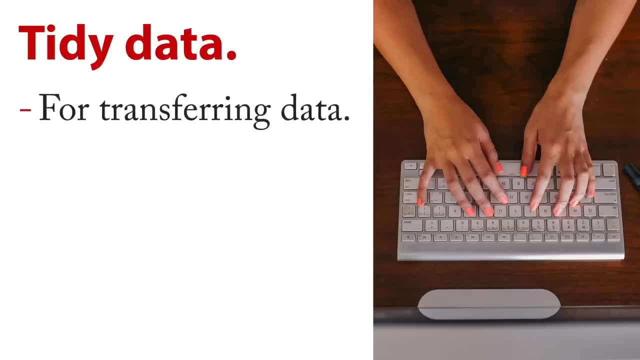 transferring data and making it work. Well, there's a few rules here that undo some of the flexibility inherent in spreadsheets. Number one: what you want to do is have a column be equivalent to the same thing as a variable. columns, variables. 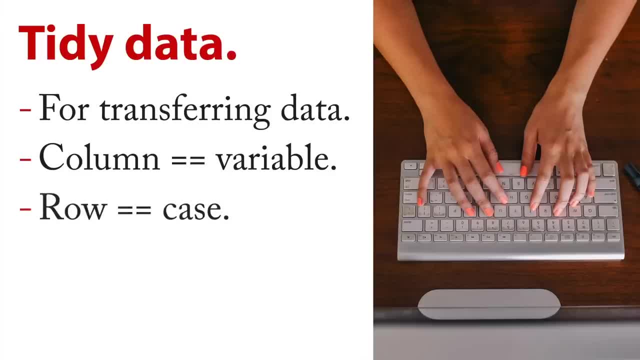 they are the same thing, And then rows are equal, exactly the same thing as cases, And then you have one sheet per file And then you have one level of measurement, say individual, then organization, then state per file. Again, this is undoing some of the flexibility that's inherent. 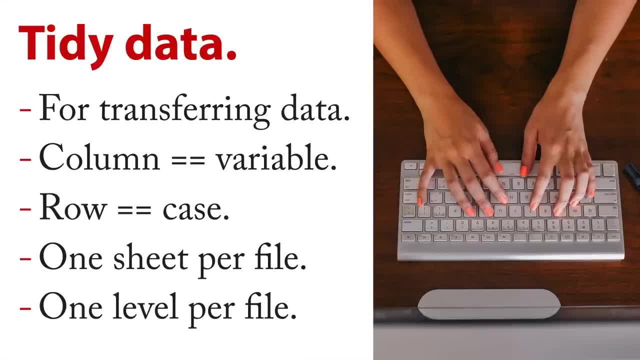 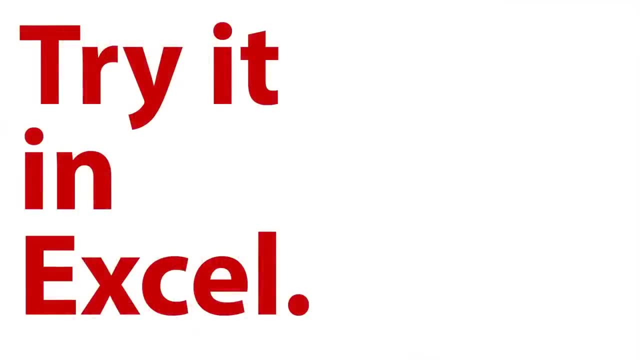 in spreadsheets, But it makes it really easy to move the data from one program to another. Let me show you how all this works. You can try this in Excel If you've downloaded the files for this course. we simply want to open up this spreadsheet. Let me go to Excel and show. 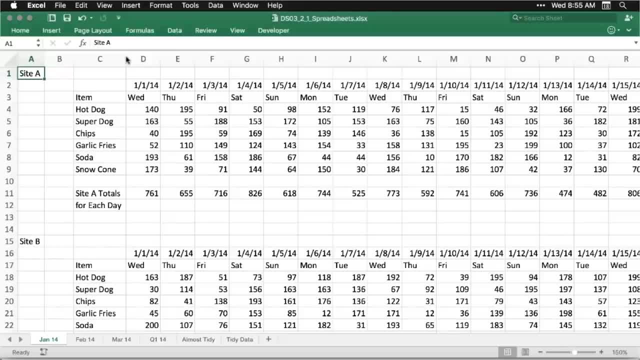 you how it works. So when you open up the spreadsheet, what you get is totally fictional data here that I made up, but it's showing sales over time of several products at two locations, like if you're selling stuff at a baseball field, And this is the way spreadsheets often appear. 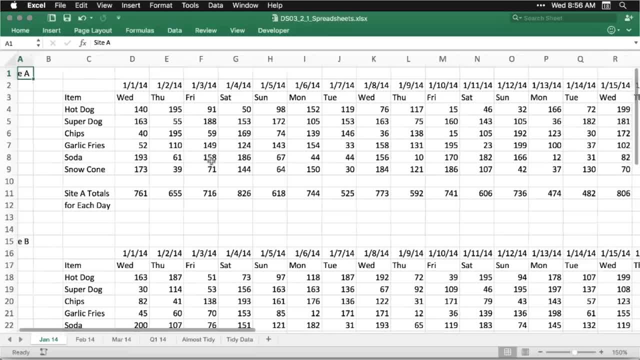 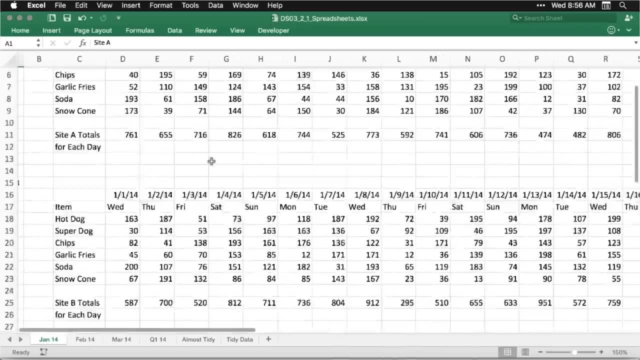 we got blank rows and columns, we got stuff arranged in a way that makes it easy for the person to process it, And we got totals here and with formulas putting them all together And that's fine, that works well for the person who made it, And then that's for one month, And then 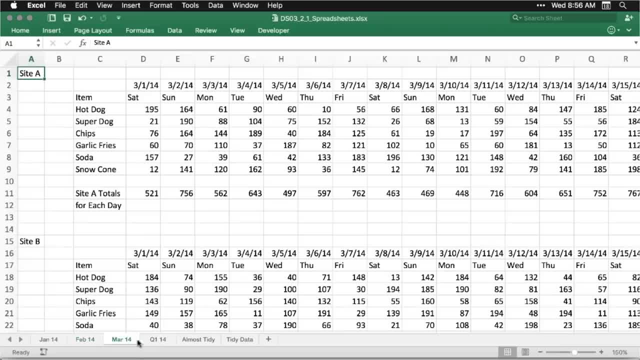 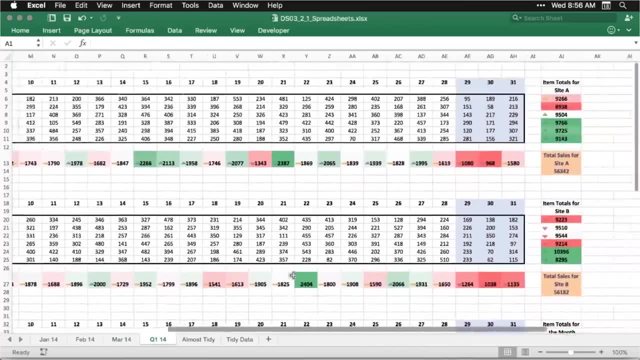 we have another month right here, And then we have another month right here, And then we combine them all for the first quarter of 2014.. We've got some headers here, we've got some conditional formatting and changes And if we come to the bottom, we've got a very busy line graphic that 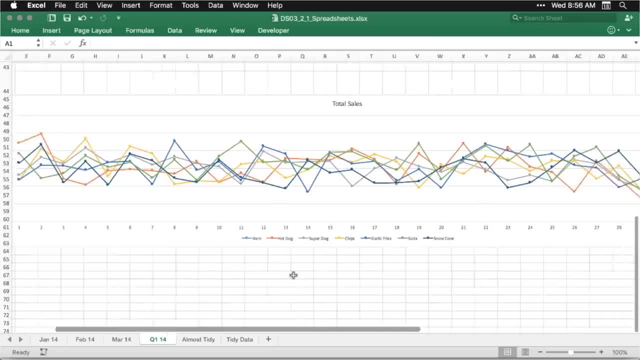 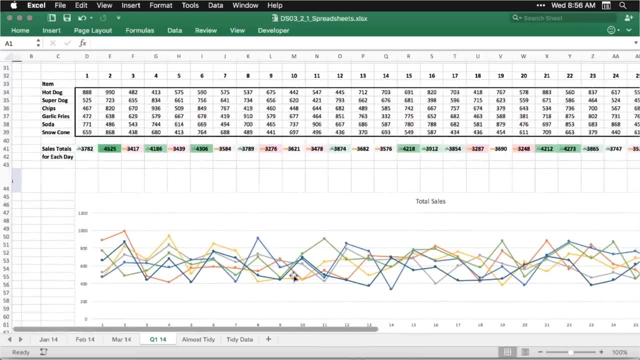 eventually loads. It's not a good graphic, by the way, But similar to what you will often find. So this is the stuff that well, it may be useful for the client's own personal use. you know you can't feed this into our Python and it'll just. 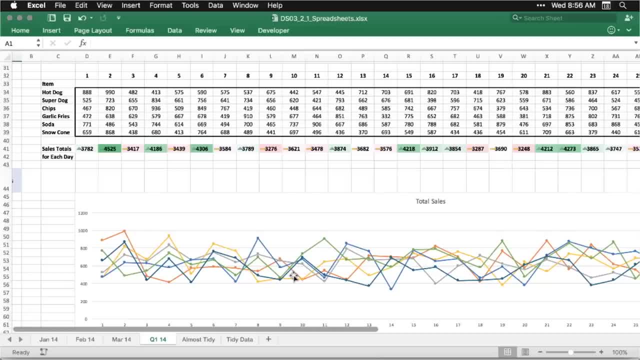 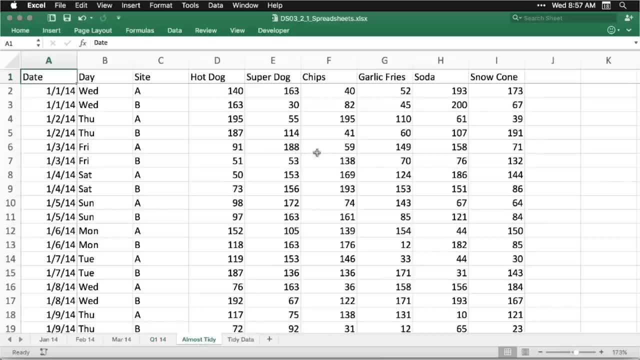 choke and it won't know what to do with it, And so you need to go through a process of tidying up the data, And what this involves is undoing some of this stuff. So, for instance, here's data that is almost tidy. Here we have a single column for the date, a single column for the day. 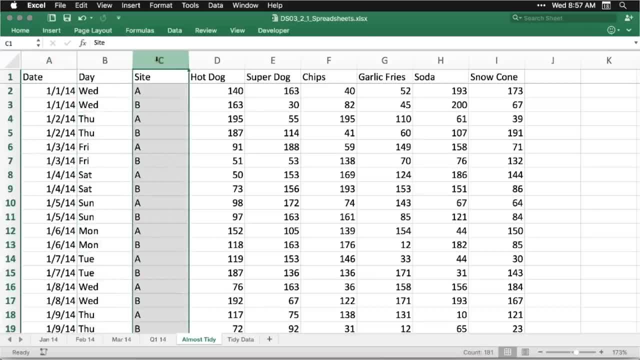 a column for the site that. so we have two locations, A and B, And then we have six columns for the six different things that are sold and how many were sold on each day. Now, in certain situations, you would want the data laid out exactly like this. If you're doing, for instance, 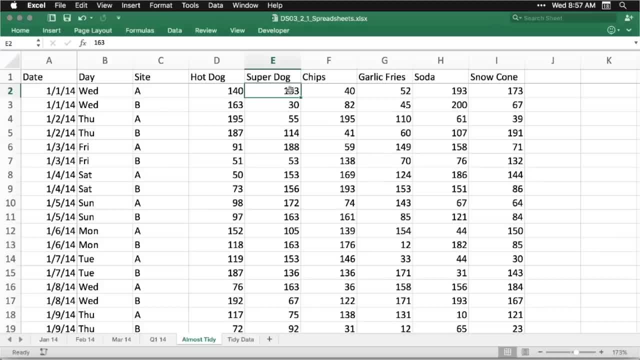 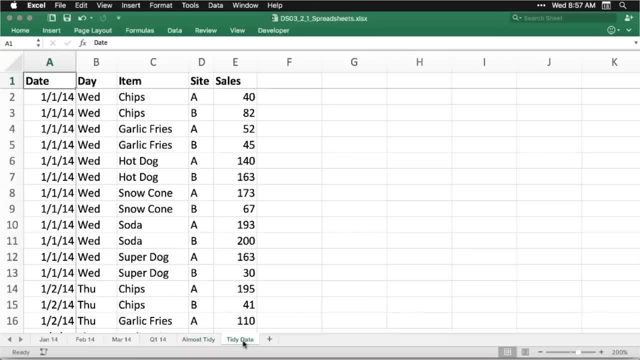 a time series, you'll do something vaguely similar to this, But for true tidy stuff. we're going to collapse it even further. Let me come here to the tidy data. And now what I've done is I've created a new column that says what is the item being sold. 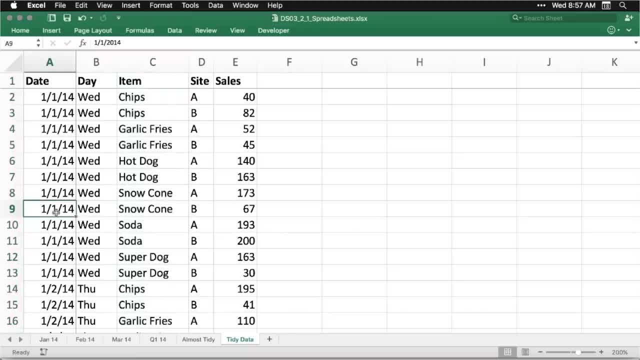 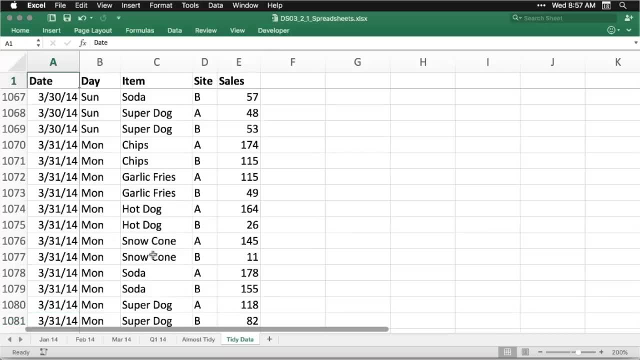 And so, by the way, what this means is that we've got a really long data set. Now it's got over 1000 rows. come back up to the top here, But what that shows you is that now it's a in a format that's. 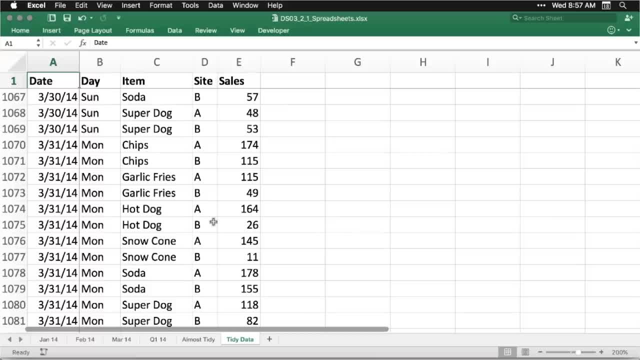 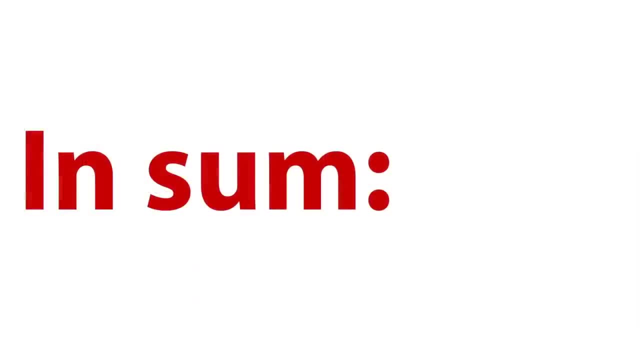 really easy to import from one program to another. that makes it tidy and you can remanipulate it however you want once you get to each of those. So let's sum up our little presentation here in a few lines. Number one: no matter who you are, no matter what you're doing in data science, you 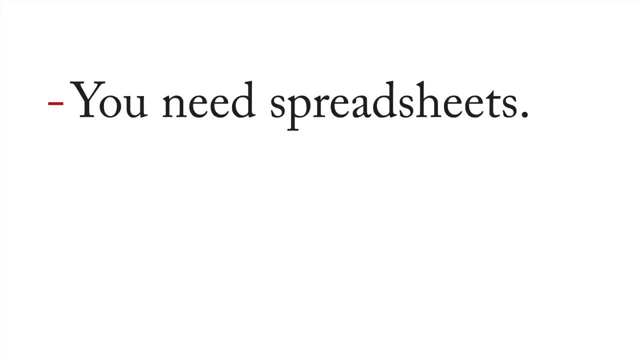 need spreadsheets, And the reason for that is that spreadsheets are often the right tool for data science. Keep one thing in mind, though, and that is, as you're moving back and forth from one language to another, tidy data, or well formatted data, is going to be important for exporting data. 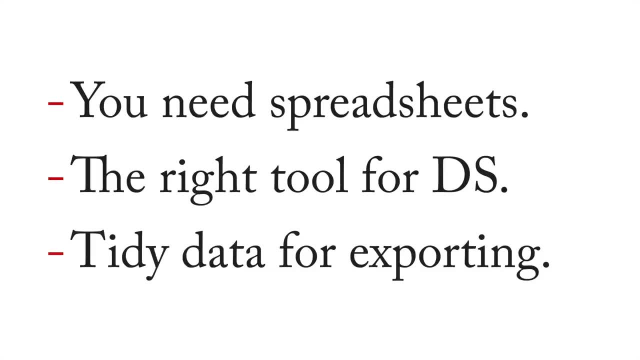 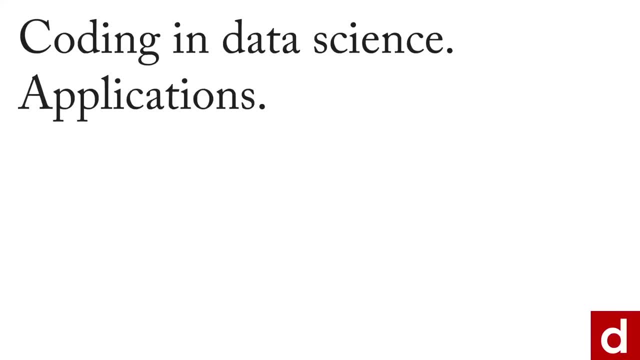 into your analytical program or language of choice. As we move through coding and data science and specifically, the applications that can be used, there's one that stands out for me more than anything else, And that's Tableau, and Tableau public. Now, if you're not familiar with these, 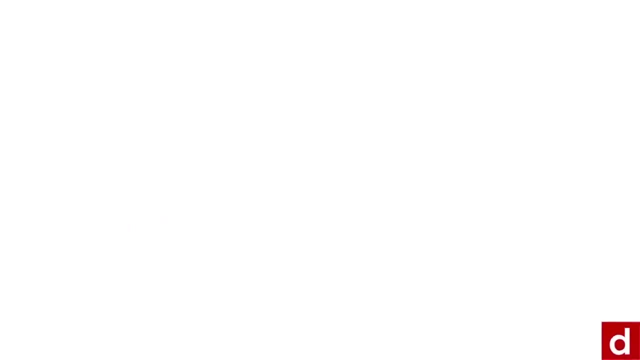 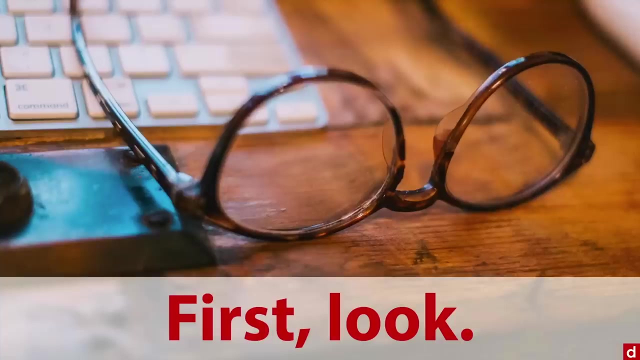 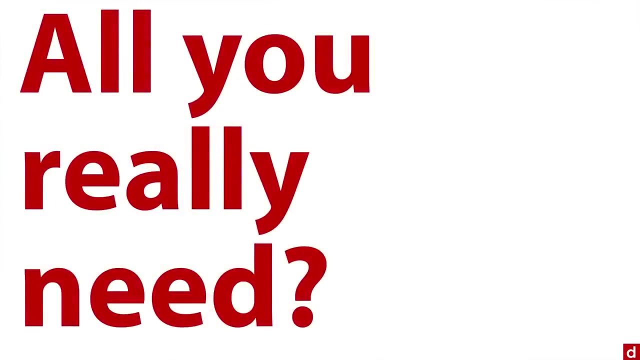 these are visualization programs. The idea here is that when you have data, the most important thing you can do is to first look and see what you have and work with it from there, And in fact I'm convinced that for many organizations, Tableau might be all that they really need. 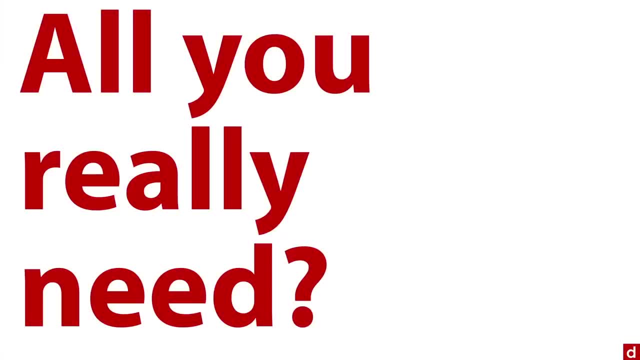 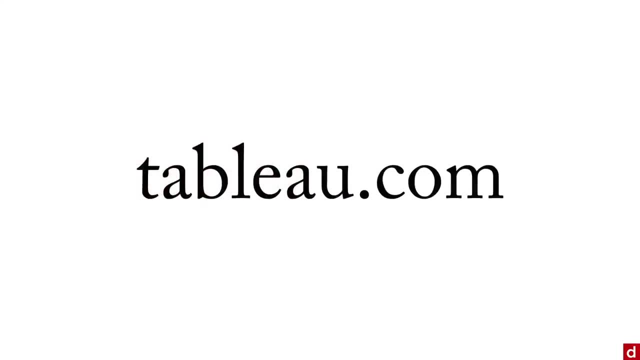 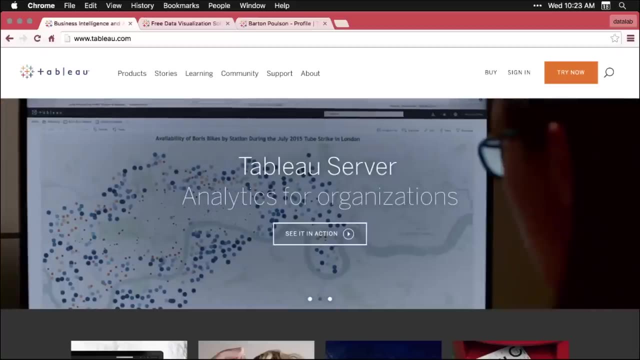 it will give them the level of insight that they need to work constructively with data. So let's take a quick look by going to tableaucom Now. there are a few different versions of Tableau. Right here we have Tableau desktop and Tableau server, And these are the. 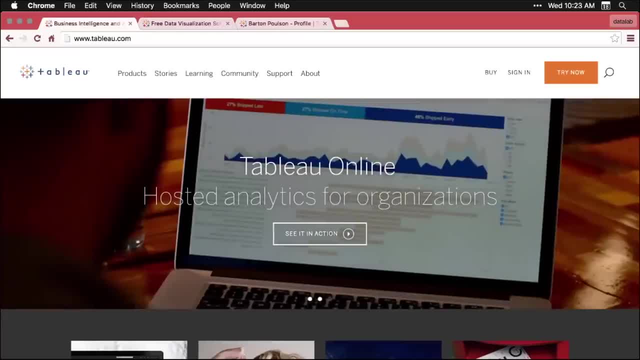 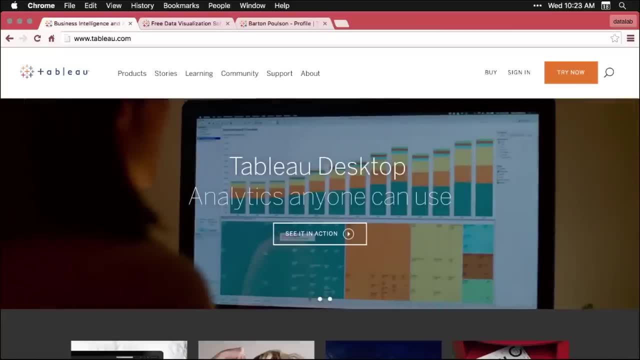 paid versions of Tableau. they actually cost a lot of money, unless you work for a nonprofit organization, in which case you can get them for free, which is a beautiful thing. What we're usually looking for, however, is a lot of money, And that's because we don't have a lot of money. 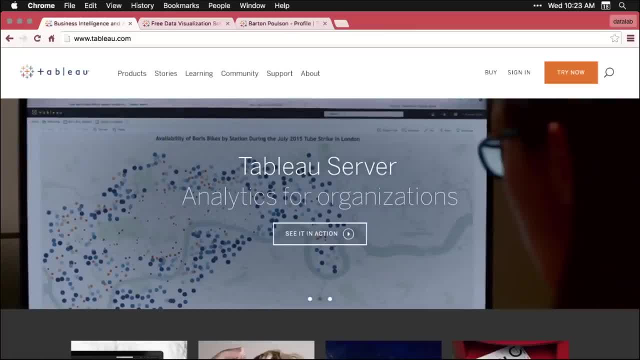 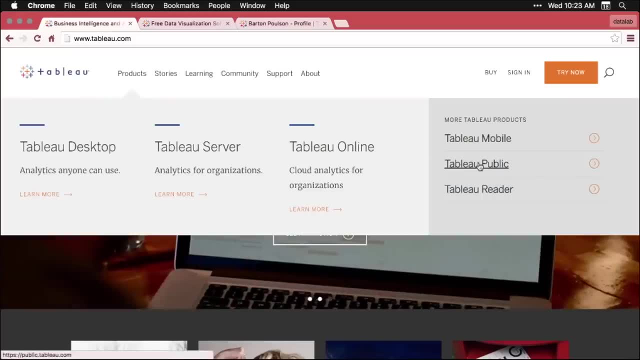 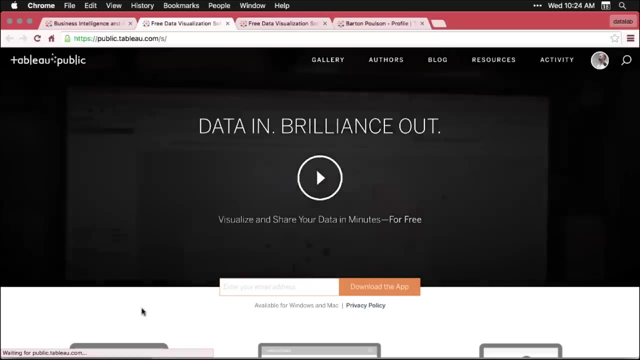 It's not this paid version, but we're looking for something called Tableau public And if you come in here and go to products and we've got these three paid ones over here to Tableau public, When we click on that it brings us to this page. it's publictableaucom. 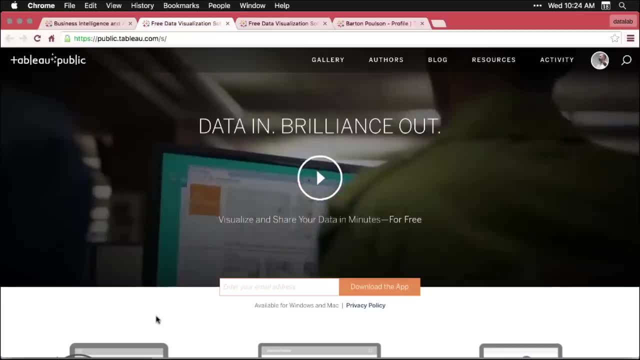 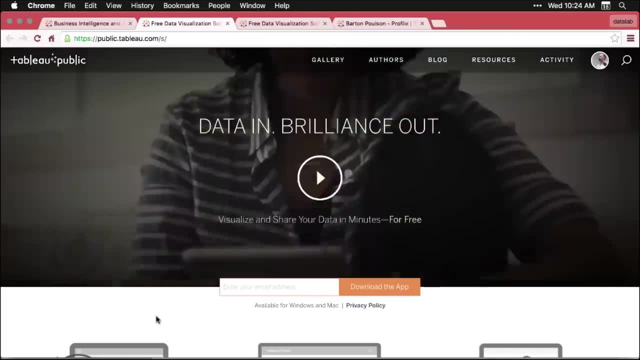 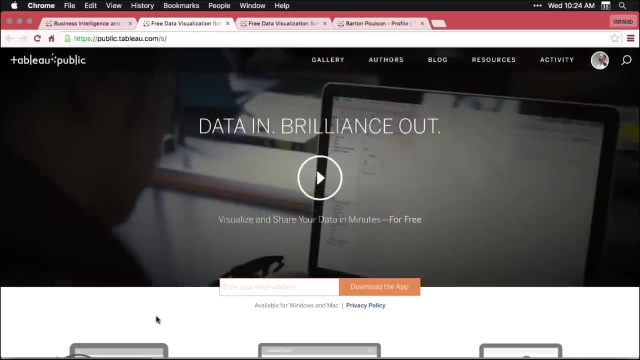 And this is the one that has what we want. It's a free version of Tableau, With one major caveat: you don't save files locally to your computer, which is why I didn't give you a file to open. Instead, it saves them to the web in a public form. So if you're willing to trade, 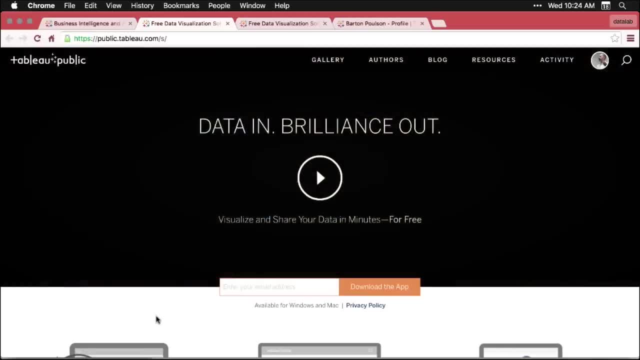 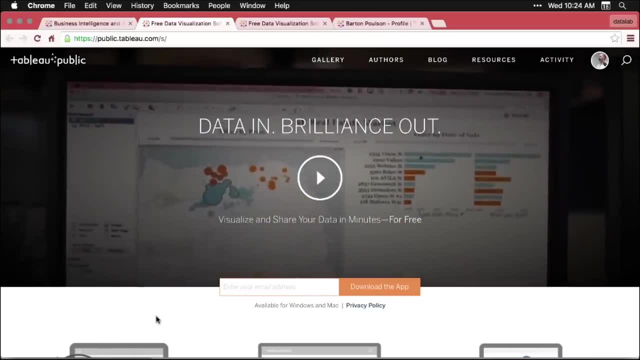 privacy, you can get an immensely powerful application for data visualization. That's a catch for a lot of people, which is why people are willing to pay a lot of money for the desktop version. And again, if you work for a nonprofit, you can get the desktop version for free. But I'm 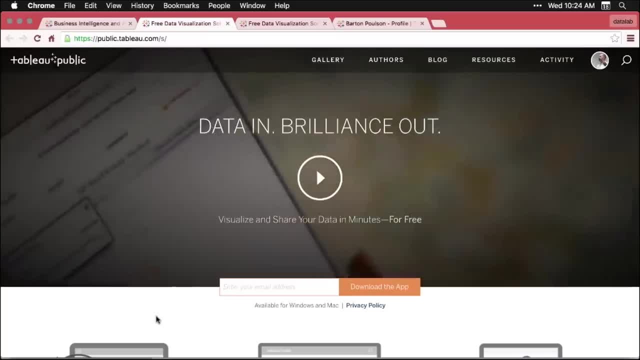 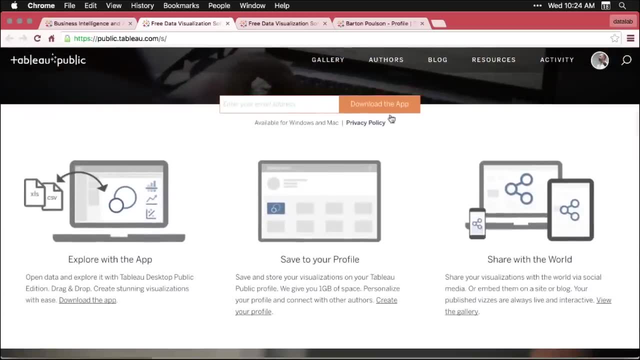 going to show you how things work in Tableau public, So that's something that you can work with personally. The first thing you want to do is you want to download it, And so you put in your email address. you download, it's going to know what you're on. It's a pretty big download And once it's, 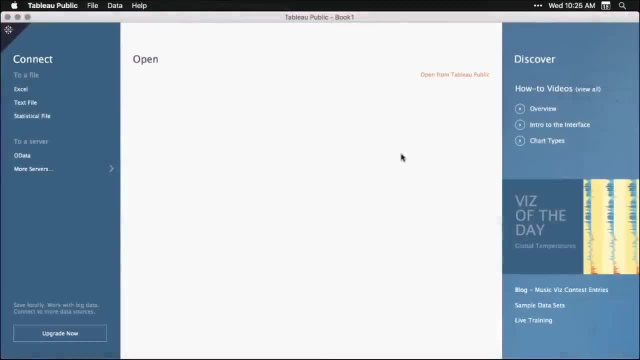 downloaded, you can install and open up the application. And here I am in Tableau public, right here. this is the blank version. By the way, you also need to create an account with Tableau in order to save your stuff online and to see it. we'll show you what that looks like, But you're 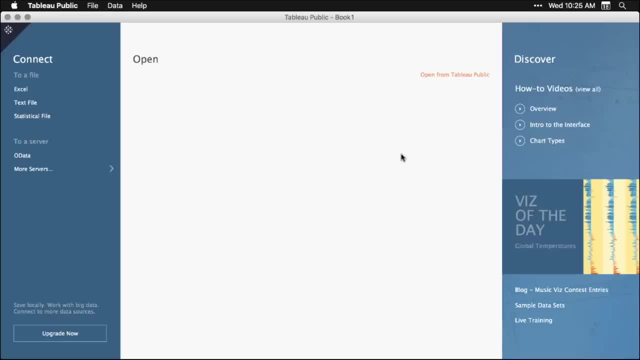 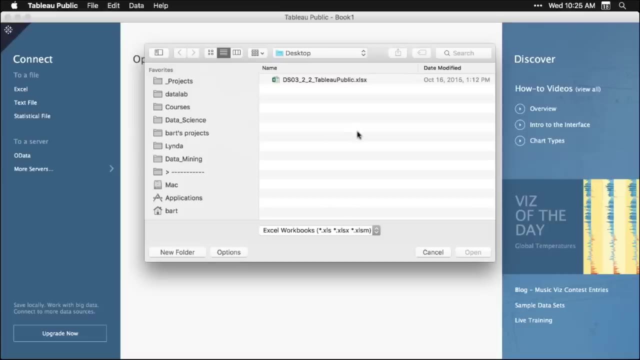 presented with a blank thing right here, And the first thing you need to do is you need to bring in some data. I'm going to bring in an Excel file Now. if you've downloaded the files for the course, you'll see that there's this one right here: dso322 tableau publicexcel sx. it's a Excel. 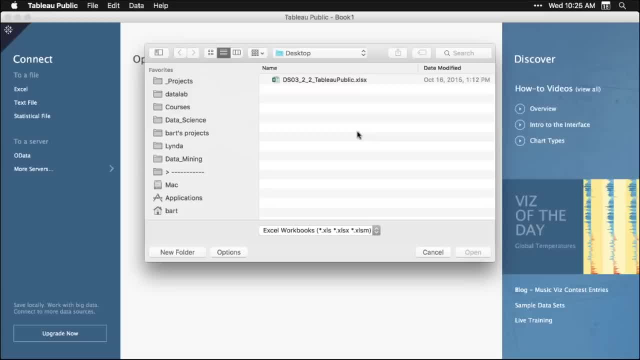 file And in fact it's the one that I use in talking about spreadsheets in the first video on this course. I'm going to select that one and I'm going to open it. And a lot of programs don't like bringing in Excel because it's got all the worksheets and all the weirdness in it. This one- 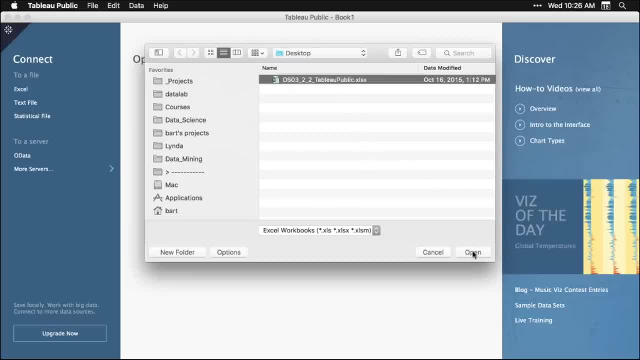 works better with it. But what I'm going to do is I'm going to take the tidy data- By the way you see that it put them in alphabetical order here- And I'm going to take tiny data. I'm just going to. 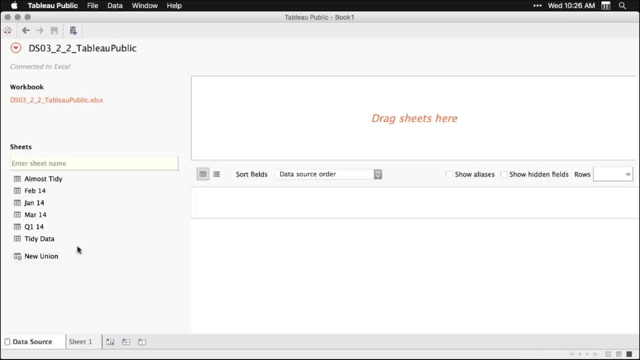 drag it over to let it know that it's the one that I want. And now what it does is it shows me a version of the data set, Along with things that you can do here, can rename it, you can. I like you can create bin groups. there's a lot of things that you can do here. I'm going to do something. 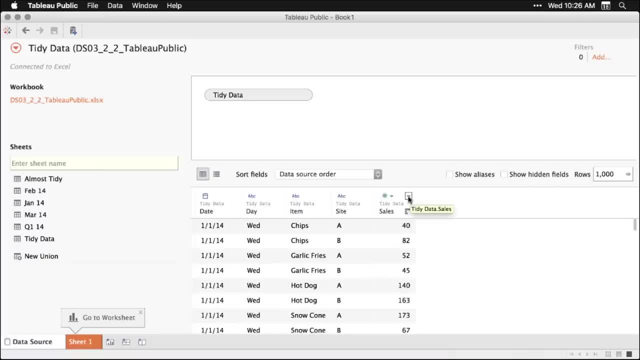 very, very quick with this, This particular one. Now I've got the data set right here. what I'm going to do now is I'm going to go to a worksheet. That's where you actually create several. cancel that and go to worksheet. 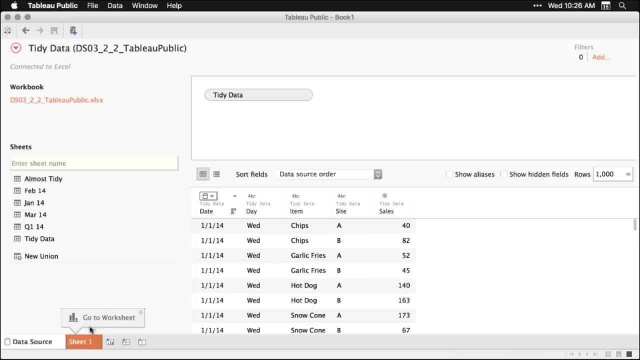 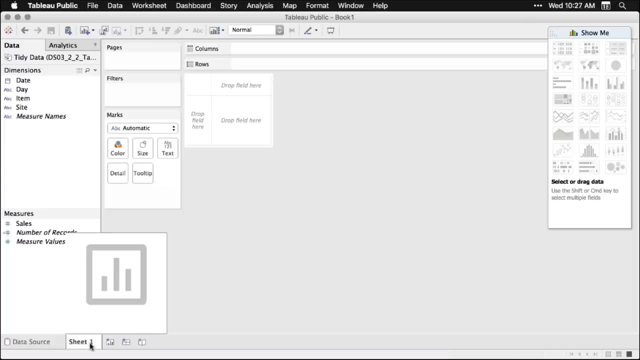 one. Okay, this is a drag and drop interface, And so what we're going to do is we're going to pull the bits and pieces of information we want to make graphics. there's immense flexibility here. I'm going to show you two. 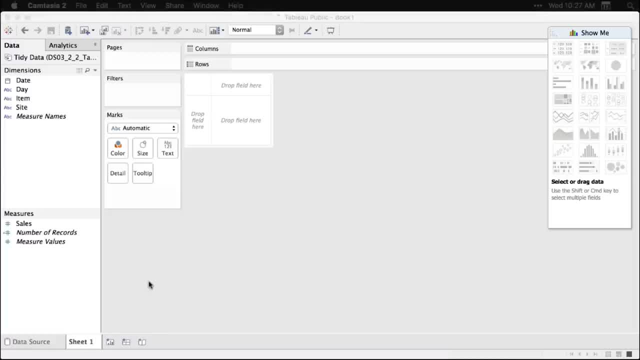 very basic ones. I'm going to look at the sales of my fictional ballpark items. So I'm going to grab sales right here And I'm going to put that as the field that we're going to measure. Okay, and you see it put it down right here And this is our total sales. we're going to break it down by item. 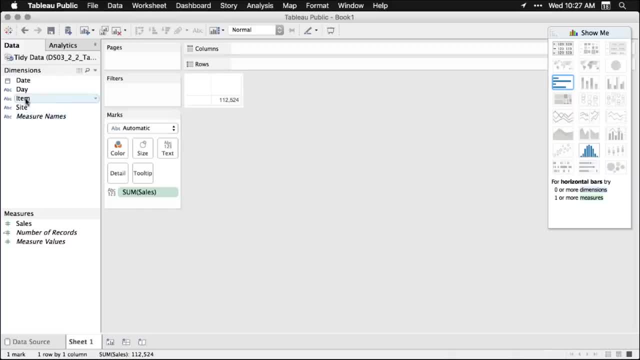 and by time. So let me take item right here And you can drag it over here, or I can put it right up here into rows. Those will be my rows And that's how many we've sold. total of each of the items. Fine, that's really easy. And then let's. 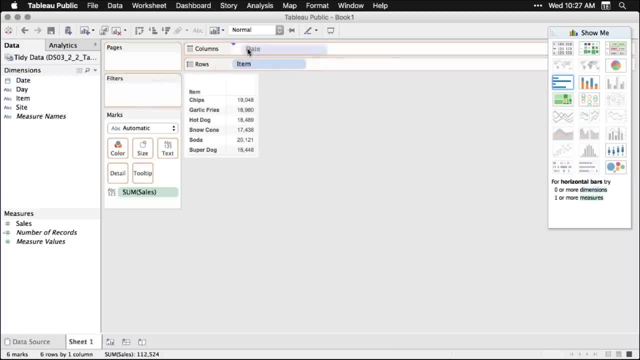 take date And we'll put that here in columns to spread it across. Now, by default, this unit by year. I don't want to do that, only have three months of data, And so what I can do is I can click right here And I can choose a different timeframe. I can go to quarter, but that's not going to help. 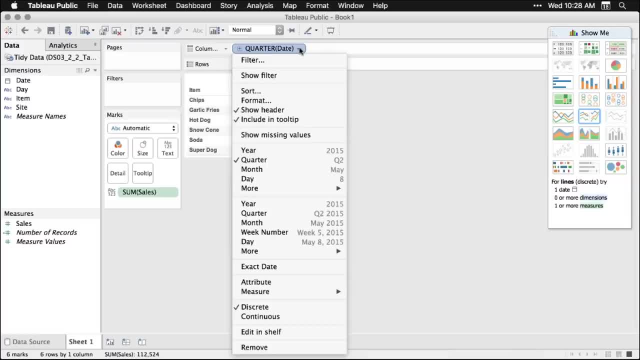 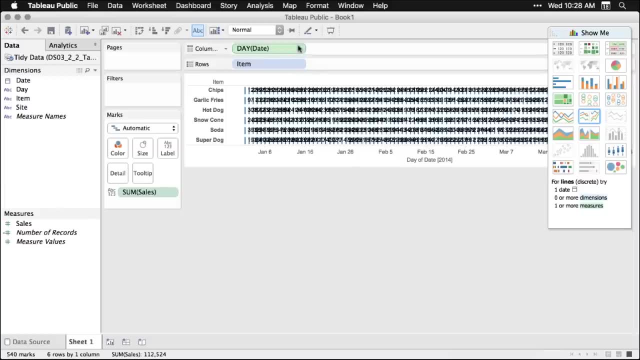 because I only have one quarters worth of data. That's three months. I'm going to come down to week. Actually, let me go today. Today, you see, it gets enormously complicated, So that's no good. So I'm going to back up to week. 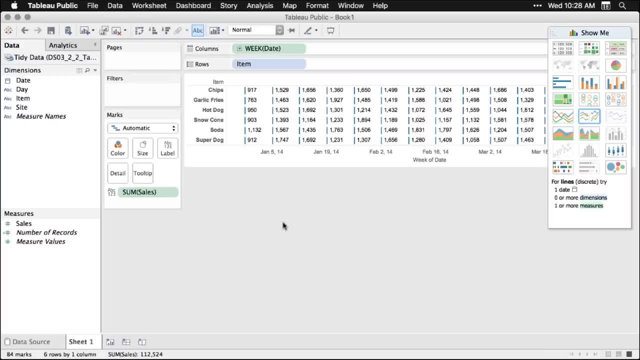 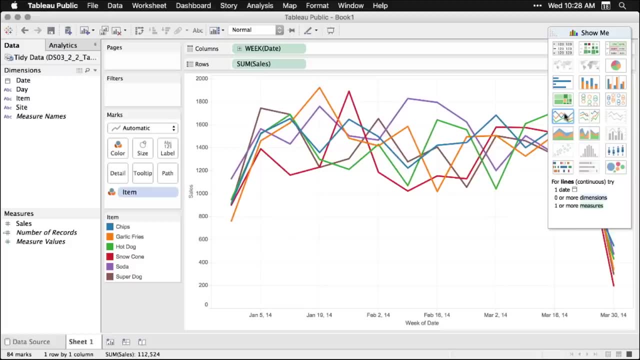 And I've got a lot of numbers there, But what I want is a graph, And so to get that, I'm going to come over here and click on this and tell it that I want a graph, And so we're seeing the information. 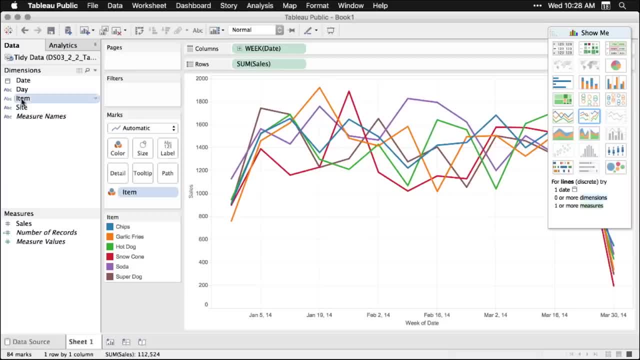 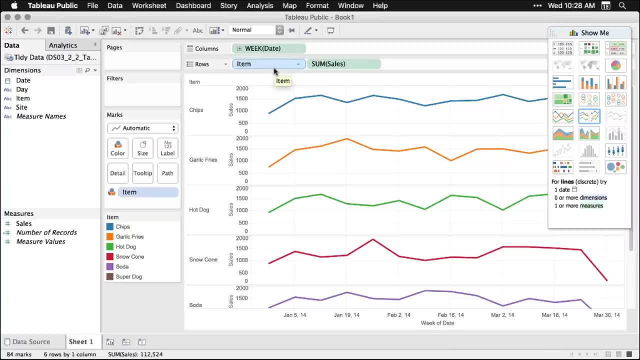 except it lost items. I'm going to bring an item and I'm going to put it back up into this graph to say this is a row for the data. And now I've got rows For sales by week for each of my items. That's great. I want to break it down one more by putting 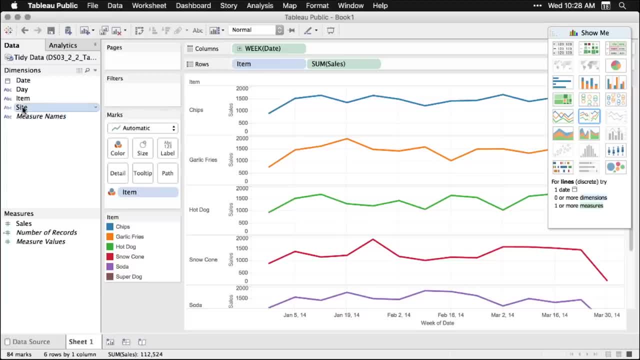 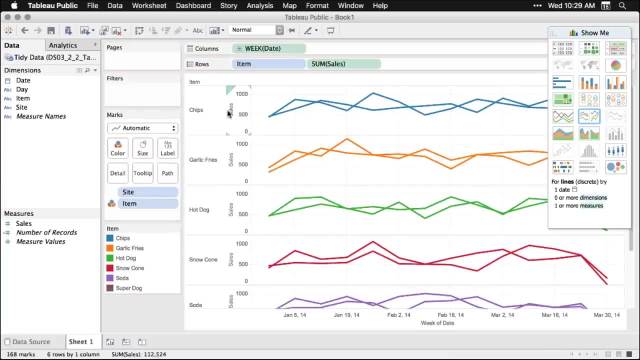 in the site, the place that it's sold, And so I'm going to grab that And I'm going to put it right over here. And now, you see, I've got it broken down by the item that is sold and the different sites, and I'm 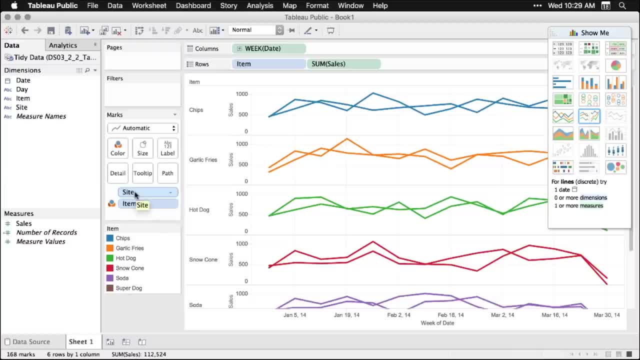 going to color the sites And all I got to do to that is I'm going to grab site and drag it onto color. Now I've got two different colors for my sites And this makes it a lot easier to tell what's going on, And in fact there's some other cool. 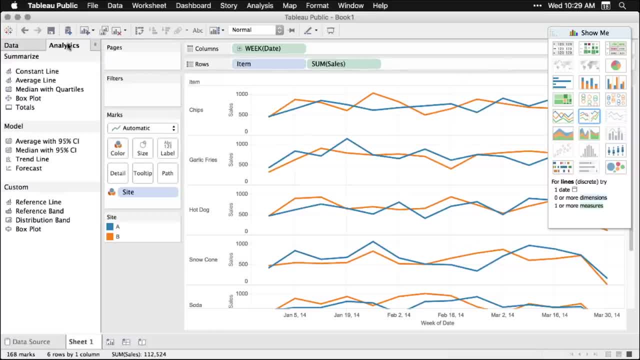 stuff you can do. One of the things I'm going to do is I can come over here to analytics And I can tell it, for instance, to put an average line through everything. So I'll just drag this over here. Say, now we have the average for each line, That's good, And I can even do forecasting. Let me 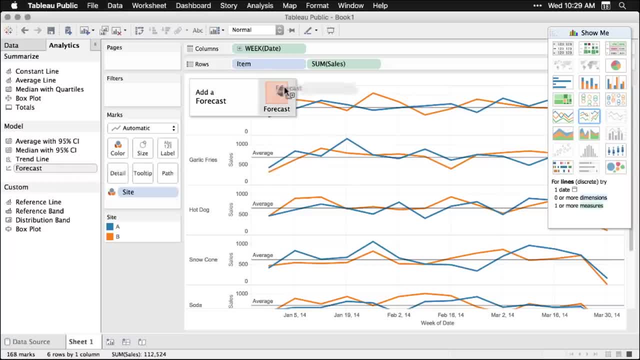 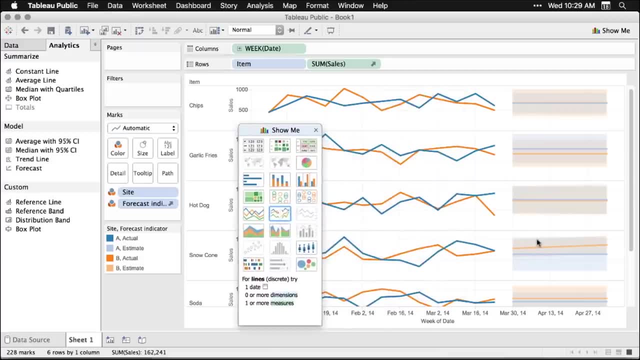 get a little bit of a forecast right here. I'll drag this on And if you go over here I can get this out of the way for a second. Now I have a forecast for the next few weeks And that's a really convenient, quick and easy thing, And again, for some organizations that might be. 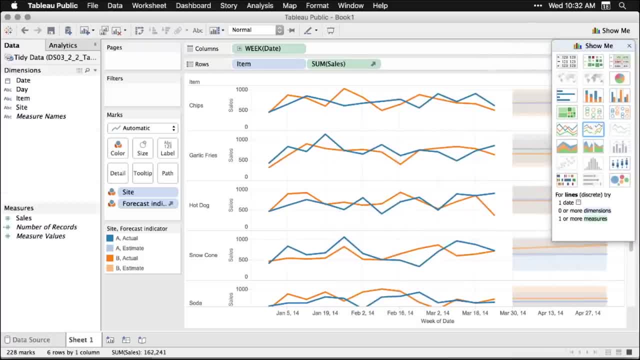 all that they really need, And so what I'm showing you here is the absolute basic operation of Tableau, which allows you to do an incredible range of visualizations and manipulate the data and create interactive dashboards. There's so much to it, And we'll show that in another video. 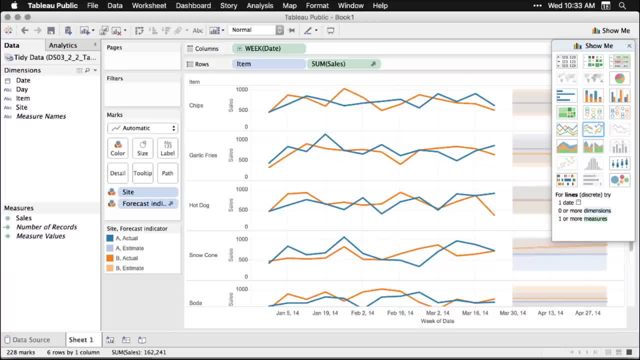 Of course, but for right now, I want to show you one last thing about Tableau public, and that is saving the files. So now, when I come here and save it, it's going to ask me to sign into Tableau public. Now I sign in and asked me how I want to save this same name as the video. There we go And I'm going to hit save. 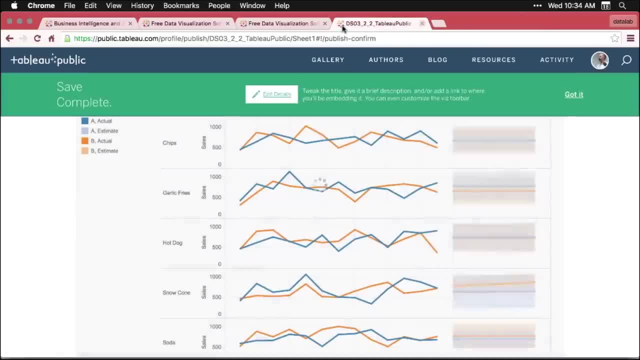 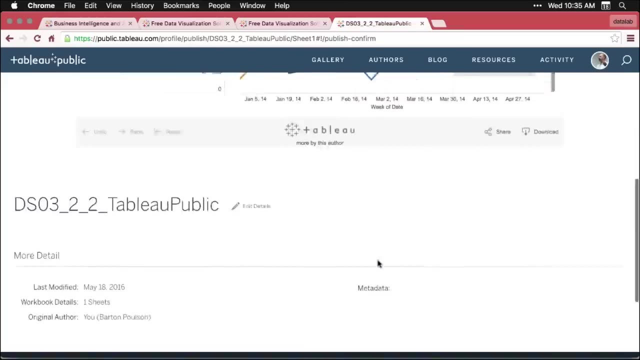 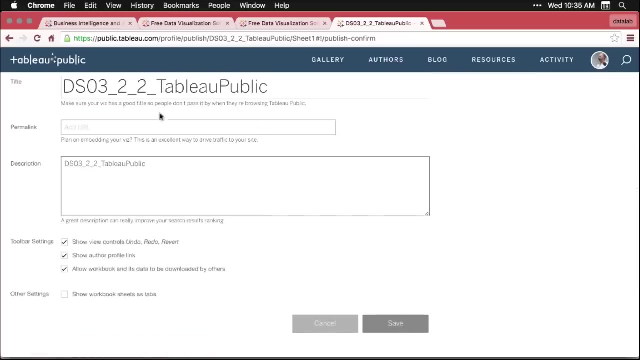 And since I learned that this was going to be the video I was going to use, I was going to click OK, Sure, so I can save it. And then that opens up a web browser, And since I'm already logged into my account- see, here's my account, my profile, Here's the page that I created, And it's got everything I need there. I'm going to edit just a few details. I'm going to say, for instance, I'm going to leave its name like that. I could put more of a description there if I wanted. I can allow people to use this page, and then I can close it too. I'm going to say, OK, here we go. And now I'm going to go ahead and give it a name. So here's the page that I created. 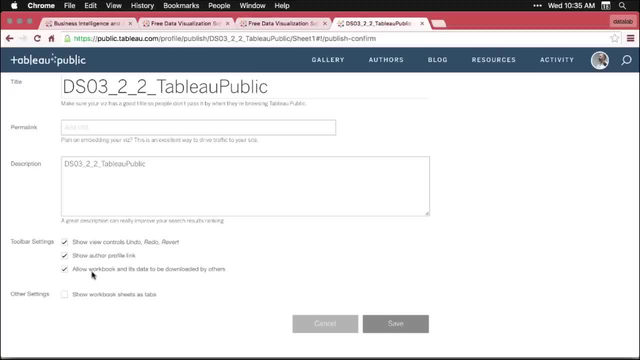 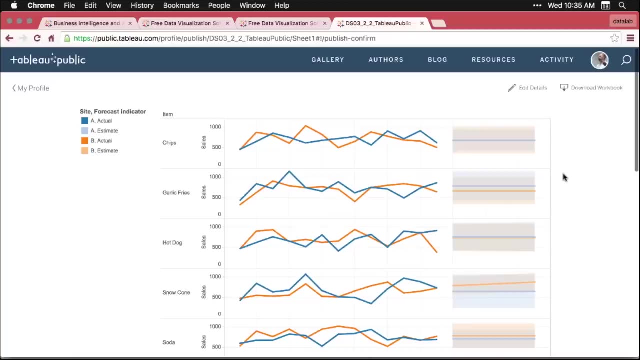 to download the workbook and its data. I'm going to leave that there So you can download it if you need to. If I had more than one tab, I would do this thing that says show the different sheets as tabs. hit save, And there's my data set And also it's published online and people can now. 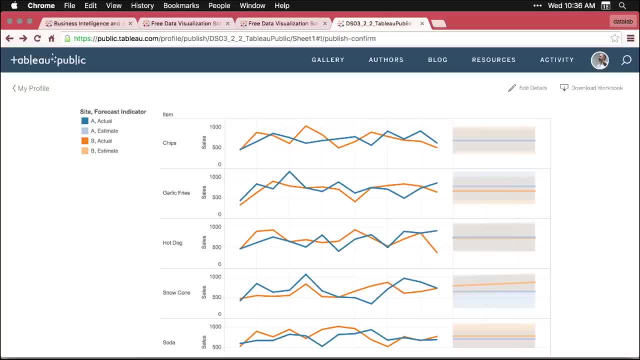 find it, And so what you have here is an incredible tool for creating interactive visualizations. you can create them with drop down menus and you can rearrange things and you can make an entire dashboard. It's a fabulous way of presenting information And, as I said before, I think that for 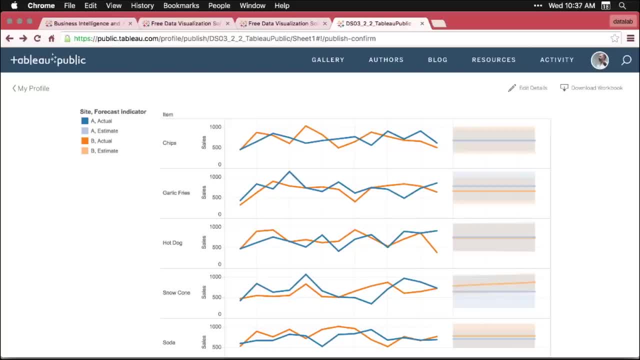 some organizations, this may be as much as they need to get really good, useful information out of their data, And so I strongly recommend that you take some time to explore with Tableau either the paid desktop version or the public version, and see what you can do to get some. 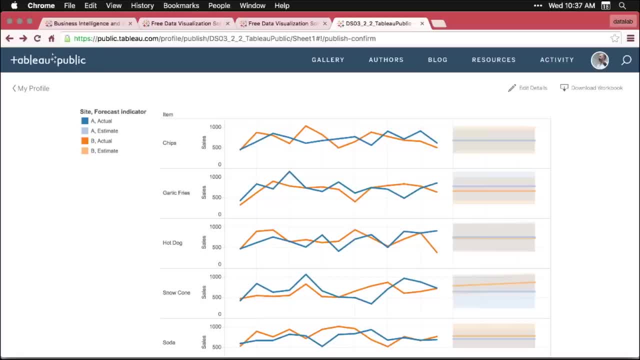 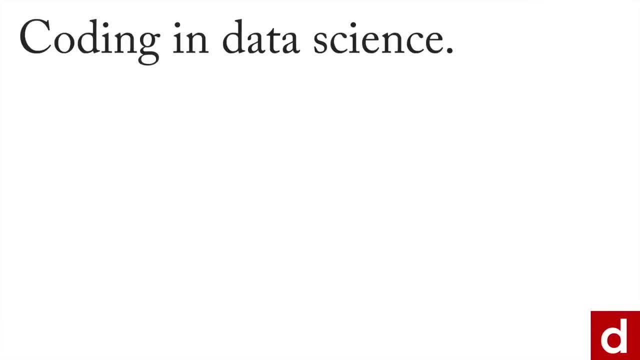 really compelling and insightful visualizations out of your work in data science. For many people, their first experience of coding and data science is with the application SPSS. Now I think of SPSS And the first thing that comes to my mind is sort of life in the ivory. 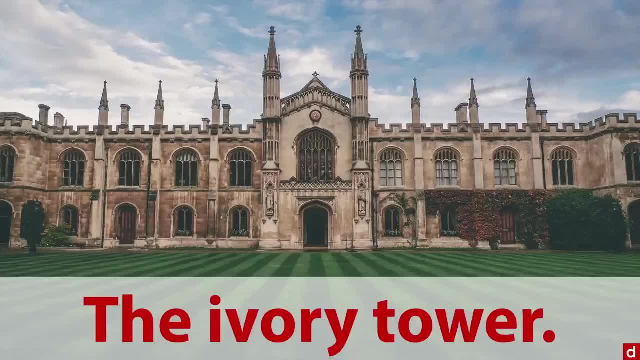 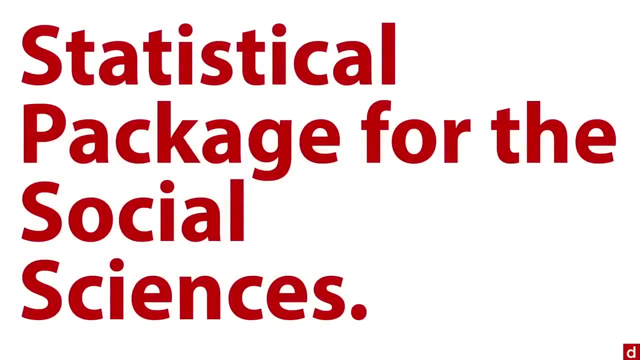 tower, though this looks more like you know Harry Potter. But if you think about it, the package name SPSS comes from statistical package for the social sciences, Although if you ask IBM about it now, they'll actually call it statistical package. 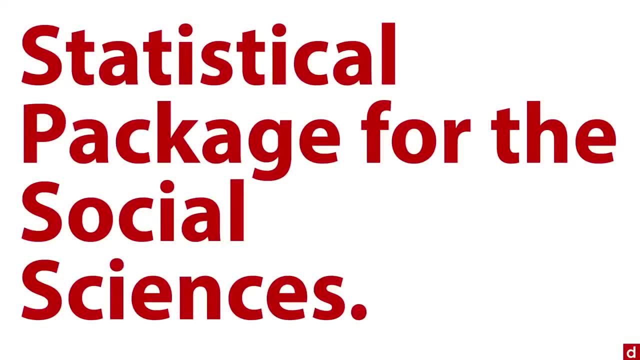 like it doesn't stand for anything, But it has its background in social science research which is generally academic And, truthfully, I'm a social psychologist And that's where I first learned how to use SPSS. But let's take a quick look at their web page: ibmcom: slash SPSS. 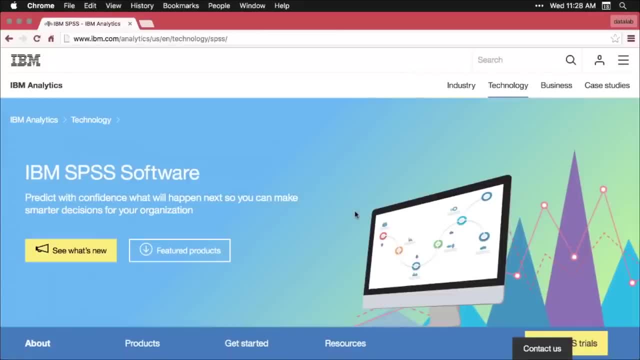 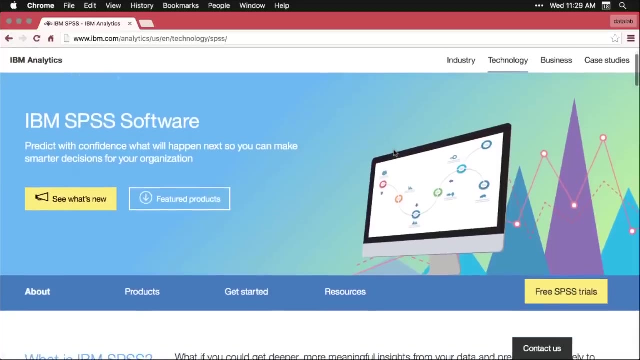 If you type that in, that'll just be a alias. it'll take you to IBM's main web page. Now IBM didn't create SPSS, but they bought it around version 16. And it was very briefly known as PASW- predictive analytics software. that only lasted briefly, And now it's back to SPSS. 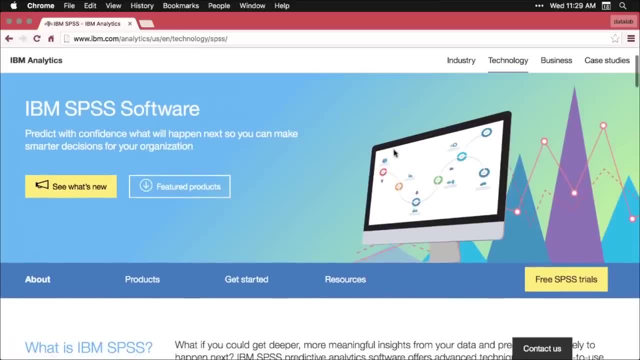 which is where it's been for a long time. SPSS is a desktop program. it's pretty big. it does a lot of things. it's very powerful. it's used in a lot of academic research. it's also used in a lot of business, consulting, management and even some medical research. 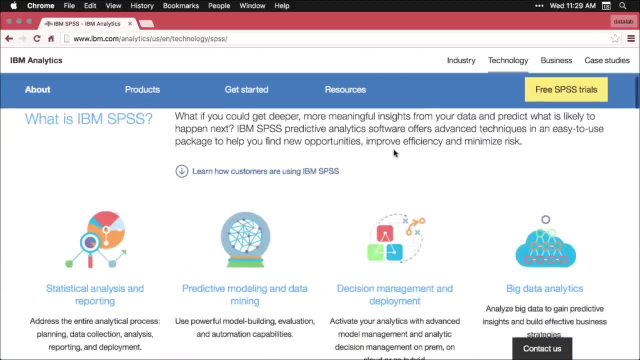 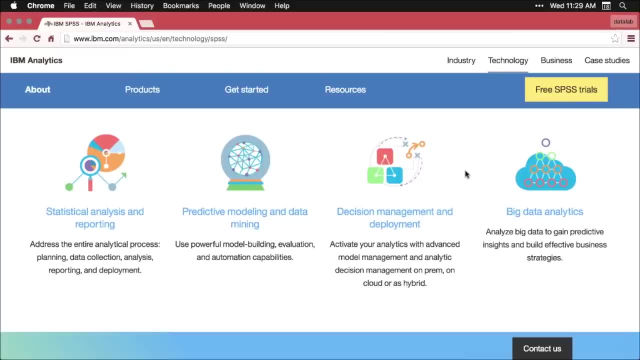 And the thing about SPSS is it looks like a spreadsheet but it has drop down menus to make your life a little bit easier compared to some of the programs programming languages that you can use. Now you can get a free temporary version. 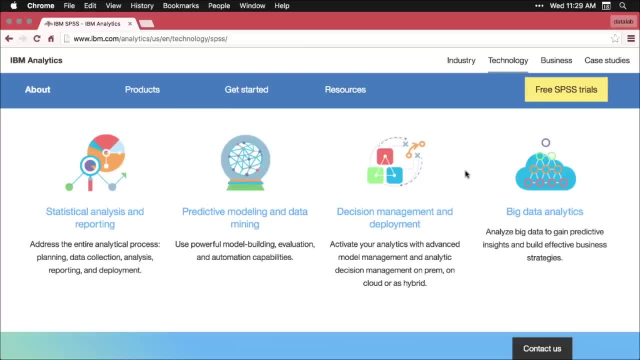 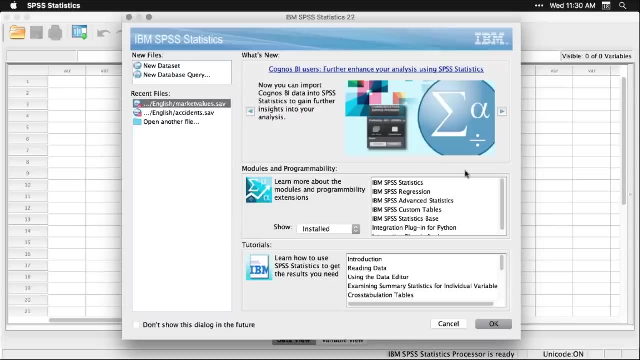 if you're a student, you can get a cheap version. Otherwise, SPSS costs a lot of money. But if you have it one way or the other, when you open it up, this is what it's going to look like. I'm showing SPSS version 22.. Now it's currently on 24. And the thing about SPSS versioning is in. 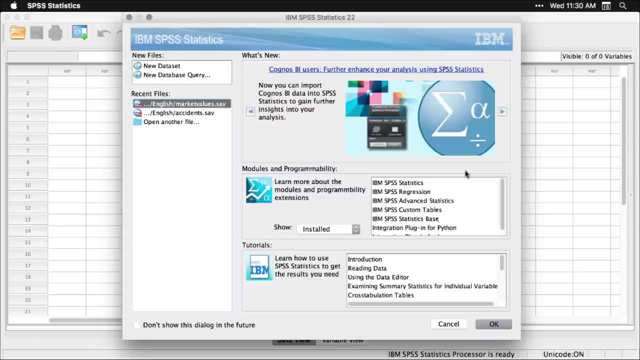 any other software package. these would be point updates. So I sort of feel like we should be on 17.3, as opposed to 22 or 24.. Because the variations are so small that anything you learn from the earlier ones is going to work in the 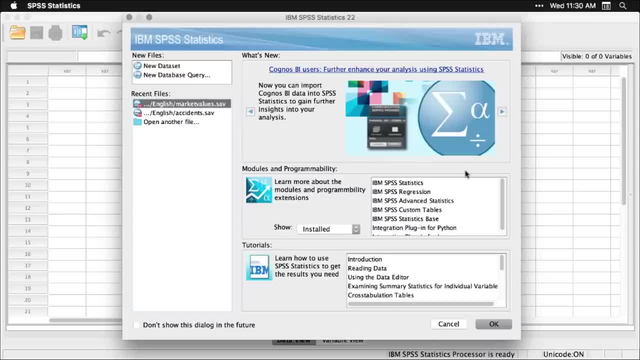 later ones, And there's a lot of backwards and forwards compatibility. So I'd almost say that this one, the version you have, practically doesn't matter. You get this little welcome splash screen And if you don't want to see it anymore you can get rid of it. I'm just going. 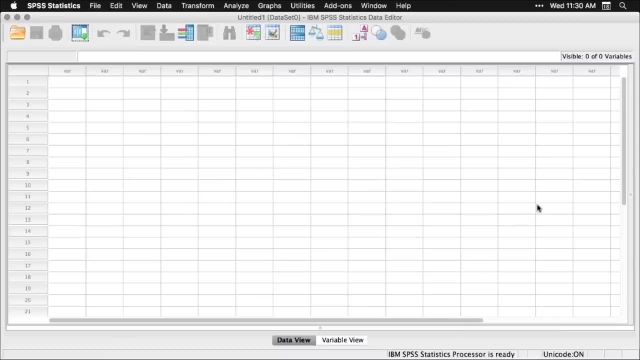 to hit cancel. here- And this is our main interface- looks a lot like a spreadsheet. the differences: you have a separate pane for looking at variable information And then you have separate windows for output and then an optional one for something called syntax. But 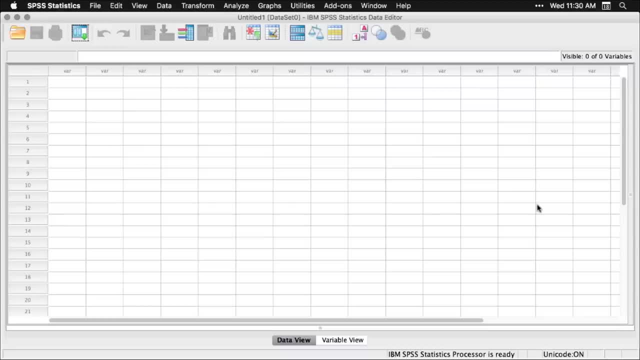 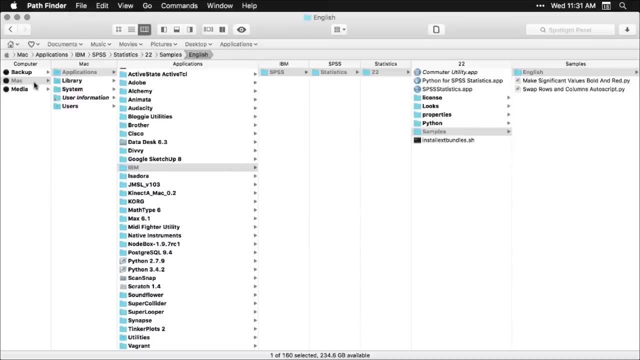 let me show you how this works by first opening up a data set. SPSS has a lot of sample data sets in them, But they're not easy to get to And they're really well hidden On my Mac, for instance. let me go to where they are In my Mac. I go to the Finder. I have to go Mac to applications, to the 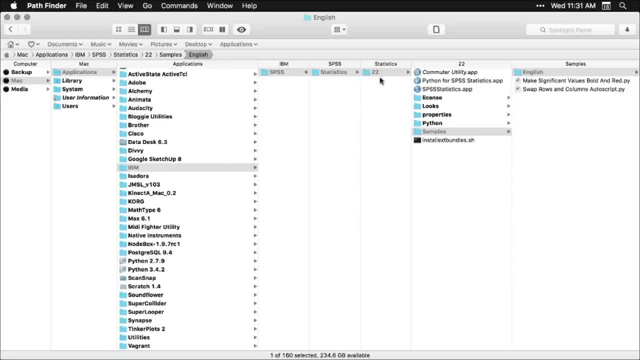 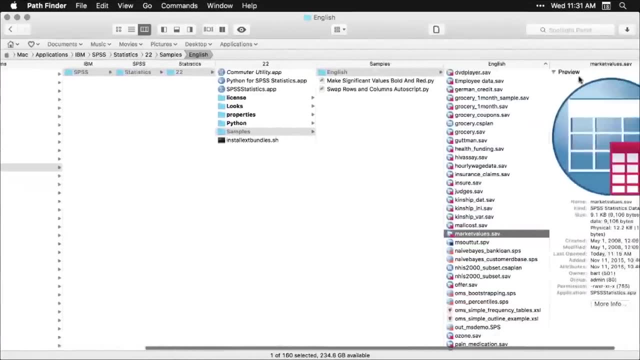 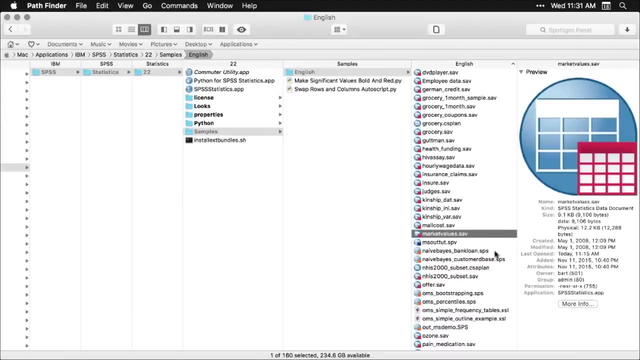 folder IBM to SPSS, to statistics, to 22,. the version number two samples. then I have to say I want the ones that are in English. And then it brings them up. The dot SAV files are the actual data files. There are different kinds in here, So dot SPS is a different kind of file. And then 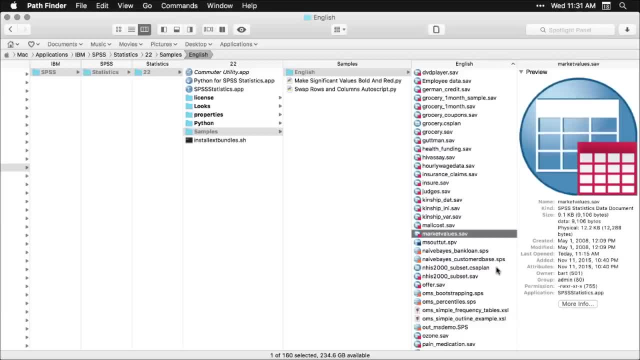 we have a different one about planning analyses, So there are versions of it. I'm going to open up a file here called market values dot SAV, the small data set in SPSS format, And if you don't have that you can open up something else. it really doesn't matter for now. 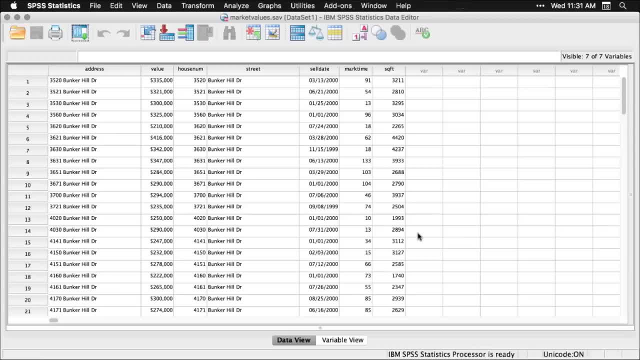 By the way, in case you haven't noticed, SPSS tends to be really, really slow when it opens It also, despite being a version 24, tends to be kind of buggy and crashes, And so when you work with SPSS, you want to get in the habit of saving your work constantly And also being patient when 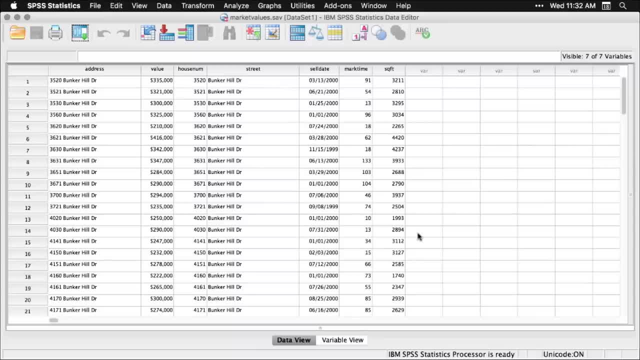 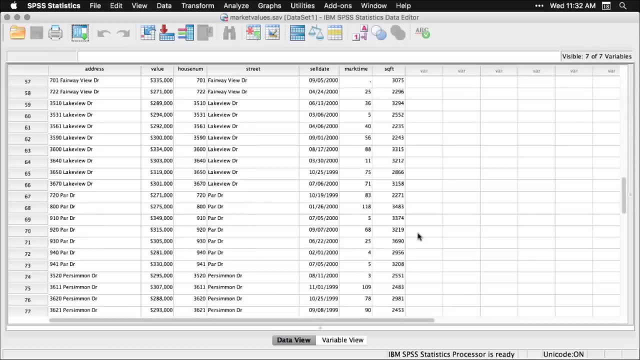 it's time to open the program. So here's a data set that just shows addresses and house values for, and square feet for, some information. This I don't even know if this is real information. that looks. it looks artificial to me, But SPSS lets you do point and click analyses, which is unusual. 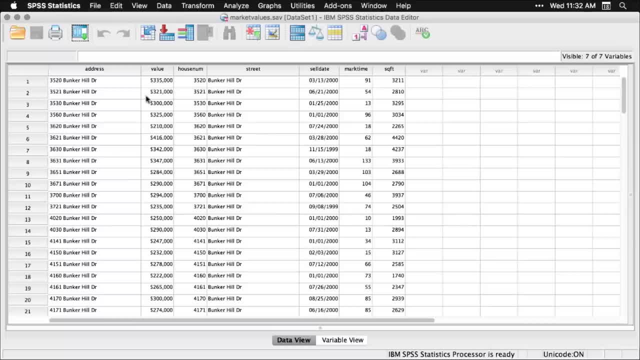 for a lot of things. So I'm going to come up here And I'm going to say, for instance, make a graph. I'm going to make a. I'm actually going to use what's called a legacy dialogue to get a histogram. 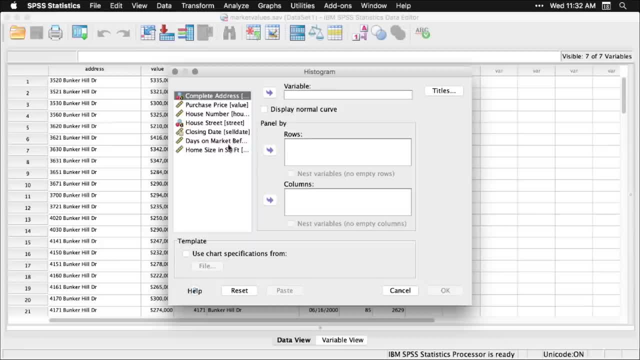 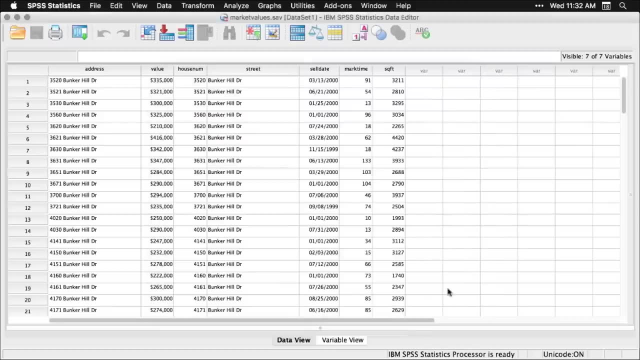 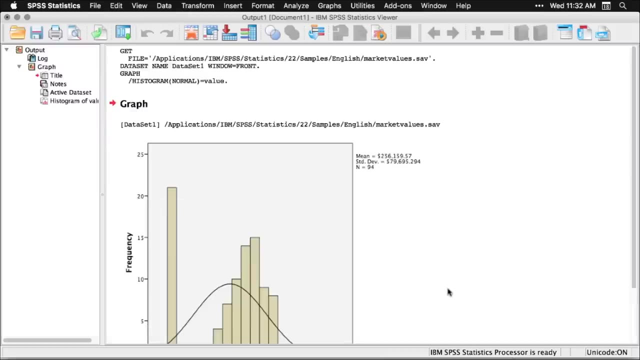 of house prices. So I simply click values, Put that right there And I'll put a normal curve on top of it and hit OK, And then it's going to open up a new window and it opened up a microscopic version of it here, So I'm going to make that bigger. This is the output. 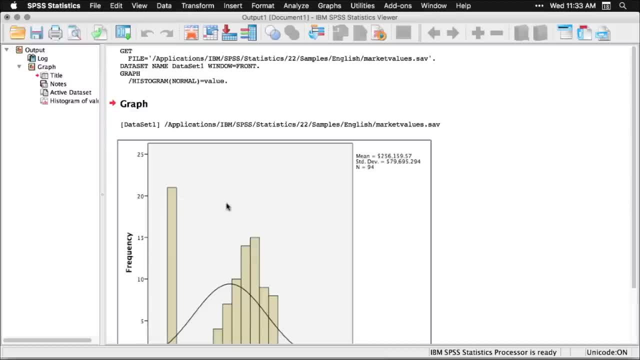 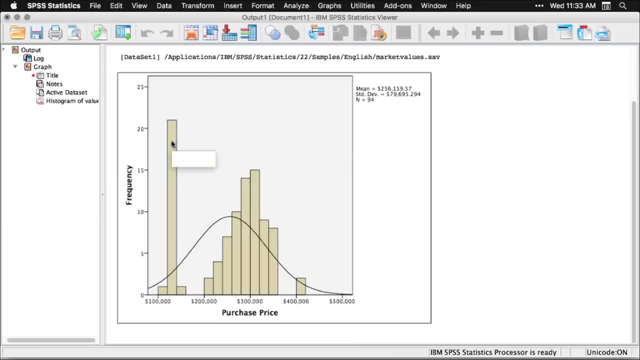 window, And so this is a separate window And it has a navigation pane here on the side. it tells me where the data came from And it saves the command here And then you know there's my default histogram, And so we see most of the houses were right around $125,000. 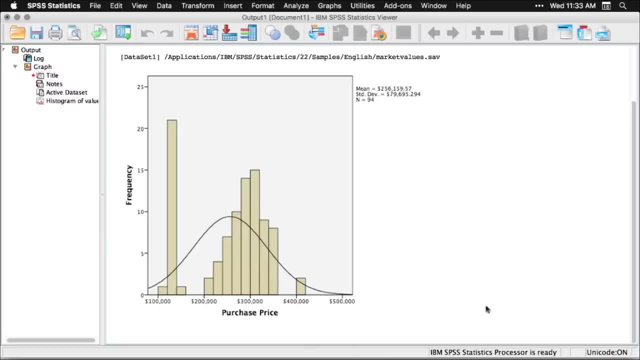 And then they went up to at least 400,000.. I have a mean of 256,000, the standard deviation of about 80,000.. And there's 94 houses in the data set. Fine, that's great. The other: 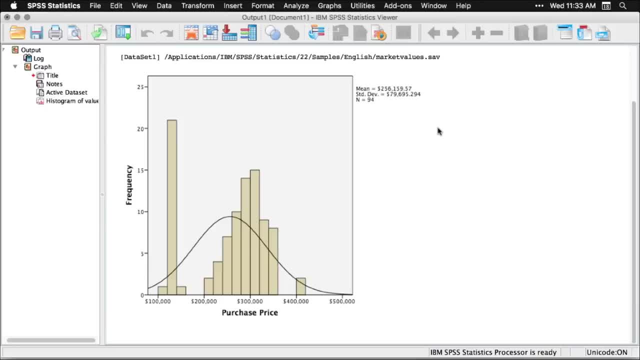 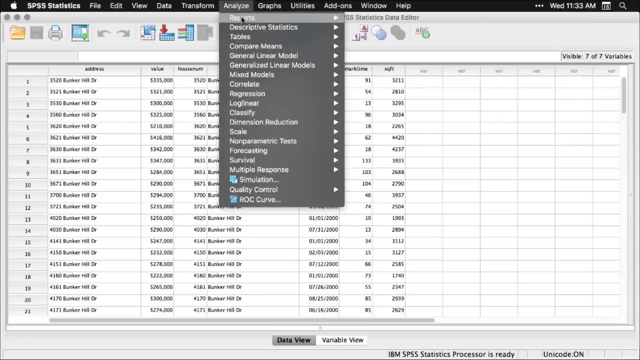 thing I can do is, if I want to do some analyses, let me go back to the data just for a moment. For instance, I can come here to analyze and I can do descriptives. I'm actually going to do, excuse me, I'm going to do one here called explore. 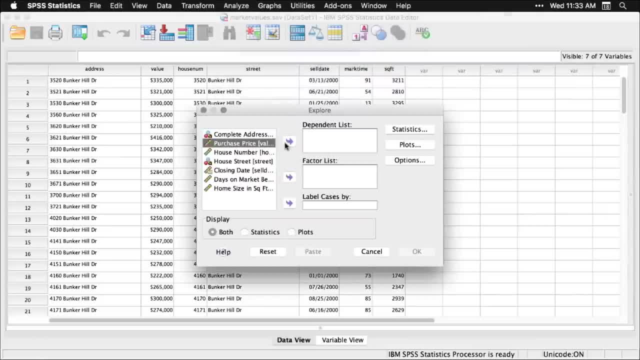 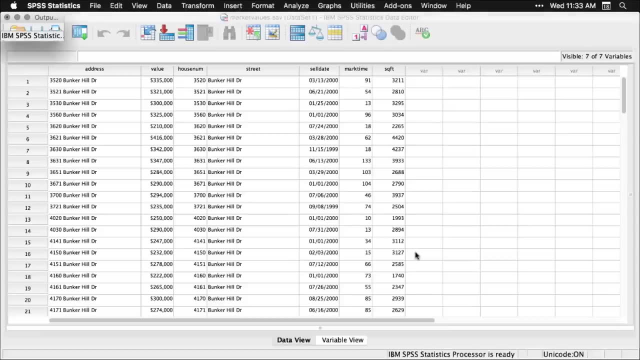 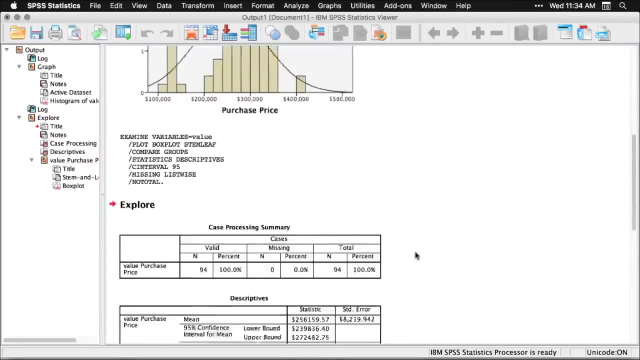 And I'll take the purchase price and I'll put it right here And I'm going to get a whole bunch of stuff, just by default. I'm going to hit OK And it goes back to the output window. Once again made it tiny, And so now you see, beneath my chart, I now have a table. 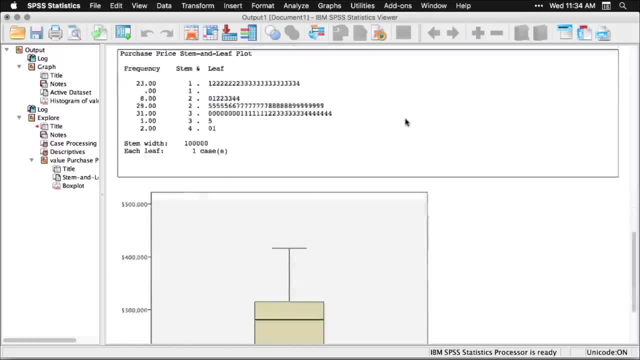 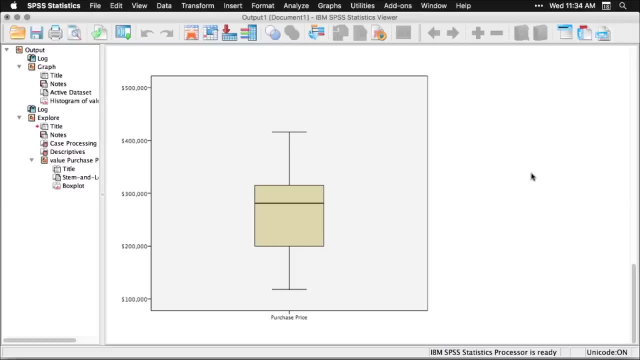 and I've got a bunch of information, a stem and leaf plot And I've got a box plot to a great way of checking for outliers, And so this is a really convenient way to save things. You can export this information As images. you can export the entire file as an HTML. you can do it. 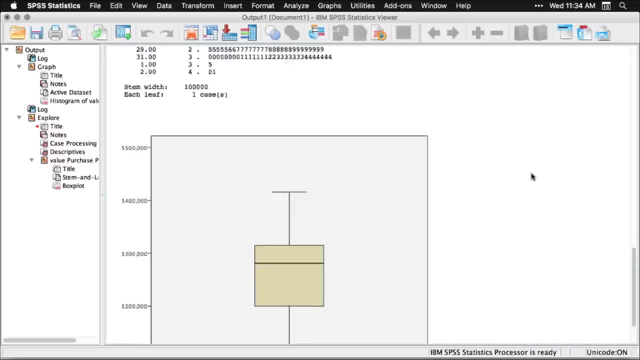 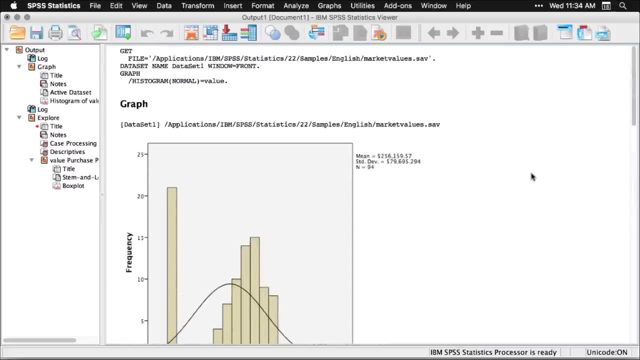 as a PDF or a PowerPoint. There's a lot of options here And you can customize everything that's on here. Now I just want to show you one more thing that makes your life so much easier in SPSS. You see right here that it's putting down these commands. it's actually 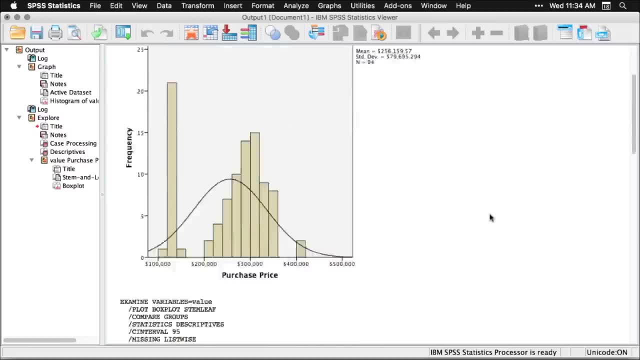 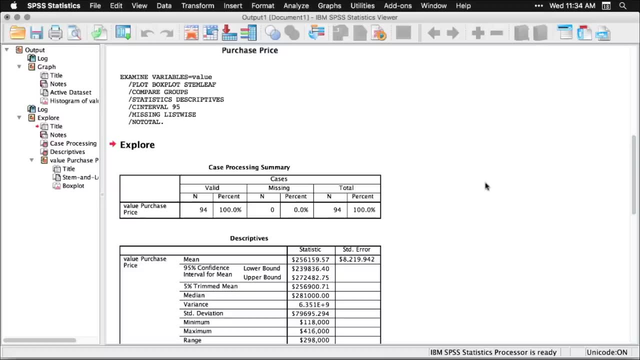 saying graph, and then histogram, normal equals value, And then down here we've got this little command right here. Most people don't know how to save their work in SPSS And they kind of just have to do it over again every time. But there's a very simple way to do this. What I'm going 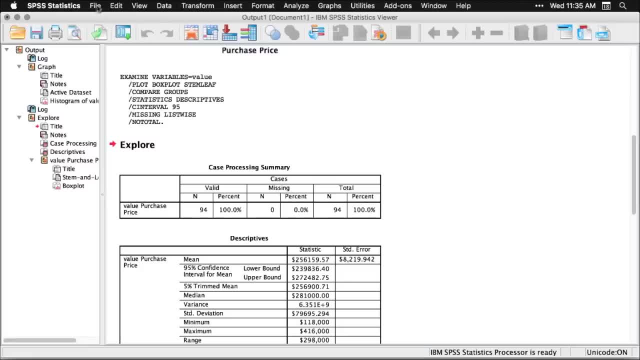 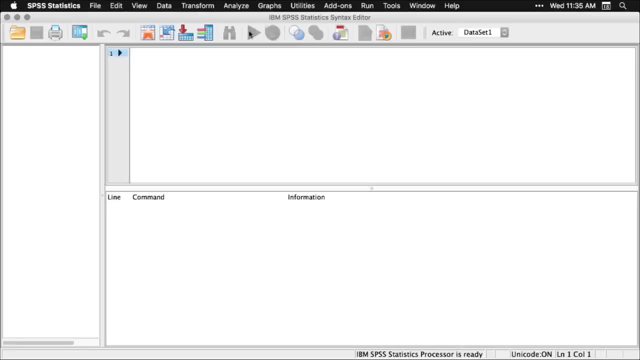 to do is: I'm going to open up something called a syntax file, I'm going to go to new syntax, And this is just a blank window. That's a programming window. It's for saving code. And let me go back to my analysis I did a moment ago. 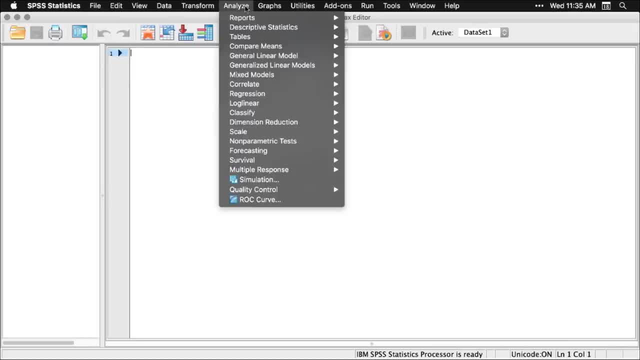 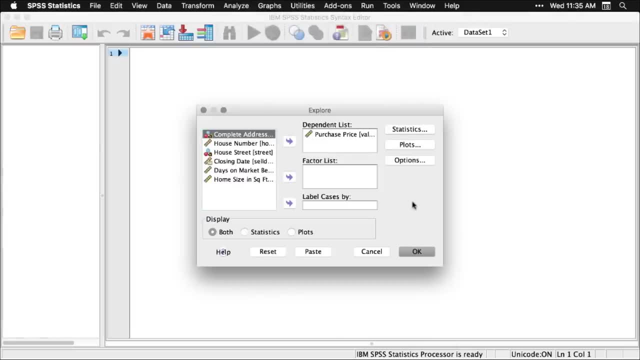 I'll go back to analyze. I can still get it right here and descriptives and explorer And my information is still there. And what happens here is, even though I set it up with drop down menus and point and click, if I do this thing, paste, then what it does is: 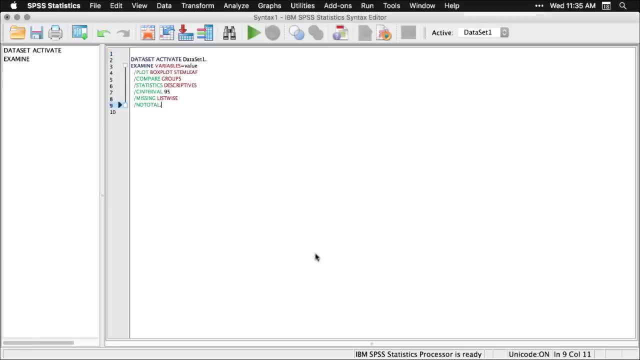 it takes the code that creates that command and it saves it to the syntax window. And this is just a text file. It saves it as dot SPSS, But it's a text file that can be opened in anything, And what's beautiful about this is it's really. 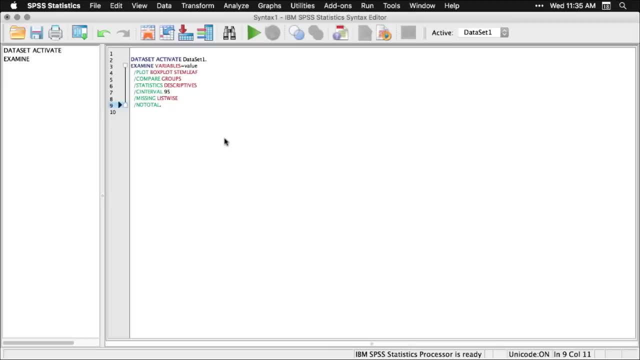 easy to copy and paste. It'll just say: this is the text file that you've saved, So you'll and paste, And you can even take this into like Word and do find and replace on it, And it's really easy to replicate the analyses. And so for me SPSS is a good program, But until you, 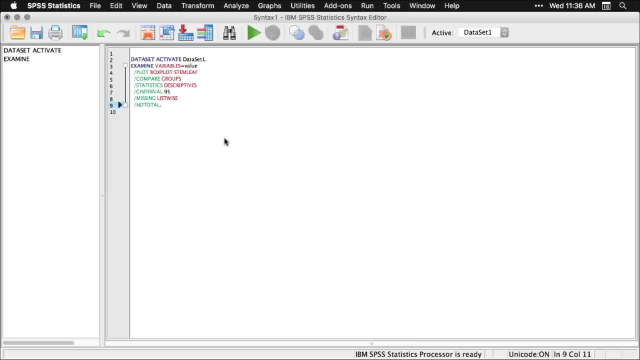 use syntax, you don't know the true power of it and it makes your life so much easier as a way of operating it. Anyhow, this is my extremely brief introduction to SPSS. All I want to say is that it's a very common program, kind of looks like a spreadsheet, but it gives you a lot more. 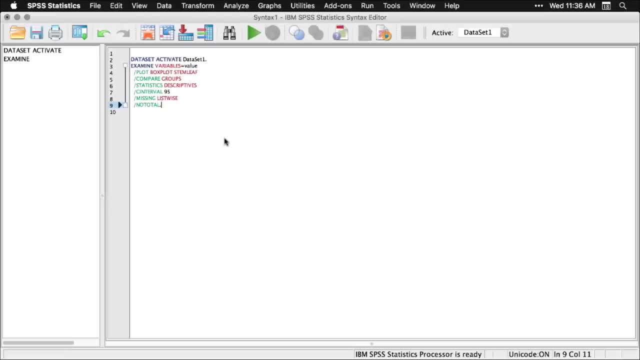 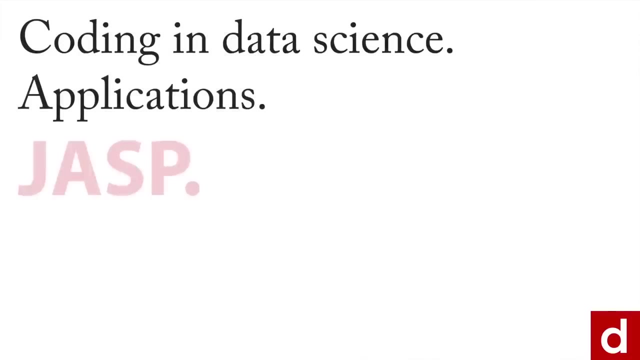 power and options, And you can use both drop down menus and text based syntax commands as well to automate your work and make it easier to replicate it in the future. I want to take a look at one more application for coding and data science. that's called jazz. This is a new application. 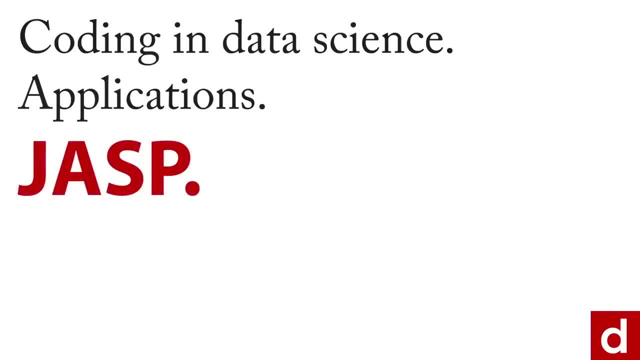 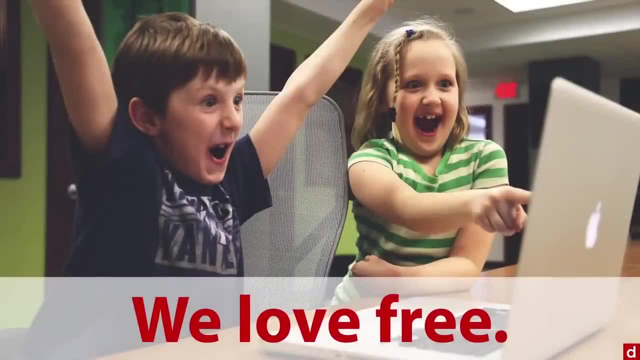 not very familiar to a lot of people and still in beta, But with amazing promise. you can basically think of it as a free application, And it's a free application that you can use for a lot of things, And it's a free version of SPSS And you know what we love free. But jazz is not just 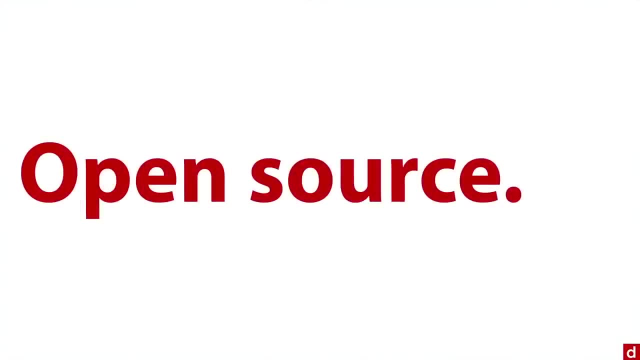 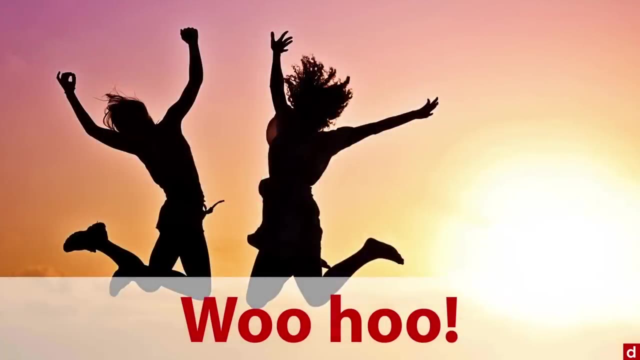 free. It's also open source And it's intuitive And it makes analyses replicable And it even includes Bayesian approaches, And so take that all together. you know we're pretty happy and we're jumping for joy. So before we move on, you just may be asking yourself, you know, 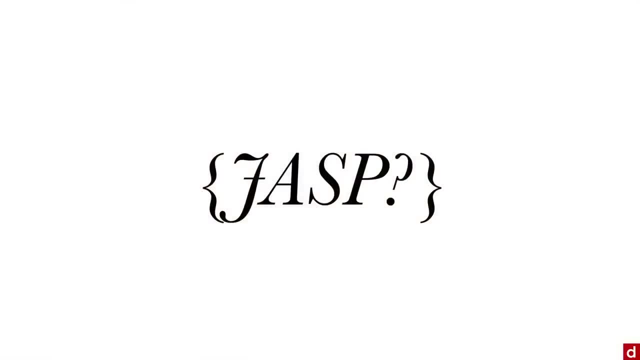 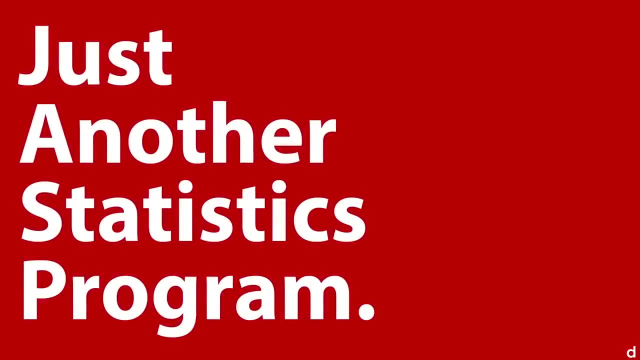 JASP. what is that? Well, the creators emphatically deny that it stands for just another statistics program. But be that as it may, we'll just go ahead and call it JASP and use it very happily. You can get to it by going to. 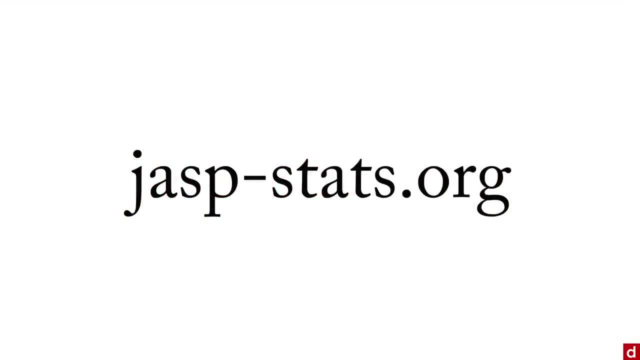 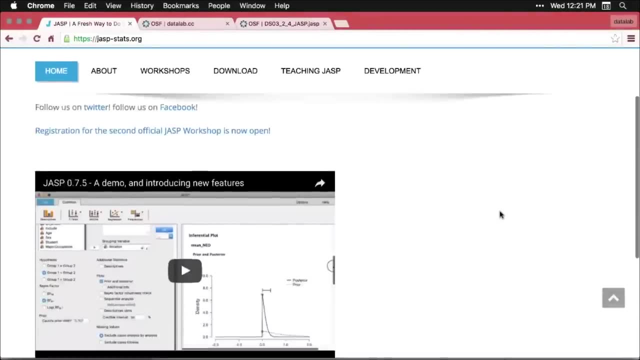 jazz, dash, statsorg, And let's take a look at that right now, Just as a new program. they say a low fat alternative to SPSS, But it is a really wonderful, great way of doing statistics. you're going to want to download it Best to find your platform. 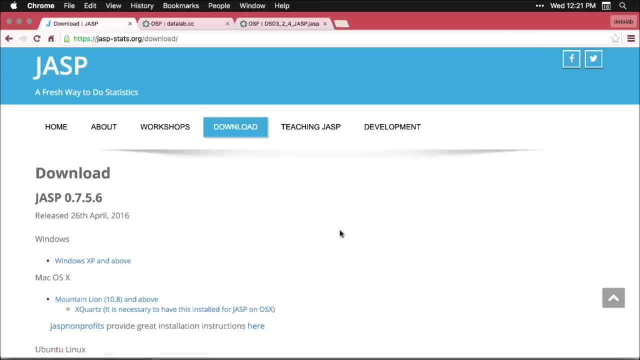 It even comes in Linux format, which is beautiful, And again, it's beta, So stay posted. things are updating regularly And if you're on Mac, you're going to need to use x quartz, But that's an easy thing to install. It makes a lot of things work better And it's a wonderful way to do analyses. 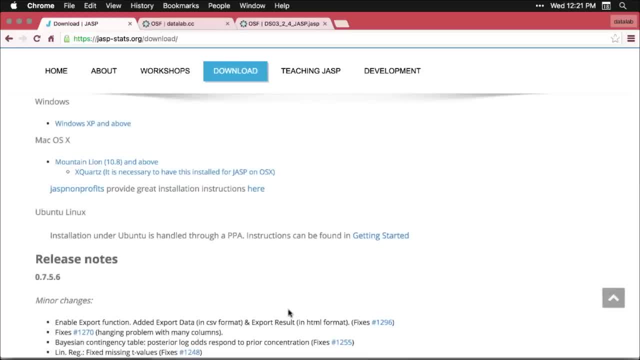 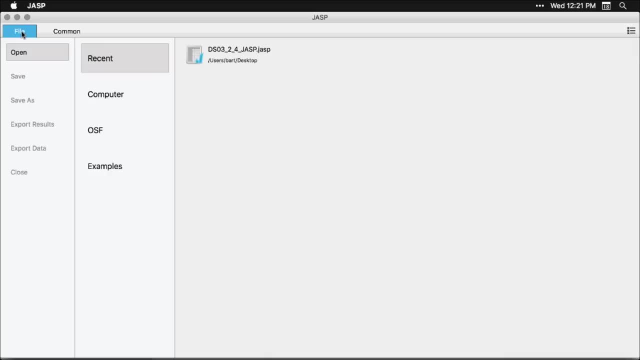 When you open up jazz it's going to look like this. It's a pretty blank interface, But it's really easy to get going with it. So, for instance, you can come over here to file And you can even use some example data sets. So, for instance, here's one called big five. that's personality. 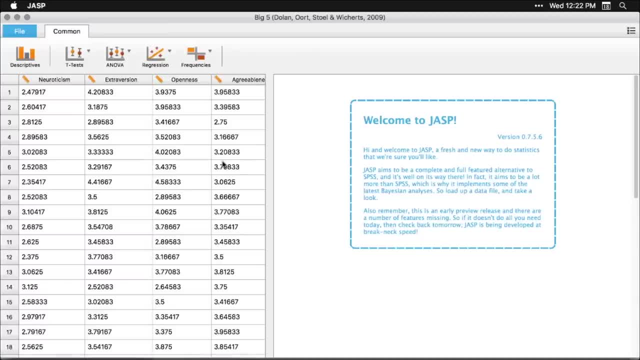 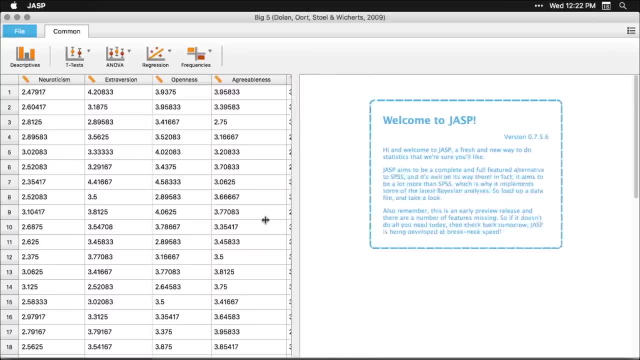 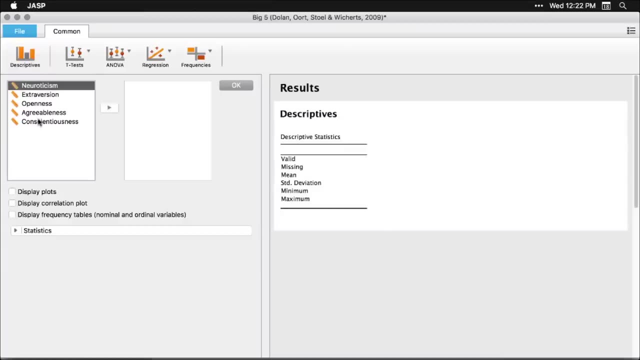 factors And you've got data here that's really easy to work with. Let me scroll this over here for a moment. So there's our five variables And let's do some quick analyses with these. say, for instance, we want to get descriptives. we can pick a few variables. Now, if you're familiar with 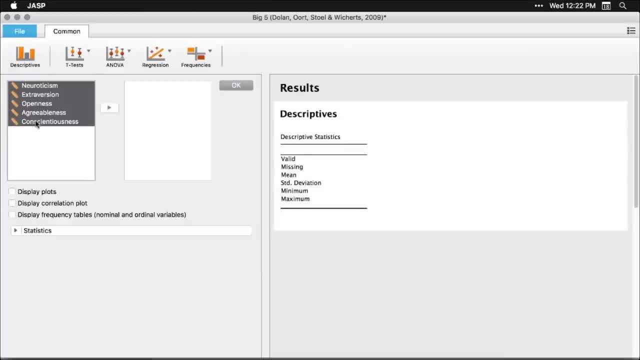 SPSS, the layout feels very much the same And the output looks a lot the same. So let's go ahead and pop. it looks a lot the same. You know? all I have to do is select what I want and it immediately. 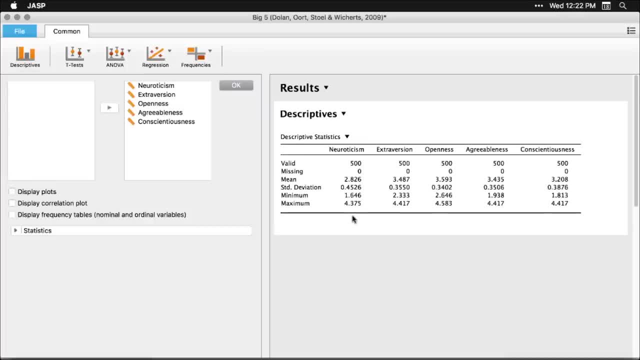 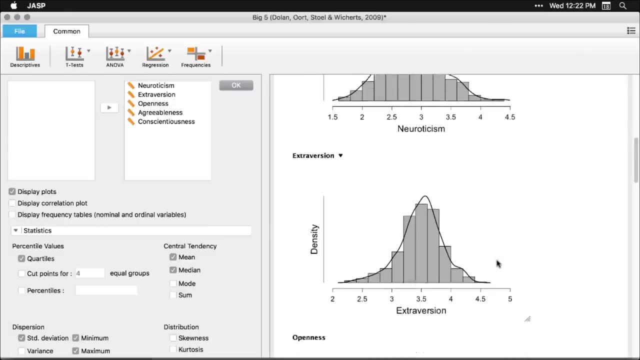 pops up over here And then I can choose additional statistics and get quartiles, I can get the median And you can choose plots. Let's get some plots. all I do is click on it and they show up, And that's a really beautiful thing, And you can modify these things a little bit. So, for instance, 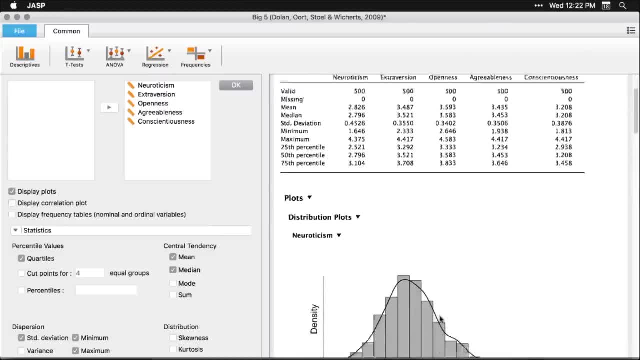 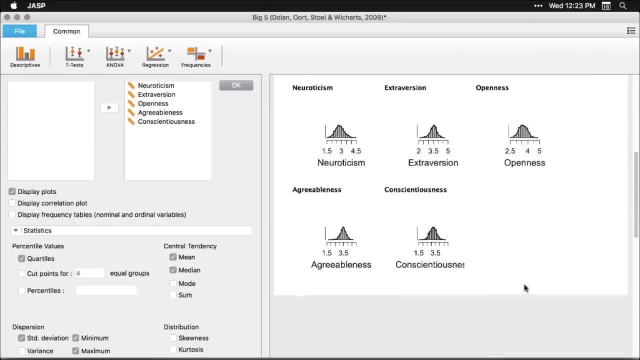 I can take the plots and let's see if I can drag that down And if I make it small enough, I can plots. well, I went a little too far on that one. Anyhow, you can do a lot of things here And I can. 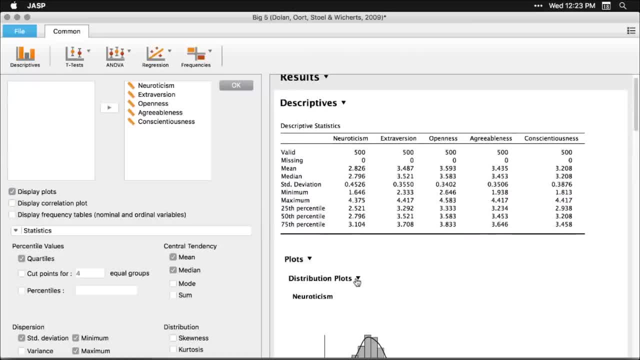 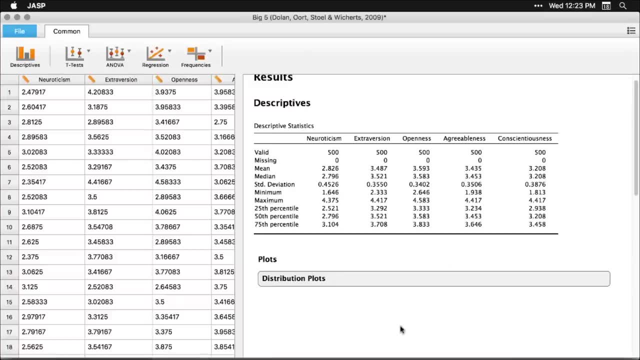 hide this, I can collapse that, And I can go on and do other analyses. Now. what's really neat, though, is when you navigate away from it, so I just clicked in the blank area of the results pane. we're back to the data here, But if I click on one of these tables like this one right here, 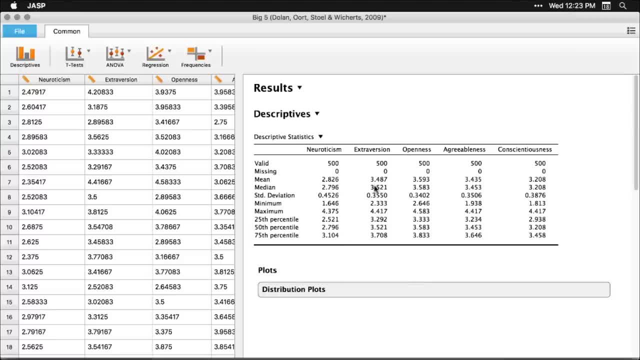 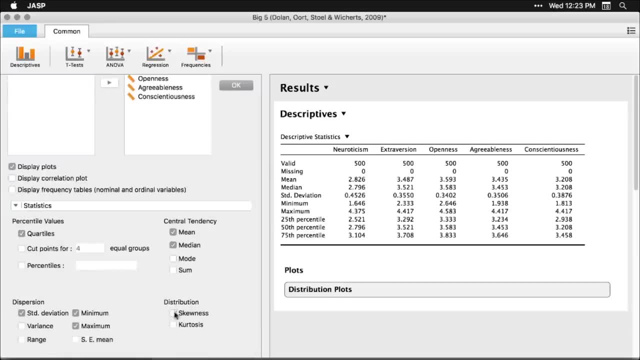 it immediately brings up the commands that produced it, And I can just modify it some more if I want to say I want skewness and kurtosis. Boom, they're in there. It's an amazing thing. And then I can come back out here, I can click away from that And I can come down to 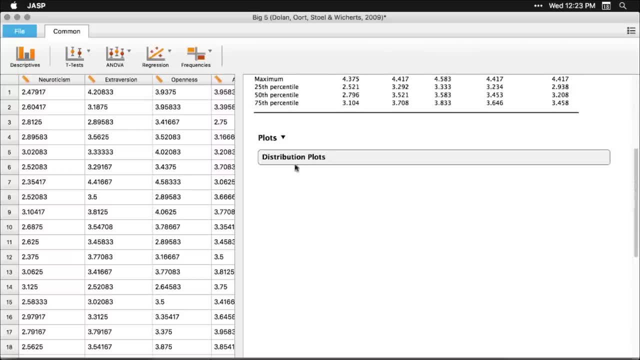 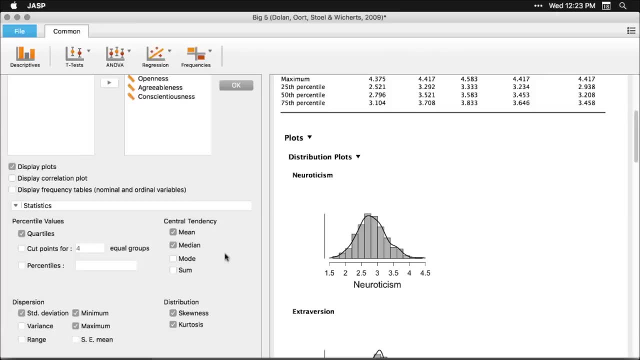 the plots, expand those, And if I click on that, it brings up the commands that made them. It's an amazingly easy and intuitive way to do things. Now there's another really nice thing about jazz, And that is that you can share the information online really well through a program called osfio That stands 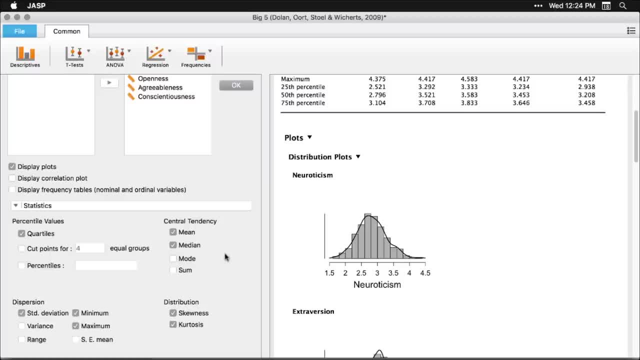 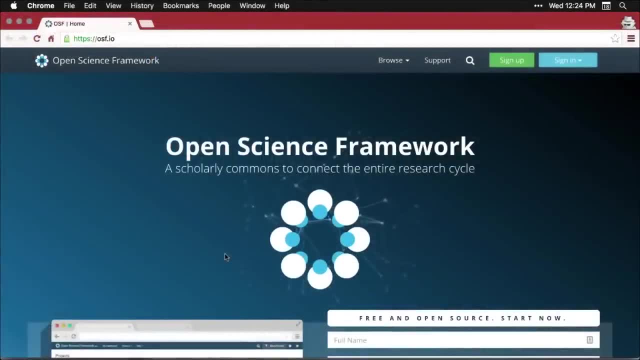 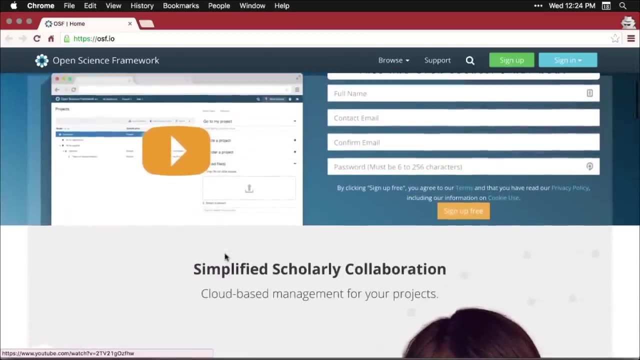 for the Open Science Foundation. That's this web address, osfio, So let's take a quick look at what that's like. Here's the Open Science Framework website, And it's a wonderful service. It's free And it's designed to support open, transparent, accessible, accountable, collaborative research. 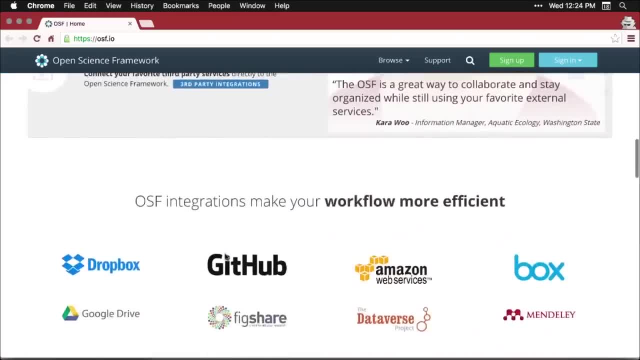 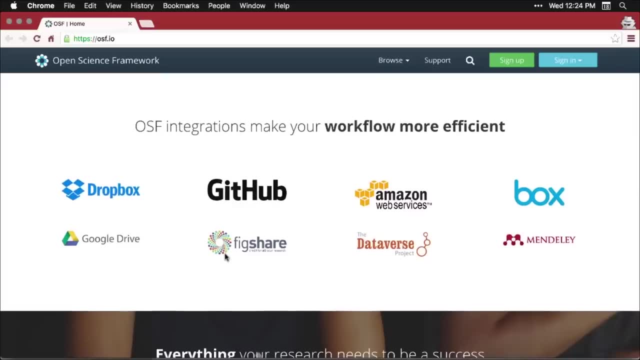 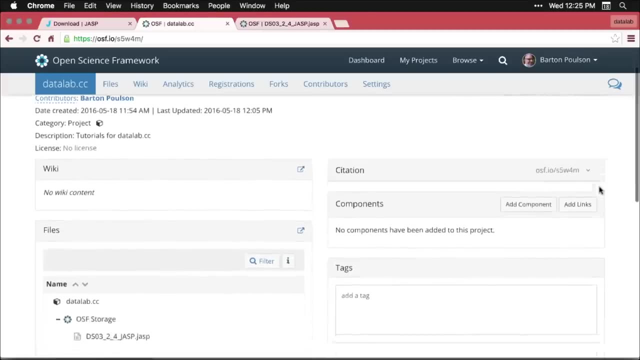 And I really can't say enough nice things about it. What's neat about this is, once you sign up for OSF, you can create your own area, And I've got one of my own. I'll go to that right now. So, for instance, here's the data lab page in Open Science. 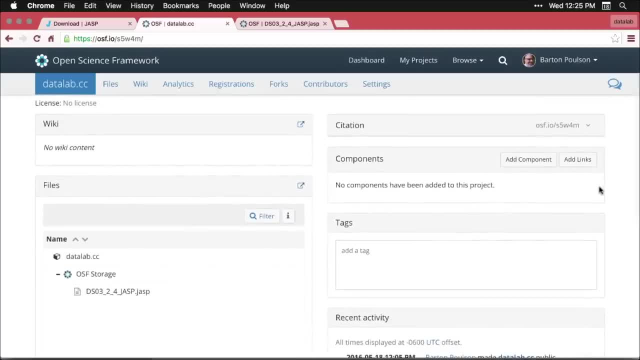 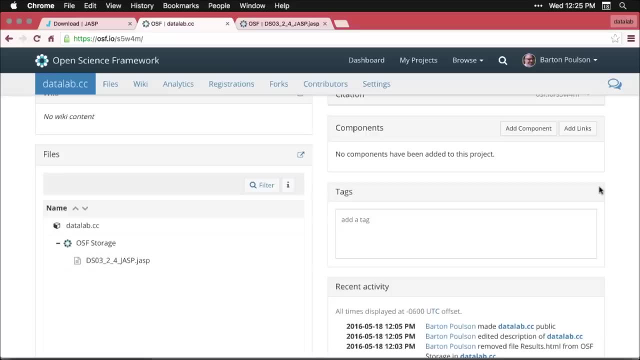 Framework, And what I've done is I created a version of this JASP analysis And I've saved it here. In fact, let's open up my JASP analysis in JASP And then I'll show you what it looks like in. 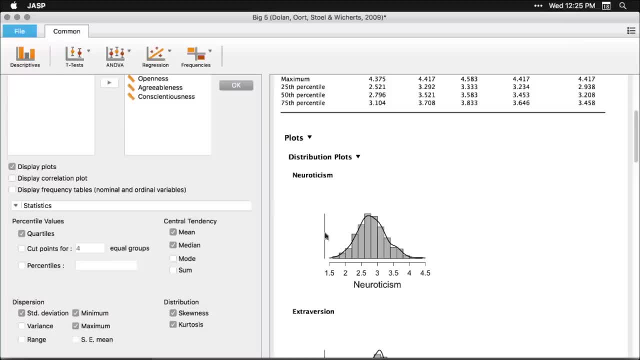 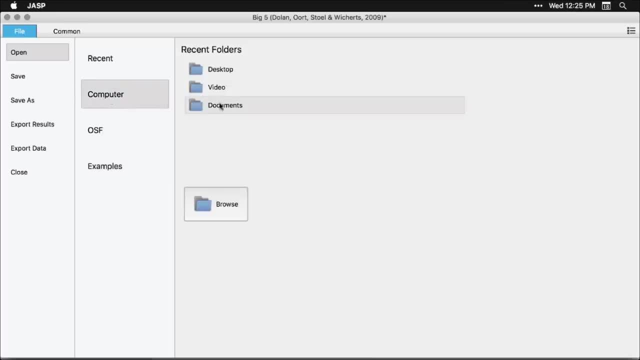 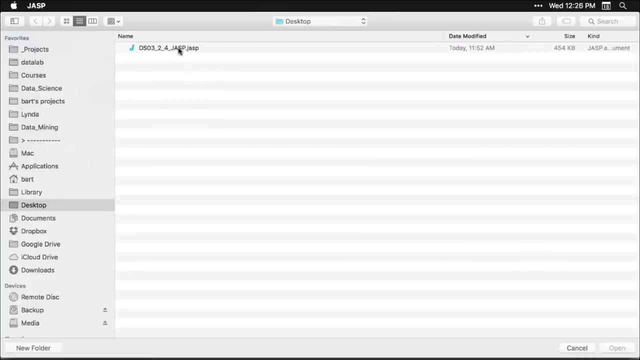 OSF. So let's first go back to JASP And when we're here we can come over to file and click computer. And I just saved this file to the desktop. Click on desktop And you will should have been able to download this with all the other files. 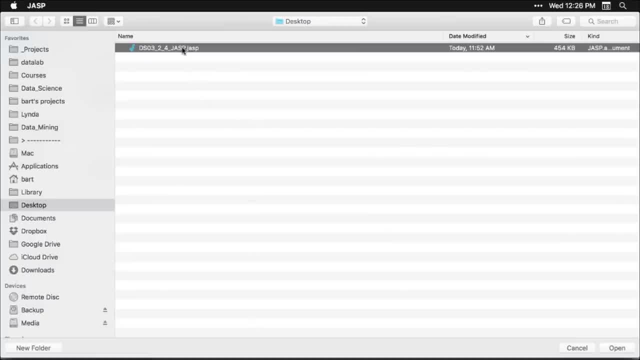 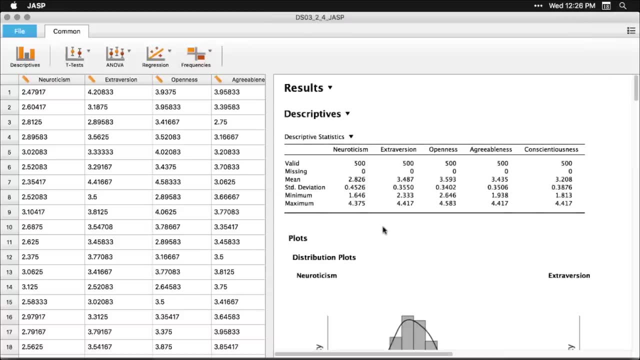 dso324 JASP And double click on that to open it. And now it's going to open up a new window And you see working with the same data set. but I did a lot more analyses. I've got these graphs. 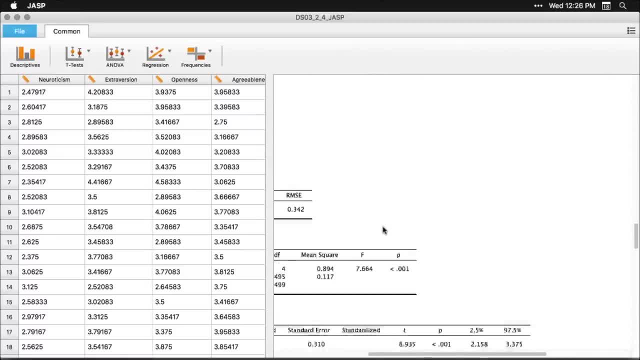 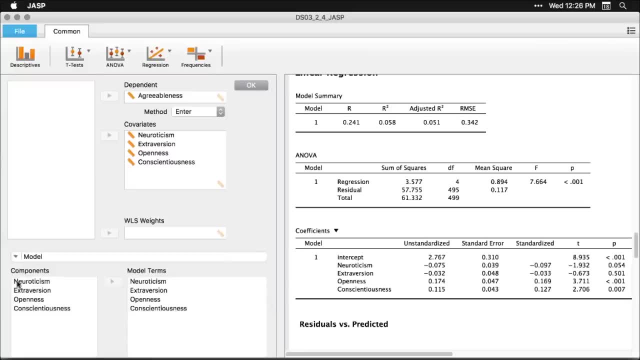 I have correlation scatter plots come down here. I did a linear regression And we just click on that And you can see the commands that produced it as well as the options. Didn't do anything special for that, But I did do some confidence intervals and specified that. 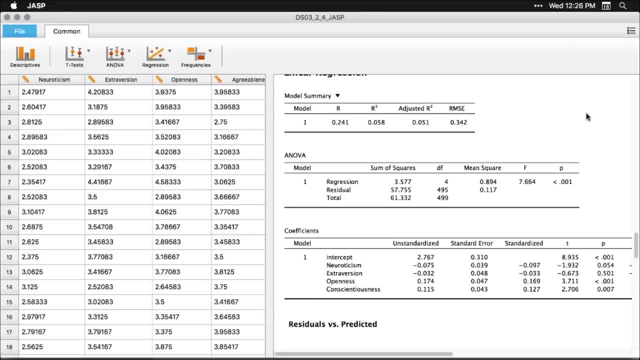 And it's really a great way to work with all this. I'll click back in an empty area And you can see the commands go away, And so I've got my output here in JASP And I've got my output here in JASP. 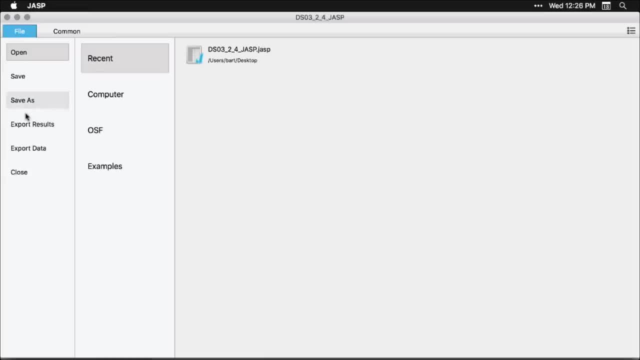 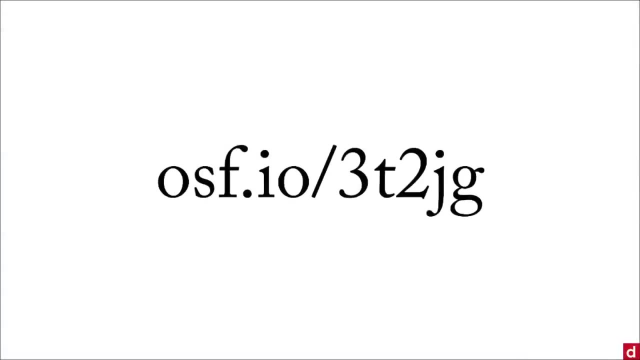 when I saved it, though, I had the option of saving it to OSF. In fact, if you go to this web page, osfio slash three, t, two, j, g- you'll actually be able to go to a page where you can. 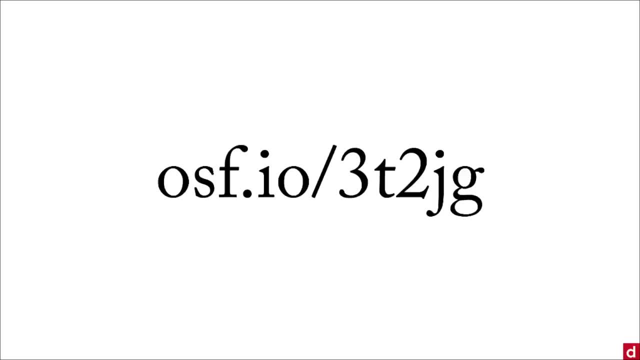 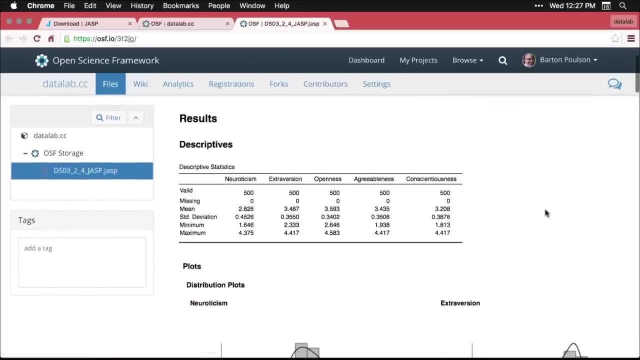 see and download the analysis that I conducted. Let's take a look. This is that page. there's the address I just barely gave you, And what you see here is the same analysis that I conducted. It's all right here. So if you're collaborating with people or if you want to show things to, 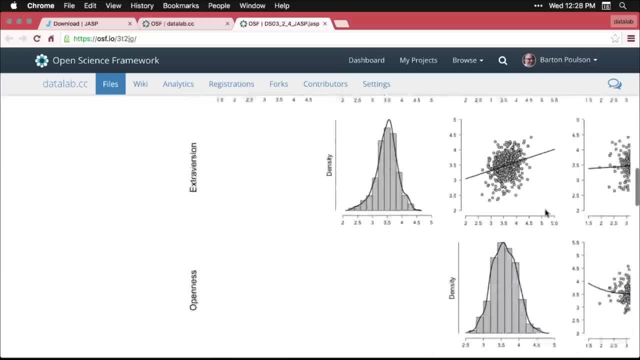 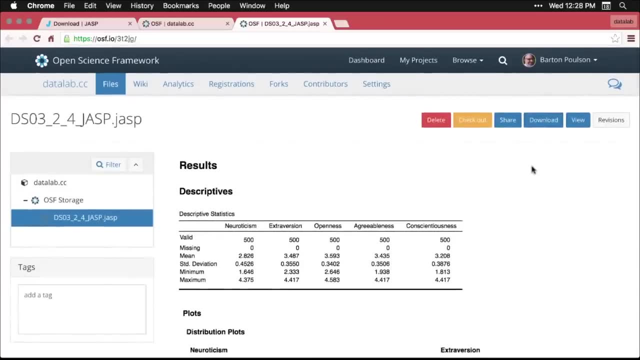 people. this is a wonderful way to do it. Everything's right there Now. this is a static image, But up at the top people have the option of downloading the original file and working with it on their own. So, in case you can't tell, I'm really enthusiastic about JASP and about its 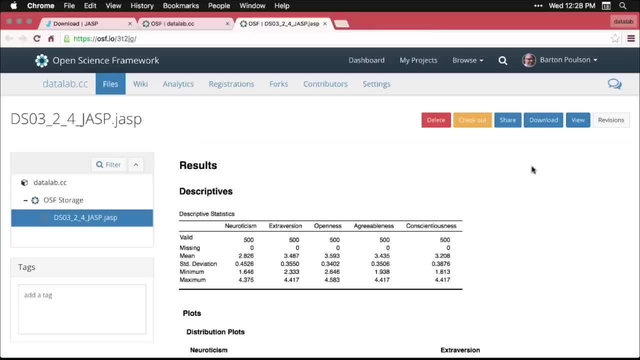 potential- still in beta, still growing rapidly. I see it really as an open source, free and collaborative replacement SPSS And I think it's going to make data science work so much easier for so many people. I strongly recommend you give JASP a close look. 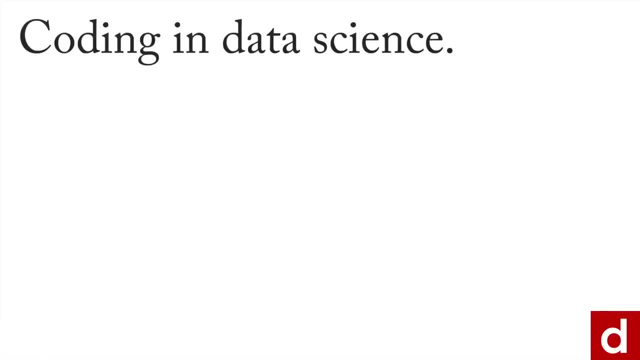 Let's finish up our discussion of coding and data science- the applications part of it- by just briefly looking at some other software choices, And I'll have to admit it gets kind of overwhelming because there are just so many choices. Now there's there's an addition to the spreadsheets. 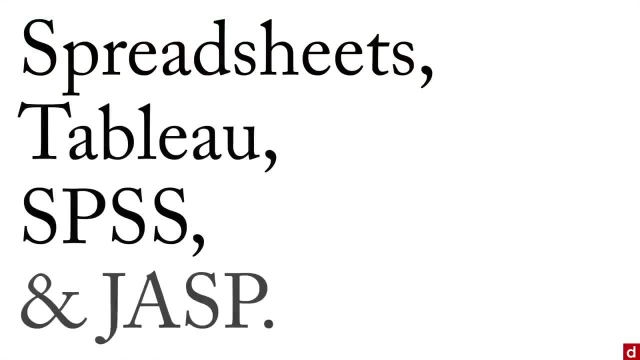 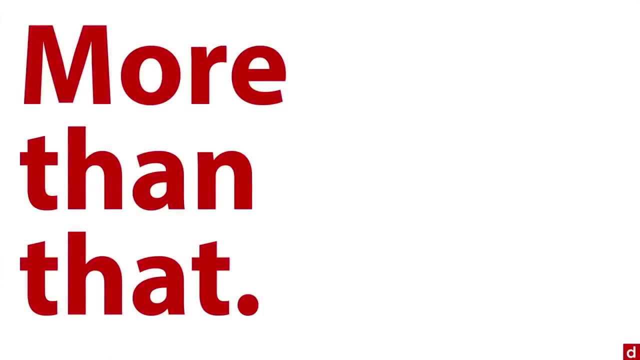 and Tableau and SPSS And JASP that we've already talked about. I mean, there's so much more than that. I'm going to give you a range of things that I'm aware of, And I'm sure I've left out some important ones or things. 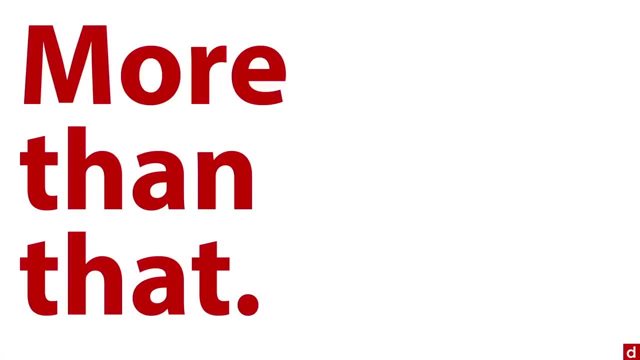 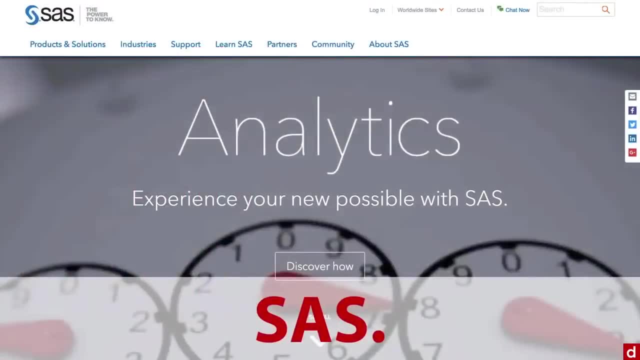 that other people like really well. But these are some common choices and some less common but interesting ones. Number one in terms of things that I did not mention is SAS. SAS is an extremely common analytical program, very powerful use for a lot of things. It's actually the first program. that I learned And, on the other hand, it can be used for a lot of other things. For example, if I want to learn something new, I can go to my computer. I can go to my computer, I can go to my. 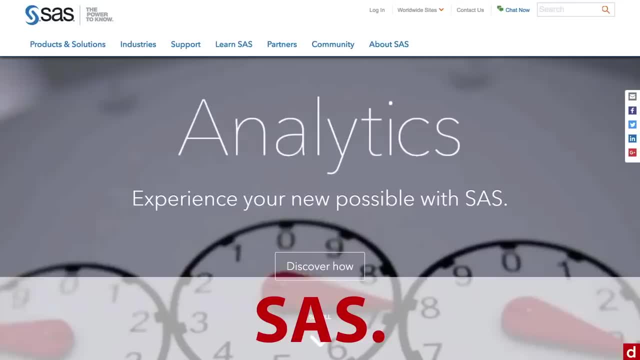 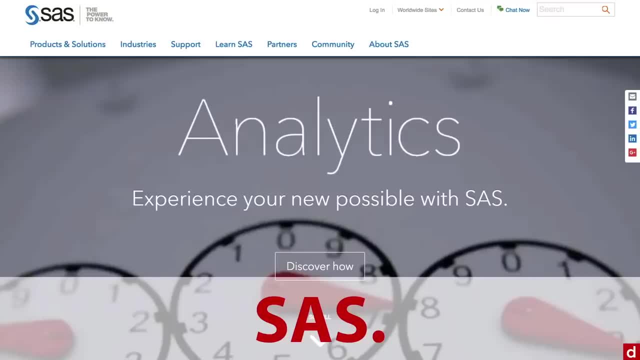 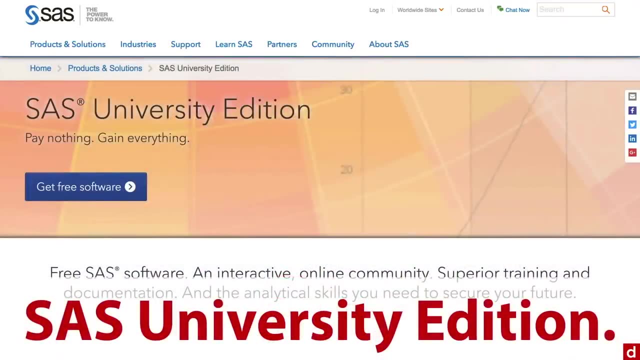 a couple of interesting alternatives. SAS also has something called the SAS University Edition. If you're a student, this is free And it's slightly reduced in what it does, But the fact that it's free and also it runs in a virtual machine, which makes it an enormous download. 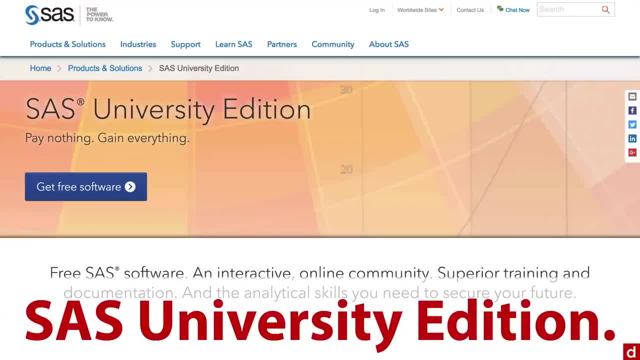 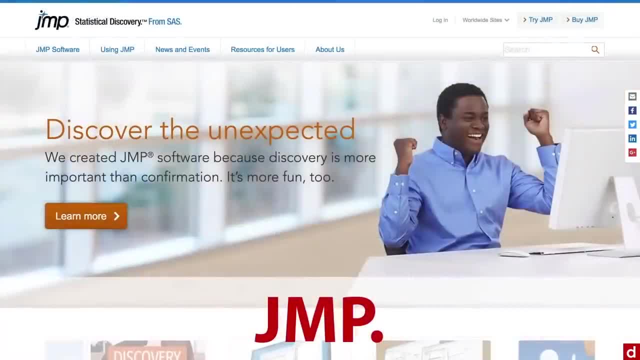 I really like And it's a program that I really like And it's a program that I really love. We're not so extraordinarily expensive And that is called jump And it's a visualization software. Think a little bit of like Tableau, how we saw you work with it visually. And this one 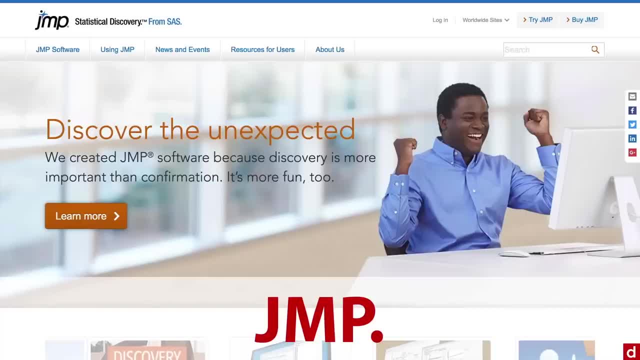 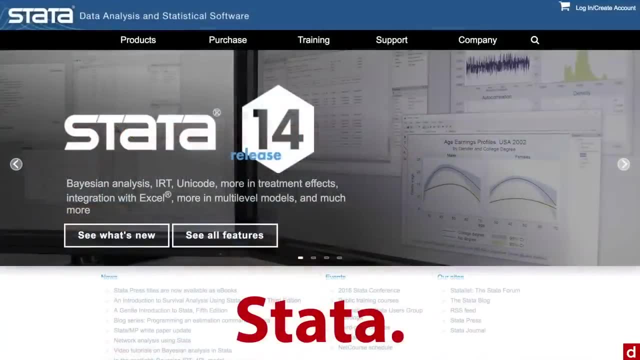 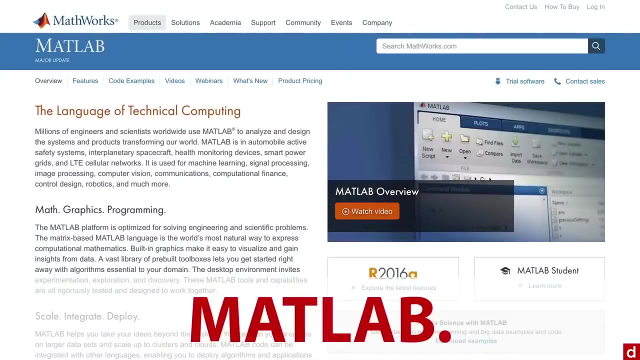 you can drag things around. It's a really wonderful program. I personally find it prohibitively expensive. Another very common choice among working analysts is Stata, And some people use mini tab. Now for mathematical people, there's MATLAB, And then, of course, 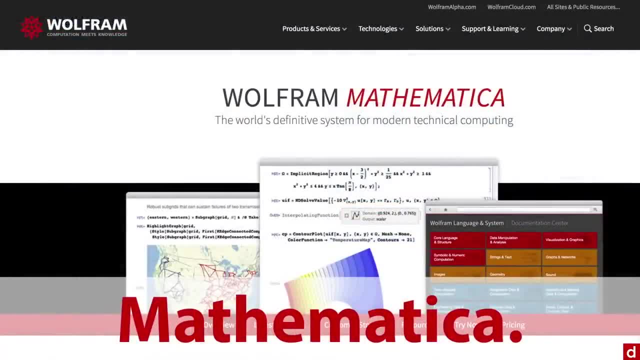 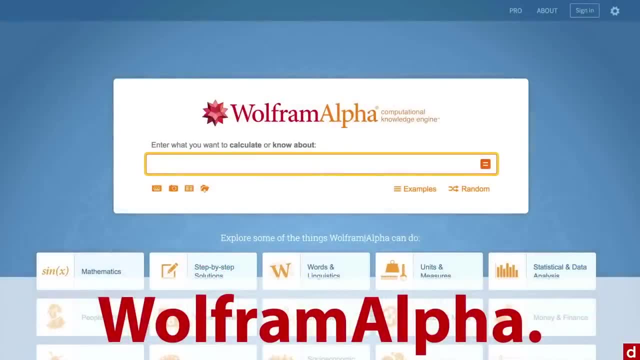 there's Mathematica itself, But that's really more a language than program. On the other hand, Wolfram, who makes Mathematica, is also the people who give us Wolfram alpha. Most people don't think of this as a stats application because you can run it on your iPhone, But Wolfram alpha is in fact. 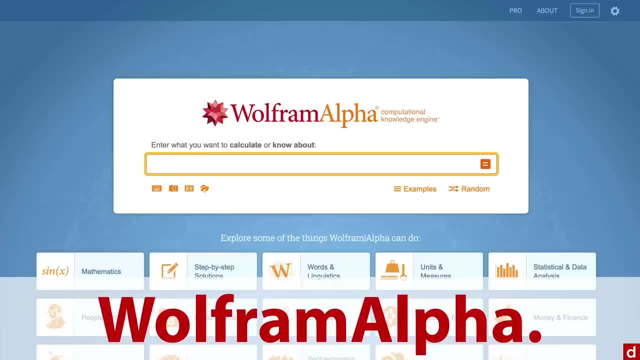 incredibly capable, And, especially if you pay for the pro account, you can do amazing things in this, including analyses, regression models, visualizations, And so it's worth taking a little closer look at that also, because it actually provides a lot of the data that you need. So 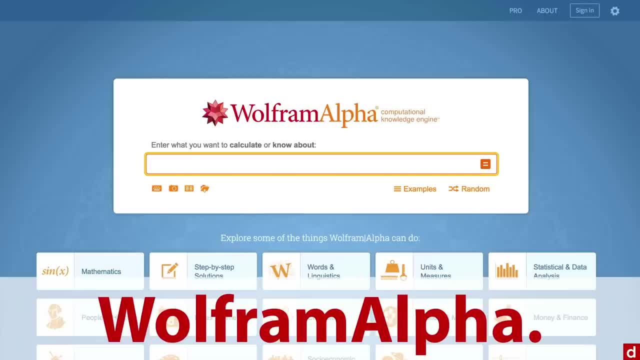 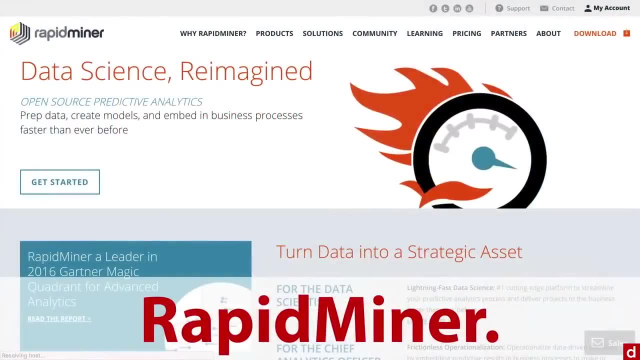 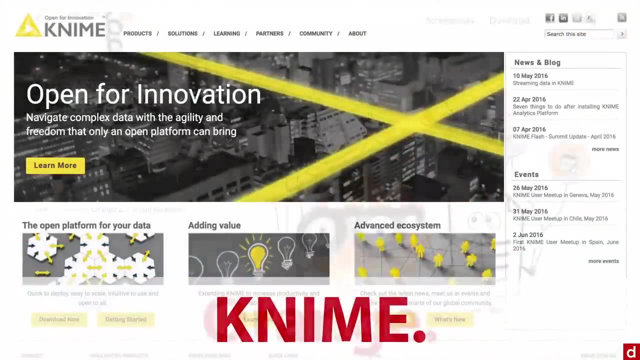 Wolfram alpha is an interesting one. Now several applications that are more specifically geared towards data mining, So you don't want to do your regular. you know little t tests and stuff on these. But there's rapid miner And there's nine and orange And those are all really nice to use. 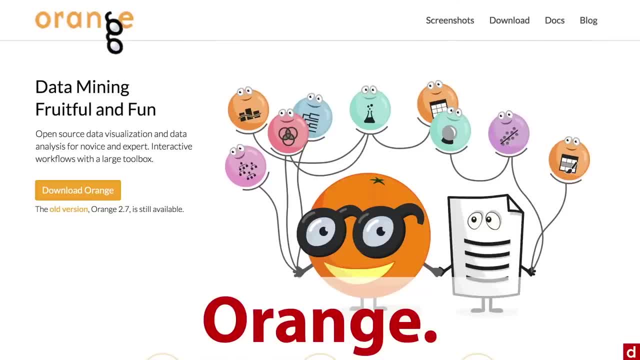 because they are control languages where you drag nodes onto a screen and you can connect them with lines And you can see how things run through. All three of them are free or have free versions And all three of them work in pretty similar manners. There's also big ml. 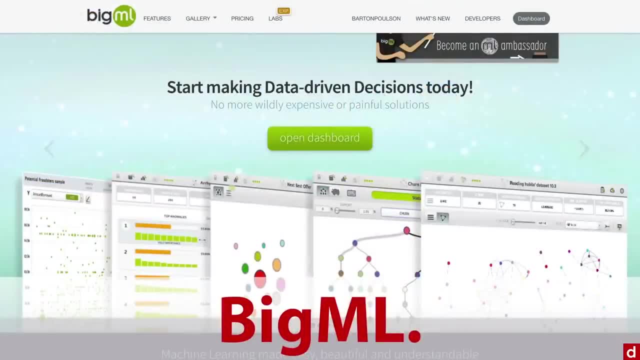 which is for machine learning, And this is unusual because it's browser based. it runs on their servers. There's a free version. although you can't download a whole lot, doesn't cost a lot to use big ml And actually is a very friendly, very accessible program. 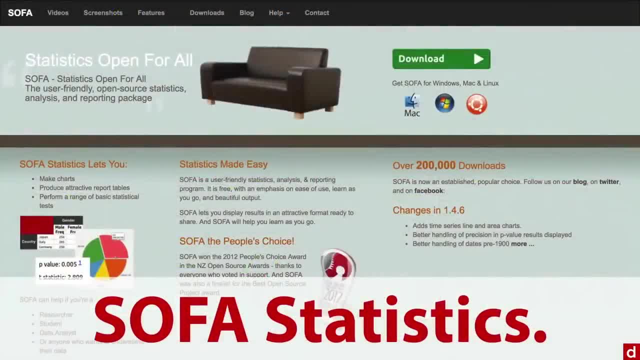 Then, in terms of programs you can actually install for free on your own computer, there's one called SOFA statistics. That means statistics open for all kind of a cheesy title, but it's a good program. And then one with a web page straight out of 1990 is past three. This is 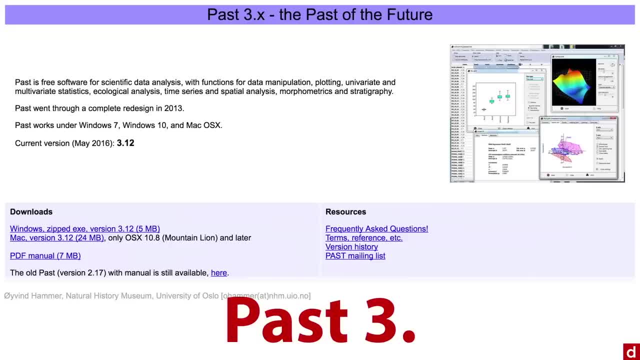 palaeontological software, on the other hand, does do very general stuff. It runs on many platforms And it's a really powerful thing And it's free, but it is relatively unknown. And then, speaking of relatively unknown, one that's near and dear to my heart is a web application called 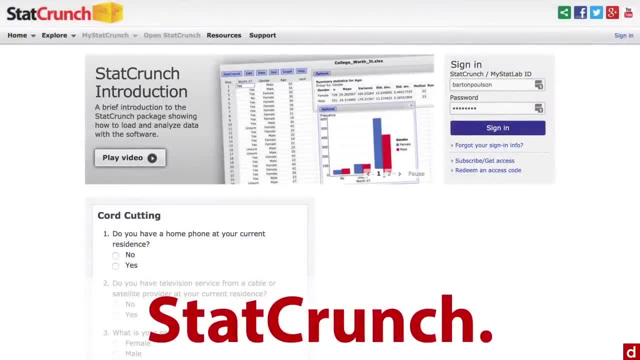 stat crunch. It costs, but it costs like six or 12 bucks a year. It's. it's really cheap And it's very good, especially for basic statistics And for learning. I used it in some of the classes that I was teaching. And then, if you're deeply wedded to Excel and you just can't stand to, 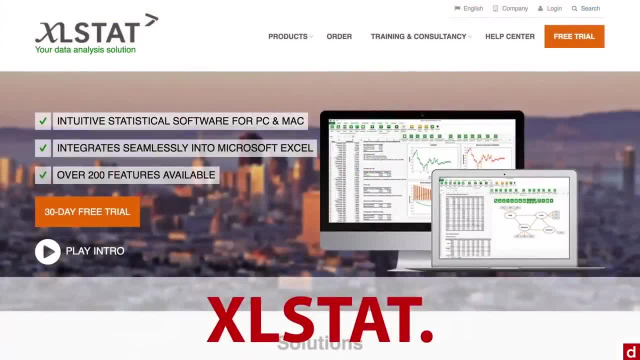 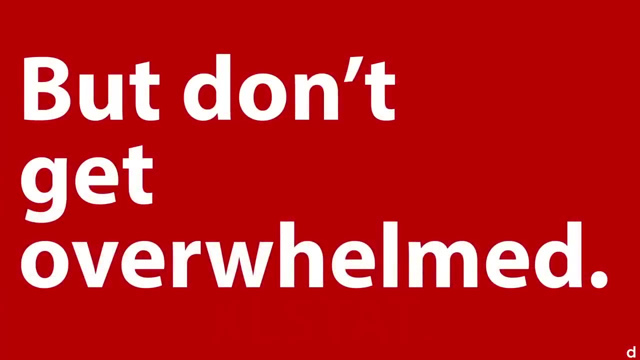 leave that environment. you can purchase add ins like Excel stat, which give you a lot of statistical functions within the Excel environment itself. That's a lot of choices And the most important thing here is: don't get overwhelmed. There's a lot of choices but you don't even have. 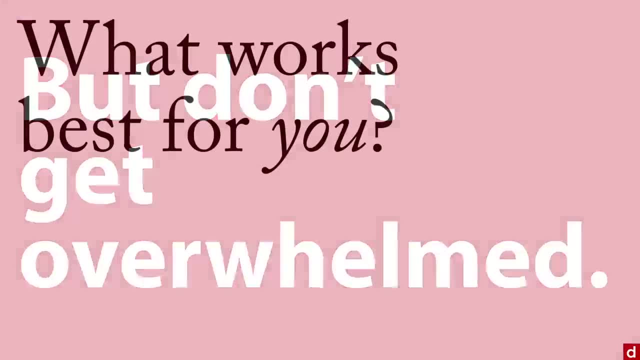 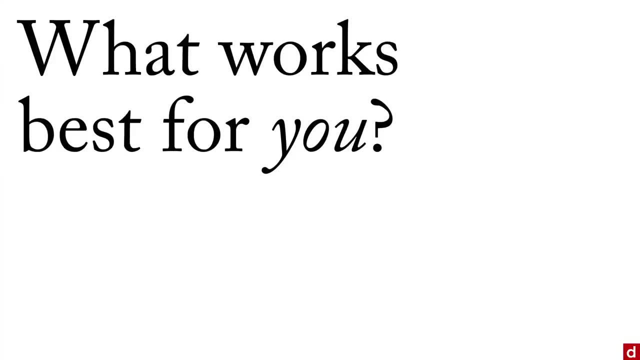 to try all of them. Really, the important question is what works best for you and the projects that you're working on. There's a few things you might want to consider in that regard. First off is functionality. Does it actually do what you want, Or does it even run on your machine? You don't. 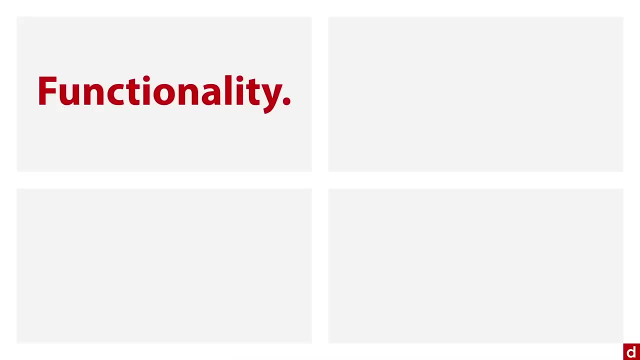 need everything that a program can do. I mean, think about all the stuff that Excel can do. People probably use one 5% of what is available. Then there's also ease of use. Some of these programs are a lot easier to use than the others. 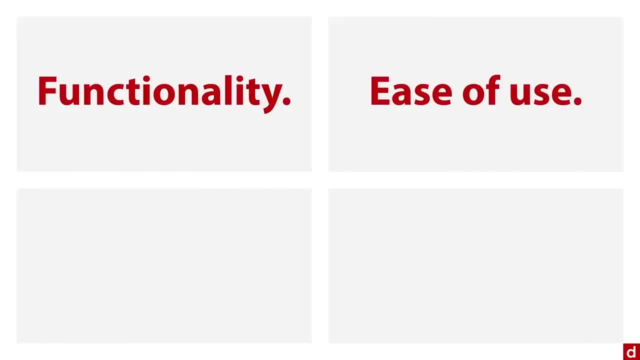 And I personally find that the ones that are easy to use I like them, And so you might say, no, I need to program because I need to do custom stuff, But I'm willing to bet that 95% of what people do does not require anything. custom Also the existence of a community Constantly. 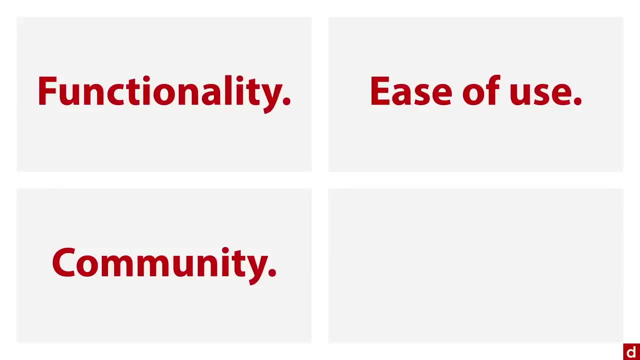 when you're working you come across problems, don't know how to solve it, and being able to simply get online and do a search for an answer and have enough of a community that there are people there who have put answers up and discuss these things- Those are wonderful. Some of these programs have very substantial communities. 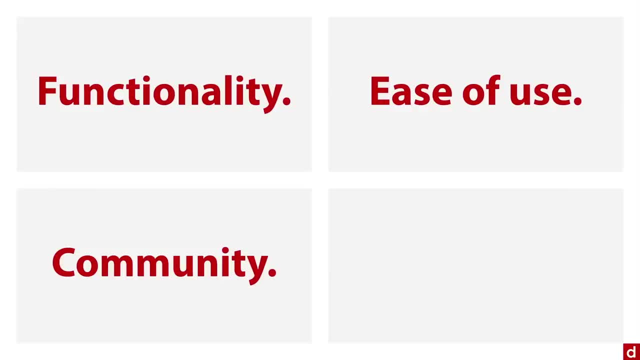 some of them it's practically non existent, and you get to decide how important that is to you. And then finally, of course, there's the issue of cost. Many of these programs I mentioned are free. Some of them are very cheap. Some of them run on sort of a freemium model and some of them are 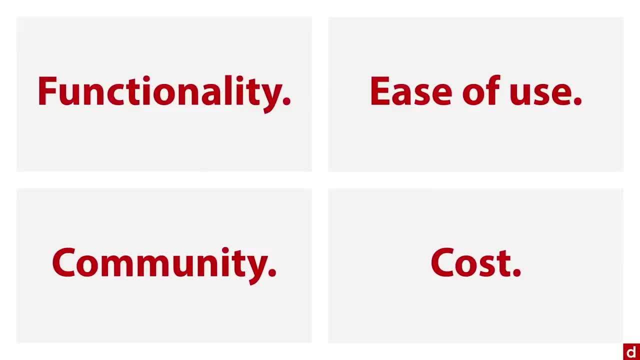 outrageously expensive, So you don't have to buy them unless somebody else is paying for it. So these are some of the things that you want to keep in mind when you're trying to look at various programs. Also, let's mention this: 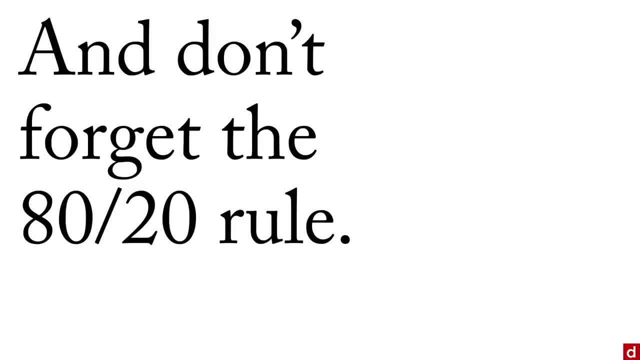 don't forget that 8020 rule. you're going to be able to do most of the stuff that you need to do with only a small number of tools. one or two, maybe three will probably be all that you ever need, So you don't need to explore the range of every possible tool. Find something that does what. 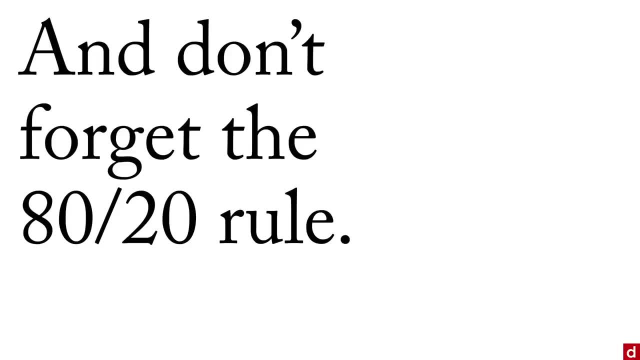 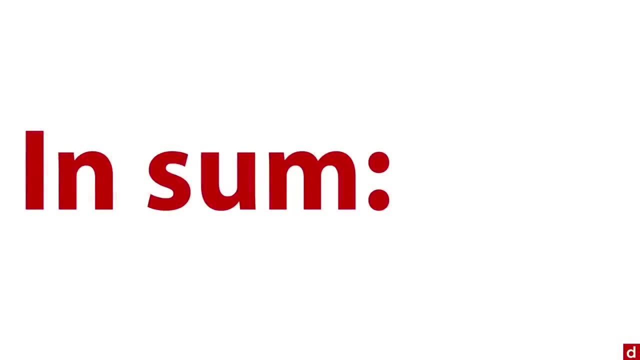 you need Find something you're comfortable with and really try to extract as much value as you can out of that. So, in sum, in our discussion of available applications for coding and data science, First remember applications are tools. they don't drive you, you use them, and that your goals are what drive the choice of your. 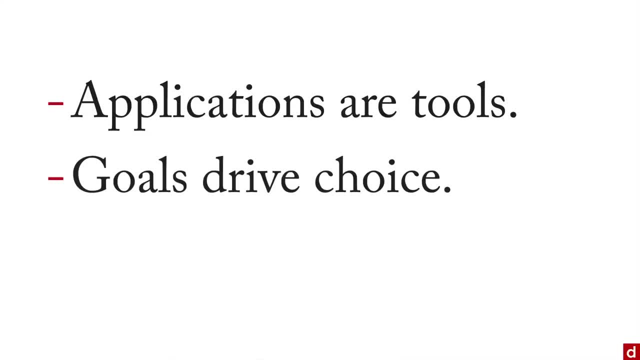 applications and the way that you do it. And the single most important thing is remember what works for you may work well for somebody else If you're not comfortable with it. if it's not the questions you address, then it's more important to think about what works for you. 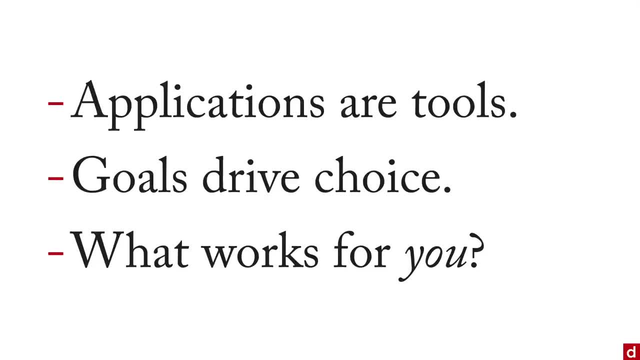 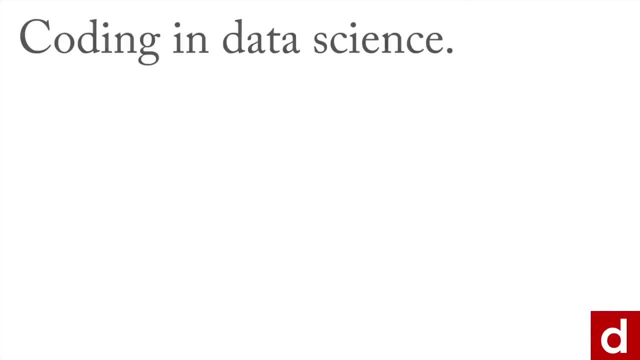 and the projects that you're working on, as you make your own choices for tools for working in data science. When you're coding in data science, one of the most important things you can do is be able to work with web data, And if you work with web data, you're going to be working with HTML. 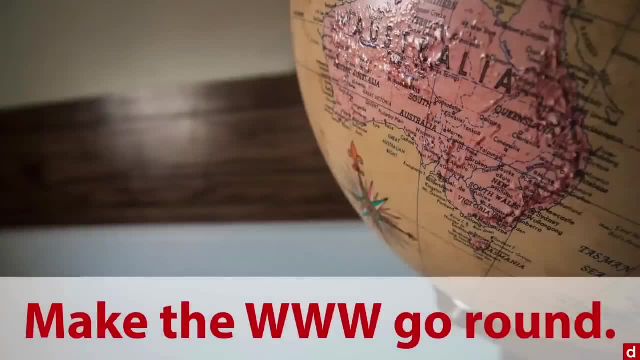 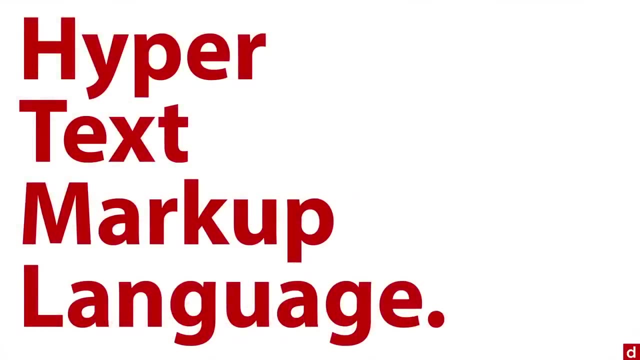 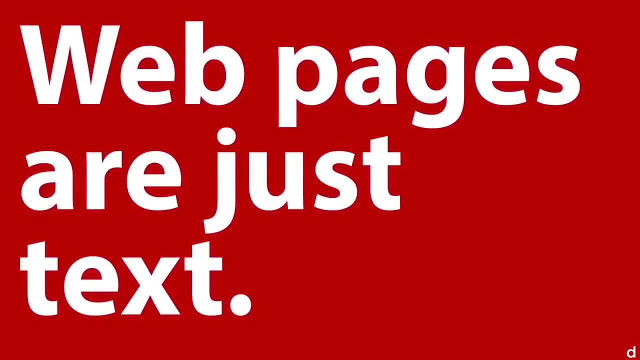 Now, in case you're not familiar with it, HTML is what makes the World Wide Web go round. What it stands for is hyper text markup language, And if you've never dealt with web pages before, here's a little secret. Web pages are just text. It's just a text document, But it uses tags to. 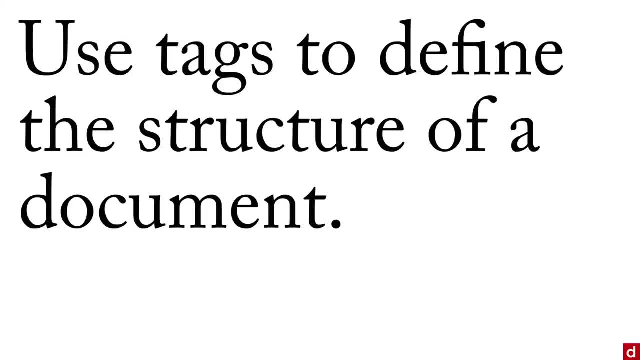 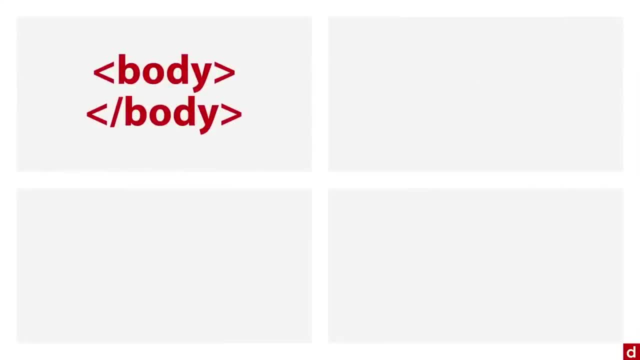 define the structure of the document And a web browser knows what those tags are and it displays them in the right way. So, for instance, some of the tags, they look like this: they're in angle bracket and then a beginning tag, so body. then you have the body, the main part of your text, And 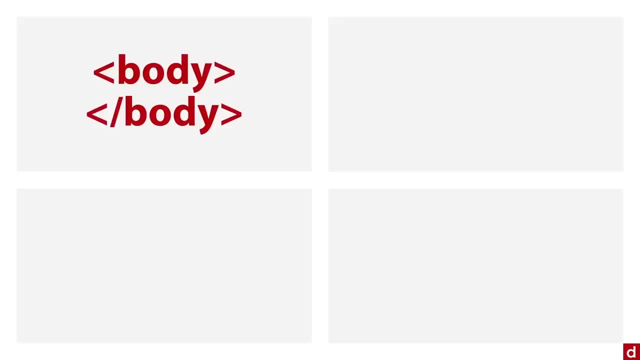 then you have an angle brackets and a backslash body to let the computer know that you're done with that part. You also have P and backslash P for paragraphs. H1 is for header one and you put it in between that text. TD is for table data or the cell in a table, And you mark it off that way. 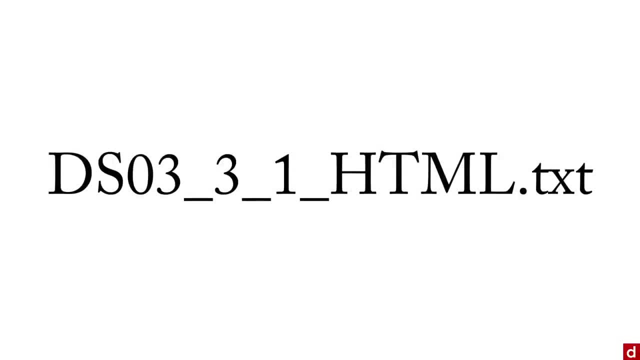 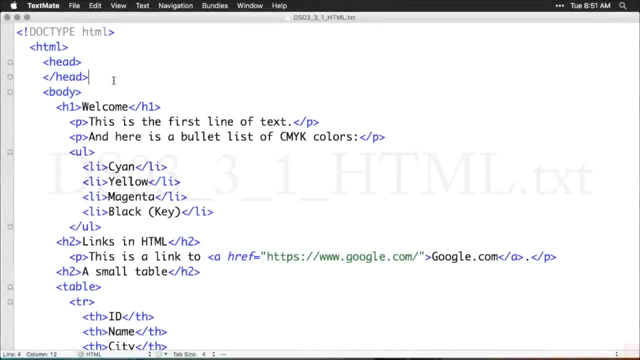 If you want to see what it looks like, just go to this document: dso3, three one html dot txt. I'm going to go to that one right now. Now, depending on what text editor you open this up, it may actually give you the web preview. I've opened it up in textmate And 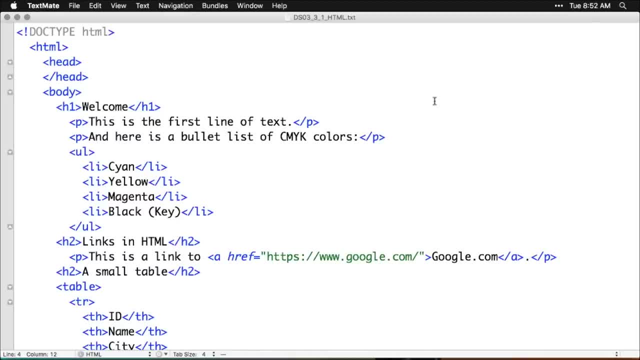 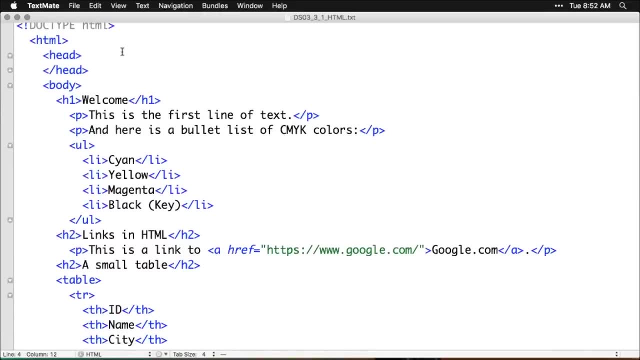 so it actually is showing the text the way I typed it. I typed this manually, just typed it all in there And I have HTML to see what a document is. I have an empty header, but that sort of needs to be there. This I saved and I'm going to put it in here And I'm going to say I'm going to type it in. 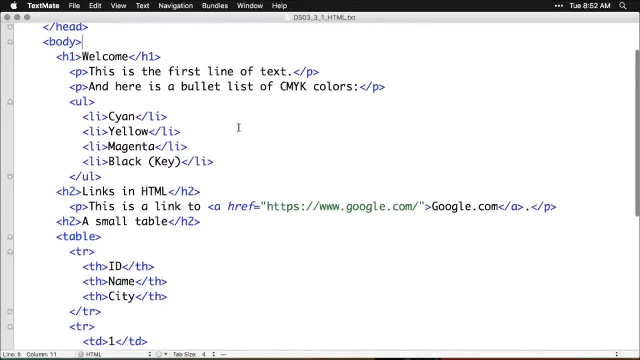 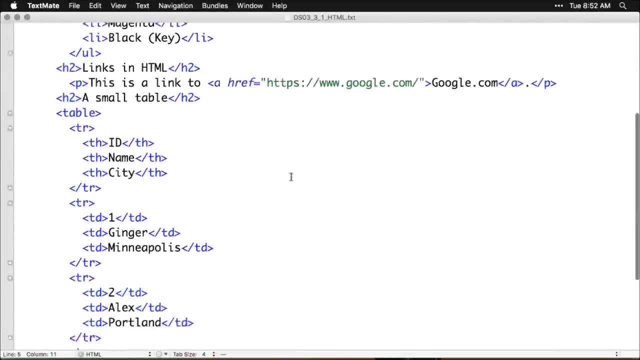 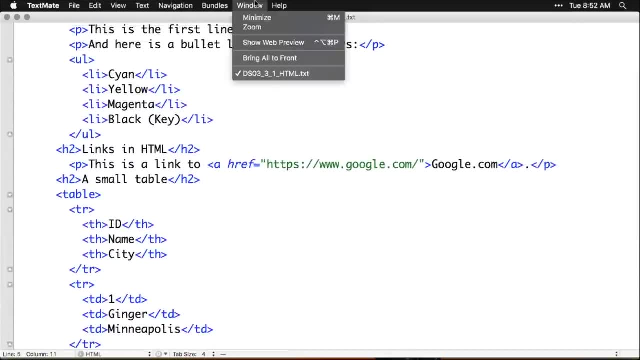 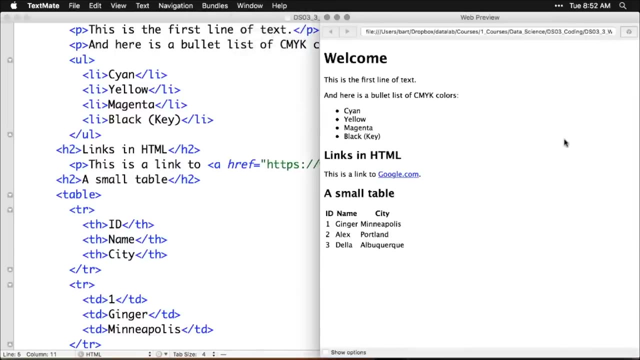 for a link to a web page, Then I have a small table And if you want to see what this looks like when it's actually displayed as a web page, we'll just go up here to window and show web preview. This is the same document, but now it's in a browser, And that's how you make a web page. 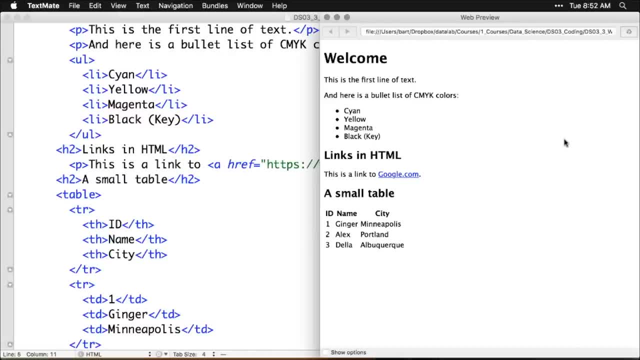 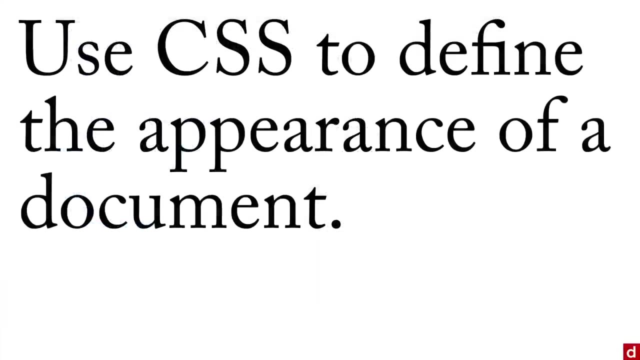 Now, I know this is very fundamental stuff, But the reason this is important is because if you're going to be extracting data from the web, you have to understand how that information is encoded in the web and is going to be in HTML most of the time for a regular web page. Now I will mention 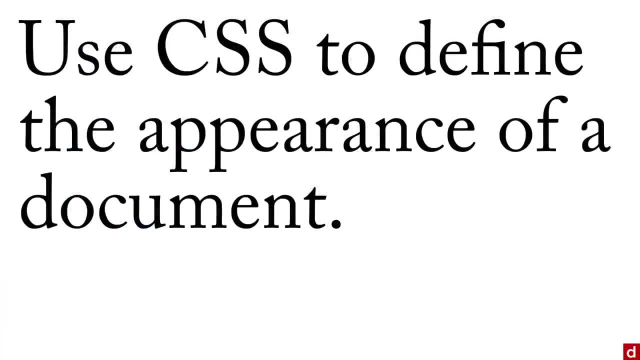 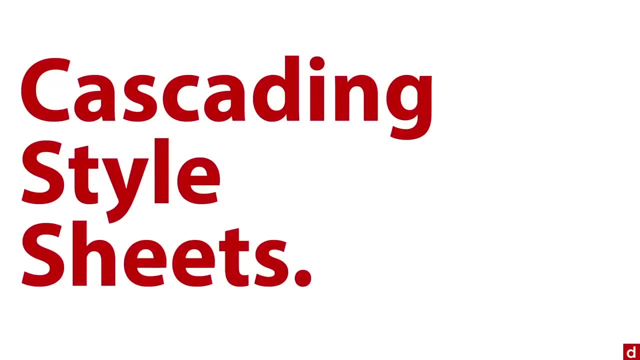 something that there's another thing called CSS, and web pages use CSS to define the appearance of a document. HTML is theoretically there to give the content and CSS gives the appearance, and that stands for cascading style sheets. I'm not going to worry about that right now, because we're 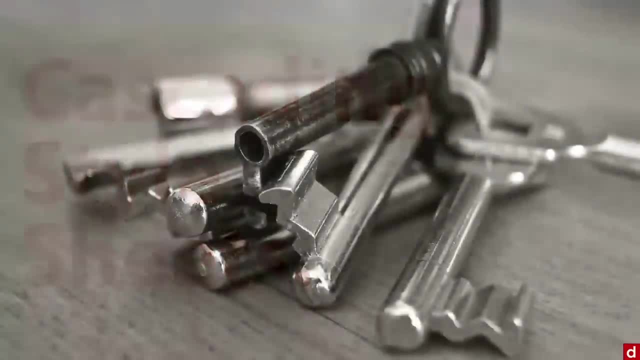 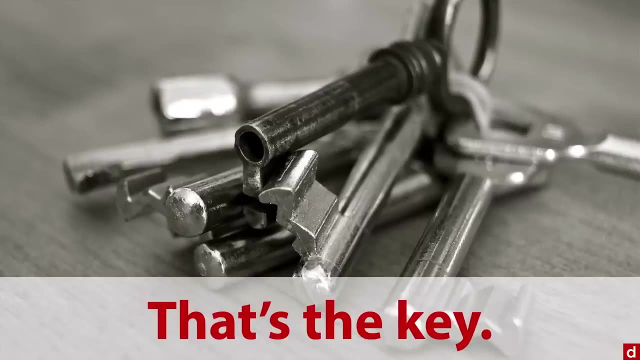 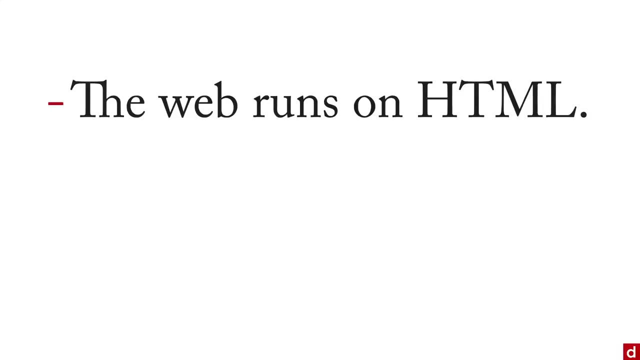 really interested in the content. And now you have the key to being able to read web pages and pull data from web pages for your data science projects. So, in sum, first, the web runs on HTML. that's what makes the web pages that are there. HTML defines the page structure and the content. 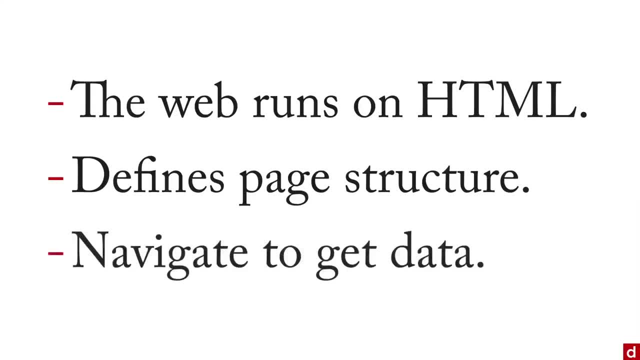 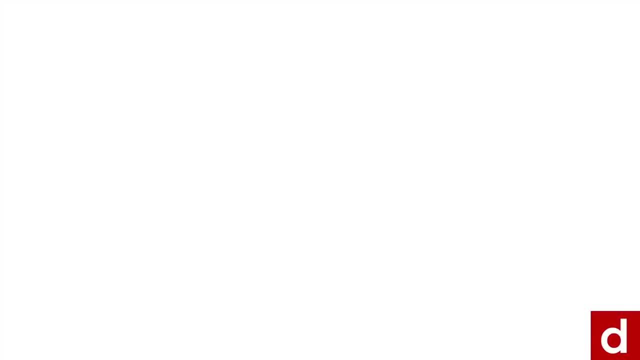 that's in the page And you need to learn how to navigate the tags And the structure in order to get data from the web pages for your data science projects. The next step in coding and data science, when you're working with web data, is to understand. 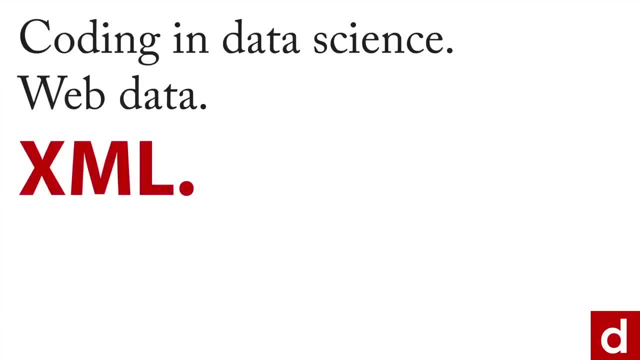 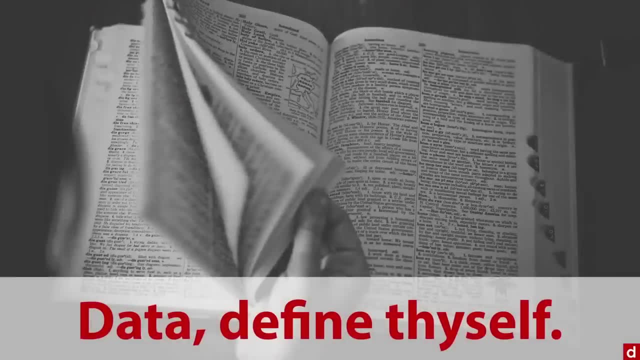 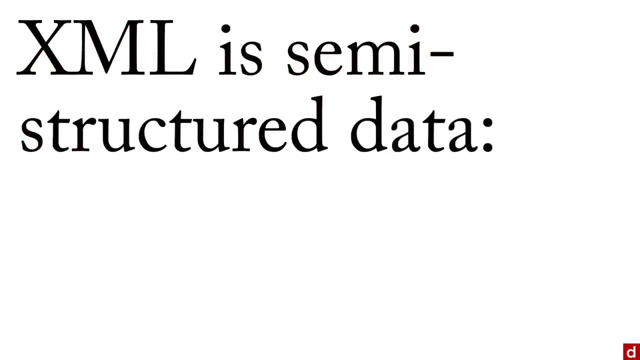 a little bit about XML. I'd like to think of this as the part of web data that follows the imperative data defined thyself. XML stands for extensible markup language, And what it is XML is semi structured data. What that means is that data is structured data, And what that means is that. 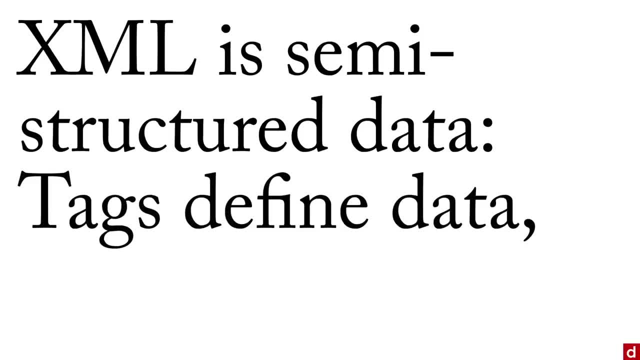 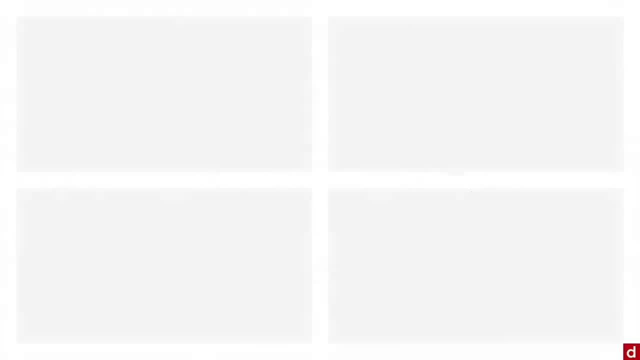 tags define data, So computer knows what a particular piece of information is. But unlike HTML, the tags are free to be defined any way you want, And so you have this enormous flexibility in there. But you're still able to specify it so the computer can read it. Now there's a couple of 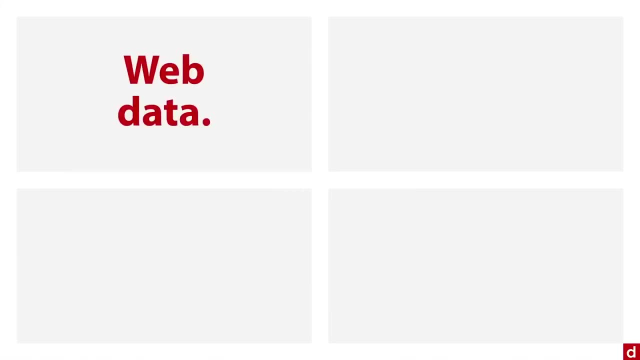 places where you're going to see XML files. Number one is in web data. HTML defines the structure of a web page, But if they're feeding data into it, then that will often come in the form of an XML File. Interestingly, Microsoft Office files if you have doc x or xls x, x part at the end stands 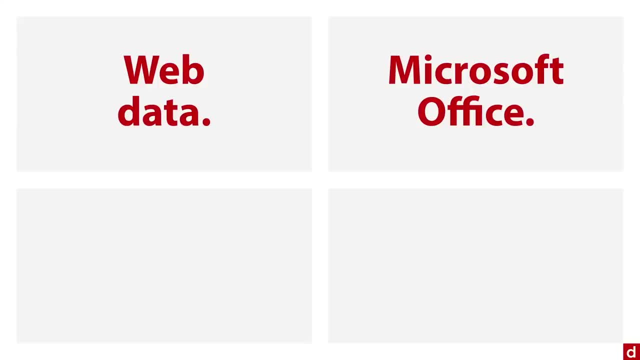 for a version of XML that's used to create these documents. If you use iTunes, the library information that has all of your artists and your genres and your ratings and stuff that's all stored in an XML file, And then, finally, data files that often go with particular programs can. 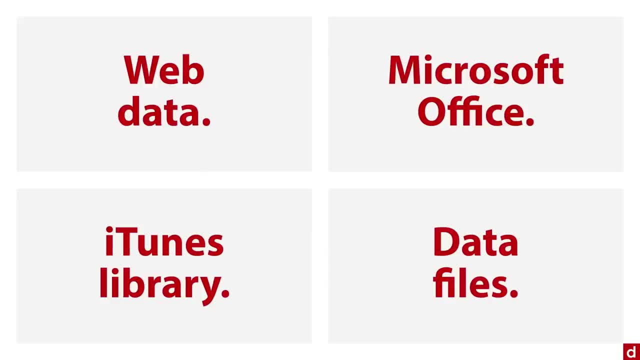 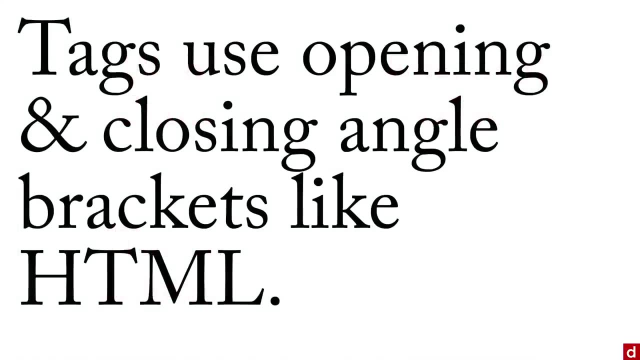 be saved as XML as well as the web pages. Now, in order to do that, you have to use a special way of representing the structure of the data to the program, And for XML tags, use opening and closing angle brackets, just like HTML did. Again, the major difference is that you're free to define. 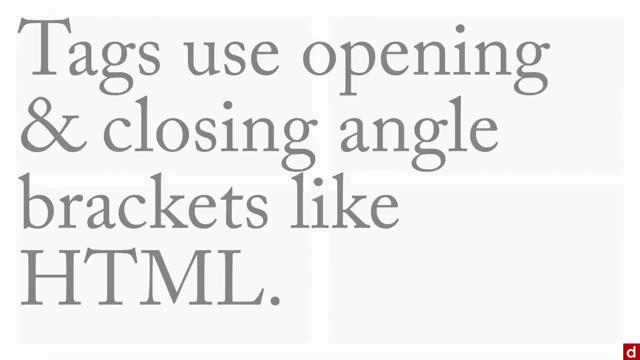 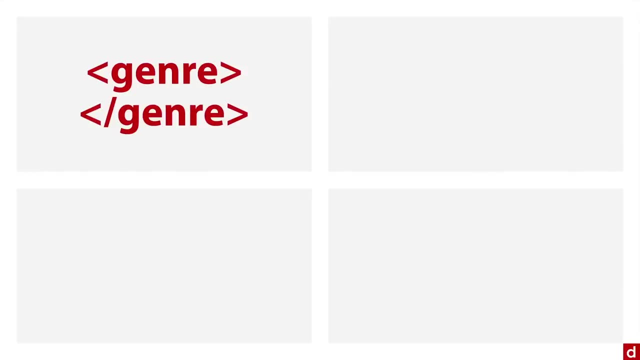 the tags however you want. So, for instance, thinking about iTunes, you can define a tag, this genre, and you have the angle brackets and genre to begin that information. And then you have the angle brackets with the backslash to let it know you're done with that piece of information. 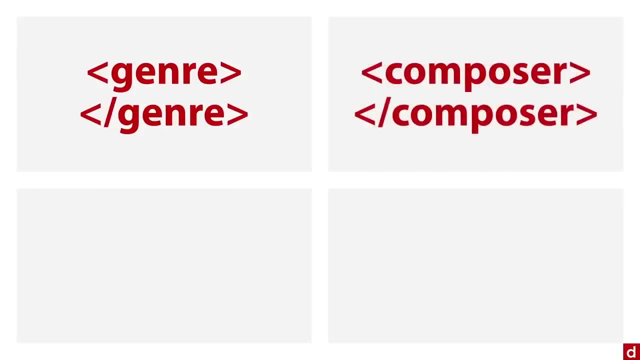 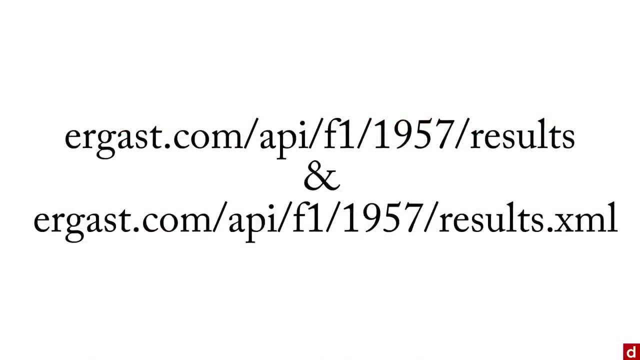 Or you can do it for composer, or you can do it for rating, or you can do it for comments, And you can create any tags you want And you put the information in between those two things. Now let's take an example of how this works. I'm going to show you a quick data set that comes. 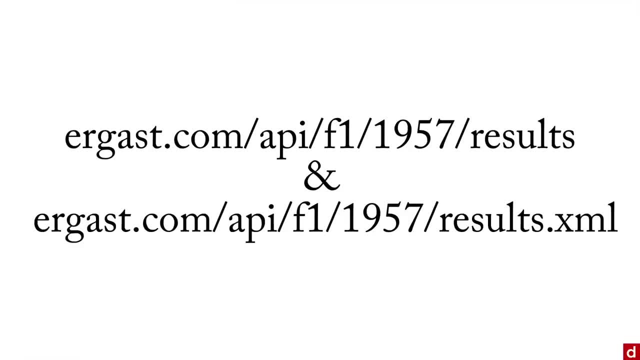 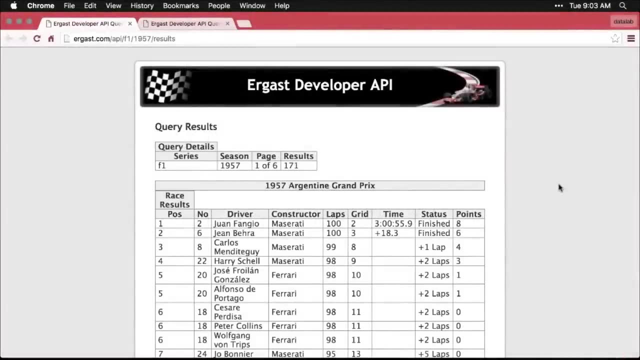 from the web. It's at air gascom And API. this is a website that stores information about automobile Formula One racing. Let's go to this web page and take a quick look at what it's like. So here we are at air gascom And it's the API for Formula One, And what I'm bringing up is 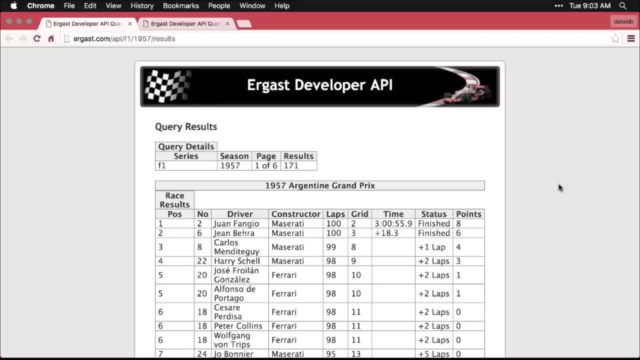 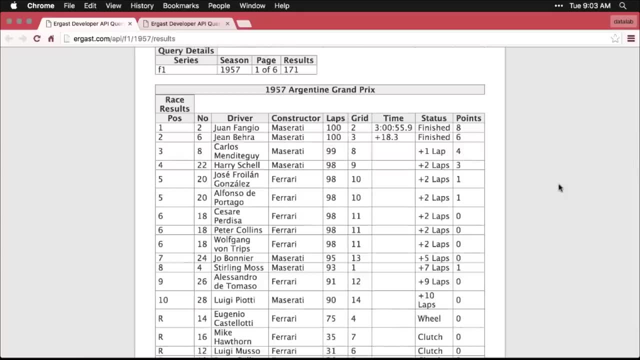 the results of the 1957 season in Formula One racing, And here you can see who the competitors were in each race and how they finished, and so on. So this is a data set that's being displayed in a web page. If you want to see what it looks like in XML, all you have to do is type XML onto. 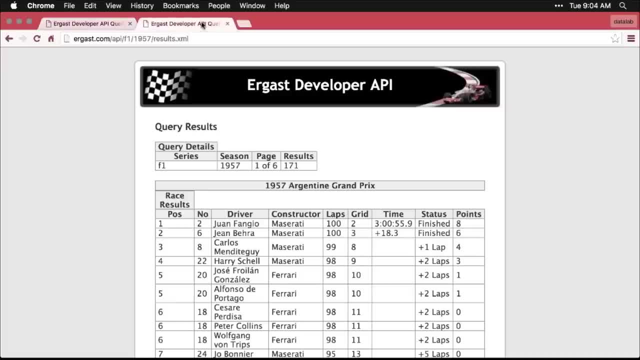 the end of this dot XML. I've done that already, So I'm just going to go to that one. And you see, it's only this little bit that I've added dot XML. Now it looks exactly the same because the web page is structuring XML data by default. But if you want to see what it looks like in its raw, 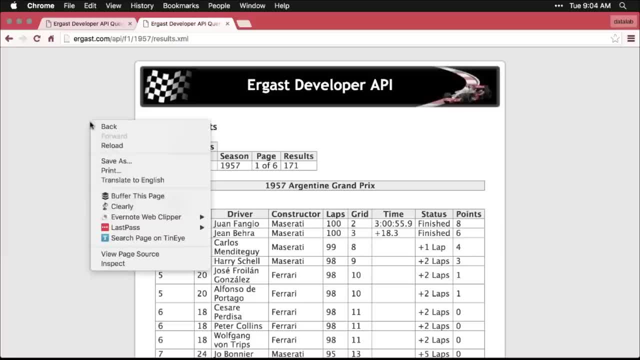 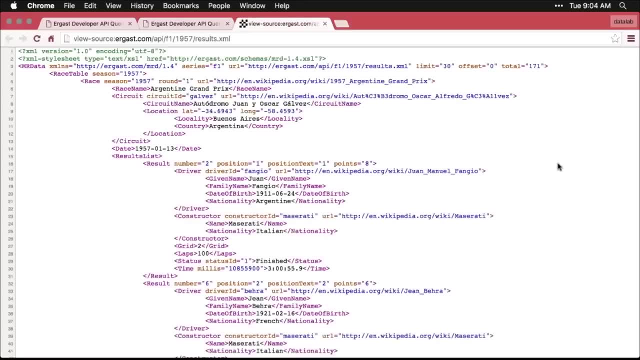 format: just do an option, click on the web page and go to view page source. at least that's how it works in Chrome. And this is the structured XML page And you can see we've got tags here. it says race name, circuit name, location And obviously these are not standard. 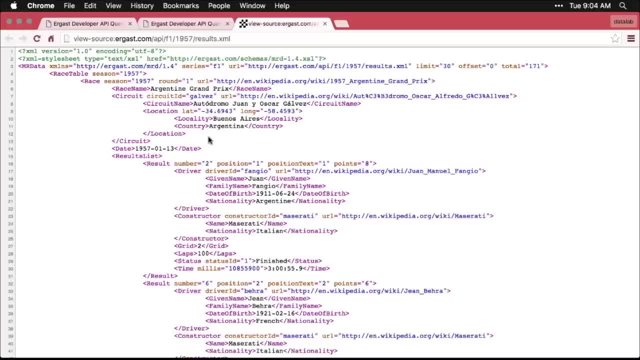 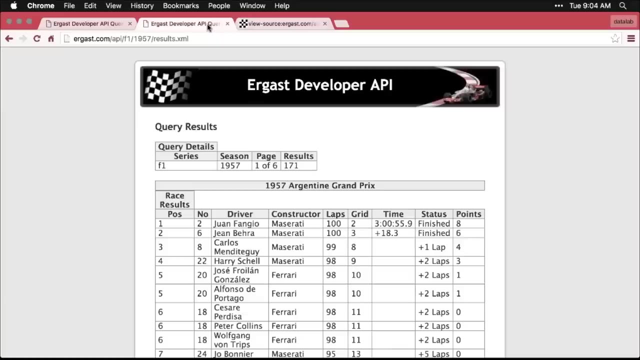 HTML tags that are defined for the purposes of this particular data set, But we begin with one. we have circuit name right there, And then we close it using the backslash right there, And so this is structured data. the computer knows how to read it, which is exactly. this is how it displays. 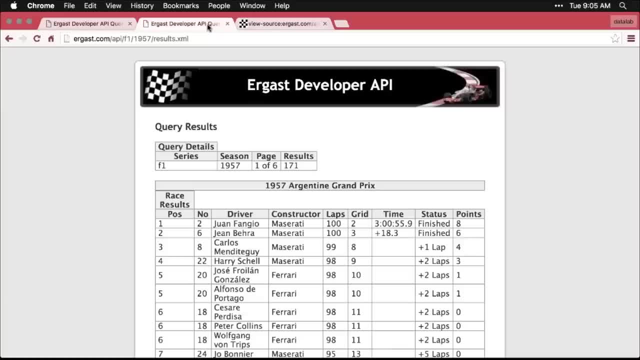 it by default, And so it's a really good way of displaying data And it's a good way to know how to pull data from the web. you can actually use what's called an API, an application programming interface, And that's what we're going to do here. So we're going to go ahead and go ahead, and 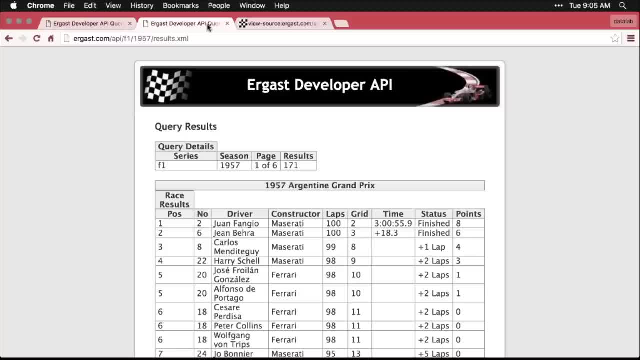 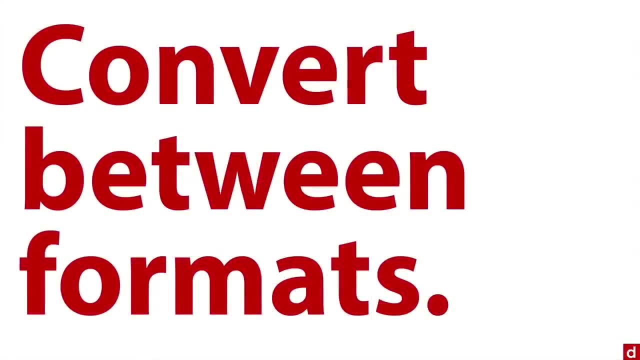 go ahead and paste all this data into this database to access this XML data, And it pulls it in along with its structure, which makes working with it really easy. What's even more interesting is how easy it is to take XML data and convert it between different formats, because it's structured. 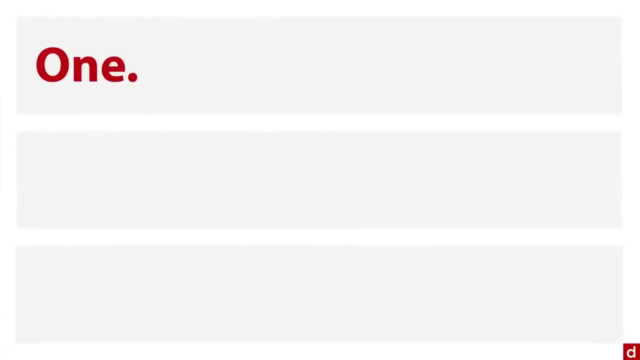 and the computer knows what you're dealing with. So, for example one, it's really easy to convert XML to CSV or comma separated value files. That's the spreadsheet format, because it knows exactly what the headings are and what piece of information goes in each column. And then you can also do a 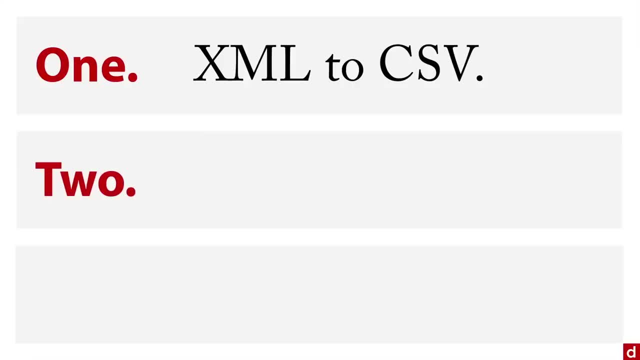 column. Example two: it's really easy to convert HTML documents to XML, Because you can think of HTML, with its restricted set of tags, as sort of a subset of the much freer XML. And three, you can convert CSV or your spreadsheet comma separated value to XML and vice versa. You can. 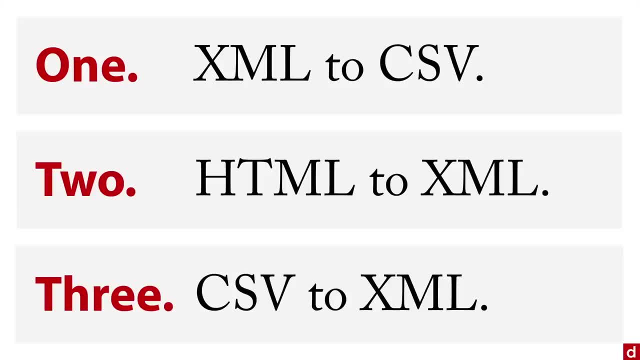 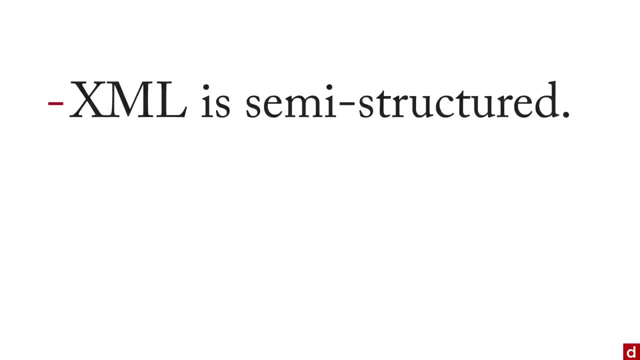 bounce them all back and forth, because the structure is made clear to the programs that you're working with. So, in sum, here's what we can say. Number one: XML is semi structured data. What that means is it has tags to tell the computer what the piece of information is. But you 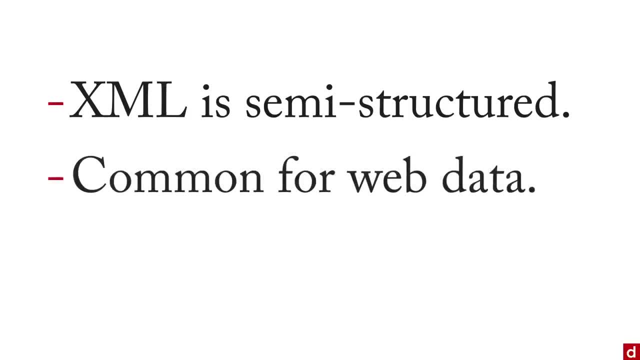 can make the tags whatever you want them to be, And XML is very common for web data And it's really easy to translate the formats: XML, HTML, CSV, so on and so forth. It's really easy to translate them back and forth. 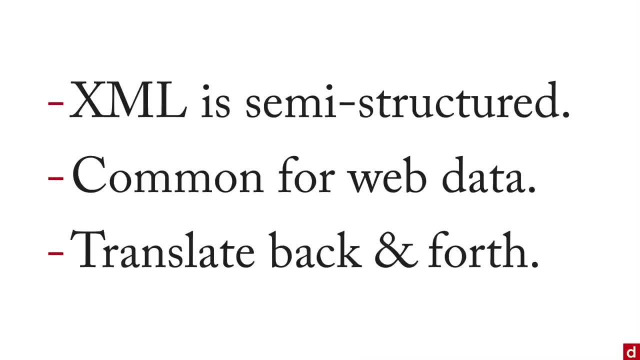 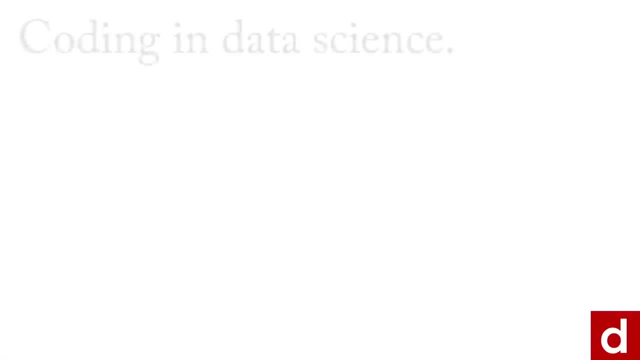 Which gives you a lot of flexibility in manipulating data So you can get into the format you need for your own analysis. The last thing I want to mention about coding and data science and web data is something called JSON, And I like to think of it as a version of. smaller is better. Now, what JSON? 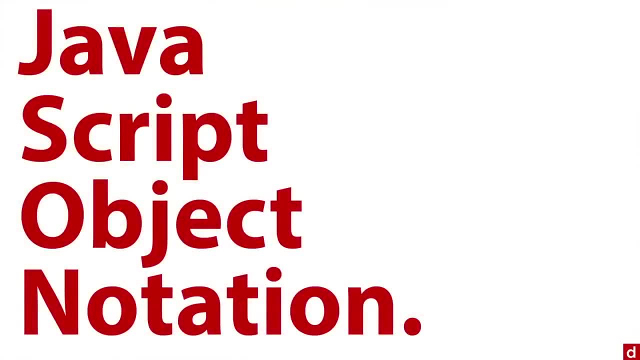 stands for is JavaScript Object Notation, although JavaScript is supposed to be one word, And what it is is that it's a way for you to be able to do things in a way that you don't want to be able to do in a 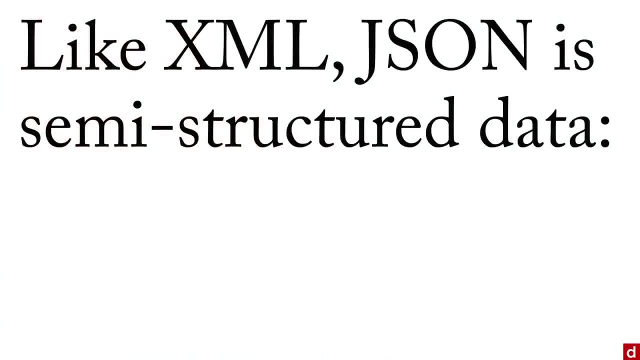 way that you don't want to be able to do. And if you want to be able to do things in a different way, you can do it in a different way. But what XML stands for is that, like XML, JSON is semi structured data, That is, you have tags that define the data, So the computer knows what. 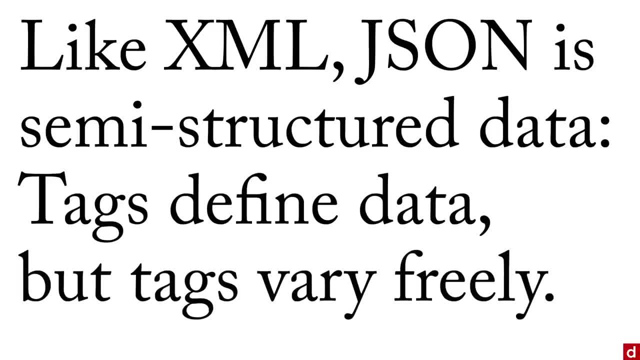 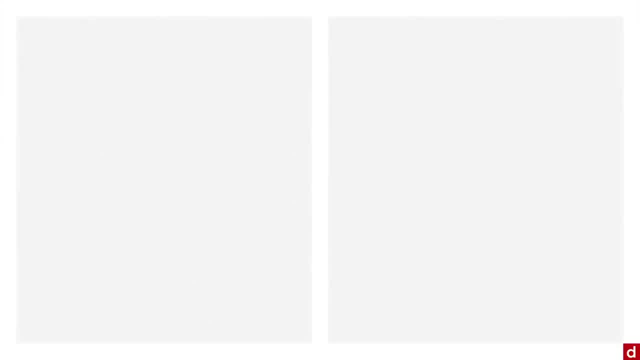 each piece of information is. But like XML, the tags can very freely, And so there's a lot in common between XML and JSON. So XML is a markup language. That's what the ml stands for And that gives meaning to the text that lets the computer know what each piece of information is. Also XML. 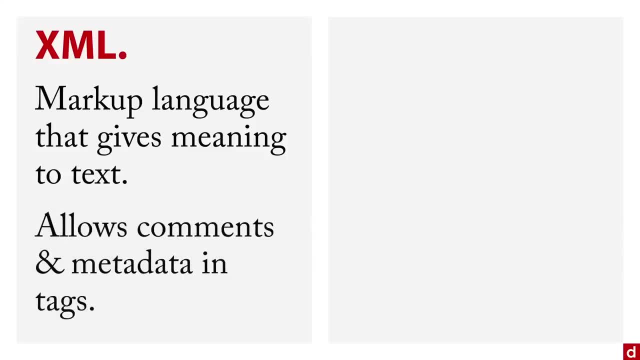 allows you to make comments in the document and it allows you to put metadata in the tags. you can actually put some information there in the angle brackets to provide additional context. JSON, on the other hand, is specifically designed for data interchange And so it's got that special focus And the structure. JSON corresponds with data. 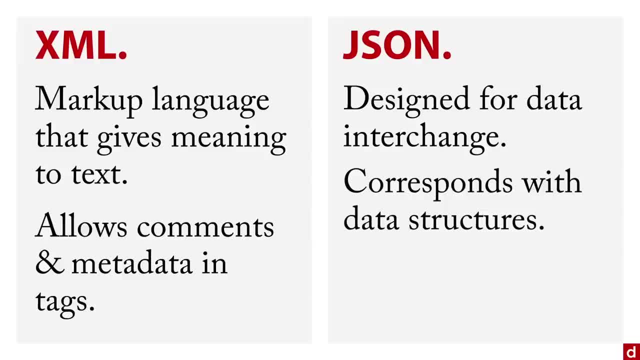 structures. you know, it directly represents objects and arrays and numbers and strings and booleans, And that works really well with the programs that use to analyze data. Also, JSON is typically shorter than XML because it does not require the closing tags. Now there are ways. 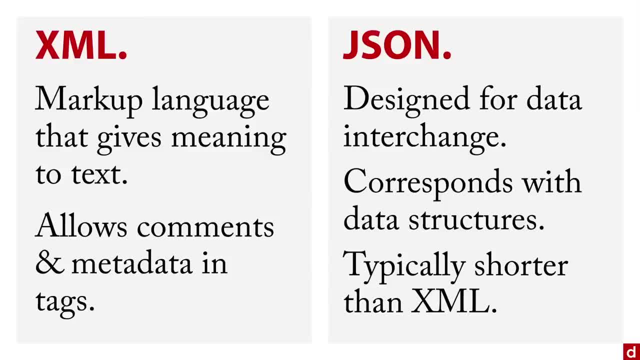 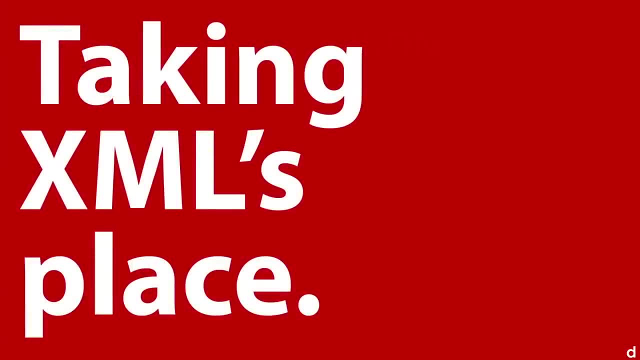 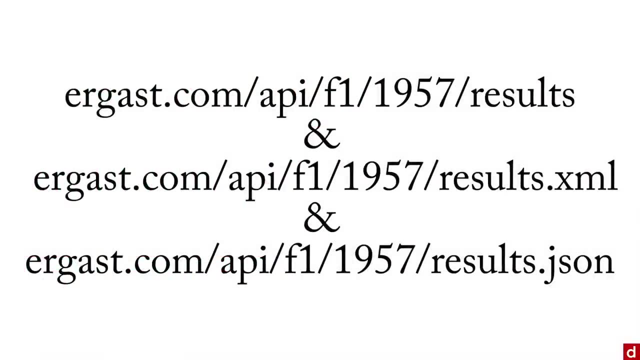 to do that with XML, But that's not typically how it's done. As a result of these differences, JSON is basically taking XML s place in web data. XML still exists, still used for a lot of things, But JSON is slowly replacing it, And we'll take a look at the comparison between the three by going back. 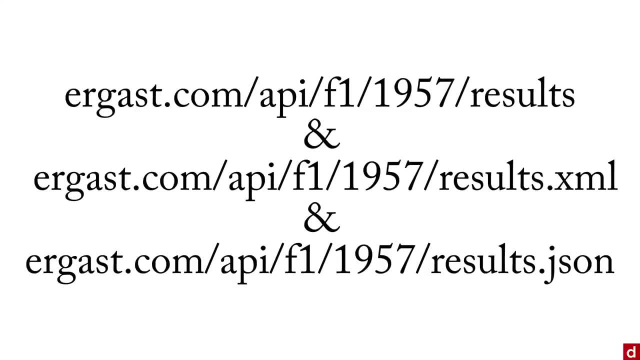 to the example we used in XML. This is data about four, five, six, seven, eight, nine, ten, eleven, 12, 12,, 12,, 12, 12, 12.. So we're going back to the first page here and we're going to add a new. 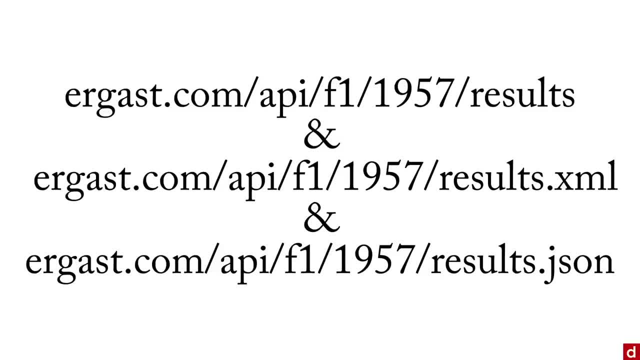 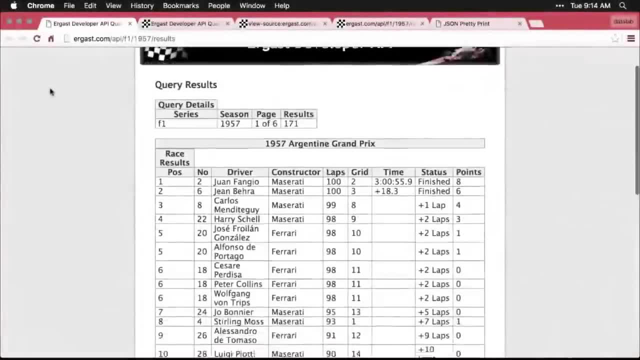 file here called the formula one car races in 1957, from airgascom, And so you can just go to the first web page here and then we'll navigate to the others from that. So this is the general page. this is, if you just type in, without the dot XML or dot JSON or anything, So it's a table of. 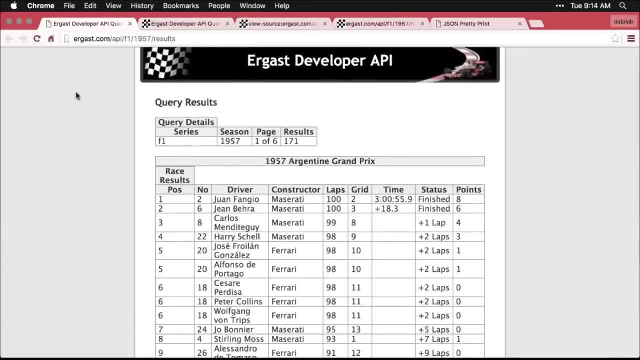 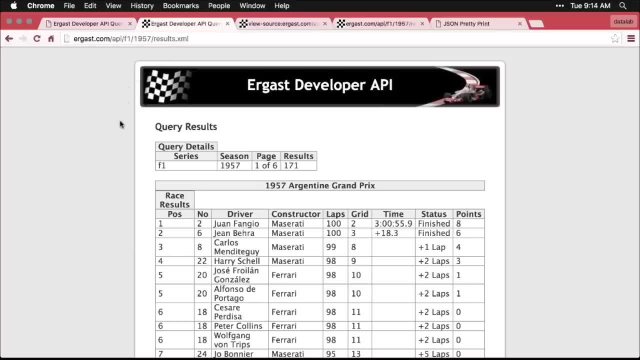 information about races in 1957.. And we saw earlier that if you add just dot XML to the end of this, it looks exactly the same. That's because this browser- the browser that I'm using- is going to have a lot of functions in there. So it's going to have a lot of functions in there And it's going. 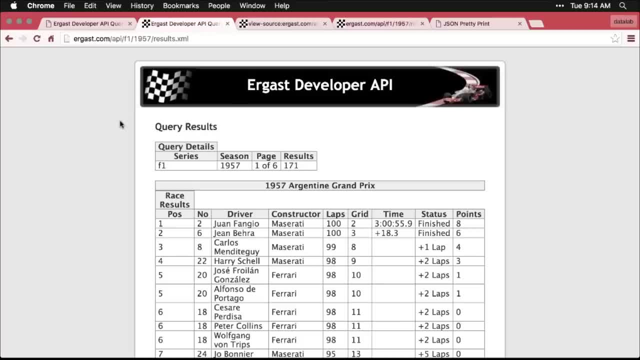 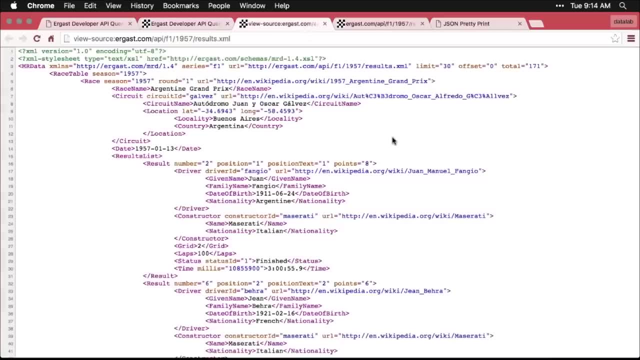 to have a lot of functions in there. So it's going to have a lot of functions in there, But if you were to right click on it and go to view page source, you would get this instead And you can see the structure. this is still XML, And so everything has an opening tag and a closing tag. 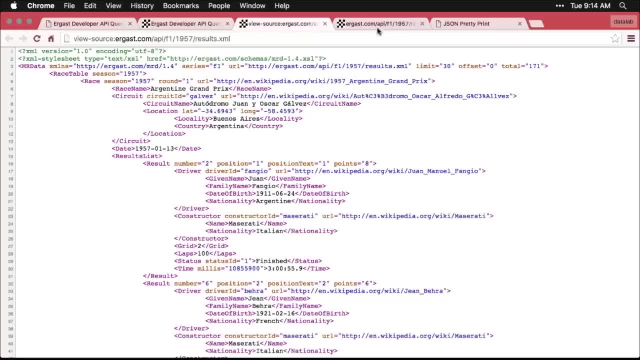 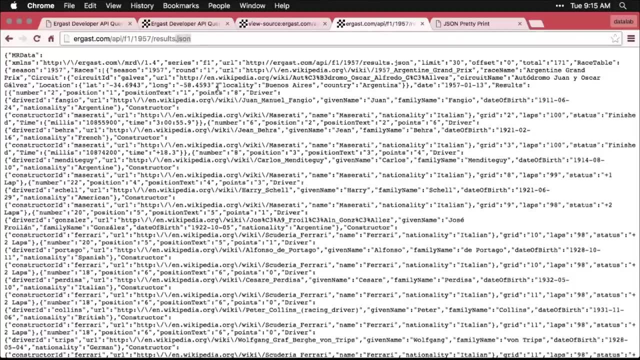 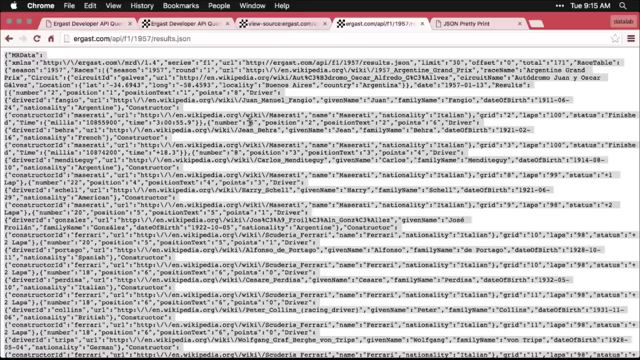 and some extra information in there. But if you type in dot JSON, what you really get is this jumbled mess. Now, that's unfortunate, because there is a lot of structure to this. So what I am going to do is I'm actually going to copy all of this data. Then I'm going to go to a little. 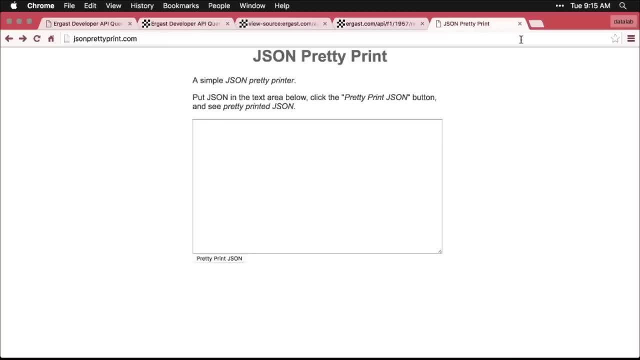 web page. there's a lot of things you can do here, And it's a cute phrase. it's called JSON pretty print And that is make it look structured So it's easier to read. I just paste that in there. 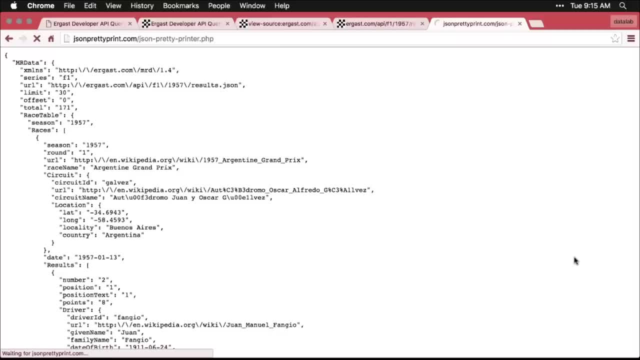 and hit pretty, print JSON, And now you can see the hierarchical structure of the data. The interesting thing is that the JSON tags only have tags at the end of the page And that's at the beginning. So it says series in quotes and then a colon, And then it gives the piece of 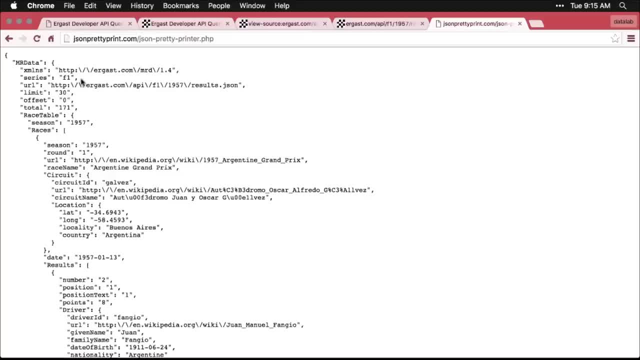 information in quotes and a comma and it moves on to the next one, And this is a lot more similar to the way that data would be represented in something like R or Python, And so it's also more compact. Again, there's things you can do with XML, But this is one of the reasons that 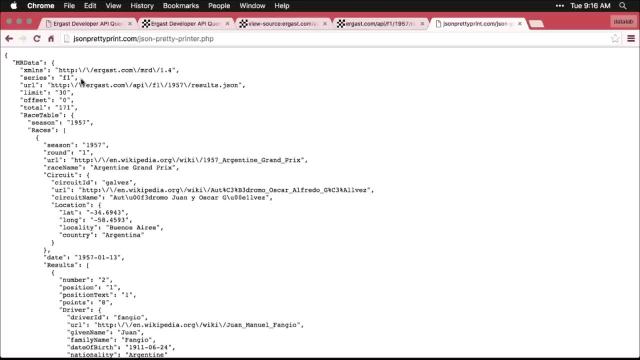 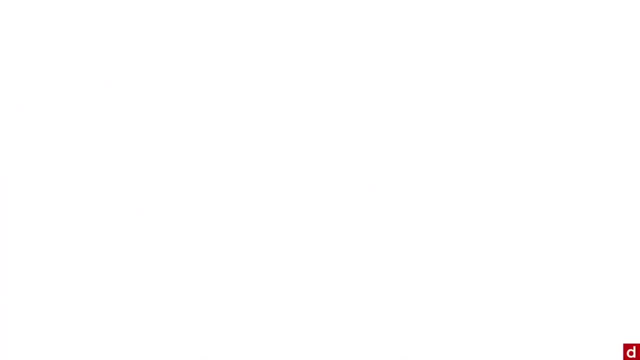 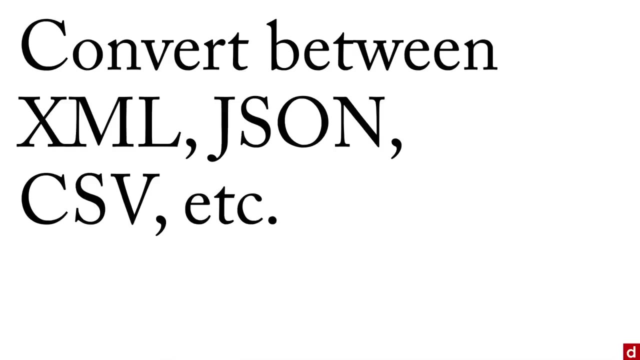 JSON is generally becoming preferred as a data carrier for websites And, as you might have guessed, it's really easy to convert between the formats. It's easy to convert between XML, JSON, CSV, etc. And so you can get a web page where you just paste one version in and you get. 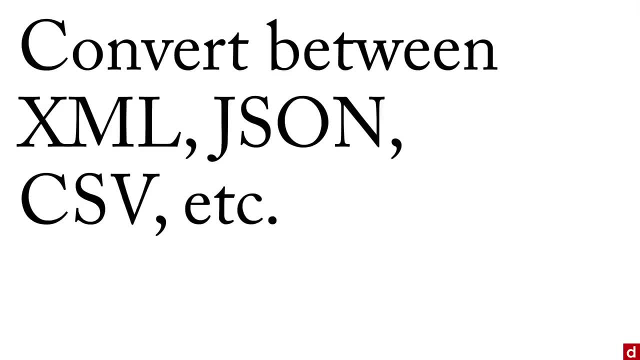 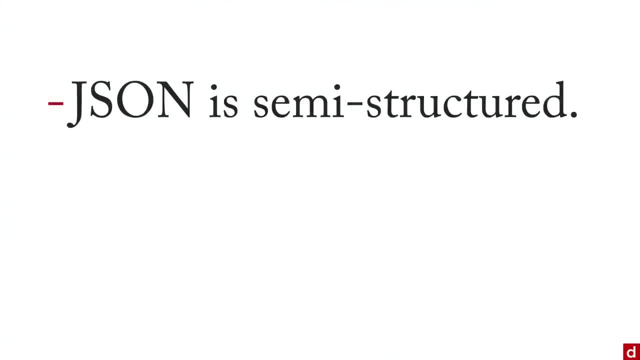 the other version out. There are some differences, but for the vast majority of situations they're just kind of interchangeable. So, in sum, what do we get from this? Like XML, JSON is semi structured data where there are tags that say what the information is. but you can. 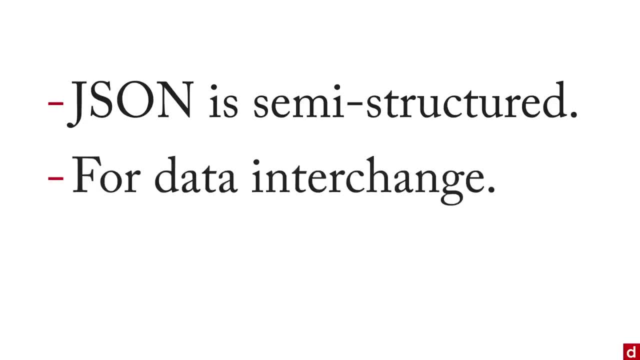 take whatever you want, And JSON is specifically designed for data interchange And because it reflects the structure of the data in the programs, that makes it really easy, And then also because it's relatively compact. JSON is replacing gradually XML on the web as a container for data. 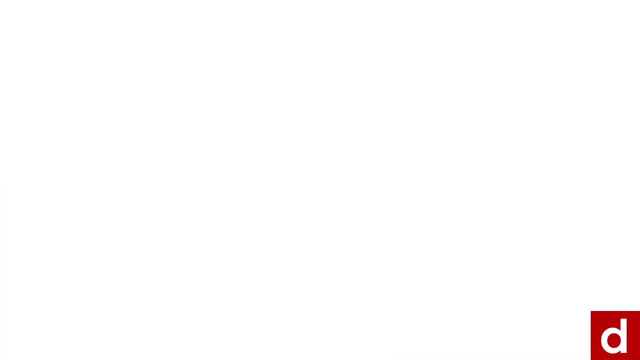 on web pages. If we're going to talk about coding and data science and the languages that are used, then first and foremost is our. the reason for that is, according to many standards are, is the language of data and data science. For example, take a look at this chart. This is a ranking based on a survey of data mining experts. 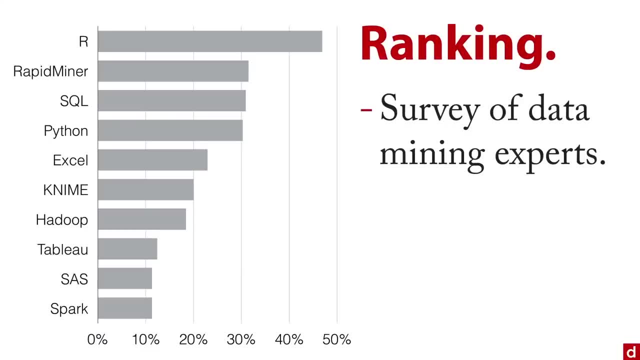 of the software that they use in doing their work, And R is right there at the top. R is first And in fact that's important, because there's Python, which is usually taken hand in hand with our for data science. But our sees 50% more use than Python And that's because we use the class root. 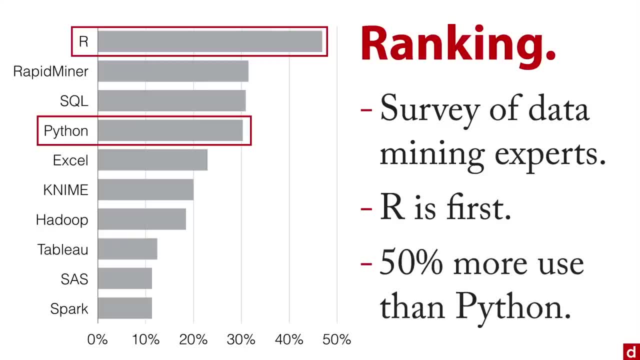 for that function because I think when you look at the class root then you automatically get a version And you can call it a code title. and if you look at the class root and when you look at the class root, Python does, at least in this particular list. Now there's a few reasons for that popularity. 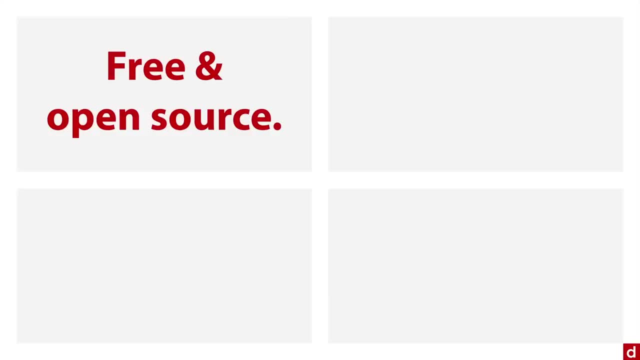 Number one: R is free and it's open source, both of which make things very easy. Second, R is specially developed for vector operations. That means it's able to go through an entire list of data without having to write for loops to go through. If you've ever had to write. 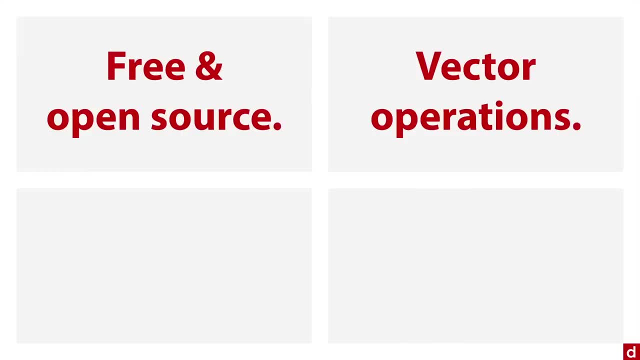 for loops. you know that that would be kind of disastrous, having to do that with data analysis. Next, R has a fabulous community behind it. it's very easy to get help on things with R. you Google it. you're going to end up in a place where you're going to be able. 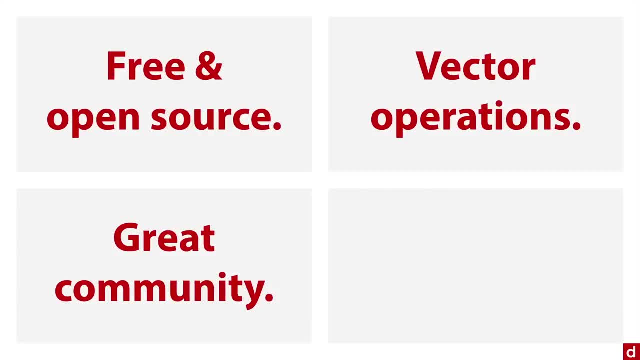 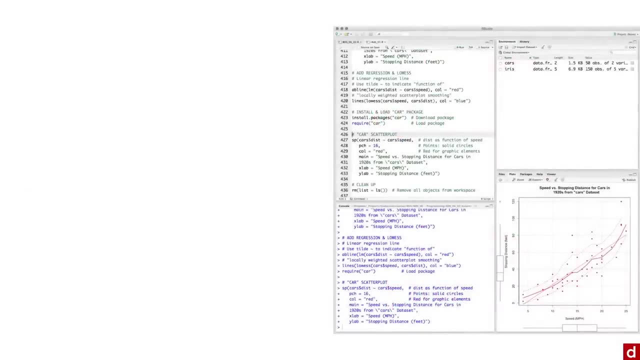 to find good examples of what you need And, probably most importantly, are very capable on its own, But there are 7000 packages- actually as many more than that- 7000 packages- that add capabilities to R. Essentially, it can do anything Now when you're working with 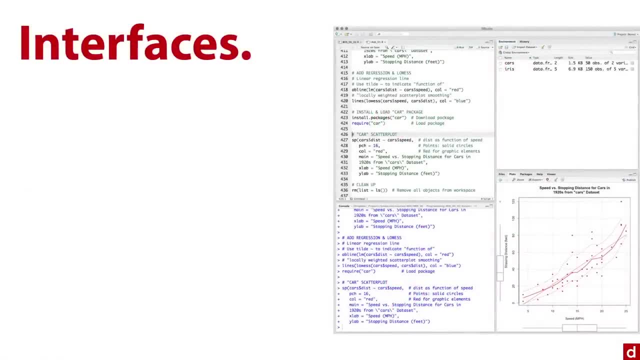 R, you actually have a choice of interfaces. that is, how do you actually do the coding and how do you get your results. R comes with its own IDE or Interactive Developmental Development environment. You can do that, Or, if you're on a Mac or Linux, you can actually. 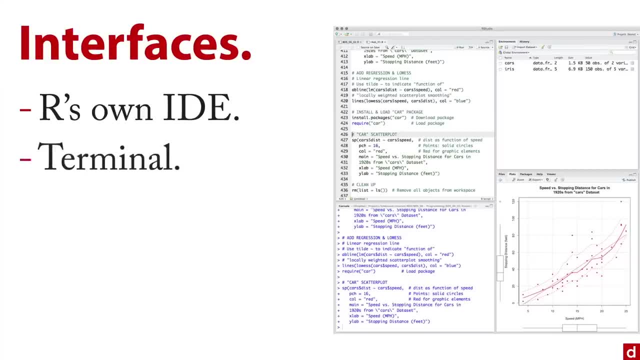 do R through the terminal, through a command line. If you've installed R, you just type R and it starts up. There's also a very popular development environment called RStudio, And that's actually the one that I use And I'll be using for all my examples, But another 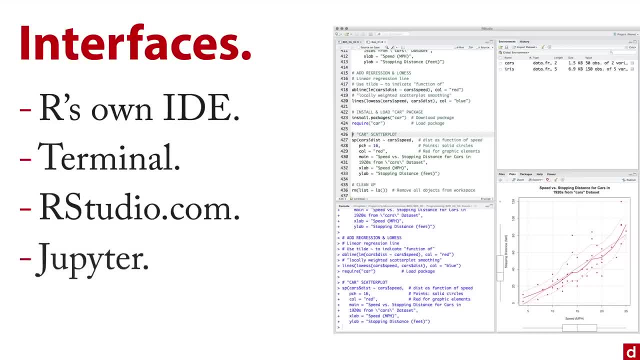 new competitor is Jupyter, which very commonly used, for Python is what I use for examples. there It works in a browser window, even though it's locally installed- And RStudio and Jupyter. there's pluses and minuses to each one of them. I'll mention them as we 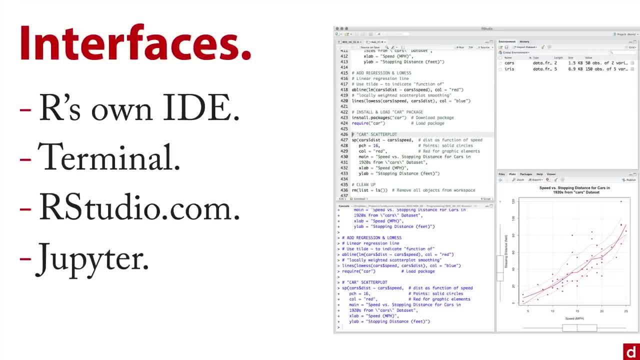 get to them. But no matter what interface you use R command line, you are typing lines of code in order to get the commands. Some people get really scared about that, But really there are some advantages to that in terms of the replicability and really the accessibility. 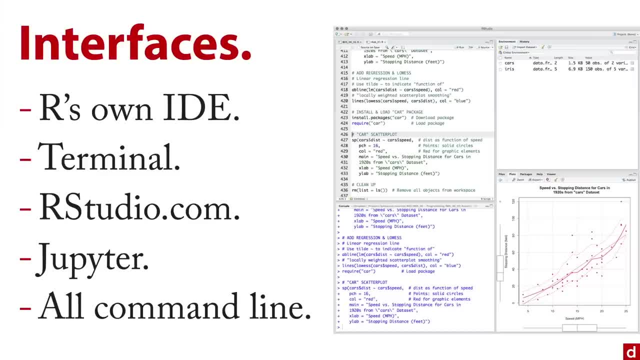 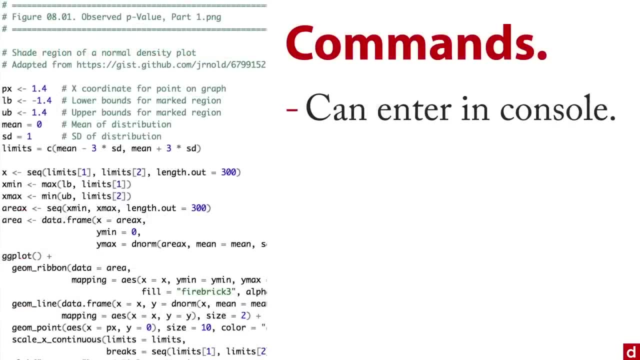 the transparency of your commands. So, for instance, here's a short example of some commands in R. you can enter them into what's called the console, And that's just like one line at a time. that's called an interactive way. Or you can save: 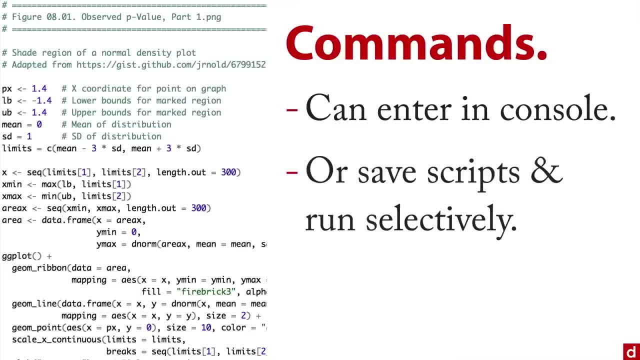 scripts and run bits and pieces of them selectively. that makes your life a lot easier, No matter how you do it. if you're familiar with programming in other languages, then you're gonna find that ours a little weird. it has an idiosyncratic model. It makes sense once you get used to. 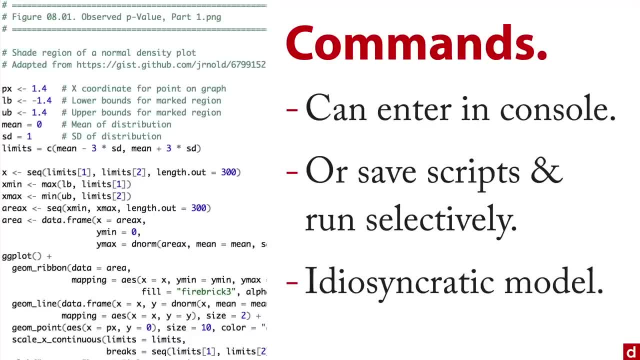 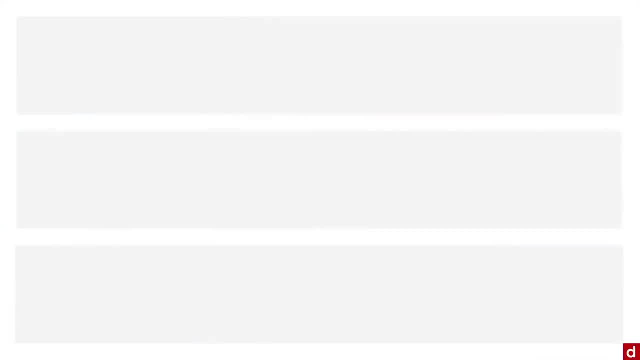 it, But it is a different approach, And so it does take some adaptation. if you're accustomed to programming in other languages. Now, once you do your programming, get your output. what you're going to get is graphs in a separate window. you're going. 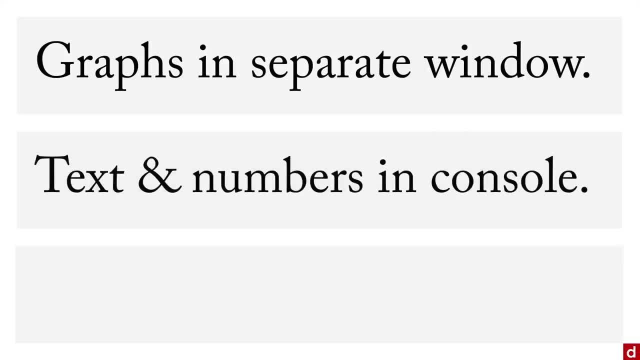 to get text in numbers, numerical output in the console. And no matter what you get, you can save the output to files, So that makes it portable. you can do it in other environments. But most importantly, I like to think of this: here's our box of chocolates where you never 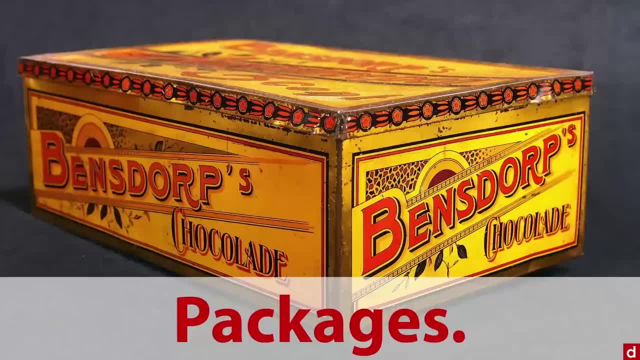 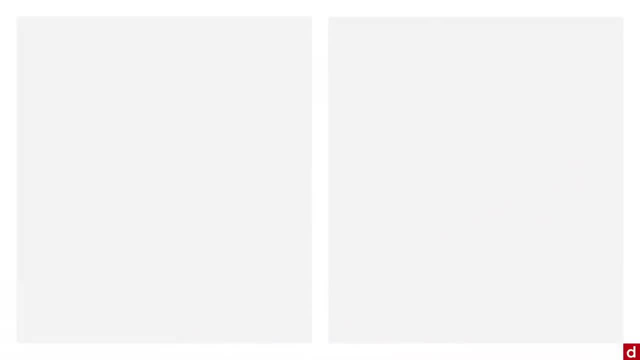 know what you're going to get. The beauty of R is in the packages that are available to expand its capabilities. Now there are two sources of packages that you can use to expand R. One goes by the name of CRAN, and that stands for the Comprehensive R Archive. 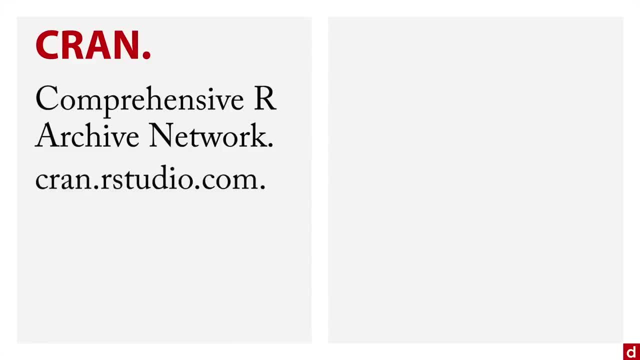 Network And that's at cranrstudiocom. And what that does is it takes the 7000 or so different packages that are available and it organizes them in topics that they call task views And for each one, if they've done their homework, you have data sets that come. 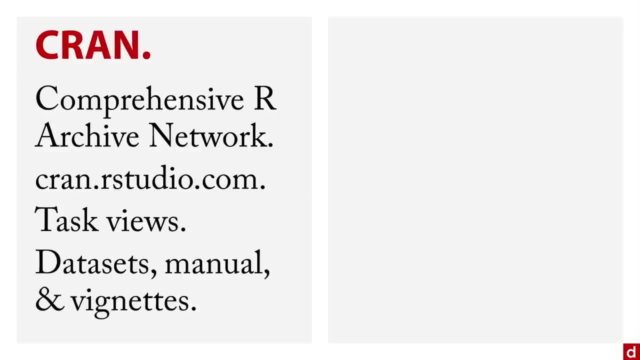 along with that package you have a manual in PDF format And you can even have vignettes where they run through examples of how to do it. Another interface is called CRANtastic, And the exclamation point is part of the title. That's at CRANtasticorg, And what this is is an alternative interface. 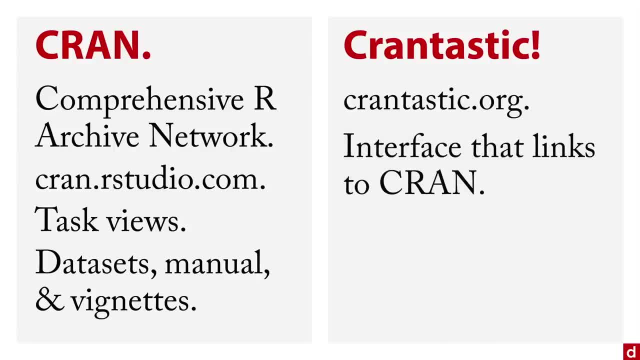 that links to CRAN. So if you find something like in CRANtastic and you click on the link, it's going to open in CRAN. But the nice thing about CRANtastic is it shows the popularity of packages And it also shows how recently they were updated And that can be a nice. 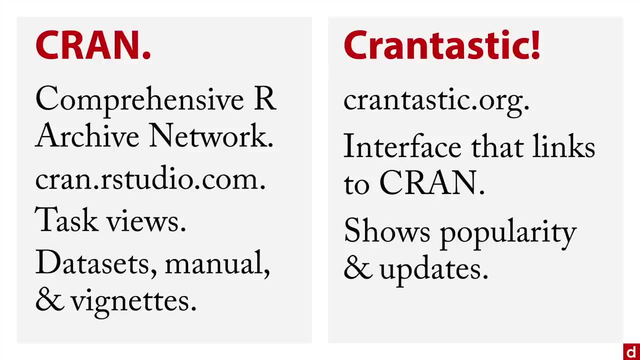 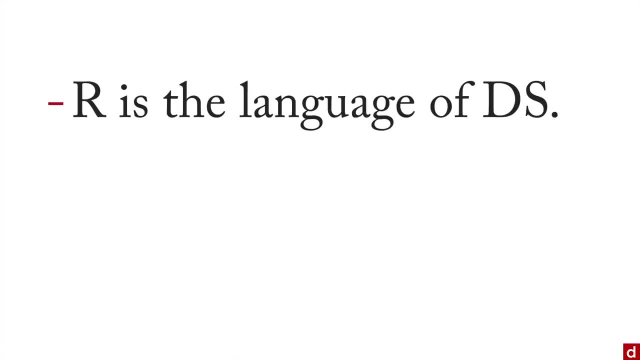 way of knowing that you're getting sort of the latest and greatest. Now, from this very abstract presentation, we can say a few things about R Number one. according to many, R is the language of data science And it's a command line interface. 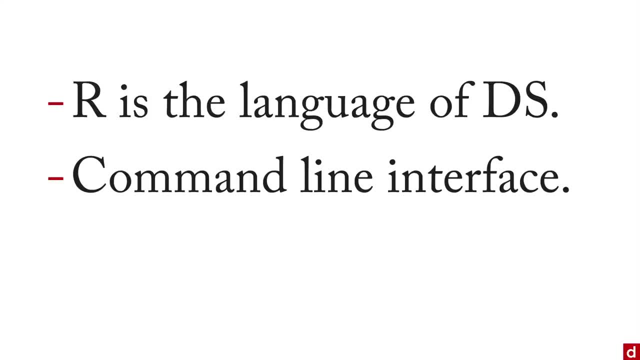 you're typing lines of code, So that gives it both a strength and a challenge for some people. But the beautiful thing is the 1000s and 1000s of packages of additional code and capability that are available for R that make it possible to do nearly anything in this. 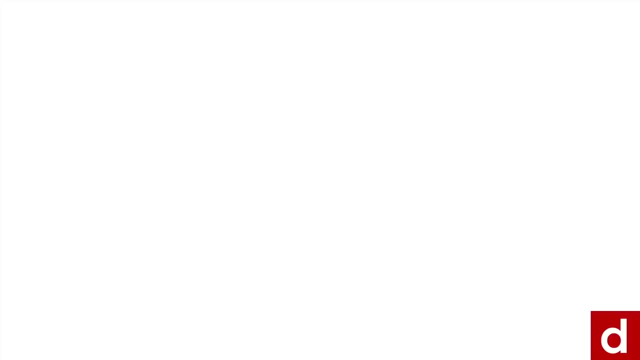 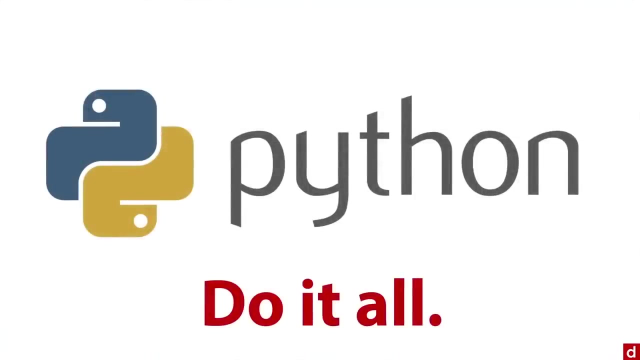 statistical programming language When talking about coding and data science- and the languages along with our- we need to talk about Python. Now, Python the snakes, is a general purpose program that can do it all, And that's its beauty. If we go back to this survey of the software used by data, 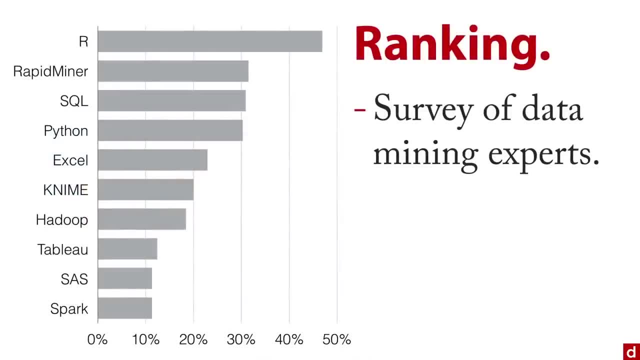 mining experts. you see that Python's there. it's number three on the list, And what's significant about that is: on this list, Python is the only general purpose programming language. It's the only one that can theoretically be used to develop any kind of application that you want. That gives it some special power compared. 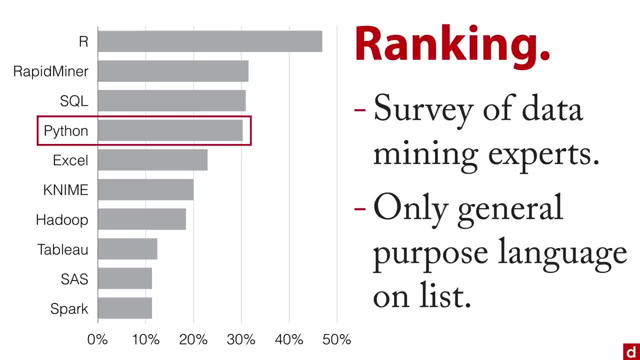 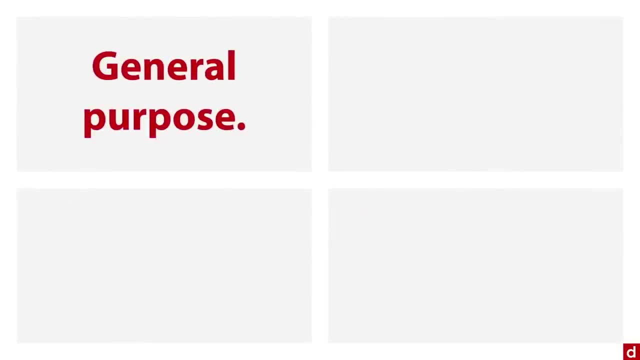 to all these others, most of which are very specific to data science work. So the nice things about Python are number one, its general purpose. It's also really easy to use And if you have a Macintosh or a Linux computer, Python is built into it Also. Python has 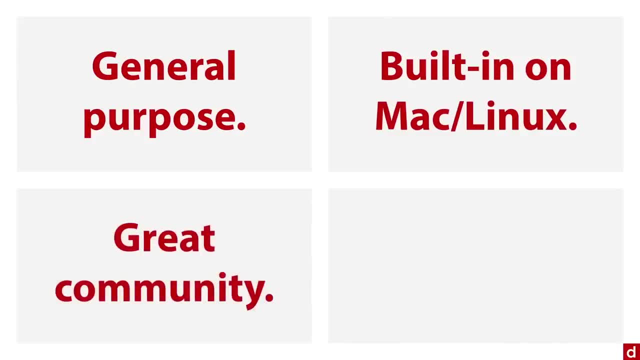 a fabulous community around it with hundreds of thousands of people involved. And also Python has thousands of packages. Now it actually has something like 70 or 80,000 packages, But in terms of ones that are specific to data, there are still thousands available. They give it some. 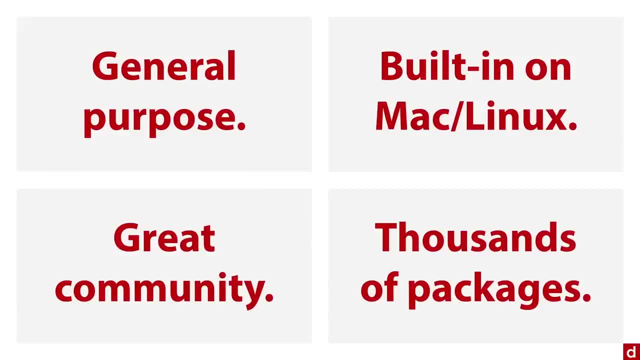 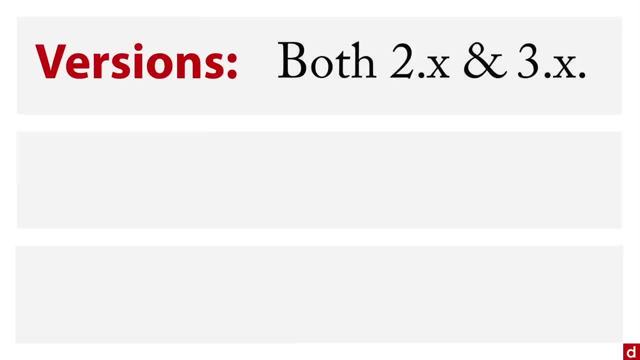 incredible capabilities. Now a couple of things to know about Python. First is about versions. There are two versions of Python that are in wide circulation. There's 2.x, So that means like 2.5, 2.6. And there's 3.x, 3.1, 3.2. Version two and version three are similar, But they're not. 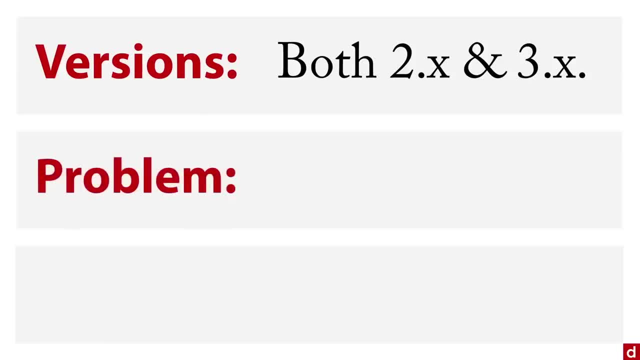 identical, And in fact, the problem is this: There are some compatibility issues where code that runs in one does not run in the other, And consequently most people have to choose between one or the other, And what this leads to is that many people still use. 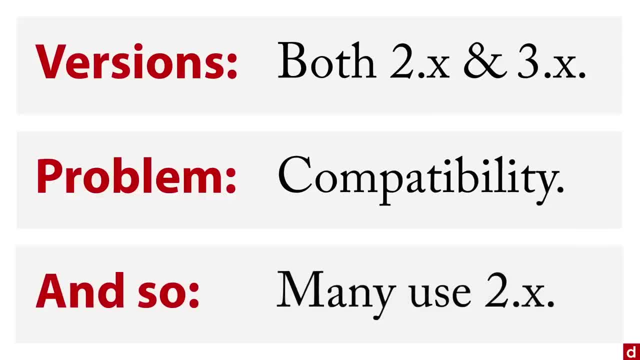 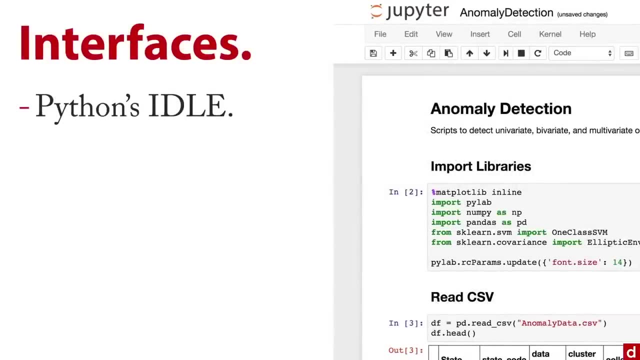 2.x. I have to admit the examples that I use. I'm using 2.x Because so many of the data science packages are developed with that in mind. Now let me say a few things about interfaces for Python. First. Python does come with its own interactive 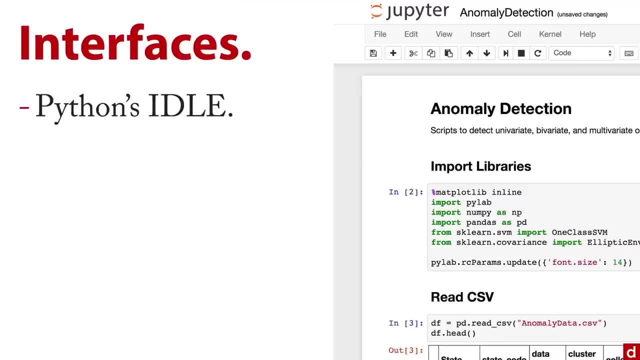 development and learning environment. They call it idle. You can also run it from the terminal or command line interface or any IDE that you have. Now a very common and very good choice is Jupiter. Jupiter is a browser based framework For programming And it was originally called IPython And that served as its initial version. So a lot. 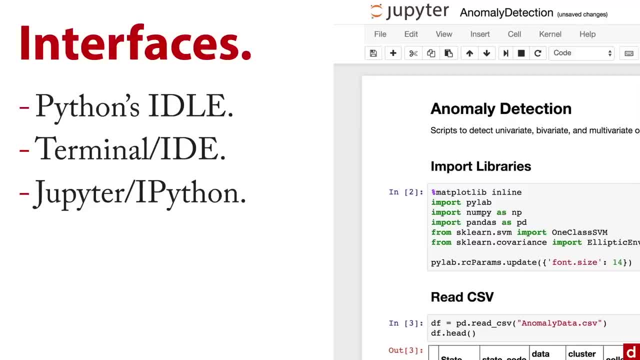 of times, when people talk about IPython, what they're really talking about is Python in Jupyter, And the two are sometimes used interchangeably. One of the neat things you can do is there are two companies there's- Continuum and Nthought, both of which have made special distributions. 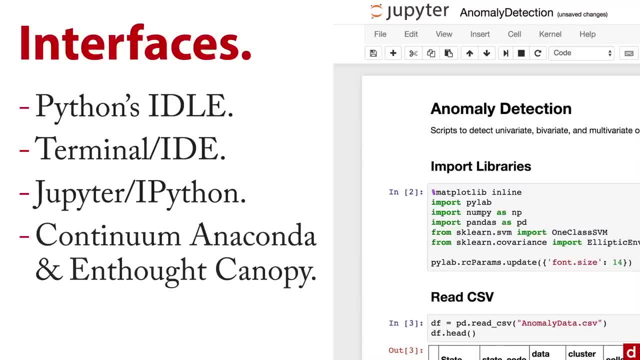 of Python with hundreds and hundreds of packages pre configured to make it very easy to work with data. I personally prefer Continuum. Anaconda is the one that I use. a lot of other people use it, But either one is going to work and it's going to get you up and running And, like I said, with 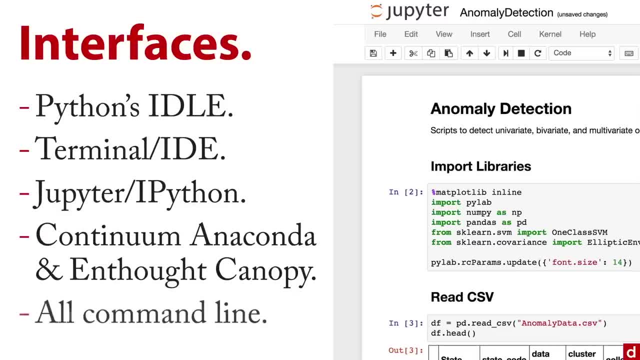 our. no matter what interface you use, all of them are command line. you're typing lines of code. Again, there are some tremendous strengths to that, but it can be intimidating to some people at first. In terms of the actual commands of Python, you have some examples here on the side. 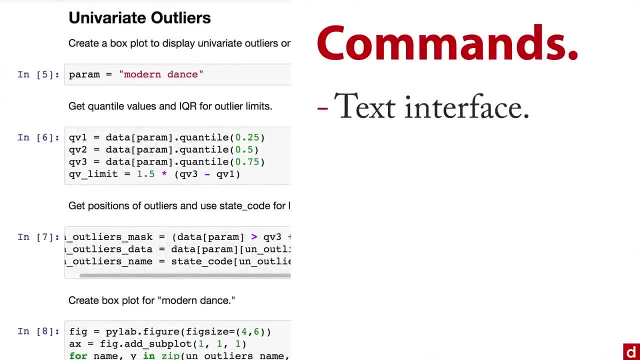 the important thing to remember is that it's a text interface. On the other hand, Python is familiar to millions of coders because it's very often a first programming language that people learn to do general purpose programming, And there are a lot of very simple 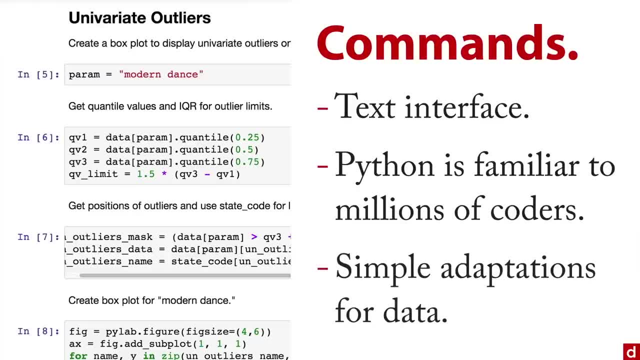 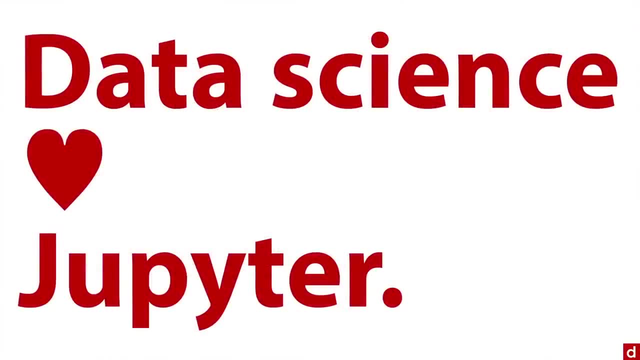 adaptations for data that make it very powerful for data science work. So let me say something else Again: data science loves Jupyter, And Jupyter is the browser based framework. it's a local installation, but you access it through a web browser that makes it possible. 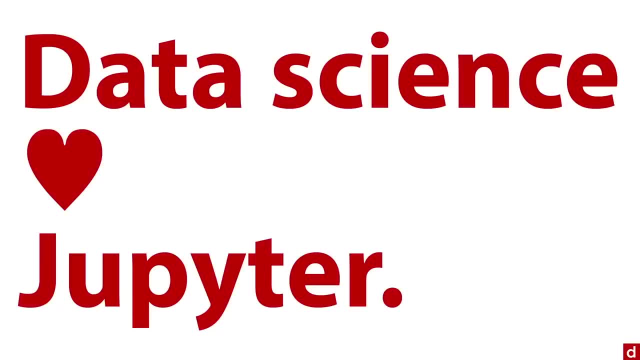 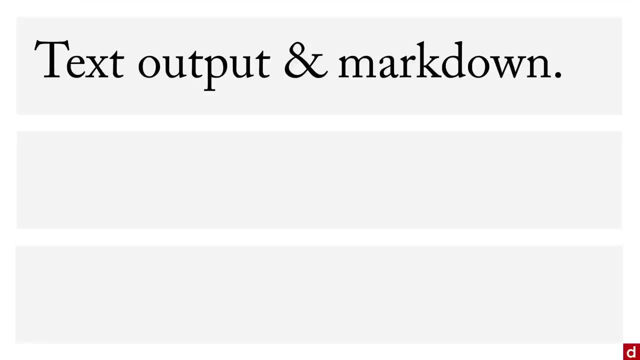 to really do some excellent work in data science. There's a few reasons for this. When you're working in Jupyter, you get text output and you can use what's called markdown as a way of formatting documents. You can get inline graphics or the graphics to show up directly beneath the code. 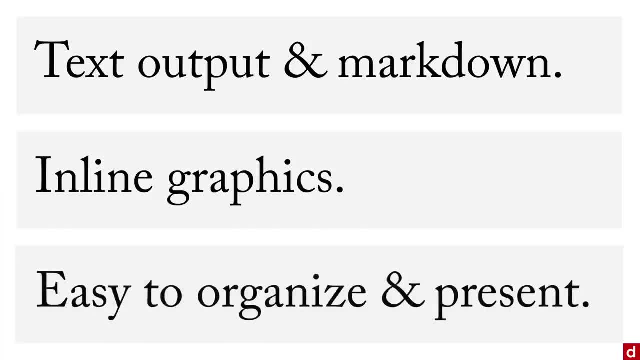 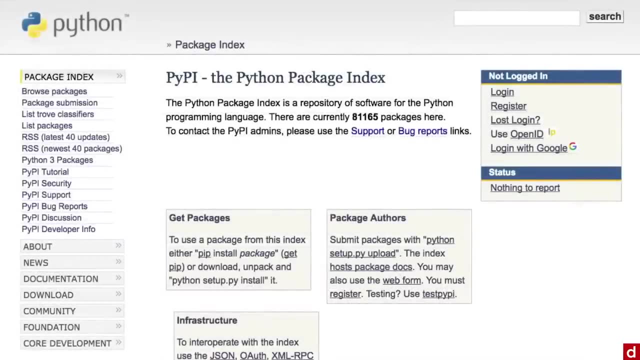 that you did it. Also, it's really easy to organize and present and to share analyses that are done in Jupyter, which makes it a strong contender for your choices in how you do data science programming. Another one of the beautiful things about Python, like R, is that there are thousands. 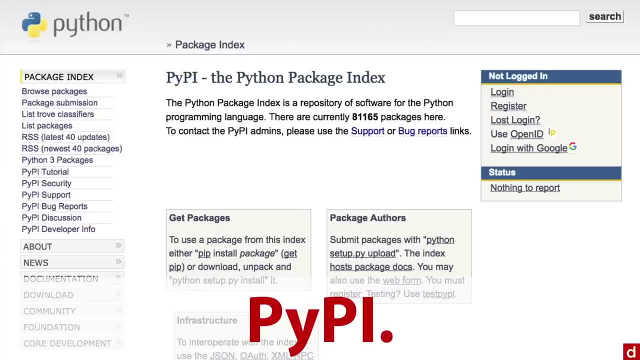 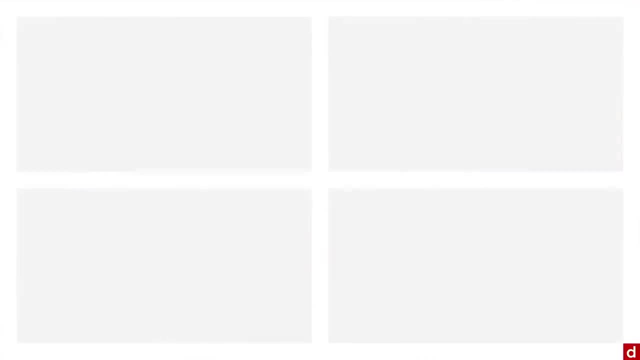 of packages available In Python. there's one main repository- it goes by the name pi pi- which is for the Python package index. Right here it says there's over 80,000 packages, and seven or 8000 of those are for data specific purposes. Now some of the packages that you'll 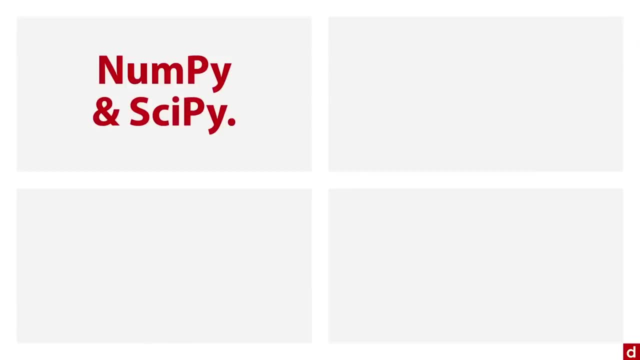 get to be very familiar with are numpy and scipy, which are for scientific computing in general. matplotlib and a development of it called Seaborn are for data visualization and graphics. pandas is the main package for doing statistical analysis And for machine learning almost. 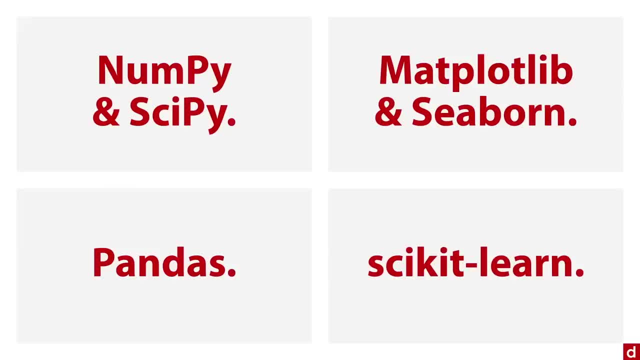 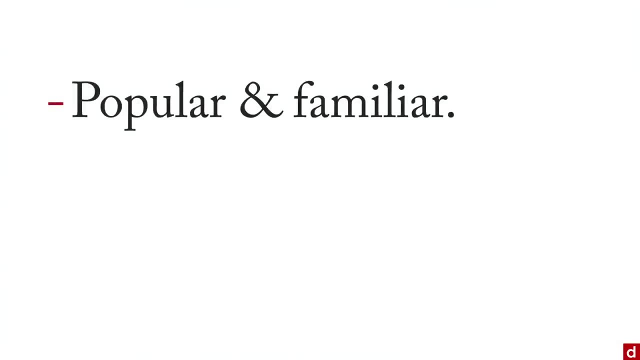 nothing beats scikit learn, And when I go through hands on examples in Python, I will be using all of these as a way of demonstrating the power of the program for working with data. So, in sum, we can say a few things. Number one, Python, is a very popular program familiar to millions of people, And that makes 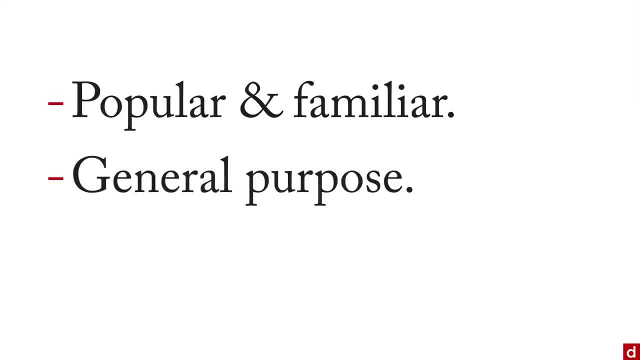 it a good choice. Second, of all, the languages we use for data science on a frequent basis. this is the only one that's general purpose, which means it can be used for a lot of things other than processing data, And it gets its power, like R does, from having thousands of. 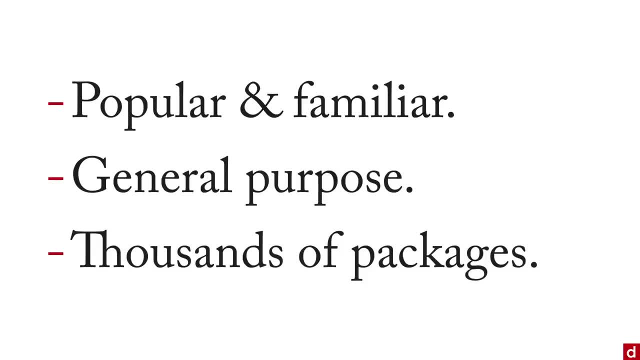 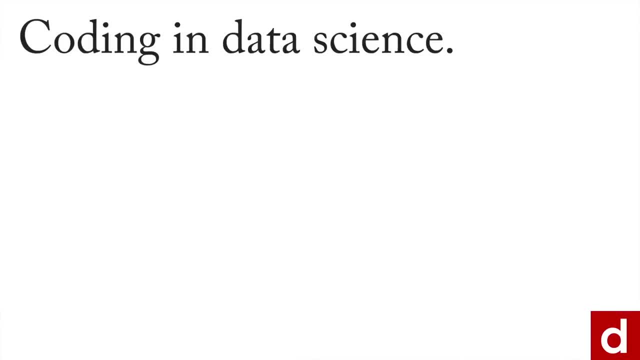 contributed packages which greatly expand its capabilities, especially in terms of doing data science work. Achieved A choice for coding in data science, one of the languages that may not come immediately to mind when they think data science is SQL or SQL, And SQL is the language of databases. 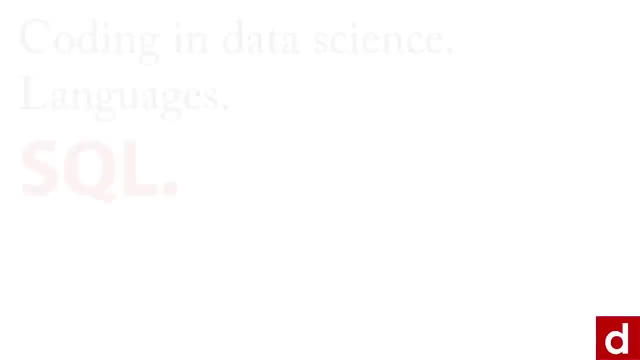 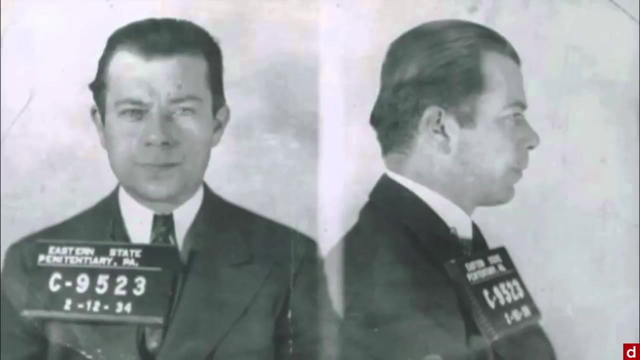 And we think: why do we want to work in SQL? Well, to paraphrase the famous bank robber Willie Sutton, who apparently explained why he robbed banks and said: because that's where the money is. The reason we would work with SQL in data science is because that's where. 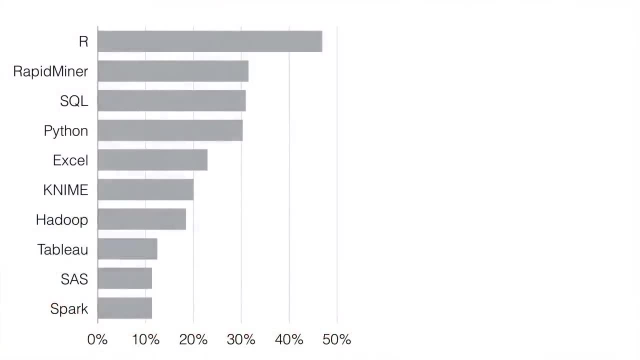 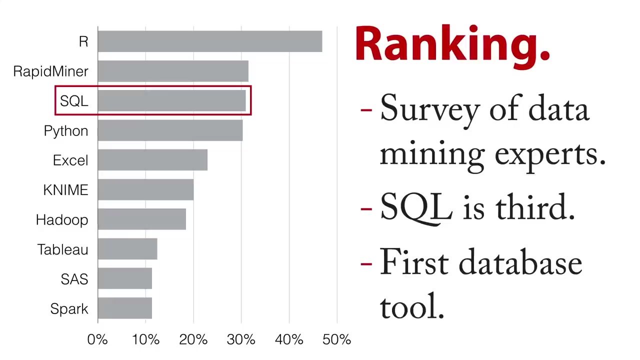 the data is, And so let's take another look at our ranking of software among data mining professionals, And their sequel is third on the list, And also of this list is the first database tool. Other tools in there, for instance, get much fancier and they're much newer, and 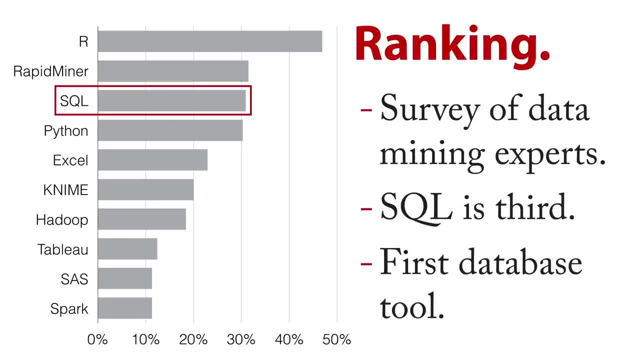 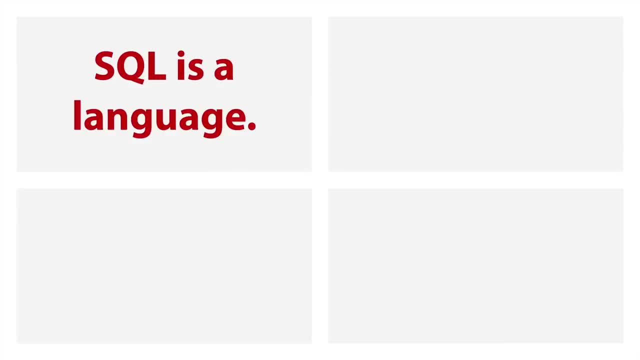 shinier, But SQL has been around for a while, is very, very capable. Now there's a few things to know about SQL. By the way you'll notice, I'm saying SQL even though that stands for something that stands for structure. 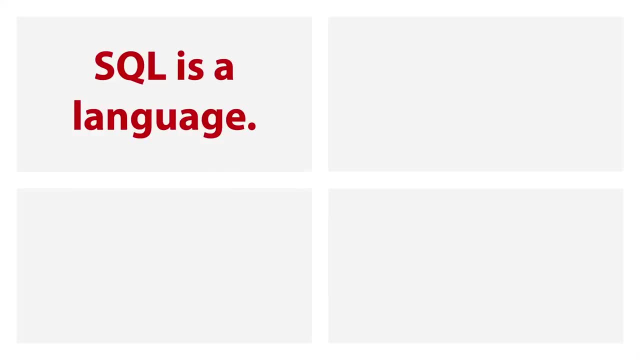 query language. SQL is a language. it's not an application. there's not a program SQL. It's a language that can be used in different applications. Primarily, SQL is designed for what are called relational databases, And those are special ways of storing structured 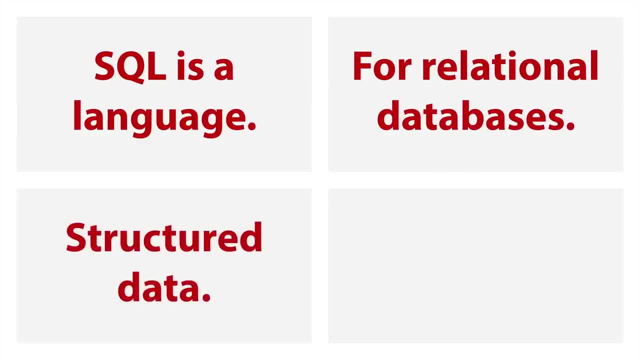 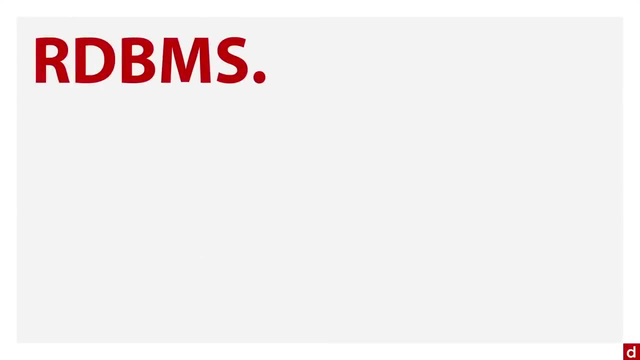 data that you can pull in. you can put things together, you can join them in special ways, you can get some summary statistics, And then what you usually do is you then export that data into your analytical application of choice. So the big word here is RDBMS, And that stands. 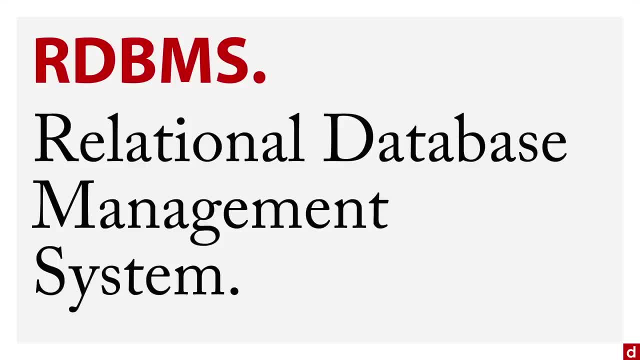 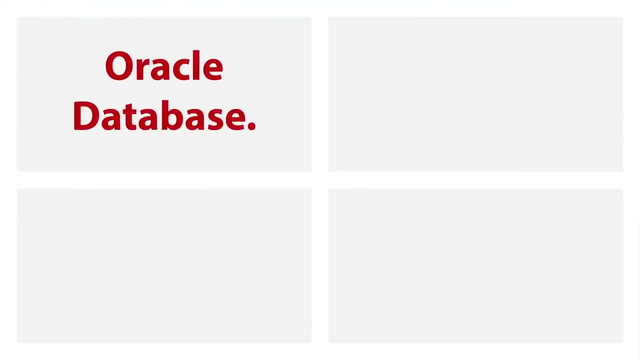 for relational database management system, And that's where you will usually see SQL as a query language being used. In terms of relational database management systems, there are a few very common choices In the industrial world. where people have some money to spend, there's Oracle database. 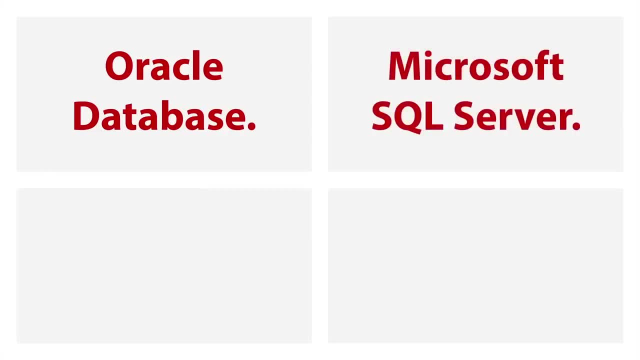 is a very common one, And more commonly there's SQL, And in the industrial world where people have some money to spend, there's Oracle. database is a very common one And more commonly there's Microsoft SQL or SQL Server. In the open source world, two very common choices are: 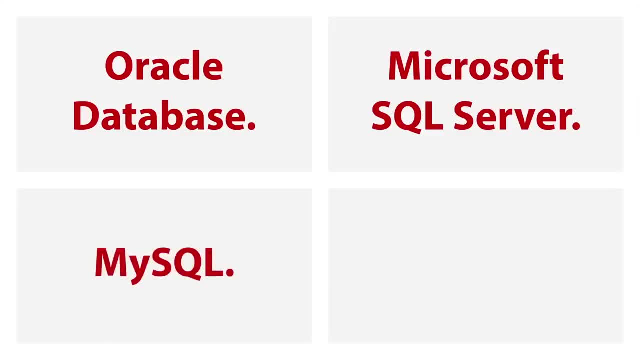 MySQL, Even though we generally say SQL when it's here, you generally say MySQL. And then another one is PostgreSQL. These are both open source, free versions of the language. They're sort of dialects of each that make it possible for you to be working with databases. 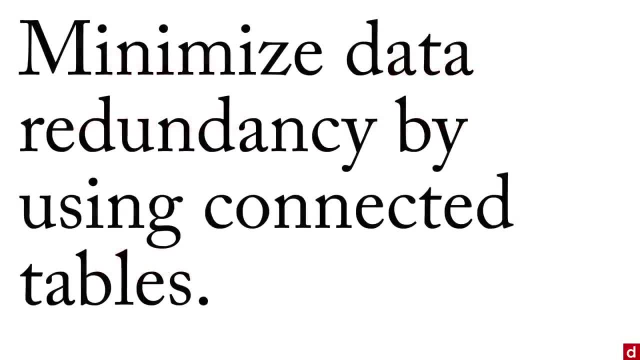 and get your data out. The neat thing about them, no matter what you do, is that databases they work with the machine. Now, scripting is a very common technique And one of the things that I've found that's in a lot of the language that tends to be used on GitHub. 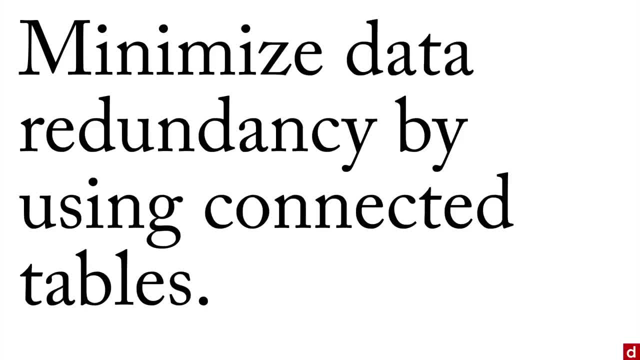 is that you can sort of force-direction and everything. You can use that to make the same work. There's also the classic programmation system, which downichten basically is that you can minimize data redundancy by using connected tables. Each table has rows and columns, and 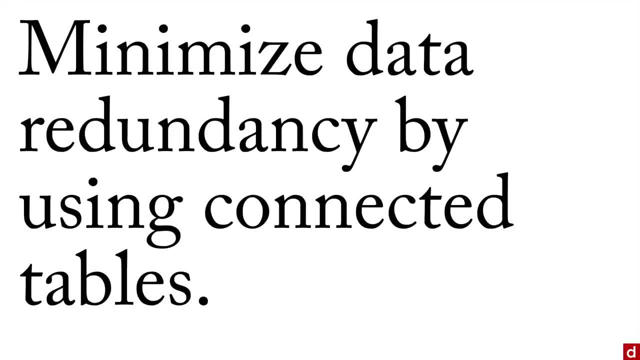 they store different levels of abstraction or measurement, which means you only have to put the information in one place and then it can refer to lots of other tables, makes it very easy to keep things organized and up to date When you're looking at a way of working with a relational database management system. 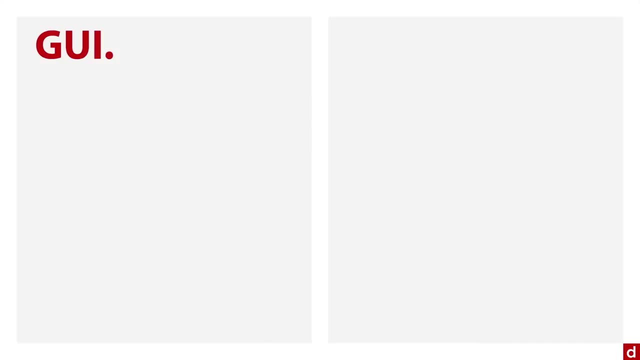 you get to choose in part between using a graphical user interface or GUI, And some. Some of those include SQL Developer and SQL Server Management Studio, two very common choices, And there are a lot of other ones like Toad and some other choices that are graphical. 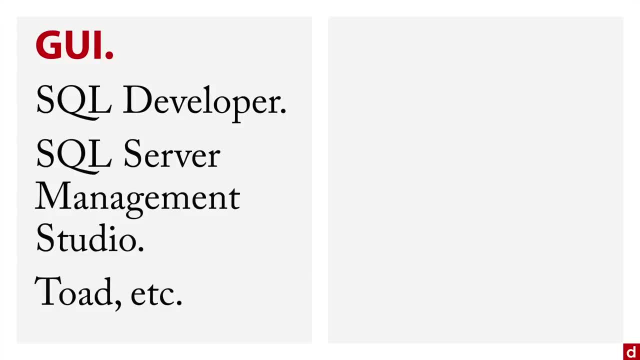 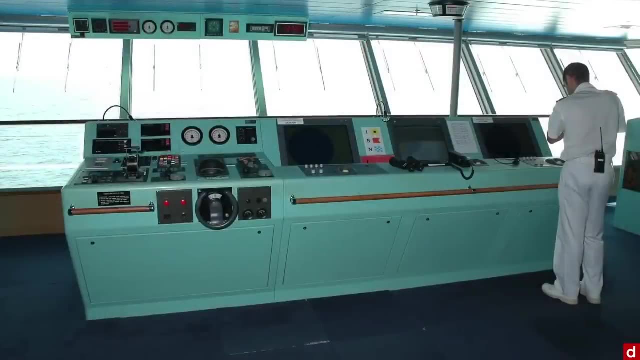 interfaces for working with these databases, And there are also text based interfaces, So really any command line interface and any interactive development environment or programming tool is going to be able to do that. Now you can think of yourself being on the command deck of your ship and learn a few. 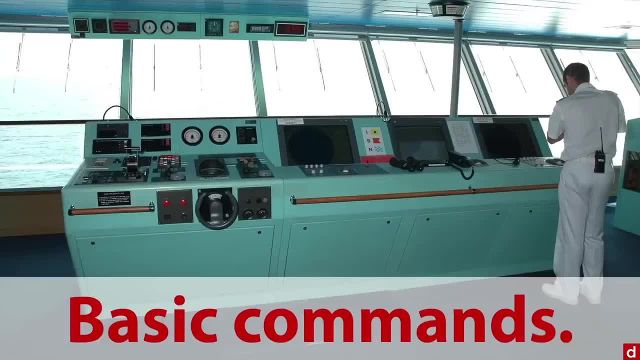 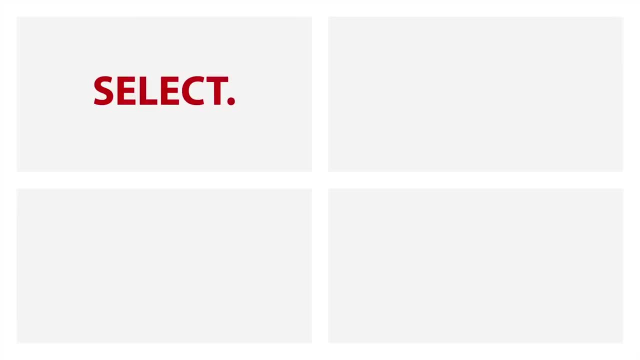 basic commands that are very important for working with SQL. There are just a handful of commands that can get you most of where you need to go. There is the select command, where you're choosing the cases that you want to include From says which tables are you going to be extracting them from. 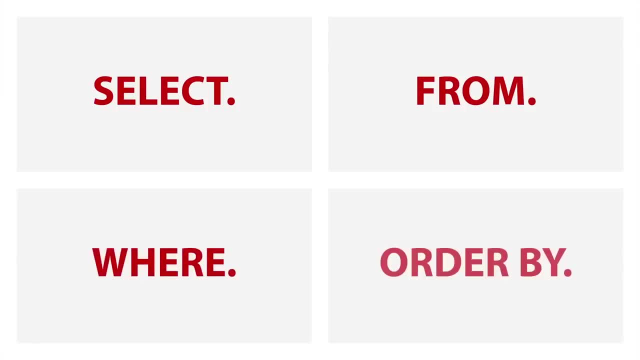 Where is a way of specifying conditions and then order by? Obviously, it's just a way of putting it all together. This works because usually when you're in a SQL database, you're just pulling out the information. you want to select it, you want to organize it. 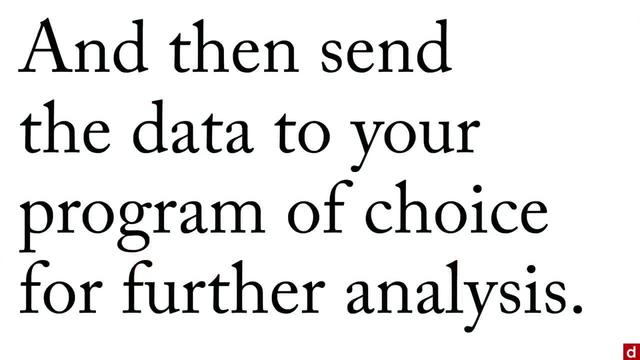 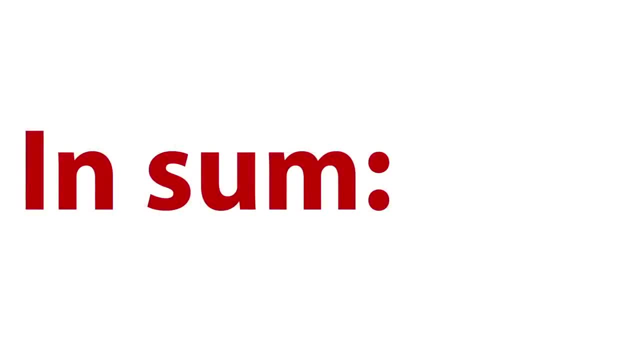 And then what you're going to do is you're going to send the data to your program of choice for further analysis, like our Python or whatever. So, in sum, here's what we can say about SQL Number one as a language. it's generally associated with relational databases, which 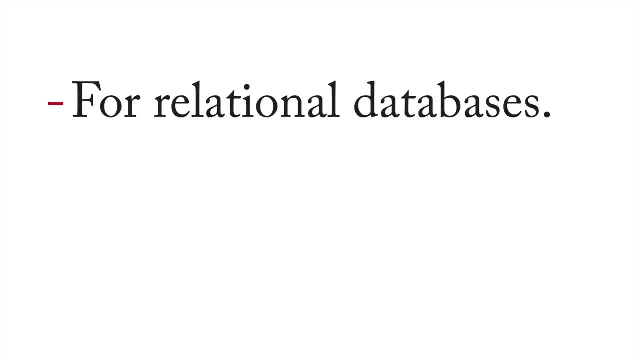 are very efficient And well structured ways of storing data. Just a handful of basic commands can be extremely useful When working with databases. you don't have to be a super ninja expert. Really. a handful 510 commands will probably get you everything you need out of a SQL database. 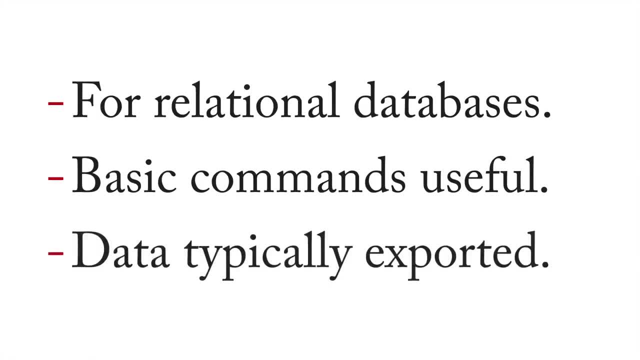 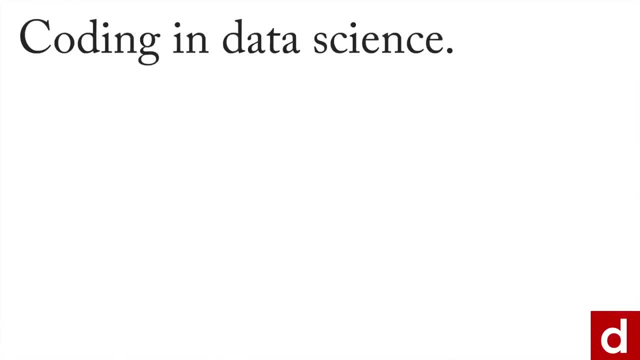 And then, once you get the data organized, it's typically exported to some other program for analysis. When you talk about coding in any field, one of the languages or one of the groups of languages That come up most often are C, C++ and Java. 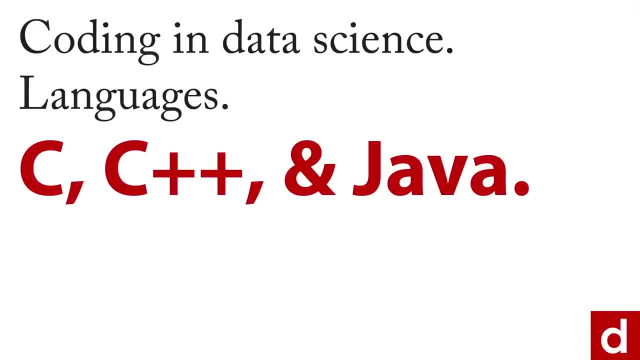 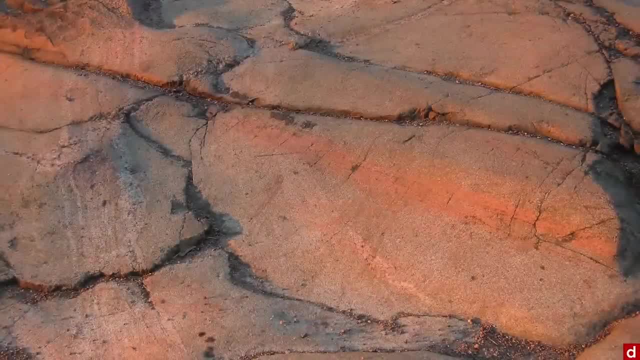 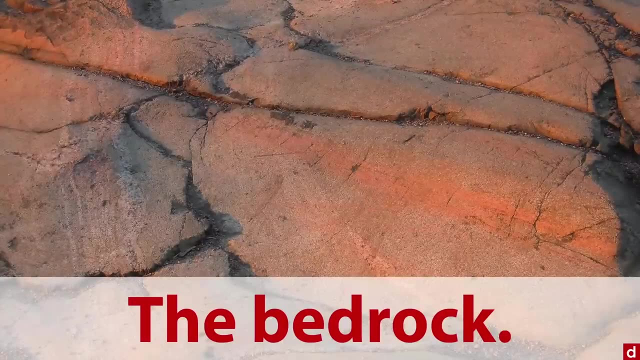 Now these are extremely powerful applications and very frequently used for sort of professional production level coding In data science. the place where you're going to see these languages most often is in the bedrock, the absolute fundamental layer that makes the rest of data science possible. 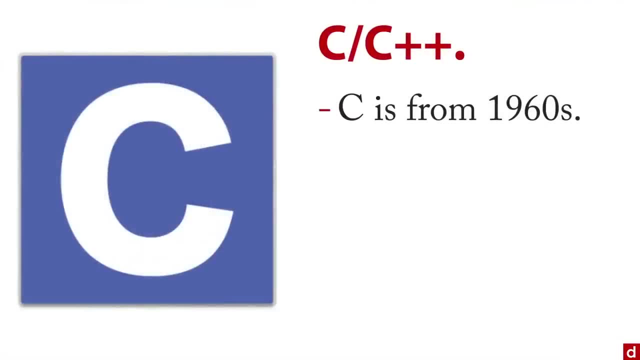 So, for instance, C and C++- C is from the 60s, C++ is from the 80s- And they have a lot of different languages And they have extraordinarily wide usage. Their major advantage is that they're really really fast. 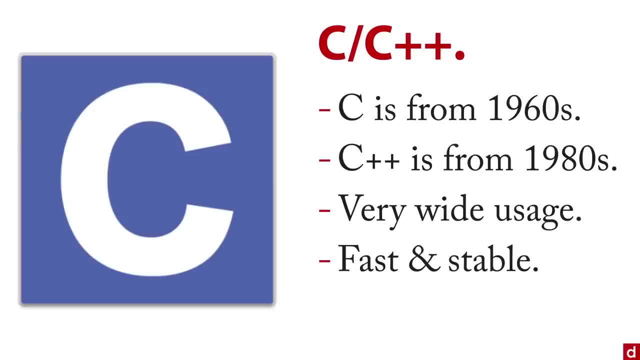 In fact, C is usually used as the benchmark for how fast is a language. They're also very, very stable, which makes them really well suited to production level code and, for instance, server use. What's really neat is that, in certain situations, if time is really important, if speed is important, 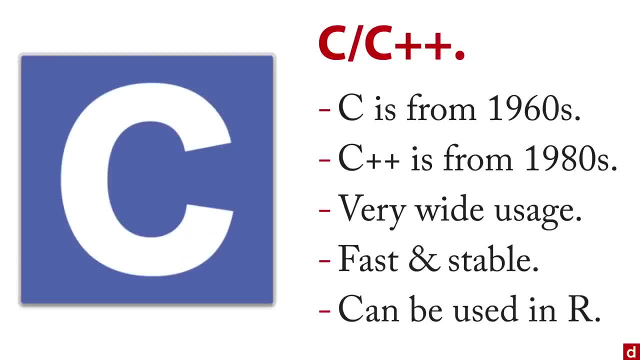 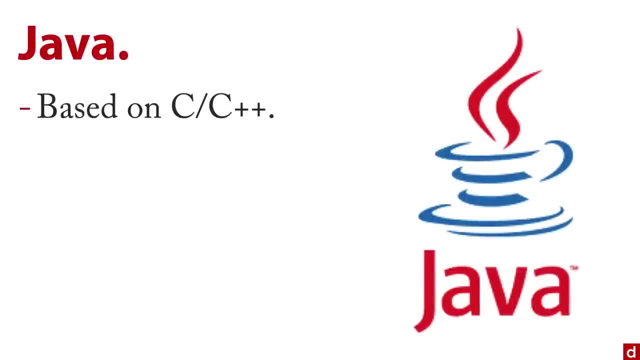 then you can actually use C code in R or other statistical languages. Next is Java. Java is based on C++. Its major contribution was the war, or write once run anywhere- the idea that you're going to be able to develop code that is portable to different machines and different environments. 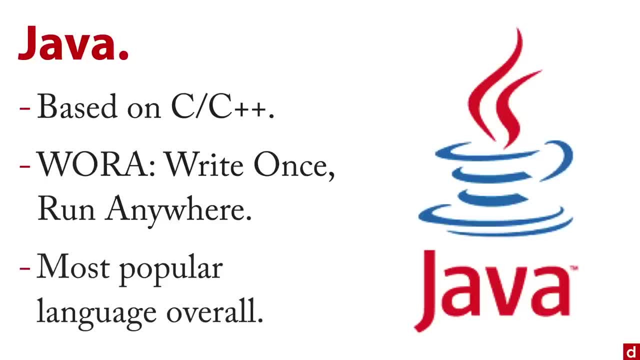 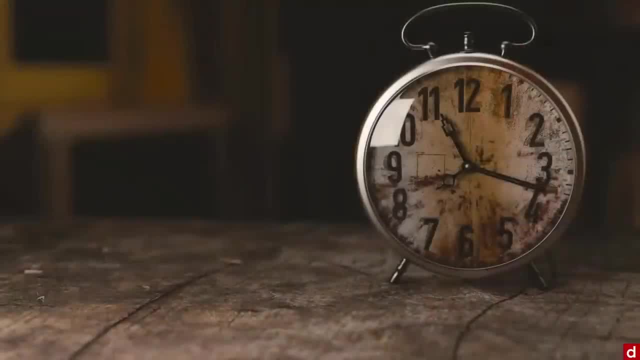 And because of that, Java is actually the most popular computer programming language overall, against all tech situations. And the place where you would use these in data science is, like I said, when time is really important, And that's where you're going to be able to develop code that is portable to different. 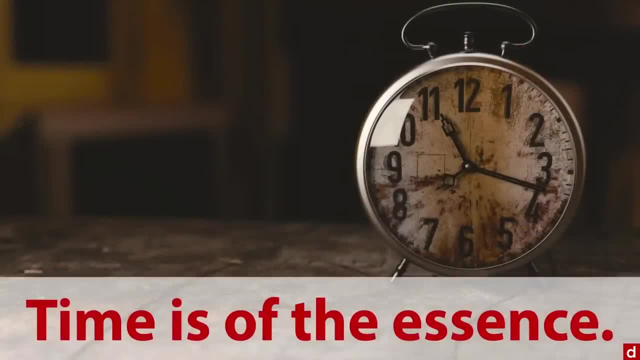 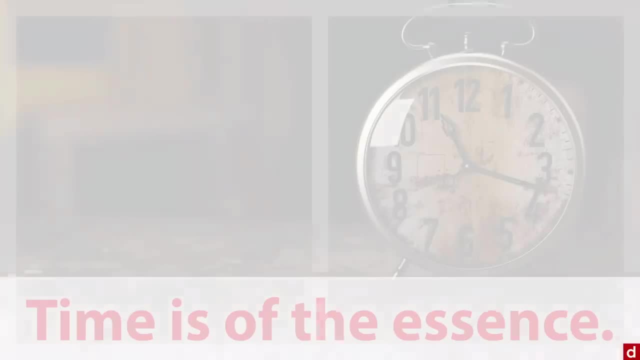 systems. So if time is of the essence- when something has to be fast, it has to get the job accomplished quickly and it has to not break- then these are the ones that you're probably going to use. The people who are going to use it are primarily going to be engineers. 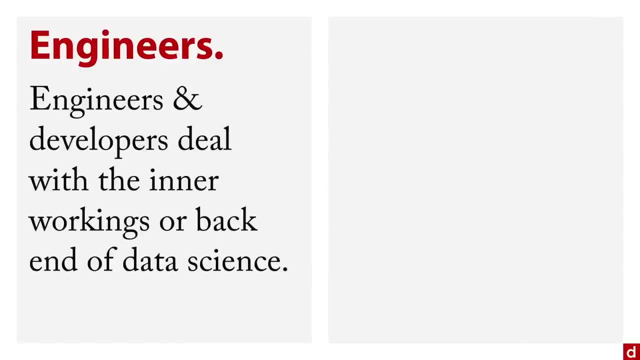 So the engineers and the developers, the software developers who deal with the inner workings of the algorithms in data science or the back end of data science, the servers and the mainframes and the entire structure that makes analysis possible. In terms of analysts, people who are actually analyzing the data typically don't do hands. 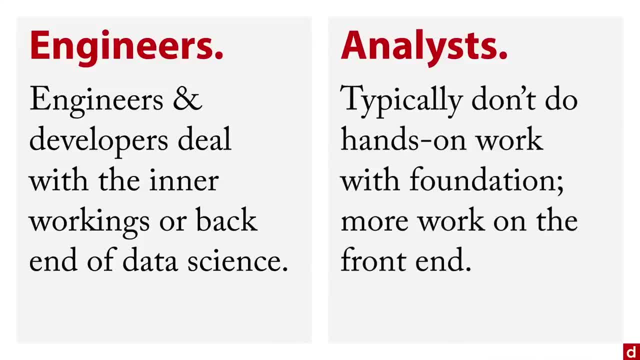 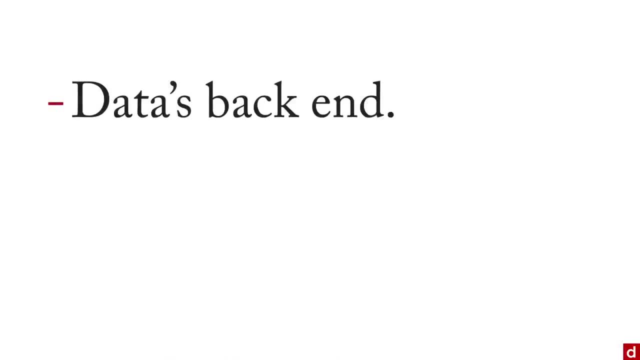 on work with the foundational elements. they don't usually touch C or C++ more. the work is on the front end or closer to the high level languages like R or Python. In sum, C, C++ and Java form a foundational bedrock and the back end of data and data. 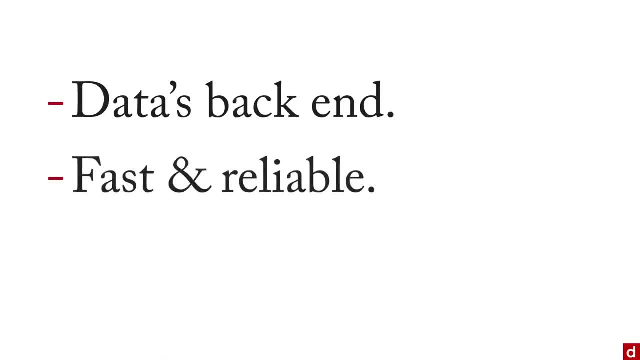 science And they do this because they're very fast And they are very fast, And they are very fast And they are very reliable. On the other hand, given their nature, that work is typically reserved for the engineers who are working with the equipment that runs in the back. that makes the rest of the analysis. 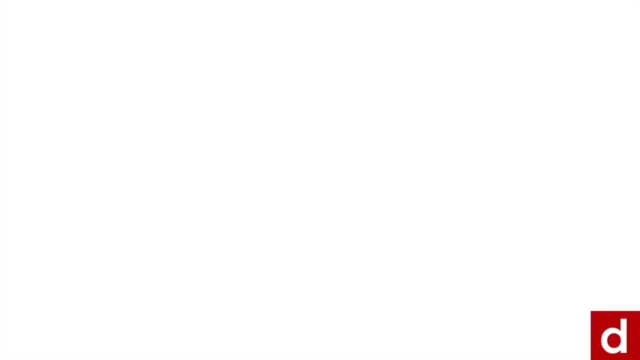 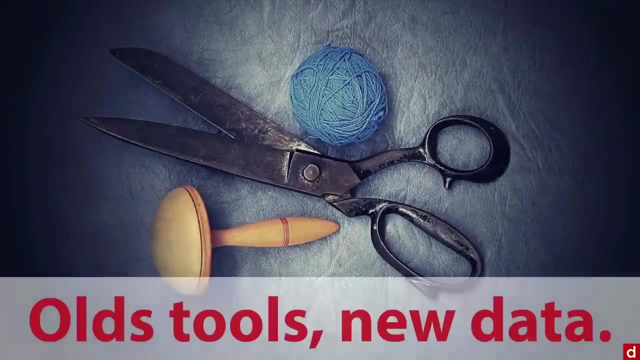 possible. I want to finish our extremely brief discussion of coding and data sciences and the languages that can be used by mentioning one other that's called bash, And bash really is a great example of old tools that have survived And are still being used actively and productively with new data. 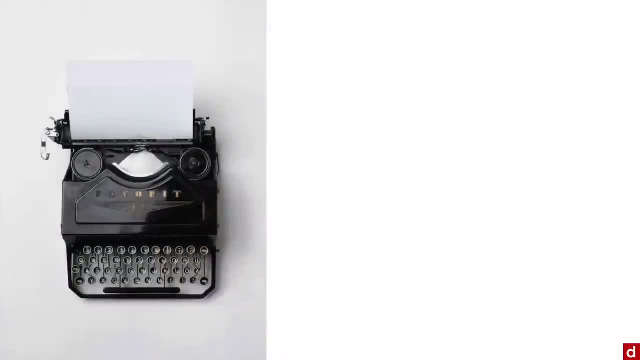 You can think of it this way: it's almost like typing on your typewriter. you're working at the command line. you're typing out code through a command line interface or a CLI. Now this method of interacting with computers practically goes back to the typewriter phase. 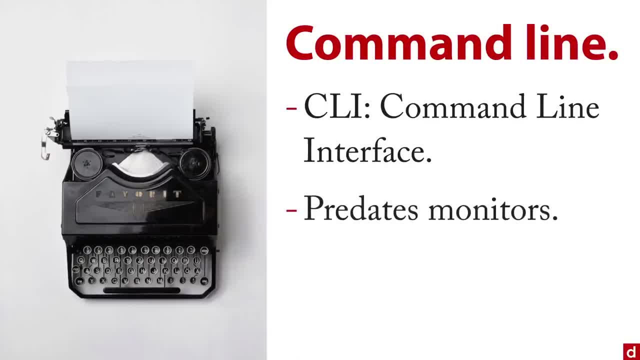 because it predates monitors. So before you even had a monitor, you would type in the code and it would print it out on a piece of paper. And the important thing to know about the command line is: it's simple. It's simple. 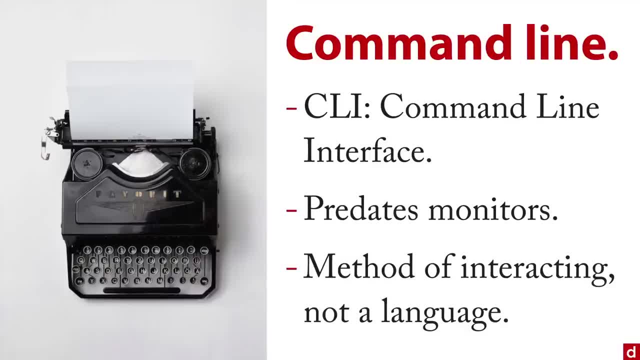 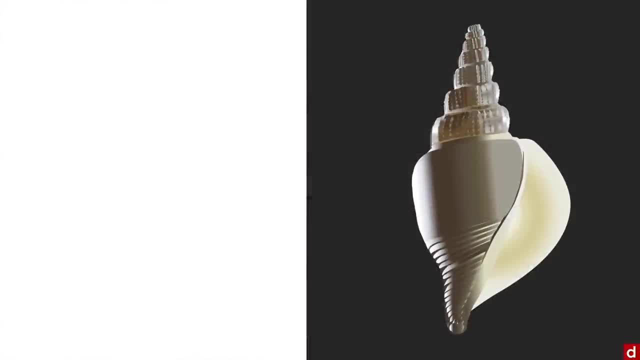 It's simply a method of interacting. It's not a language, because lots of different languages can run at the command line. So, for instance, it's important to talk about the concept of a shell Now. in computer science, a shell is a language or something that wraps around the computer. 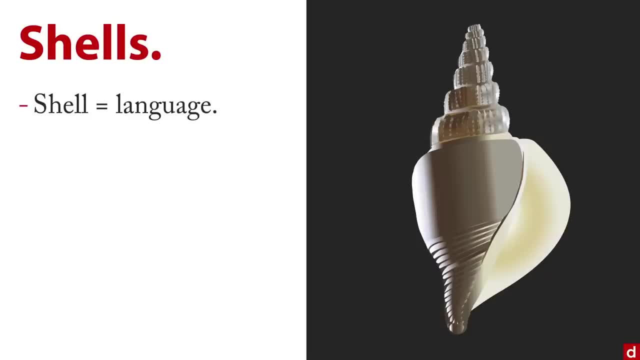 to shell around the language. That is the interaction level for the user to get things done at the lower levels that aren't really human friendly. On Mac computers and Linux, the most common is bash, Which is short for born again shell. On Windows computers, the most common version is PowerShell. 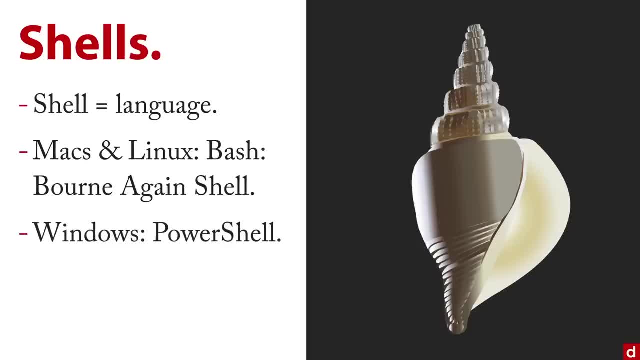 But whatever you do, there actually are a lot of choices. There's the born shell, There's the C shell- which is why I have a C shell right here- The Z shell, There's fish for friendly interactive shell and a whole bunch of other choices. 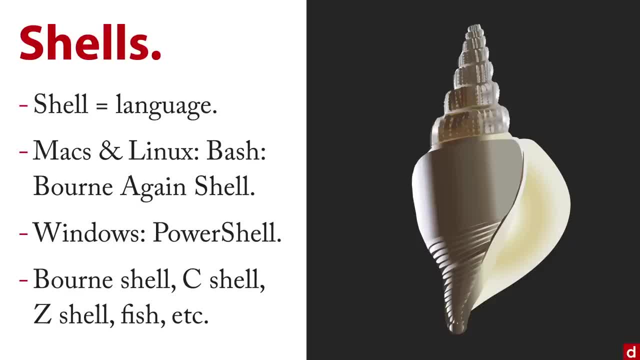 But bash is the most common on Mac and Linux, And PowerShell is the most common. It's the most common on Windows as a method of interacting with the computer at the command line level. Now there's a few things you need to know about this. 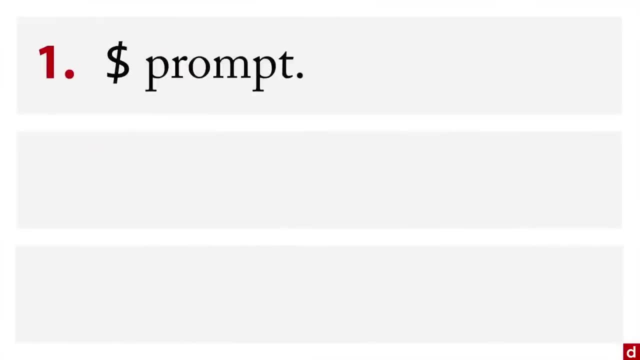 First you have a prompt of some kind and bash, it's a dollar sign And that just means type your command here. Then the other thing is you type one line at a time. It's actually amazing how much you can get done with what's called a one liner program. 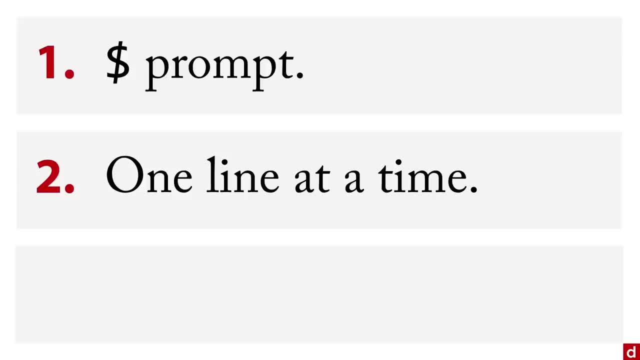 by sort of piping things together, So one feeds into the other. You can run more complex commands If you use a script, And so you call a text document that has a bunch of things in it, and you can get much more elaborate analyses done. 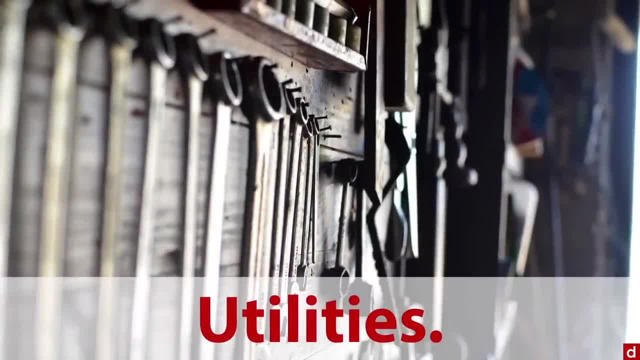 Now we have our tools. here in bash We talk about utilities and what these are are specific programs that accomplish specific tools. Bash really thrives on do one thing and do it very well. There are two general categories of utilities for bash. Number one: 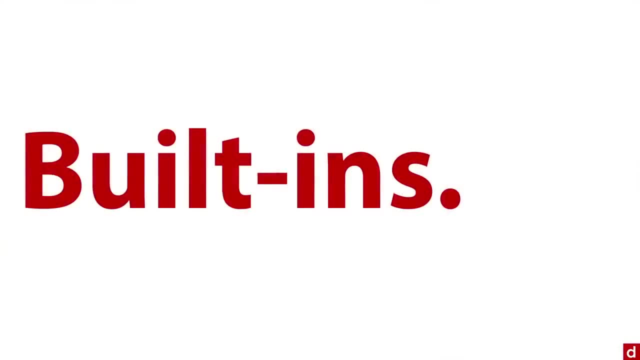 Is the built-ins. These are the ones that come installed with it, And so you're able to use them at any time by simply calling in their name. Some of the most common ones are cat, which is for cat Nate, and that's to put information. 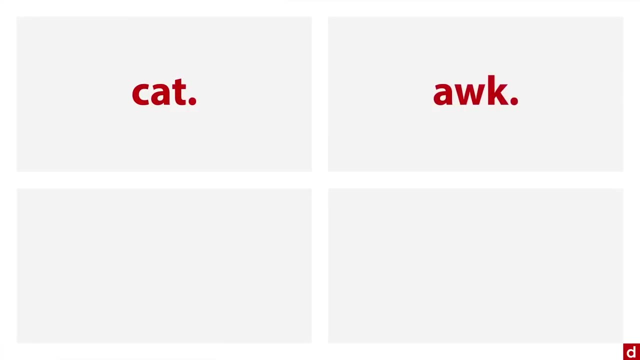 together. There's awk, which is its own interpreted programming language, but it's often used for text processing from the command line. By the way, the name awk is comes from the initials of the people who created it. Then there's grep. 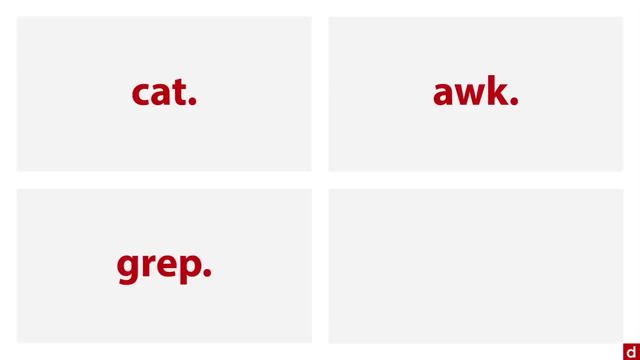 Okay. And then there's set, which stands for global search with a regular expression and print, It's a way of searching for information. And then there's sed, which stands for stream editor, and its main use is to transform text. You can do an enormous amount with just these four utilities. 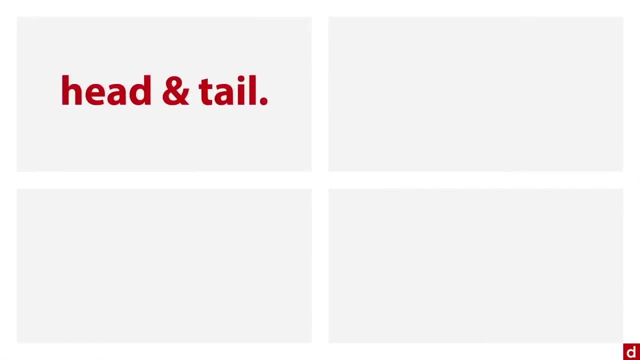 A few more are head and tail that display the first or last 10 lines of a document. sort and unique, which sort and count the number of unique answers in a document. Wc, which is for word count, and printf, which formats the output that you get in your console. 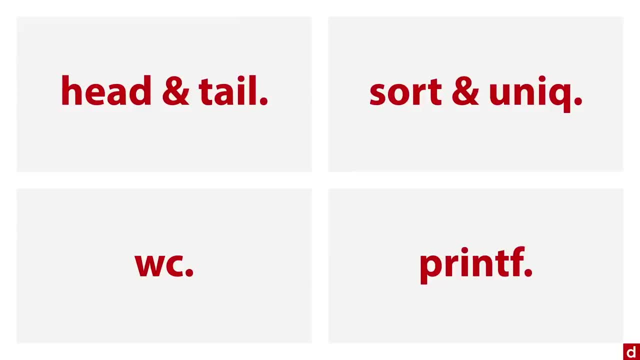 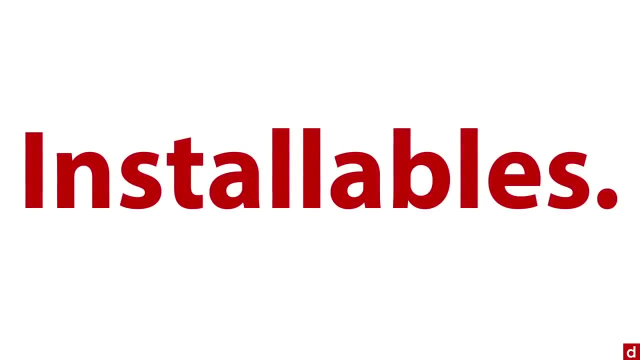 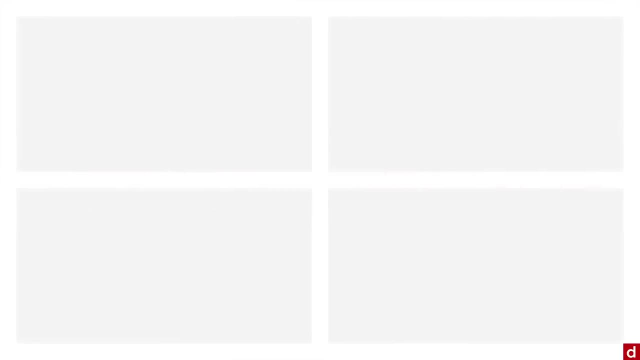 And while you can get a huge amount of work done with just this small number of built in utilities, there are also a wide range of installables or other command line utilities that you can add to bash or to whatever program you're using. So, for instance, some really good ones that have been recently developed are jq, which 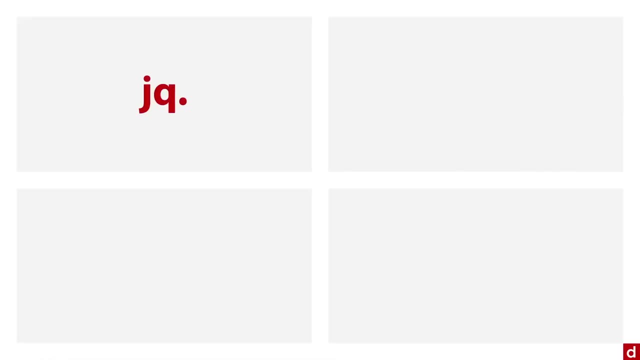 is for pulling in JSON or JavaScript object notation data from the web. And then there's JSON to CSV, which is a way of converting JSON to CSV format, which is what a lot of statistical programs are going to be happier with. There's Rio, which allows you to run a wide range of commands from the statistical programming. 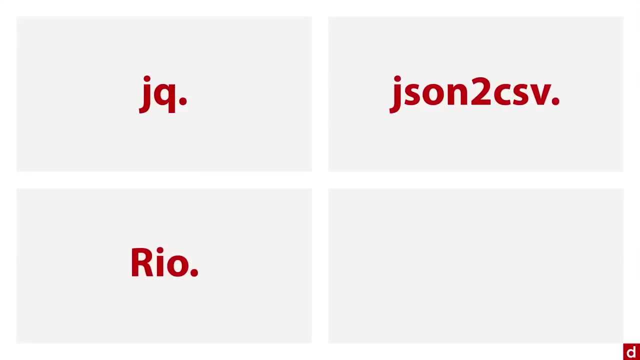 language are in the command line as part of bash. And then there's big M L R, And this is a command line tool that allows you to access big M L's. It allows you to run machine learning servers through the command line. Normally you do it through a web browser and it accesses their servers remote. 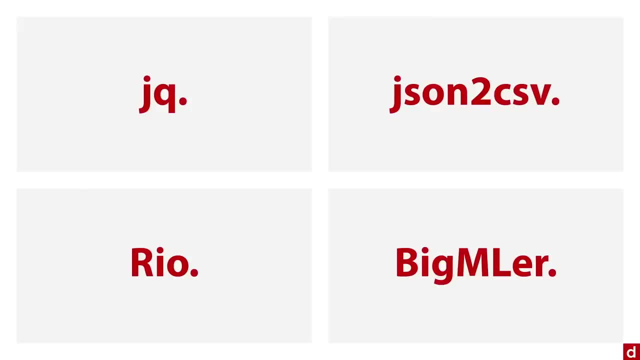 It's an amazingly useful program, but to be able to just pull it up when you're in the command line is an enormous benefit. What's interesting is that, even though you have all these opportunities, all these different utilities, you can do amazing things, and that there still is active development of utilities. 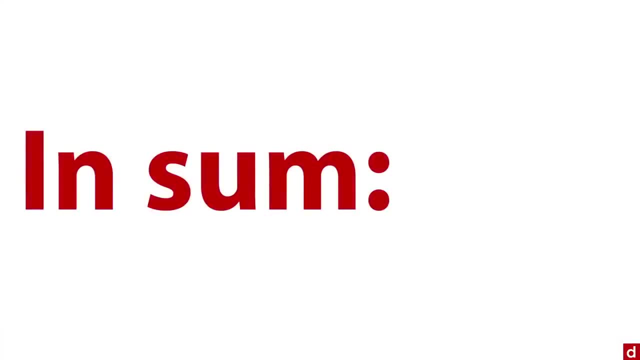 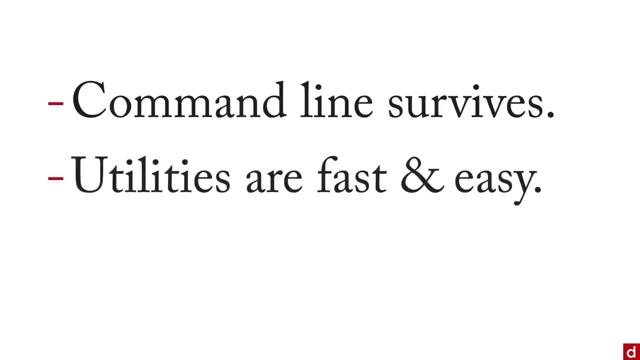 for the command line. So let's say this in some- Yeah, In one sense, as old as the dinosaurs. the command line survives because it is extremely well evolved and well suited to its purpose of working with data. The utilities, both the built in and the installables, are fast and they are easy and generally they 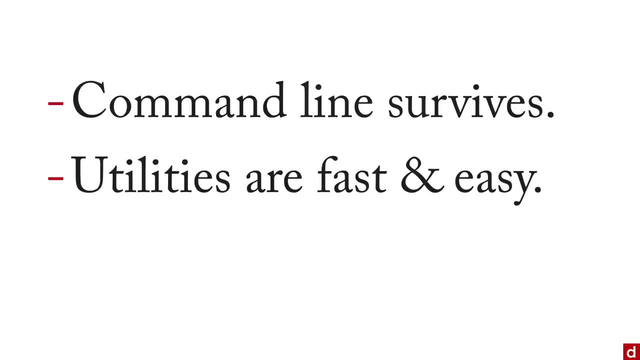 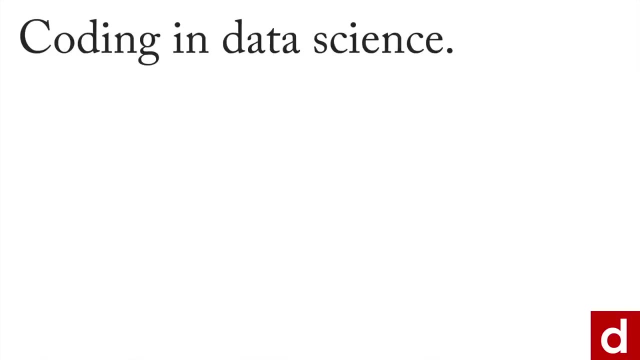 do one thing and they do it very, very well, And then, surprisingly, there is an enormous amount of very active development of command line utilities for these purposes, especially with data science. One critical task when you're coding in data science is to be able to find the things that 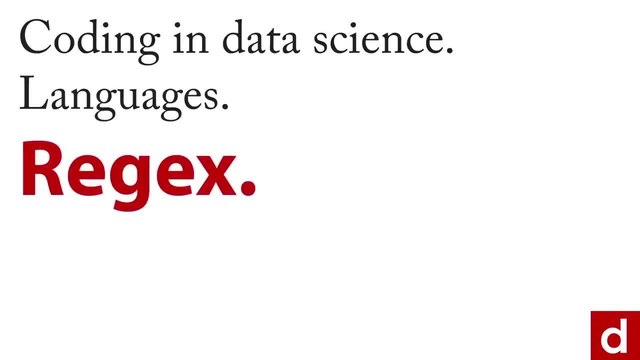 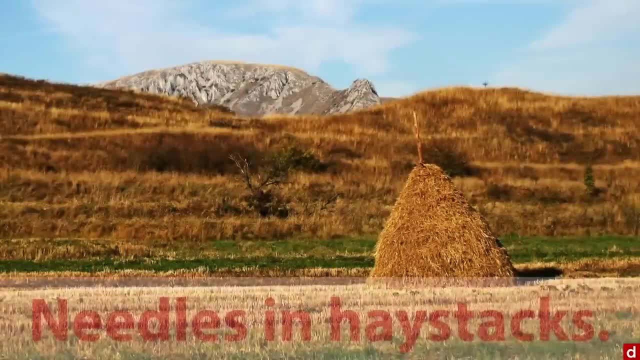 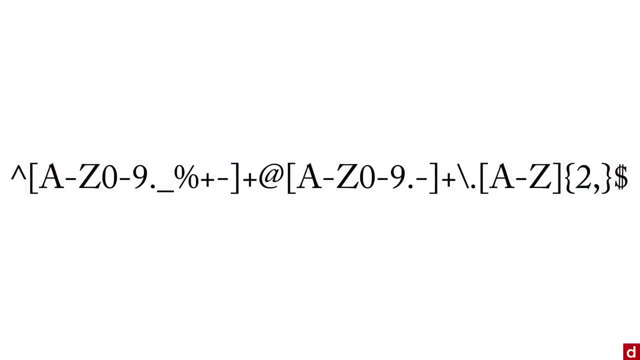 you're looking for, And regex, which is short for regular expressions, is a wonderful way to do that. You can think of it as the supercharged method for finding needles in haystacks. Now, regex tends to look a little cryptic. So, for instance, here's an example of something that's designed to determine whether something 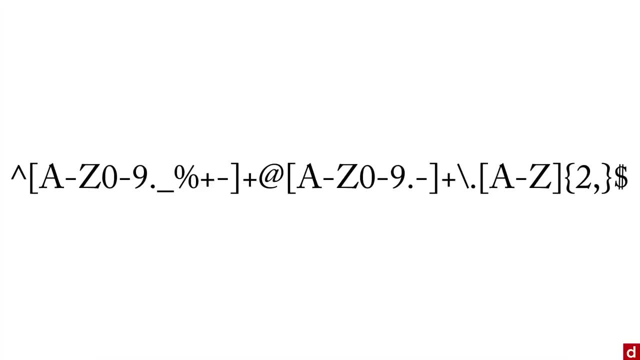 is a valid email address and it specifies what can go on the beginning, Yeah. In the middle, Then you've got a certain number of numbers and letters, and then you have to have a dot, something at the end, And so this is a special kind of code for indicating what can go where. 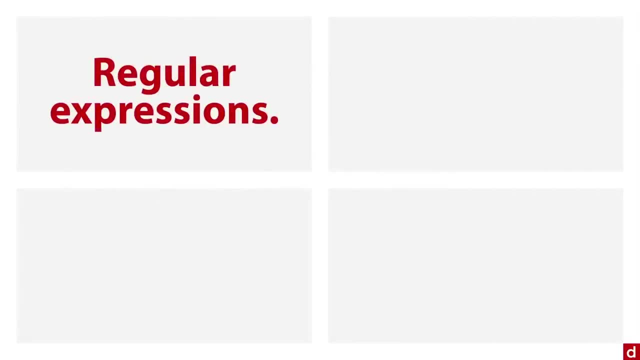 Now, regular expressions or regex are really a form of pattern matching in text And it's a way of specifying exactly what needs to be where what can vary and how much it can vary. And you can write both specific patterns. say, I only want a one letter variation here. 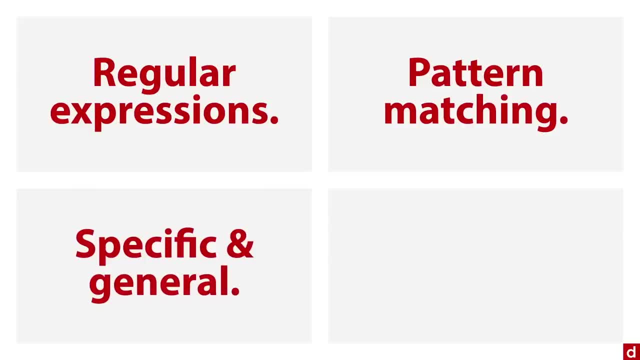 or very general, like the email validator that I have here, And you can write both specific patterns- say, I only want a one letter variation here. or very general, like the email validator that I showed you, And the idea here is you can write this search pattern, your little wildcard thing. 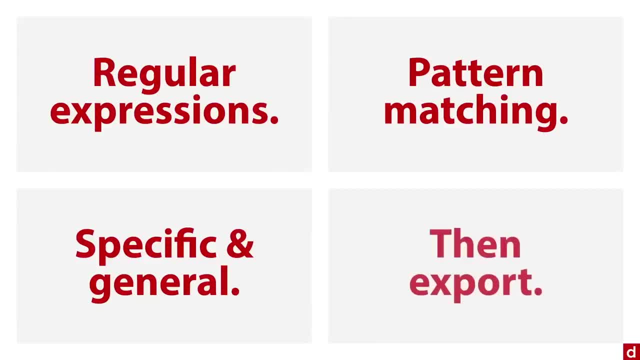 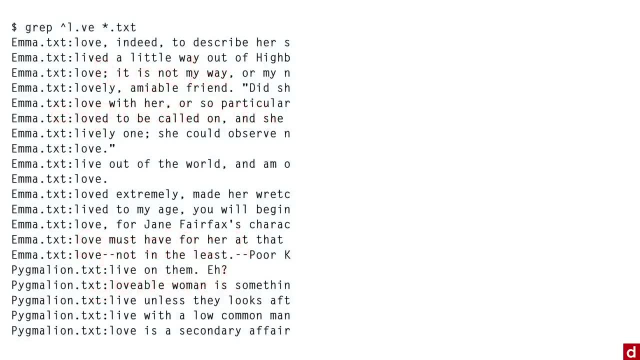 You can find the data and then, once you identify those cases, then you can export them into another program for analysis. So here's a short example of how it can work. What I've done is I've taken some text documents. They're actually the text to Emma and to Pygmalion, two books I got off of Project Gutenberg. 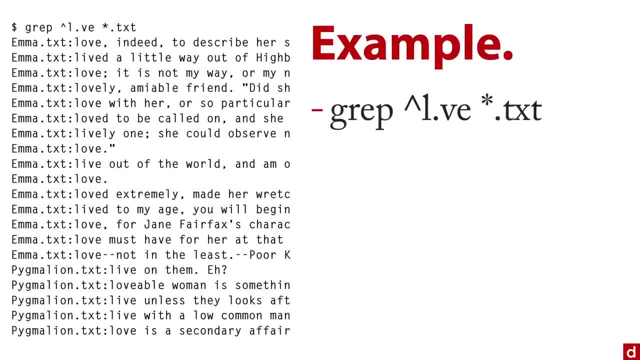 And this is the command: grep, caret, L, dot V, E, space, Asterisk, dot txt. So what I'm looking for are lines in either of these books that start with L, Then they have one character- can be whatever- And then that's followed by V, E, And then the dot txt means search for all of the text. 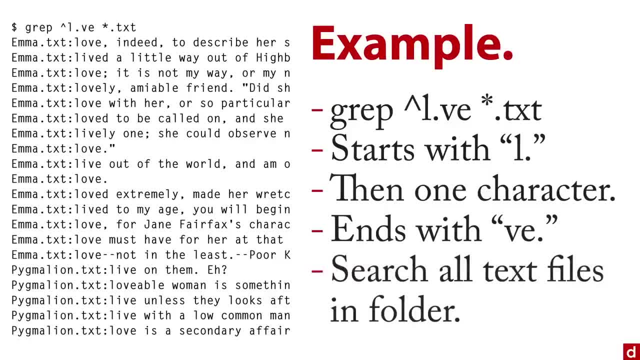 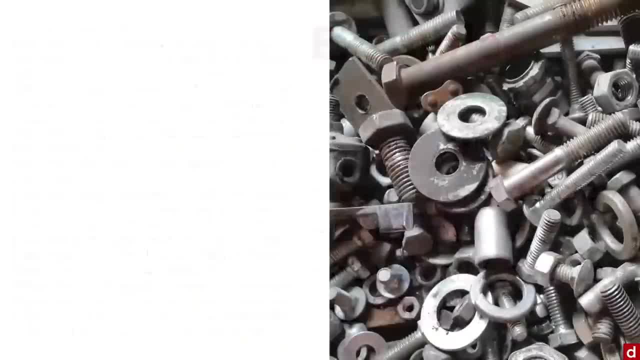 files in that particular folder And what it found is lines that began with love and lived and lovely and so on. Now, in terms of the actual nuts and bolts of regular text: There are expressions, there are some certain elements, There are literals. 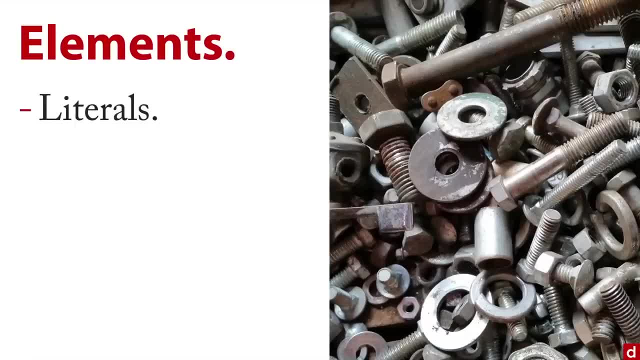 And those are things that mean exactly what they are. you type the letter L, you're looking for the letter L. There are also meta characters which specify, for instance, things needs to go here. they they're characters, but they actually really code that give representations. 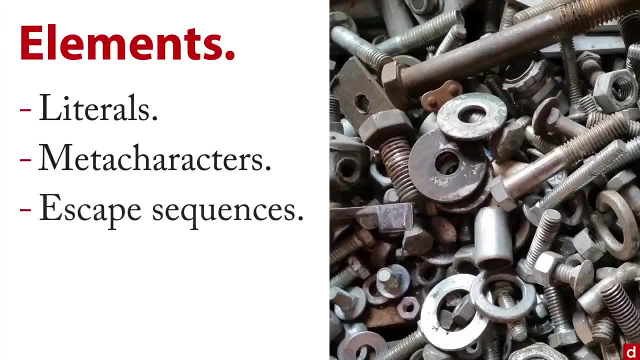 There are also escape sequences, which are something that you use to say: well, normally this character is used as a variable, but I actually want to really look for a period as opposed to a place Holder. Then you have the entire search expression that you create. 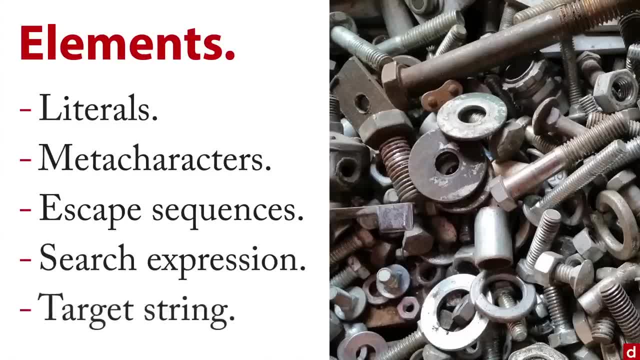 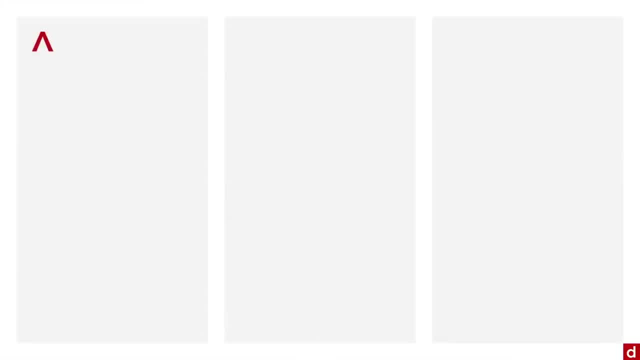 And then you have the target string, the thing that is searching through. So let me give a few very short examples. This is the carrot, it's the sometimes called a hat or, in French, a circle and flex, And what that means is you're looking for something that's at the beginning of the text. 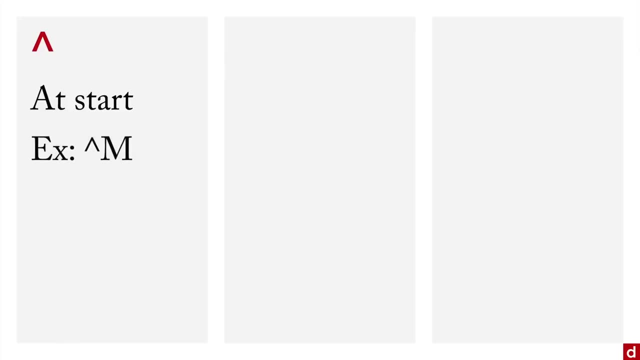 that you're searching. So, for example, you can have carrot and capital M. that means you need something that begins with a capital M. So, for instance, the word Mac, true, it will find that, But if you have iMac, there's a capital M, but it's not the first thing. 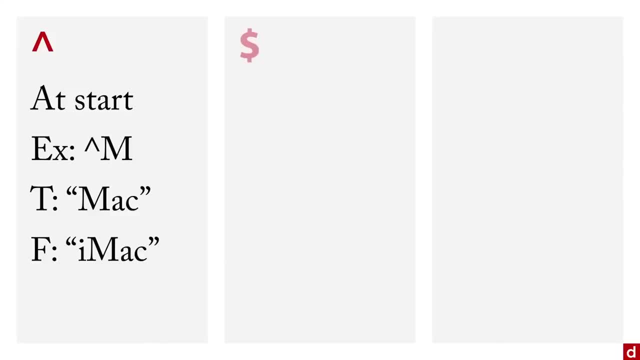 So that'll be false. it won't find that The dollar sign means you're looking for something that is at the end of the string. So, for example, ing and then dollar sign, that'll find the word fling because it ends. 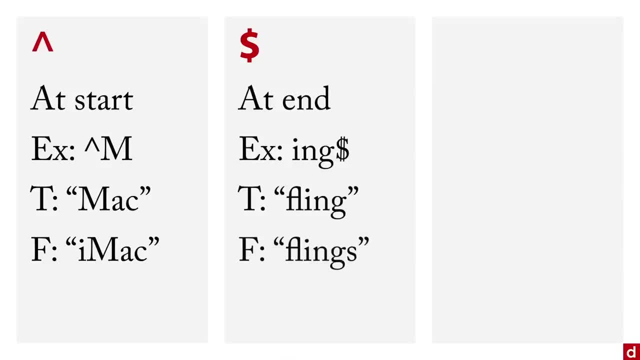 with ing, But it won't find the word flings because it actually ends with an S And then the dot. the period simply means we're looking for one letter, And it can be anything. So, for example, you can write AT: period: 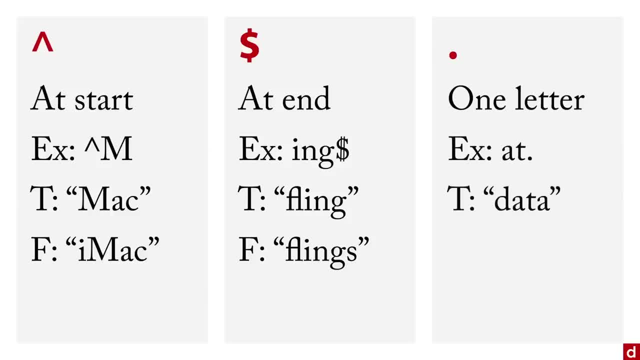 And that will find data, because it has an A, a, T and then one letter after it, But it won't find flat, because flat doesn't have anything after the AT. And so these are extremely simple examples of how it can work. Obviously, it gets more complicated and the real power is when you start combining these. 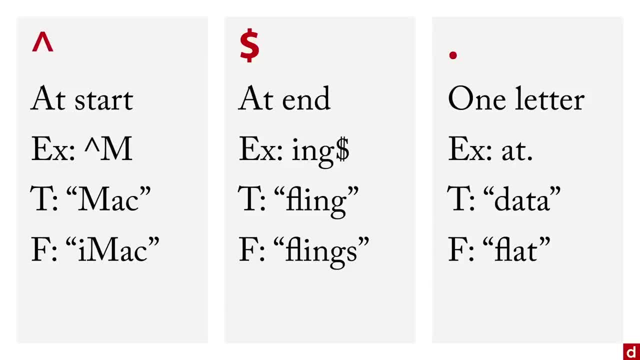 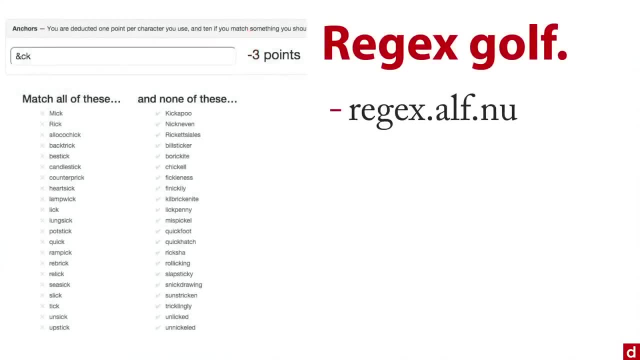 bits and elements. Now, one interesting thing about this is you can actually treat this as a game. I love this website. it's called RegEx Golf And it's at regxalfnu, And what it does is it brings up lists of words, two columns, and your job is to write. 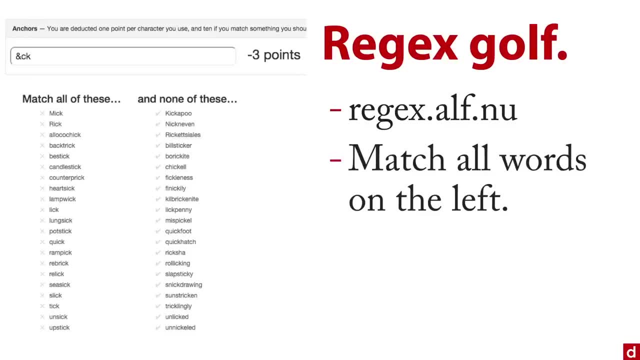 a regular expression in the top that matches all the words on the left column and none of the words on the right And that uses the fewest characters possible, you get a score, And it's a great way of learning how to do regular expressions. 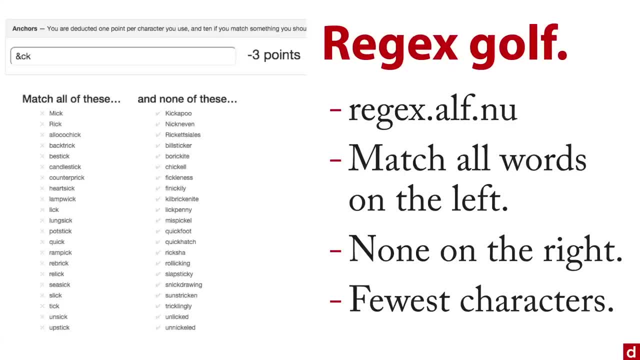 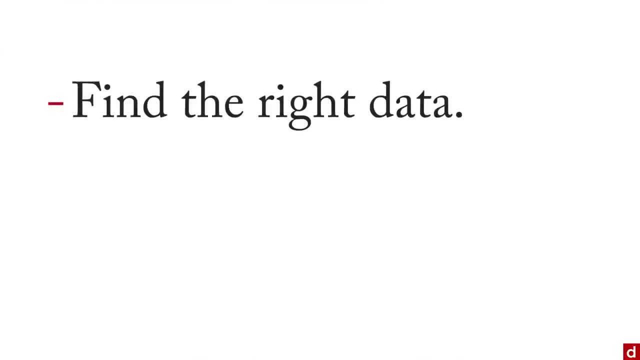 And And how to search in a way that's going to get you the data that you need for your projects. So, in sum, RegEx, or regular expressions, help you find the right data for your project. They're very powerful and they're very flexible. 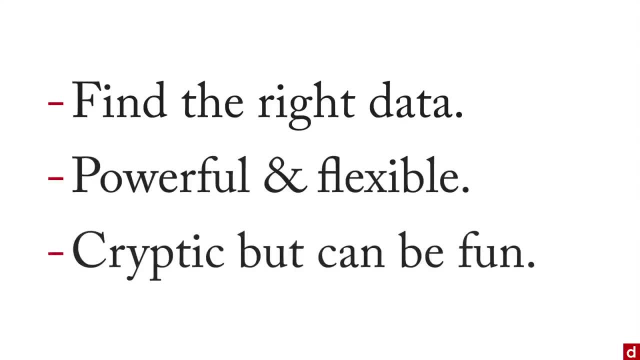 Now, on the other hand, they are cryptic, at least when you first look at them. But at the same time, it's like a puzzle and it can be a lot of fun if you practice it and you see how you can find what you need. 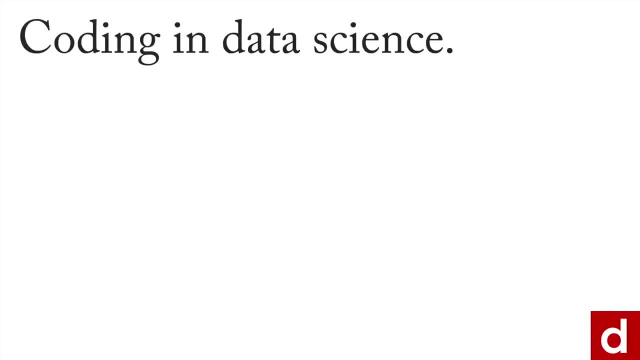 I want to thank you for joining me in coding Data science, and we'll wrap up this course by talking about some of the specific next steps that you can take for working in data science. The idea here is that you want to get some tools and you want to start working with those. 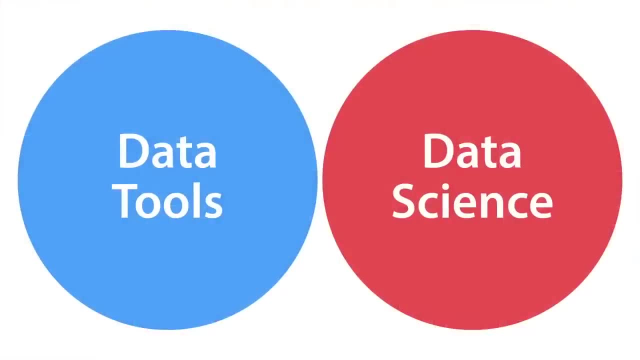 tools. Now please keep in mind something that I've said at another time: Data tools and data science are related. they're important, But don't make the mistake of thinking that, if you know the tools, that you have done the same thing as actually conducted data science. 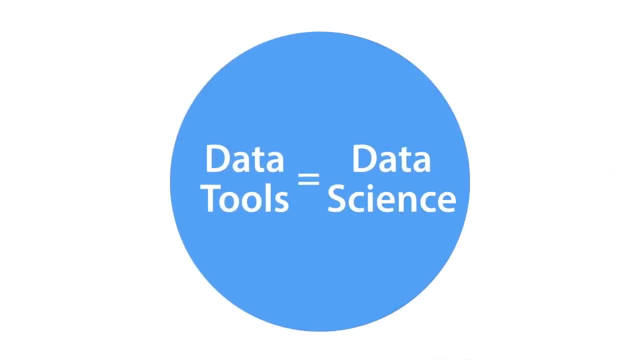 That's not true. Data tools sometimes get a little enthusiastic and they get a little carried away. What you need to remember is the relationship really is this: Data tools are an important part of data science, but data science itself is much bigger than just the tools. 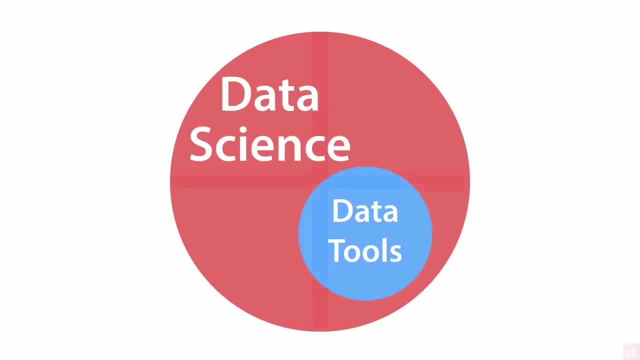 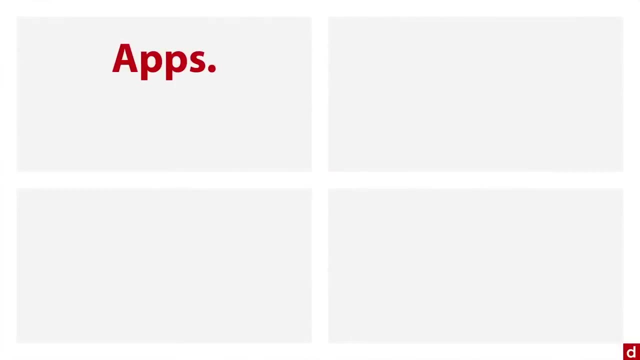 Now, speaking of tools, remember there's a few kinds that you can use and that you might want to get some experience with these. Number one, in terms of apps, or just specific built applications, Excel and Tableau are really fundamental for both Getting the data from clients or doing some basic data browsing, and Tableau is really 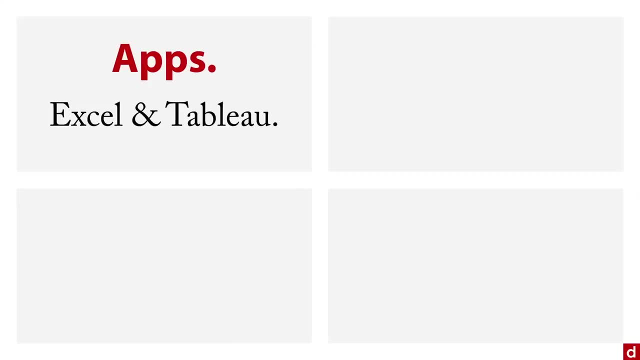 wonderful for interactive data visualization. I strongly recommend that you get very comfortable with both of those. In terms of code, it's a good idea to learn either R or Python, or ideally, to learn both, because you can use them hand in hand. In terms of utilities, it's a great idea to learn how to work with Bash, the command line. 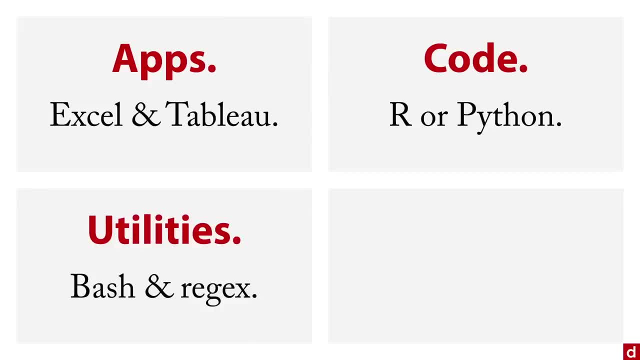 utility. You can actually use regular expressions or regex. You can actually use those in lots and lots of programs, regular expressions, and so they can have a very wide application. And then, finally, data science requires some kind of domain expertise. You're going to need some sort of field experience or intimate understanding of a particular 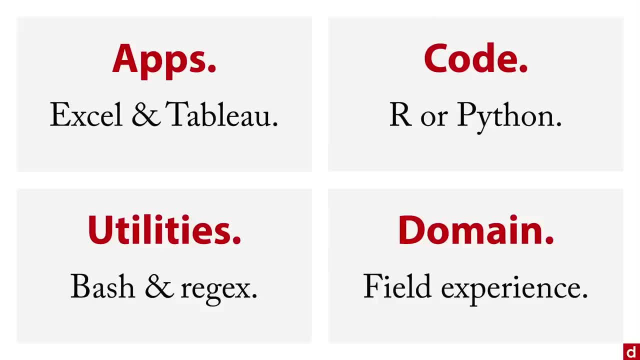 domain and the challenges that come up and what constitutes workable answers and the kind of data that's available. Now, as you go through all of this, you don't need to build this monstrous List of things. Remember, you don't need everything. 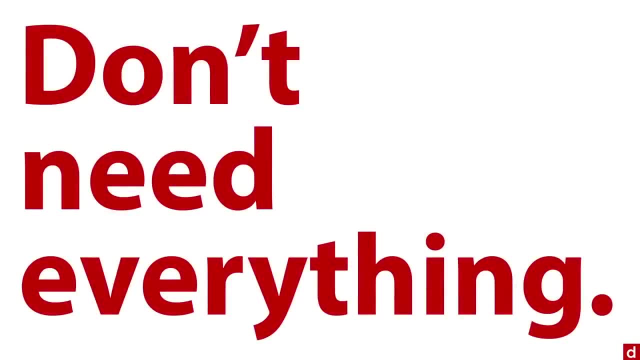 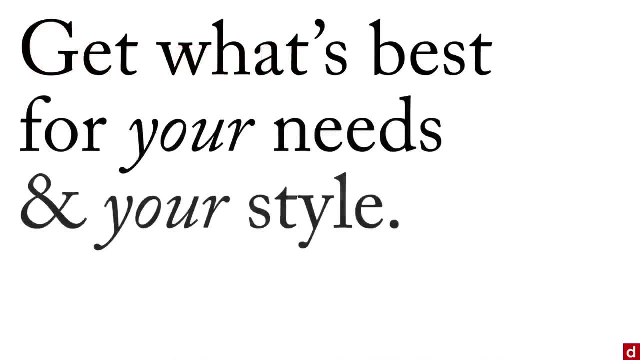 You don't need every tool, You don't need every function, You don't need every approach. Instead, remember, get what's best for your needs and for your style, But no matter what you do, remember tools are tools. They're a means to an end. 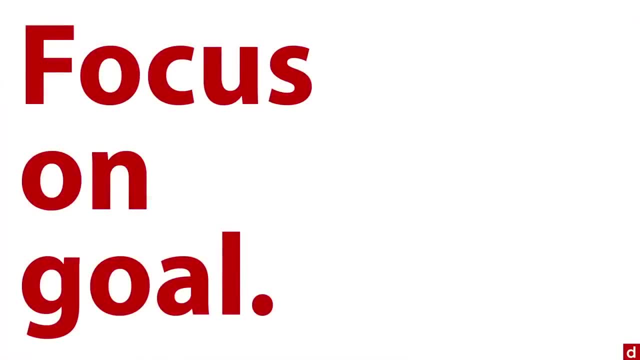 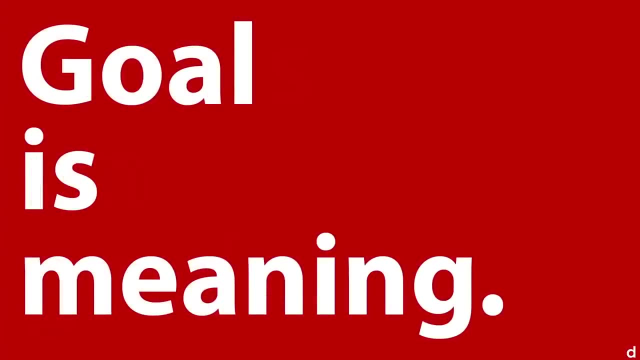 Instead, you want to focus on the goal of your data science project, whatever it is, And I can tell you, really, the goal is a meaning Extracting. Extracting meaning out of your data to make informed choices. In fact, I'll say a little more. 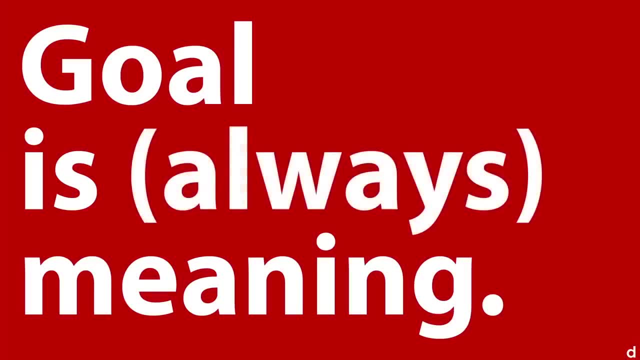 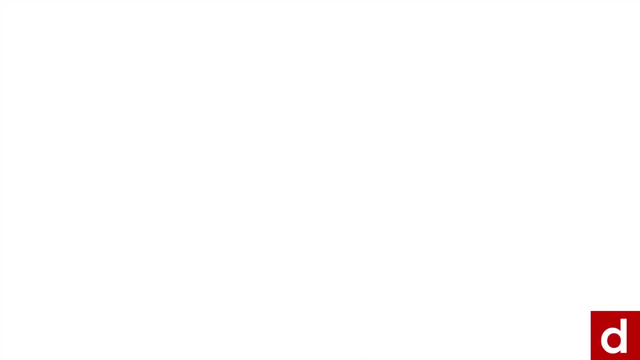 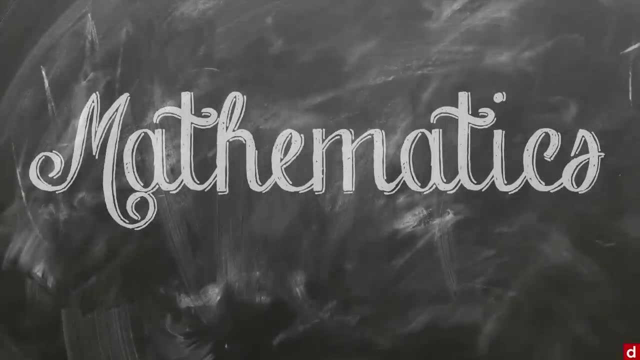 The goal is always meaning, And so, with that, I strongly encourage you, get some tools, get started in data science and start finding meaning in the data that's around you. Welcome to mathematics and data science. I'm Barton Poulson, And we're going to talk about how mathematics matters for data science. 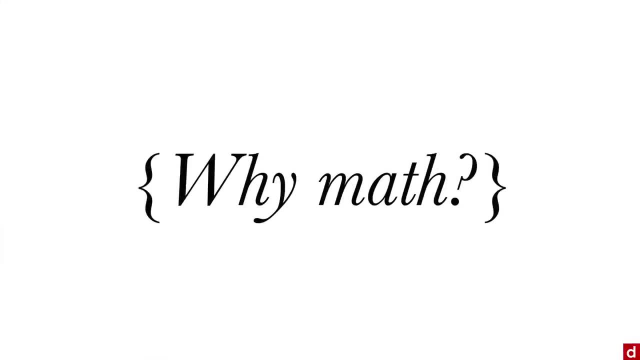 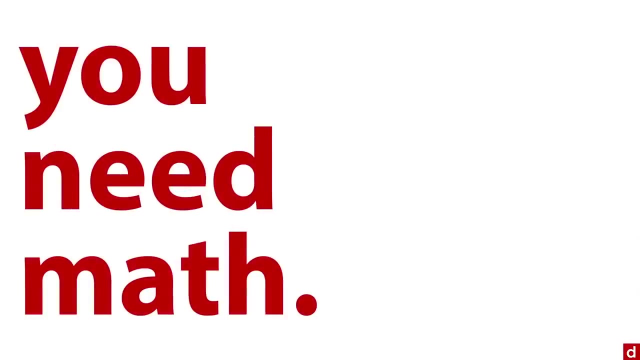 Now you may be saying to yourself why math And computers can do it. I don't need to do it And, really fundamentally, I don't need math. I'm just here to do my work. Well, I'm here to tell you: no, you need math. 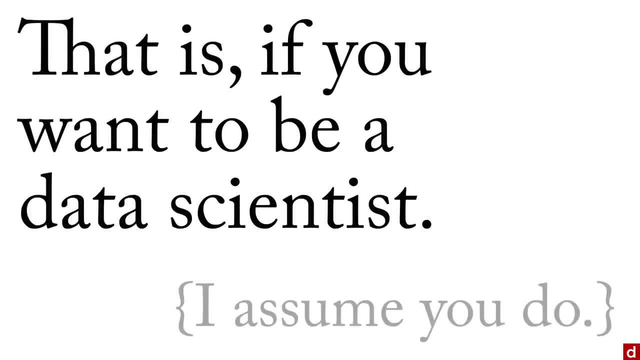 That is, if you want to be a data scientist- and I assume that you do So. we're going to talk about some of the basic elements of mathematics really at a conceptual level and how they apply to data science. There are a few ways that math really matters to data science. 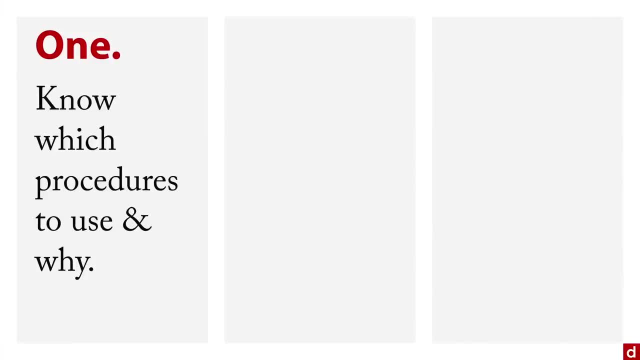 Number one: It allows you to know which procedures to use and why, So you can answer your questions in a way that's the most informative and most useful. Two: if you have a good understanding of math, then you know what to do when things don't. 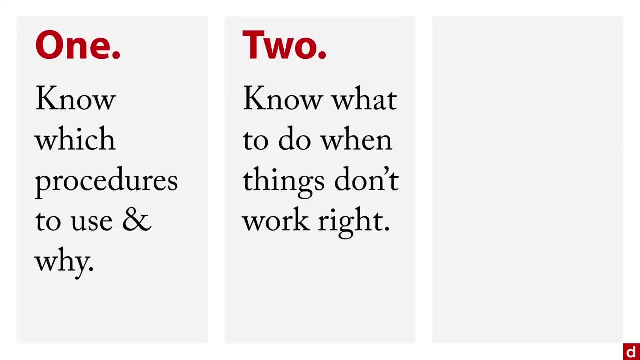 work right, that you get impossible values or things won't compute, And that makes a huge difference. And then three: an interesting thing is that some mathematical procedures are easier and quicker to do, And then by actually firing up the computer. And so, for all three of these reasons, it's helpful to have at least a grounding in mathematics. 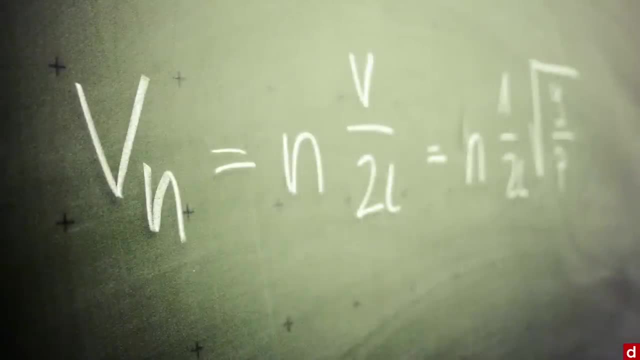 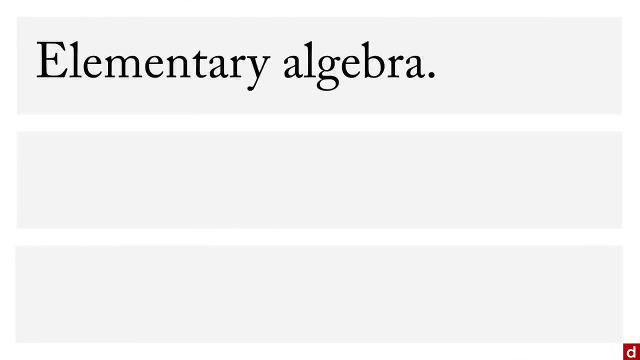 if you're going to do work in data science Now probably the most important thing to start with is algebra, And there are three kinds of algebra that we want to mention. The first is elementary algebra, that's the regular x plus y. Then there's linear or matrix algebra, which looks more complex, but it's conceptually. 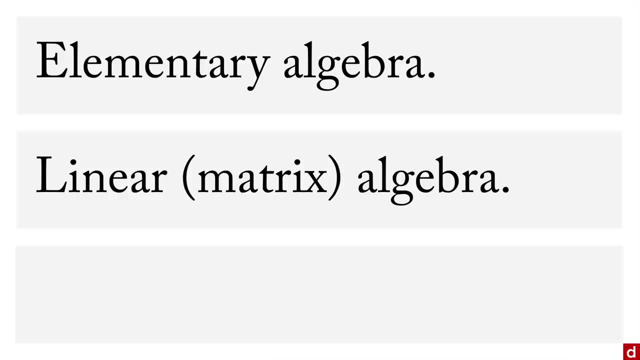 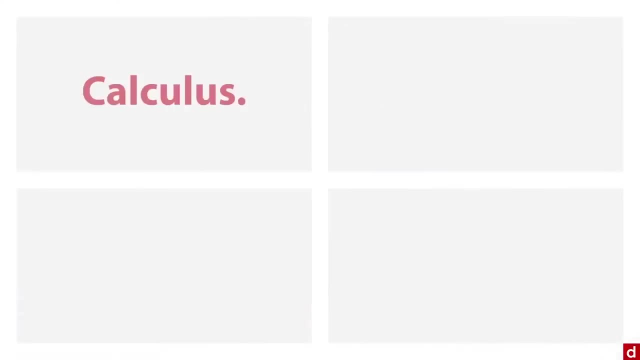 simpler and it's used by computers to actually do the calculations. And then, finally, I'm going to mention systems of linear equations, where you have multiple equations simultaneously that you're trying to solve. Now there's more math than just algebra. A few other things that I'm going to cover in this course: a little bit of calculus. 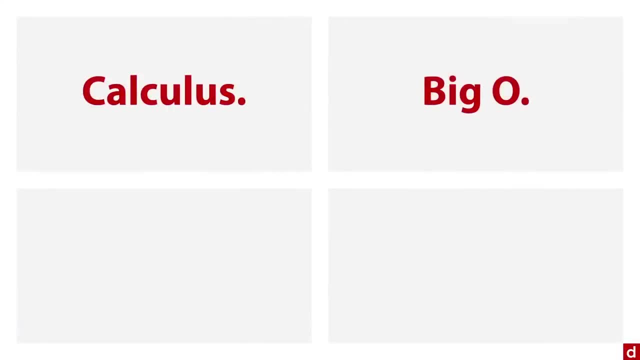 a little bit of big O or order, which has to do with the speed or the complexity of operations, a little bit of probability theory and a little bit of Bayes or Bayes theorem, which is used for getting posterior probabilities and changes the way that you interpret the. 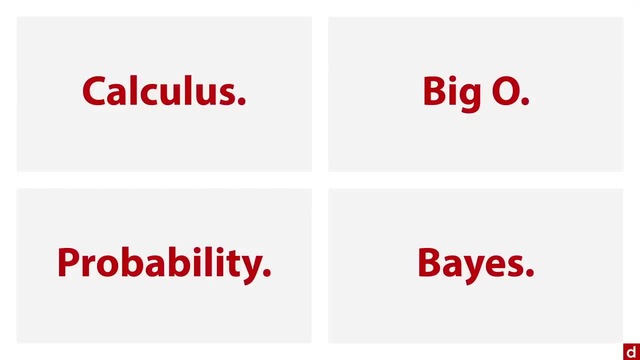 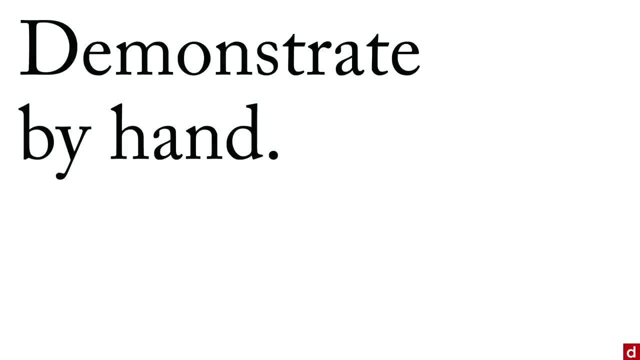 results of an analysis And, for the purposes of this course, I'm going to demonstrate the procedures by hand. Of course, you would use software to do this in the real world, but we're dealing with simple problems at conceptual levels And really the most important thing to remember is, even though a lot of people get put off, 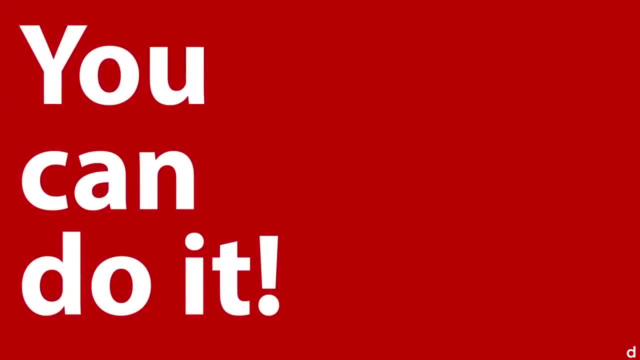 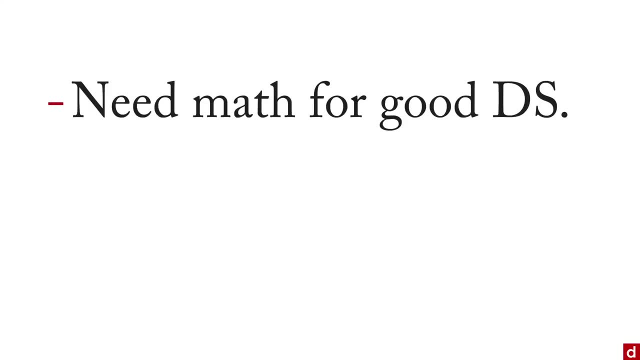 by math. really, you can do it. And so, in sum, let's say these three things about math. First off, you do need some math to do good data science. It helps you diagnose problems, It helps you choose the right procedures. 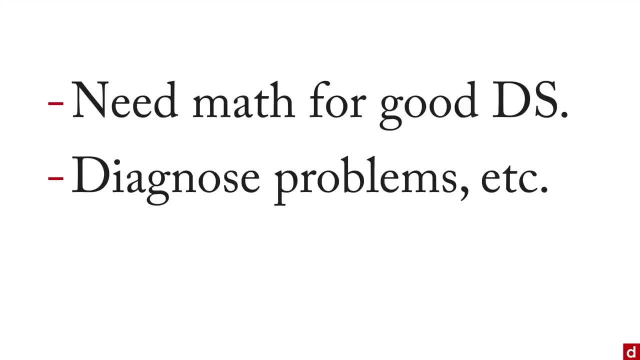 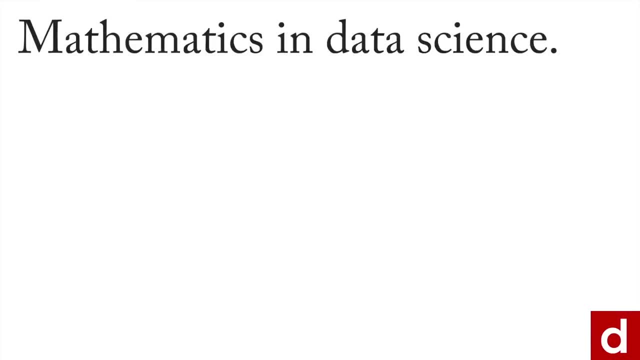 And, interestingly, you can do a lot of it by hand, or you can use software computers to do the calculations as well. As we begin our discussion of the role of mathematics and data science, we'll, of course, begin with the foundational elements. 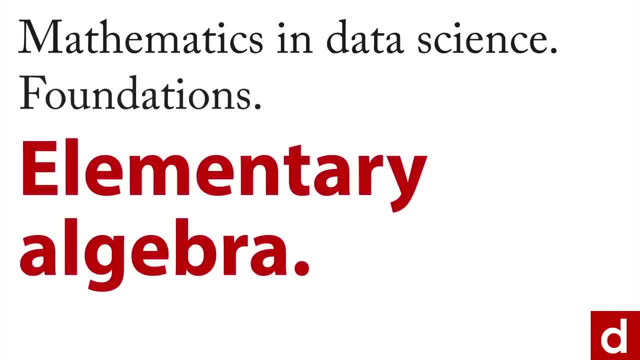 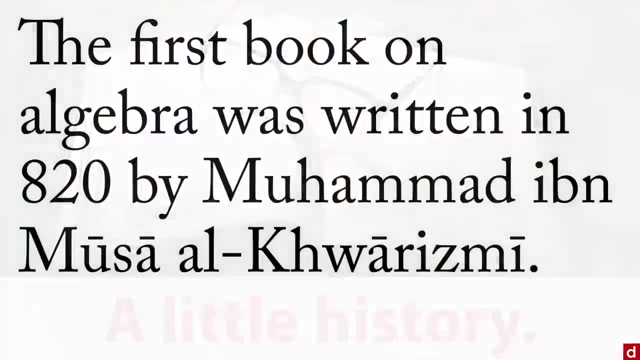 And in data science, nothing is more foundational than elementary algebra. Now I'd like to begin this with really just a little bit of history. In case you're not aware, The first book on algebra. It was written. It was written in 820 by Muhammad ibn Musa al-Khwarizmi and it was called the Compendious. 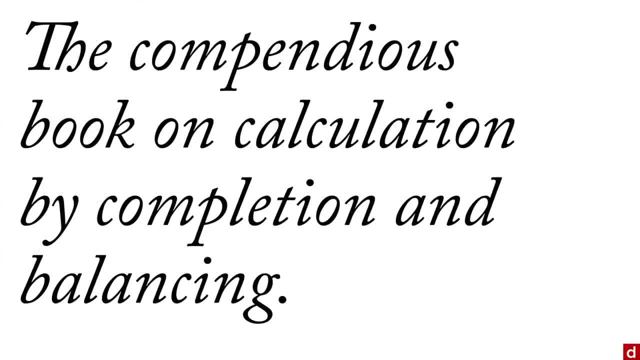 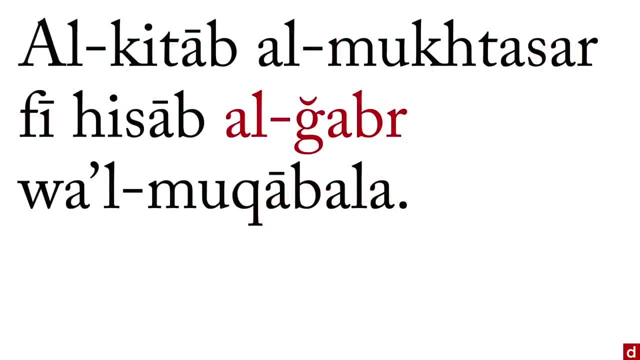 Book on Calculation by Completion and Balancing. Actually it was called this, which, if you transliterate that comes out to this, But look at this word right here. That's the algebra, which means restoration. Any case, that's where it comes from. 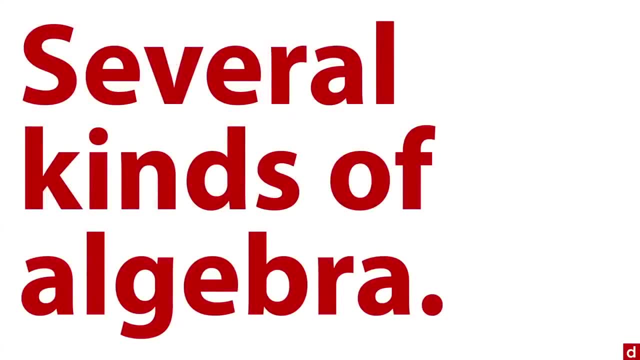 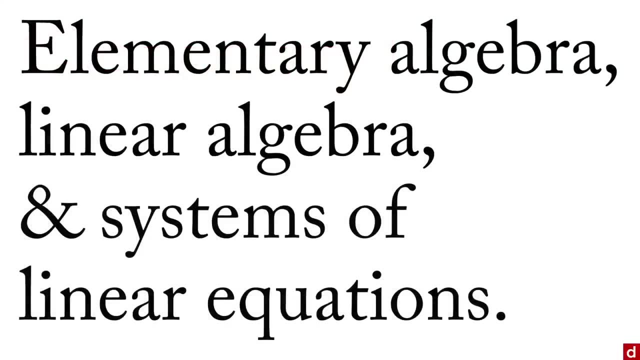 And for our concerns. there are several kinds of algebra that we're going to talk about. There's elementary algebra, There's linear algebra And there's linear algebra And there are systems of linear equations. We'll talk about each of those in different videos. 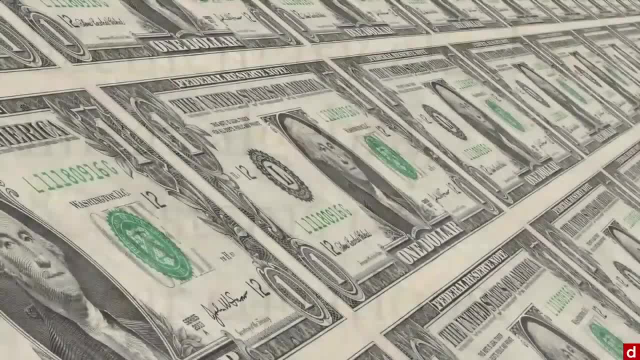 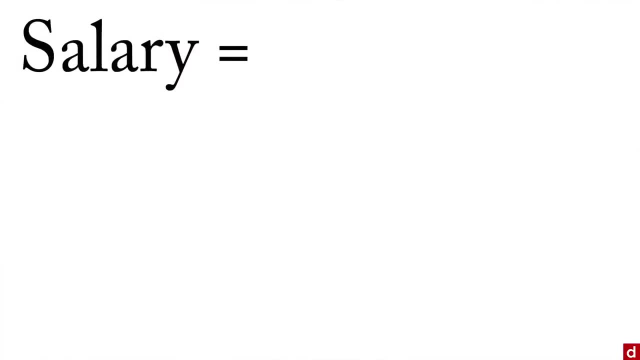 But to put it into context, let's take an example here of salaries. Now, this is actually based on real data from a survey of the salary of people employed in data science And, to give a simple version of it, the salary was equal to a constant. 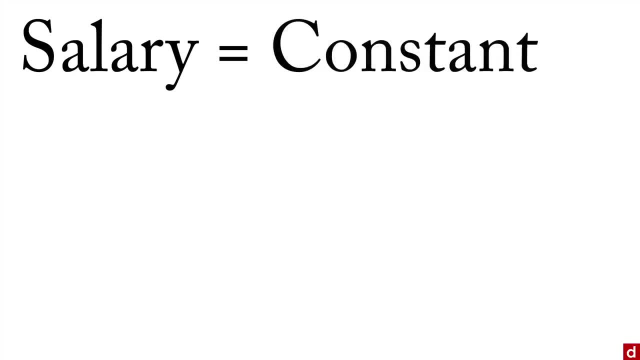 That's sort of an average value that everybody started with And to that you added years and then you added some measure of bargaining skills and how many hours they worked per week, And that gives you a prediction, But because it wasn't exact, there's also some error to throw into it. to get to the 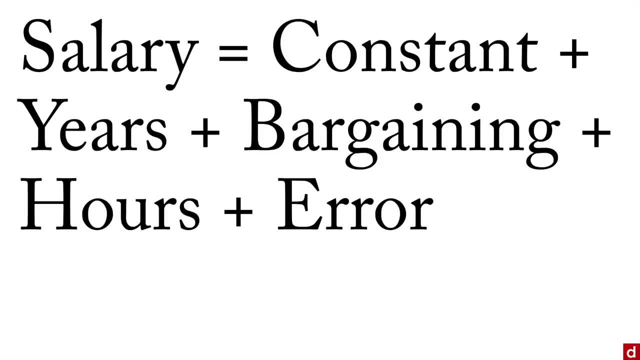 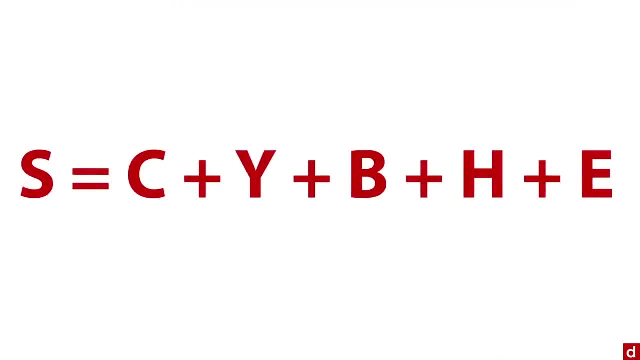 precise value that each person has. Now, if you want to abbreviate this, you can write it kind of like this: s plus c plus y plus b plus h plus e, although it's more common to write it, and although it's more common to write it symbolically like this: 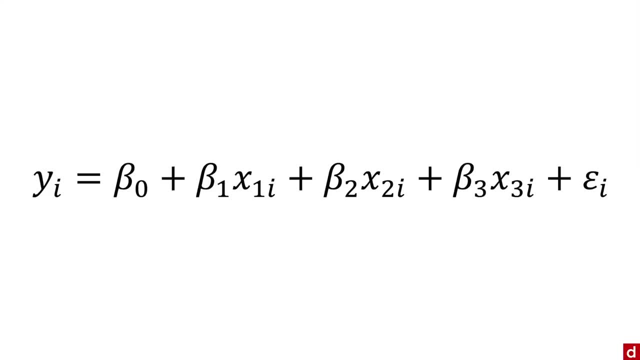 And let's go through this equation very quickly. The first thing we have is outcome. We call that y The variable. y For person i. i stands for each case in our observations. So here's outcome: y for person i. This letter right here is a Greek beta. 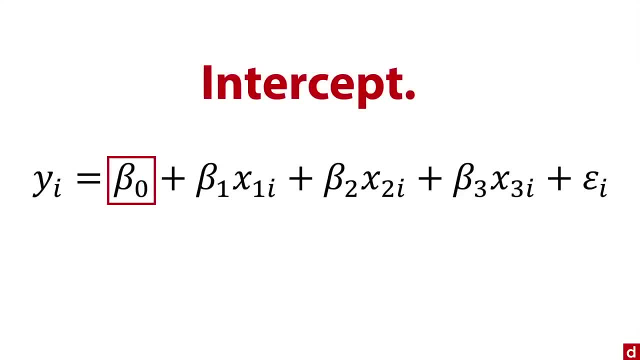 And it represents the intercept or the average. that's why it has a zero, because we don't multiply it times anything. But right next to it we have the coefficient for variable one, So beta, which means a coefficient sub one for the first variable. 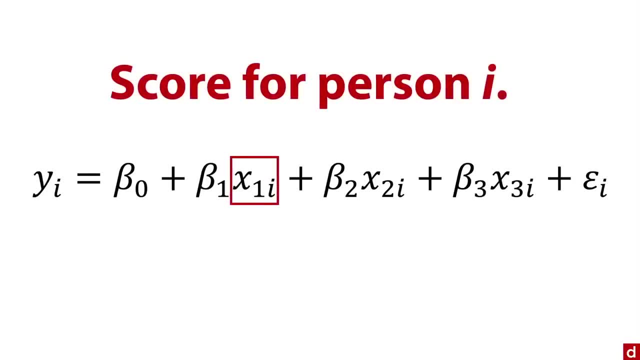 And then we have variable one, and then x one means variable one, and then the i means it's the score on that variable for person i, whoever we're talking about. Then we do the same thing for variables two and three, and then at the end we have little. 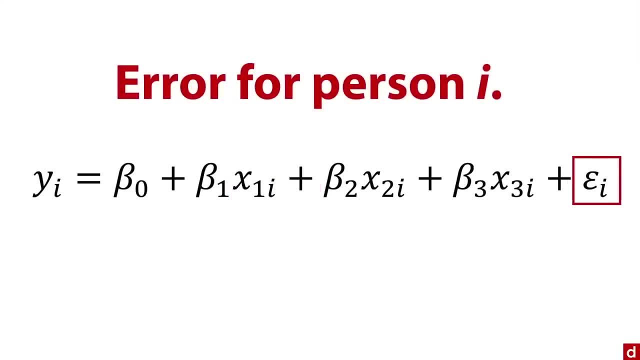 epsilon here with an i for the error term for person i, which says how far off the prediction was from their actual score. Now I'm going to run through some of these procedures and we'll see how they can be applied to data science, But for right now let's just say this in sum: 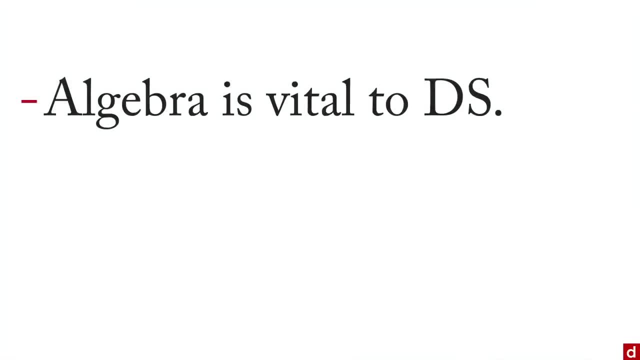 First off, algebra is vital to data science. It allows you to combine multiple scores, get a single outcome, do a lot of other manipulations And really the calculations are easy for one case at a time, especially when you're doing it by hand. 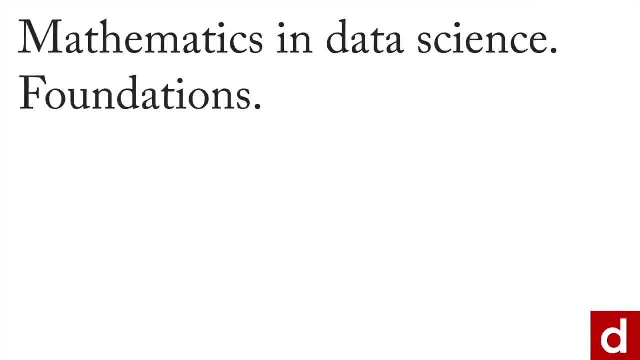 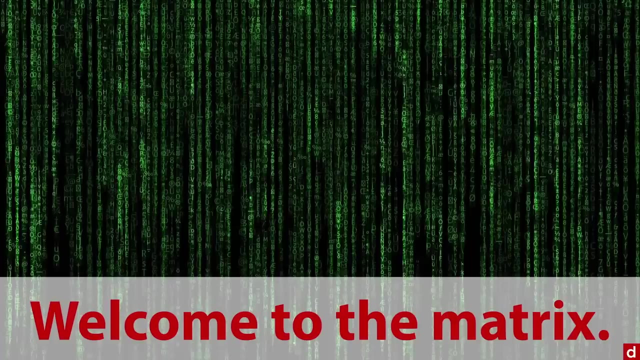 The next step in mathematics for data science foundations is to look at linear algebra, or an extension of elementary algebra, And, depending on your background, you may know this by another name And I like to think: welcome to the matrix, Also known as matrix algebra, because we're dealing with matrices. 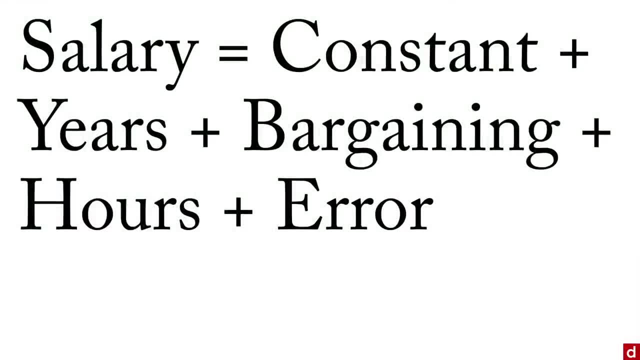 Now let's go back to an example I gave in the last video about salary, where salary is equal to a constant plus years plus bargaining, plus hours plus error. Okay, that's a way to write it out in words And if you want to put it in symbolic form, it's going to look like this: 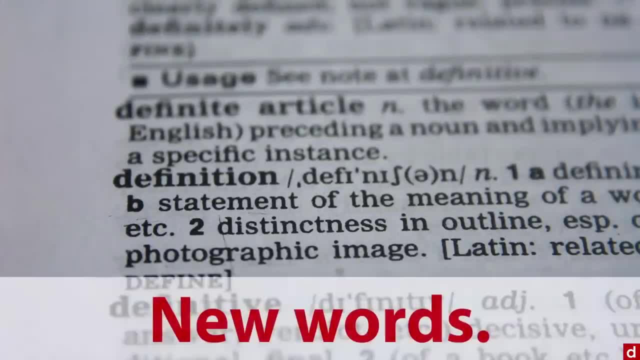 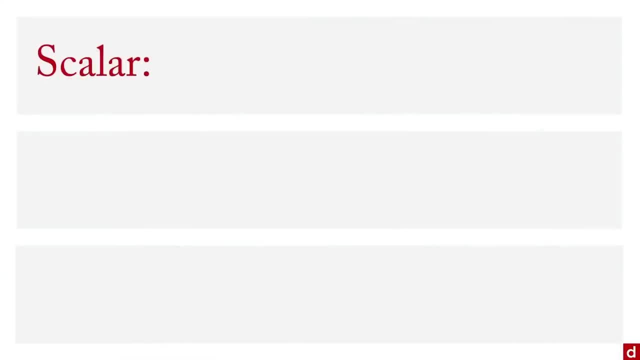 Now, before we get started with matrix algebra, we need to talk about a few new words. Maybe you're familiar with them already. The first is scalar, And this means A single number, And then a vector is a single row or a single column of numbers that can be treated as like. 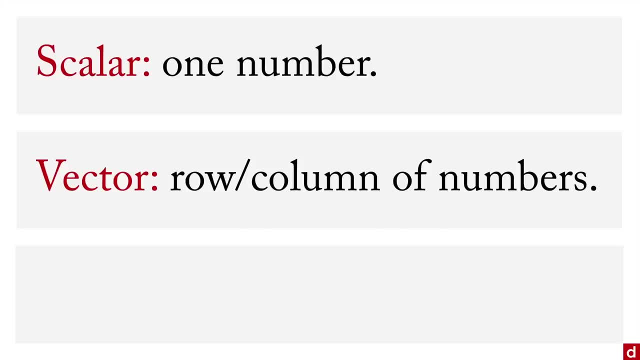 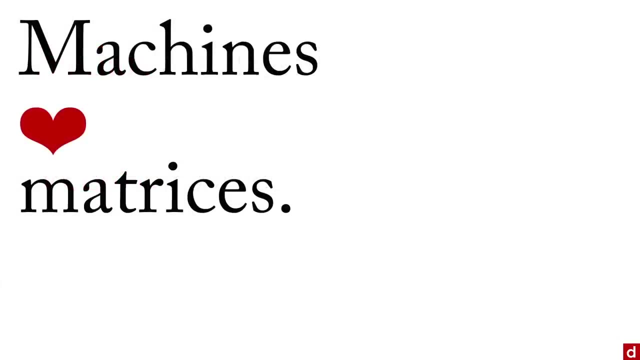 a collection. that usually means a variable. And then, finally, a matrix consists of many rows and columns, sort of a big rectangle of numbers. The plural of that, by the way, is matrices, And the thing to remember is that machines love matrices. 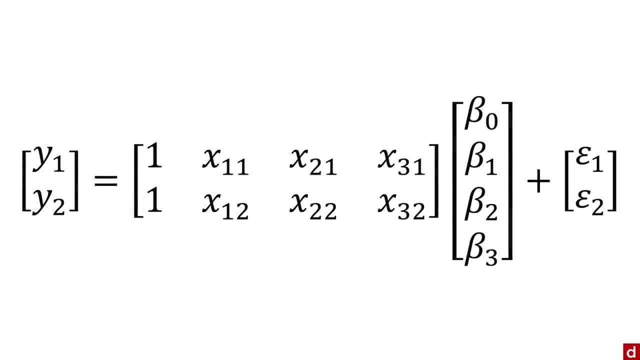 Now let's take a look at a very simple example. Here is a very basic representation of matrix algebra or linear algebra, where we're showing data on two people on four variables. So over here on the left we have the outcomes for cases one and two. are people one and two? 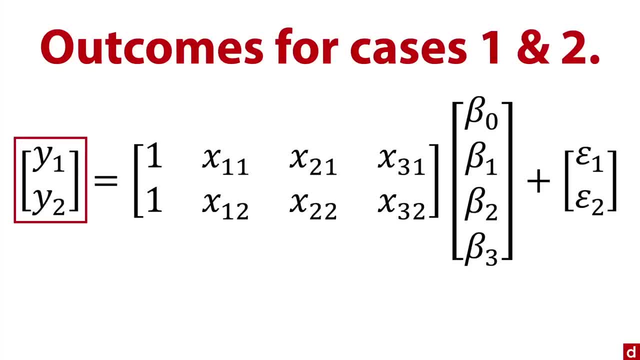 And you put them in the square brackets to indicate that it's a vector or a matrix. Here on the far left, it's a vector because it's a single column of values. And then on the left we have the outcomes for cases one and two. are people one and two? 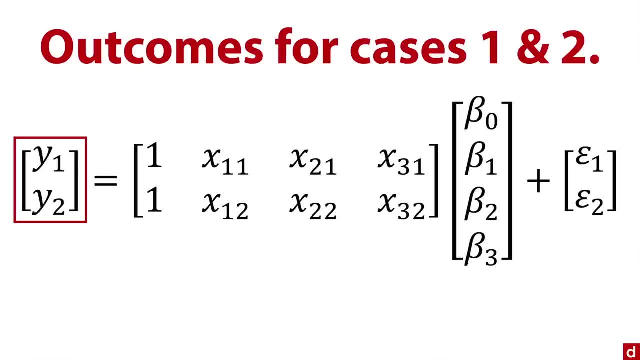 And you put them in the square brackets to indicate that it's a vector or a matrix. Next is that is a matrix that has here on the top the scores for case one, which I've written as: x is x. one as four: variable one: x twos. for variable two: 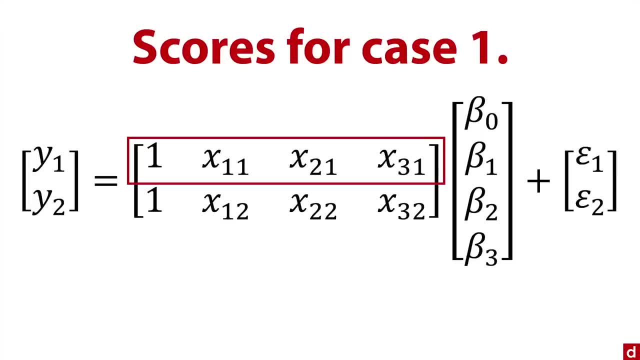 And the second subscript is indicated as per person. one Below that are the scores for case to this second person, and then over here and another vertical column are the regression coefficients. that's a beta there that we're using. then, finally, we've got a tiny little vector here at the end which contains the error terms for: 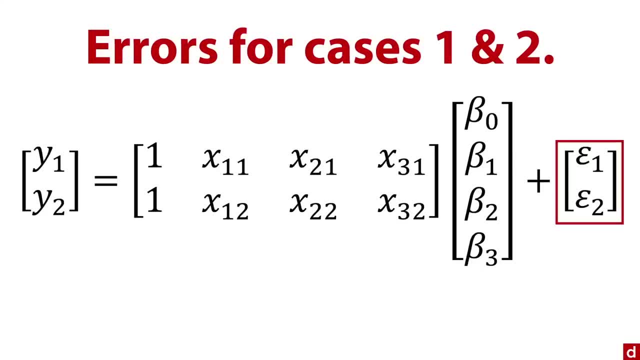 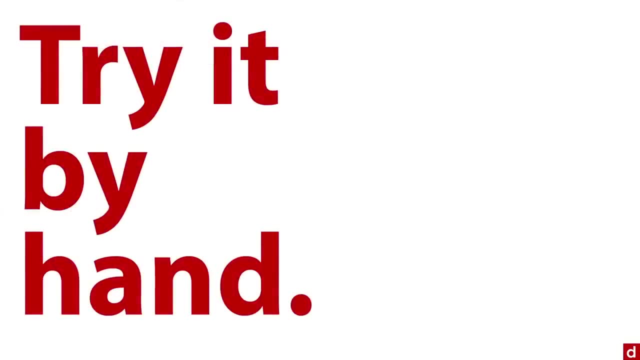 cases one and two. Now, even though you would not do this by hand, it's kind of helpful to run through the procedure, So I'm going to show it to you by hand. And we're going to take two fictional people. This will be fictional person number one. we'll call her Sophie. we'll say that she's 28. 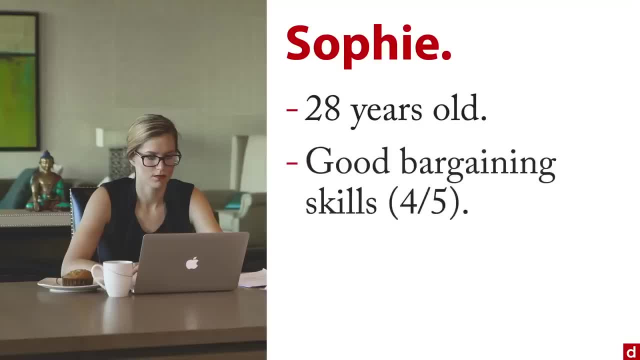 years old And we'll say that she has good bargaining skills of four on a scale of five, and that she works 50 hours a week and that her salary is 118,000.. Our second fictional person: we'll call him Lars and we'll say that he's 34 years old and he has moderate bargaining skills. 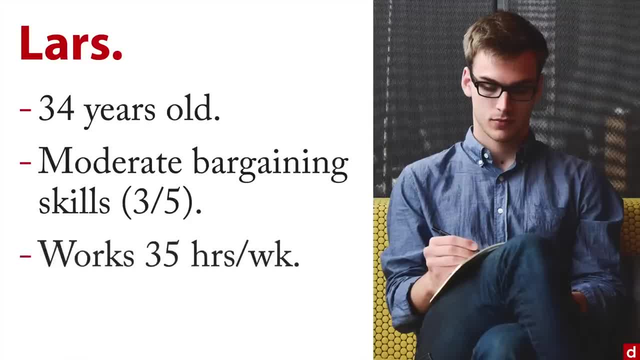 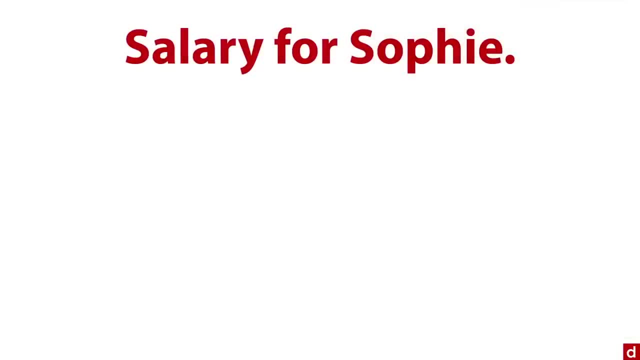 three out of five works 35 hours per week and has a salary of $84,000. And so if we're trying to look at salaries, we can go back to our matrix representation that we had here, with our variables indicated, with their Latin and English, And we can go back to our matrix representation that we had. 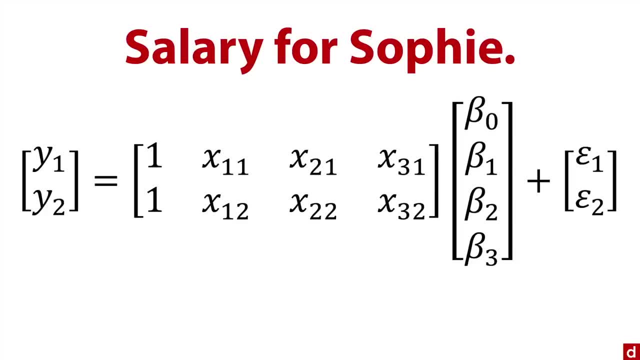 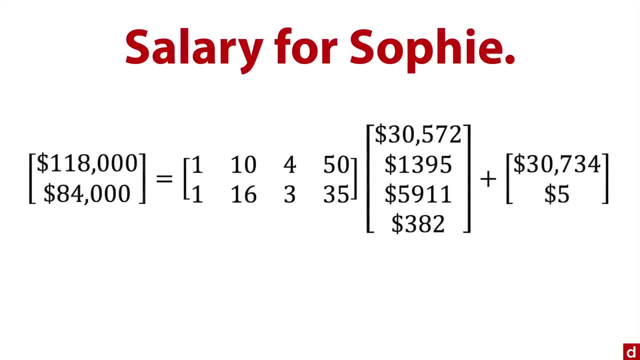 in sometimes Greek symbols, And we're going to replace those variables with actual numbers So we can get the salary for Sophie, our first person. So let me plug in the numbers here And let's start with the result here: Sophie salaries 118,000.. And here's how these numbers. 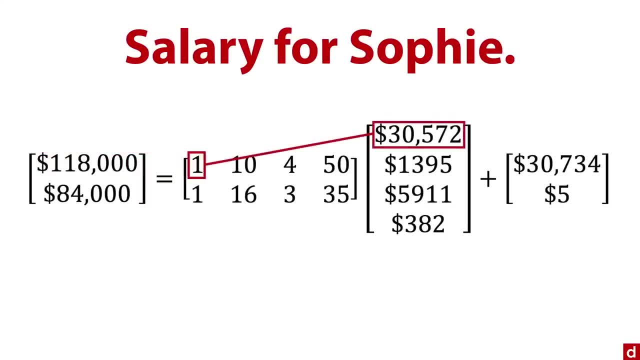 all add up to get that. The first thing here is the intercept, and we just multiply that times one, So that's sort of the starting point. And then we get this number 10, which actually has to do with years over 18.. 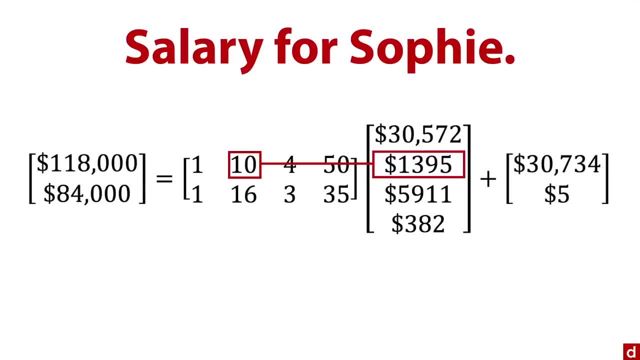 So we get this number 10, which actually has to do with years over 18.. So that's 10 years over 18, we multiply each year by 1395.. Next is bargaining skills. she's got a four out of five And for each step up you get $5,900.. By the way, these are real coefficients. 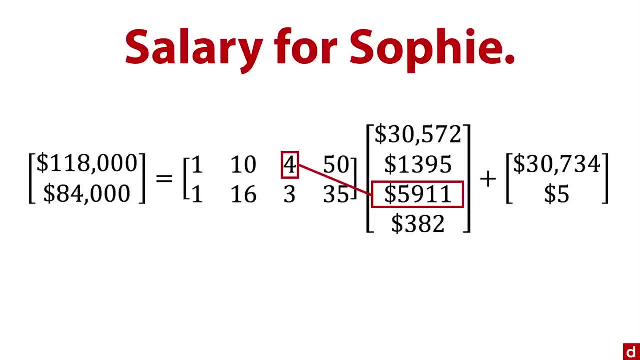 from study of survey of salary of data scientists, And then finally, hours per week. For each hour you get $382.. Now we can add those up and we can get a predicted value for her, But it's a little low. It's 30,000.. 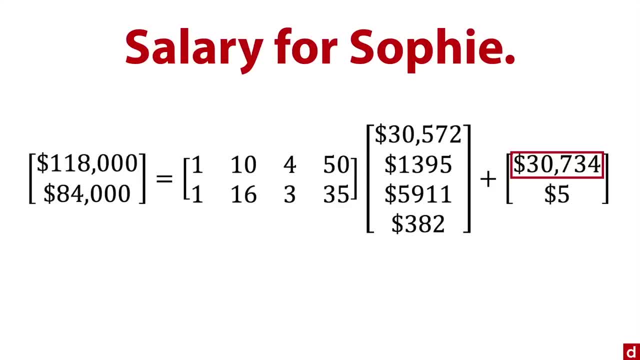 Low, which you may say: well, that's really messed up. Well, that's because there's like 40 variables in the equation, including she might be the owner. And if she's the owner, yeah she, she's going to. 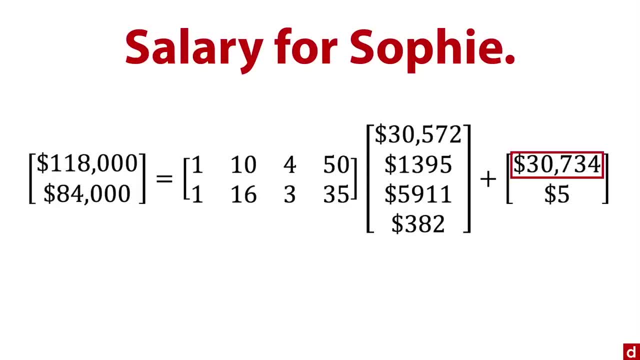 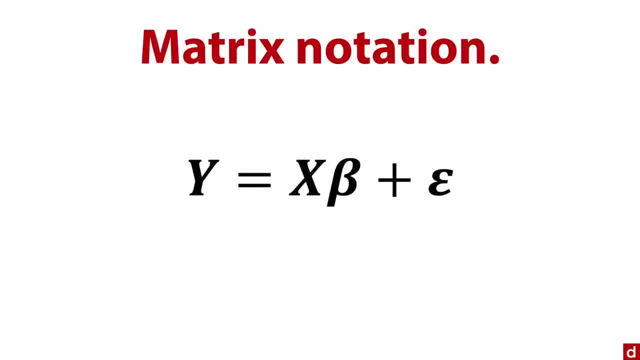 make a lot more, And then we do a similar thing for the second case. But what's neat about matrix algebra or linear algebra is that you can use matrix notation, And this means the same stuff, And what we have here are these bolded variables that stand in for entire vectors or matrices. 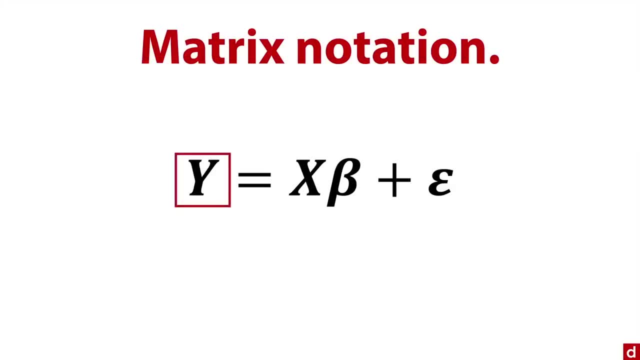 So, for instance, this y- a bold y- stands for the vector of outcome scores. This bolded x is the entire matrix of values that each person has on each variable. This bolded beta is all of the regression coefficients. And then this bolded epsilon is the entire vector of error terms. 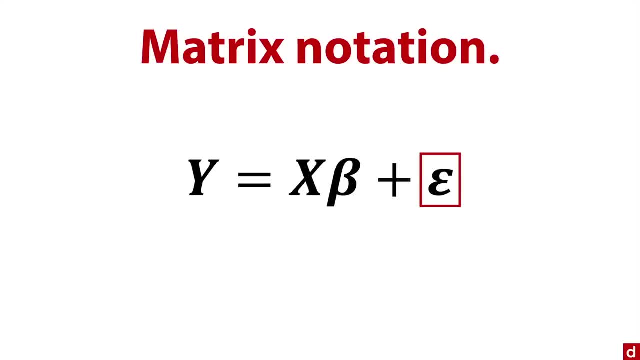 And so it's really super compact way of representing the entire collection of data and coefficients that you use in predicting values. So in some- let's say this first off- computers use matrices. they like to do linear algebra to solve problems, And it's 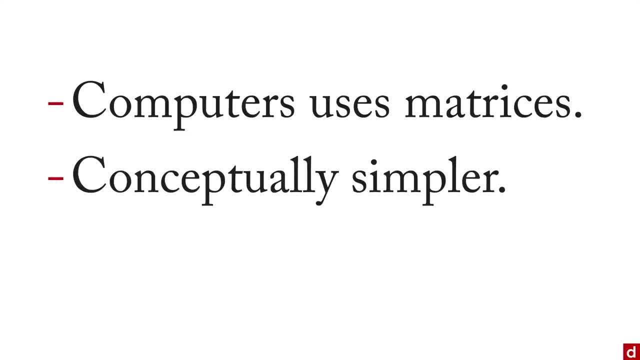 conceptually simpler because you can put it all there in this tight formation. In fact, it's a very compact notation and allows you to manipulate entire collections of numbers pretty easily, And that's the major benefit of learning a little bit about linear or matrix algebra. 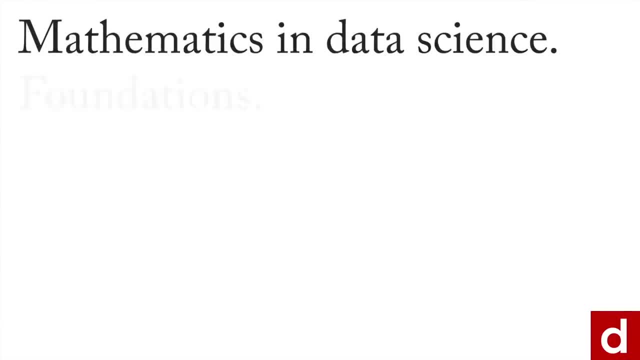 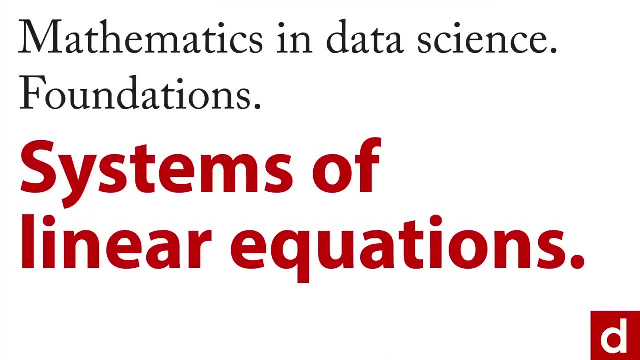 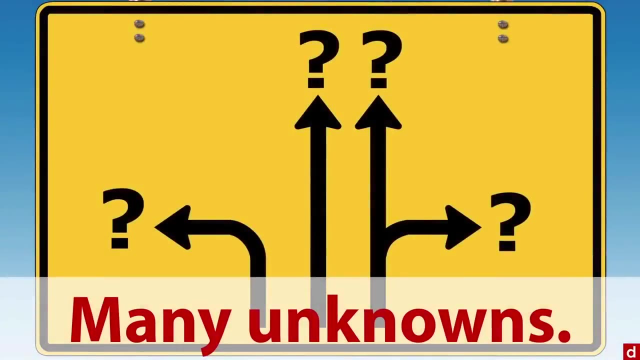 Our next step in mathematics for data science foundations is systems of linear equations, And maybe you're familiar with this, but maybe you're not. And the idea here is: there are times when you actually have many unknowns and you're trying to solve for all of them simultaneously. And what? 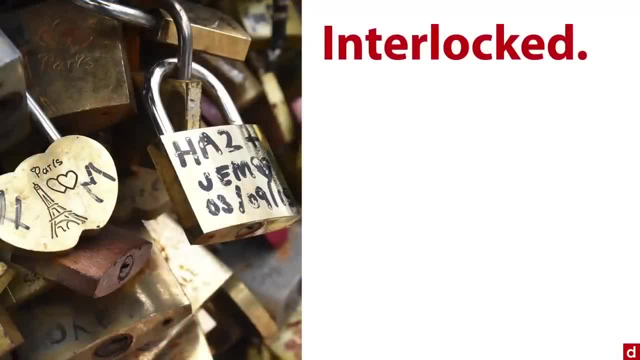 makes this really tricky, as a lot of these are interlocked. Specifically, that means x depends on y, But at the same time, y depends on x. What's funny about this is it's actually pretty easy to solve these by hand, And you can also use 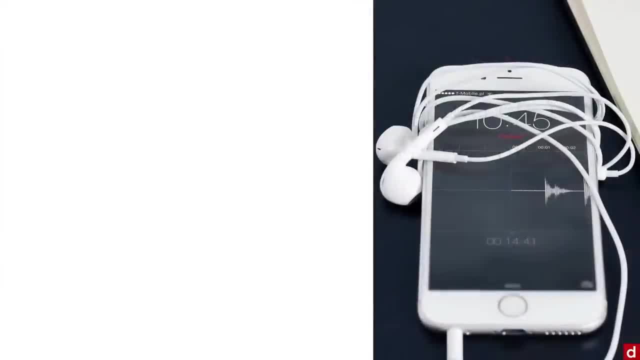 linear matrix algebra to do it. So let's take a little example here of sales. Let's imagine that you've got a company and you've sold 1000 iPhone cases- so they're not running around naked like in this picture- And that some of the cases sold for $20 and others sold for $5. You made a total. 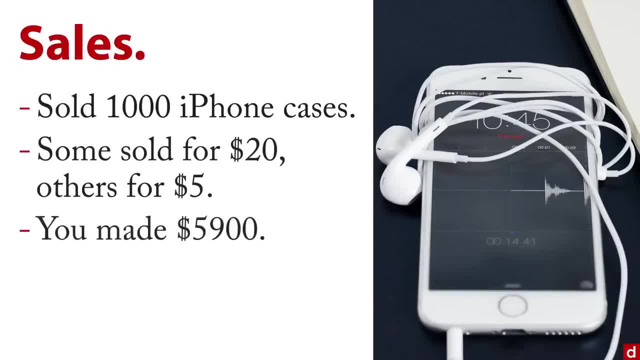 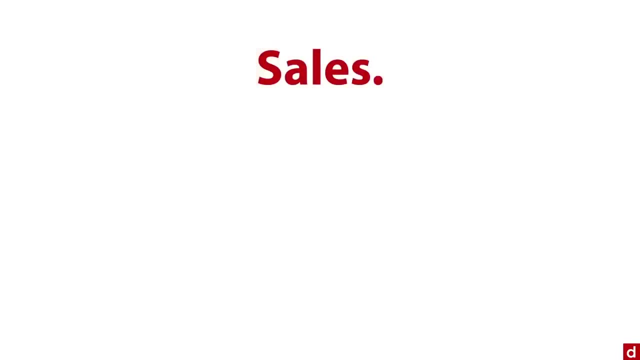 of $5,900. And so the question is how many were sold at each project? And so you've got a company and you've got a price. Now, hopefully you were keeping your records, But you can also calculate it from this little bit of information. And to show you, I'm going to do it by hand. Now we're. 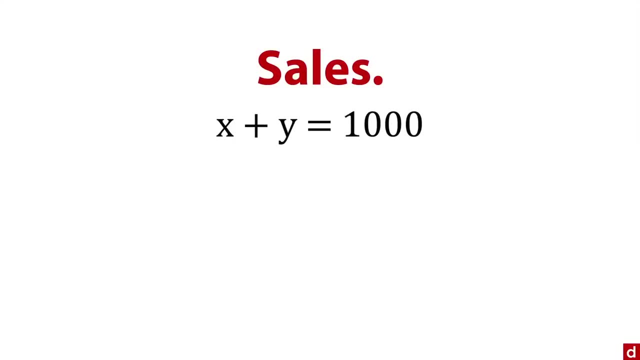 going to start with this. we know that sales- the two price points x and y add up to 1000 total cases sold. And for revenue, we know that if you multiply a certain number times $20, and another number times $5,000, you create a separate number. So between the two of those we can figure out the. 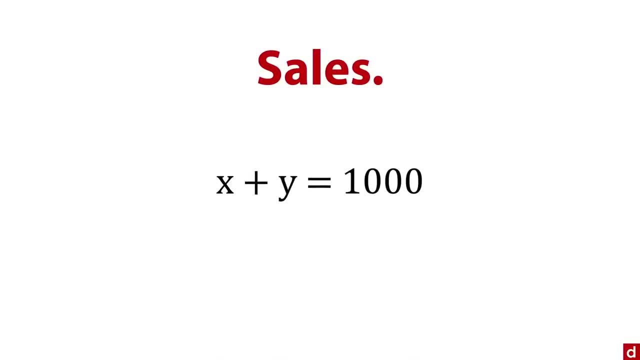 rest, Let's start with sales. Now, what I'm going to do is I'm going to try to isolate the values, And I'm going to do that by putting in this minus y on both sides, And then I can take that and I can. 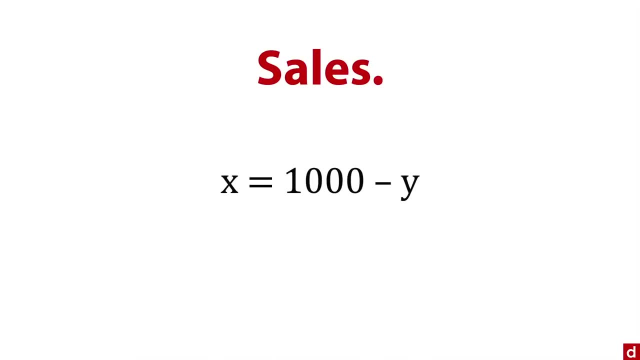 subtract it, so I'm left with: x is equal to 1000 minus y. Normally you solve for y, but I solve for x. you'll see why in just a second. Then we go to revenue And we know from earlier that our sales at 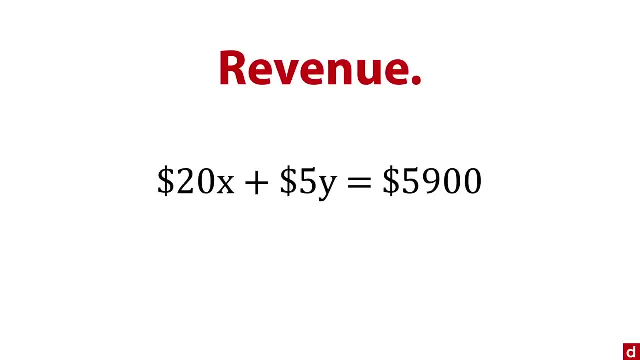 sales of these two price points add up to $5,900 total. Well, what we're going to do is we're going to take this x- that's right here- and we're going to replace it with the equation we just got, which is 1000 minus y. then we multiply that through and we get 20,000 minus 20 y plus five y. 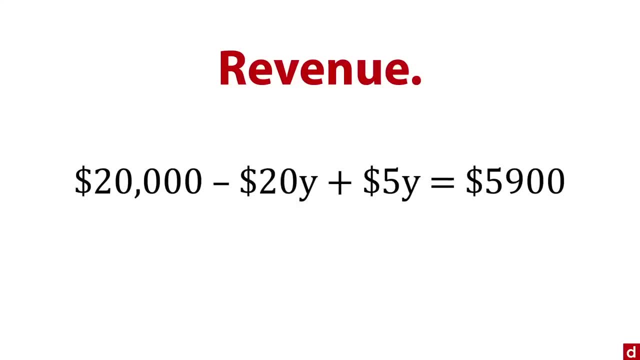 equals 5900.. Well, we can subtract these two because they're on the same thing. So 20 y and we get 15 y, and then we subtract 20,000 from both sides. So there it is right, there on the left. 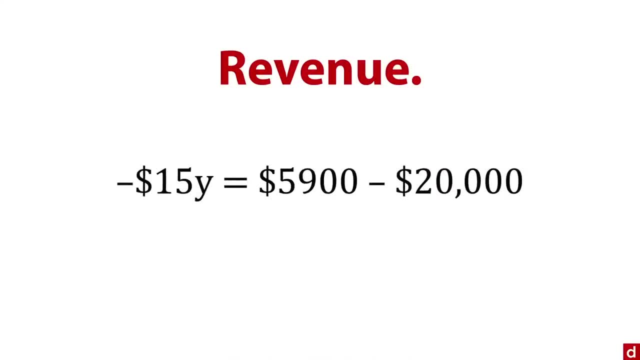 And that disappears. And then I get it over on the right side And I do the math there and I get minus $14,100.. Well then I divide both sides by negative $15. And when we do that we get: y is equal to 940.. Okay, so that's one of our values for 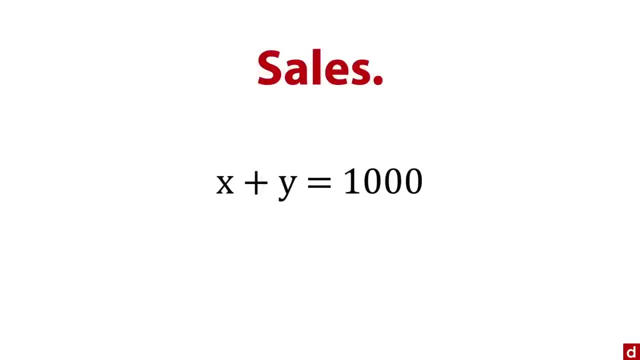 sales. So let's go back to sales. we have: x plus y equals 1000.. We take the value that we just got, 940, we stick that into the equation And then we can solve for x. just subtract 940 from each side. 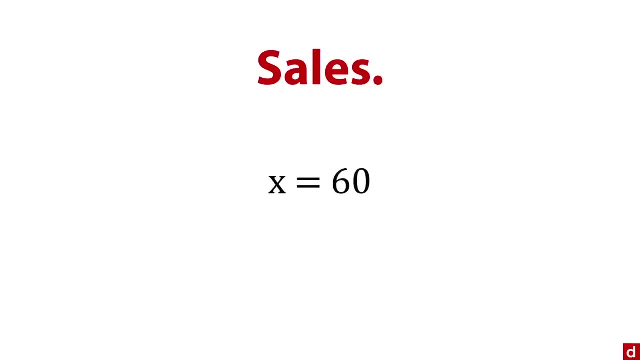 there we go, we get. x is equal to 60. So let's put it all together Just to recap what happened. What this tells us is that 60 cases were sold at $20 each and that 940 cases were sold at $5 each. 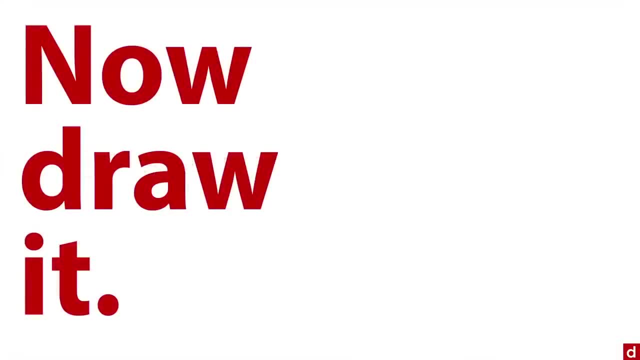 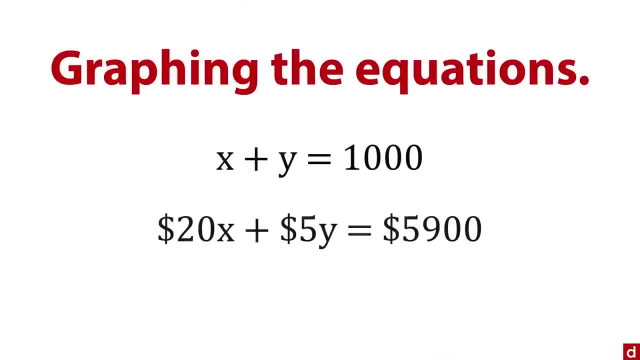 Now, what's interesting about this is: you can also do this graphically. we're going to draw it, So I'm going to graph the two equations. Here are the original ones we had. this one predicts sales. this one gives price. The problem is, these really aren't in the canonical form for creating graphs. 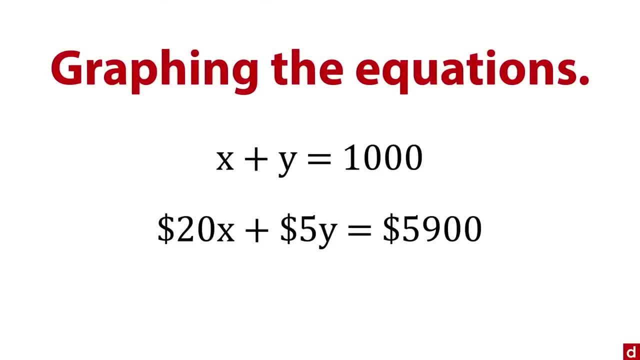 that needs to be. y equals something else. So we're going to solve both of these. for y, we subtract x from both sides- there it is on the left. we subtract that and then we have y is equal to minus x plus 1000.. That's something that we can graph. 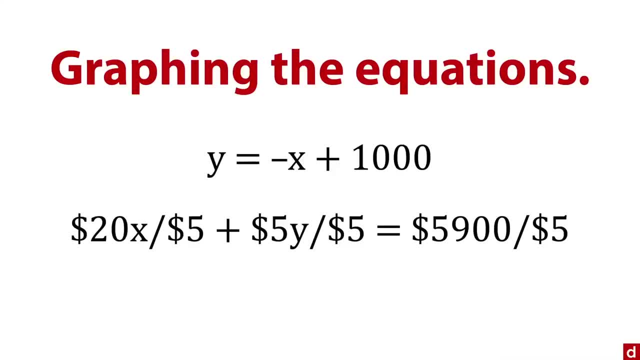 Then we do the same thing for price. Let's divide by five all the way through. that gets rid of that. And then we've got this four x, and then let's subtract four x from each side, And what we're left with is minus four x, plus 1180.. That's also something that we can graph. 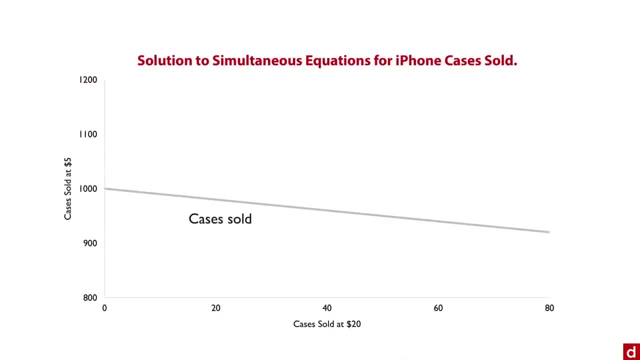 So here's the first line. this indicates cases sold. It originally said: x plus y equals 1000. But we rearrange it to: y is equal to minus x plus 1000.. 1000. And so that's the line we have here. And then we have another line which indicates earnings. 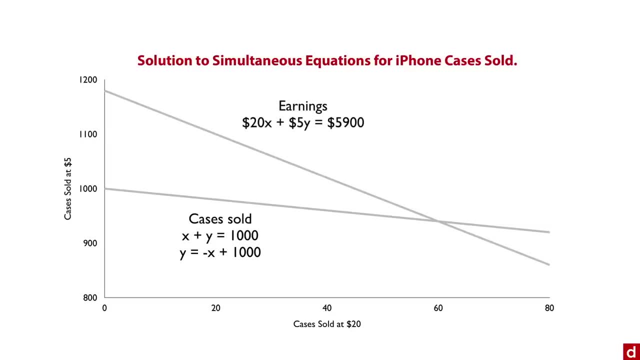 And this one was originally written as: $20 times x plus $5 times y equals $5,900 total. we rearrange that to y equals minus four, x plus 1180.. That's the equation for the line, And then the solution is right. here at the intersection, There's our intersection. 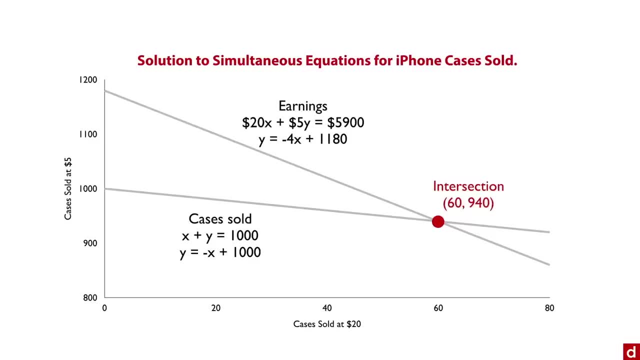 and it's at 60 on the number of cases sold at $20 and 940 on the number of cases sold at $5.. And that also represents the solution of these joint equations, And so it's a graphical way of solving a system of linear equations. So, in sum, systems of linear equations allow us to. 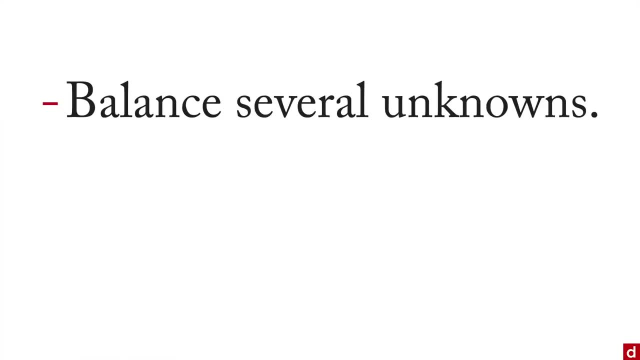 balance several unknowns and find the unique solution, And in many cases it's easy to solve by hand And it's really easy with linear algebra when you use software to do it. at the same time As we continue our discussion of mathematics and data science and the foundational principles, 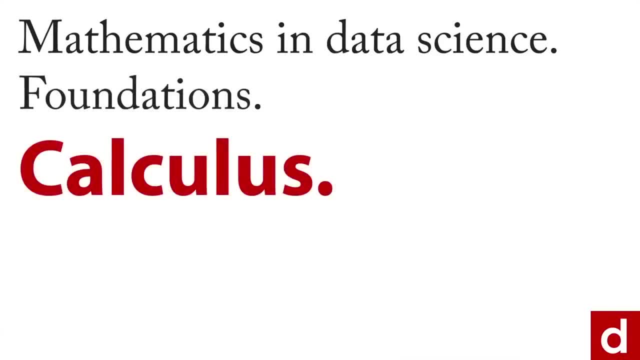 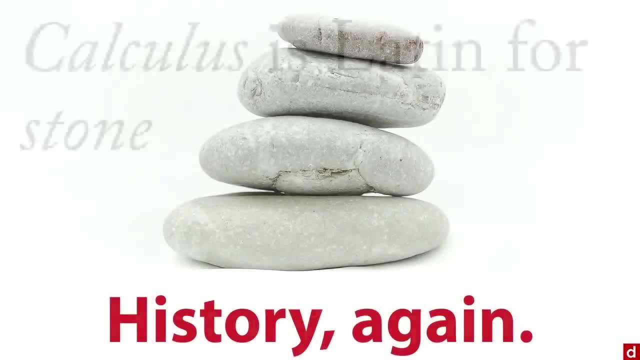 the next thing we want to talk about is calculus, And I'm going to give a little more history right here. The reason I'm showing you pictures of stones is because the word calculus is Latin for stone, as in a stone used for tallying, where people would actually have a little bag of stones. 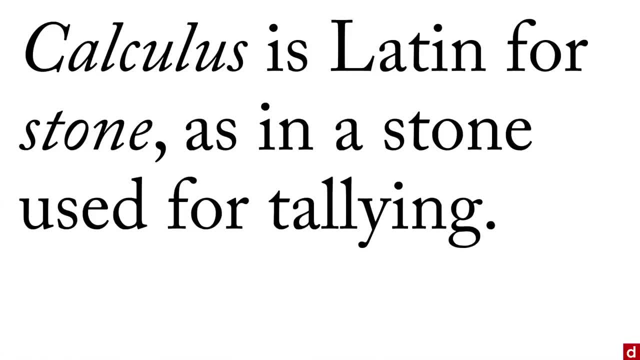 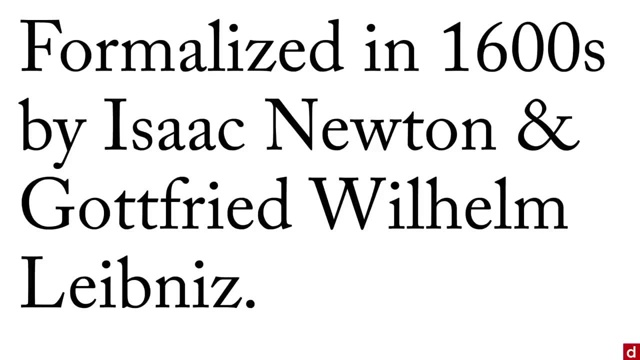 and they would move them, and they would use it to count stones. And the system of calculus was formalized in the 1600s simultaneously independently by Isaac Newton and Gottfried Wilhelm Leibniz. And there are three reasons why calculus is important for 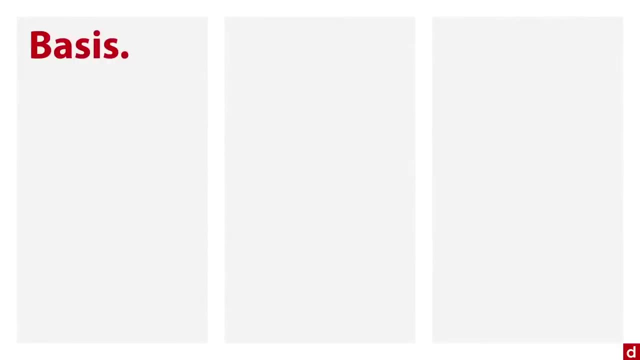 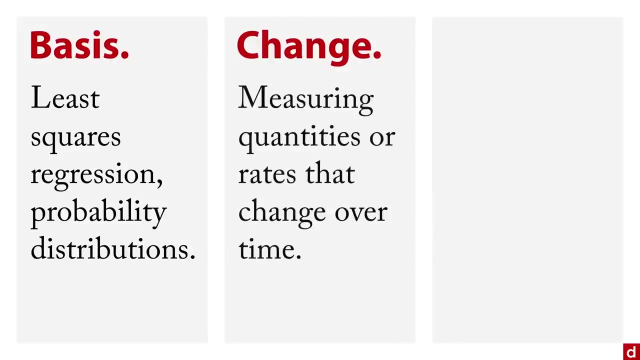 data science. Number one: it's the basis of most of the procedures that we do, Things like least squares, regression and probability distributions. They use calculus in getting those answers. Second one is if you're studying anything that changes over time, so if you're measuring quantities or rates that change over time, then you have to use calculus. 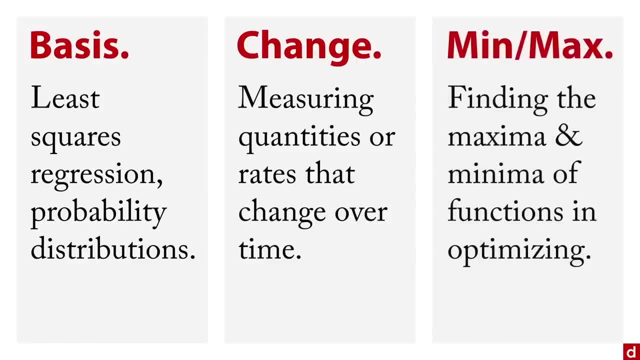 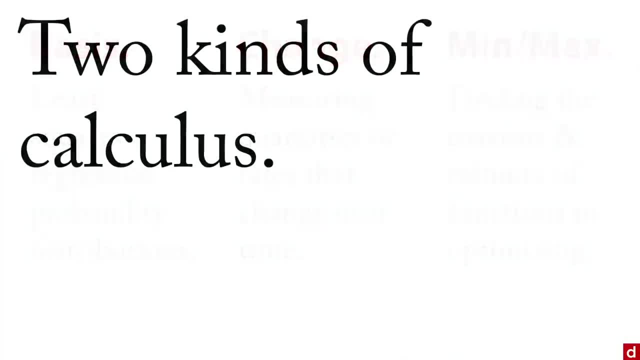 Calculus is used in finding the maximum and the minimum of functions, especially when you're optimizing, which is something I'll show you separately. Also, it's important to keep in mind there are two kinds of calculus. The first is differential calculus, which talks about rates of 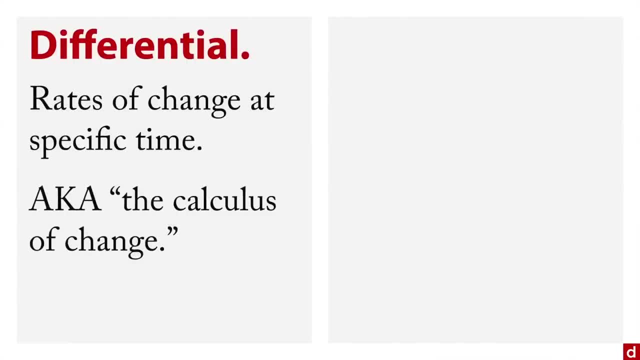 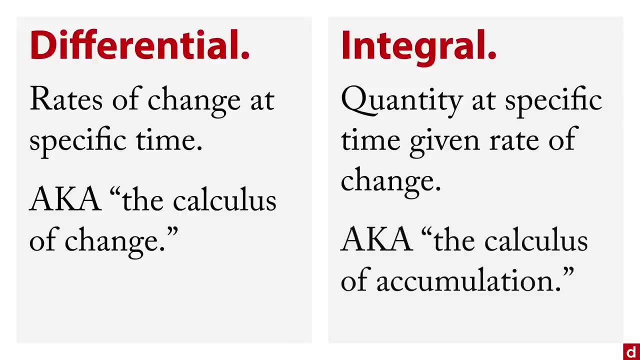 change at a specific time. It's also known as the calculus of change. The second kind of calculus is where you're trying to calculate the quantity of something at a specific time, given the rate of change, And it's also known as the calculus of accumulation. So let's take a look at how this. 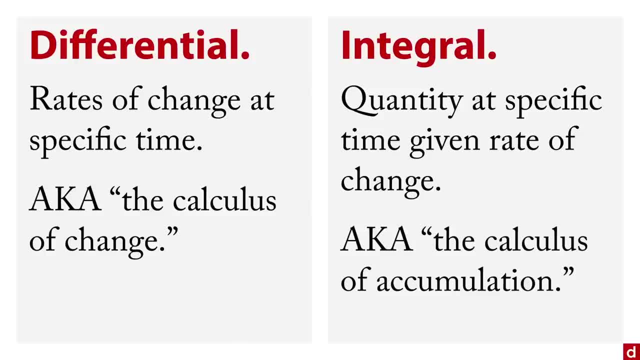 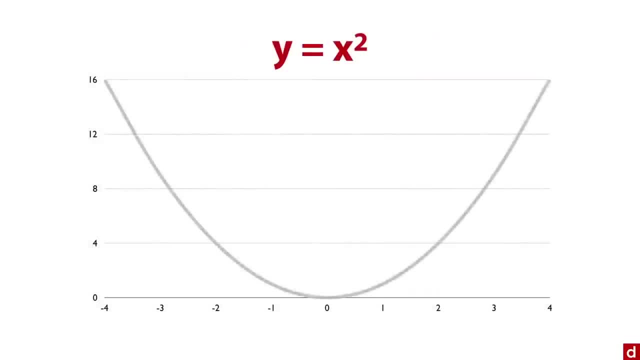 works And we're going to focus on differential calculus. So I'm going to graph an equation here. I'm going to do: y is equal to x squared, a very simple one. But it's a curve which makes it harder to calculate things like the slope. So let's take a point here that's at minus. 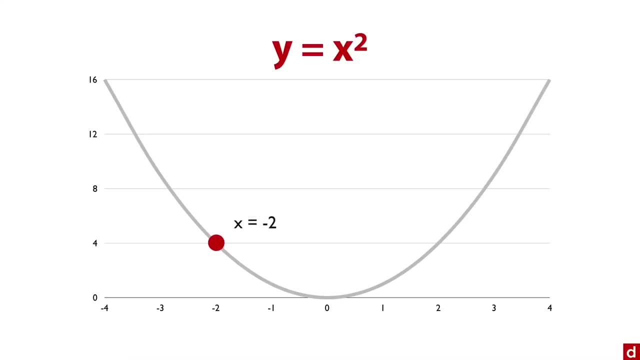 two. that's my little red dot we have at. x is equal to minus two, And because y is equal to x squared, if we want to get the y value all we got to do is take that negative two and square and that gives us four. So that's pretty easy. So the coordinates for that red point are minus two on x. 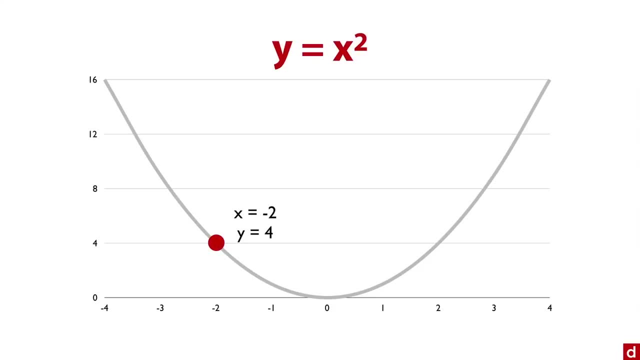 and plus four on y. Here's a harder question: What is the slope of the curve at that exact point? Well, it's actually a little tricky because the curve is always curvy and there's no flat part on it, But we can get the answer by getting the derivative of the function. Now there are several. 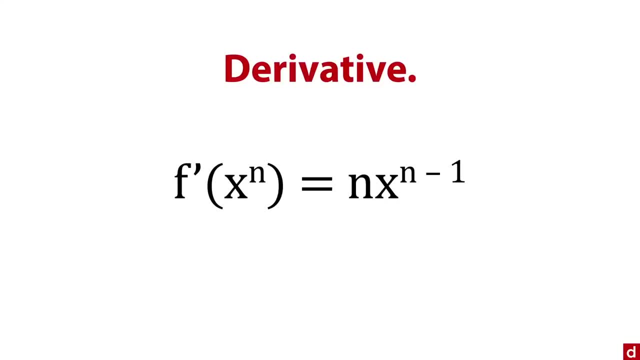 different ways of writing this. I'm using the one that's easiest to type. And let's start by this. what we're going to do is the n here And that is the squared apart. So we had x squared And you see that same n turns into the squared, And then we come over here and we put that same value. 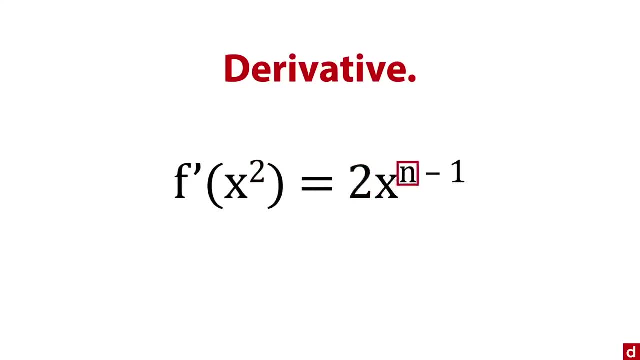 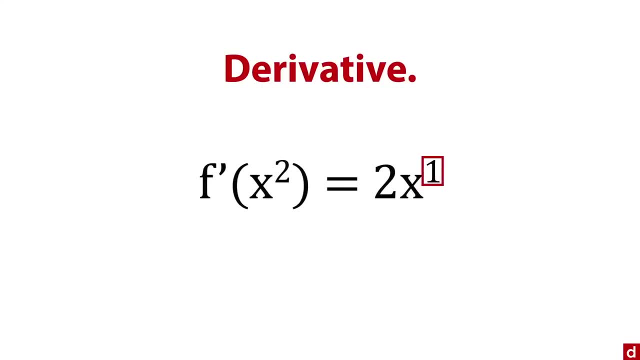 And then we come over here and we put the two in right here, And then we come over here and we can do a little bit of subtraction: two minus one is one And truthfully you can just ignore that and you get two x. that is the. 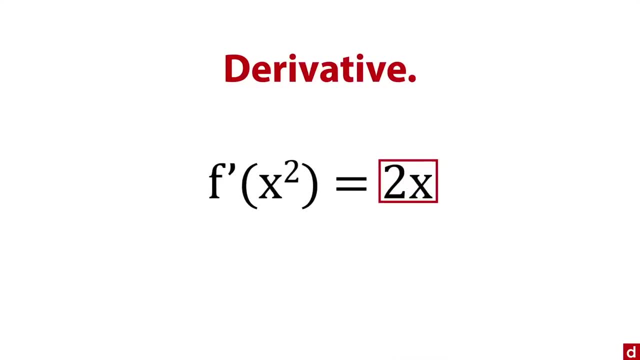 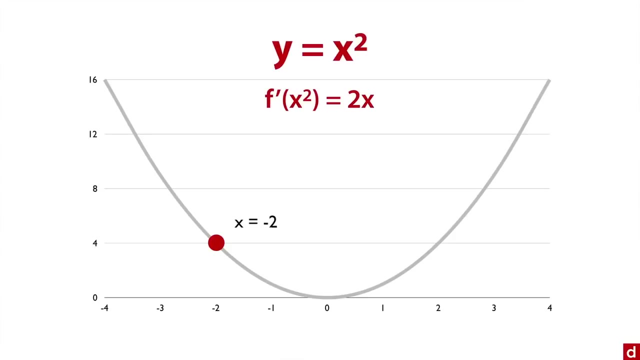 derivative. So what we have here is the derivative of x squared is two x. That means the slope at any given point of the curve is two x. So let's go back to what we had a moment ago. Here's our curve, Here's our point at x minus two, And so the slope is equal to two x. Well, we put in the minus two. 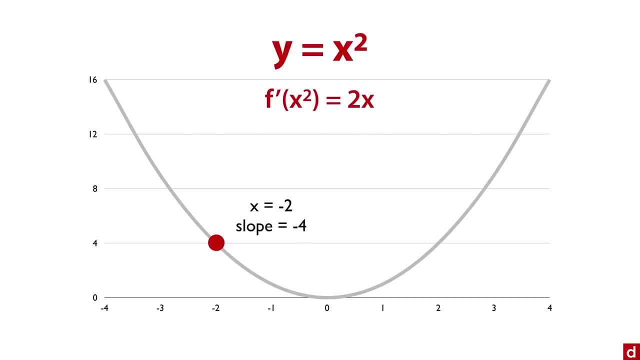 and we multiply it and we get minus four. So that is the slope at this exact point on the curve. Okay, what if we choose a different point? let's say we come over here to x is equal to three, all the slopes equal to two x. 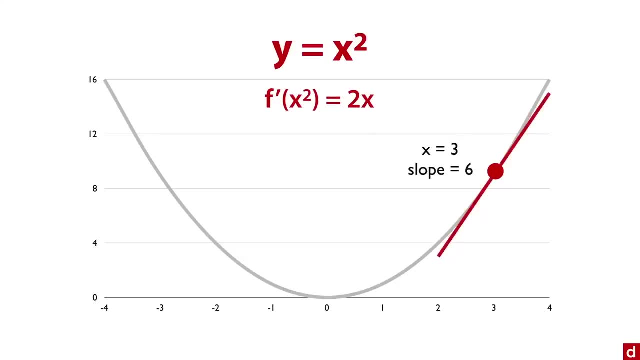 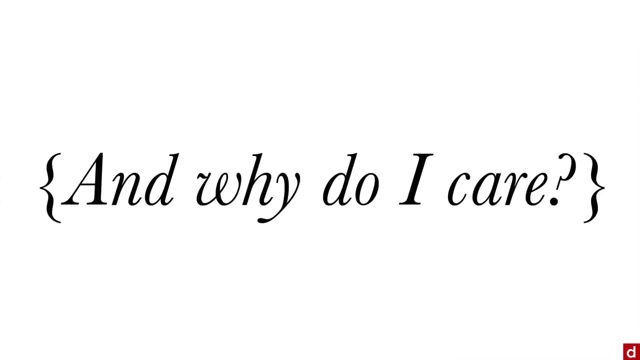 So that's, two times three is equal to six, Great. And on the other hand, you might be saying to yourself: and why do I care about this? There's a reason that this is important, And what it is is that you can use these procedures to optimize decisions. 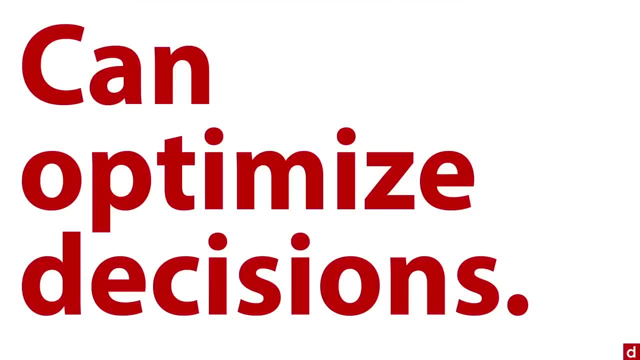 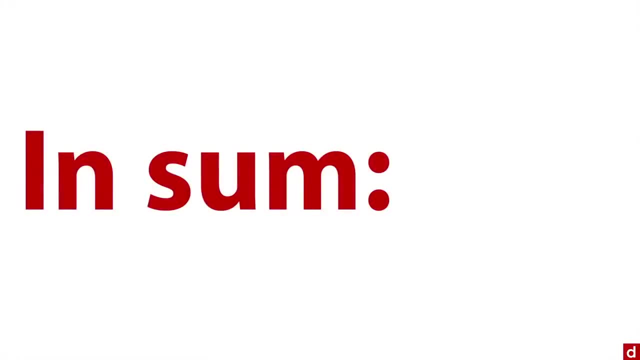 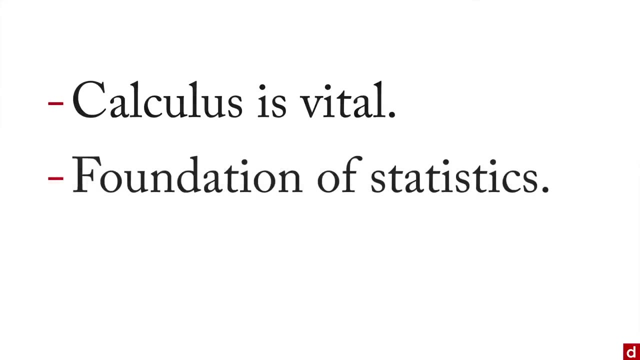 And if that seems a little too abstract to you, that means you can use them to make more money, And I'm going to demonstrate that in the next video. But for right now, in sum, let's say this calculus is vital to practical data science. It's the foundation of statistics and it forms the 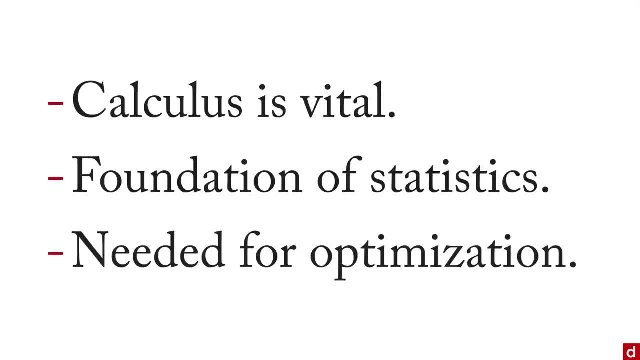 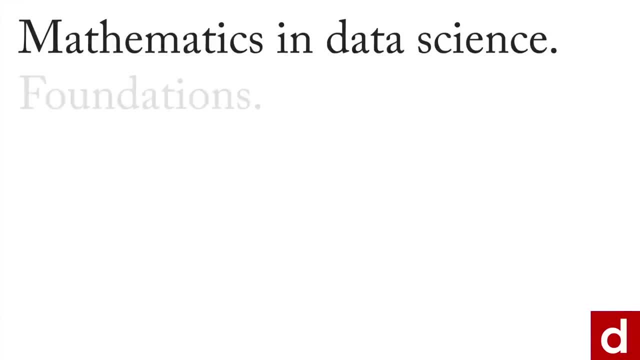 core that's needed for doing optimization. In our discussion of mathematics and data science foundations. the last thing I want to talk about today is how to optimize data science. So let's go ahead and get started. So let's go ahead and get started. So let's go ahead and get started. So let's. 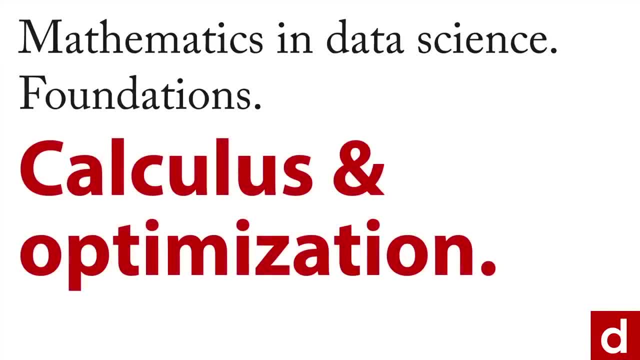 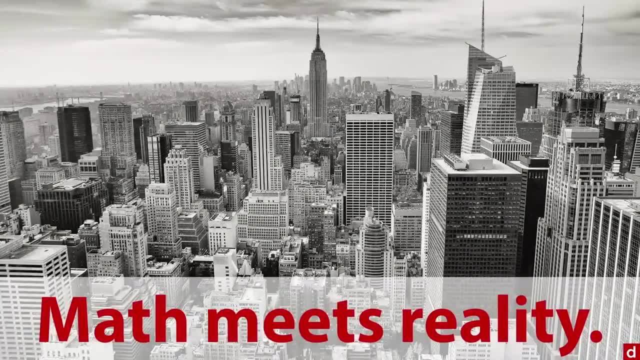 talk about right here is calculus and how it relates to optimization. I'd like to think of this, in other words, as the place where math meets reality, or it meets Manhattan, or something. Now, if you remember this graph I made in the last video, y is equal to x squared. 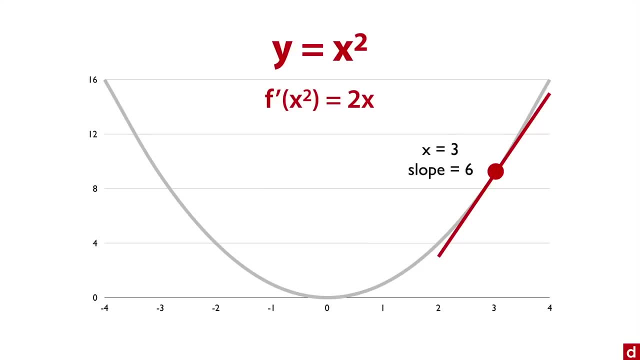 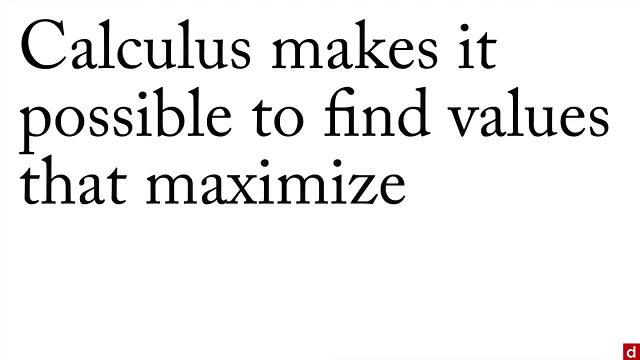 that shows this curve here, and we have the derivative that the slope can be given by two- x- And so when x is equal to three, the slope is equal to six. fine, And this is where this comes into play. Calculus makes it possible to find values that maximize or minimize outcomes, And 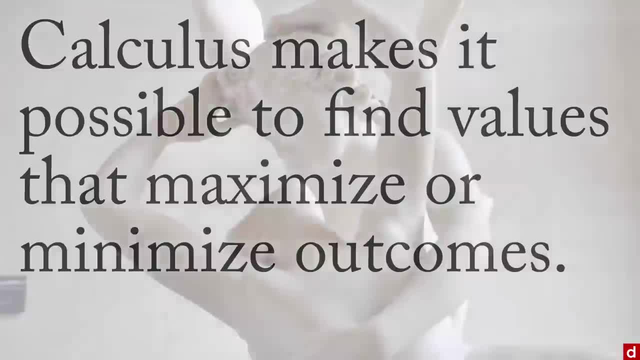 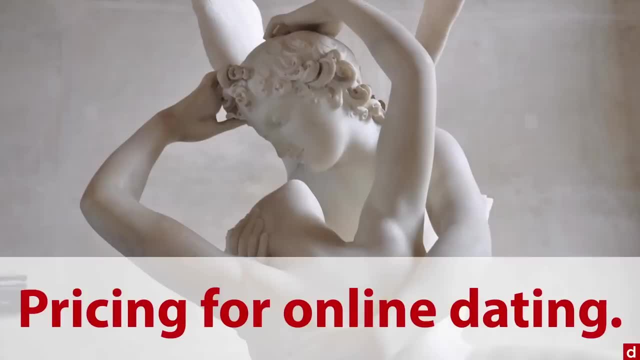 if you want to make something a little more concrete out of this, let's think of an example here. By the way, that's Cupid and psyche. Let's talk about pricing for online dating. Let's assume you've created a dating service and you want to figure out. 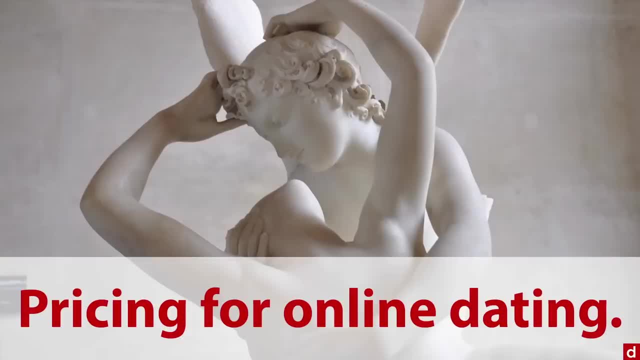 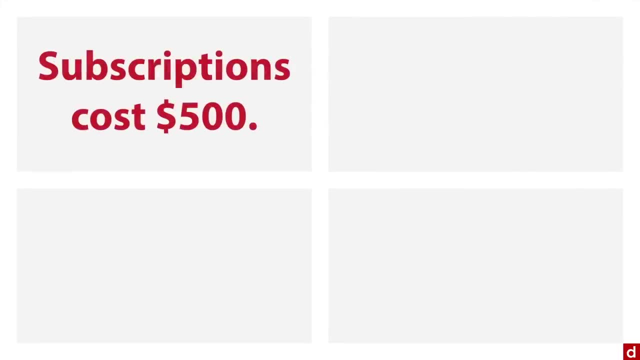 how much can you charge for it? that will maximize your revenue. So let's get a few hypothetical parameters. So let's get a few hypothetical parameters. So let's get a few hypothetical parameters involved. First off, let's say that subscriptions, annual subscriptions, currently, 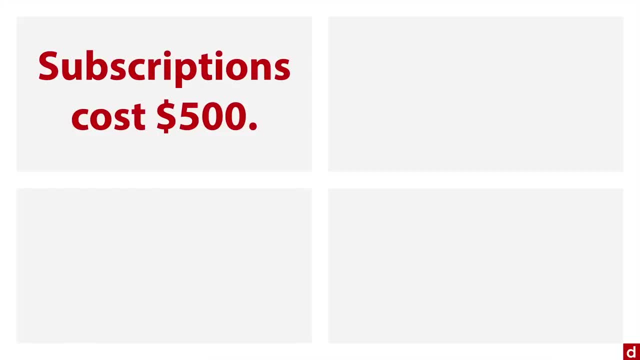 costs $500 a year And you can charge that for a dating service. And let's say you sell 180 new subscriptions every week. On the other hand, based on your previous experience manipulating prices around, you have some data that suggests that for each $5, you discount from the price of 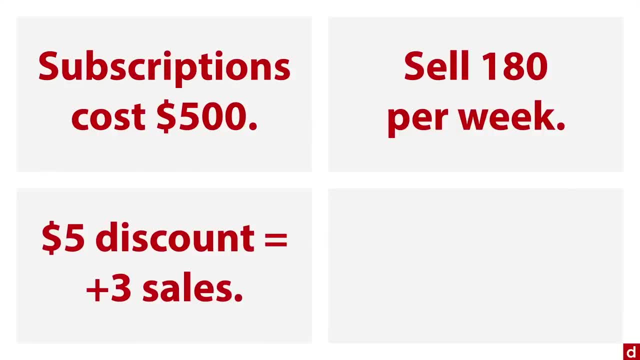 $500, you will get three more sales, Also because it's an online service. let's say you've created a dating service, And let's say you've created a dating service. And let's say you've created a dating service And let's say you've created a dating service. Let's just 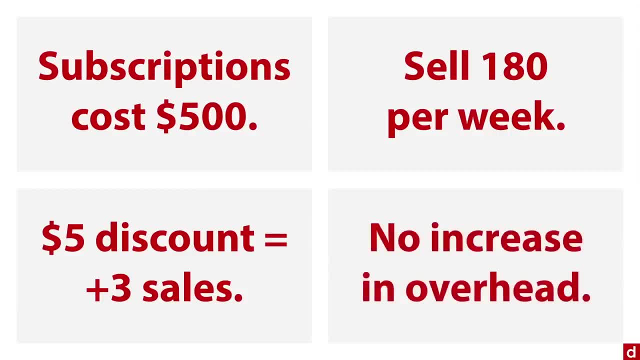 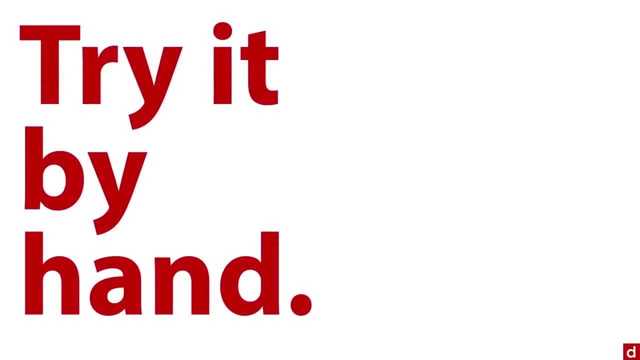 make our lives a little simpler right now and assume that there is no increase in overhead. It's not really how it works, but we'll do it for now, And I'm actually going to show you how to do all this by hand. Now let's go back to price. First we have this: $500 is the current annual. 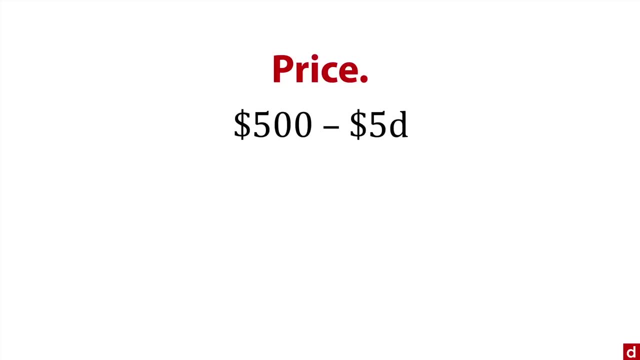 subscription price And you're going to subtract $5 for each unit of discount. That's what I'm giving D, So one discount is $5, two discounts is $10, and so on. And then we have a little bit of data about sales: that you're currently selling 180 new subscriptions per week and that you will. 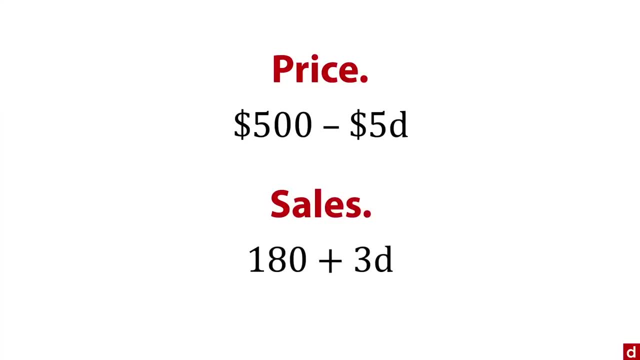 add three more for each unit of discount that you give. So what we're going to do here is we're going to find sales as a function of price. Now, to do that, the first thing we have to do is get the y intercept. So we have price here. $500 is the current annual subscription price minus $5 times D. 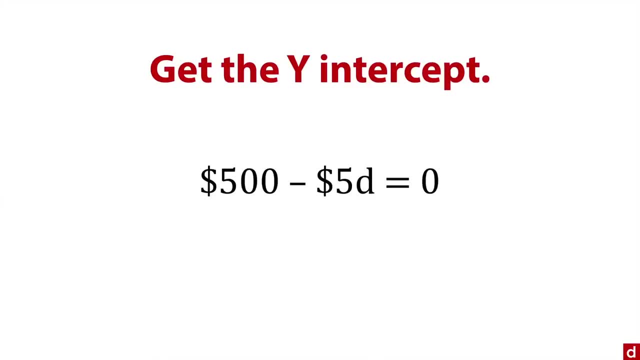 And what we're going to do here is we're going to add three more for each unit of discount. We're going to do is we're going to get the y intercept by solving when does this equals zero. Okay, well, we take the 500, we subtract that from both sides And then we end up with minus five D. 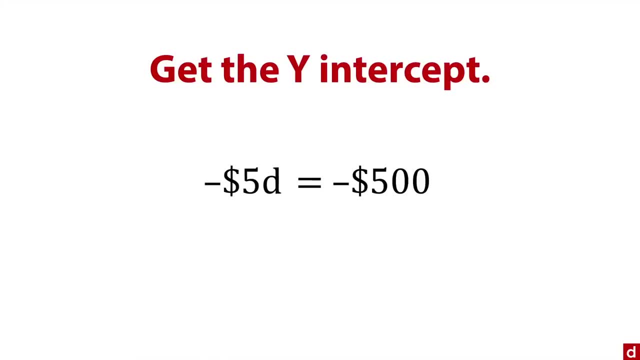 is equal to minus 500.. Divide both sides by minus five and we're left with D is equal to 100. That is when D is equal to 100, x is zero, And that tells us how we can get the y intercept. But to: 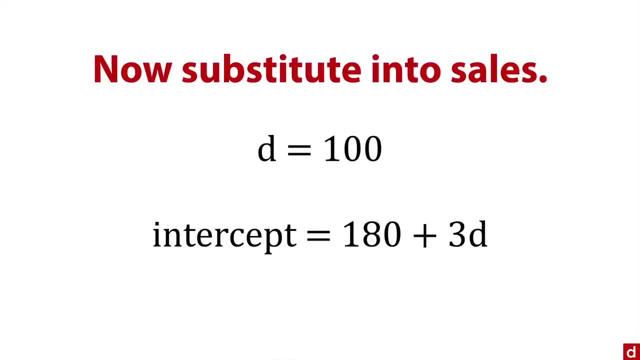 get that we have to substitute this value, And that's what we're going to do here. we're going to substitute this value into sales. So we take, D is equal to 100. And the intercept is equal to 180 plus 3,. 180 is the number of new subscriptions per week. And then we take the three, and then we 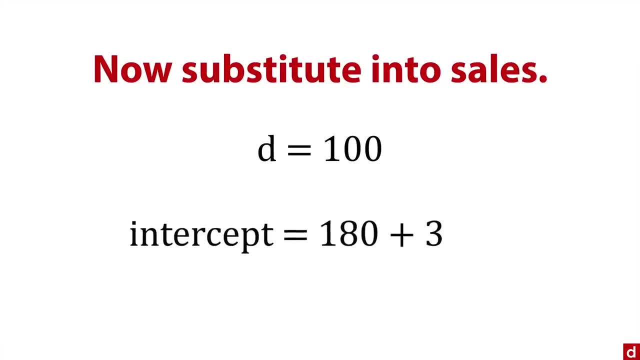 multiply that times our 100. So 180 times three times 100 is equal to 300. Add those together and you get 480. And that is the y intercept in our equation. So when we've discounted sort of price to zero when price is zero, then we've discounted the price to zero When price is zero. 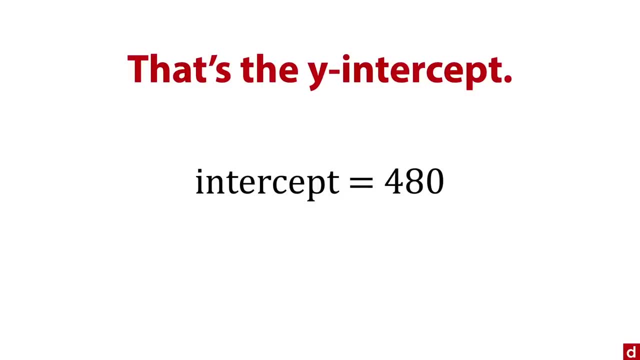 then the expected sales is 480.. Of course, that's not going to happen in reality, But it's necessary for finding the slope of the line. And so now let's get the slope. the slope is equal to the change in y on the y axis divided by the change in x. One way we can get this is by looking at sales. 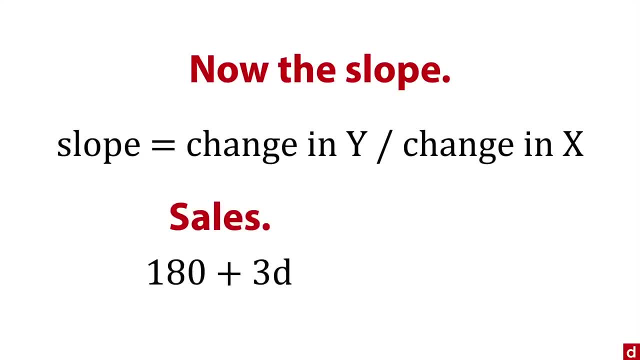 we get our 180 new subscriptions per week, plus three for each unit of discount, And we take our information on price- $500 per year minus $5 for each unit of discount- And then we take these, the 3d and the 5d, and those will give us the slope. So it's plus three divided by minus five, and that's. 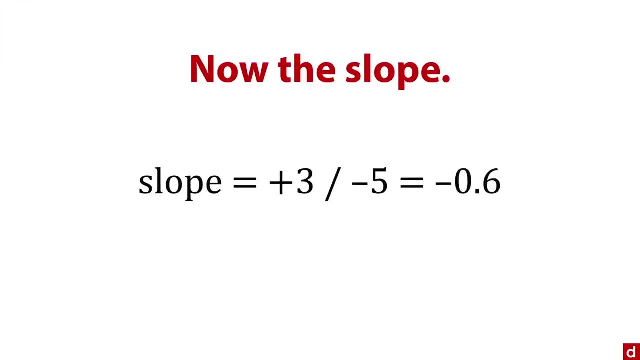 just minus point six. And so that is the slope of the line. slope is equal to minus 0.6.. And so what we have from this is sales as a function of price where sales is equal to 480.. Because that's the y intercept. When x is equal to zero, when price is zero minus 0.6 times price. 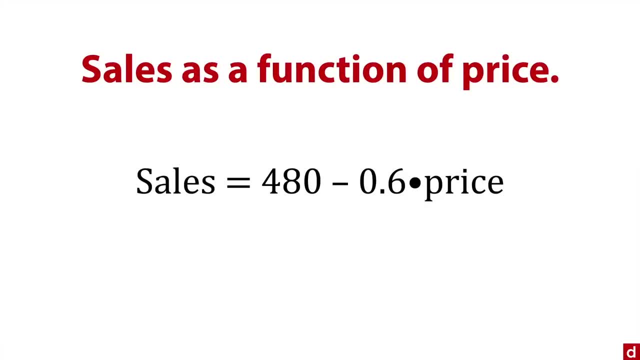 So this isn't the final thing. Now. what we have to do is we turn this into revenue. So there's another stage to this. Now revenue is equal to sales time, the price. you know how many things did you sell And how much did it cost? Well, we can substitute in some information here If we 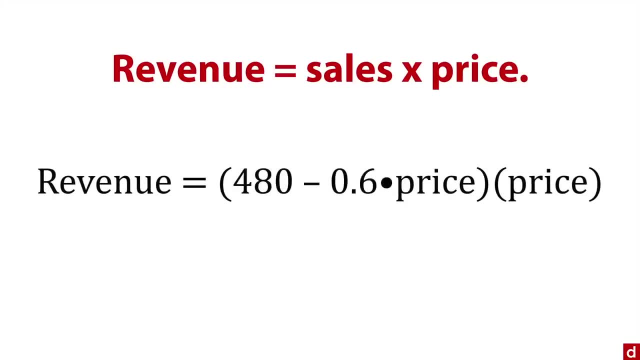 take sales and we put it in as a function of price, because we just calculated that a moment ago. we get this and then we do a little bit of multiplication and then we get that revenue is equal to 480 times the price minus 0.6 times the square of the price. Okay, 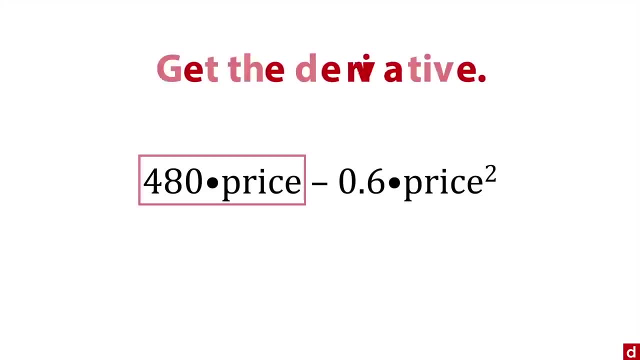 that's a lot of stuff going on there. What we're going to do now is we're going to get the derivative- that's the calculus that we talked about- Well, the derivative of 48 in the price. where price is sort of the x, the derivative is simply 480. And the minus zero. 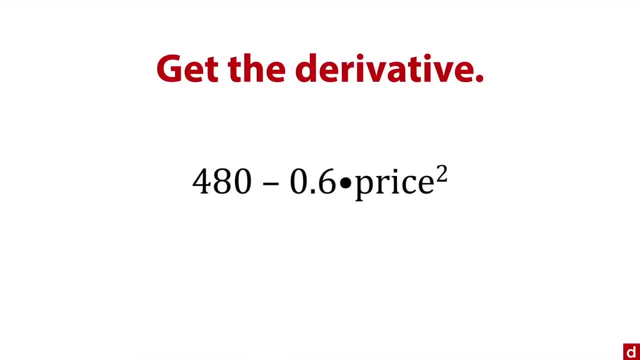 point six times the square of the price. Well, that's very similar to the thing we did with the curve, And what we end up with is 0.6 times two is equal to 1.2 times the price. This is the. 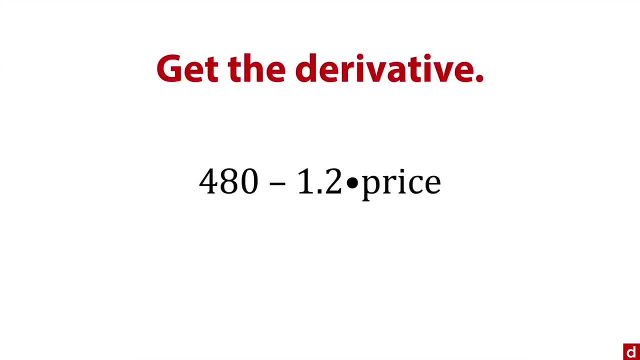 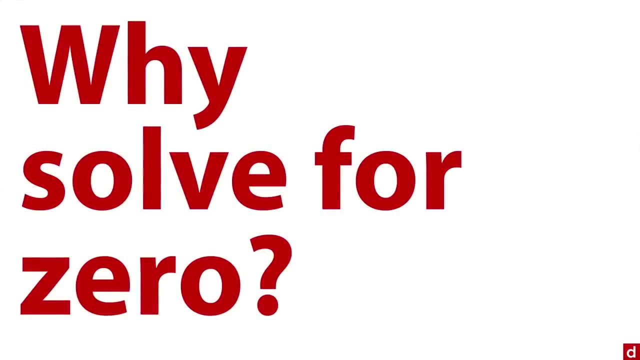 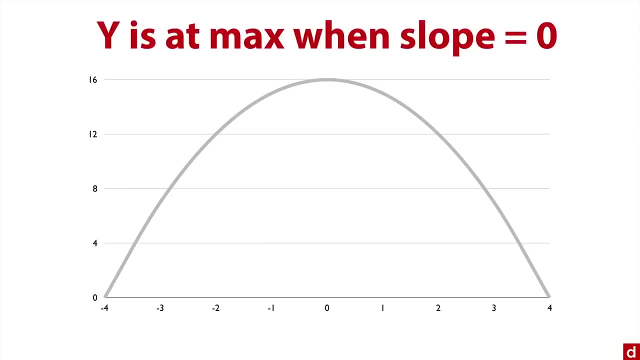 derivative of the original equation. we can solve that for zero. now, And just in case you're wondering, why do we solve it for zero? because that is going to give us the place when y is at a maximum. Now we had a minus squared, so we have to invert the shape And we're trying to look for this. 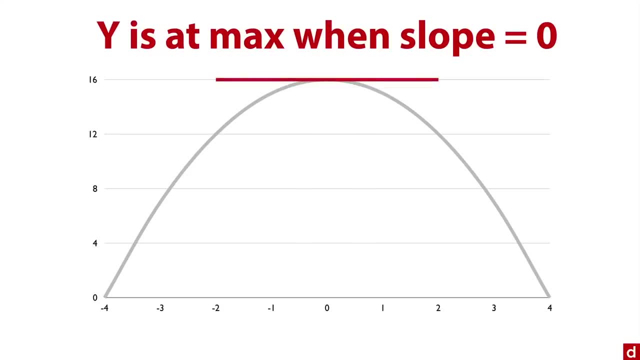 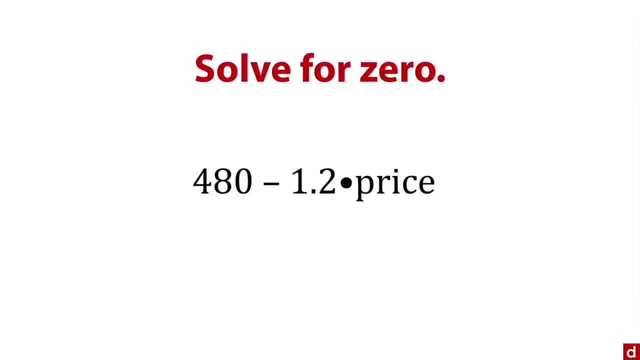 value right here, when it's at the very tippy top of the curve, because that will indicate maximum revenue. Okay, so what we're going to do is we're going to solve for zero. Let's go back to our equation here. We want to find out: when is that equal to zero? Well, we subtract 480 from each. 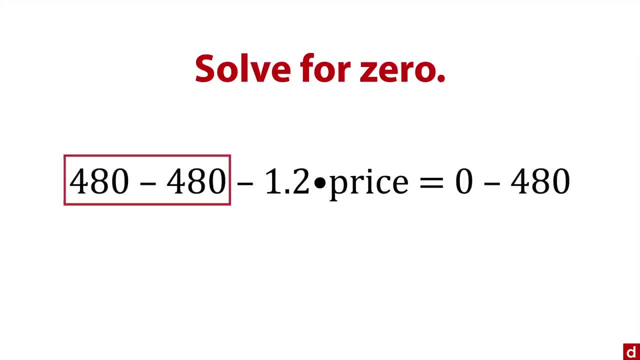 side. There we go And we divide by minus 1.2 on each side And this is our price for maximum revenue. So we've been charging $500 a week, but this says we'll have more total income if we charge 400 instead And 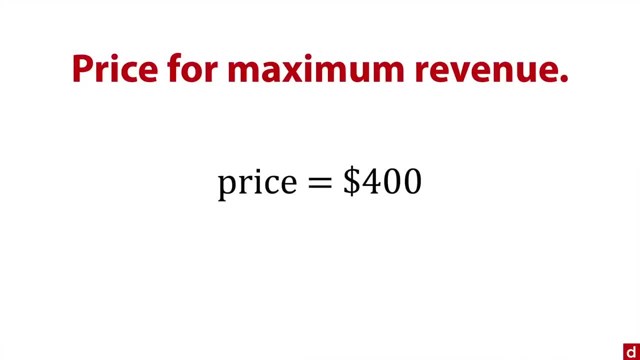 if you want to find out how many sales we can get- currently we have 480.. And if you want to know what the sales volume is going to be for that, Well, you take the 480, which is the hypothetical y intercept when the price is zero, but then we put in our actual price of 400.. Multiply that, we get to 40,. 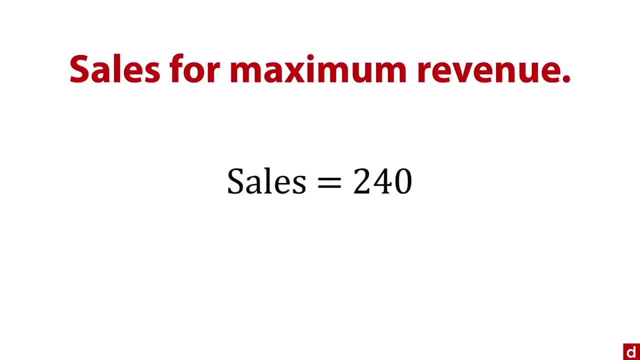 do the subtraction and we get 240 total. So that would be 240 new subscriptions per week. So let's compare this. the current revenue is 180 new subscriptions per week at $500 per year And that means that our current revenue is $90,000 per year. I know it sounds, it sounds. 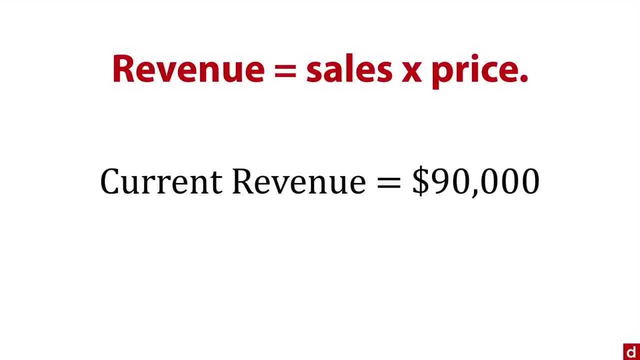 really good, But we can do better than that, Because the formula for maximum revenue is 240 times 400.. When you multiply those, you get 96,000., And so the improvement is just the ratio of those two. 96,000 divided by 90,000 is equal to 1.07.. And what that means is a 7% increase, and 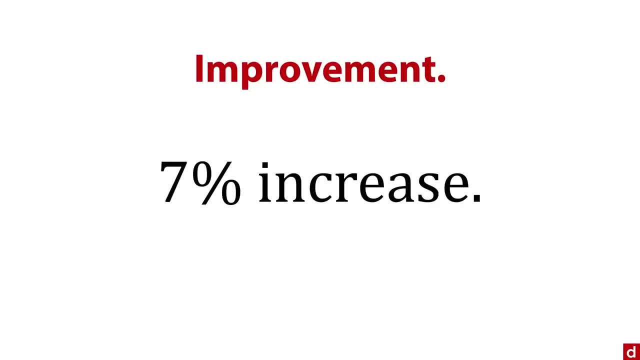 anybody would be thrilled to get a 7% increase in their business simply by changing the price and increasing the overall revenue. So that's the formula for maximum revenue. So let's summarize what we found here. If you lower the cost by 20%, go from $500 per year to $400. 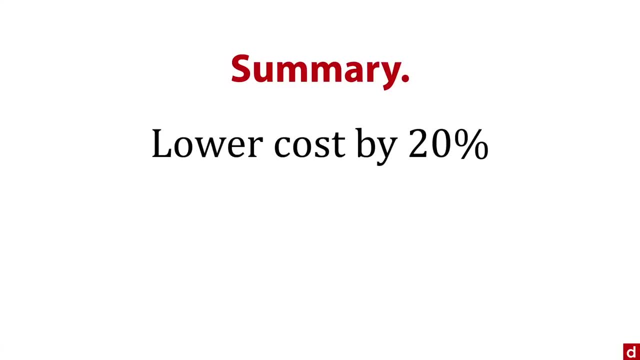 per year. assuming all of our other information is correct, then you can increase sales by 33%. That's more than the 20 that you had, And that increases total revenue by 7%, And so we can optimize the price to get the maximum total revenue. And it has to do with this little. 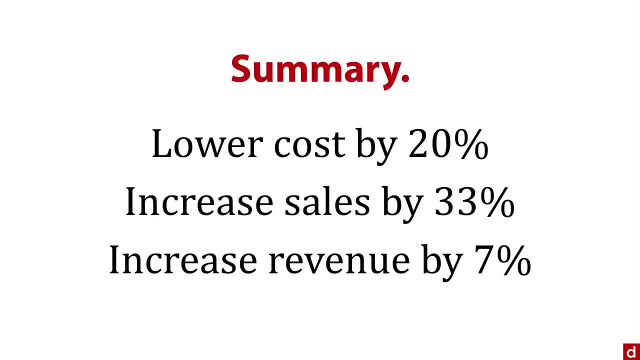 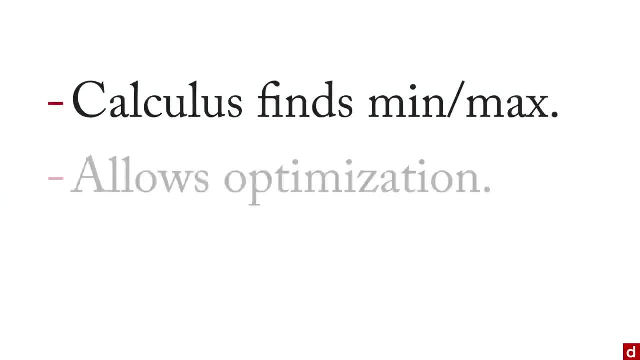 bit of calculus and the derivative of a function. So, in sum, calculus can be used to find the minima and the maxima of functions, including prices. It allows for optimization And that, in turn, allows you to make better business decisions. 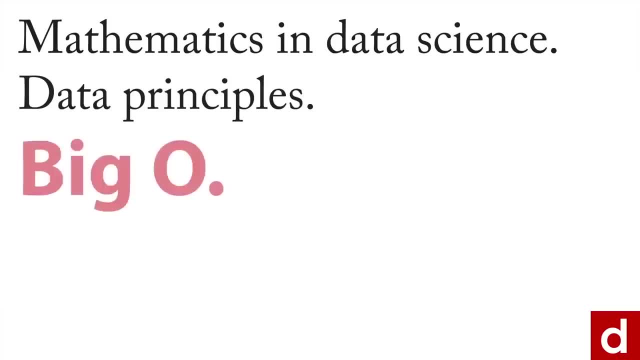 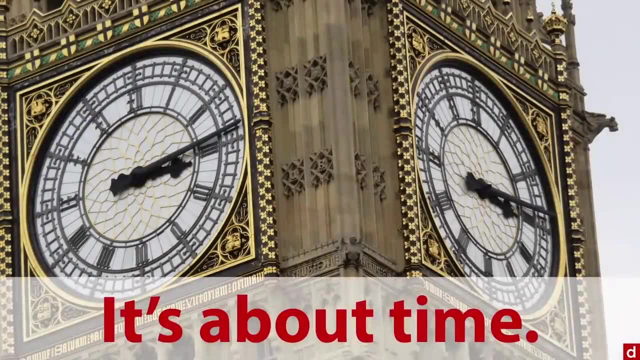 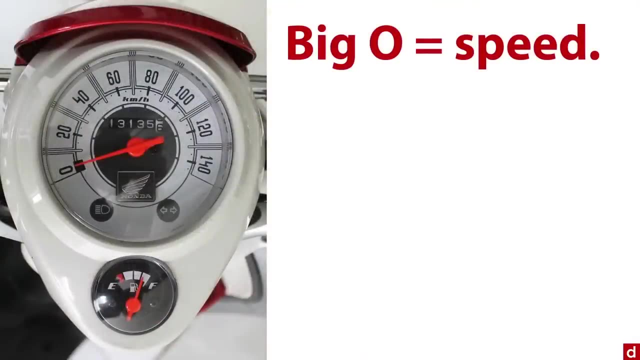 Our next topic in mathematics and data principles is something called Big O. And if you're wondering what Big O is all about, well, it is about time, Or you can think of it as how long does it take to do a particular operation? it's the speed of the operation, If you want to be really precise. 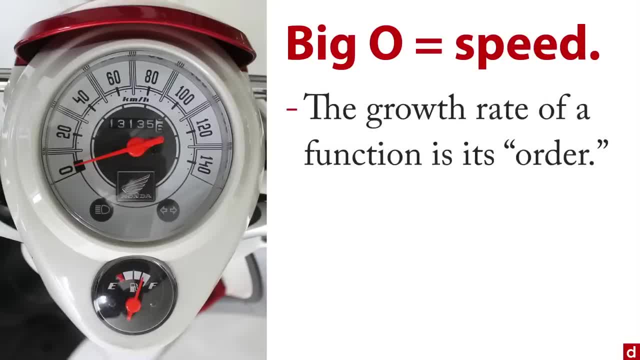 the growth rate of a function, how much more it requires, as you add elements, is called its order. That's why it's big oh, that's for order, And big O gives the rate of how things grow as number of elements grows. And what's funny is there can be really surprising differences. Let me show you. 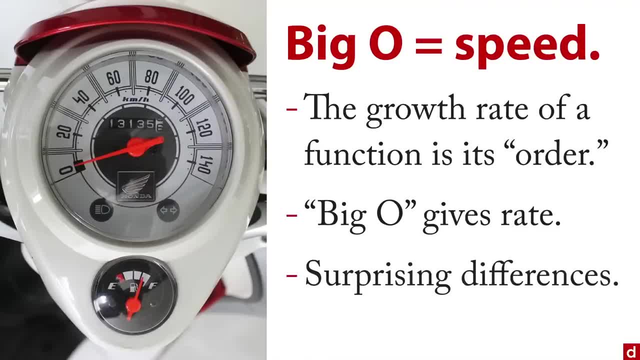 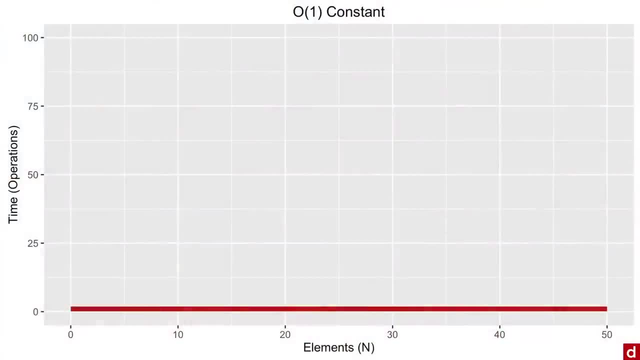 how it works with a few different kinds of growth rates, or big Oh. first off there's the ones that I say are sort of just on the spot. you can get stuff done right away. The simplest one is Oh one, and that is a constant order, And that's something that takes the same amount of time, no matter what. 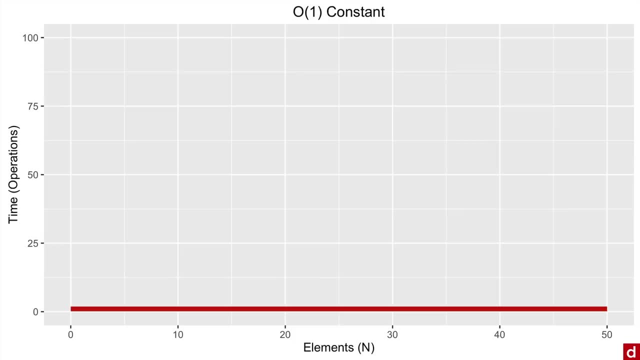 you can send out an email to 10,000 people. just hit one button, it's done. The number of elements, number of people, the number of operations, it just takes the same amount of time. Up from that is logarithmic. where you take the number of operations, you get the logarithm of that. 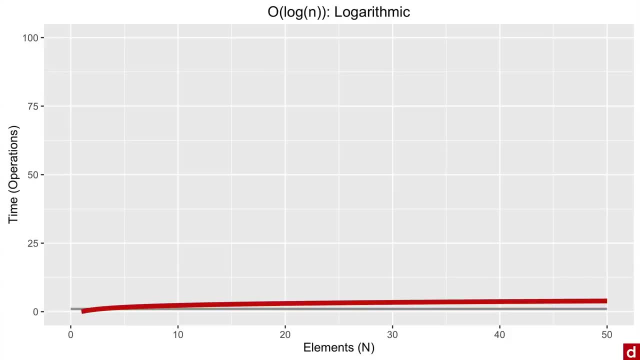 And you see it's increased, but it's really only a small increase and it tapers off really quickly. So an example is: finding an item in a sorted array- not a big deal. Next one up from that. Now this looks like a big change, But in the grand schemes it's not a big change. This is a linear. 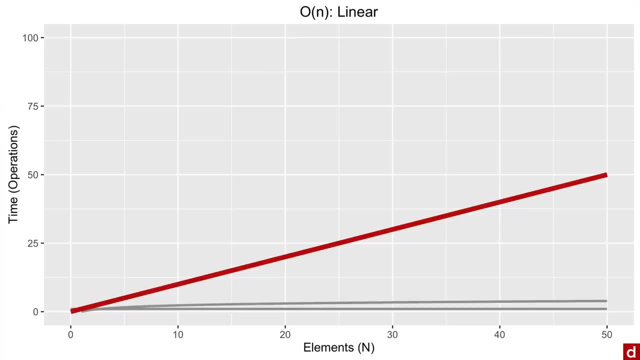 function where each operation takes the same unit of time, And so if you have 50 operations, it takes 50 units of time. if you're storing 50 things, it takes 50 units of space. So find an item in an unsorted list. 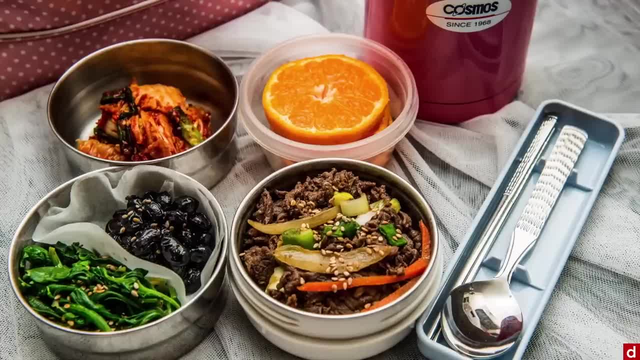 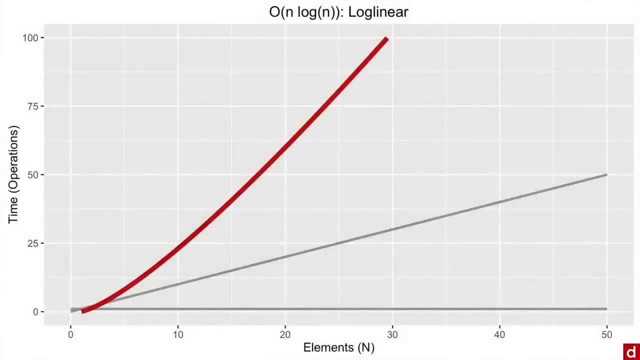 it's usually going to be linear time. Then we have the functions where I say: you know you better just pack a lunch because it's going to take a little while. The best example of this is what's called log linear. that's where you take the number of items and you multiply that. 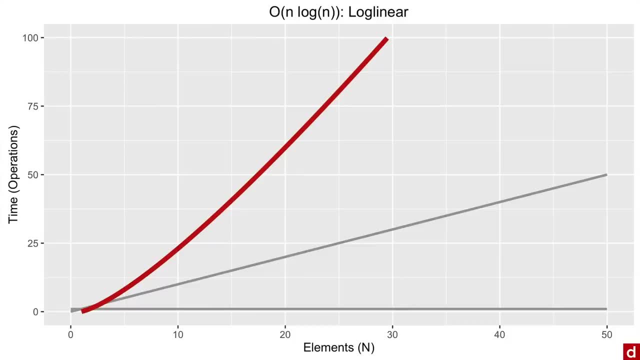 number times, the log of the items, And an example of this is something called a fast Fourier transform, which is used for dealing, for instance, with sound or anything that's over time. You can see it takes a lot longer. if you got 30 elements, you're way up there at the top of this. 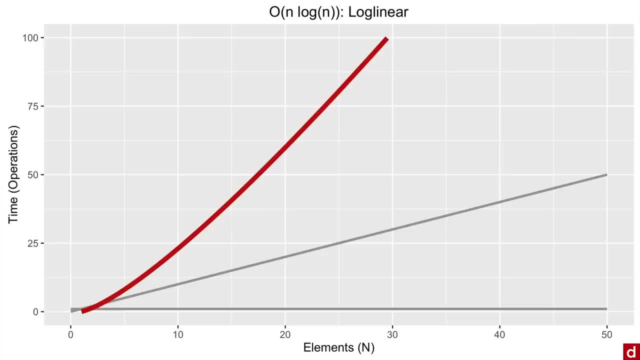 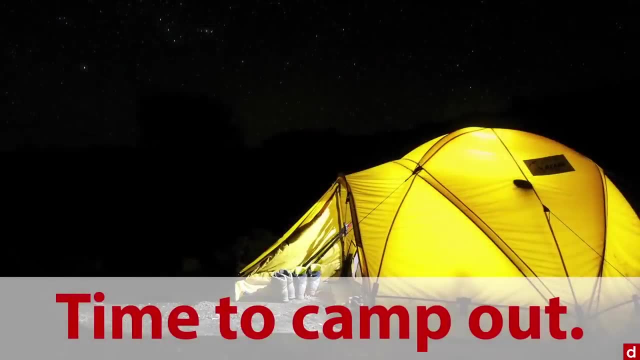 particular chart at 100 units of time or 100 units of space, or however you want to put it, And it looks like a lot, But really that's nothing compared to the next set where I say: you know, you're just gonna be camping out, you might as well go home. 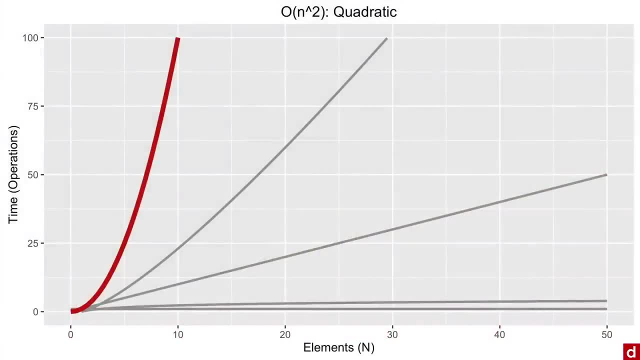 That includes something like the quadratic. you square the number of elements and see how that just kind of shoot straight up. that's quadratic growth And so multiplying two n digit numbers. so if you're multiplying two numbers that each have 10 digits, it's going to take you that long. 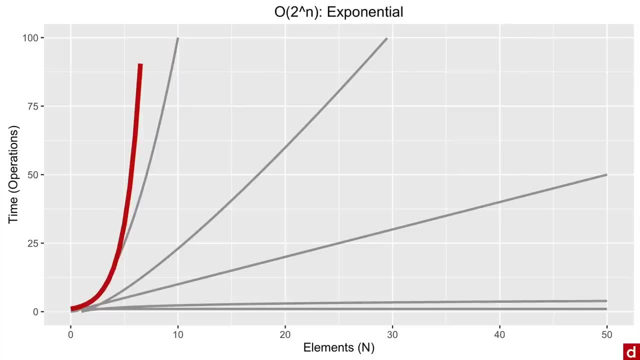 it's gonna take a long time. Even more extreme is this one. this is the exponential to raise to the power of the number of items you have. you'll see, by the way, the red line here doesn't even go to the top. That's because the graphing software that I'm using doesn't draw it when it goes above my. 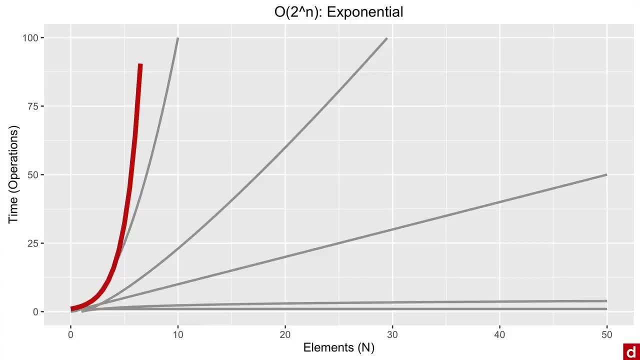 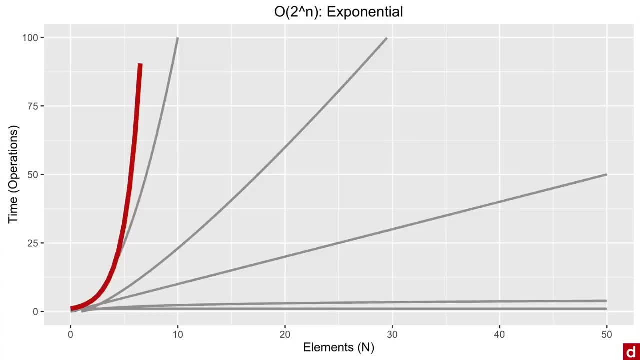 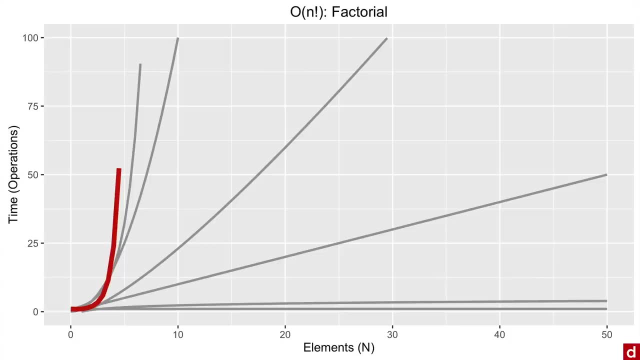 catastrophic- is factorial. you take the number of elements and raise that to the you know exclamation point- factorial- And you see that one cuts off really soon because it basically goes straight up. you have any number of elements of any size. it's going to be hugely demanding And 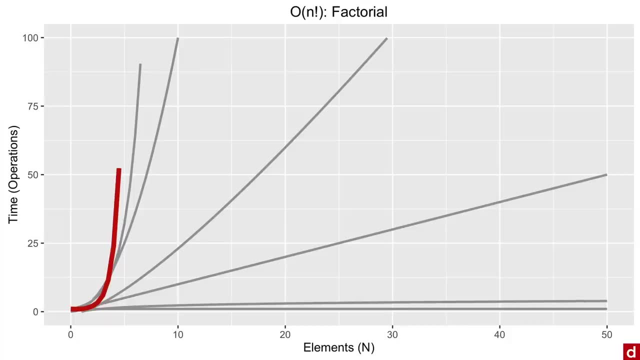 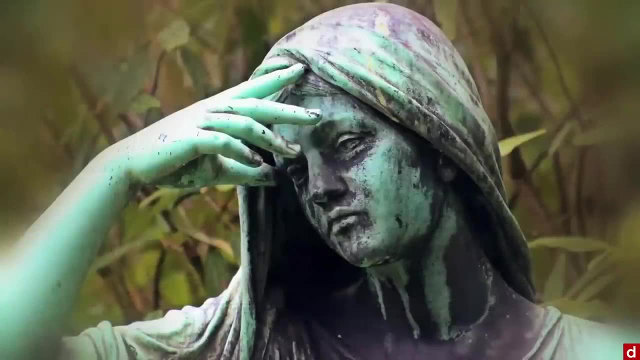 for instance, if you're familiar with the traveling salesman problem, that's trying to find a solution to what's called the traveling salesman problem using dynamic programming, a solution through the brute force search. it just takes an extraordinary amount of time And so you know, before something like that's done, you're probably just gonna, you know. 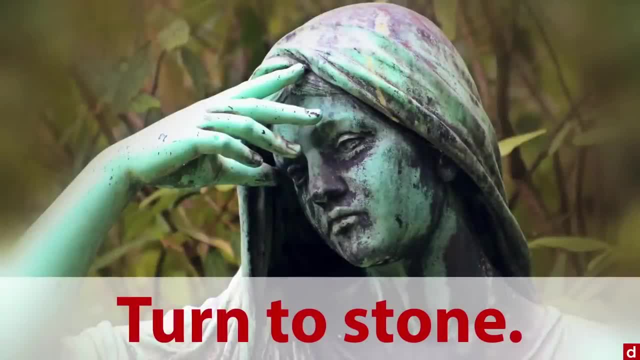 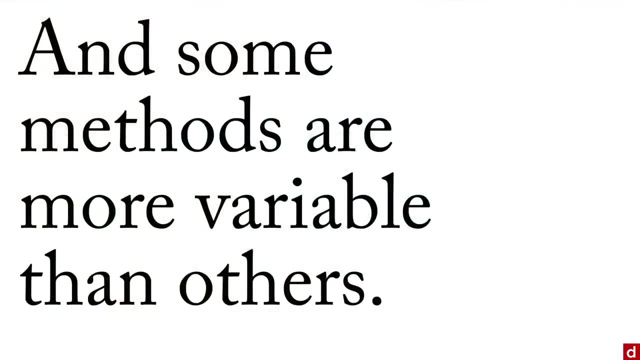 turn to stone and wish you never even started. The other thing to know about this is: not only do some things take longer than others, some of these methods, some functions, are more variable than others, So, for instance, if you're working with data that you want to sort, there are different. 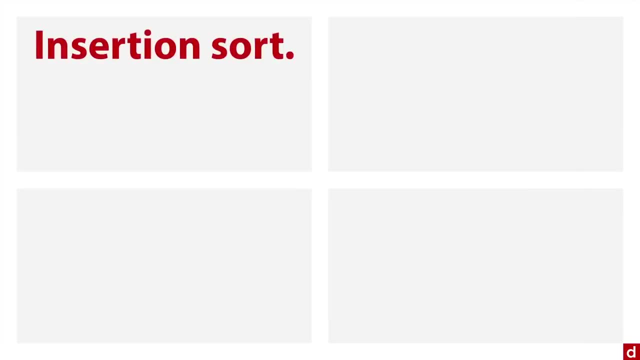 kinds of sorts or sorting methods. So, for instance, there's something called an insertion sort And what you find is that on its best day it's linear, it's O of n. that's not bad. On the other hand, the average is quadratic, And that's a huge difference between the two Selection sorts. 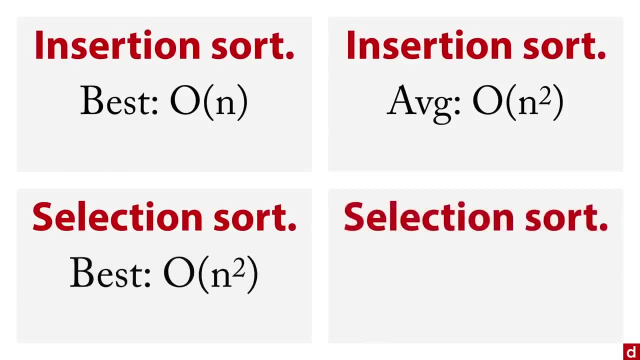 on the other hand, the best is quadratic and the average is quadratic. it's always consistent. So it's kind of funny. it takes a long time, but at least you know how long it's going to take- versus the variability of something like an insertion sort. So 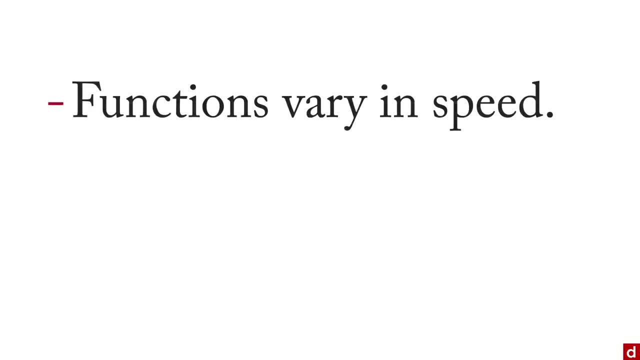 in sum, let me say a few things about big O. Number one: you need to know that certain functions or procedures vary in speed, And the same thing applies to making demands on a computer's memory or storage space or whatever. They vary in their demands. Also, some of them are inconsistent. 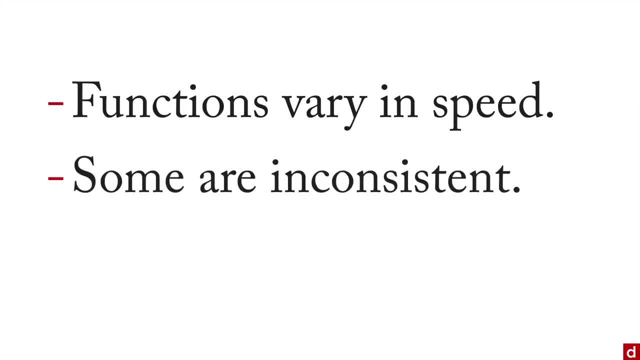 some of them are really efficient sometimes and really slow or really difficult the others. Probably the most important thing here is to be aware of the demands of what you're doing, that you can't, for instance, just run through every single possible. 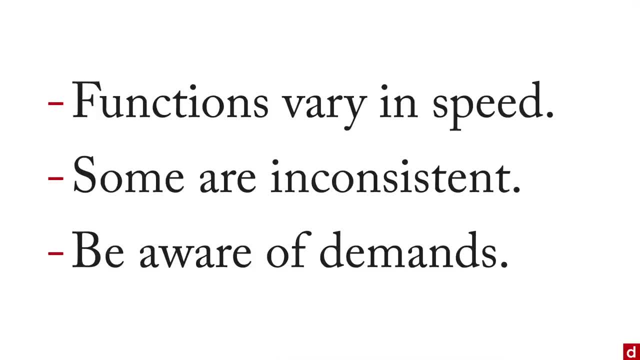 solution or, you know, your company will be dead before you get an answer. So be mindful of that, So you can use your time well and get the insight you need in the time that you need it. A really important element of the mathematics and data science and one of its 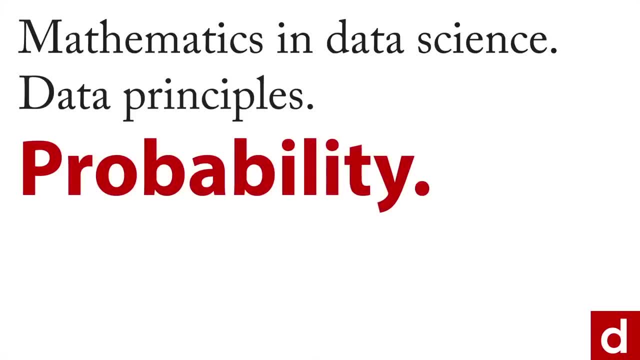 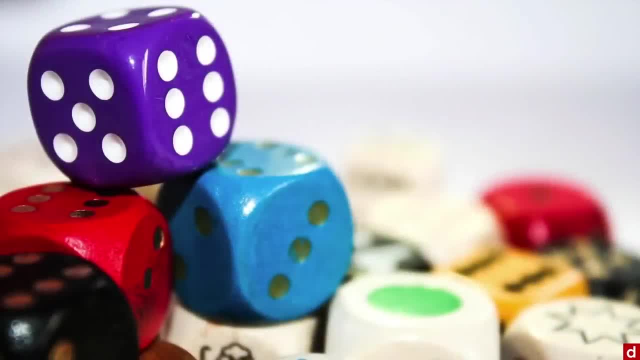 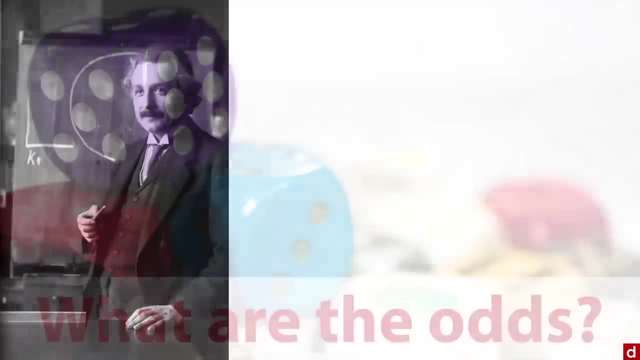 foundational principles is probability. Now, one of the things that probability comes in intuitively for a lot of people is something like rolling dice or looking at sports outcomes And really the fundamental question: what are the odds of something that gets at the heart of probability? Now let's take a look at some of the basic. 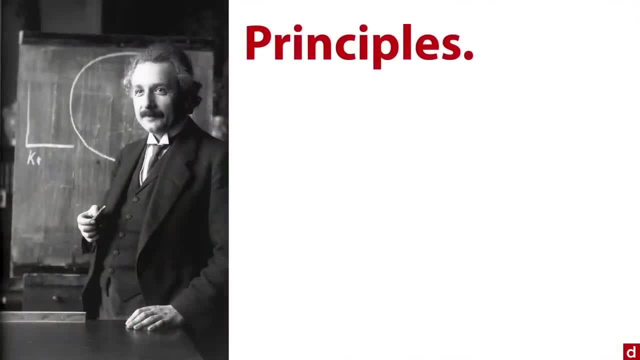 principles. We got our friend Albert Einstein here to explain things. The principles of probability work this way: Probabilities range from zero to one, that's like 0% to 100% chance. When you put P, that stands for probability, and then in parentheses here a, that means the 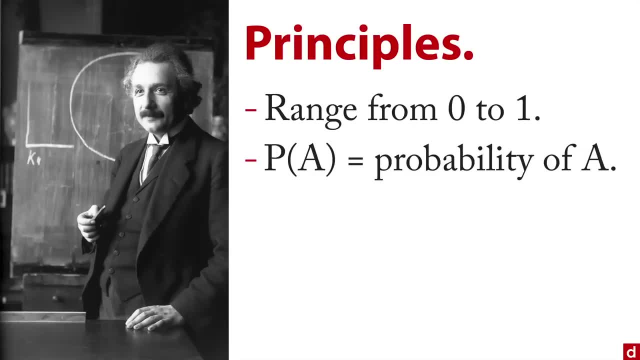 probability of whatever in parentheses. So P a means the probability of a, and then P of B is the probability of B. When you take all of the probabilities together, you get what's called the probability space, And that's why we have s, And it all adds up to one, because you've now covered. 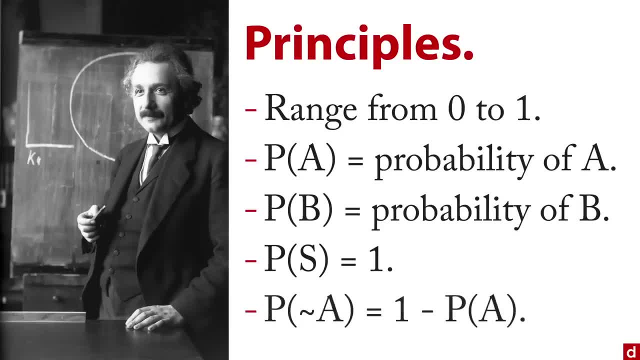 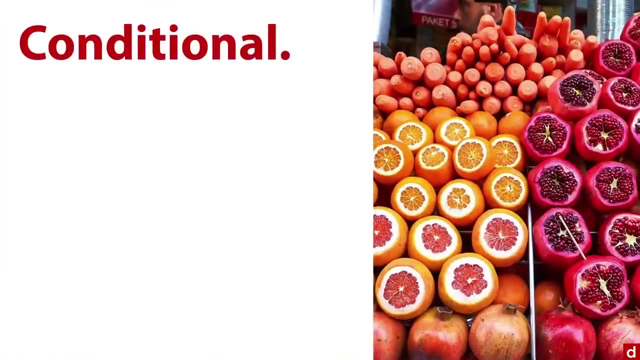 100% of the possibilities. Also, you can talk about the compliment. the tilde here is used to say: probability of not a is equal to one minus the probability of a, because those have to add up. So let's take a look at something also about conditional probabilities, which is really. 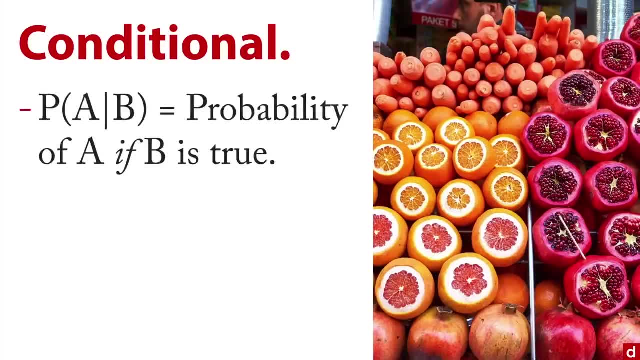 statistics. A conditional probability is the probability of something. if something else is true, You write it this way: the probability of, and that vertical line is called a pipe And it's read as assuming that or given that. so you can read this as probability of a given B is the 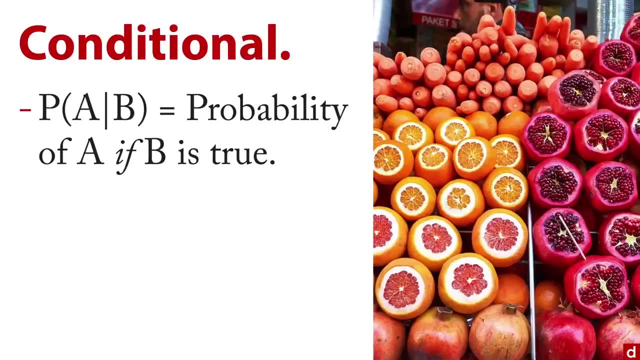 probability of a occurring if B is true, And so you can say, for instance, what's the probability if something's orange, What's the probability that's a carrot, given this picture? Now, the place this comes in, really important for a lot of people is the probabilities of type one and type two. 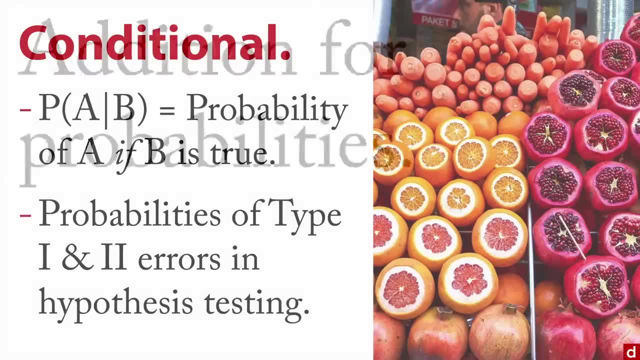 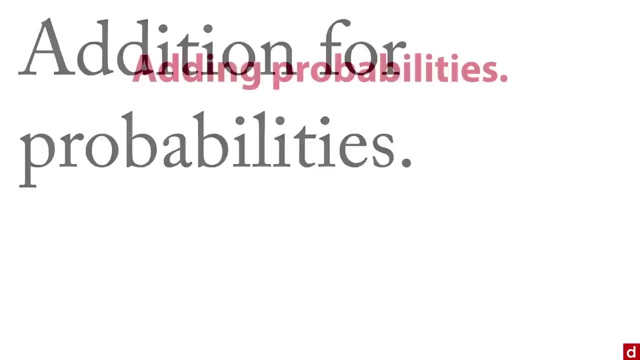 errors and hypothesis testing, which we'll mention at some other point. But I do want to say a few things about arithmetic with probabilities, because it doesn't always work the way that people think it will. Let's start by talking about adding probabilities. Let's say: you have 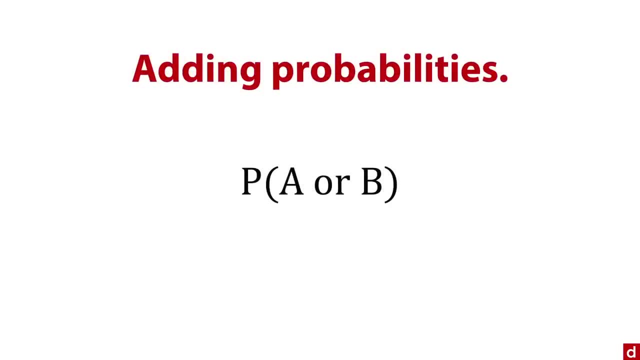 two events, A and B, And let's say you want to find the probability of either one of those events. So that's like adding the probabilities of the two events. Well, it's kind of easy: you've take the probability of event A and you add the probability of event B. However, you may have to. 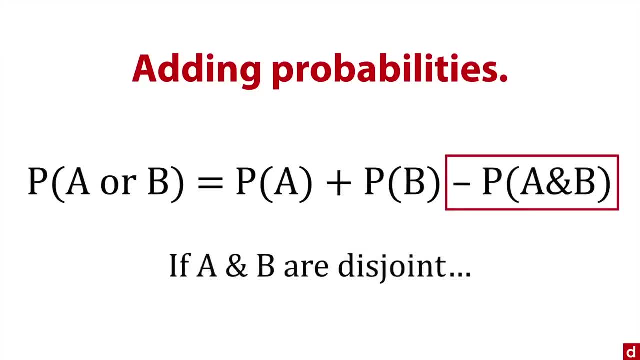 subtract something. you may have to subtract this little piece, because maybe there's some overlap between the two of them. On the other hand, if A and B are disjoint, which means they never occur together, then that's equal to zero, And then you can, you know, subtract zero, which is you get back. 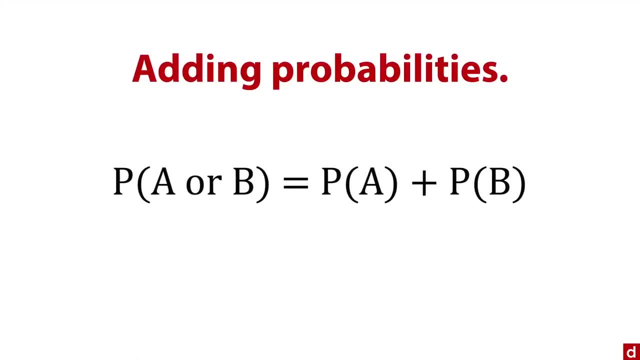 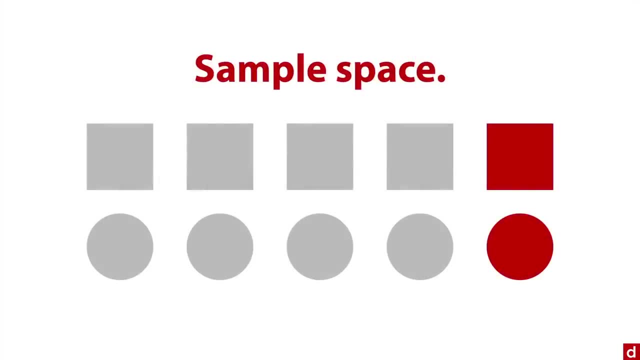 to the original probabilities. But let's take a really easy example of this. I've created my super simple sample space. I have 10 shapes. I got five squares on the top, five circles on the bottom. I've got a couple of red shapes on the right side. Let's say we want to find the probability of a. 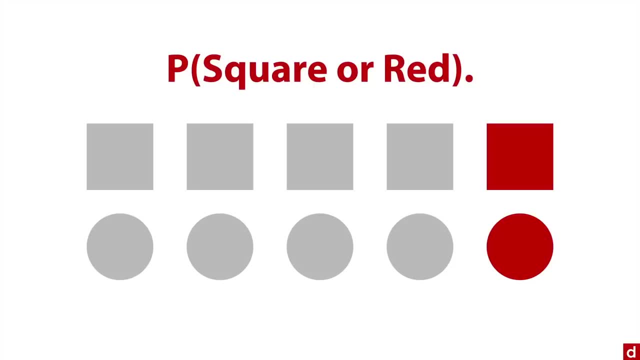 square or a red shape. So we are adding the probabilities, but we have to adjust for the overlap between the two. Well, here's our squares: on top, five out of the 10 are squares, And over here on the right we have two red shapes, two out of 10.. So let's go back to our formula here And 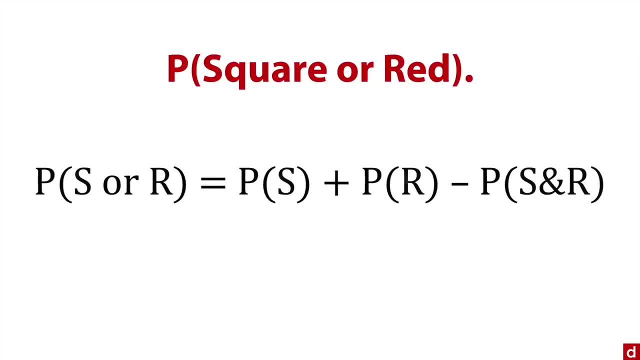 let's change the formula here. So let's go back to our formula here And let's change the formula here. And let's go back to our formula here And let's change the formula here And let's change a little bit. change the A and the B to s and r for square and red. Now we can start this way. 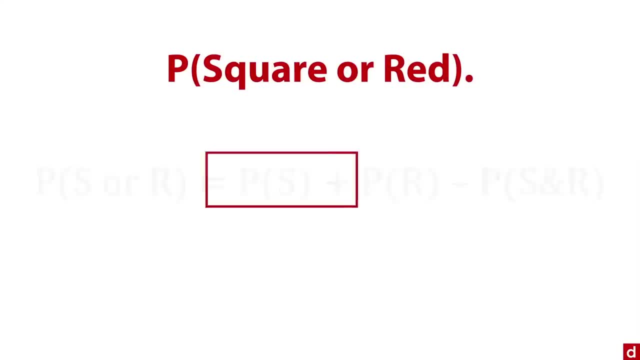 let's get the probability that something is a square. Well, we go back to our probability space. you see, we have five squares out of 10 shapes total. So we do five over 10, that reduces to 0.5.. Okay, next up the probability of something red in our sample space. Well, we have 10 shapes total. 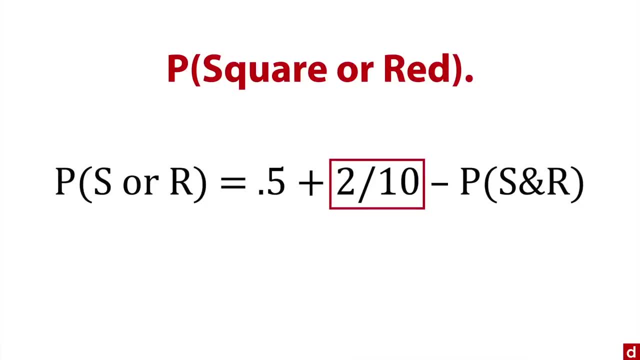 two of them on the far right are red, So that's two over 10.. And you do the division, you get point two. Now the trick is the overlap between these two categories. do we have anything that is both square and red? because we don't want to count that twice, So we have to subtract it. So let's. 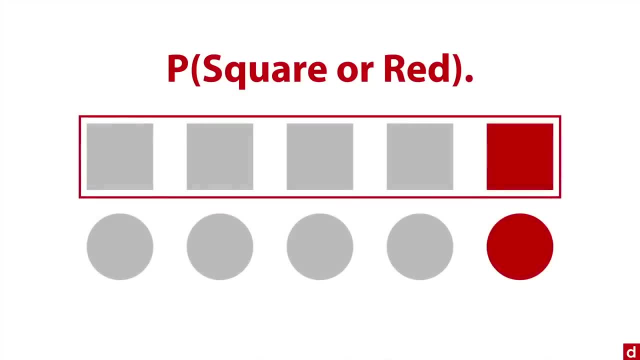 go back to our sample space And we're looking for something that is square. there's the squares on top And there's the things that are red on the side, And you see they overlap And this is our little overlapping red square. So there's one shape that meets both of those, one out of 10.. So we can. 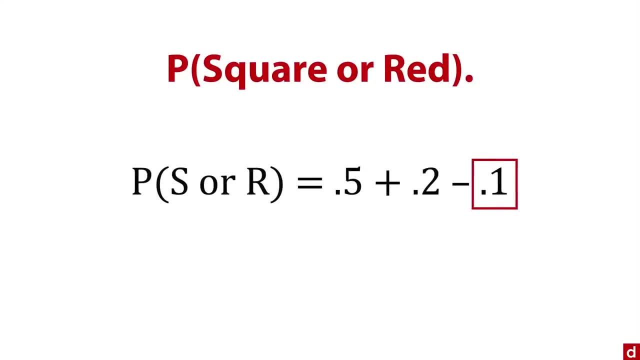 back here. we do one out of 10, that reduces to point one, And then we just do the addition And subtraction here. point five plus point two minus point one gets us point six. And so what that means is there's a 60% chance of an object being square or red, And you can look at it right here. 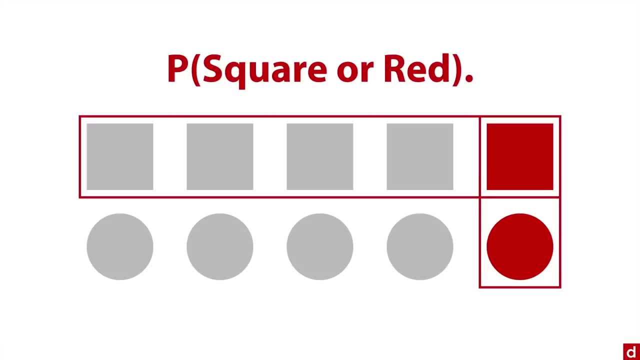 we got six shapes outlined now, And so that's the visual interpretation that lines up with the mathematical one we just did. Now let's go to our sample space And we're going to add all these six shapes to our sample space, And then we're going to add all the squares and reds to our sample space. 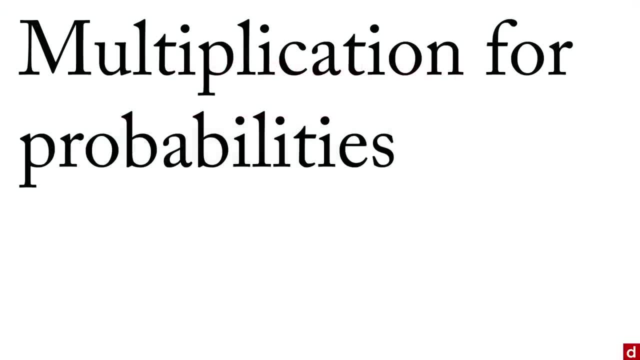 We've also added two shapes to our sample size And we're going to create our own model. And then we're going to add: Now let's talk about multiplication for probabilities. Now, the idea here is, you want to get what are called joint probabilities are the probability of two things occurring together simultaneously. 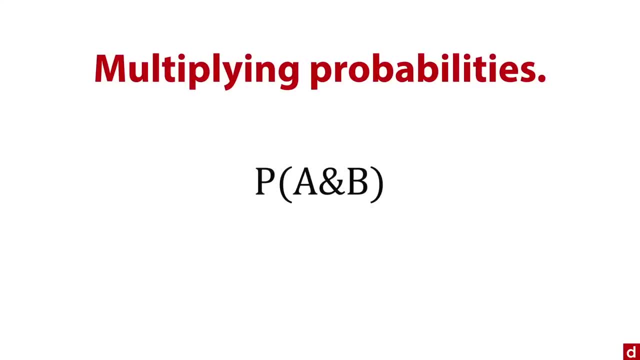 And what you need to do here is you need to multiply the probabilities and we can say probability of A and B, because we're asking about A and B occurring together, a joint occurrence, And it's equal to the probability of A times the probability of B. that's easy, But you 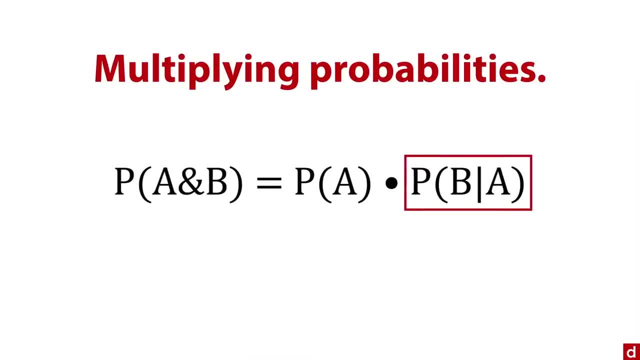 do have to expand it just a little bit, because you can have the problem of things overlapping a little bit, And so you actually need to expand it to an conditional probability. the probability rephrase, the probability of B given a. again, that's the vertical pipe. 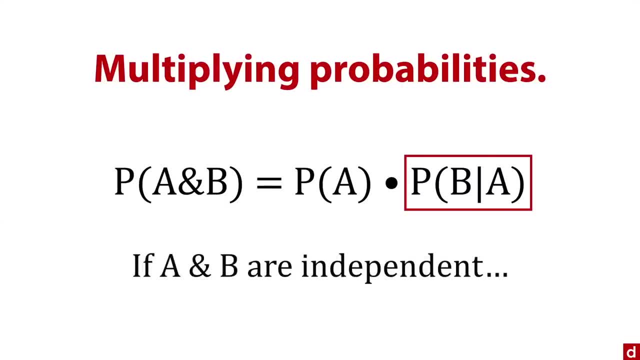 there. On the other hand, if A and B are independent, if they never co occur or they, B is no more likely to occur. if A happens, then it just reduces to the probability of B and you get your slightly simpler equation. But let's go and take a look. 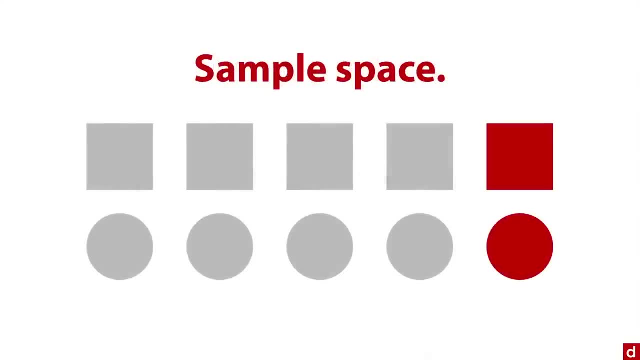 At our sample space right here. So we've got our 10 shapes, five of each kind and then two that are red, And we're going to look at, originally, the probability. something means square or red. Now we're going to look at the probability of it being square and red. 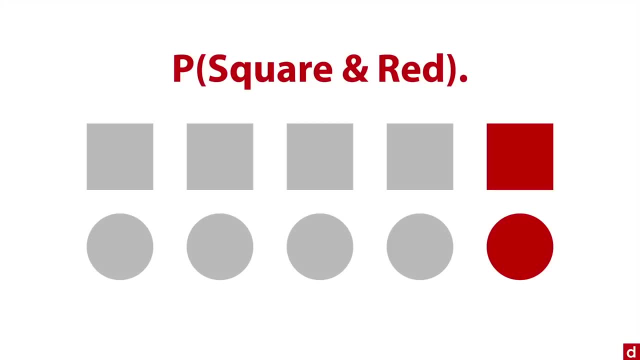 Now, I know we can eyeball this one really easy, but let's run through the math. The first thing we need to do is get the ones that are square. there's those five on the top and the ones that are red, and there's those two on the right in terms of the ones. 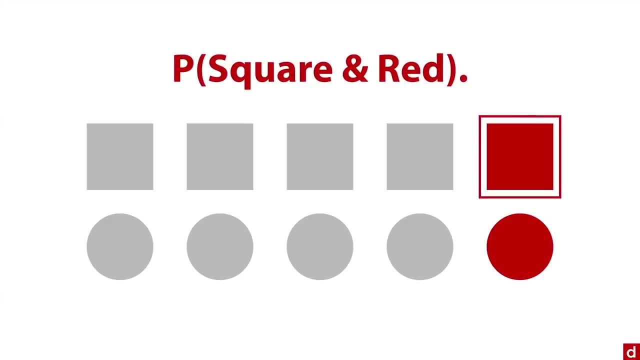 that are both square And red. yeah, obviously there's just this one red square at the top right. But let's do the numbers here. We change our formula to be SNR for square and red. we get the probability of square Again. that's those five out of 10.. So we would do five out of 10 reduces. 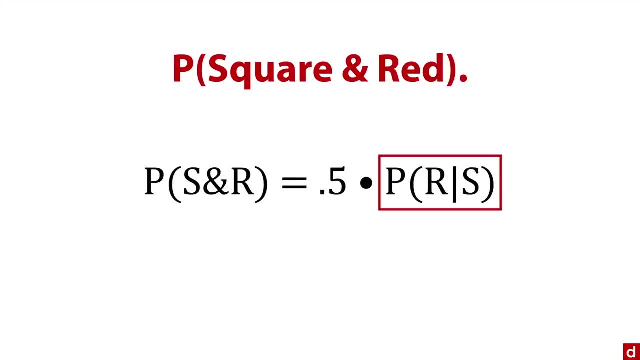 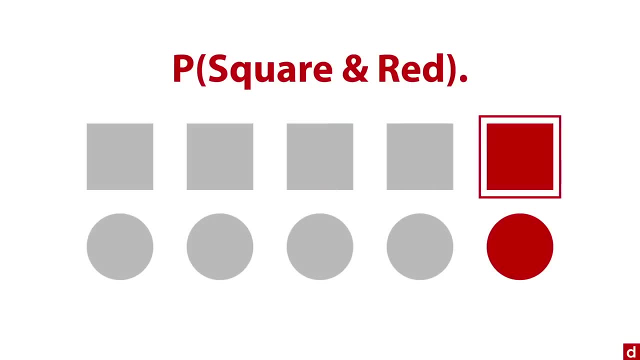 to point five. And then we need the probability of red, given that it's a square. So we only need to look at the squares. here There's the squares, five of them, and one of them is red. So we're going to do point five. that reduces to point two. you multiply those two numbers. 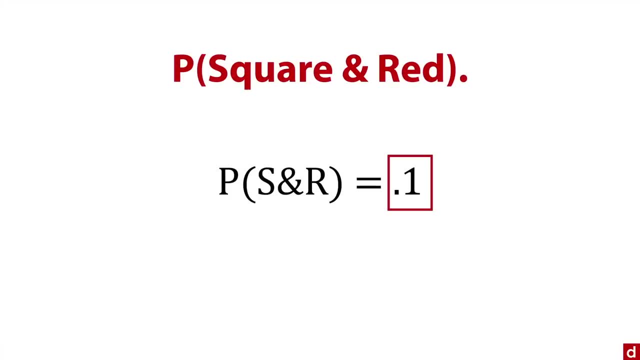 point five times point two and what you get is point one or a 10% chance, or 10% of our total sample space is red squares. And you come back and you look at it, you say yeah, there's one out of 10.. So that just confirms what we were able to do intuitively. So that's. 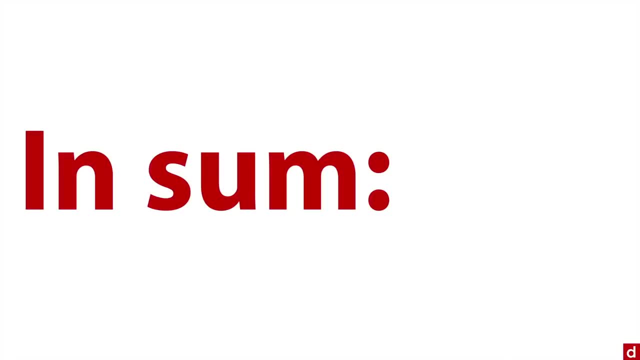 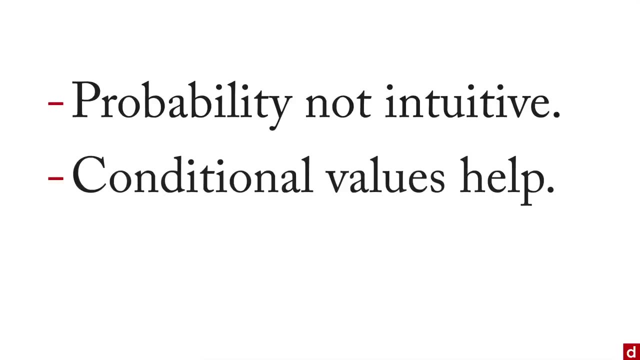 our short presentation on probabilities And, in sum, what do we get out of that? Number one, probability- it's not always intuitive. And also the idea that conditional probability, conditional values, can help in a lot of situations, but they may not work the way you expect them. 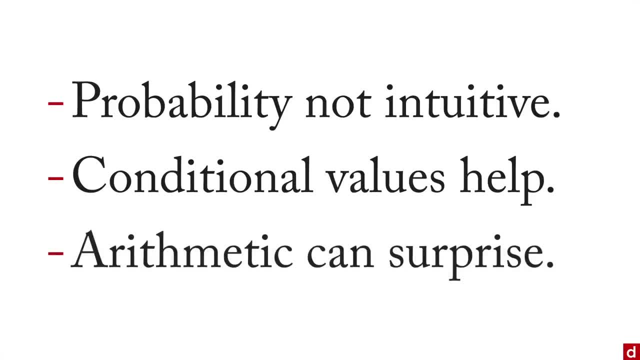 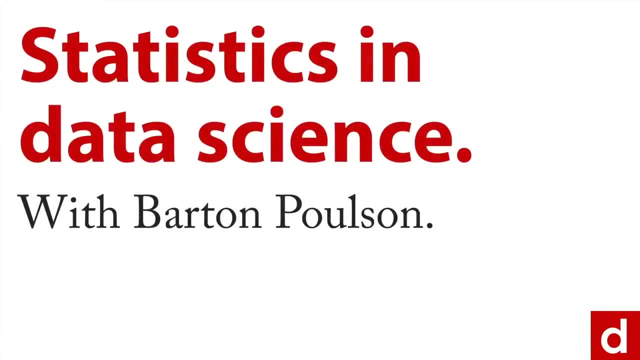 to, And really the arithmetic of probability can surprise people, So pay attention when you're working with it, So you can get a more accurate conclusion in your own calculations. Welcome to statistics in data science. I'm Barton Poulson, And what we're going to be. 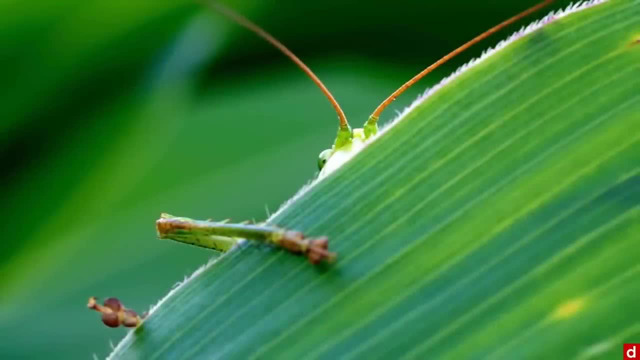 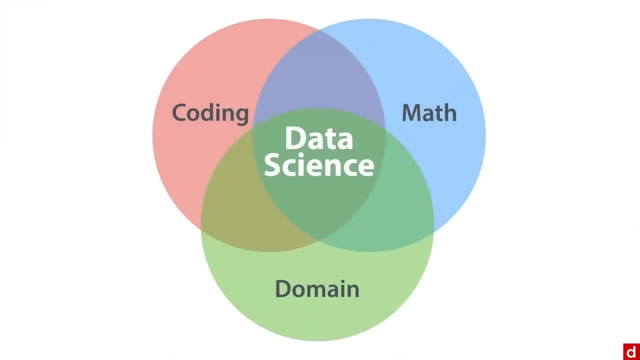 doing in this course is talking about some of the ways that you can use statistics to see the unseen, to infer what's there, even when most of it doesn't exist. So if you're hidden now, this shouldn't be surprised, if you remember the data science Venn. 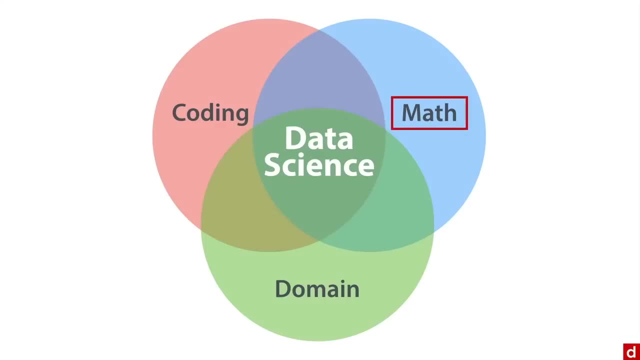 diagram that we talked about a while ago. we have math up here in the top right corner, but if you were to go to the original description of this Venn diagram, its full name was math and stats, and let me just mention something, in case it's not completely obvious, about why statistics matters to data science and 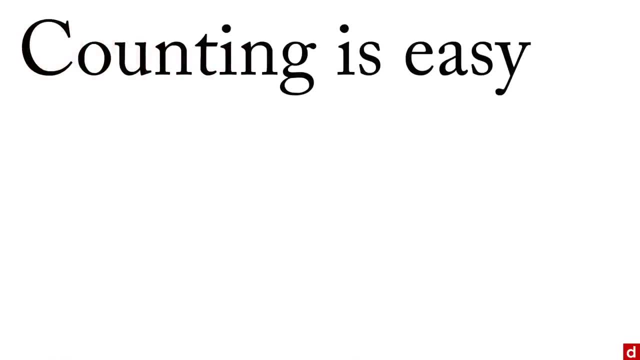 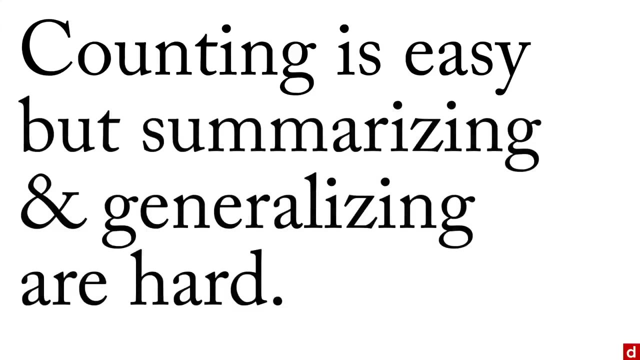 the idea is this: counting is easy. it's easy to say how many times a word appears in a document. it's easy to say how many people voted for a particular candidate in one part of the country. counting is easy, but summarizing and generalizing those things are hard, and part of the problem is there's no such 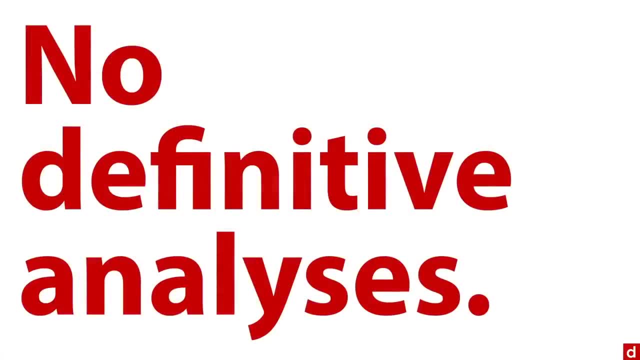 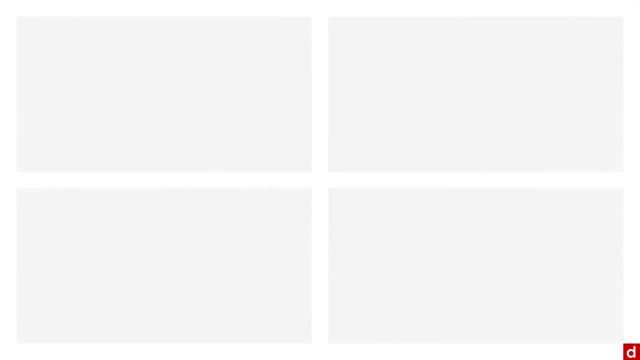 thing as a definitive analysis. all analyses really depend on the purposes that you're dealing with. so, as an example, let me give you a couple of pairs of words and try to summarize the difference between them into just two or three words. I mean in a word or two. how is a souffle different? 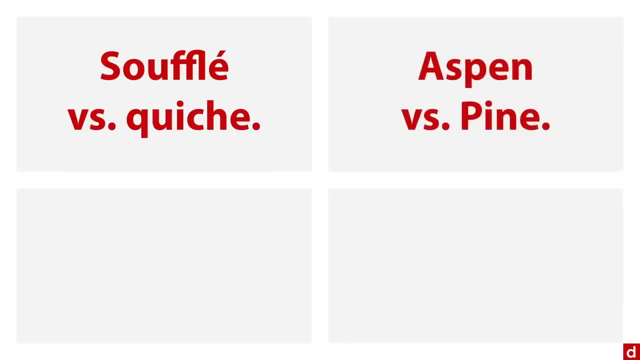 from a quiche, or how is an aspen different from a pine tree, or how is baseball different from cricket, and how are musicals different from opera? it really depends on who you're talking to, it depends on your goals and it depends on sort of the shared knowledge, and so there's not a single definitive answer. 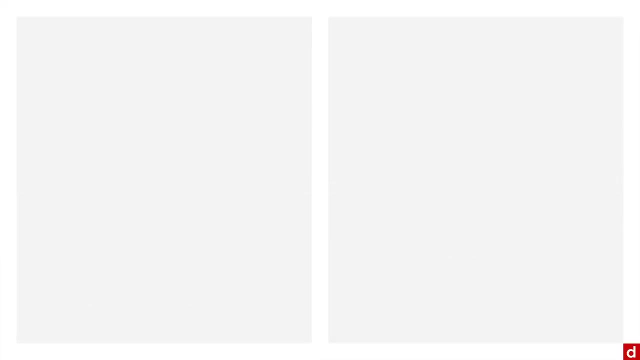 and then there's a matter of generalization. think about again. take music, listen to three words in a sentence and then think about how many words are being used. and then think about how many words are being used, how do they have a specific meaning? what are the key words that are important? 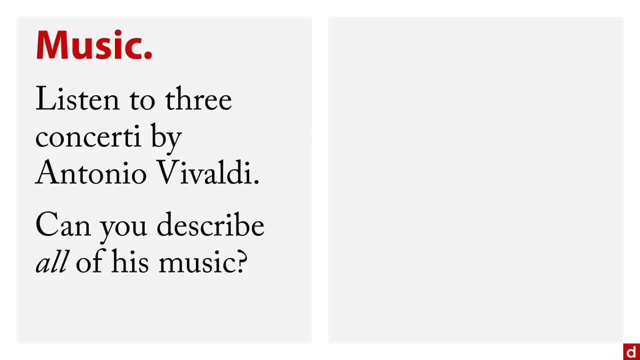 do you think you can safely and accurately describe all of his music? now? I actually chose Vivaldi on purpose because Igor Stravinsky said you could. he said he didn't write 500 concertos. he wrote the same concerto 500 times. but 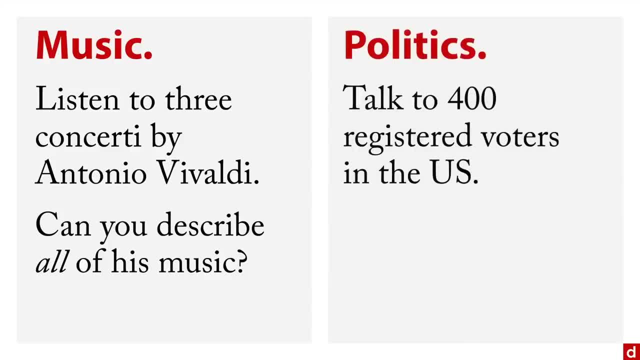 take something more real-world like politics. if you talk to 400 registered voters in the US, can you then accurately predict the behavior of all of the voters? there's about a hundred million voters in the US, And that's a matter of generalization, and that's the sort of thing that we try to take. 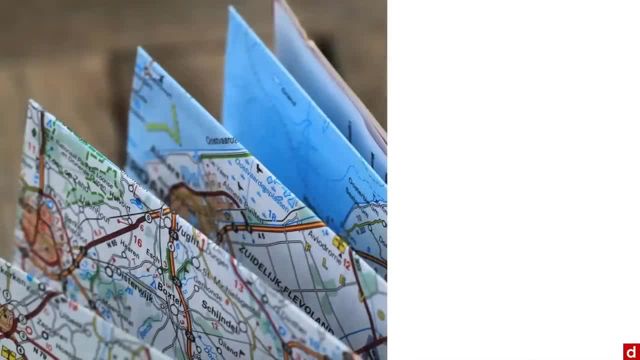 care of with inferential statistics. Now, there are different methods that you can use in statistics, and all of them are designed to give you sort of a map, a description of the data you're working with. There are descriptive statistics, there are inferential statistics, there's the inferential. 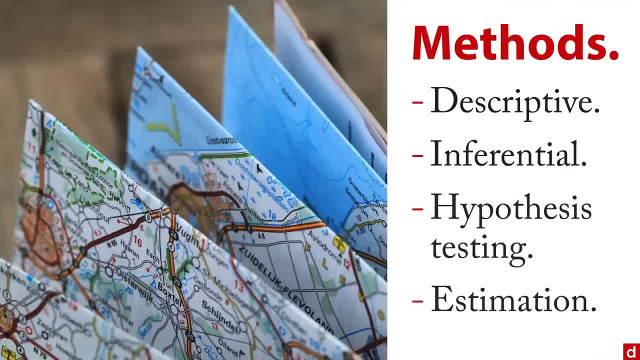 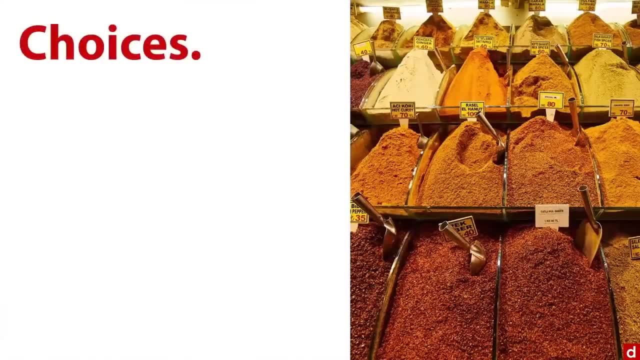 procedure, hypothesis testing, and there's also estimation, And I'll talk about each of those in more depth. There are a lot of choices that have to be made, and some of the things I'm going to discuss in detail are, for instance, the choice of estimators. that's different from estimation. 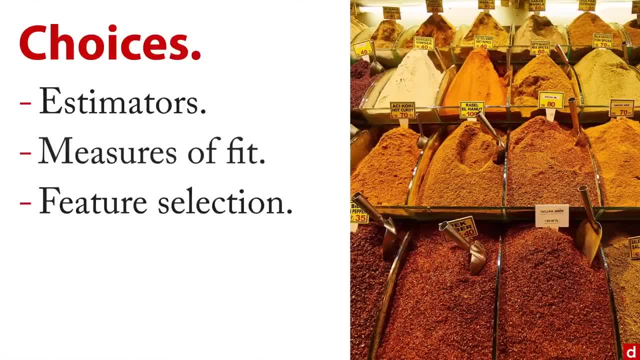 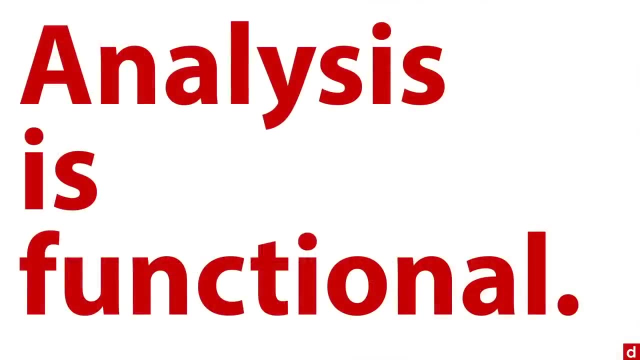 different measures of fit, feature selection for knowing which variables are the most important in predicting your outcome. also common problems that arise when trying to model data and the principles of model validation. But through this, all the most important thing to remember is that analysis is functional. 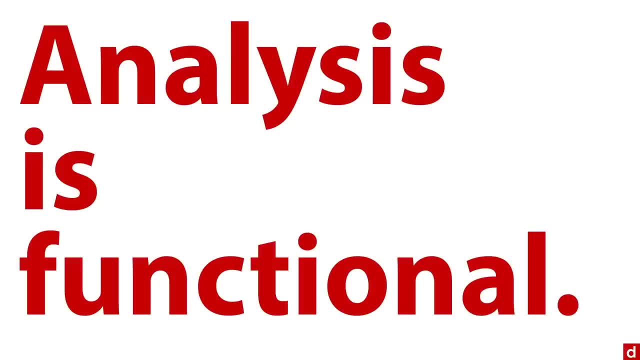 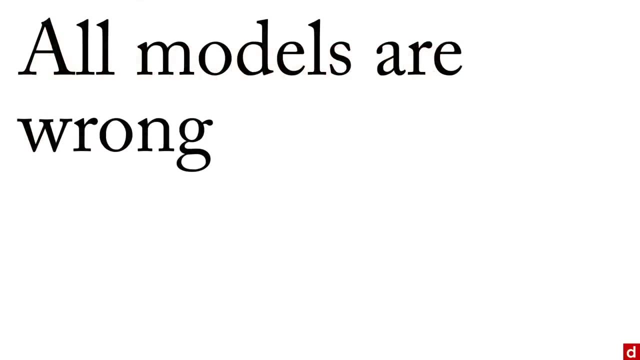 It's designed to serve a particular purpose. And there's a very wonderful quote within the statistics world that says: all models are wrong, All statistical descriptions of reality are wrong because they're not exact depictions, they're summaries, But some are useful. 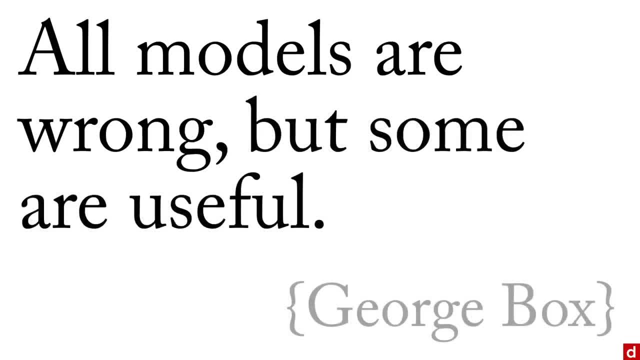 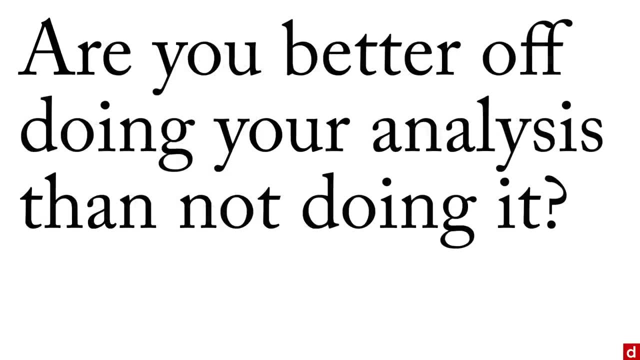 And that's from George Box. And so really the question is: you're not trying to be totally, completely accurate, because in that case you just wouldn't do an analysis. The real question is: are you better off doing your analysis than not doing it? 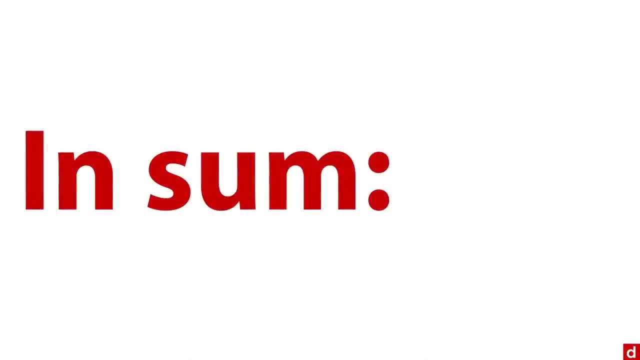 And truthfully, I bet you are. So, in sum, we can say three things. Number one: you want to use statistics to both summarize your data and to generalize from one group to another, if you can. On the other hand, there's no one true answer with data. 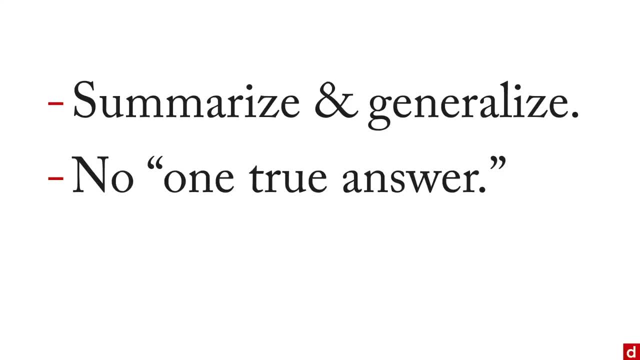 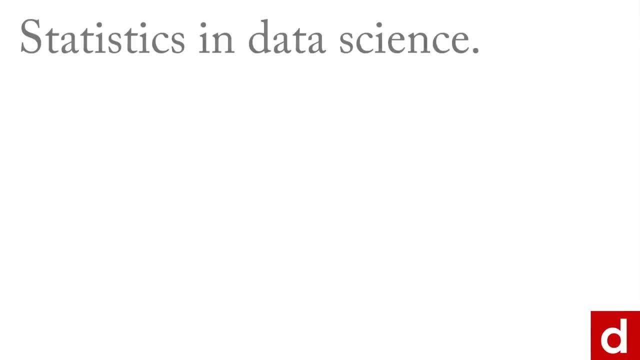 You got to be flexible in terms of what your goals are and the shared knowledge, And no matter what you're doing, the utility of your analysis should guide you in your decisions. The first thing we want to cover in statistics and data science is the principle of exploring. 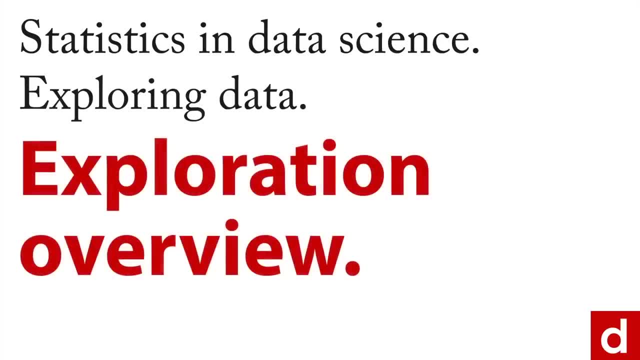 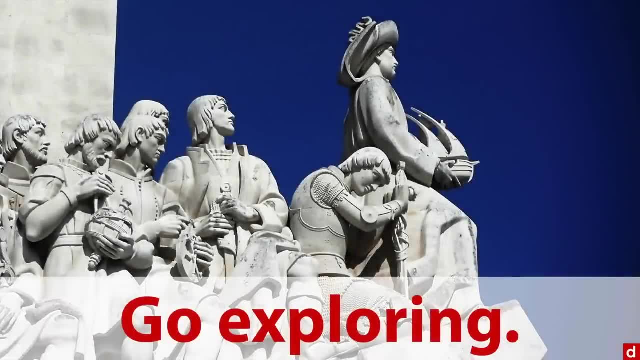 data, And this video is just designed to give an exploration overview. So we like to think of this: the intrepid explorers. they're out there exploring and seeing what's in the world. You can see what's in your data. More specifically, you want to see what your data set is like. 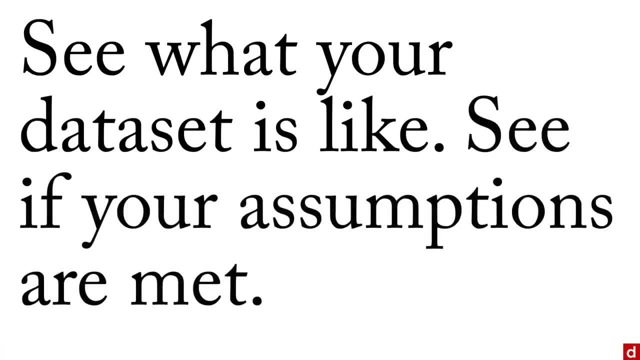 You want to see if your assumptions are met so you can do a valid analysis with your chosen procedure. And really, something that may seem very weird is you want to listen to your data. If something's not working out, if it's not going the way you want, then you need to pay. 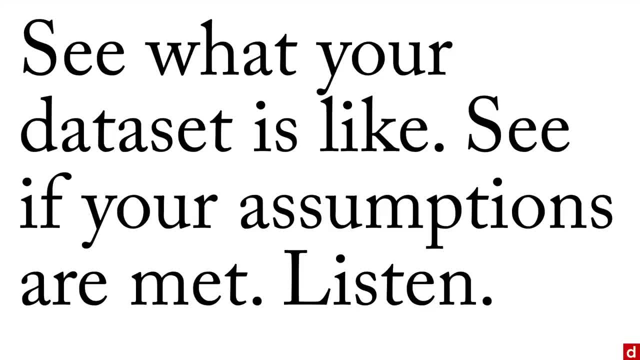 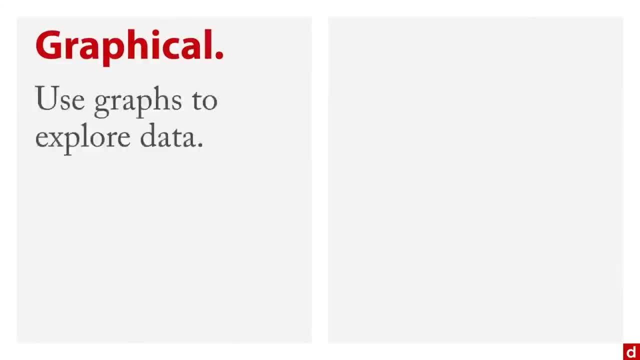 a little more attention Now. there are two general approaches to this. First off, there's a graphical exploration, So you use graphs and pictures and visualizations to explore your data. The reason you want to do this is that graphics are very dense in information. 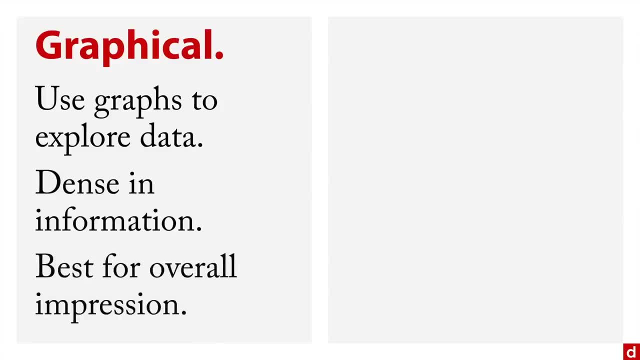 They're also really good, in fact the best way to get the overall impression of your data. Second to that, there's numerical exploration. I make it very clear: This is the second step. You want to do the visualization first, then do the numerical part. 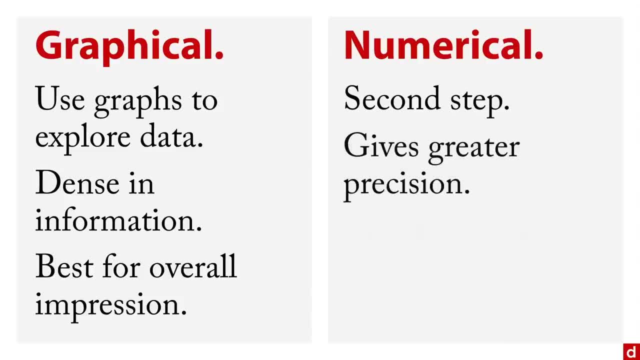 Now you want to do this because it can give greater precision and this is also an opportunity to try variations on the data. You can actually do some transformations, move things around a little bit and try different methods and see how that affects the results and see how it looks. 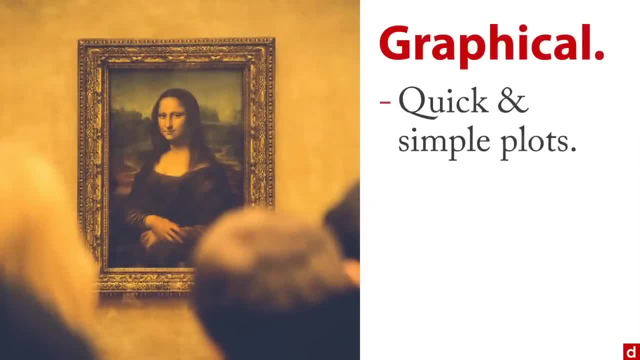 So let's go first to the graphical part. There are very quick and simple plots that you can do. Those include things like bar charts and histograms and scatter plots. It's very easy to make and very quick way of getting an understanding of the variables. 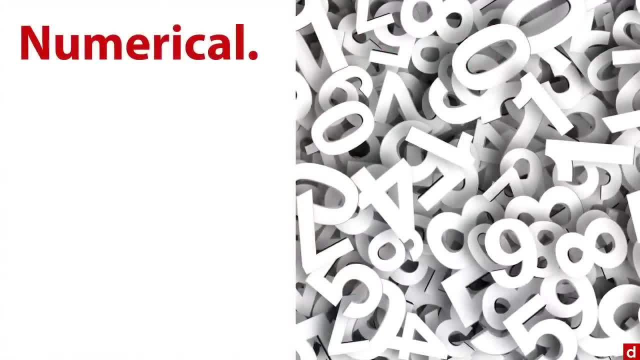 in your data set. In terms of numerical analysis, again after the graphical methods, you can do things like transform the data, that is, take like the logarithm of your numbers. You can do empirical estimates of population parameters and you can use robust methods. 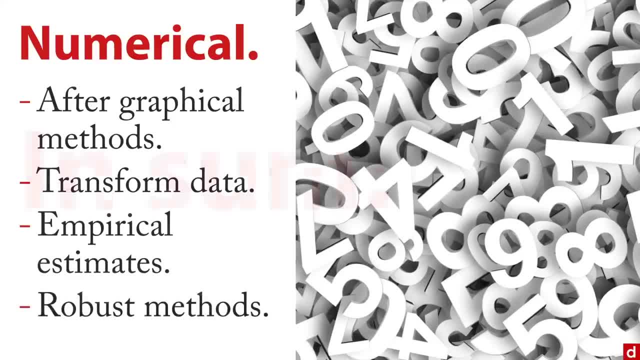 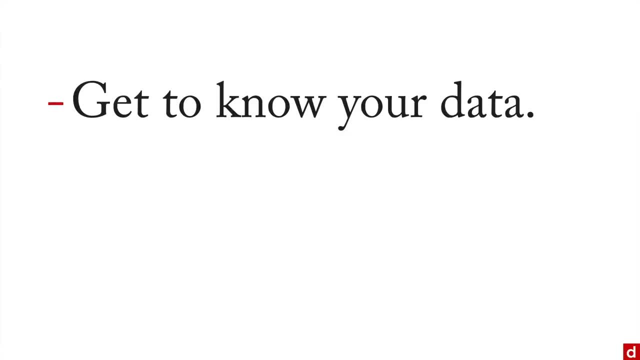 And I'll talk about all of those in more length in later videos, But for right now I can sum it up this way: The purpose of exploration is to help you get to know your data, And also you want to explore your data thoroughly before you start modeling it before you. 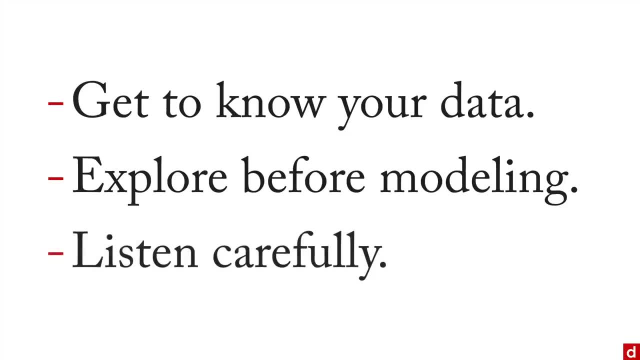 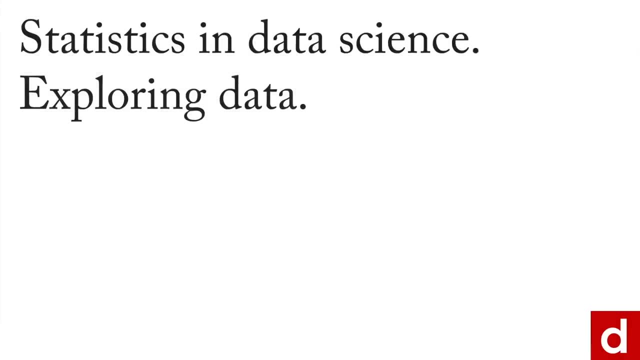 build statistical models And all the way through, you want to make sure you listen carefully so that you can find hidden or unassumed details and leads in your data. As we move in our discussion of statistics and exploring data, the single most important, 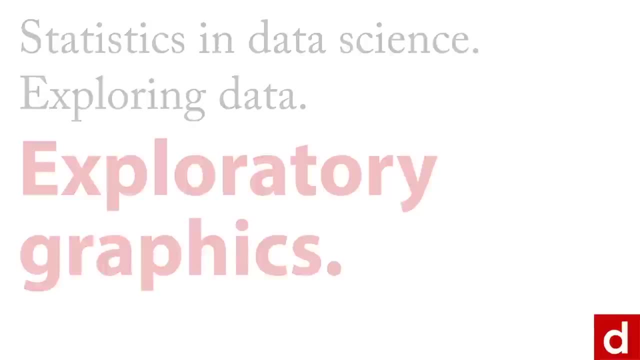 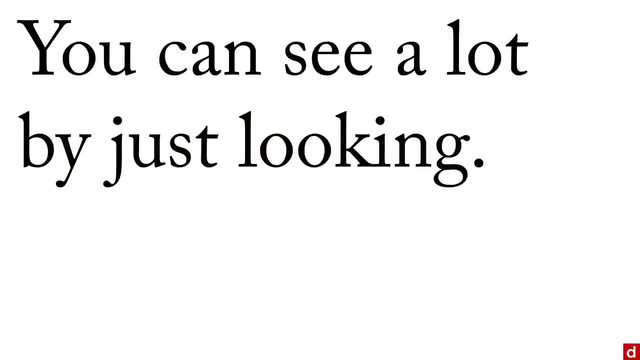 thing we can do is exploratory graphics. In the words of the late great Yankees catcher, Yogi Berra, You can see a lot by just looking. That applies to data as much as it applies to baseball. Now there's a few reasons you want to start with graphics. 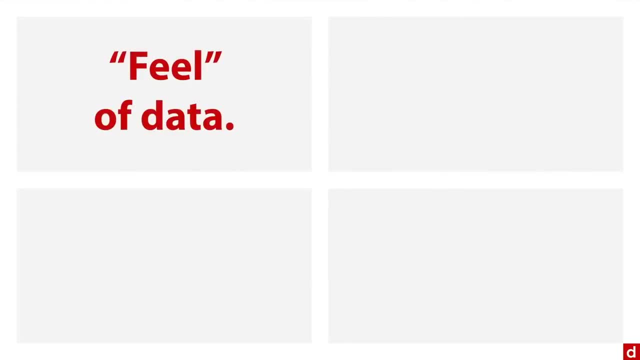 Number one is to actually get a feel for the data. I mean, what's it distributed like? What's the shape? Are there strange things going on? Also, it allows you to check the assumptions and see how well your data match the requirements. 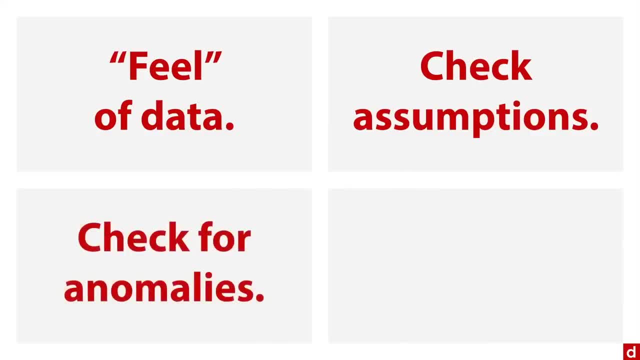 of the analytical procedures you hope to use. You can check for anomalies like outliers and unusual distributions, And you can also check for anomalies. And you can also check for anomalies like outliers and unusual distributions. And you can check for anomalies like outliers and unusual distributions. 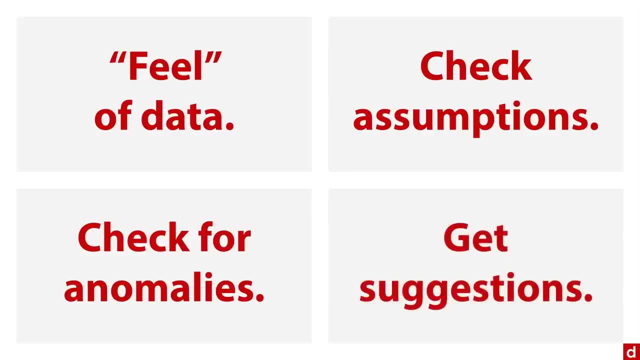 And you can also check for anomalies like outliers and unusual distributions. And you can also check for anomalies like outliers and unusual distributions. And you can also check for anomalies like outliers and unusual distributions. And also you can get suggestions. If something unusual is happening in the data, that might be a clue that you need to pursue. 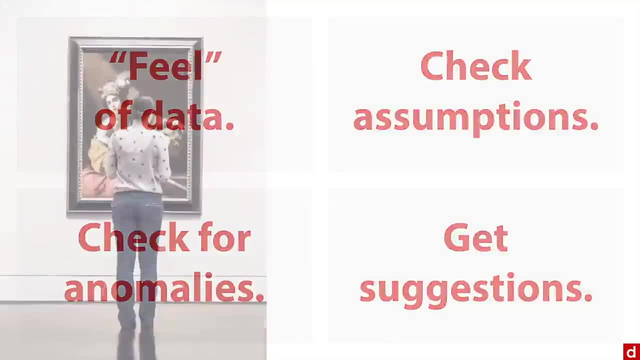 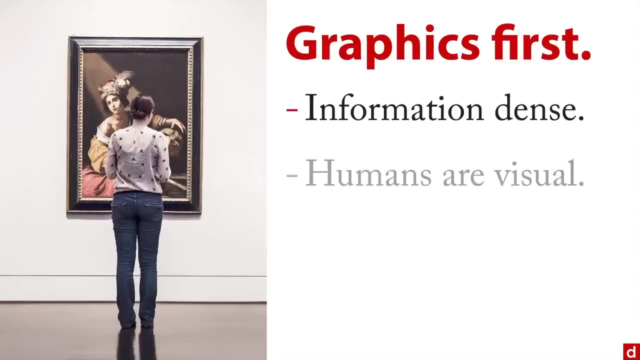 a different angle or do a deeper analysis. Now we want to do graphics first, for a couple of reasons. Number one is they're very information dense and fundamentally, humans are visual. It's our single highest bandwidth way of getting information. It's also the best way to check for shape and gaps and outliers. 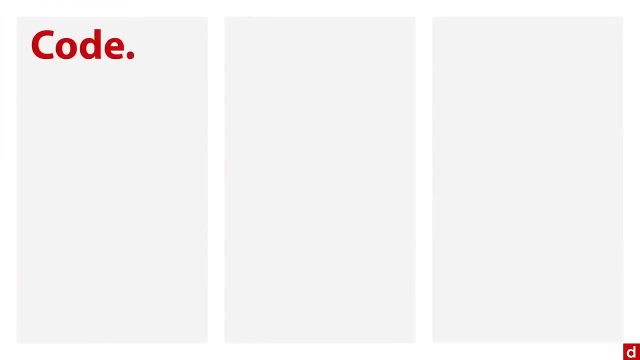 There are a few ways you can do this, if you want to. The first is with programs that rely on code, So you can use the statistical programming language R, the general purpose programming language, Python. You can actually do a huge amount in JavaScript, especially in D3.js. 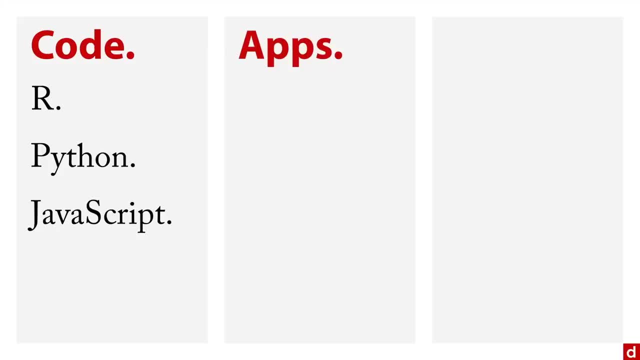 Or you can use apps that are specifically designed for exploratory analysis. That includes Tableau, both the desktop and the public versions, Qlik, and even Excel is a good way to do this. And then, finally, if you really want to know, you can do this by hand. 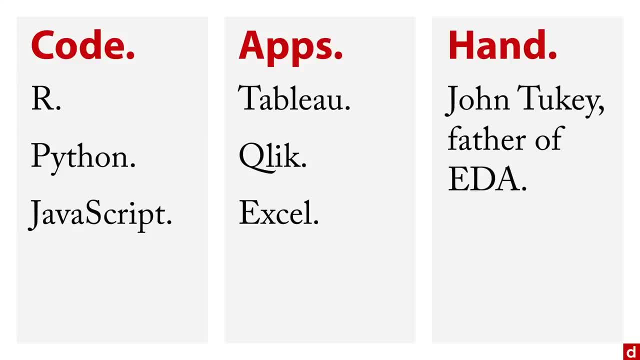 John Tukey, who's the father of exploratory data analysis, wrote his seminal book, a wonderful book where it's all hand graphs And actually it's a wonderful way to do it. But let's start the process for doing these graphics. 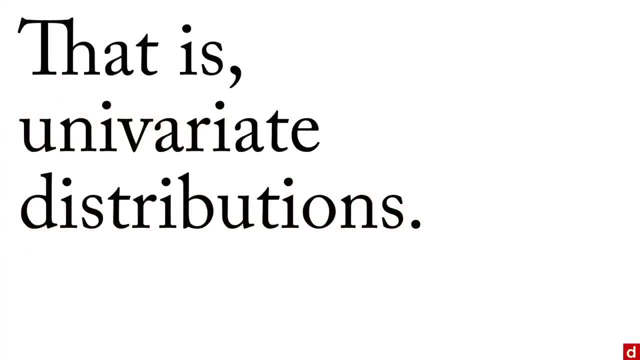 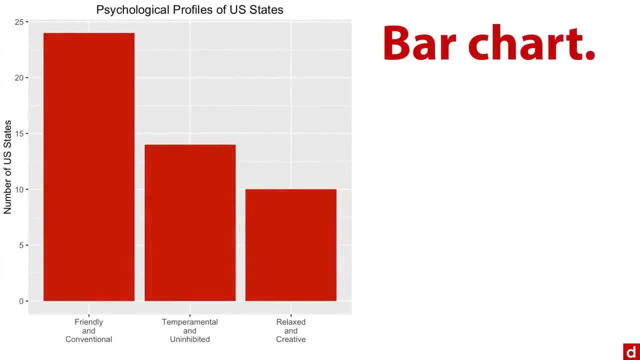 We start with one variable, that is, univariate distributions, And so you're going to get something like this: The fundamental chart is the bar chart. This is when you're dealing with categories and you're simply counting how many cases there are in each category. 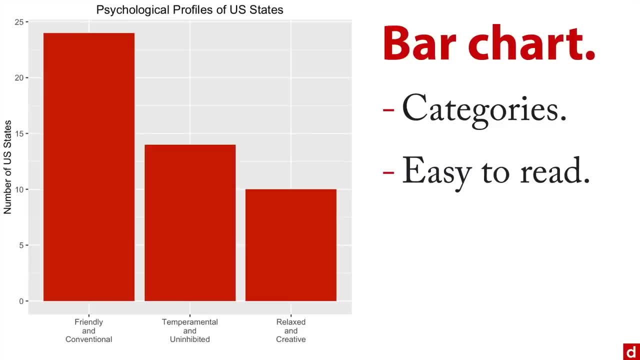 The nice thing about this, The nice thing about bar charts, is they're really easy to read. Put them in descending order and maybe have them vertical, maybe have them horizontal, Horizontal can be nice to make the labels a little easier to read. This is about psychological profiles of the United States. 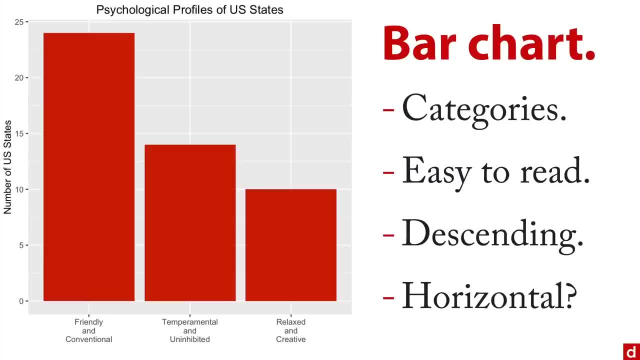 This is real data And that we have the most states in the friendly and conventional, a smaller number in temperamental and uninhibited, and the least common of the United States is relaxed and creative. Next you can do a box plot, or sometimes called a box and whisker. 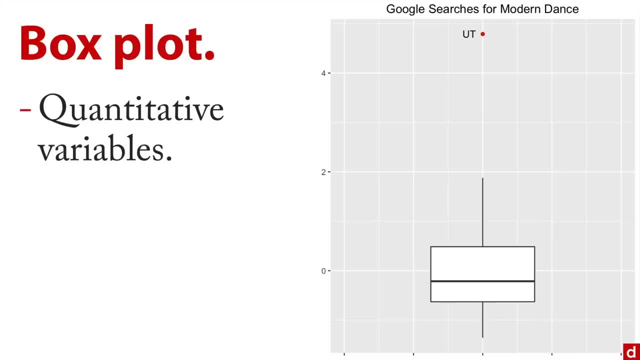 This is when you have a quantitative variable, something that's measured, and you can say how far apart scores are. A box plot shows quartile values. It also shows outliers. So, for instance, this is: Google searches for modern dance and that's Utah at five standard. 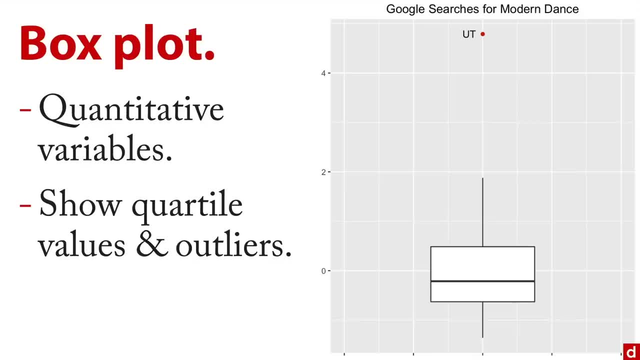 deviations above the national average. That's where I'm from And I'm glad to see that there also. it's a nice way to show many variables side by side If they're on proximally similar scales. next, if you have quantitative variables, you're. 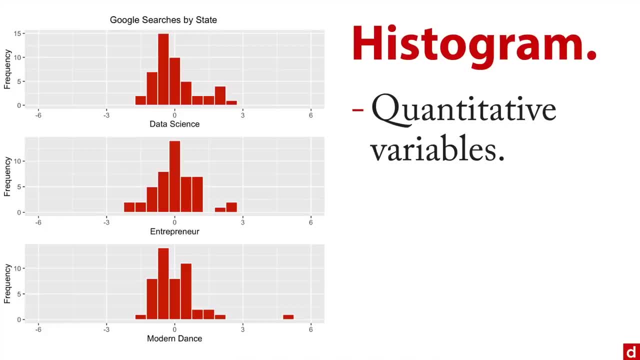 going to want to do a histogram, again quantitative, So interval or ratio, level or measured variables, and these let you see the shape of a distribution and potentially compare many. So here are three histograms for Google searches on data science and entrepreneur and modern dance. 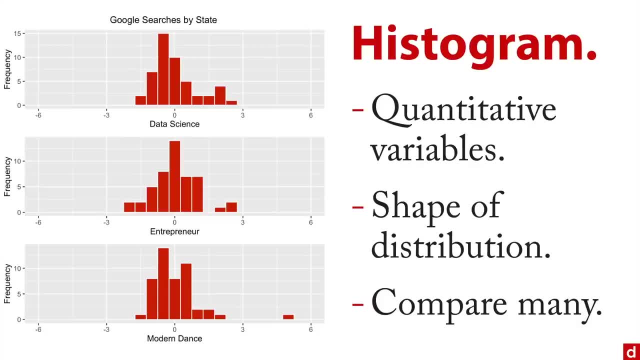 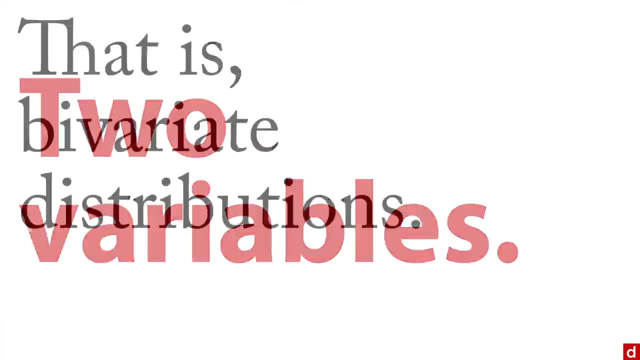 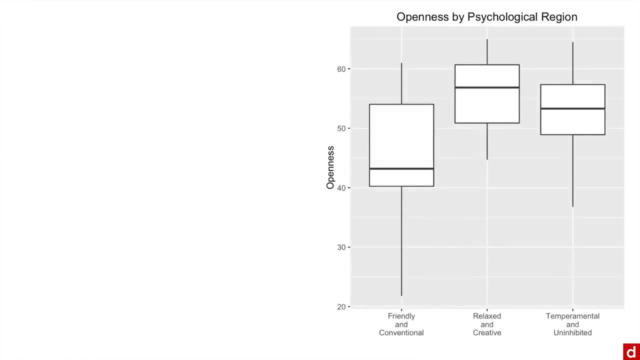 And you can see mostly for the part, normally distributed with a couple of outliers. Once you've done one variable or the univariate analysis, you're going to want to do two variables at a time, That is, bivariate distributions or joint. Now one easy way to do this is with grouped plots. 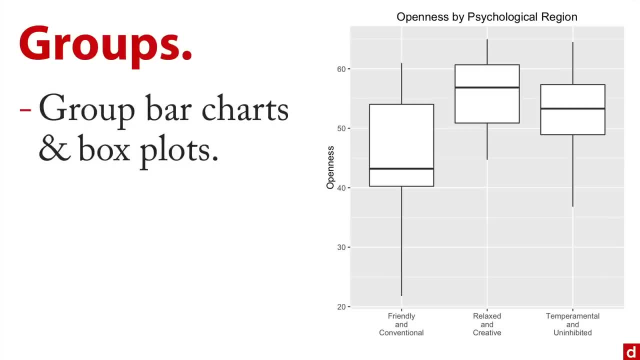 So you can do grouped bar charts and box plots. What I have right here is grouped box plots. I have my three regions- psychological regions of the United States- and I'm showing how they rank on openness. That's a psychological characteristic And what you can see is that the relaxing, creative or highest, and the friendly, conventional 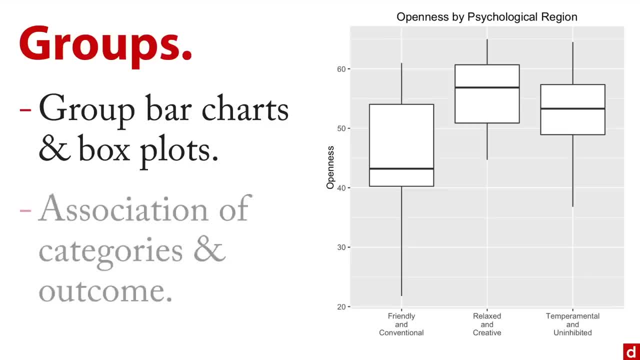 tend to go to the lowest, And that's kind of how that works. It's also a good way of seeing the association Between a categorical variable, like region of the United States psychologically, and a quantitative outcome, which is what we have here with openness. 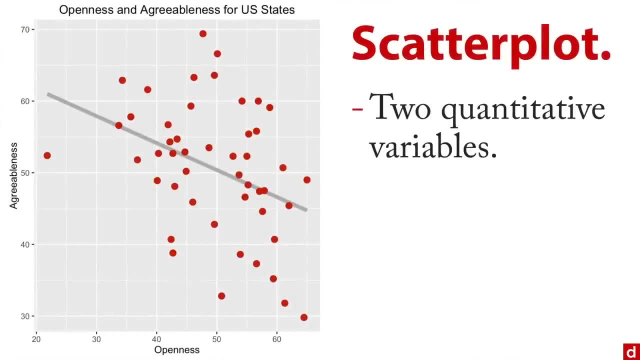 Next, you can also do a scatter plot. That's where you have two quantitative variables, And what you're looking for here is: is it a straight line? That is, is it linear? Do we have outliers? and also the strength of association. 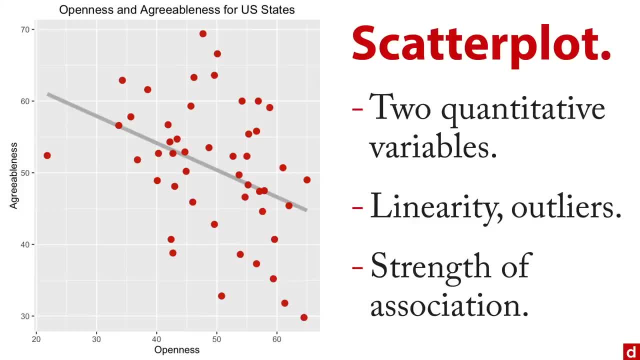 How closely do the dots all come to the regression line that we have here in the middle? And this is an interesting one For me because we have openness across the bottom, So more open as you go to the right and agreeableness. 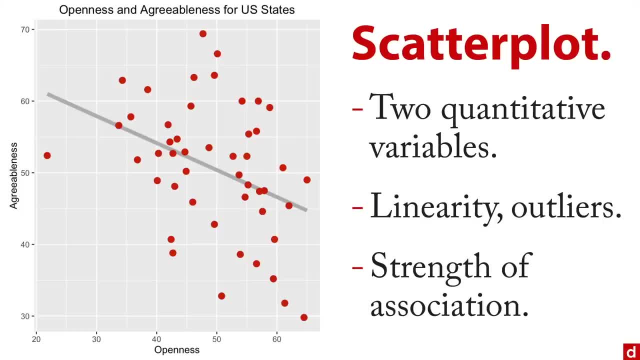 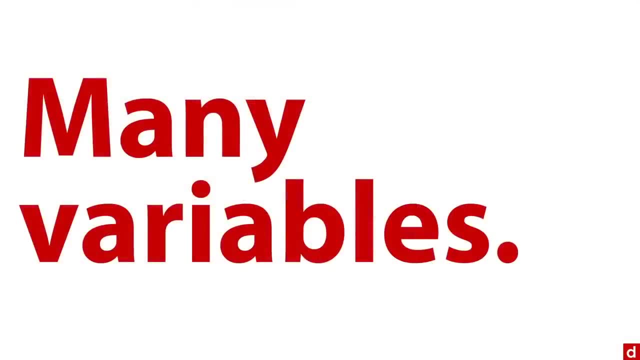 And what we see is there's a strong downhill association. The states in the United States that are the most open, apparently, are also the least agreeable, So we're going to have to do something about that. And then, finally, you want to go to many variables, that is, multivariate distributions. 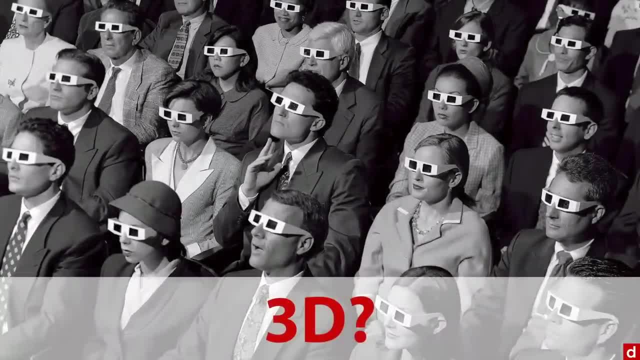 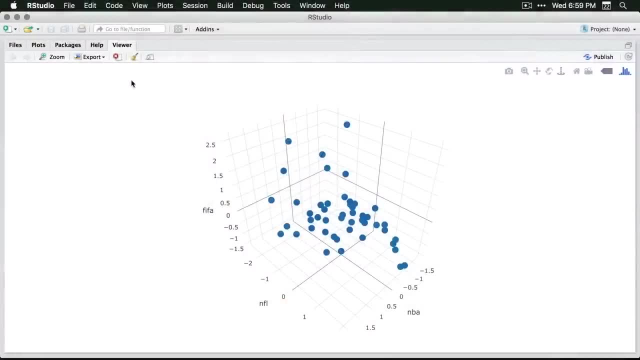 Now, one big question here is 3D or not 3D. Let me actually make an argument. I'm going to go over not 3D. So what I have here is a 3D scatter plot of three variables about Google searches. 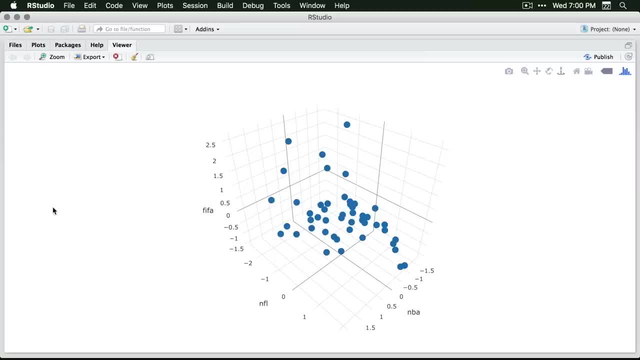 Up the left I have FIFA, which is for professional soccer Down there. on the bottom left, I have searches for NFL, and on the right I have searches for NBA. Now, I did this in R, and what's neat about this is you can click and drag and move it. 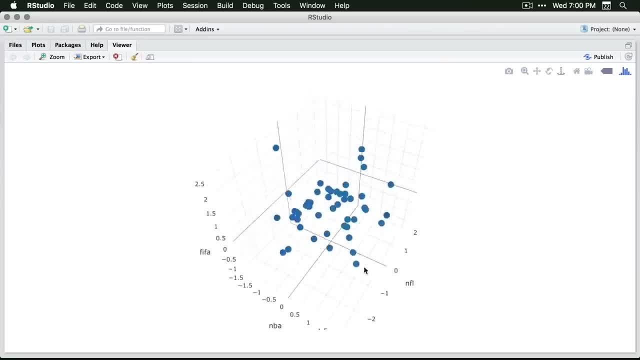 around And you know that's kind of fun. It kind of spin around and it gets kind of nauseating as you look at it. And this particular version I'm using Plotly in R allows you to actually click on a point. 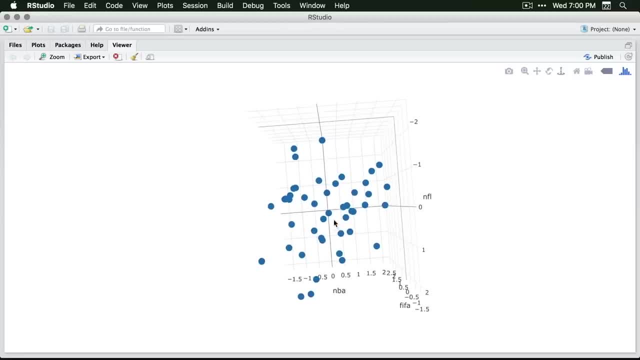 and see. let me see if I can get the floor in the right place. you got to click on a point and see where it ranks on each of these characteristics, You can see. however, this thing is hard to control and once it stops moving, it's not. 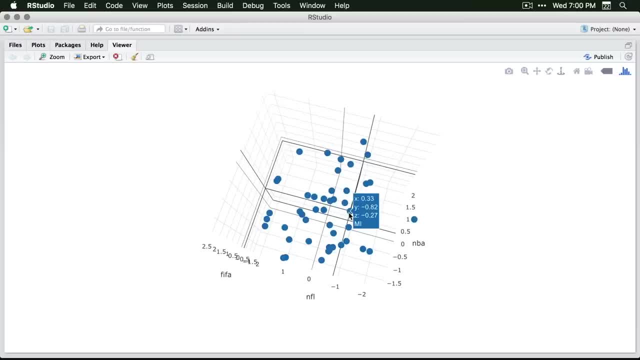 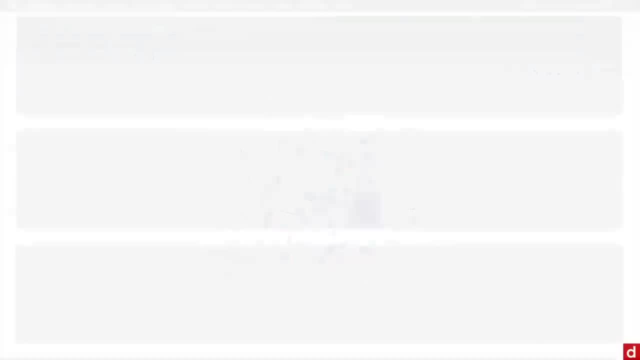 much fun And, truthfully, most 3D plots I've worked with are just kind of nightmares. They seem like they're a good idea, but not really. So here's the deal: 3D graphics like the one I just showed you, because they're actually 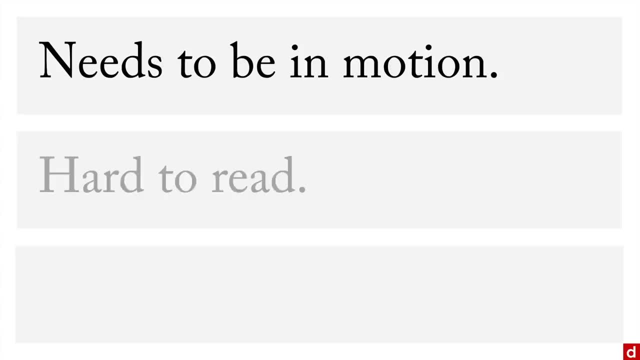 being shown in 2D. they have to be in motion for you to tell what's going on at all And fundamentally, they're hard to read and confusing. Now it's true, they might be useful for finding clusters in three dimensions. 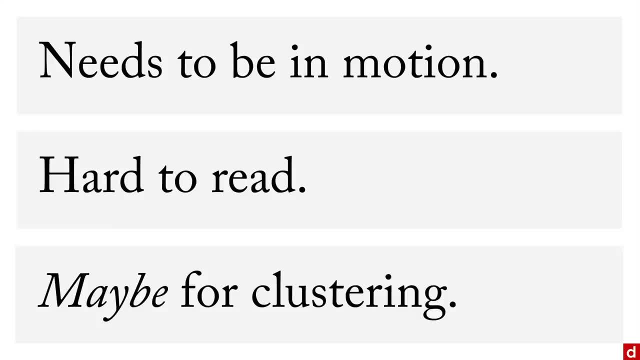 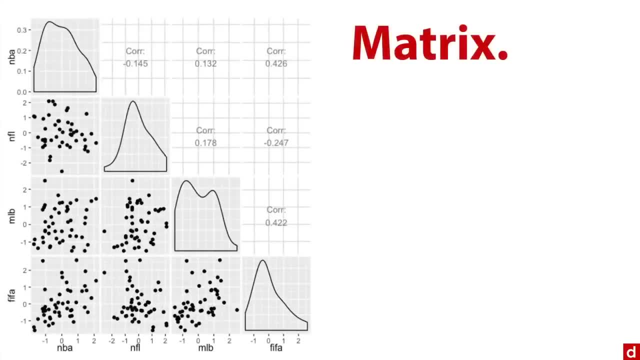 We didn't see that in the data we had, but generally, I just avoid them like the plague. What you want to do, however, is see the connection between several variables. You might want to use a matrix of plots. This is where you have, for instance, many quantitative variables. 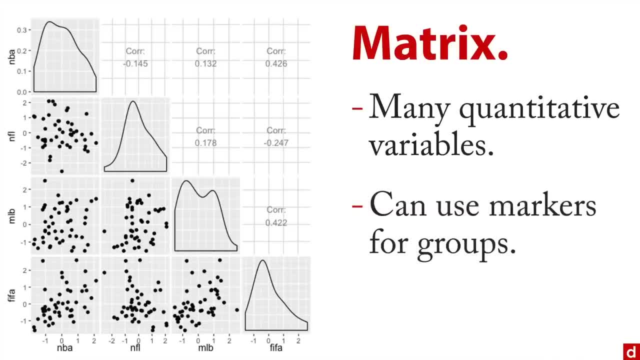 You can use markers for group membership if you want, And I find it to be much clearer than 3D. So here I have the relationship between four search terms: NBA, NFL, MLB for Major League Baseball- and FIFA. You can see the individual distributions, you can see the scatter plots you can get. 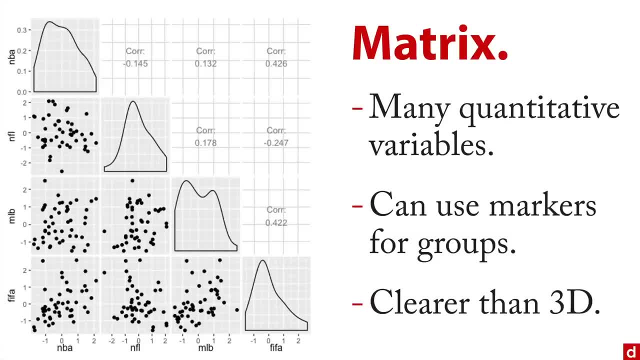 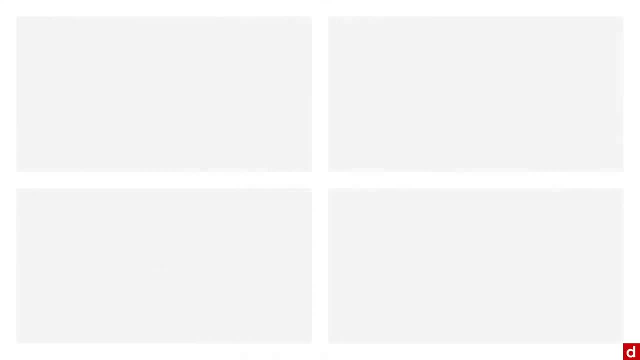 the correlation. Truthfully, this for me is a much easier kind of chart to read and get the richness that we need from a multidimensional display. So the questions you're trying to answer overall are number one: do you have what you need? 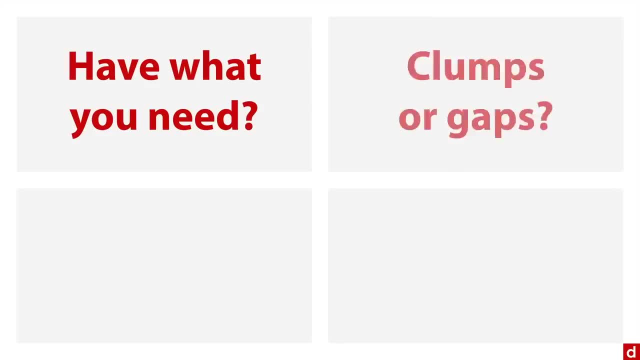 Do you have the variables you need? Do you have the variability that you need? Are there clumps or gaps in the distributions? Are there exceptional cases, anomalies that are really far out from everybody else, or spikes in the scores? And, of course, are there errors in data? 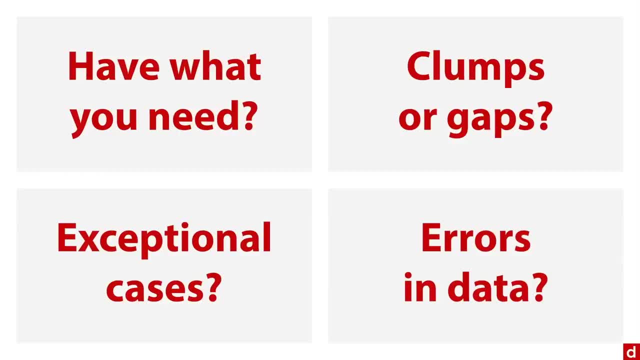 Were there mistakes in coding? Did people forget to answer questions? Are there impossible combinations? And these kinds of things are easiest to see with a visualization that really just kind of puts it right there in front of you, And so, in sum, I can say this about graphical exploration: 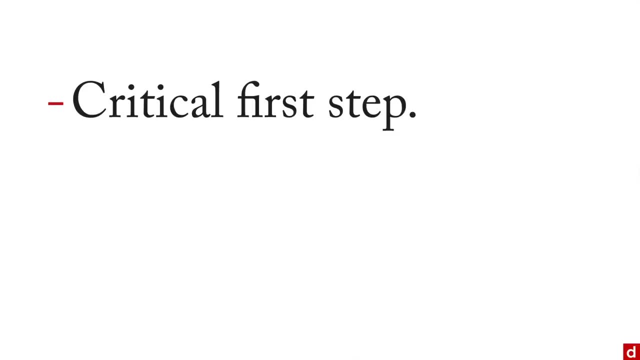 It's a critical first step. This is basically where you always want to start and you want to use the quick and easy methods. Again, bar charts, scatter plots are really easy to make and they're very easy to understand. And once you're done with the graphical exploration, then you can go to the second step, which 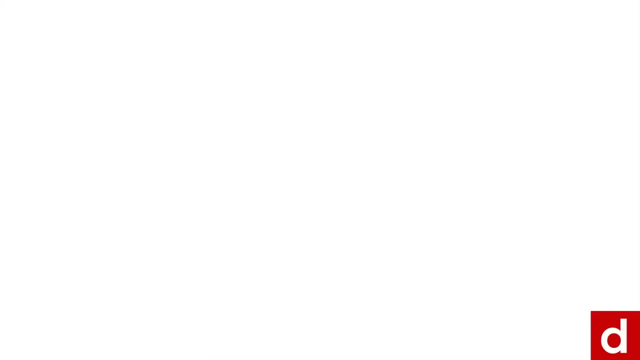 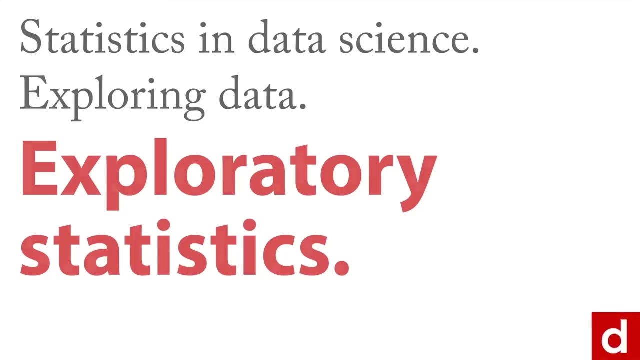 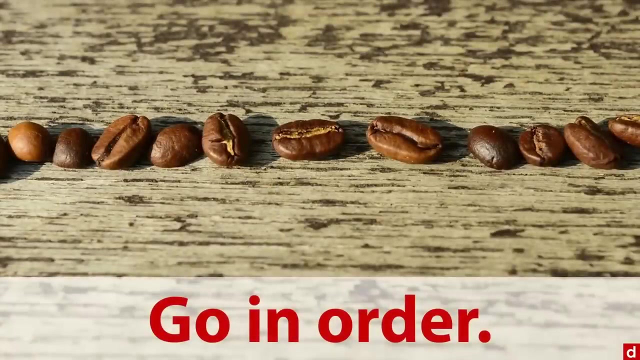 is exploring the data through numbers. The next step in statistics and exploring data is exploratory statistics, or numerical exploration of data. I like to think of this as go in order: First you do visualization, then you do the numerical part, And a couple of things to remember here. 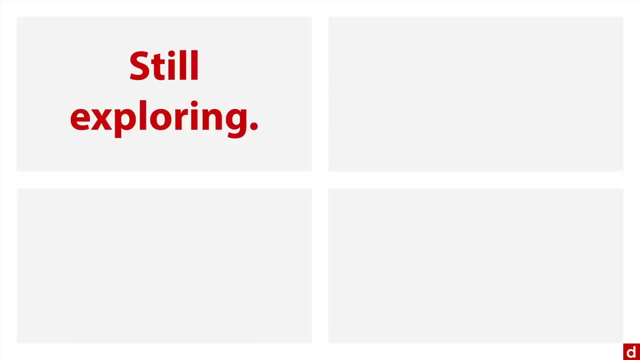 Number one is: you're still exploring the data. You're not modeling yet, but you are doing a quantitative exploration. This might be an opportunity to get empirical estimates, that is, of population parameters, as opposed to theoretically based ones. It's a good time to manipulate the data and explore the effects of manipulating the data. 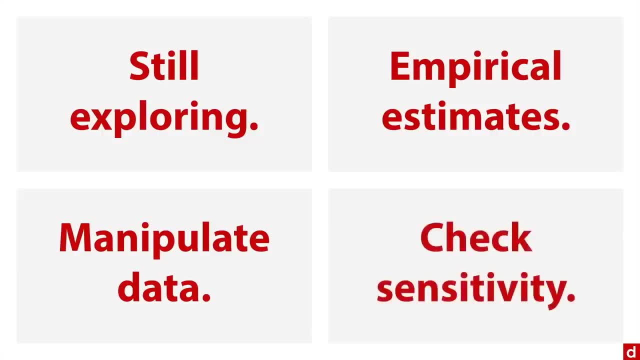 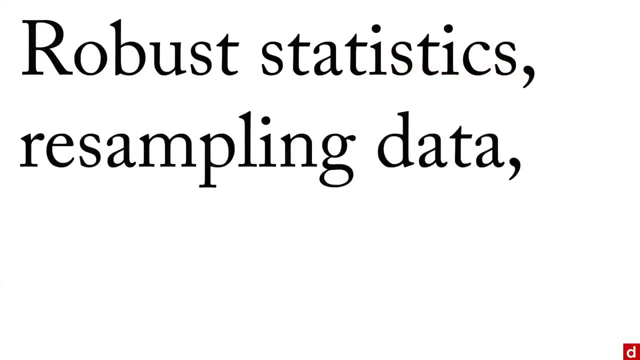 looking at subgroups, Looking at transforming variables. Also, it's an opportunity to check the sensitivity of your results. Do you get the same general results if you test under different circumstances? So we're going to talk about things like robust statistics and resampling data and transforming. 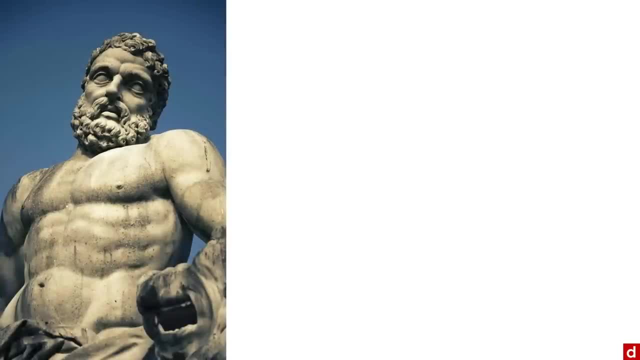 data. So we'll start with robust statistics. This, by the way, is Hercules, a robust mythical character, And the idea with a robust statistics is that they are stable. They are stable And that, even when the data varies in sort of unpredictable ways, you still get the same. 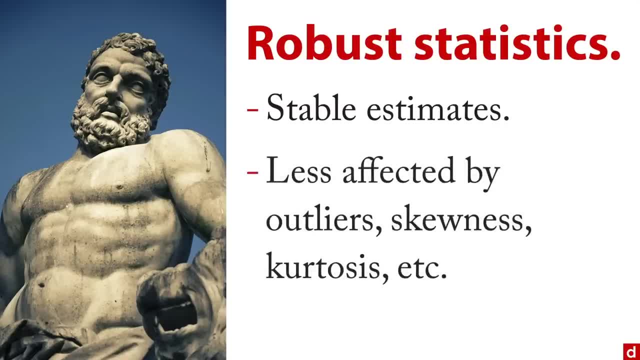 general impression. This is a class of statistics- it's an entire category that's less affected by outliers and by skewness and kurtosis and other abnormalities in the data. So let's take a quick look. This is a very skewed distribution I created 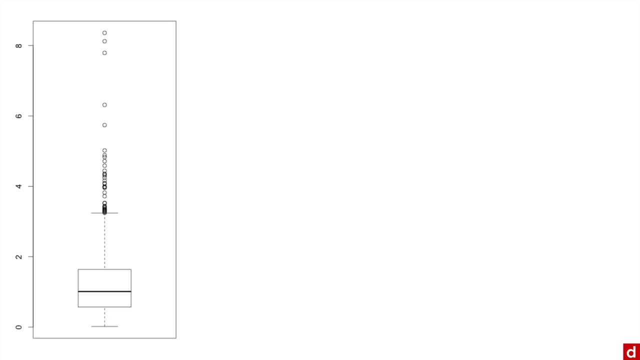 The median, which is the dark line there in the box, is right around one, And I'm going to look at two different kinds of robust statistics: The trimmed mean and the windsorized mean. With the trimmed mean you take a certain percentage of the data from the top and the 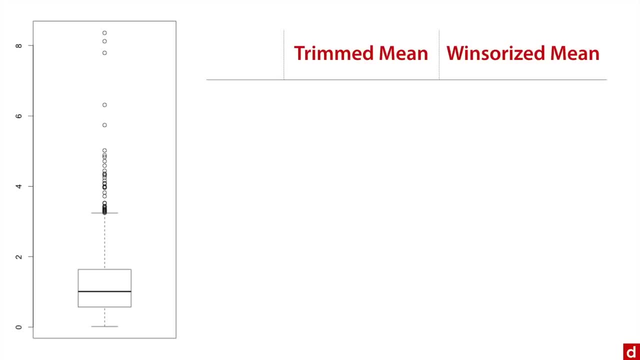 bottom and you just throw it away and you compute the mean for the rest With the windsorized. you take those and then you move those scores in to the highest non-outline score. Now the 0% is exactly the same as the regular mean and here it's 1.24.. 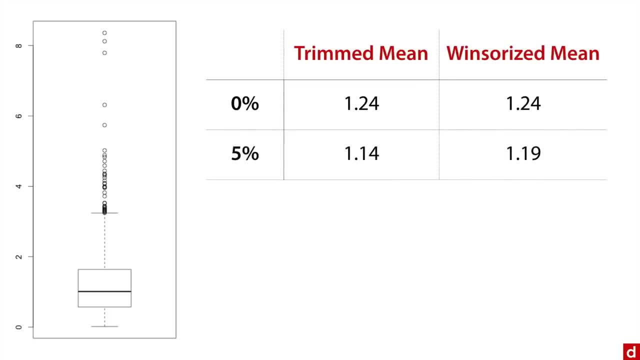 But as we trim off 5% or move in 5%, you can see that the mean shifts a little bit. then 10%, It comes in a little bit more To 25%. Now we're throwing away 50% of the data. 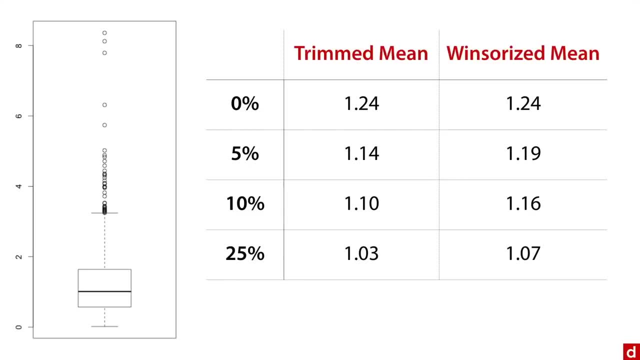 25% on the top, 25% on the bottom, And we get a mean here of 1.03, that's the trimmed mean- and a windsorized of 1.07.. When we throw away 50%, when we trim 50%, that actually means that we're leaving just 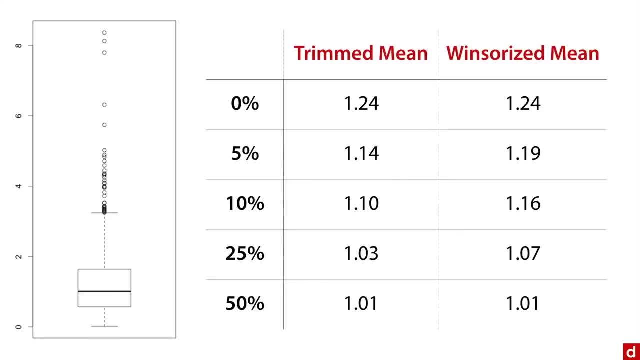 the median, Only the middle score is left. Then we get 1.01.. What's interesting is how close we get to that, even when we have 50% of the data left, And so that's an interesting example of how you can use robust statistics. 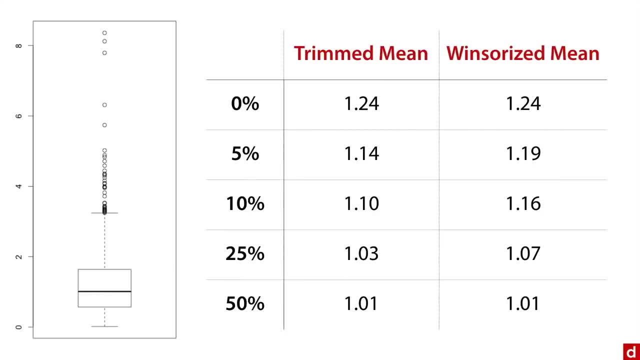 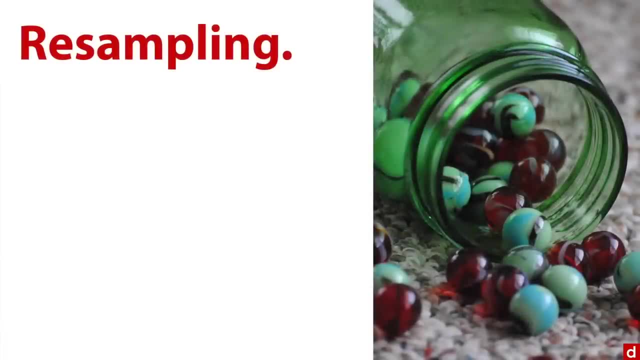 Robust statistics to explore data, even when you have things like strong skewness. Next is the principle of resampling, And that's like pulling marbles repeatedly out of a jar, counting the colors, putting them back in and trying again. That's an empirical estimate of sampling variability. 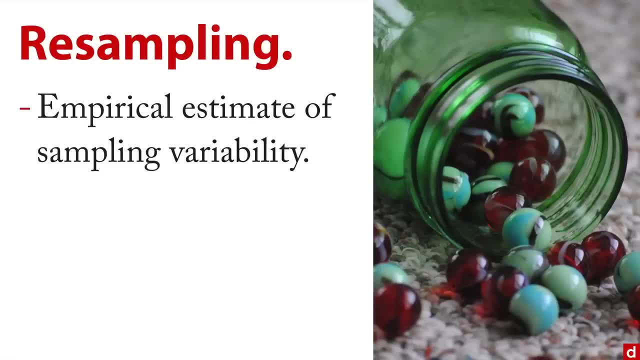 So sometimes you get 20% red marble, sometimes you get 30,, sometimes you get 22, and so on. There are several versions of this that go by the names, the jackknife and the bootstrap and the permutation And the basic principle of resampling is also key to the process of cross-validation. 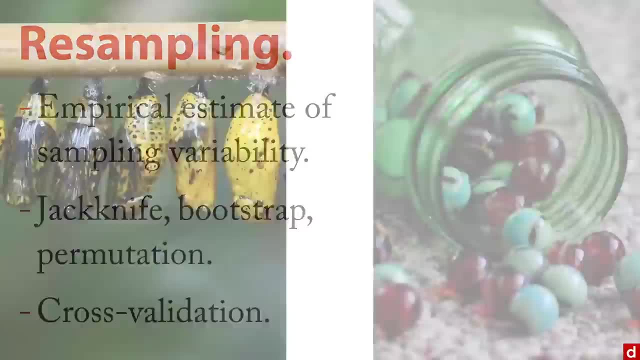 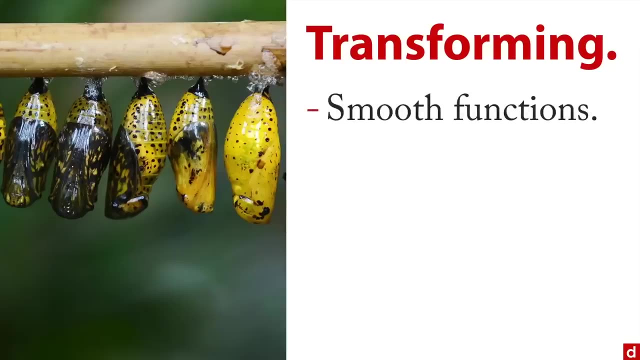 I'll have more to say about validation later. And then, finally, there's transforming variables. Here's our caterpillars in the process of transforming into butterflies. But the idea here is you take a sort of difficult data set and then you do what's called a smooth 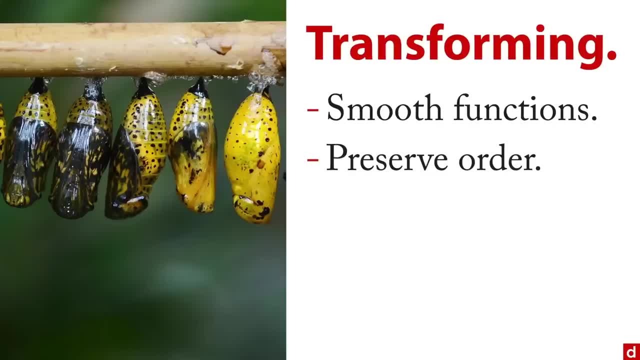 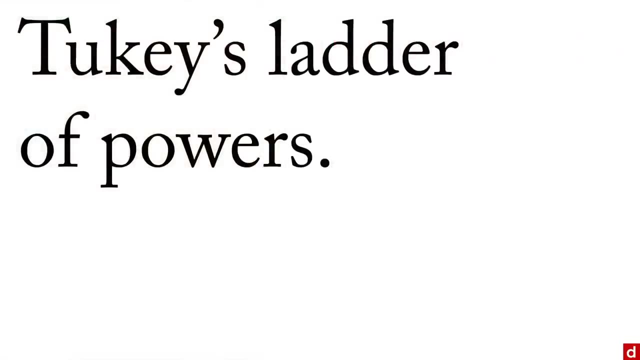 function- There's no jumps in it- And something that preserves the order and allows you to work on the full data set. If you have skewed data and in a scatterplot you might have a curved line, you can fix that, And probably the best way to look at this is with something called Tukey's ladder of. 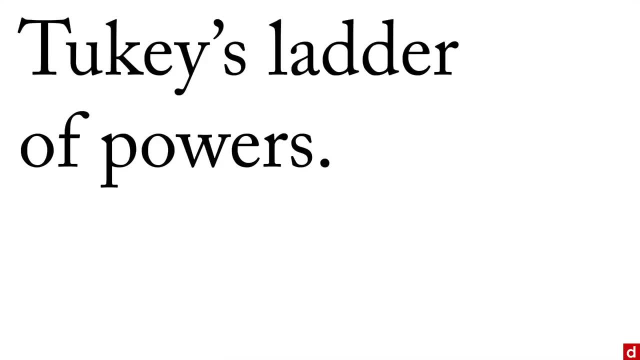 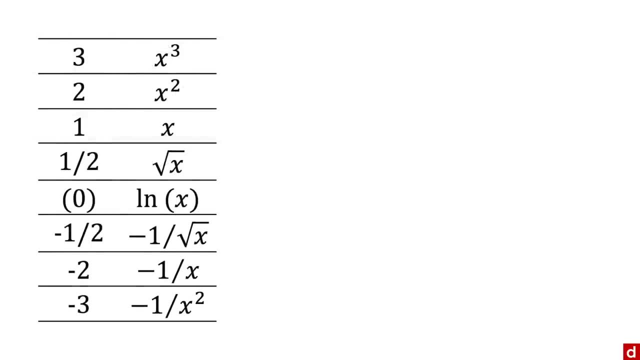 powers. I mentioned before John Tukey, the father of exploratory data analysis. He talked a lot about transformations. This is his ladder, starting at the bottom with the minus one over x, squared up to the top with his x cubed, And here's how it works. 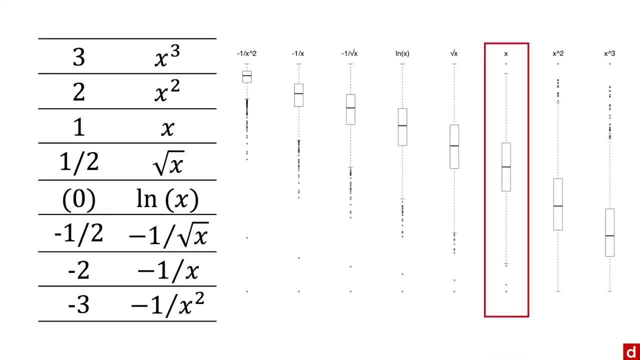 This distribution over here is a symmetrical network. It's a normally distributed variable And as you start to move in one direction and you apply the transformation, you take the square root. you see how it moves the distribution over to one end, Then the logarithm and you get to the end. you get this minus one over the square of 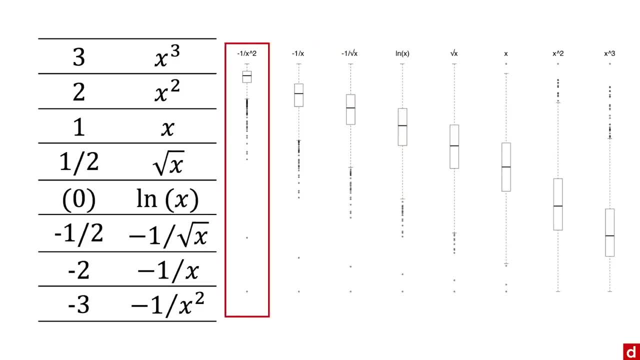 the score And that pushes it way, way, way over. If you go the other direction, for instance you square the scores, it pushes it down in the one direction. you cube it and then you see how it can move it around in ways that. 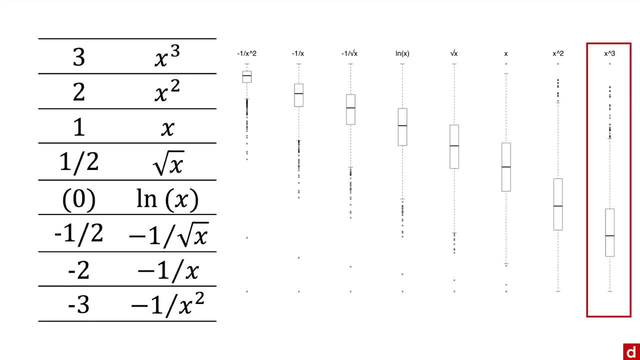 allow you to. you can actually undo this. You can undo the skewness to get back to a more centrally distributed distribution, And so these are some of the approaches that you can use in the numerical exploration of data. In sum, let's say this: 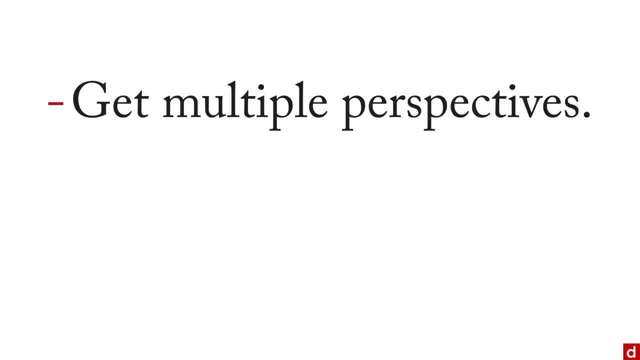 Statistical or numerical exploration allows you to get multiple perspectives on your data. It also allows you to check the stability, see how it works with outliers and skewness and mixed distributions and so on And, perhaps most importantly, it sets the stage for the statistical modeling of your 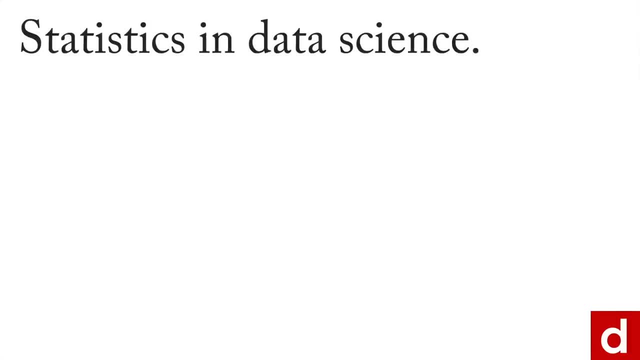 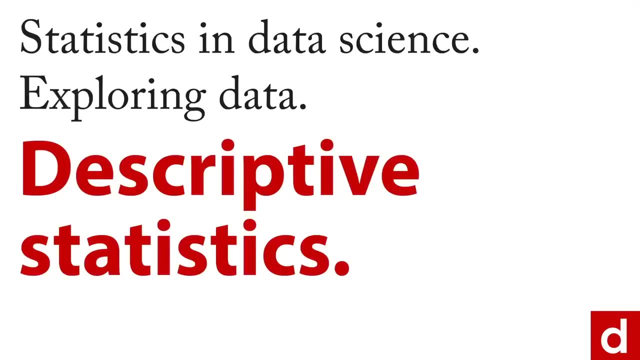 data. As a final step of statistics and exploring data, I'm going to talk about something that's not usually considered exploring, but is basic, descriptive statistics. I like to think of it this way: You've got some data and you are trying to tell a story. 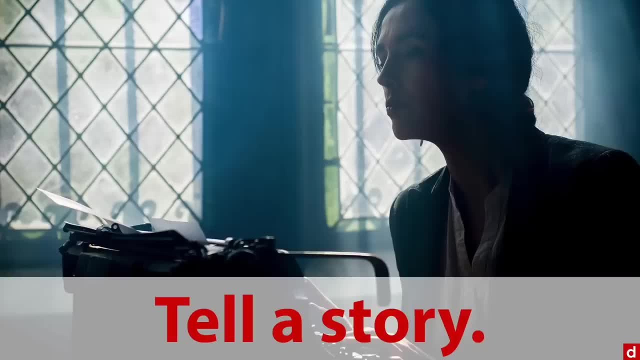 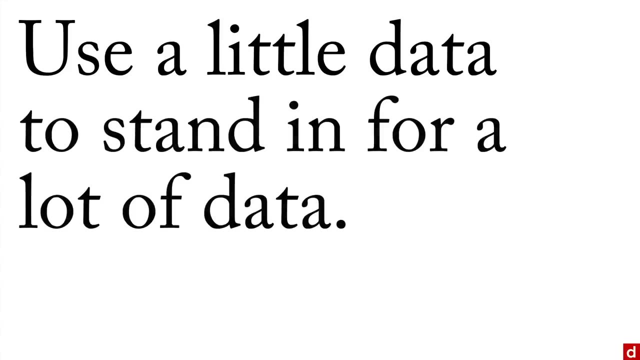 More specifically, you're trying to tell your data's story, And with descriptive statistics. you can think of it as trying to use a little data to stand in for a lot of data, using a few numbers to stand in for a large collection of numbers. 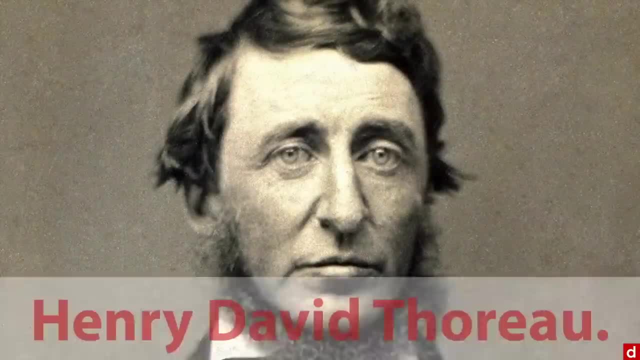 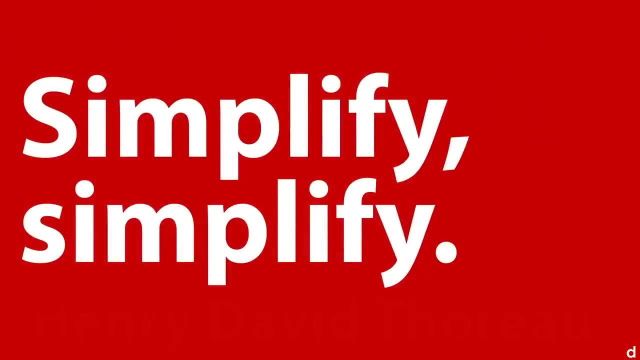 And this is consistent with a lot of data. And this is consistent with a lot of data, And this is consistent with the advice that we get from good old Henry David Thoreau, who told us: simplify, simplify. If you can tell your story with more carefully chosen and more informative data, go for it. 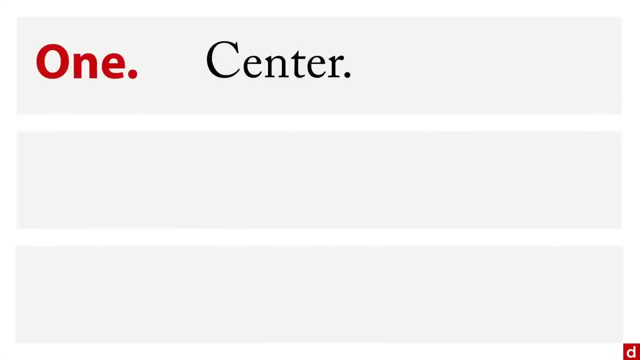 So there's a few different procedures for doing this. Number one: you want to describe the center of your distribution of data. That's, if you're going to pick a single number, use that. Two: if you can give a second number, give something about the spread or the dispersion. 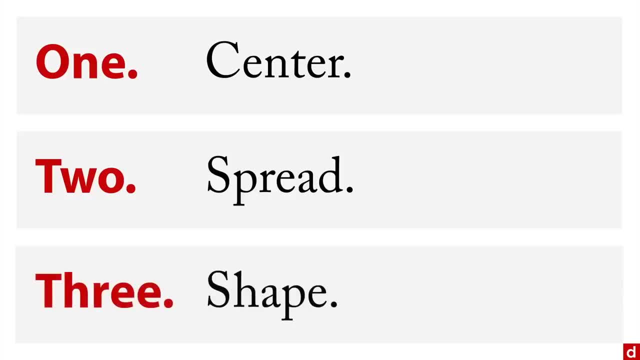 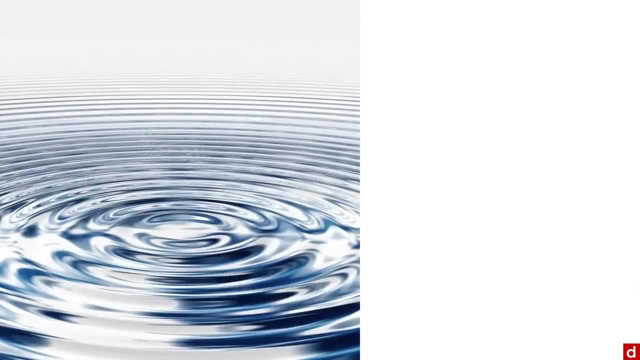 of the variability. it's also nice to be able to describe the shape of the distribution. Let me say more about each of these in turn. First, let's talk about center. We have the center of our rings here. Now there are a few very common measures of center, or location or central tendency of a distribution. There's: 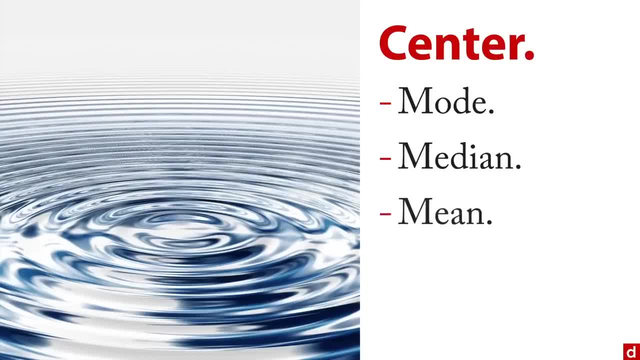 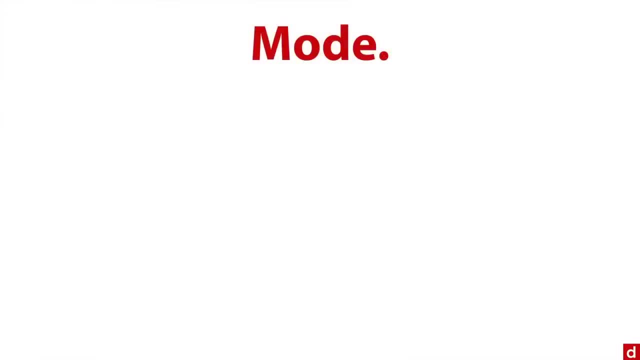 the mode, and there's the median and there's the mean. Now there are many, many others, but those are the ones that are going to get you most of the way. Let's talk about the mode first. Now I'm going to create a little data set here on a scale from 1 to 11, and I'm going to put individual 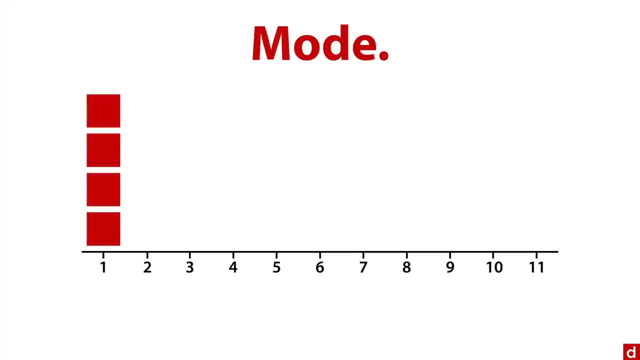 scores. There is a 1 and another 1, and another 1 and another 1.. Then we have a 2, 2,, then we have a score way over at 9 and another score over at 11.. So we have 8 scores, and this is the. 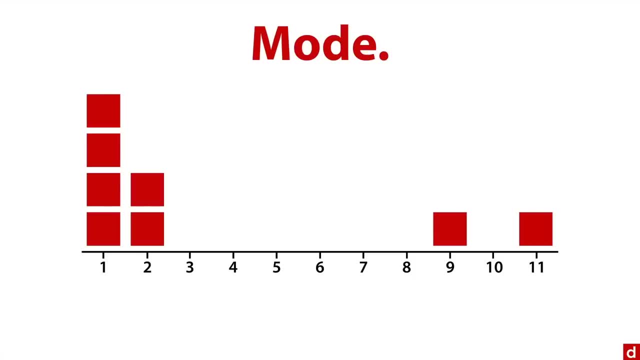 distribution. This is actually a histogram of the data set. The mode is the most commonly occurring score or the most frequent score. Well, if you look at how tall each of these go, we've got more ones than anything else, and so 1 is the mode because it occurs four times and nothing else. 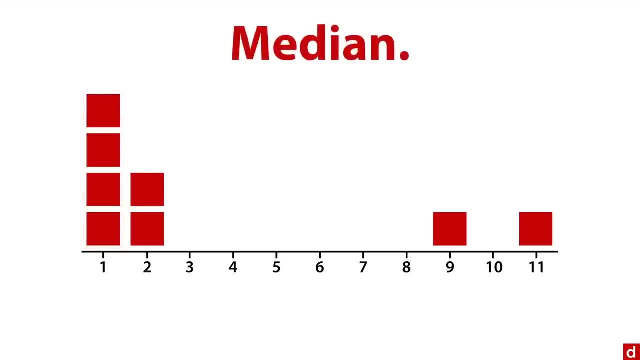 comes close to that. The median is a little different. The median is looking for the score that is at the center. if you split it into two equal groups, We have eight scores. so we want to get one group of four that's down here and then the other group of four. is this really big one? 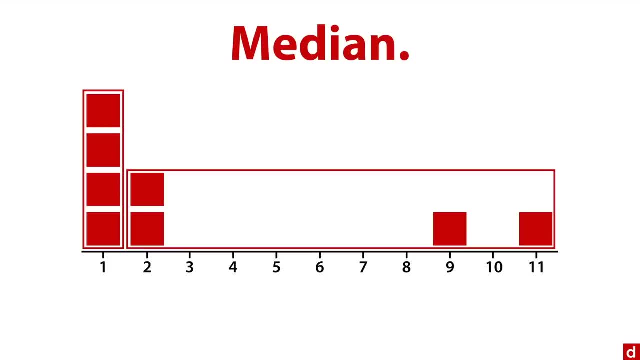 because it ranges way out and the median is going to be the place on the number line that splits those into two groups. That's going to be right here at one and a half. So that's going to be half. Now the mean is a little more complicated, even though people understand means in general. 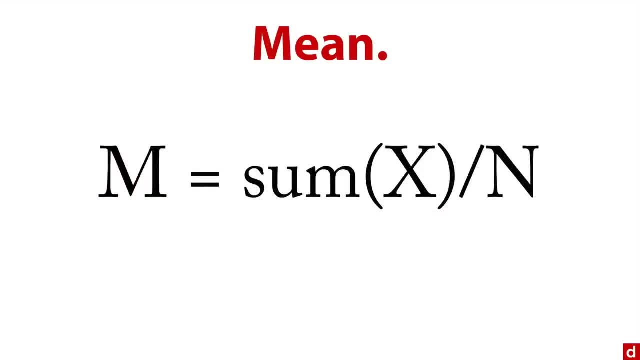 It's the first one we have here that actually has a formula where m for the mean is equal to the sum of x, that's our scores on the variable divided by n, the number of scores. You can also write it out with Greek notation, if you want, like this: where that's sigma, a capital sigma is the summation. 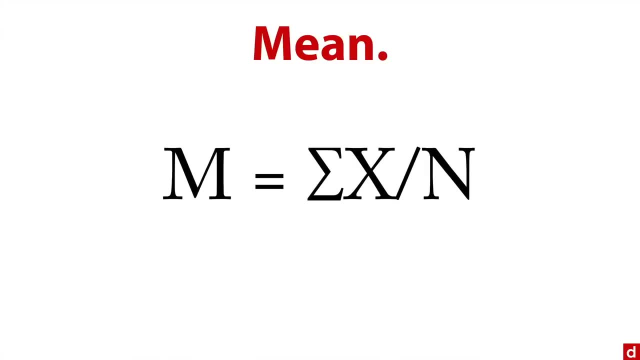 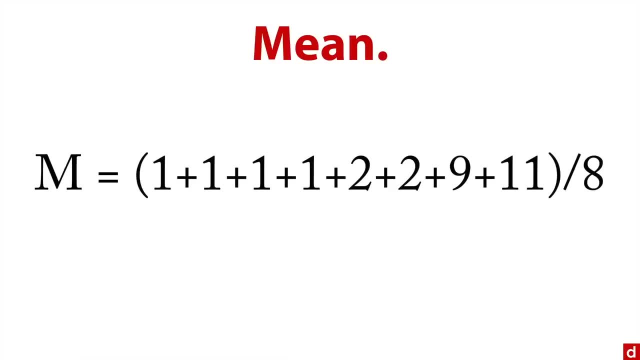 9 plus 11.. Add those all up and divide by 8, because that's how many scores there are. Well, that reduces to 28 divided by 8, which is equal to 3.5.. If you go back to our little chart here, 3.5 is: 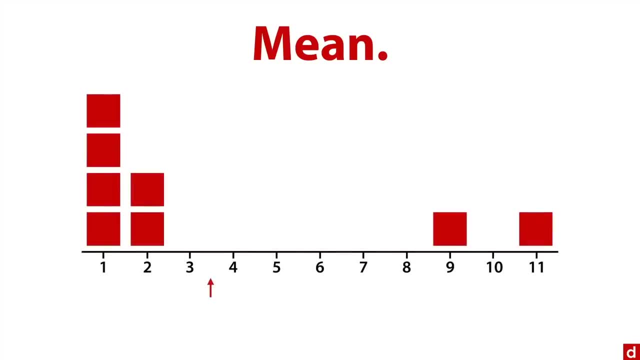 right over here. You'll notice there aren't any scores really exactly right there. That's because the mean tends to get very distorted by outliers. It follows the extreme scores. But a really nice- I say it's more than just a visual analogy- is that if this number line were a seesaw, 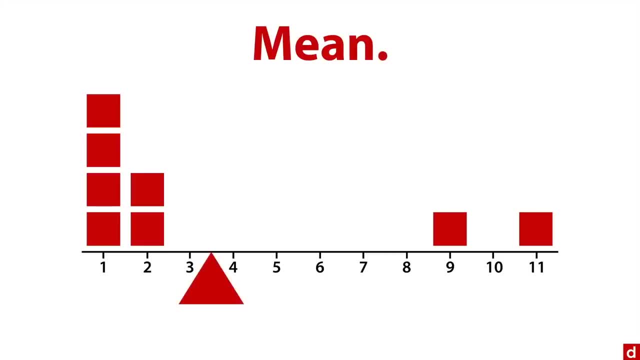 then the mean is exactly where the balance point or the fulcrum would be for these to be equal. People understand that If somebody weighs more, they've got to sit in closer to balance somebody who weighs less, who has to sit further out, And that's how the mean works. Now let me give a 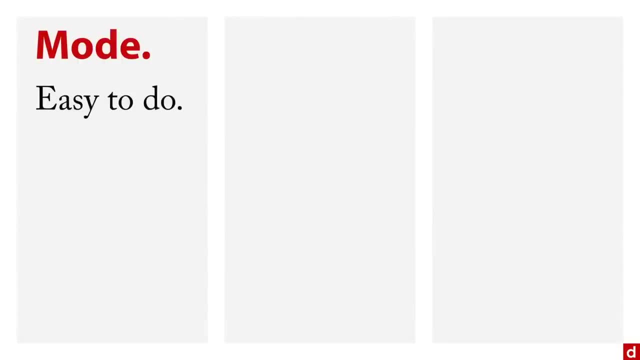 little bit of the pros and cons of each of these, For the mode. mode's really easy to do: You just count how common it is. On the other hand, it may not be close to what appears to be the center of the data. The median: it splits the data into two sets. The median: it splits the data into two sets. 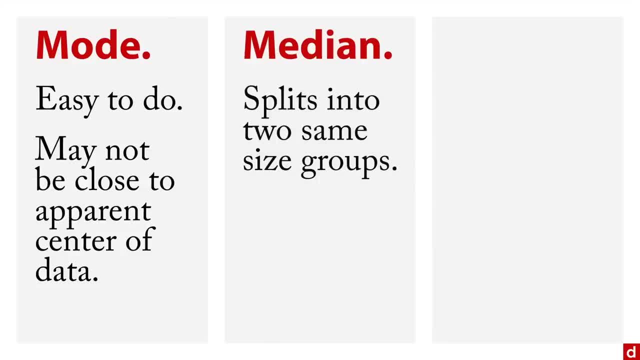 Same size groups, the same number of scores in each, And that's pretty easy to deal with. But unfortunately it's hard to use that information in many statistics after that. And then finally, the mean of these three is the least intuitive. It's the most effective by outliers and skewing. 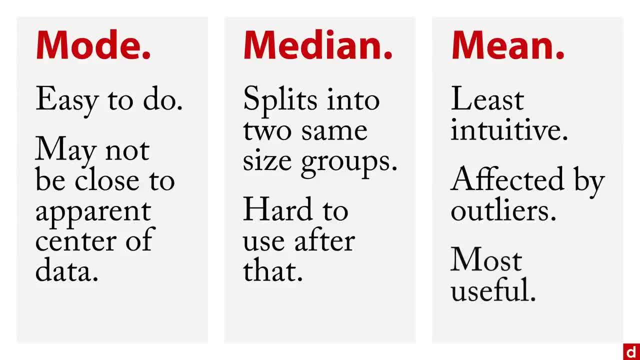 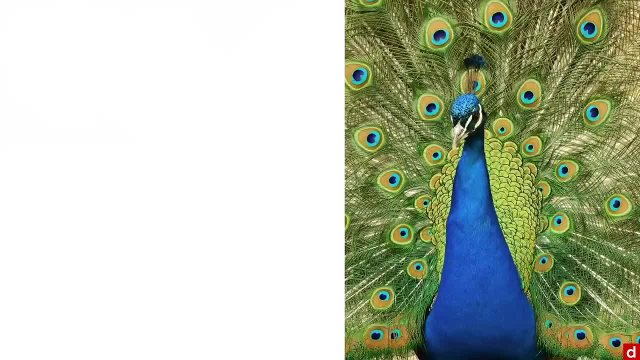 us, And that may really strike against it, But it is, however, the most useful statistically, And so it's the one that gets used the most often. Next, there's the issue of spread- spread your tail feathers, And we have a few measures here that are very common also. 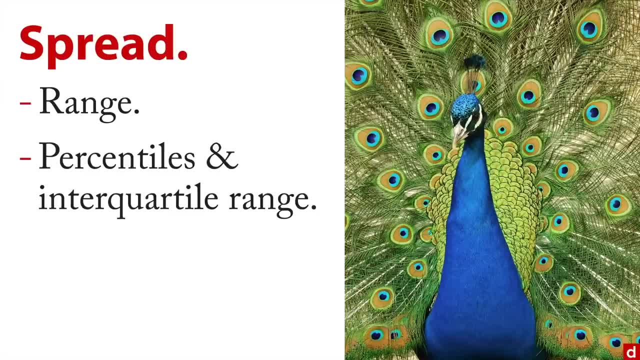 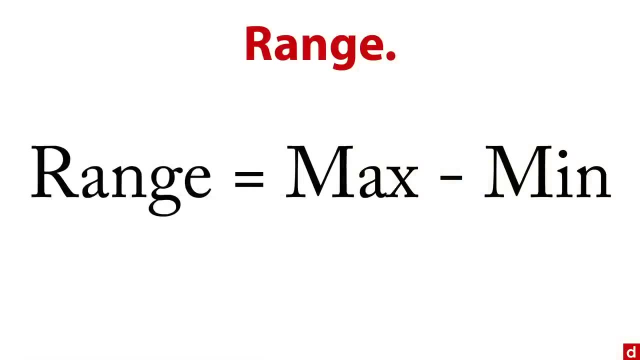 There's the range, There are percentiles and interquartile range And there's the variance and the standard deviation. I'll talk about each of those. First, the range. The range is simply the maximum score minus the minimum score, And in our case that's just 11 minus 1, which is equal. 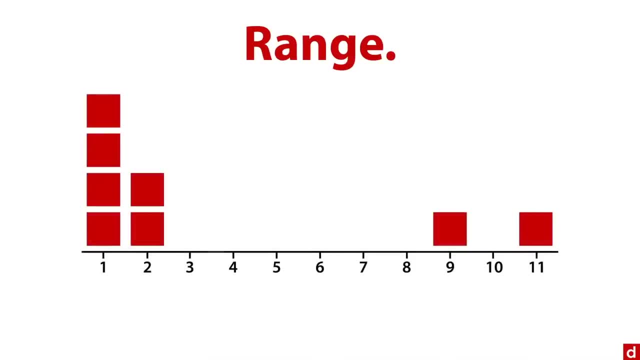 to 10.. So we have a range of 10. And I can show you that here on our chart It's just that line there at the bottom, from the 11 down to the 1. That's a range of 10.. The interquartile range. 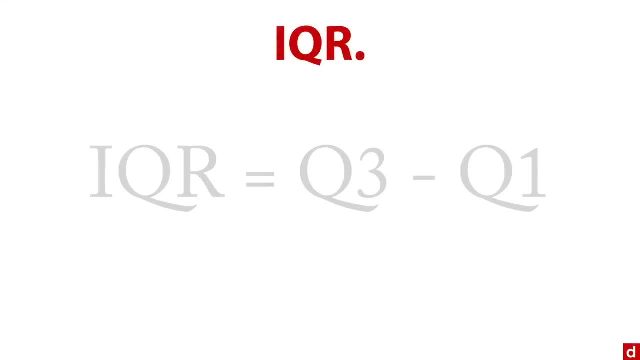 which actually is usually referred to simply as the IQR, is the distance between Q3,, which is the third quartile score, and Q1,, which is the first quartile score. If you're not familiar with quartiles, it's the same as the. 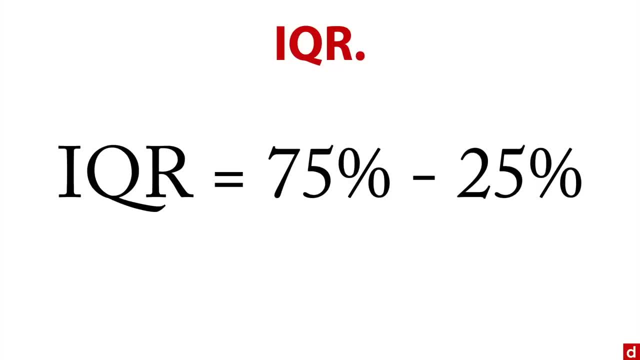 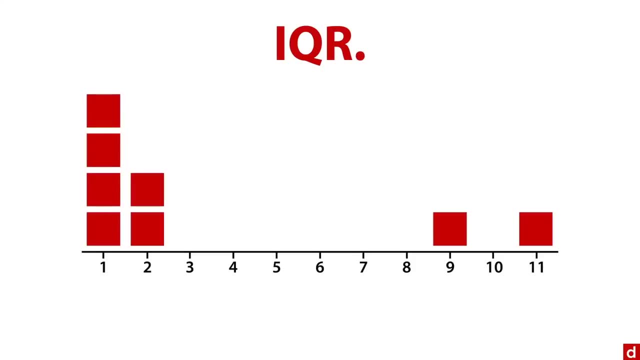 75th percentile score and the 25th percentile score. Really, what it is is you're going to throw away some of the data, So let's go to our distribution here. First thing we're going to do is we're going to throw away the two highest scores. There they are, They're grayed out now. 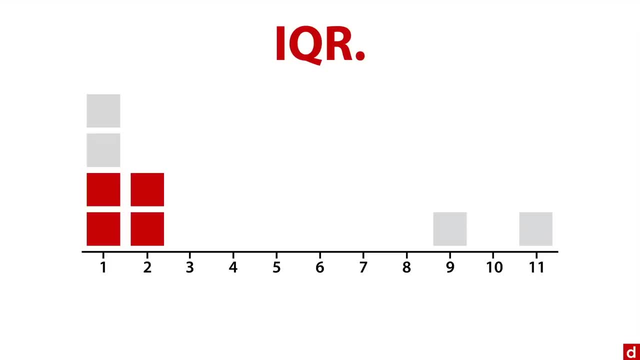 And then we're going to throw away two of the lowest scores. They're out there, And then we're going to get the range for the remaining ones. Now, this is complicated by the fact that I've got this big gap in between 2 and 9.. And different methods of calculating quartiles. 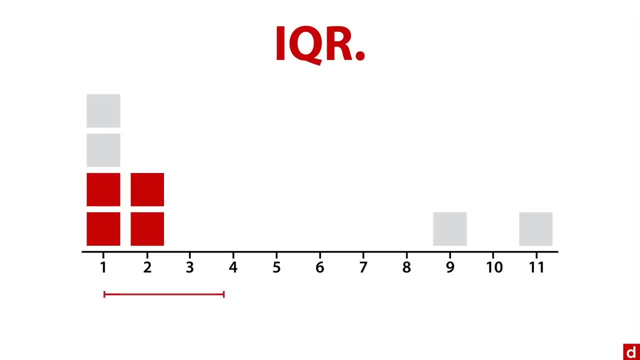 do something with that gap. So if you use a spreadsheet, it's actually going to do an interpolation process And it will give you a value of 3.75, I believe, and then down to 1 for the first quartile. So not so intuitive with this graph, but that is how it works usually. 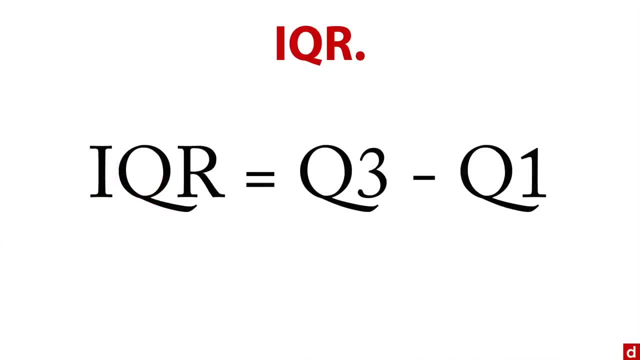 If you want to write it out, you can do it like this: The interquartile range is equal to Q3 minus Q1.. And in our particular case, that's 3.75 minus 1. And that, of course, is equal to just 2.75.. And there you have it. 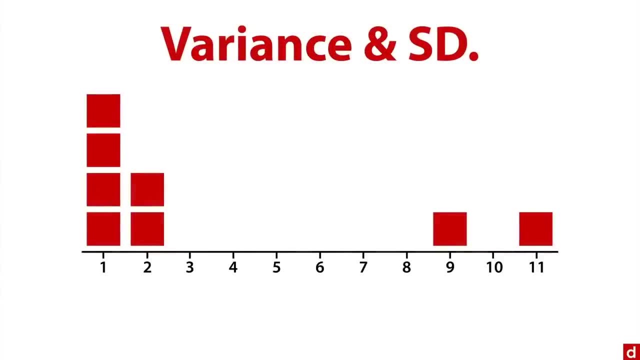 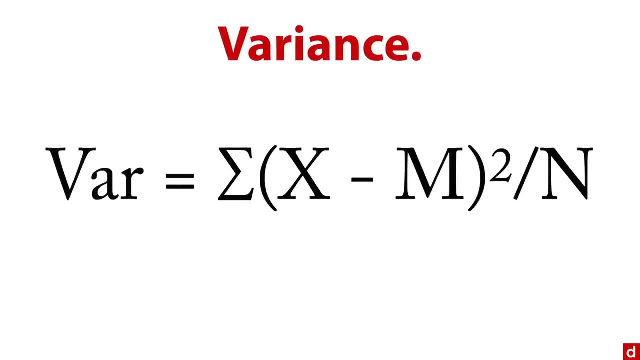 Now our final measure of spread, or variability, or dispersion, is two related measures: the variance and the standard deviation. These are a little harder to explain and a little harder to show, But the variance, which is at least the easiest formula, is this: The variance is equal to: 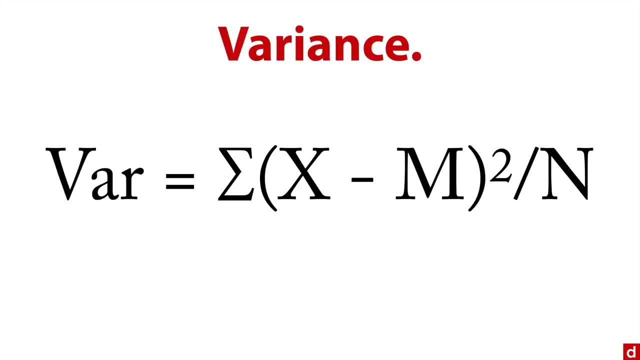 that's the sum. the capital sigma is the sum of X minus M. That's how far each individual score is from the mean. And then you take that deviation there and you square it. you add up all the deviations and then you divide by the number. So the variance is the average square deviation. 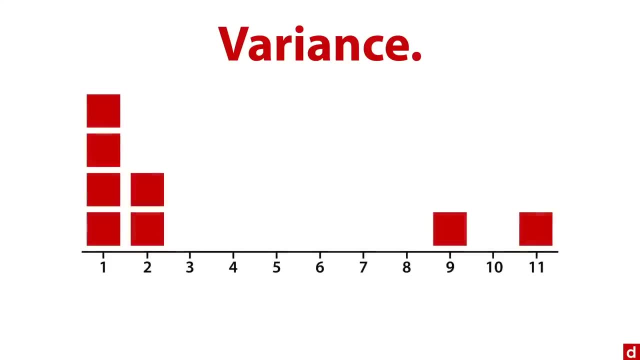 from the mean. I'll try to show you that graphically. So here's our data set And there's our mean, right there at 3.5.. Let's go to one of these twos: We've got a deviation and we've got a. 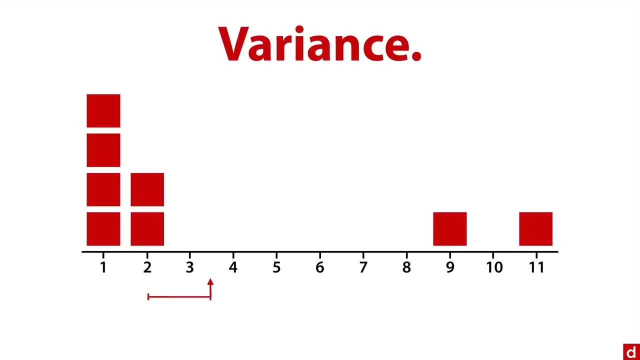 deviation there of 1.5.. And if we make a square, that's 1.5 points on each side. well, there it is. We can do a similar square for the other score at 2.. If we're going down to 1, then it's going to be. 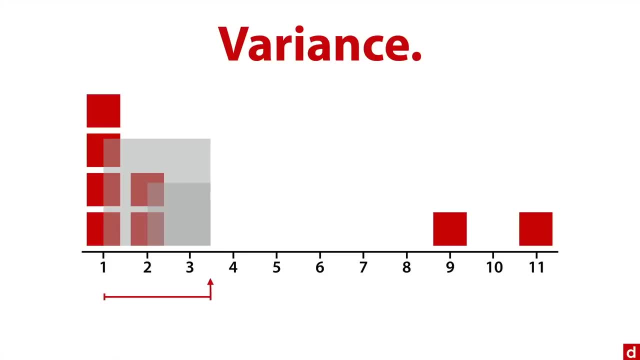 2.5 squared and it's going to be that much bigger And we can draw one of these squares for each of our eight points. The squares for the scores at 9 and 11 are going to be huge and go off the page so I'm not going to show them. But once you have all those squares, you add up the area. 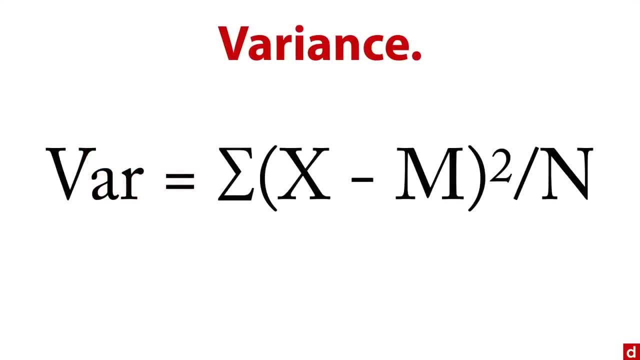 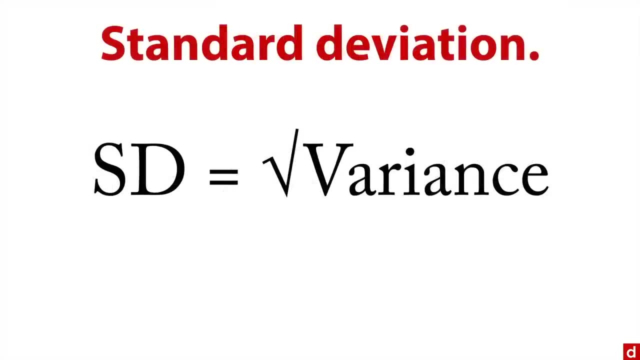 and you get the variance. So this is the formula for the variance. But now let me show the standard deviation, which is also a very common measure. It's closely related to this Specifically. it's just the square root of the variance. Now there's a catch here. The formulas for the 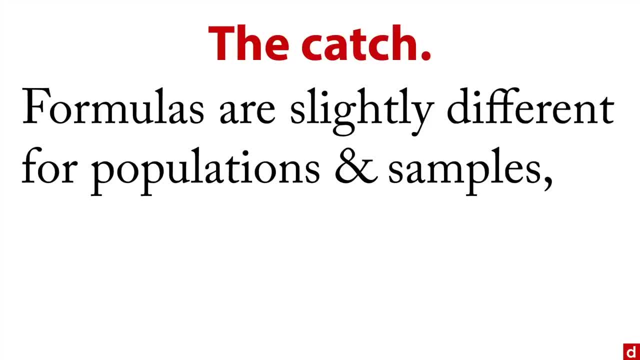 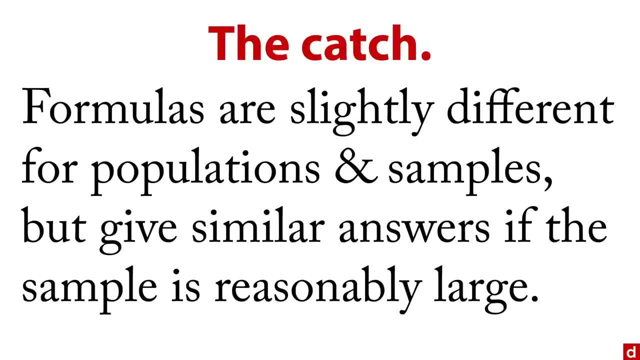 variance and the standard deviation are slightly different for populations and samples in that they use different denominators, But they give similar answers- not identical but similar. if the sample is reasonably large, say over 30 or 50,, then it's going to be really just a negligible. difference. So this is the formula for the variance. But now let me show the standard deviation, which is also a very common measure. So this is the formula for the variance. But now let me show the standard deviation, which is also a very common measure. So this is the formula for the variance. 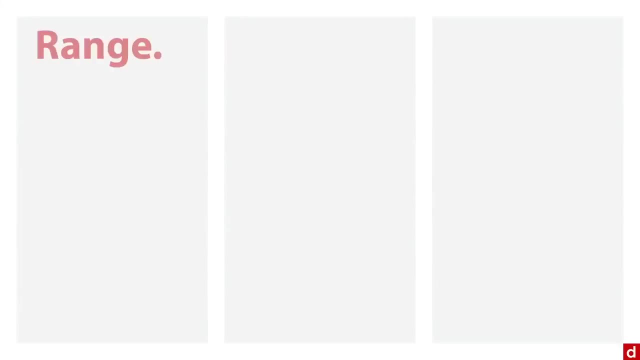 So let's do a little pro and con of these three things. First, the range. It's very easy to do. It only uses two numbers, the high and the low, But it's determined entirely by those two numbers And if they're outliers you've got really a bad situation. The interquartile range, or IQR. 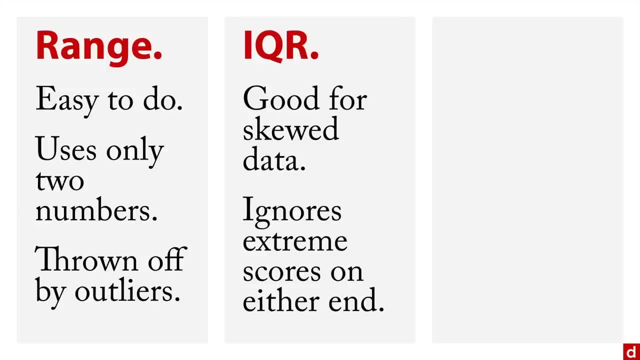 it's really good for skewed data, And that's because it ignores extremes on either end, So that's nice. And the variance and the standard deviation: while they are the least intuitive and they are the most affected by outliers, they are also generally the most effective, So that's. 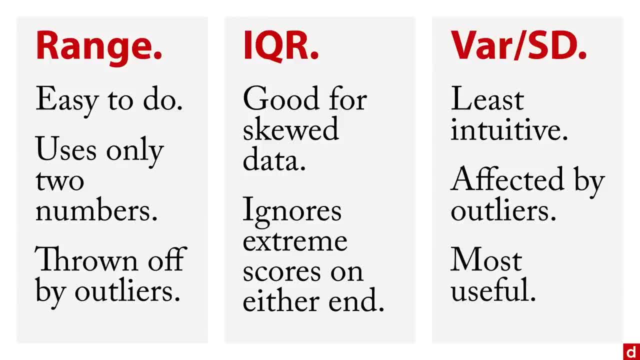 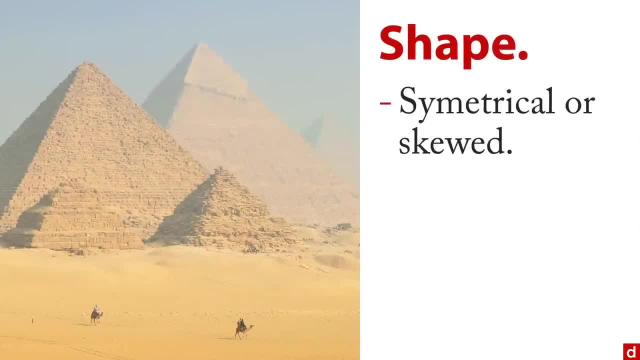 the most useful because they feed into so many other procedures that are used in data science. Finally, let's talk a little bit about the shape of a distribution. You can have symmetrical or skewed distributions, unimodal, uniform or U-shaped. You can have 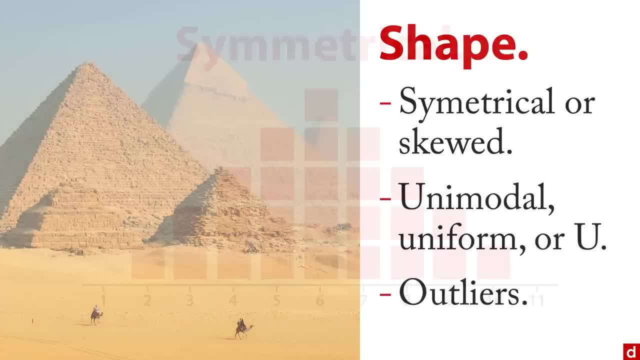 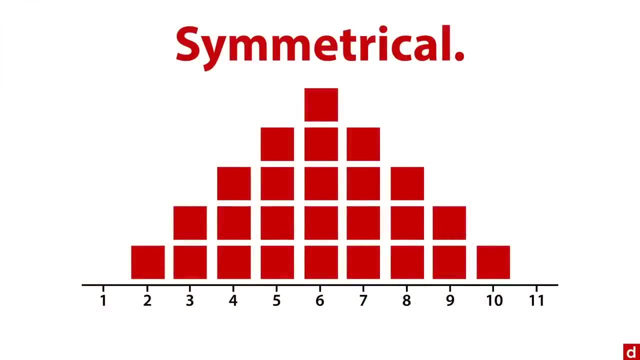 outliers. There's a lot of variations. Let me show you a few of them. First off is a symmetrical distribution Pretty easy. They're the same on the left and on the right, And this little pyramid shape is an example of a symmetrical distribution. 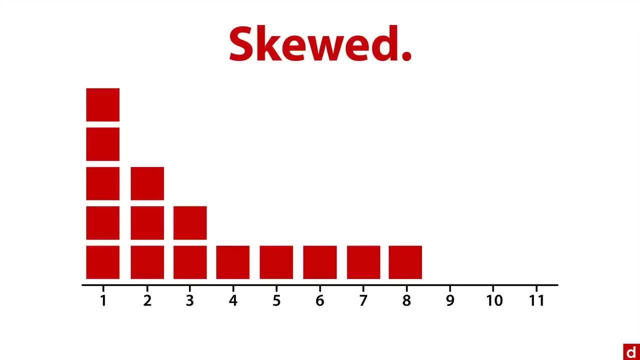 There are also a number of variations. There are a number of variations. There are a number of skewed distributions where most of the scores are on one end and then they taper off. This right here is a positively skewed distribution where most of the scores are at the low end and the 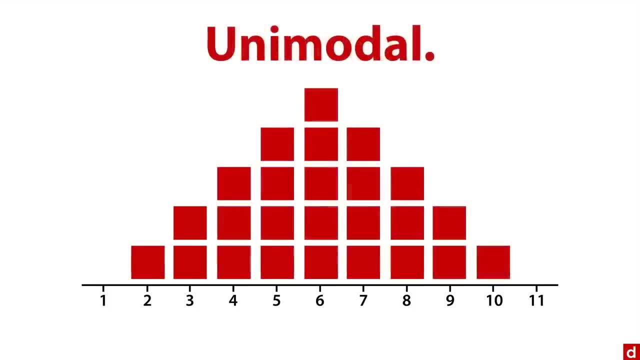 outliers are on the high end. This is unimodal. It's our same pyramid shape. Unimodal means it has one mode, or really kind of one hump in the data. That's contrasted, for instance, to bimodal, where you have two modes, And that usually happens when. 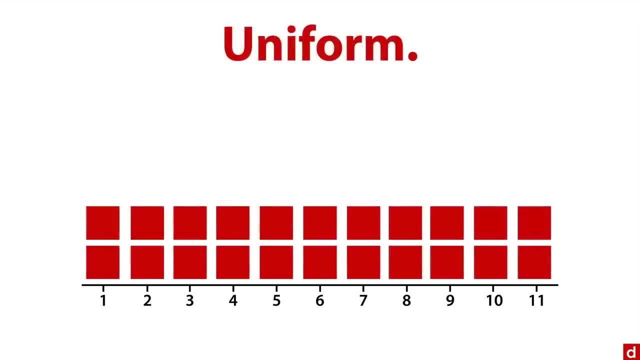 you have two distributions that got mixed together. There's also uniform distributions where every response is equally common. There's U-shaped distributions where people tend to pile up at one end or the other and a big dip in the middle, And so there's a lot of different variations And 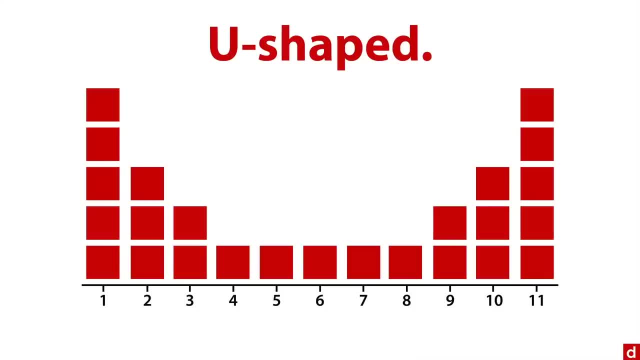 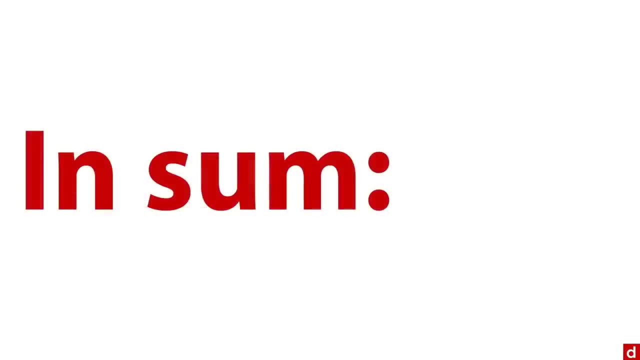 you want to get those, the shape of the distribution, to help you understand and put the numerical summaries, like the mean and like the standard deviation, and put those into context. In sum, we can say this When you use descriptive statistics: 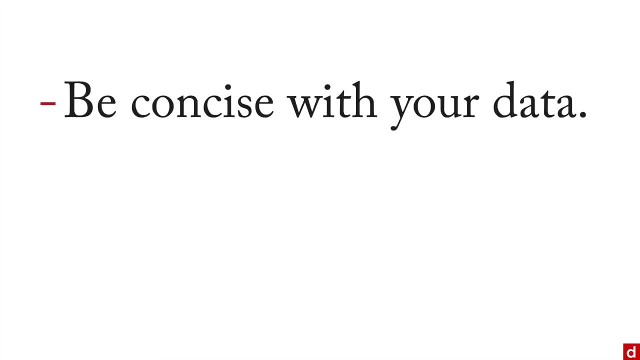 that allows you to be concise with your data, Tell the story and tell it succinctly. You want to focus on things like the center of the data, the spread of the data, the shape of the data And, above all, watch out for anomalies, because they can exercise. 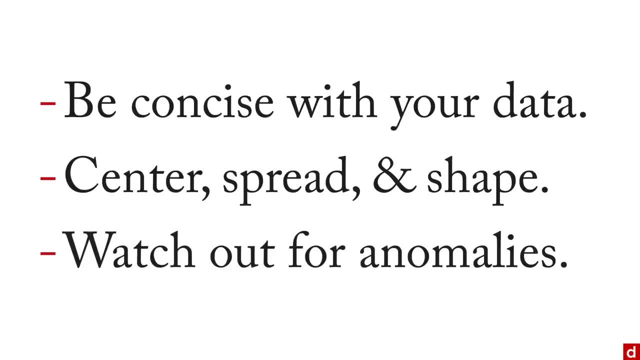 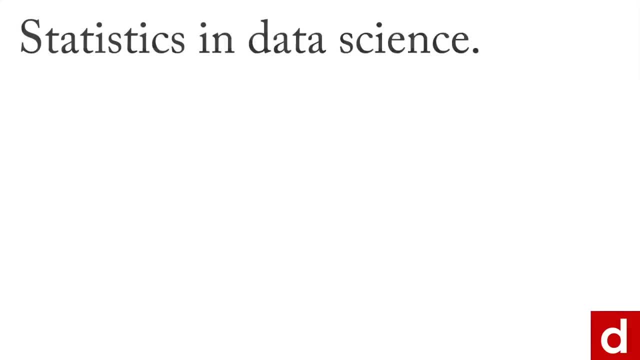 really undue influence on your interpretation, But this will help you better understand your data and prepare you for the steps that follow. The next step in our discussion of statistics and inference is hypothesis testing, a very common procedure in some fields of research. I like to think of it as put your money where your mouth is. 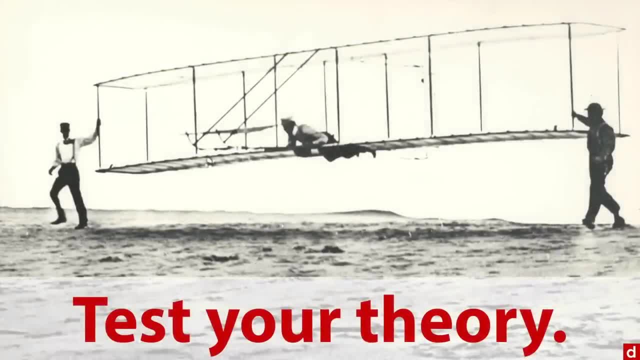 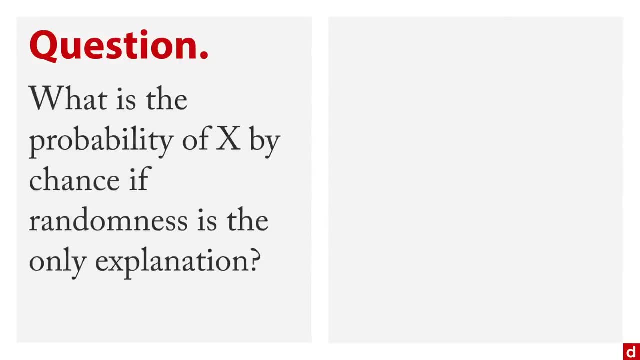 and test your theory. Here's the Wright brothers out testing their plane. Now, the basic idea behind hypothesis testing is this: You start with a question and it's something like: what is the probability of X occurring by chance if randomness or meaningless sampling variation is the only explanation? Well, the response is this: 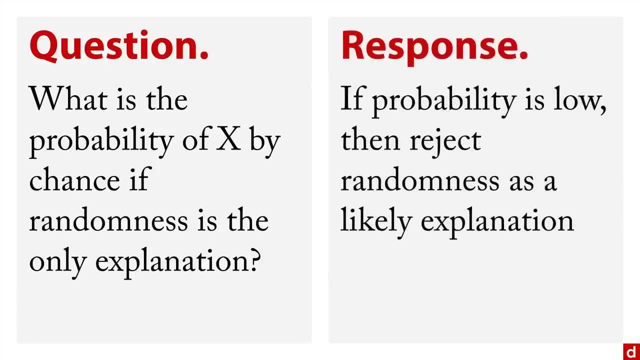 If the probability of that data arising by chance when nothing's happening is low, then you would have to project randomness as a likely explanation. Okay, there's a few things I can say about this. Number one: it's really common in scientific 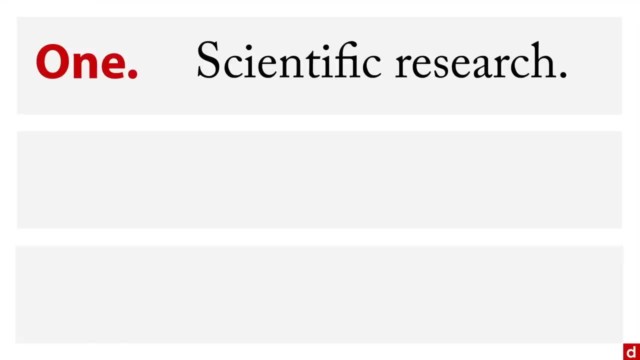 research Say, for instance, in the social sciences it's used all the time. Number two: this kind of approach can be really helpful in medical diagnostics, where you're trying to make a yes-no decision: Does a person have a particular disease? And three really. 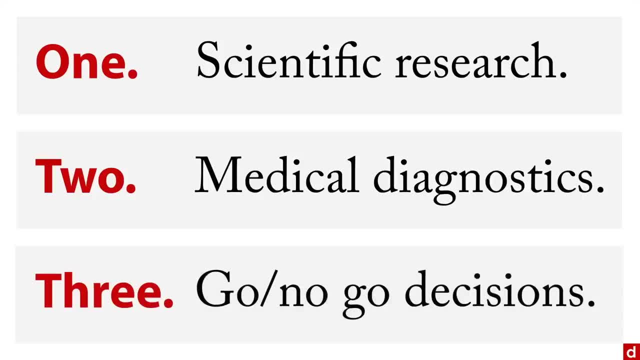 anytime you're trying to make a go-no-go decision, which might be made, for instance, with a purchasing decision for a school district or implementing a particular law, you base it on the data and you have to make a yes-no Hypothesis. testing might be helpful in those situations. 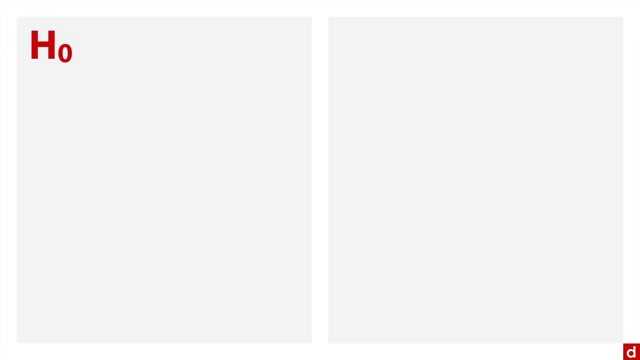 Now you have to have hypotheses to do hypothesis testing. You start with H sub zero, which is the shorthand version for the null hypothesis, and what that is in larger term rephrase, and what that is in lengthier terms, is that there is no 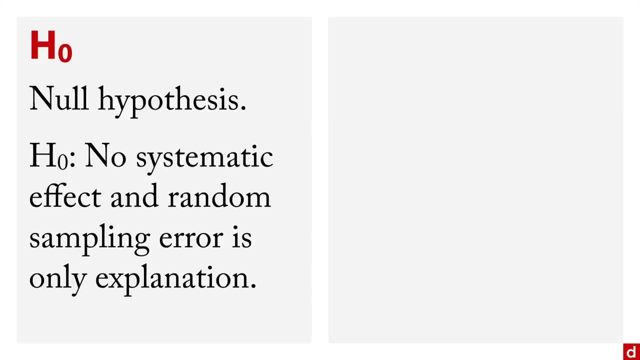 systematic effect between groups. there's no association between variables and random sampling error is the only explanation for any observed differences that you see. And then contrast that with H sub A, which is the alternative hypothesis, And this really just says that there's a systematic effect, that there is in fact a correlation. 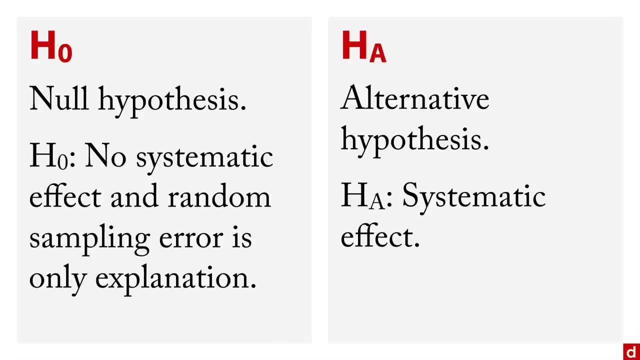 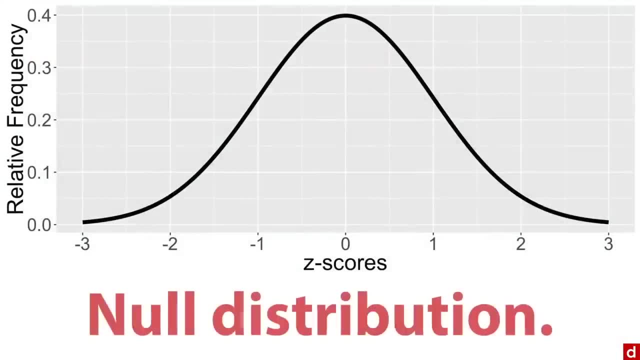 between variables, that there is in fact a difference between two groups, that this variable does in fact predict the other one. Let's take a look at the simplest version of this, statistically speaking. Now, what I have here is a null distribution. This is a bell curve. 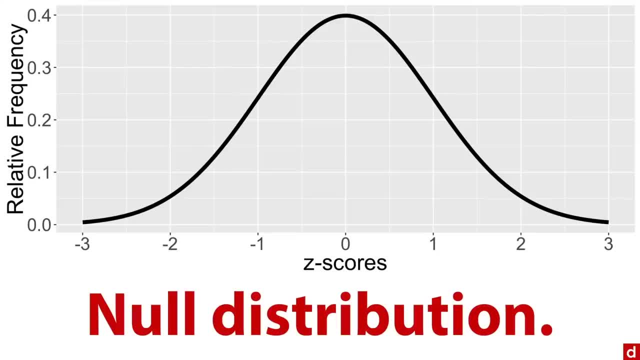 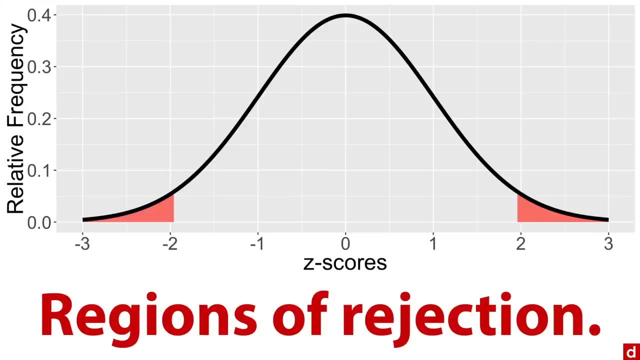 It's actually the standard normal distribution which shows z-scores and relative frequency, And what you do with this is you mark off what are called regions of rejection, And so I've actually shaded off the highest 2.5% of the distribution and the lowest 2.5%. 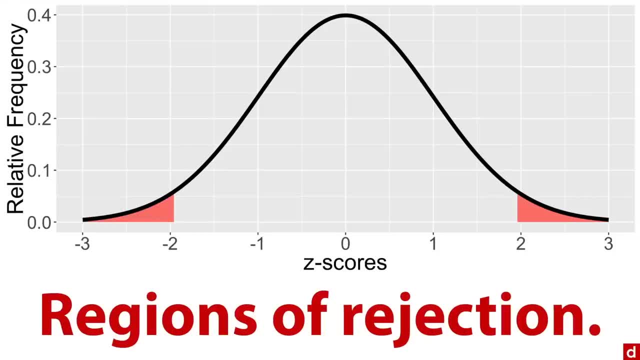 What's funny about this is, even though I draw it to plus and minus 3 and it looks like it hit 0, it's actually infinite and asymptotic. But that's the highest and lowest: 2.5% collectively. That leaves 95% in the middle. 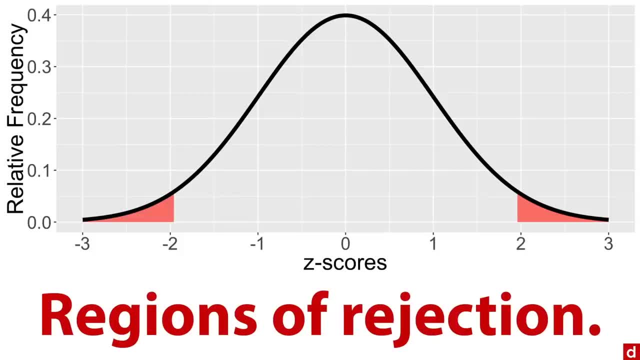 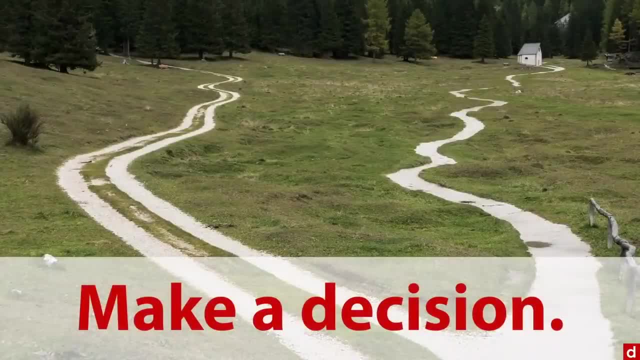 Now the idea is then you gather your data, you calculate a score for your data and you see where it falls in this distribution. And I like to think of that, as you have to go down one path or the other. You have to make a decision. 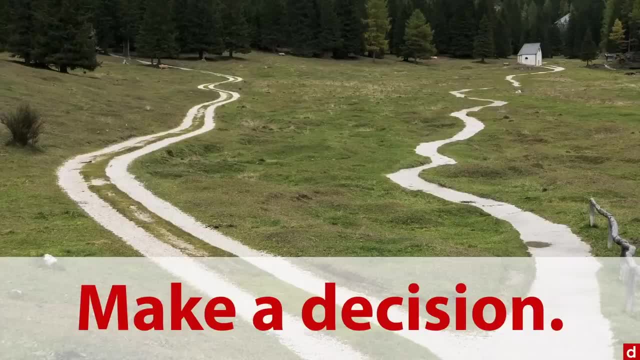 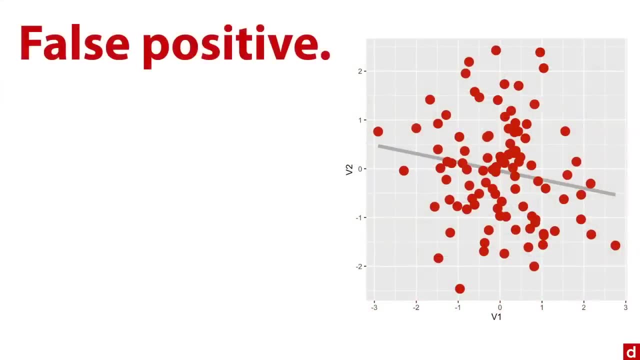 And you have to decide whether to retain your null hypothesis- maybe it is random- or reject it and decide no, I don't think it's random. The trick is things can go wrong. You can get a false positive. This is when the sample shows some kind of statistical effect. 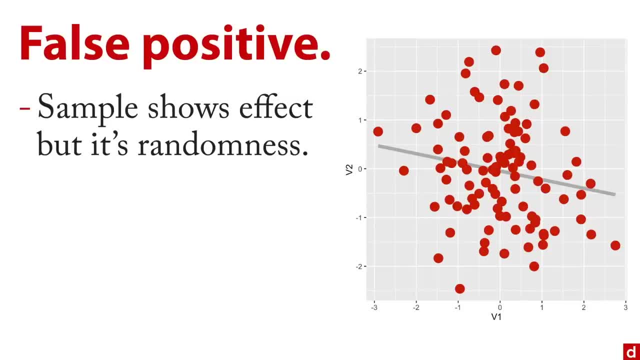 But it's really randomness And so, for instance, this scatterplot I have right here- you can see a little downhill association here, But this is in fact drawn from data that has a true correlation of zero And I just kind of randomly sampled from it until I got this. 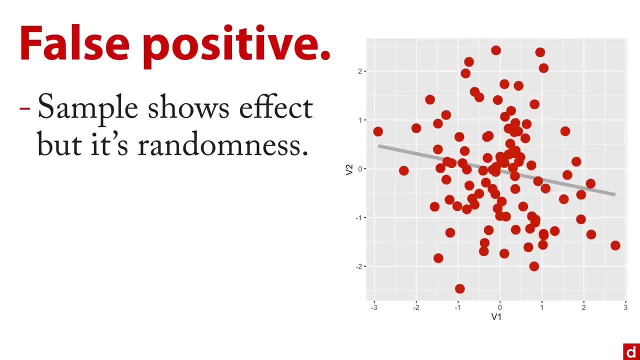 It took about 20 rounds But it looks negative, but there's really nothing happening. The trick about false positives is that's conditional on rejecting the null. The only way you can get a false positive is if you actually conclude that there's a positive. 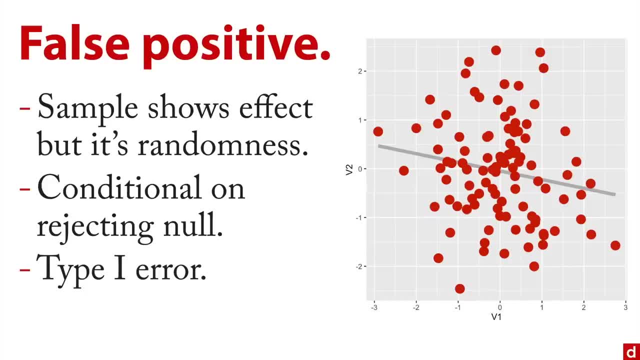 result. It goes by the highly descriptive name of a type one error, But you get to pick a value for it and .05 or 5% risk. if you reject the null hypothesis, that's the most common value. Then there's a false negative. 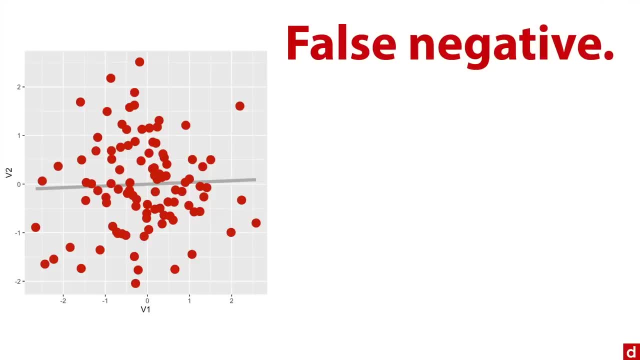 This is when the data looks random, but in fact it is systematic or there's a relationship. So, for instance, this scatterplot: it looks like it's pretty much a zero relationship, But in fact this came from two variables that were correlated at .25,. that's a pretty 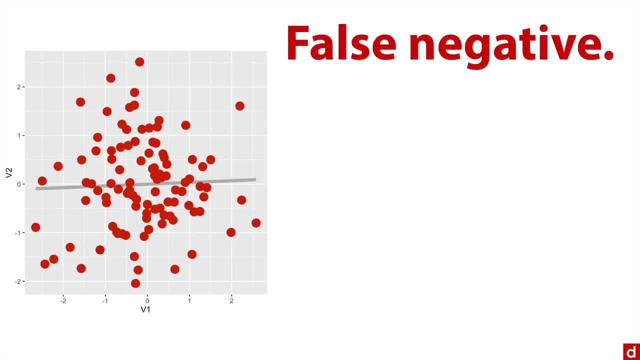 strong association. Again, I randomly sampled from the data until I got a set that happened to look pretty flat And a false negative is conditional on not rejecting the null. You can only get a false negative. if you get a negative, you say there's nothing there. 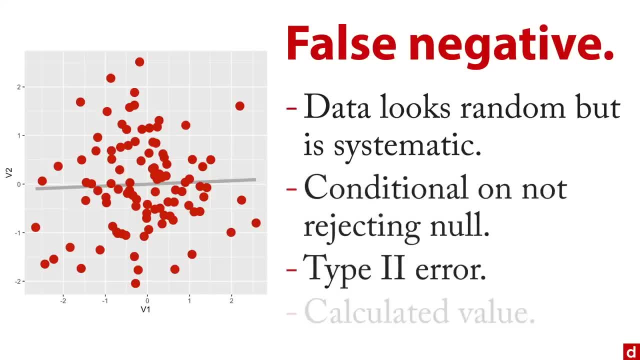 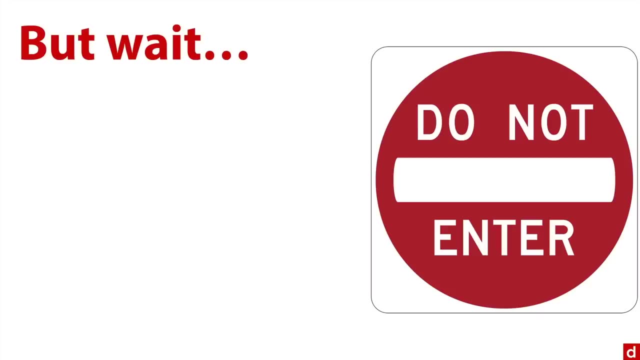 It's also called a type two error, And this is a value that you have to calculate based on several elements of your testing framework, So it's something to be thoughtful of. Now I do have to mention one thing: big security notice, But wait, the problem with hypothesis testing. there's a few. 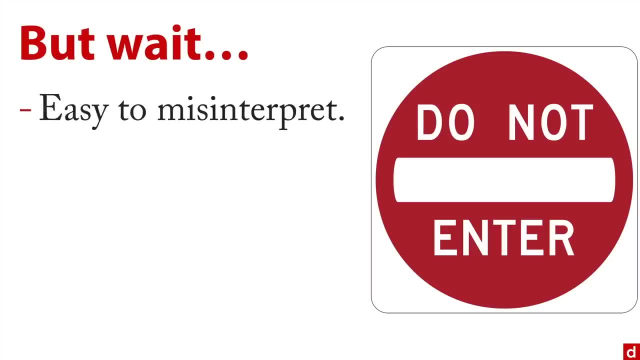 Number one. it's really easy to misinterpret it. A lot of people say, well, if you get a statistically significant result, it means that is something big and meaningful. And that's not true, because it's confounded with sample size and a lot of other things. 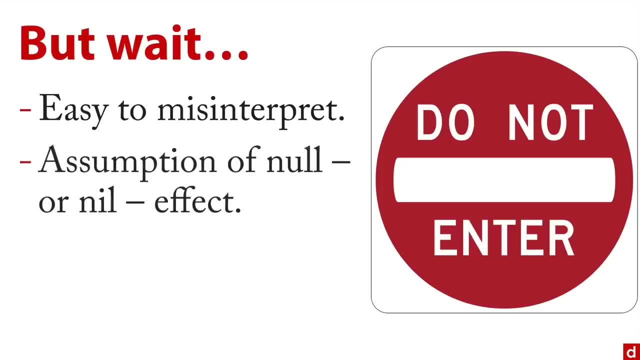 that just don't really matter. Also, a lot of people take exception with the assumption of a null effect or even a nil effect, that there's zero difference at all. That could be in certain situations. it could be an absurd claim, So got to watch out for that. 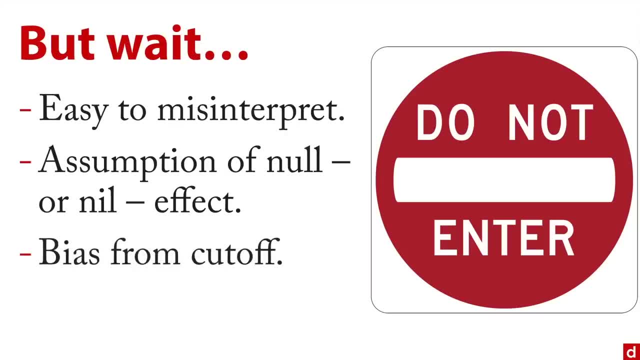 There's also bias from the use of a cutoff. Anytime you have a cutoff, you're going to have problems. where you have cases that would have been just slightly higher, slightly lower. it would have switched on the dichotomous outcome. 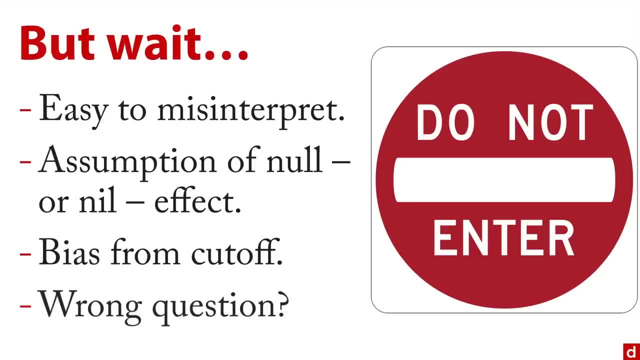 So that is a problem. And then a lot of people say that it just answers the wrong question because of what it's telling you is: what's the probability of getting this data at random? That's not what most people care about. They want it the other way, which is why I mentioned previously Bayes theorem and I'll 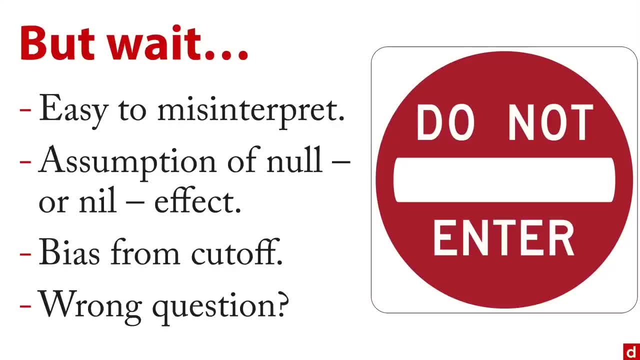 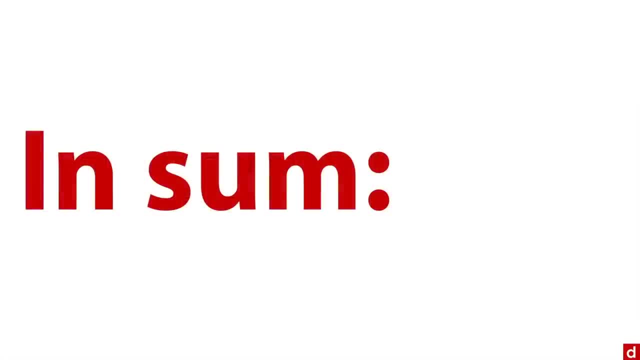 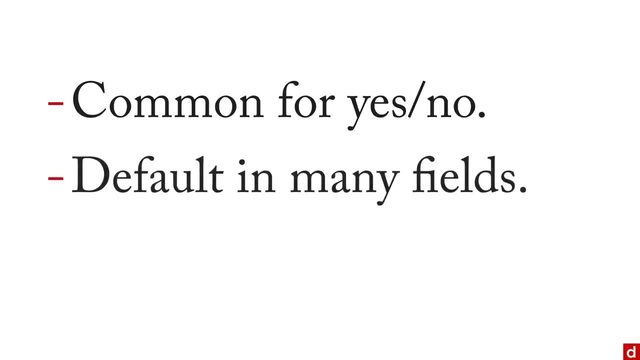 say more about that later. That being said, hypothesis testing is still very deeply ingrained, very useful in a lot of questions and it's gotten us really far in a lot of domains. So, in sum, let me say this: Hypothesis testing is very common for yes-no outcomes and it's the default in many fields. 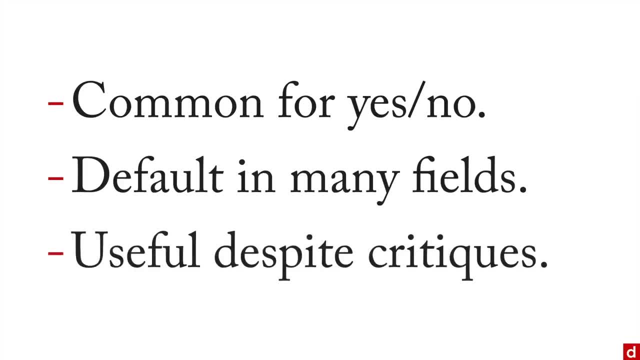 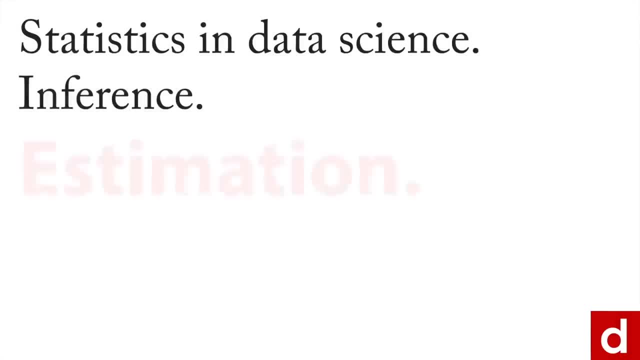 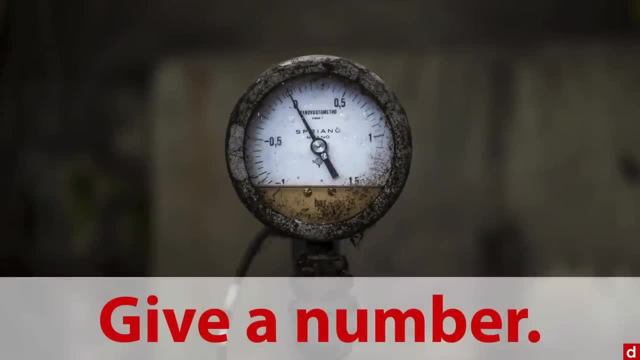 And I argue that it is still useful and informative, despite many of the well-substantiated critiques. We'll continue in statistics and inference by discussing estimation. Okay Now, as opposed to hypothesis testing, estimation is designed to actually give you a number. 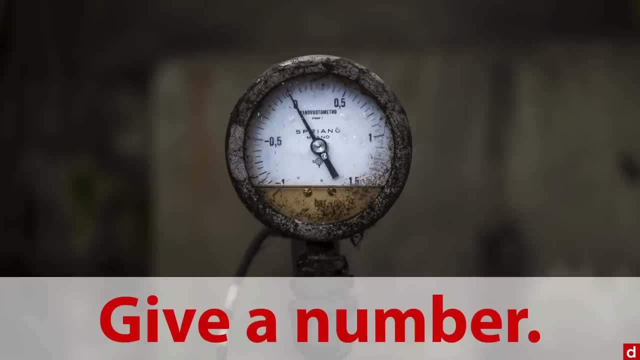 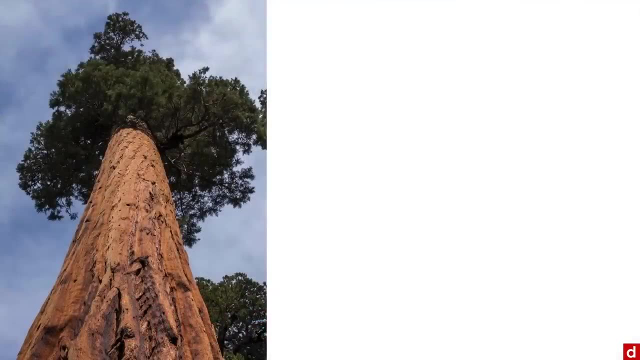 give you a value, not just a yes-no, go-no-go, but give you an estimate for a parameter that you're trying to get. I like to think of it as sort of a new angle, looking at something from a different way. 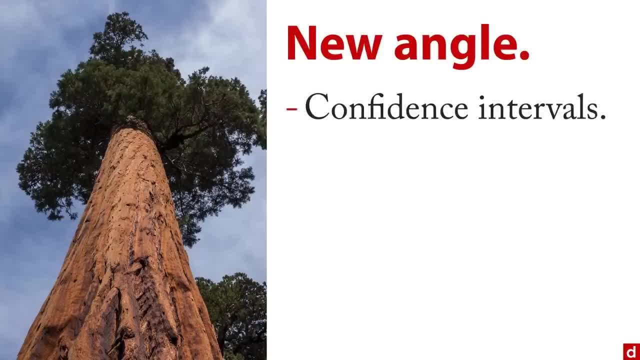 The most common approach to this is confidence intervals. Now, the important thing to remember is this is still an inferential procedure. You're still using sample data and trying to make conclusions about a larger group or population. The difference here is, instead of coming up with a yes-no, you instead focus on likely. 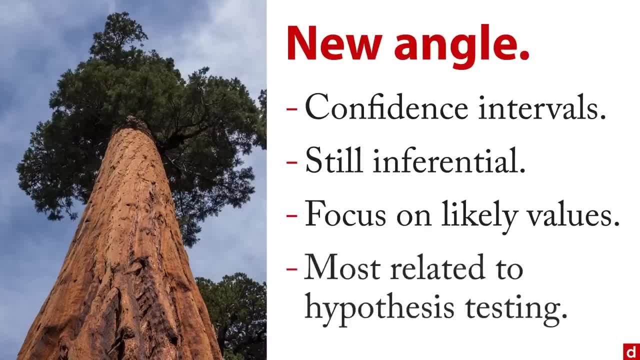 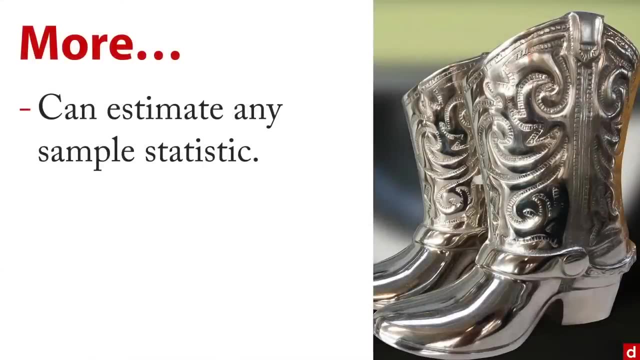 values for the population value. Most versions of estimation are closely related to hypothesis testing, sometimes seen as the flip side of the coin, and we'll see how that works in later videos. Now I like to think of this as an ability to estimate any sample statistic, and there's 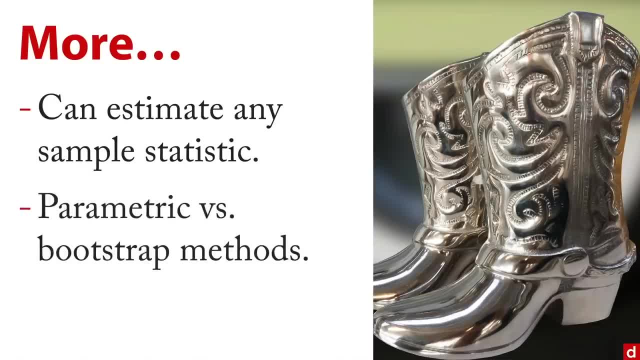 a few different versions. We have parametric versions of estimation and bootstrap versions. Okay, This is why I got the boots here, And that's where you just kind of randomly sample from the data in an effort to get an idea of the variability. 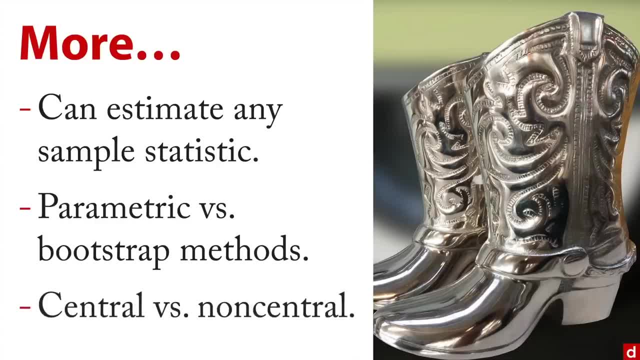 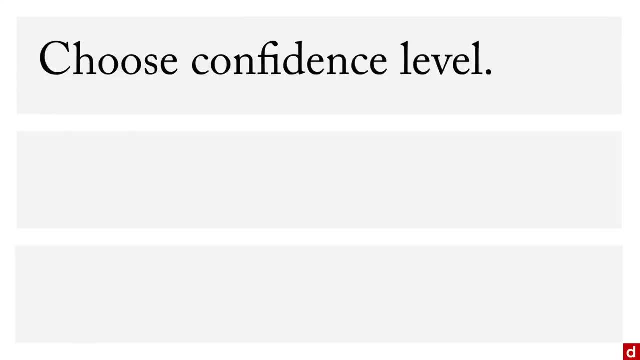 You can also have what are called central versus non-central confidence intervals in estimation, but we're not going to deal with those Now. there are three general steps to this. First, you need to choose a confidence level anywhere from say, well, you can't have zero. 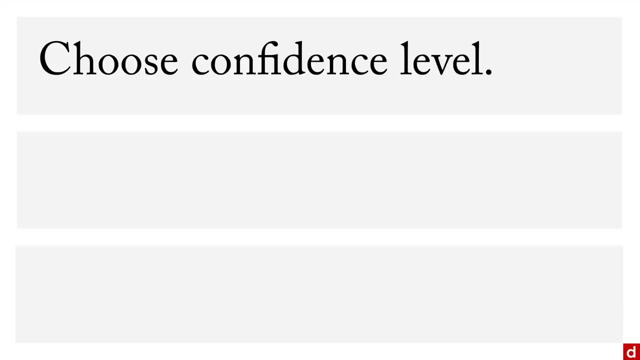 It has to be more than zero and it can't be 100%. Choose something in between- 95% is the most common- And what it does is it gives you a range of numbers, a high and a low, And the higher your level of confidence, the more confident you want to be, the wider the 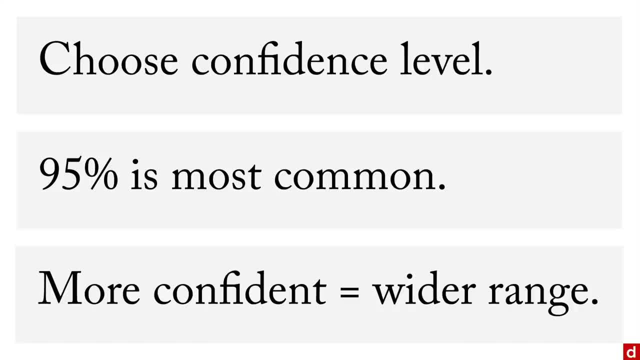 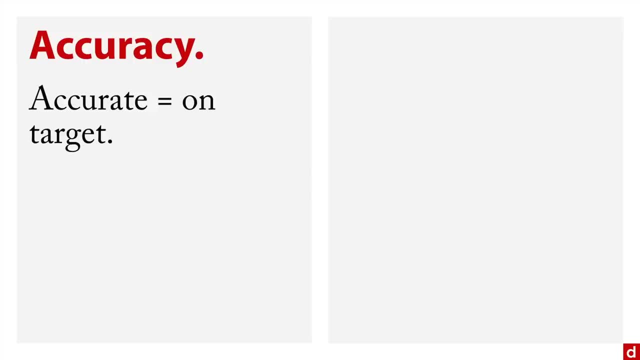 range is going to be between your high and your low estimates. Now there's a fundamental trade-off in what's happening here, and it's the trade-off between accuracy, which means you're on target, or, more specifically, that your interval contains. 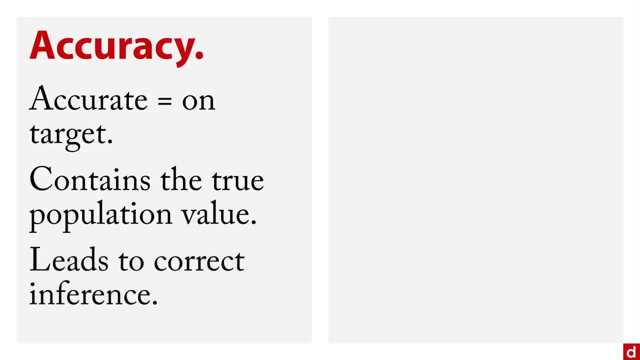 the true population value, and the idea is that leads you to the correct inference. There's a trade-off between accuracy. There's a trade-off between accuracy and what's called precision in this context, And precision means a narrow interval and it's a small range of likely values. 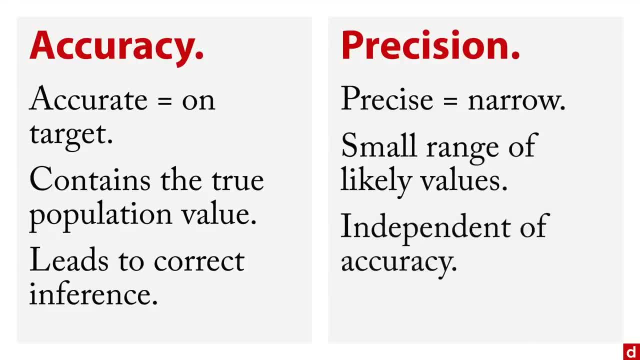 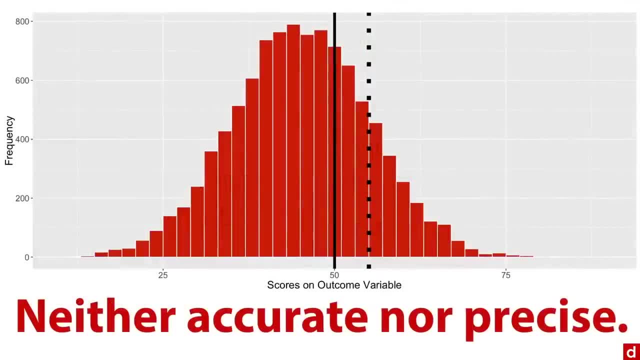 And what's important to emphasize is this is independent of accuracy. You can have one without the other, or neither or both. In fact, let me show you how this works. What I have here is a little hypothetical situation. I've got a variable that goes from- maybe you know- 10 to 90.. 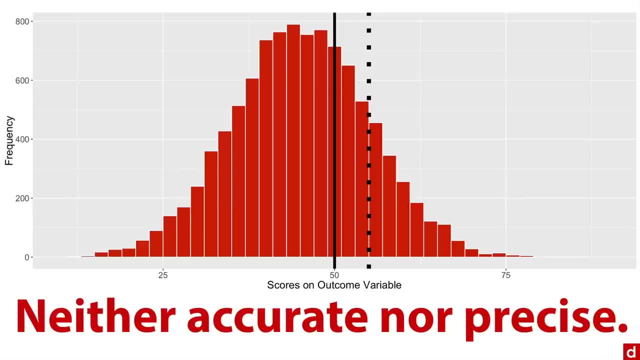 And I've drawn a thick black line At 50. If you think of this in terms of percentages and political polls, it makes a very big difference if you're on the left or the right of 50%. And then I've drawn a dotted vertical line at 55 to say that that's our theoretical true. 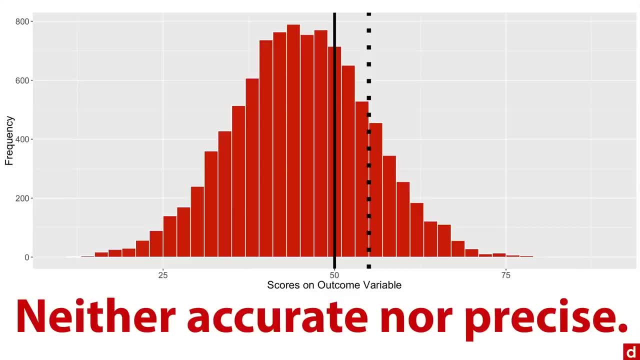 population value, Then what I have here is a distribution that shows possible values based on our sample data, And what you get here is it's not accurate because it's centered on the wrong thing. It's actually centered on 45 as opposed to 55.. 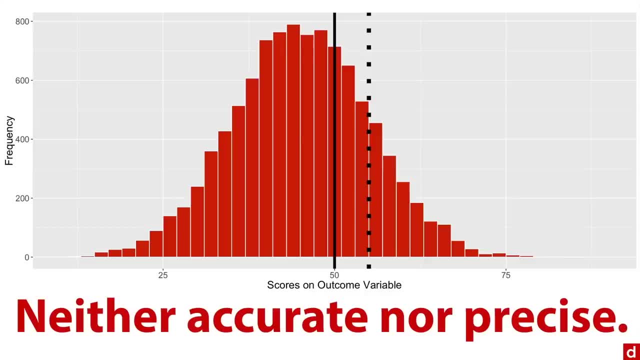 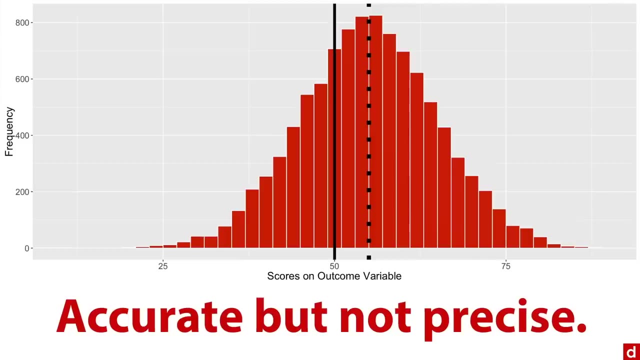 And it's not precise because it's spread way out, from maybe 10 up to almost 80.. So this situation- the data- is no help really at all. Now here's another one. This is accurate because it's centered on the true value. 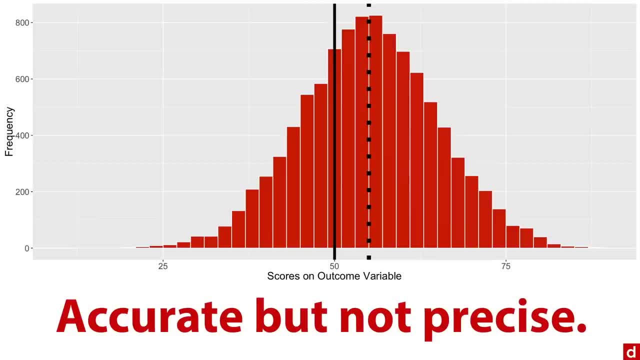 That's nice, But it's still really spread out and you see that about 40% of the values are going to be on the other side of 50% might lead you to reach the wrong conclusion, So that's a problem. Now here's the nightmare situation. 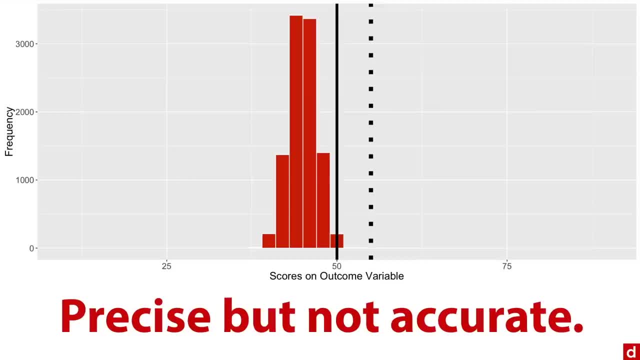 This is when you have a very, very precise estimate, but it's not accurate, It's wrong, And this leads you to a very false sense of security and understanding of what's going on And you're going to totally blow it all the time. 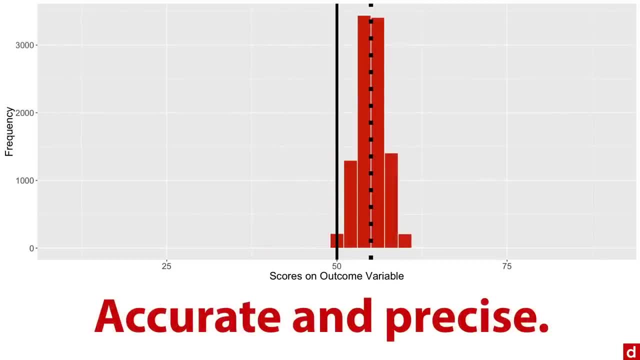 The ideal situation is this: You have an accurate estimate where the distribution of sample values is really close to the true population value and is precise. It's really tightly knit And you can see that About 95% of it is on the correct side of 50.. 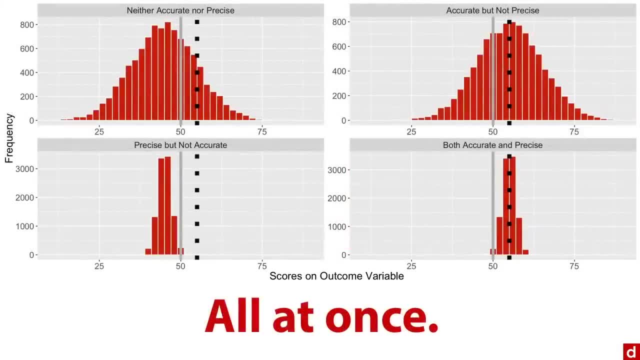 And that's good. If you want to see all four of them here at once. we have the precise two on the bottom, the un-precise ones on the top, the accurate ones on the right, the inaccurate ones on the left. 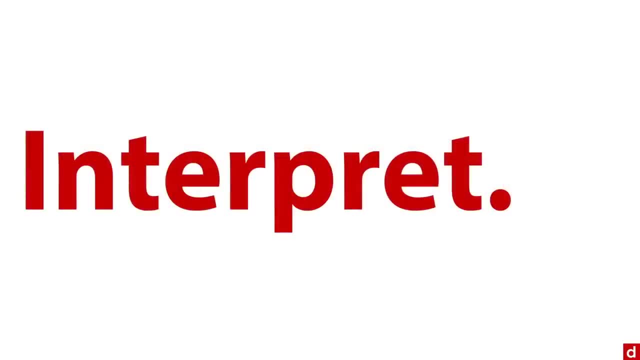 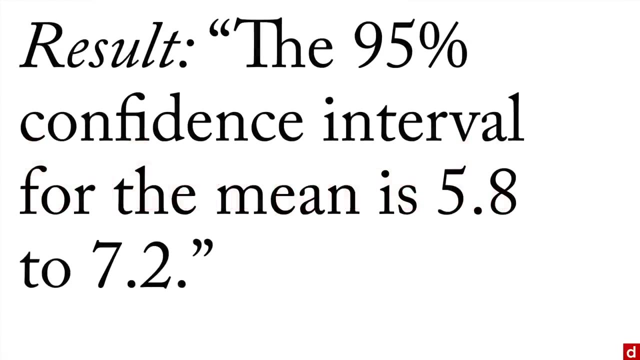 And so that's a way of comparing it. But no matter what you do, you have to interpret a confidence interval. Now, the statistically accurate way that has very little interpretation is this: you would say the 95% confidence interval, And the actual confidence interval for the mean is 5.8 to 7.2.. 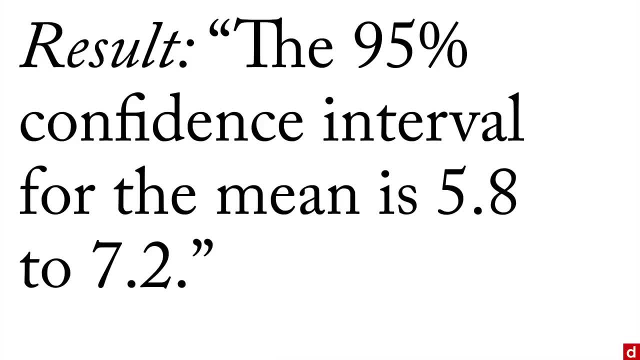 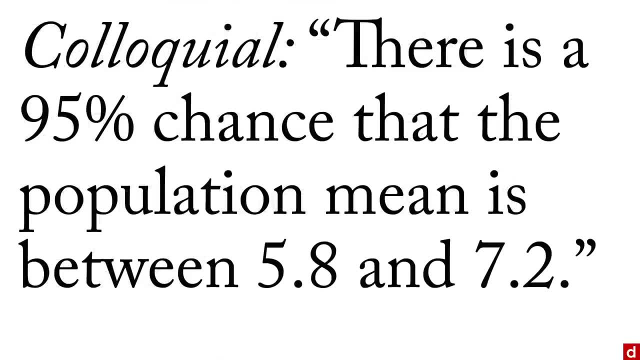 Okay, So that's just kind of taking the output from your computer and sticking it into sentence form. The colloquial interpretation of this goes like this: There's a 95% chance that the population mean is between 5.8 and 7.2.. 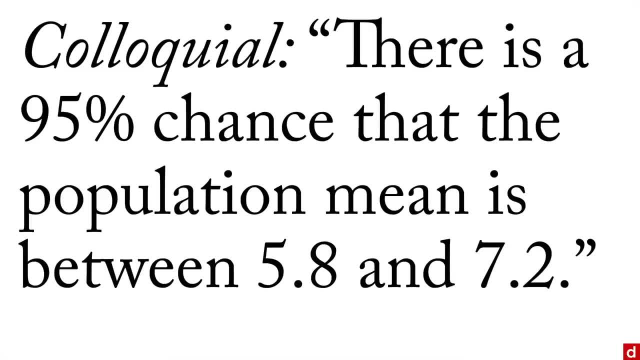 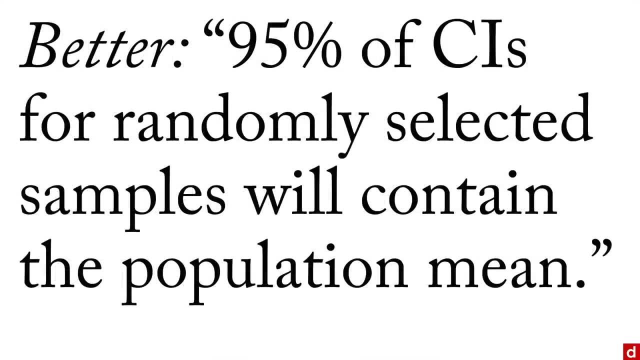 Well, in most statistical procedures- specifically frequentist as opposed to Bayesian- you can't do that. That implies that the population mean shifts. That's not usually how people do it. Instead, a better interpretation is this: 95% of confidence intervals for randomly selected. 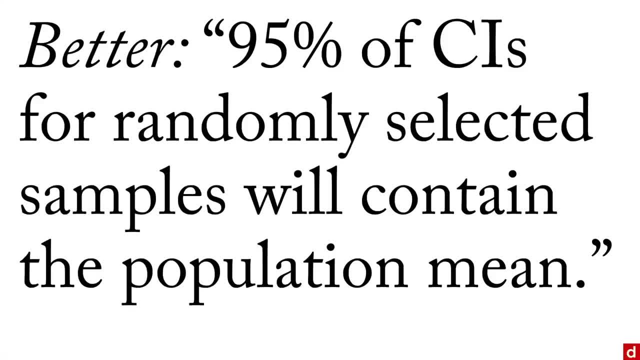 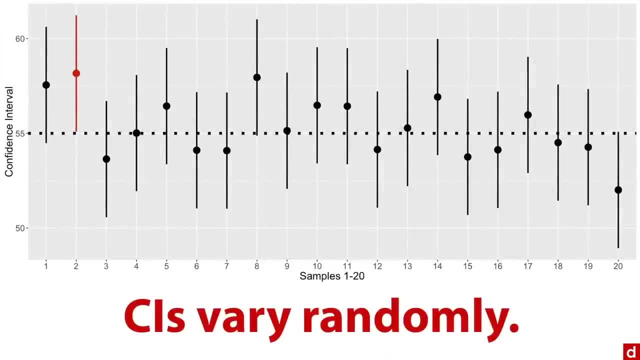 samples will contain the population mean. Now I can show you this really easily with a little demonstration. This is where I randomly generated data from a population with a mean of 55, and I got 20 different samples And I got the confidence interval for each sample and I've charted the high and the 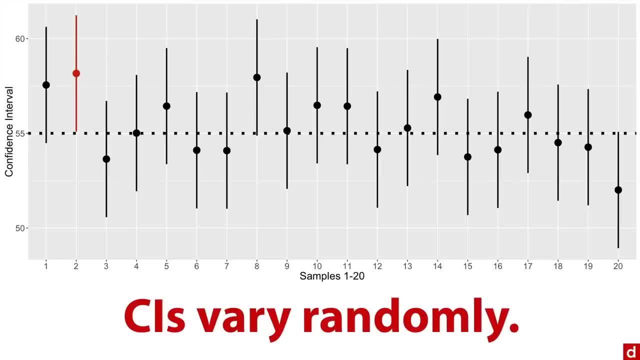 low. The question is: did it include the true population value? And you can see that of these 20,, 19 of them included it. Some of them barely made it. If you look at sample number one on the far left, barely made it. 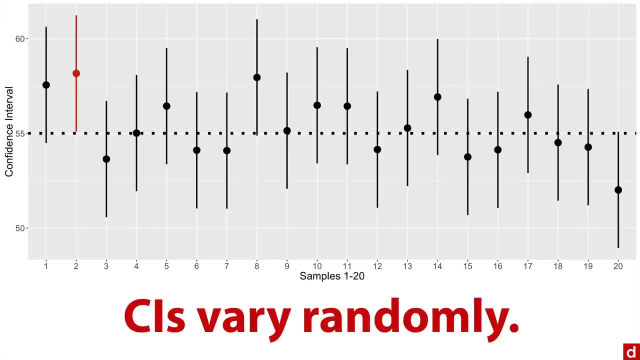 Sample number eight. it doesn't look like it made it. Sample 20 on the far right, barely made it on the other end. Only one of them missed it completely: that sample number two which is shown in red on the left. 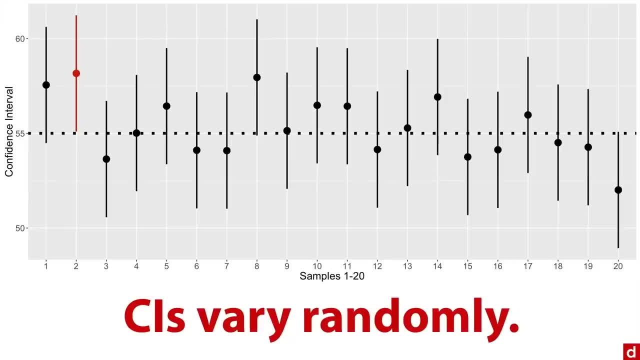 Now it's not always just one out of 20.. I actually had to run the simulation about 18 times Because it gave me either zero or three, or one or two, And I had to run it until I got exactly what I was looking for here. 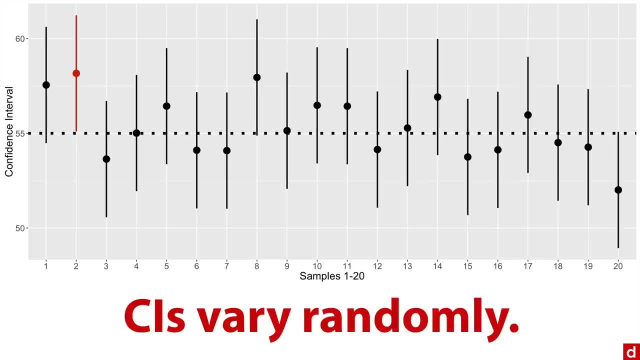 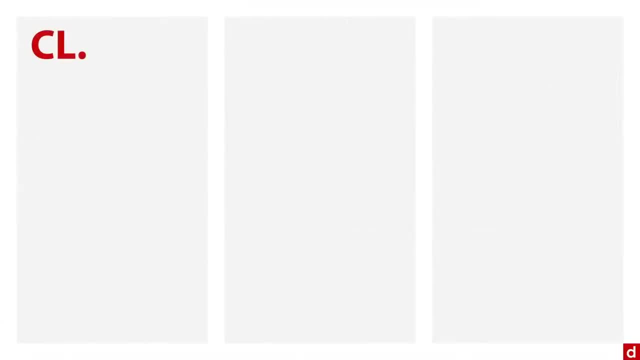 But this is what you would expect on average. So let's say a few things about this. There are some things that affect the width of a confidence interval. The first is the confidence level, or CL. Higher confidence levels create wider intervals. The more certain you have to be. you're going to give a bigger range to cover your basis. 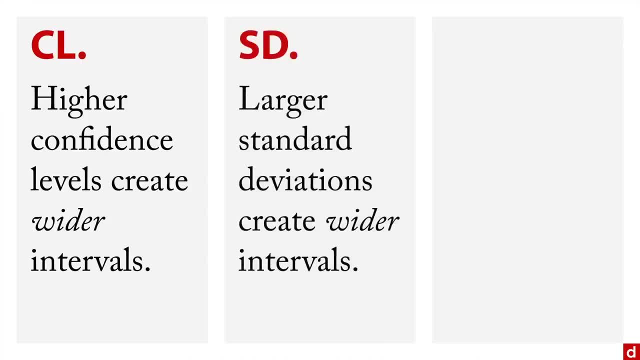 Second, the standard deviation, where larger standard deviations create wider intervals. If the thing that you're studying is inherently really variable, then of course your estimate of the range is going to be more variable as well. And then, finally, there's the N, or the sample size. 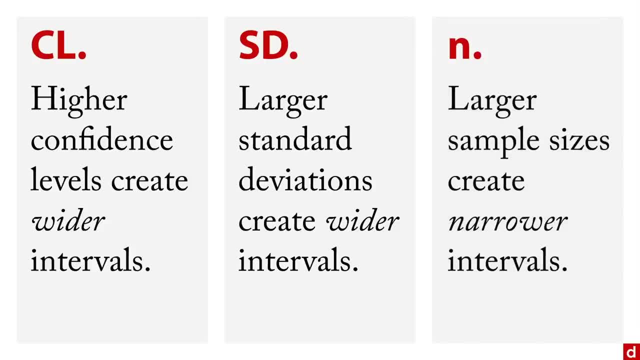 This one goes the other way. Larger sample sizes create narrower intervals. The more observations you have, the more precise and the more reliable things tend to be. I can show you each of these things graphically. Here we have a bunch of confidence intervals. 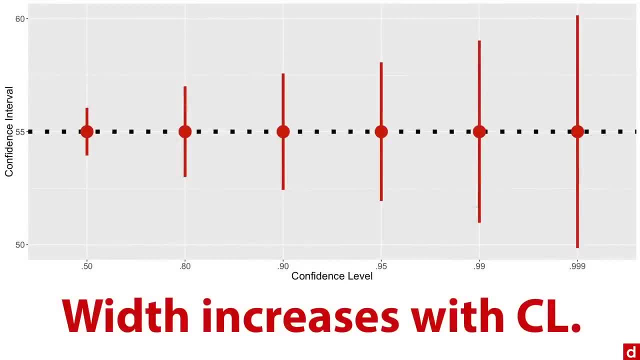 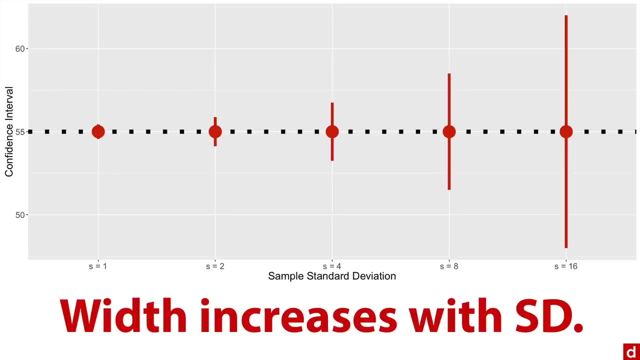 I'm simply changing the confidence level from .50 at the left side up through .999.. And you can see it gets much bigger as we increase. Next one is standard deviations. As the sample standard deviation increases from 1 to 16, you can see that the interval 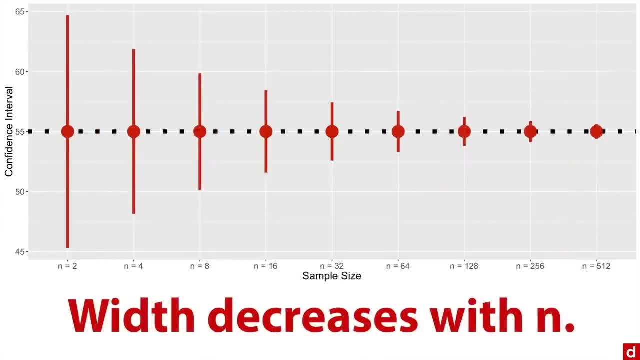 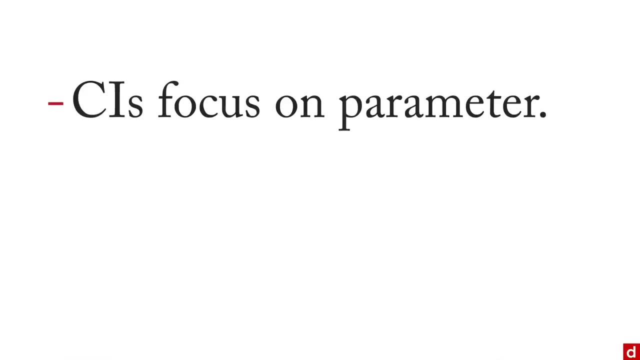 gets a lot bigger. And then we have sample size going from just 2 up to 512.. I'm doubling it at each point And you can see how the interval gets more and more and more precise as we go through. And so let's say this to sum up our discussion of estimation: 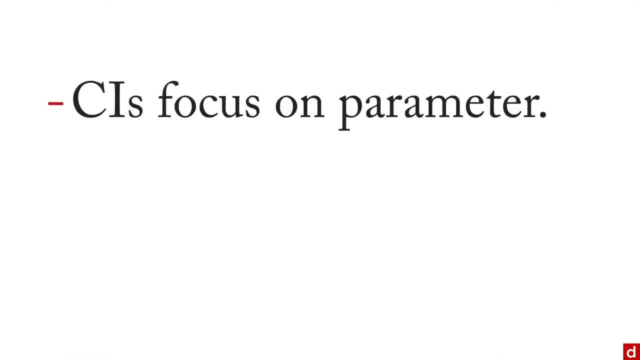 Confidence intervals, which are the most common version of estimation, focus on the population parameter, And the variation in the data is explicitly included in that estimation. Also, you can argue that they're more informative because not only do they tell you whether the population value is likely, but they give you a sense of the variability of the data. 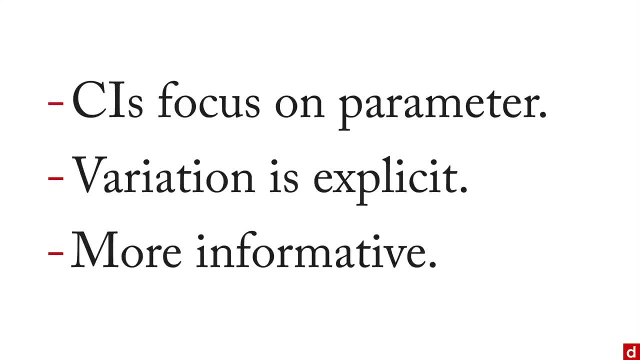 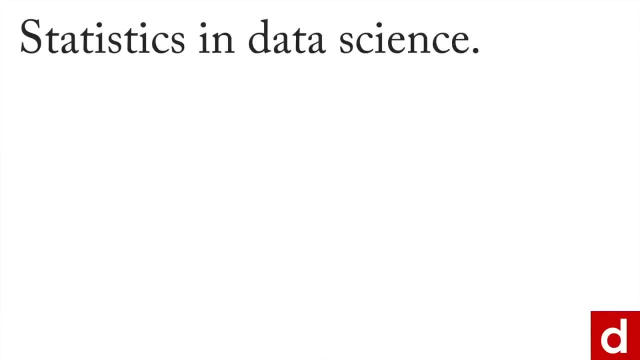 itself, And that's one reason that people argue that confidence intervals should be a very effective way to calculate value- nearly always be included in any statistical analysis. As we continue our discussion on statistics and data science, we need to talk about some of the choices that you have to make, some of the trade-offs and some of the effects. 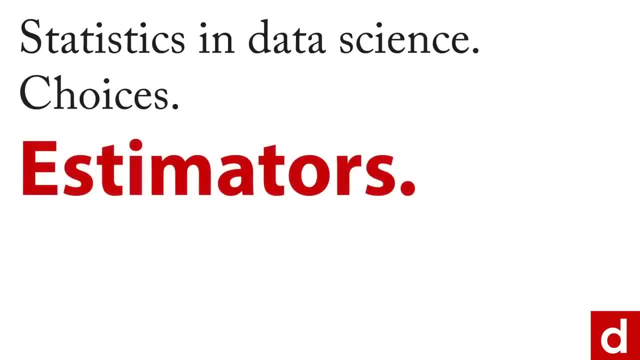 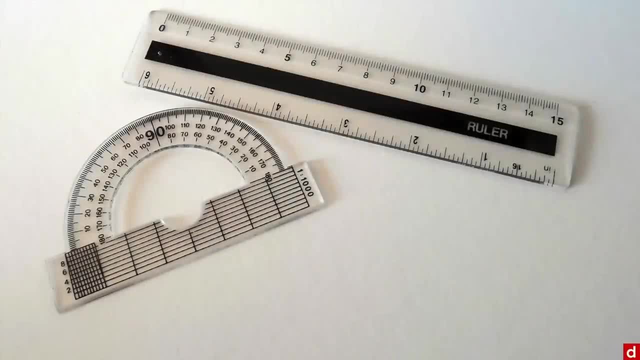 that these things have. We'll begin by talking about estimators, that is, different methods for estimating parameters. I like to think of this as: what kind of measuring stick or standard are you going to be using? Now we'll begin with the most common. 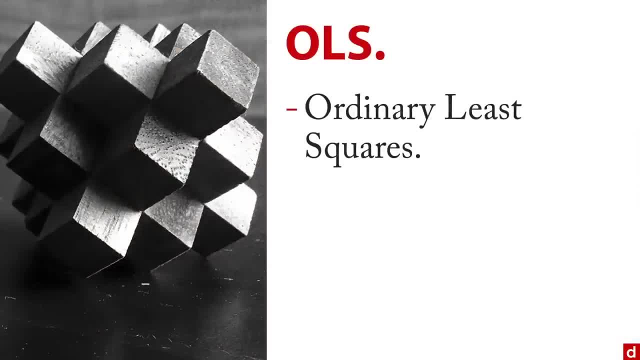 This is actually called OLS, which is short for Ordinary Least Squares. This is a very common approach. It's used in a lot of statistics and it's based on what's called the sum of squared errors, And it's characterized by an acronym called BLUE, which stands for Best Linear, Unbiased. 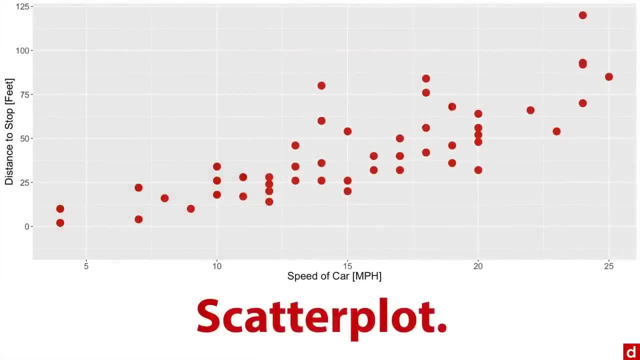 Estimator. Let me show you how that works. Let's take a scatterplot here of an association between two variables. This is actually the speed of a car and the distance to stop from about the 20s. I think We have a scatterplot here. 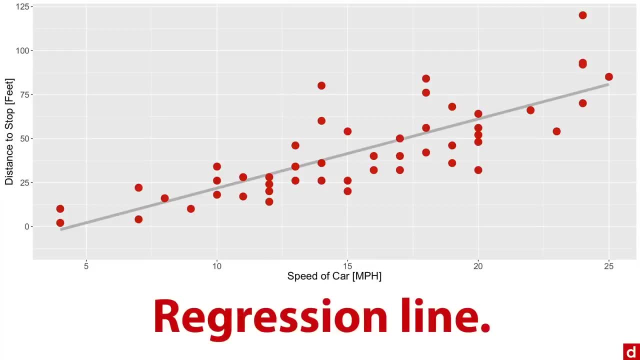 And we can draw a straight regression line through it. Now, the line that I've used is, in fact, the best linear, unbiased estimate, But the way that you can tell that is by getting what are called the residuals, If you take each data point and draw a perfectly vertical line up or down to the regression. 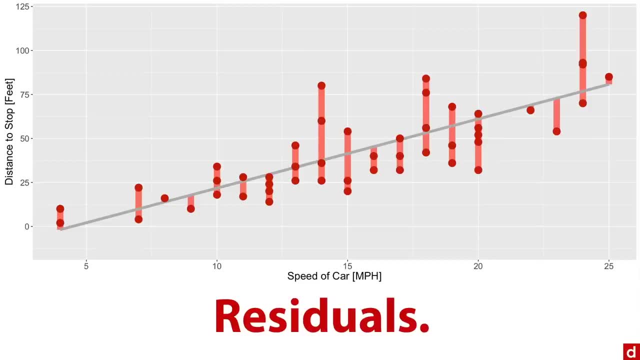 line, because the regression line predicts what the value would be for that value on the x-axis. those are the residuals. Each of those individual vertical lines is a residual. You square those And you add them up And this regression line, the gray angled line here, will have the smallest sum of squared. 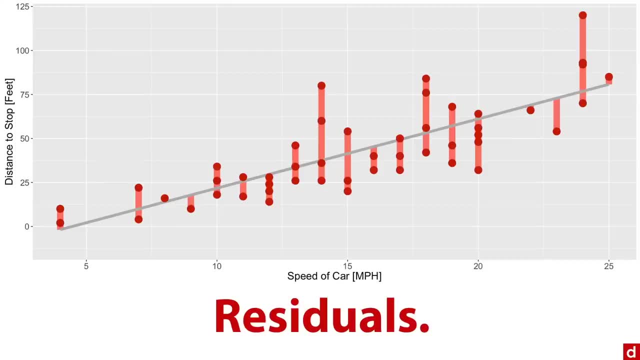 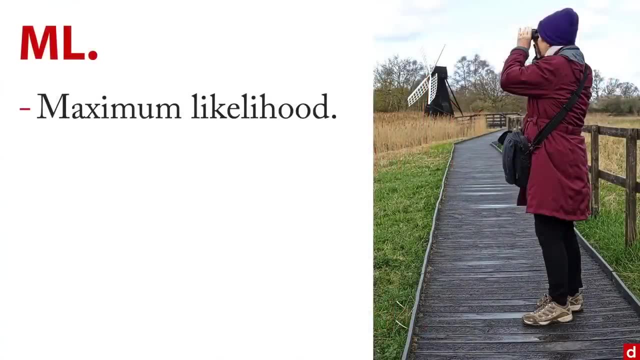 residuals of any possible straight line that you can run through it Now. another approach is ML, which stands for Maximum Likelihood, And this is when you choose parameters that make the observed data most likely. It sounds kind of weird, but I can demonstrate it. 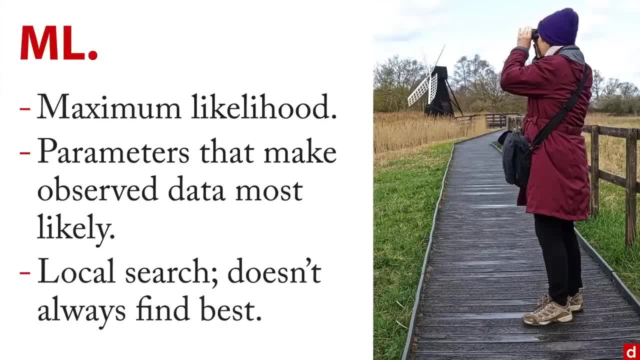 And it's based on a kind of logic. It's called local search. It doesn't always find the best. I like to think of it like a person here with binoculars looking around them, trying hard to find something, But you could theoretically miss something. 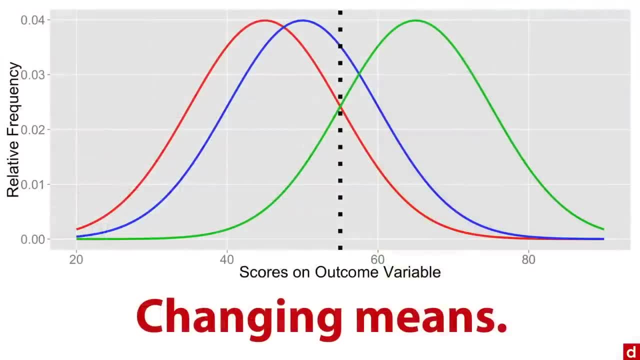 Let me give a very simple example of how this works. Let's assume that we're trying to find parameters that maximize the likelihood of this dotted vertical line here at 55. And I've got three possibilities. I've got my red distribution, which is off to the left, the blue, which is a little more. 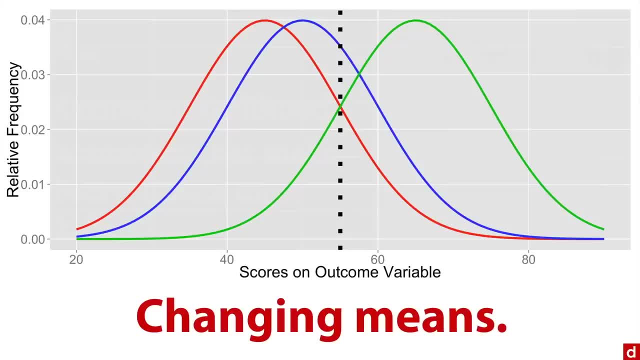 centered, and the green which is far to the right. So I've got my red distribution, which is off to the left, the blue which is a little more centered, and the green which is far to the right, And these are all identical except they have different means. 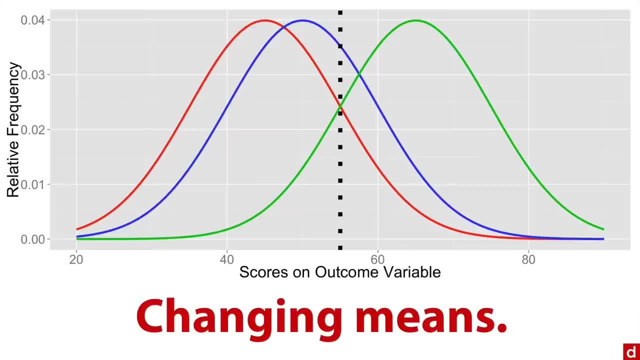 And by changing the means, you see that the one that is highest where the dotted line is is the blue one, And so if the only thing we're doing is changing the mean and we're looking at these three distributions, then the blue one is the one that has the maximum likelihood for this particular 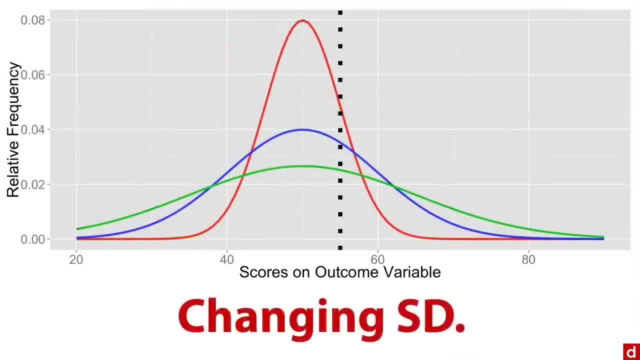 parameter. On the other hand, we could give them all the same mean- right around 50, and vary their standard deviations Instead, and so they spread out different amounts. In this case, the red distribution is highest at the dotted vertical line, and so it has. 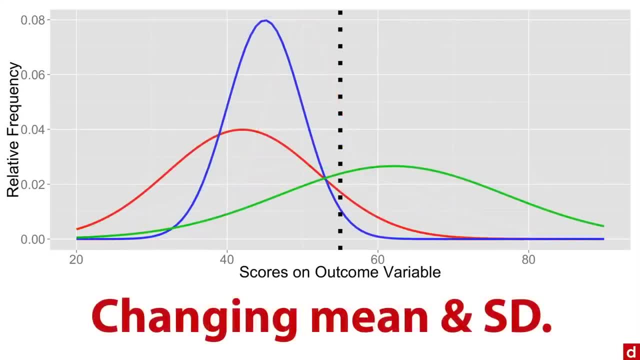 the maximum value. Or, if you want to, you can vary both the mean and standard deviation simultaneously, And here the green gets a slight advantage. Now, this is really a caricature of the process, because obviously you would just want to center it right there on the 55 and be done with it. 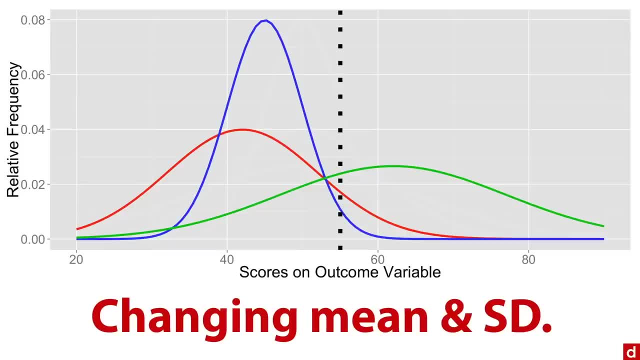 The question is: when you have many variables in your data set, then it's a very complex process of choosing values that can maximize the mean. It's a very complex process of choosing values that can maximize the mean, and it's a very complex process of choosing values that can maximize the mean. 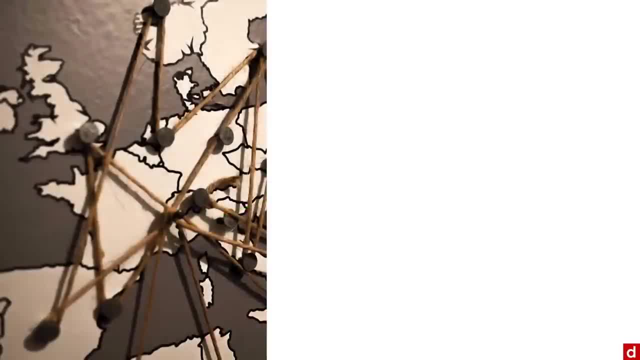 But you get a feel for how it works with this. The third approach that's pretty common is something called MAPMAP for maximum a posteriori. This is a Bayesian approach to parameter estimation And what it does is it adds the prior distribution and then it goes through sort of an anchoring. 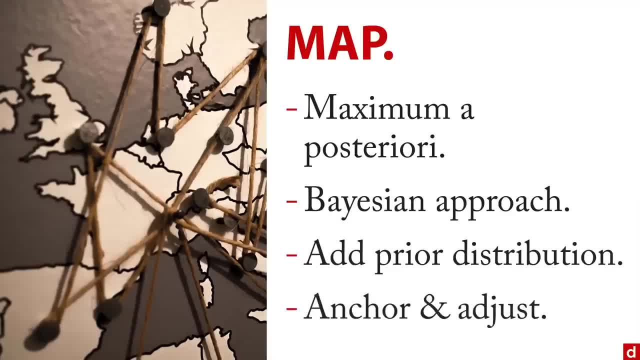 and adjusting process. What happens, by the way, is that stronger prior estimates exert more influence on the estimate. That might mean, for instance, a larger sample or more extreme values, And those have a greater influence on the posterior estimate of the parameters. 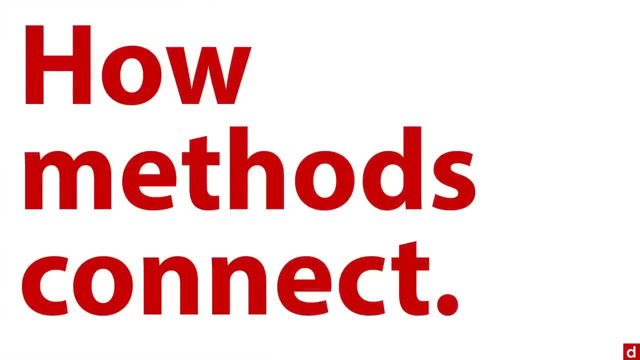 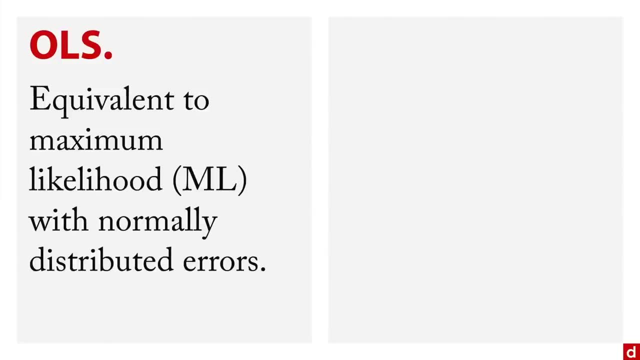 Now what's interesting is that these three methods all connect with each other. Let me show you exactly how they connect. The ordinary least squares: OLS: this is equivalent to maximum likelihood when it has normally distributed error terms And maximum likelihood. ML is equivalent to maximum likelihood when it has normally 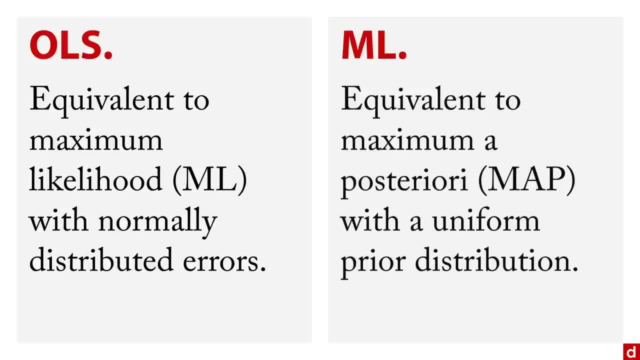 distributed error terms And maximum likelihood. ML is equivalent to maximum likelihood when it has normally distributed error terms And maximum likelihood ML is equivalent to maximum likelihood when it has normally distributed error terms. And this today is on the OLS aspect. 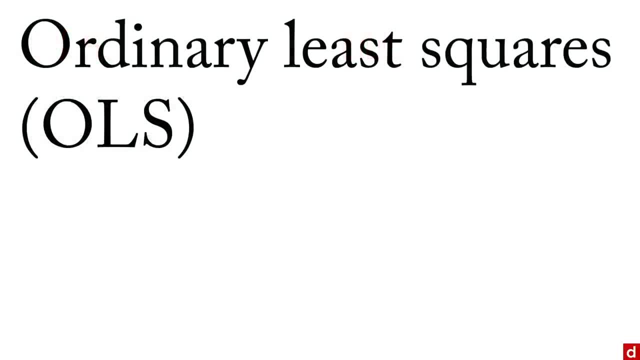 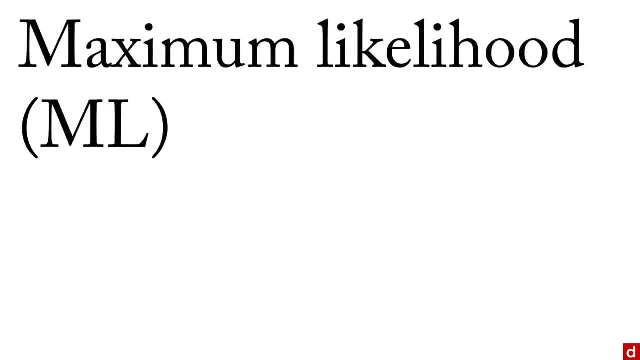 So, to sum it up, OLS can be used to place a maximum a posteriori or map with a uniform prior distribution. You wanna put it another way? ordinary least squares, or OLS, is a special case of maximum likelihood, and then maximum likelihood, or ML, is a special case of maximum a posteriori. 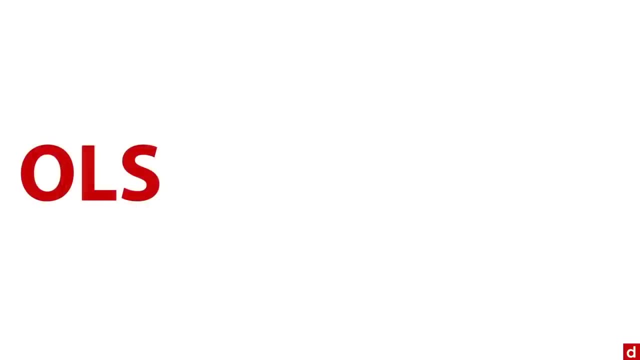 And, just in case you like it, we can put it in set notation: OLS is a subset of ML, it's a subset of MAP, And so there are connections between these sets, between these three methods of estimating population parameters. Let me just sum it up. 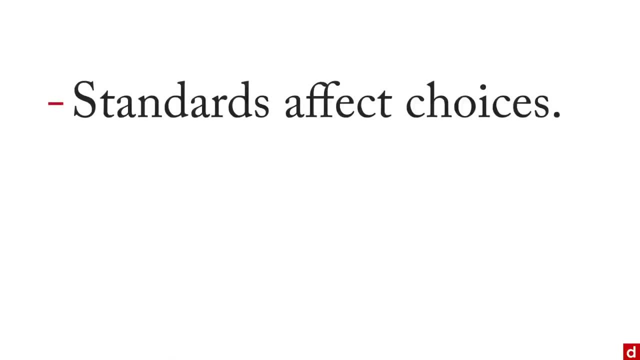 briefly this way: The standards that you use- OLS, ML, MAP. they affect your choices and the ways that you determine what parameters best estimate what's happening in your data. Several methods exist And there's obviously more than what I showed you right here, But many are closely. 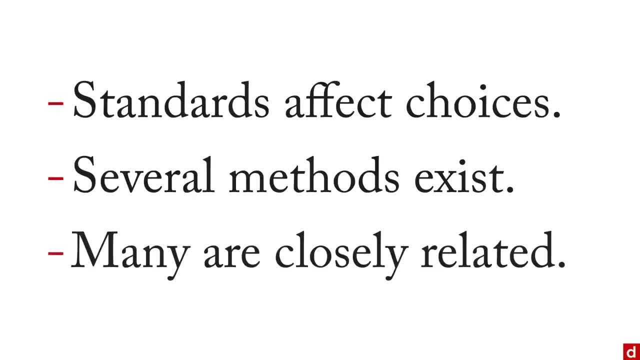 related And, under certain circumstances, they're all identical, And so it comes down to exactly what are your purposes And what do you think is going to best work with the data that you have, to give you the insight that you need in your own project. 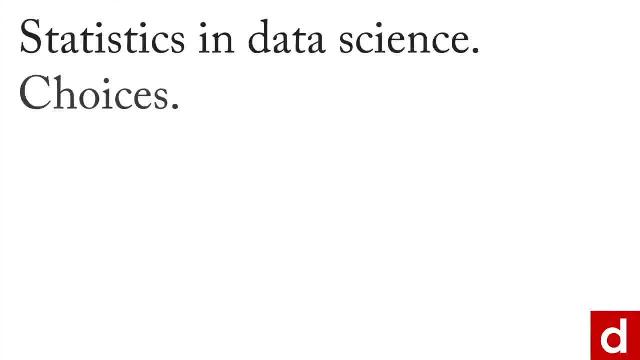 The next step we want to consider in our statistics and data science and the choices that we have to make, has to do with measures of fit, or the correspondence between the data that you have and the model that you create. Now it turns out there's a lot of different ways to measure this. 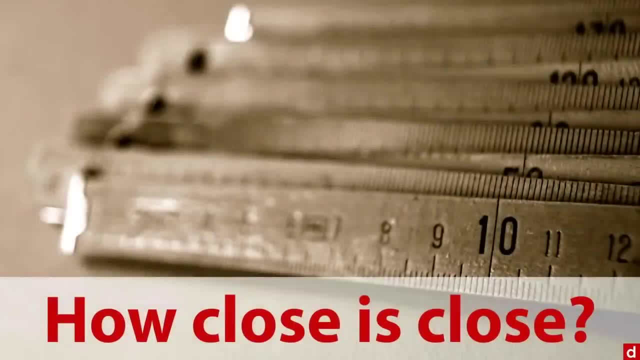 And one big question is: how close is close enough? Or how can you see the difference between the data that you have and the model that you create? How can you see the difference between the model and reality? Well, there's a few really common. 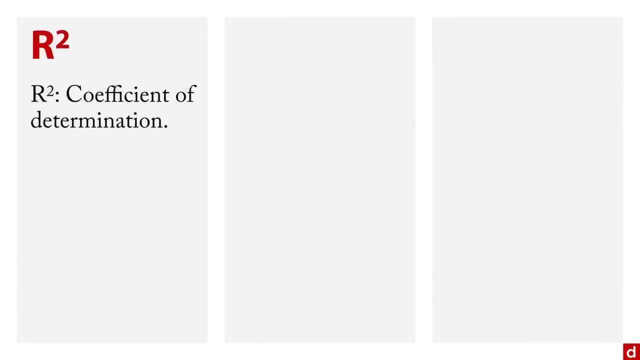 approaches to this. The first one of us called R squared- It's got a longer name. that's the coefficient of determination. There's a variation adjusted R squared which takes into consideration the number of variables. Then there's minus 2LL, which is based on the likelihood ratio. 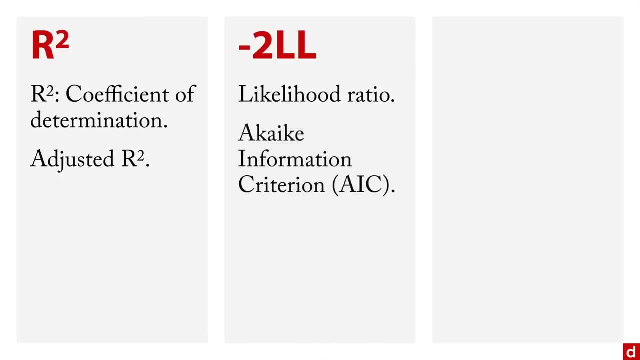 And a couple of variations: the Ikeki information criterion, or AIC, and the Bayesian information criterion, or BIC. And then there's also the Ikeki information criterion, or AIC. And then there's also chi squared Now, that's actually a Greek C there. It looks like an X, but it's a C And that's chi. 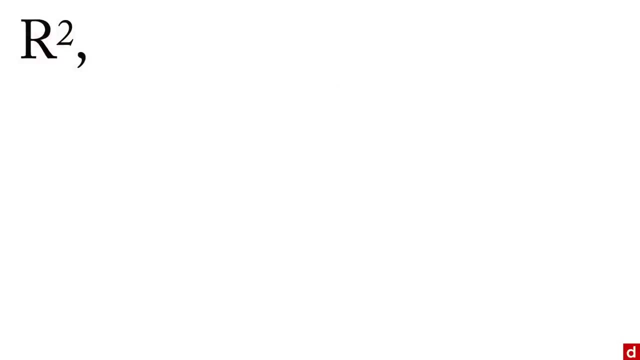 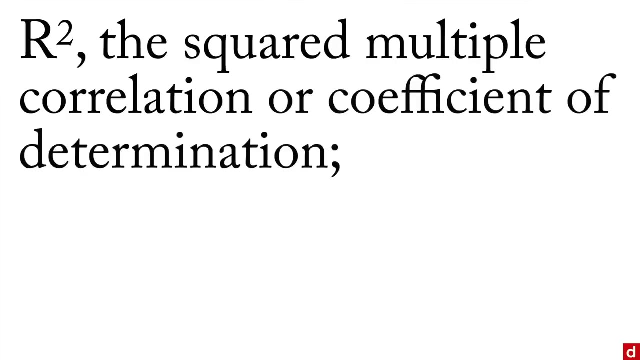 squared, And so let's talk about each of these in turn. First off is R squared. This is the squared multiple correlation, or the coefficient of determination, And what it does is it compares the variance of Y. So if you have an outcome variable, it looks at the total variance of that. 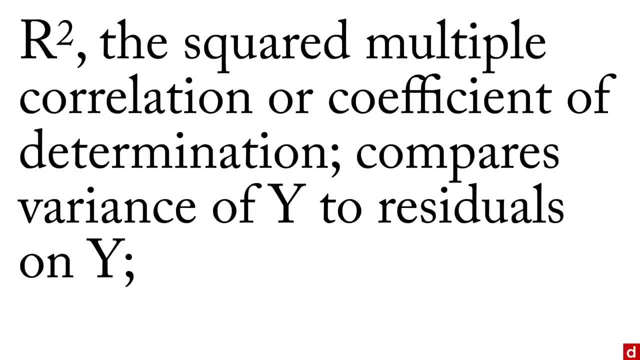 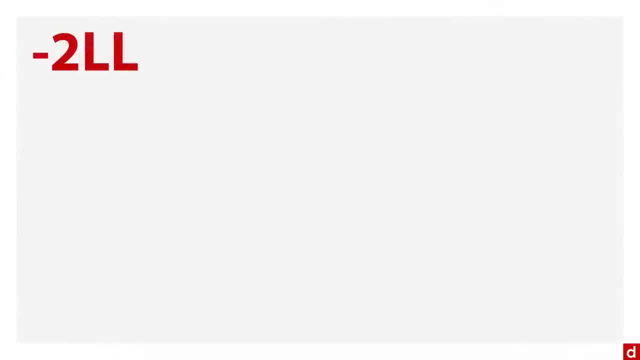 and compares it to the residuals on Y after you've made it, And then it compares it to the variance of Y after you've made your prediction. The scores on R squared range from 0 to 1, and higher is better. The next is minus 2: log likelihood, That's the likelihood ratio, or as I just 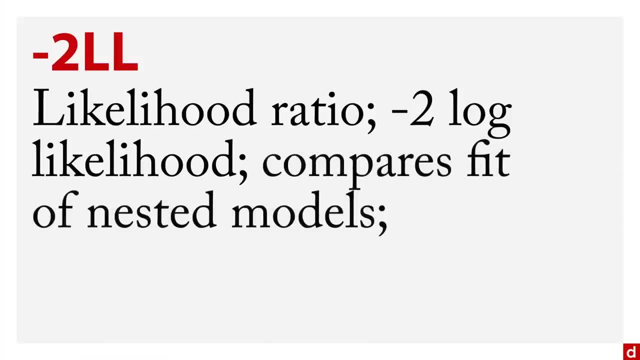 said it, the minus 2 log likelihood, And what this does is compares the fit of nested models. We have a subset, then a larger set, then a larger set overall. This approach is used a lot in logistic regression when you have a binary outcome And, in general, smaller. 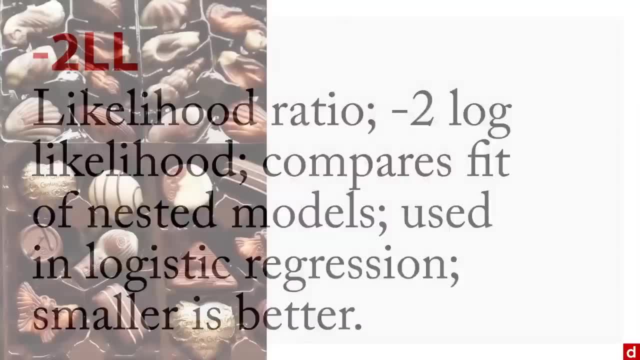 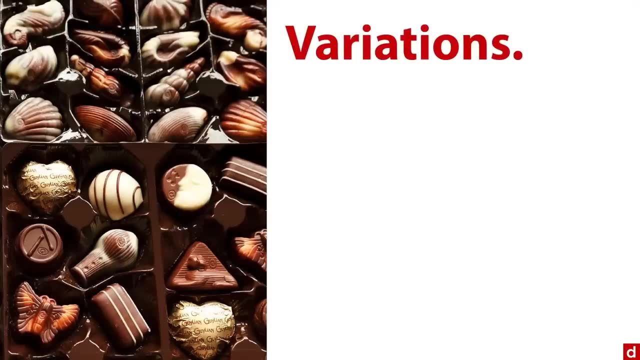 values are considered better fit. Now, as I mentioned, there's some variations of this. I like to think of variations of chocolate, The minus 2 log likelihood. there's the Akaiki information criterion, the AIC, and the Bayesian information criterion, BIC, And what both of these do is they adjust for the 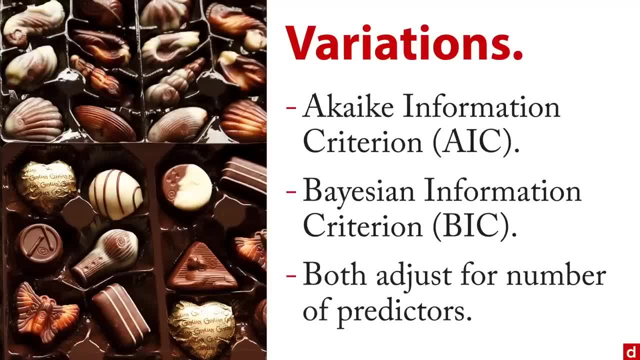 number of predictors, Because obviously if you have a huge number of predictors you're going to get a really good fit, But you're probably going to have what's called overfitting, where your model is tailored too specifically to the data you currently have and doesn't generalize. 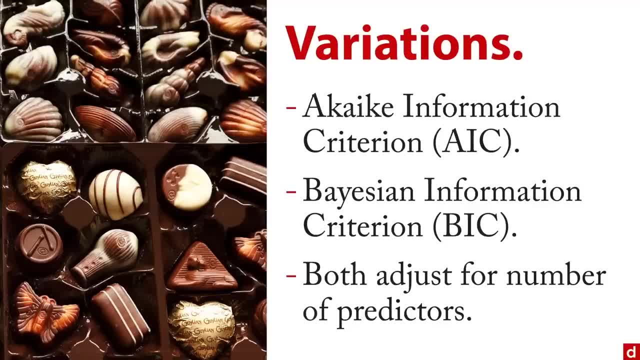 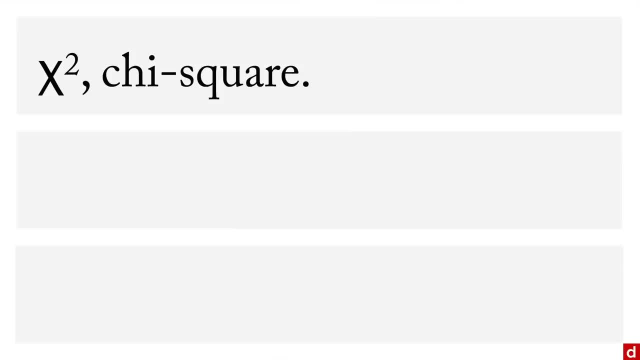 overfitting. These both attempt to reduce the effect of overfitting. And then there's chi-squared again. It's actually a lowercase Greek C looks like an X, And chi-squared is used for examining the deviations between two data sets, specifically between: 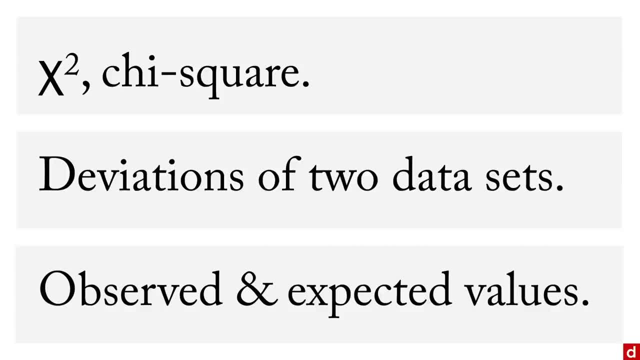 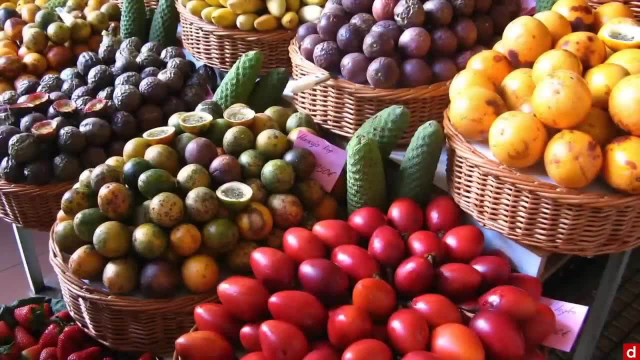 the observed data set and the expected values or a model you create that we expect this many frequencies in each category. Now I'll just mention like go ahead. There's a lot of other choices, but these are some of the most common standards. 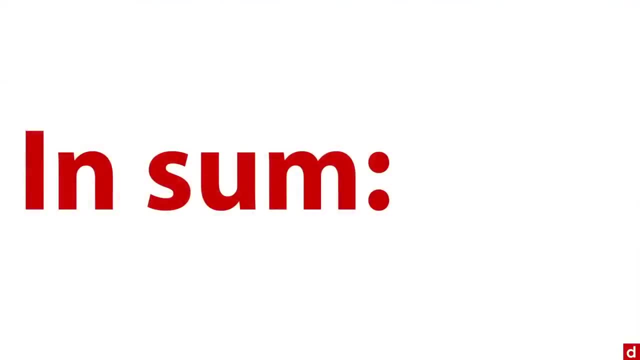 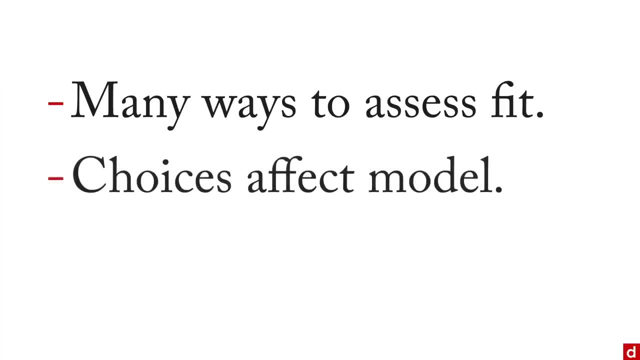 particularly the R-squared. And I just want to say in sum, there are many different ways to assess the fit, the correspondence between a model and your data, And the choices affect the model you know especially. are you going to penalize for throwing in too many variables relative to? 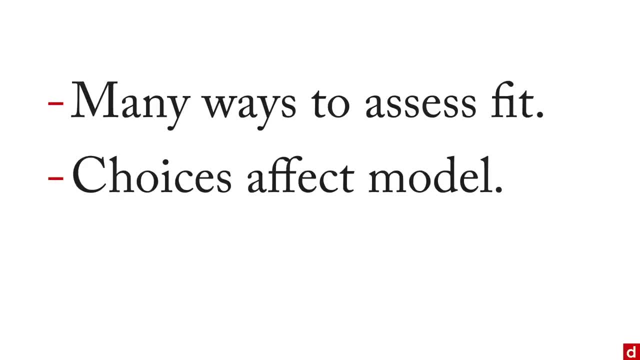 your number of cases? Are you dealing with a quantitative or a binary outcome? Those things all matter, And so the most important thing- as a always my standing advice- is: keep your goals in mind and choose a method that seems to fit best with your analytical strategy and the insight you're trying to get from your 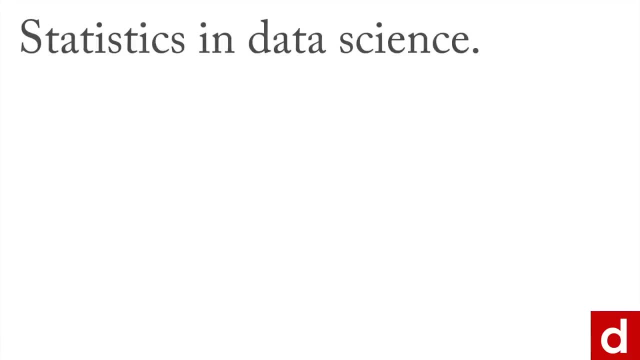 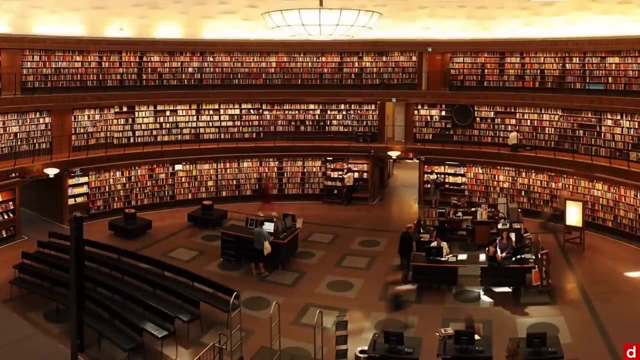 data, The statistics and data science offers a lot of different choices. One of the most important is going to be feature selection, or the choice of variables to include in your model. It's sort of like confronting this enormous range of information and trying to choose what matters. 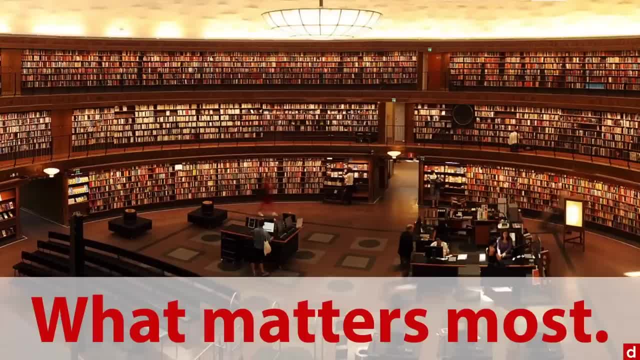 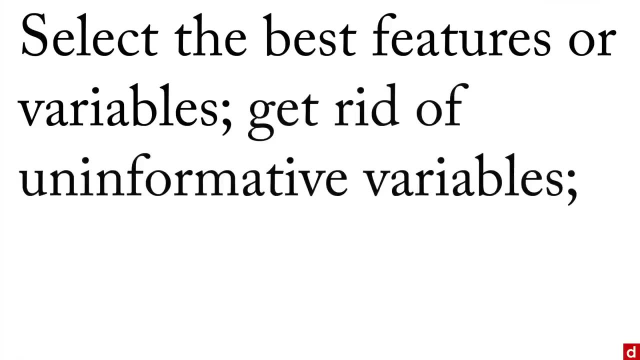 most. The goal of feature selection is to select the best features or variables and get rid of uninformative and noisy variables and simplify the statistical model that you're creating, because that helps avoid overfitting or getting a model that works too well with the current data. 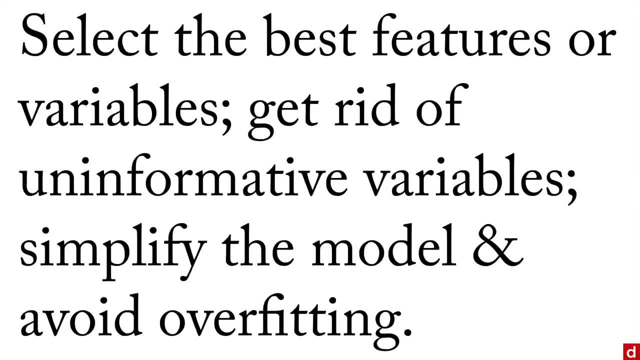 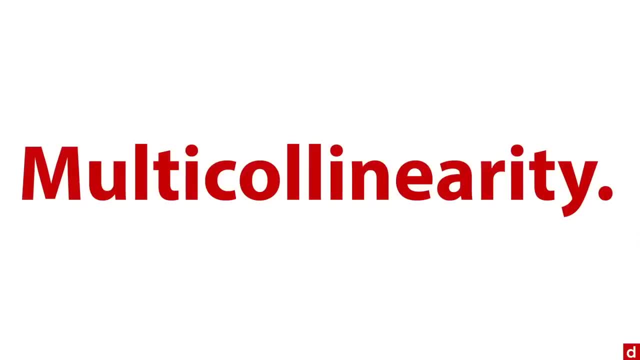 and works less well with other data. The major problem here is multi-collinearity- very long word that has to do with the relationship between the model and the data, And that's what we're going to talk about today. So let's talk about the relationship between the predictors and the model. I can show it. 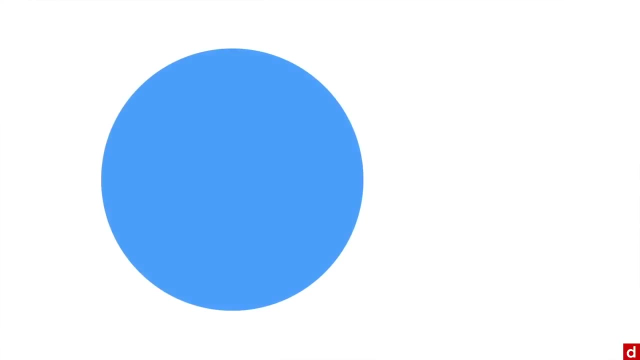 to you graphically here. Imagine, for instance, we've got a big circle here to represent the variability in our outcome variable. We're trying to predict it And we've got a few predictors. So we've got predictor number one over here and you see it's got a lot. 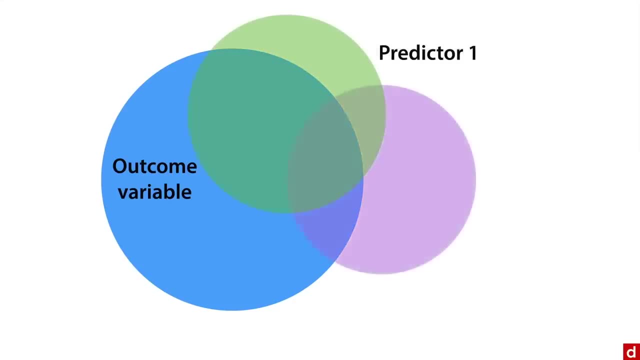 of overlap, That's nice. Then we've got predictor number two here. It also has some overlap with the outcome, but it also overlaps with predictor one. And then finally down here we've got predictor three, which overlaps with both of them, And 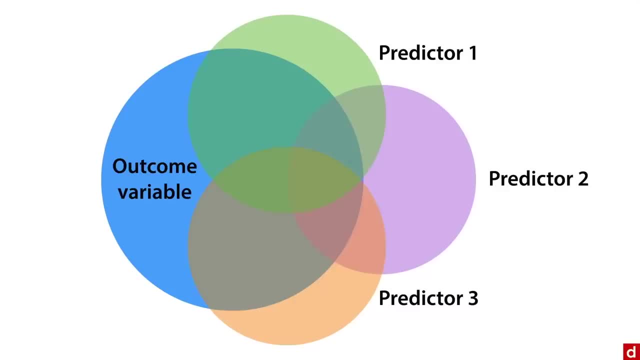 the problem here is that predictor one overlaps with predictor two. And then finally down here we've got predictor three, which overlaps with both of them, And the problem is that predictor three, which overlaps with predictor two, summarizes the overlap between the predictors and the outcome variable. 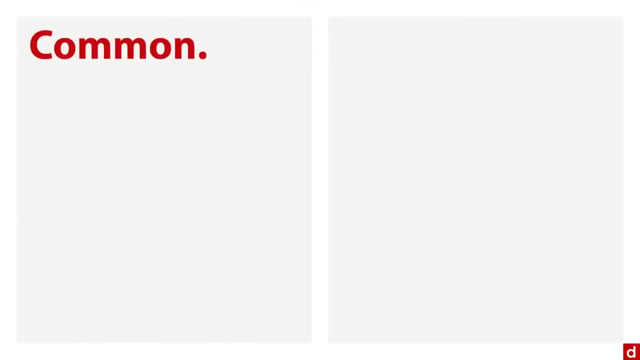 Now there's a few ways of dealing with this. Some of these are pretty common. So, for instance, there is the practice of looking at probability values and regression equations. There are standardized coefficients and there's variations on sequential regression. There are also newer procedures for dealing with the disentanglement of the association between the predictors. 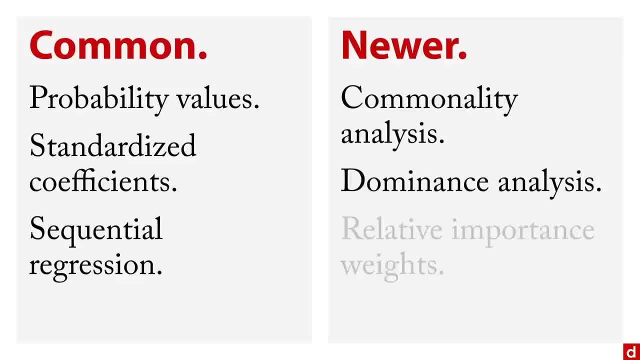 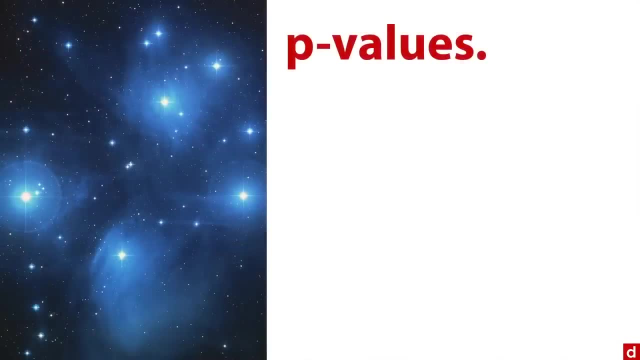 There's something called commonality analysis, there's dominance analysis and there are relative importance weights. Of course, there are many other choices in both the common and the newer, But these are a few that are worth taking special look at. First is p values or probability values. This is the simplest method. 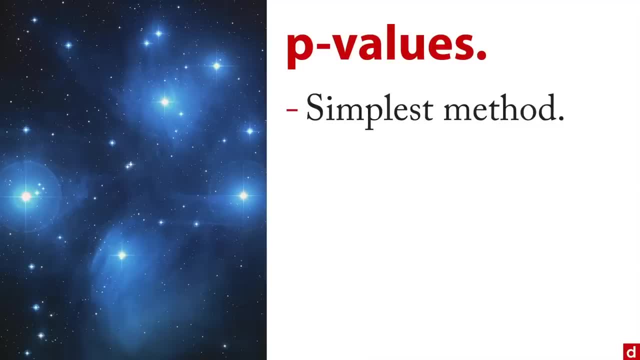 because most statistical packages will calculate probability values for each predictor And they'll put little asterisks next to it, And so what you're doing is you're looking at the p values, the probabilities for each predictor, or, more often, the asterisks next to it, which sometimes 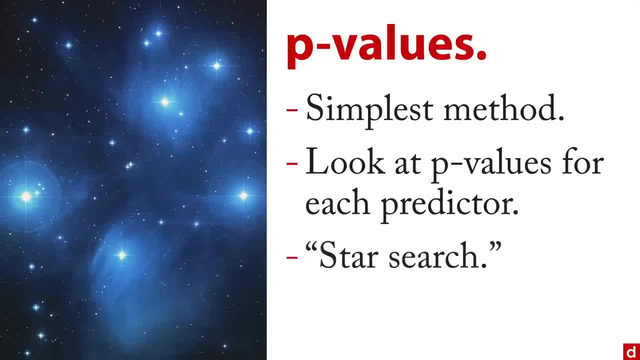 give it the name of star search, just kind of cruising through a large output of data and just looking for the stars or asterisks. This is fundamentally a problematic approach for a lot of reasons. The problem here is you're looking individually and it inflates false positives. 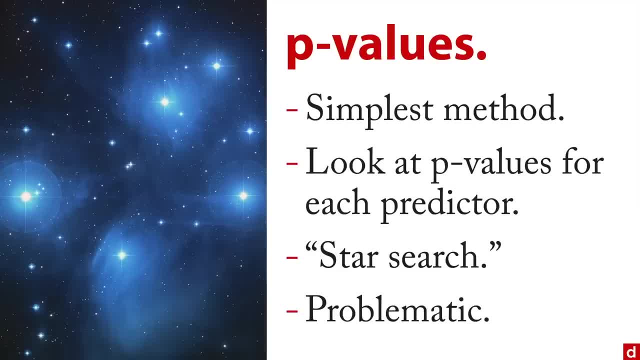 say you have 20 variables, each is entered and tested with an alpha or false positive of 5%, If you end up with nearly a 65% chance of at least a false one- false positive in there. it's distorted by sample size. 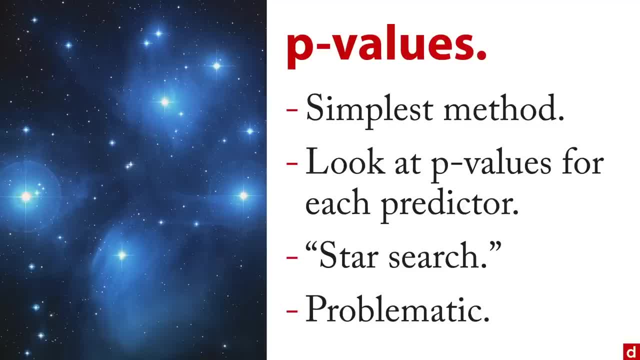 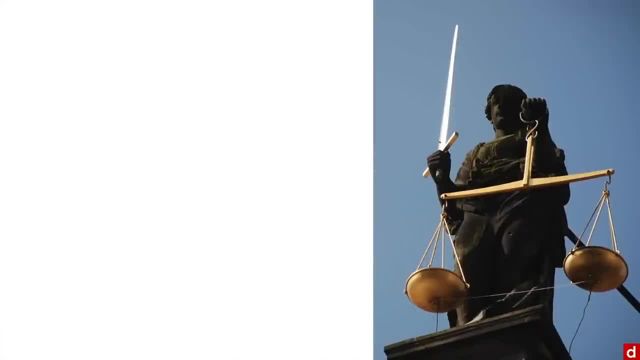 because with a large enough sample, anything becomes statistically significant, And so relying on p values can be a seriously problematic approach. slightly better approach is to use betas or standardized regression coefficients, And this is where you put all the variables on the same scale, So usually standardized from zero and then to either minus. 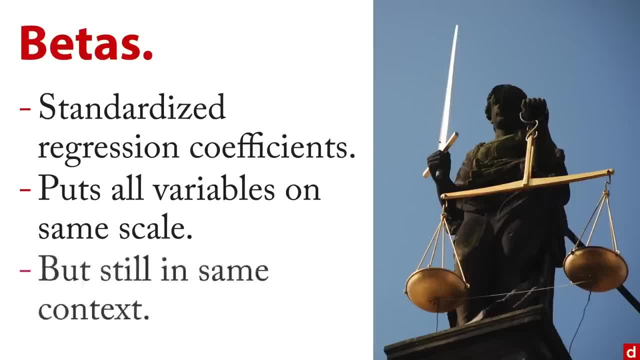 one plus one or with a standard deviation of one. The trick is, though, they're still in the same context of each other And you can't really separate them, Because those coefficients are only valid when you take that group of predictors as a whole. So one way to try to get around that. 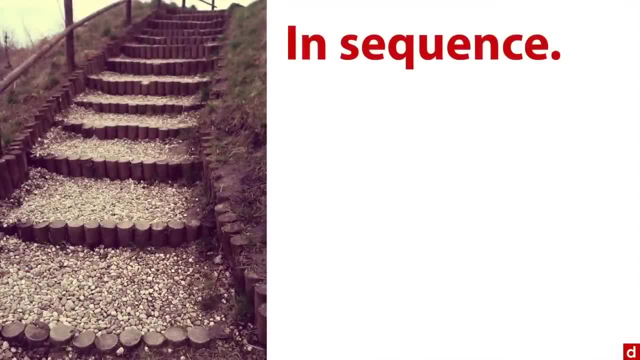 is to do what they call stepwise procedures, where you look at the variables in sequence. There are several versions of sequential regression that allow you to do that. you can put the variables into groups or blocks and enter them in blocks and look at how the equation 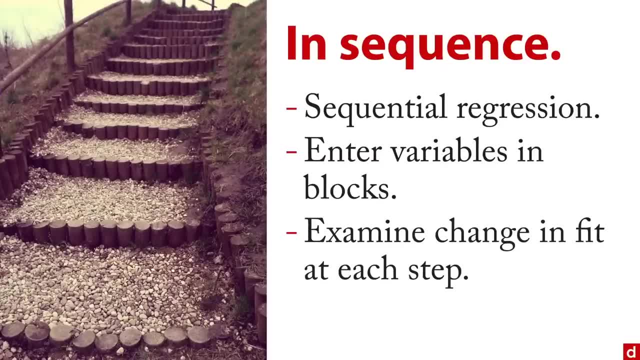 changes Overall, you can examine the change in fit at each step. The problem with a stepwise procedure like this is it dramatically increases the risk of overfitting, which again is a bad thing if you want to generalize your data And so to deal with this there's a whole collection. 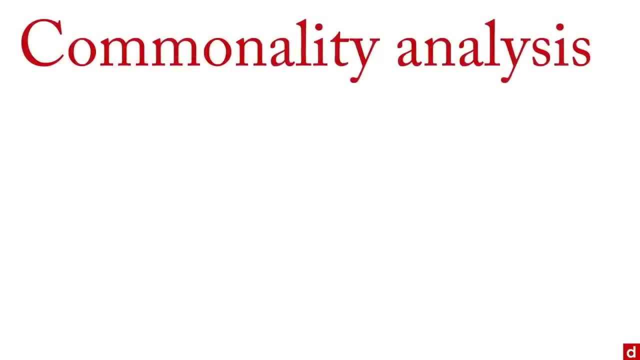 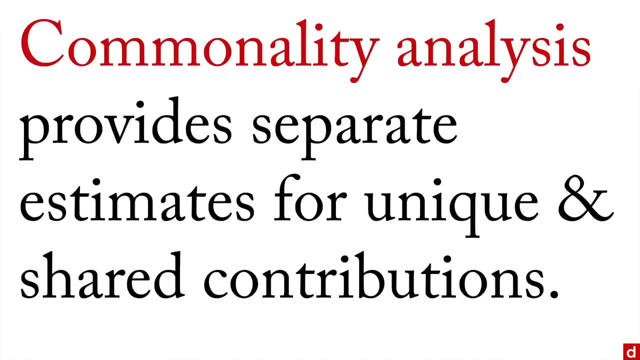 of newer methods. A few of them include commonality analysis, which provides separate estimates for the unique and shared contributions of each variable. Well, that's a neat statistical trick, but that's a different story. So let's take a look at the commonality analysis, which provides separate estimates for the unique and shared contributions of each variable. Well, that's a neat statistical trick, but 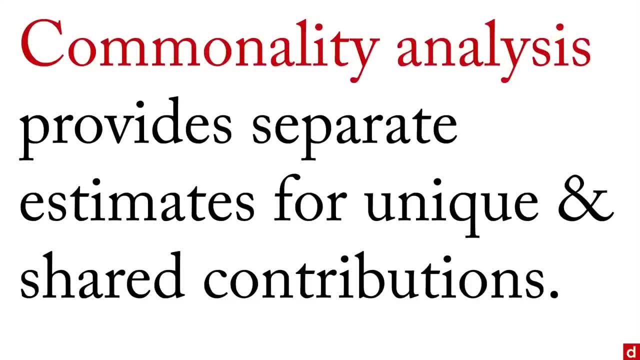 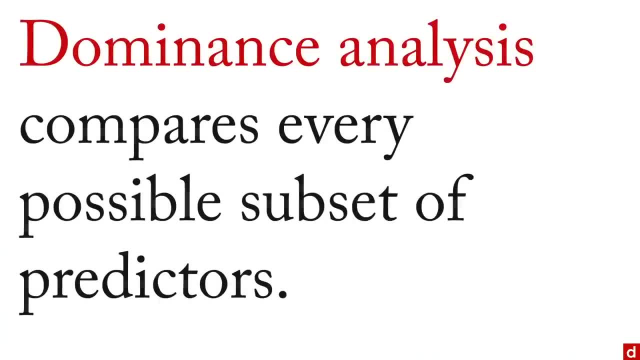 the problem is it just moves the problem of disentanglement to the analyst, So you're really not better off than you were. as far as I can tell, There's dominance analysis which compares every possible subset of predictors. Again, sounds really good, But you have the problem known as. 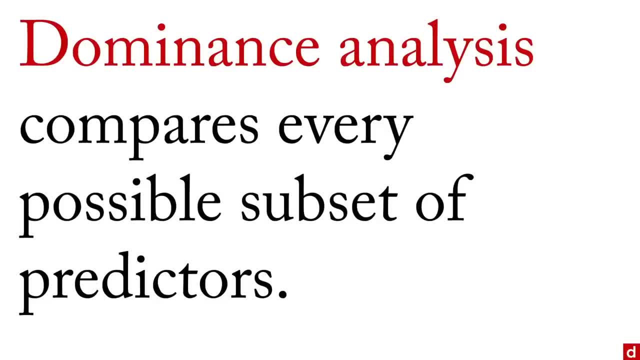 the combinatorial explosion. If you have 50 variables that you could use- and I, there are some that have millions of variables. With 50 variables, you have over one quadrillion possible combinations. You're not going to finish that in your lifetime And it's also really hard to get things like 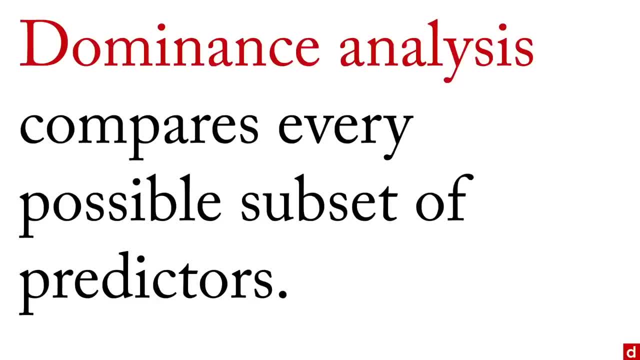 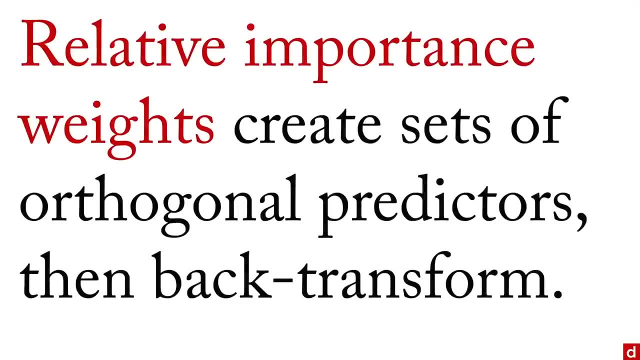 standard errors and perform inferential statistics with this kind of model. Then there's also something that's even more recent than these others, called relative importance weights, And what this does is it creates a set of predictors that are orthogonal or uncorrelated with each other, basing them off of the originals, And then it predicts the scores, and then 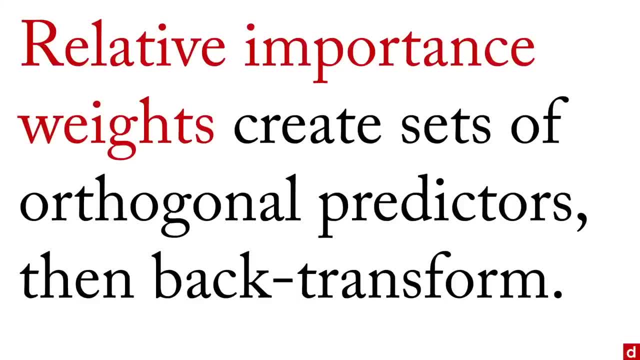 it can predict the outcome without the multi collinear cases. New predictors are uncorrelated. It then rescales the coefficients back to the original variables- That's the back transform, And then from that it assigns relative importance or a percentage of explanatory power to each predictor variable. Now, despite this very different approach, 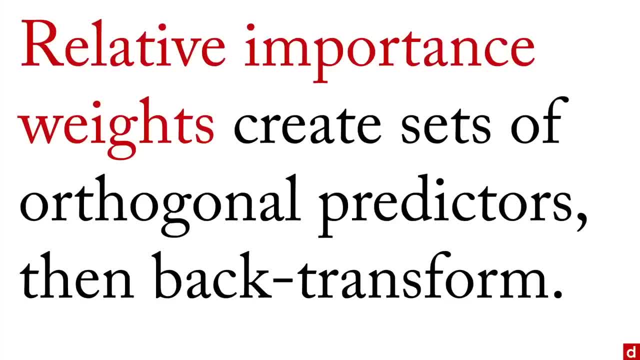 it tends to have results that resemble dominance analysis. It's actually really easy to do. There are websites you just plug in your information and it does it for you, And so that's yet another way of dealing with the problem of multi collinearity. 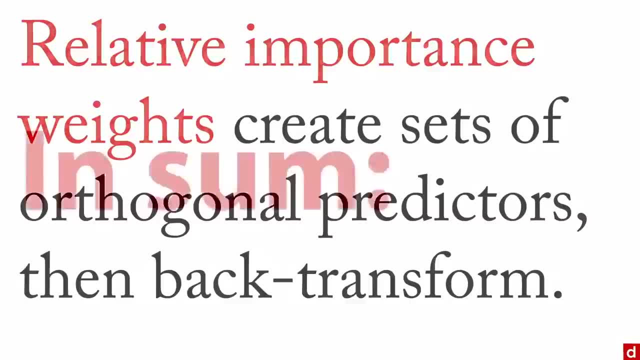 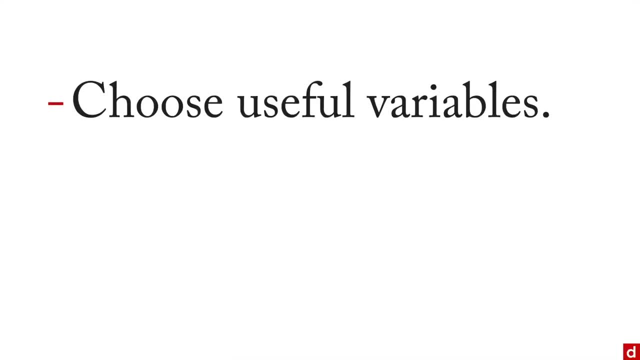 And trying to disentangle the contribution of different variables. In sum, let's say this: What you're trying to do here is choose the most useful variables to include into your model. make it simpler, be parsimonious. Also, reduce the noise and distractions in. 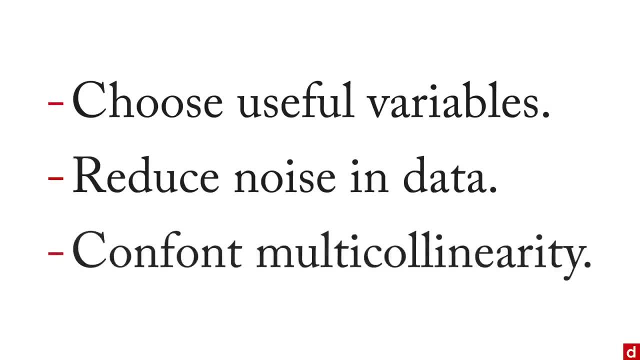 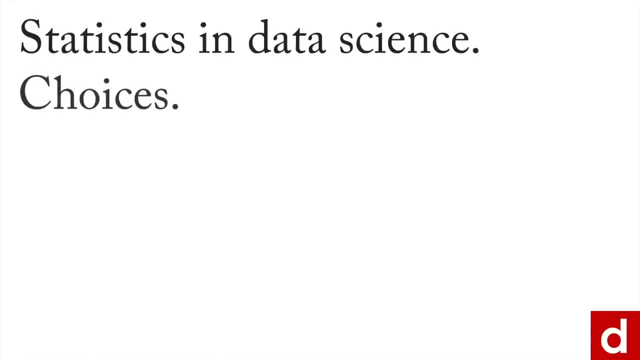 your data And in doing so, you're going to always have to confront the ever present problem of multi collinearity or the association between the predictors in your model, with several different ways of dealing with that. As we continue our discussion of statistics and the choices that are made, one important 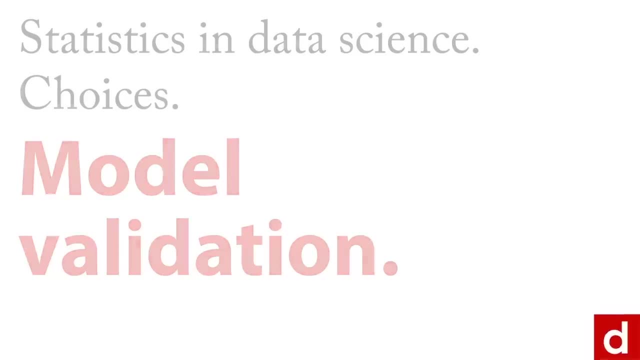 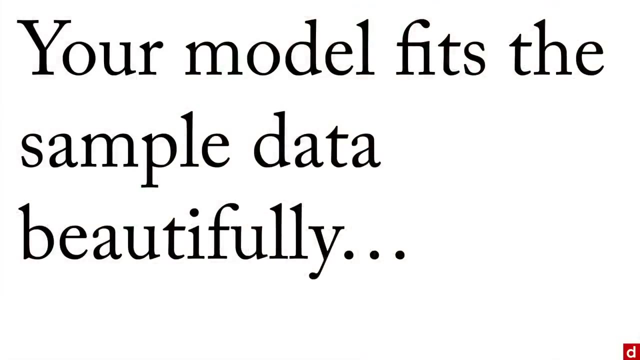 consideration is model validation And the idea here is: as you're doing your analysis, are you on target? More specifically, your model that you create through regression or whatever you do, your model fits the sample data beautifully. you've optimized it there. 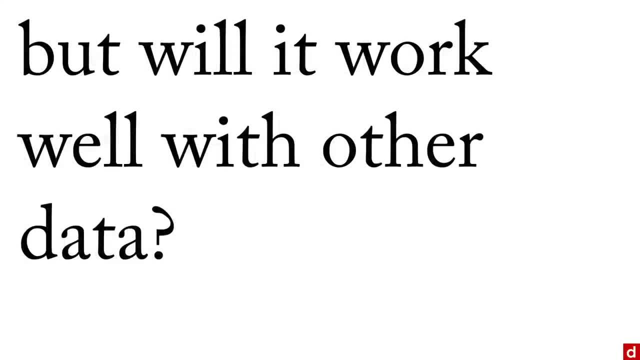 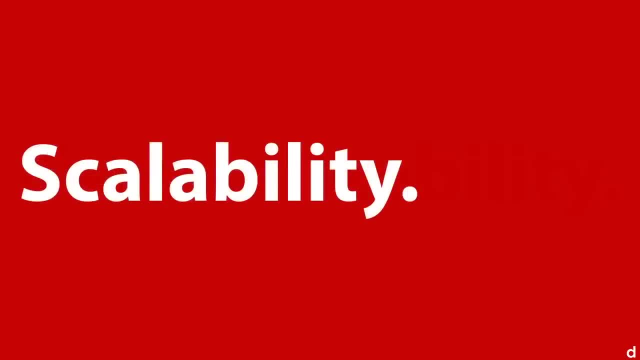 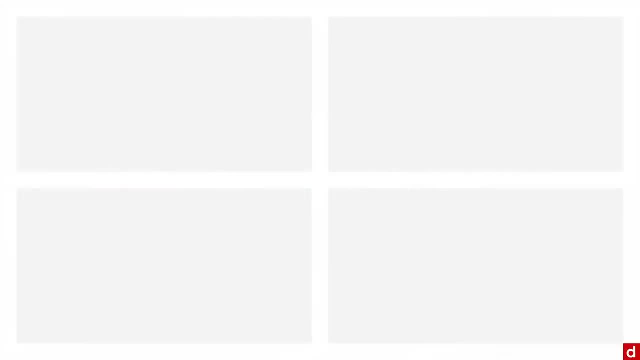 but will it work well with other data? Fundamentally, this is the question of: well, what's the generalizability, Also sometimes called scalability, because you're trying to apply it in other situations And you don't want to get too specific, or it won't work in other situations. 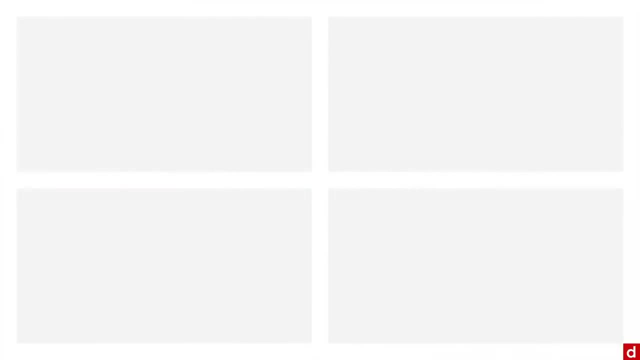 Now there are a few general ways of dealing with this and trying to get some sort of generalizability. Number one is Bayes, a Bayesian approach. Then there's replication, Then there's something called holdout validation, And then there's cross validation. I'll discuss each of these. 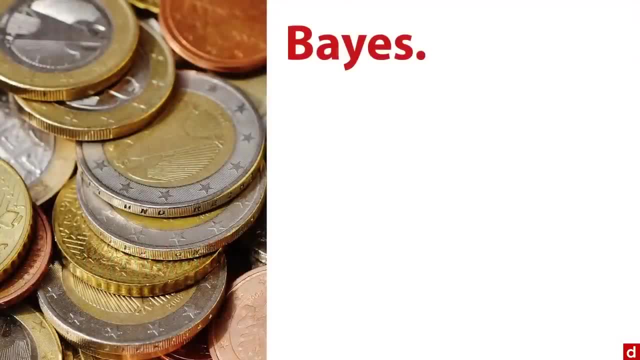 very briefly in conceptual terms. The first one is Bayes, And the idea here is you want to get what are called posterior probabilities. Most analyses give you a probability value for the data given the hypothesis. So you have to start with an assumption about the hypothesis, But instead it's possible. 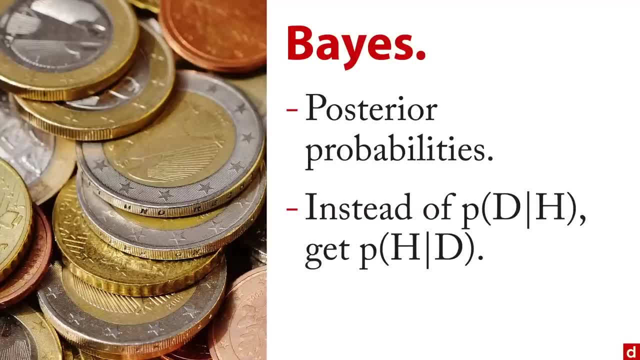 to flip that around by combining it with special kinds of data to get the probability of the hypothesis given the data. And that is the purpose of Bayes' theorem, which I've talked about elsewhere. Another way of finding out how well things are going to work is through replication. 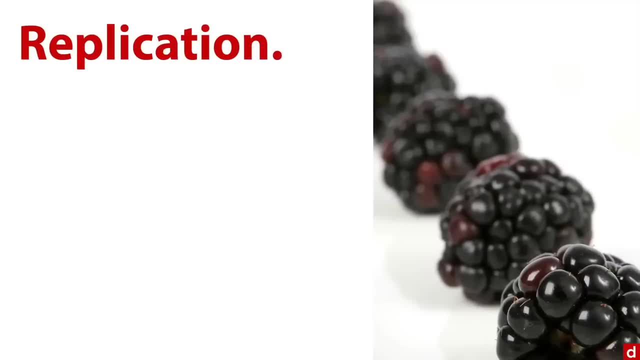 That is, do the study again. It's considered the gold standard in many different fields. The question is whether you need an exact replication or a conceptual one that is similar in certain respects. You can argue for both ways, But one thing you want to do is when. 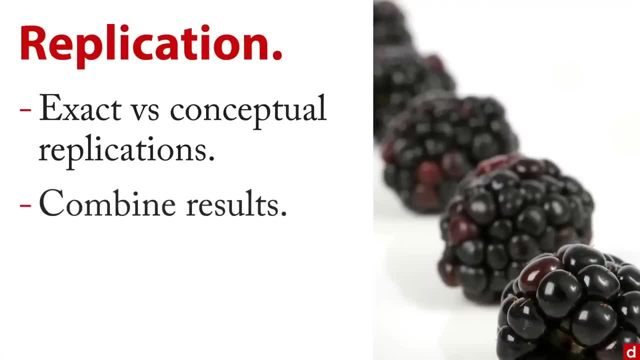 you do a replication, then you actually want to combine the results And what's interesting is the first study can serve as the Bayesian prior probability for the second study, So you can actually use meta-analysis or Bayesian methods for combining the data from the two. 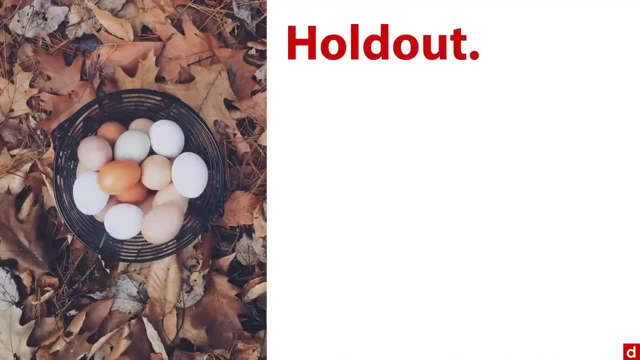 of them. Then there's holdout validation. This is where you build your statistical model on one part of the data and you test it on another. I like to think of it as the eggs in separate baskets. The trick is that you need a large sample in order to have enough to do these. 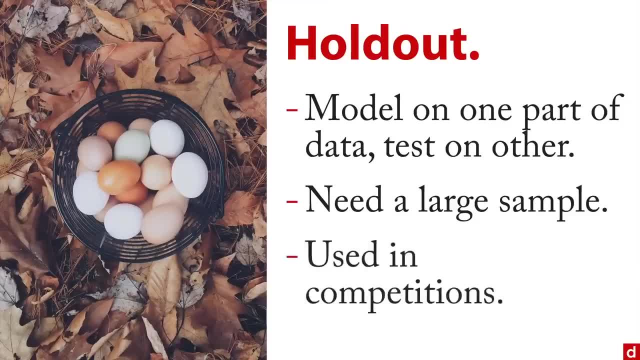 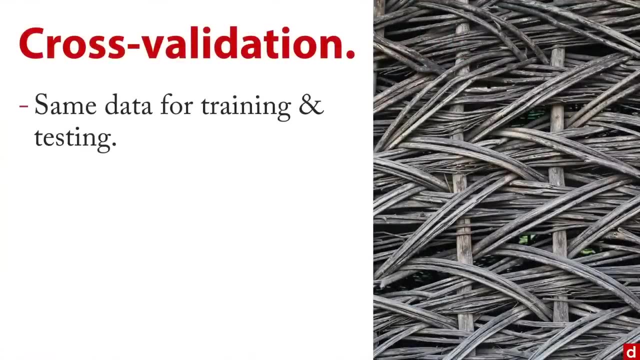 two steps separately. On the other hand, it's also used very often in data science competitions as a way of having a sort of gold standard for a sample. Finally, I'll just mention one more, and that's cross-validation. This is when you 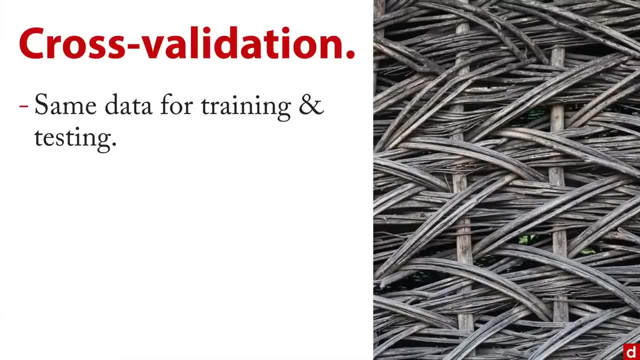 use the same data for both training and for testing or validating. There are several different versions of it and the idea is you're not using all the data at once, but you're kind of cycling through and weaving the results together. There's leave-one-out where you 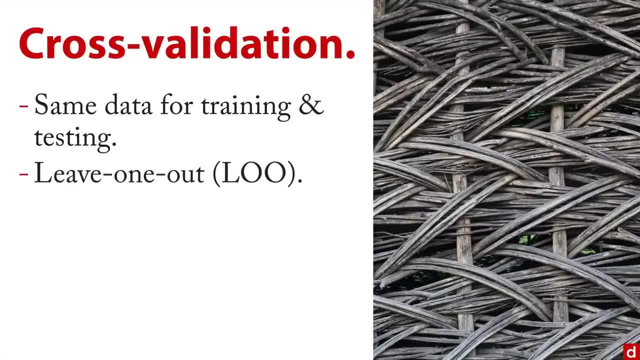 leave out one case at a time, also called LOO- L-O-O. There's leave-P-out, where you leave out a certain number of cases at a time, also called LOO- L-O-O. There's leave-P-out. 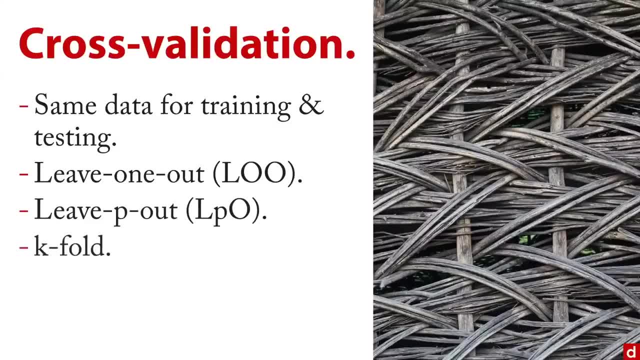 where you leave out a certain number at each point. There's K-fold, where you split the data into, say for instance, 10 groups and you leave out one and you develop it on the other nine, and then you cycle through And there's repeated random subsampling where 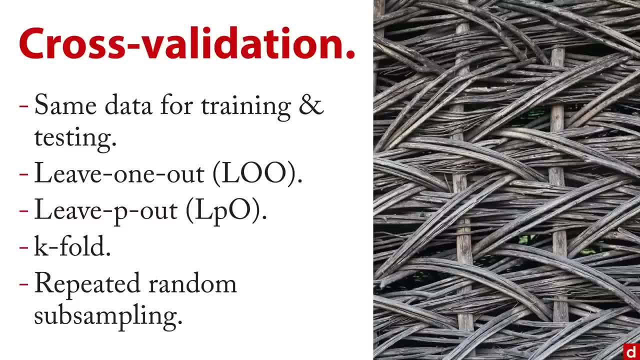 you use a random process at each point. Any of those can be used to develop the model on one part of the data and test it on another, and then cycle through to see how well it holds up under different circumstances. And so, in sum, I can say this about validation: You want to make your analysis count by your 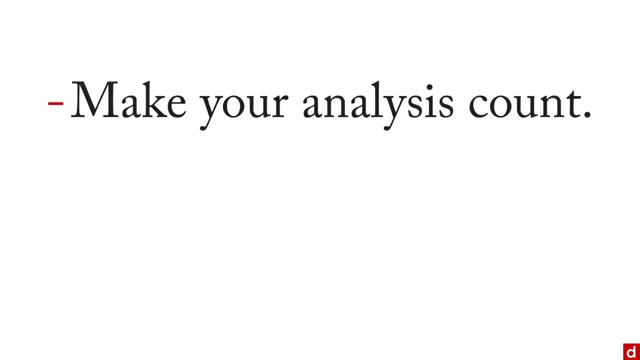 testing how well your model holds up, from the data you developed it on, to other situations, because that's really what you're trying to accomplish. This allows you to check the validity of your analysis and your reasoning and it allows you to build confidence in the utility. 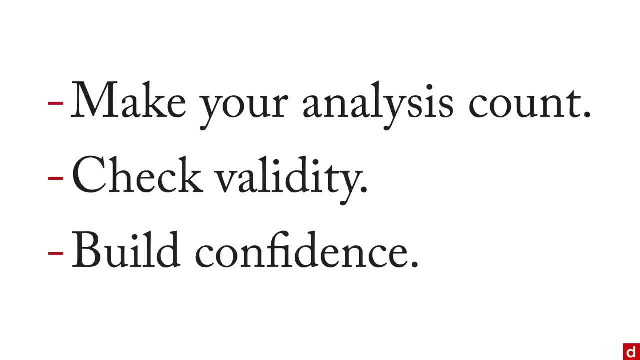 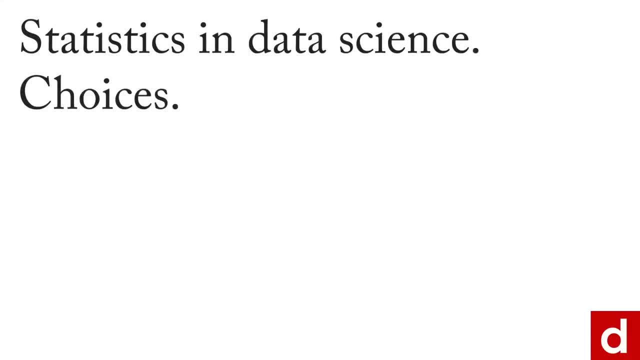 of your results. To finish up our discussion of statistics and data science and the choices that are involved, I want to mention something that really isn't a choice, but more an attitude, and it's DIY for do-it-yourself. The idea here is really: you just need to get started. 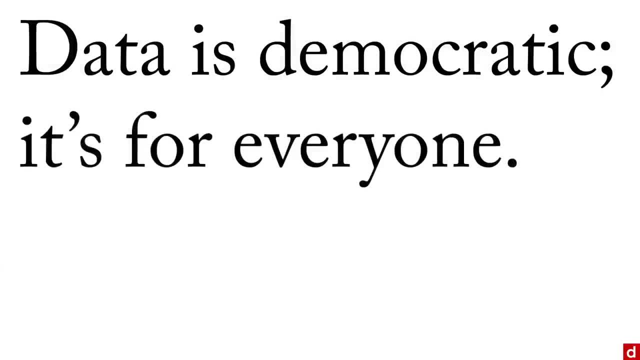 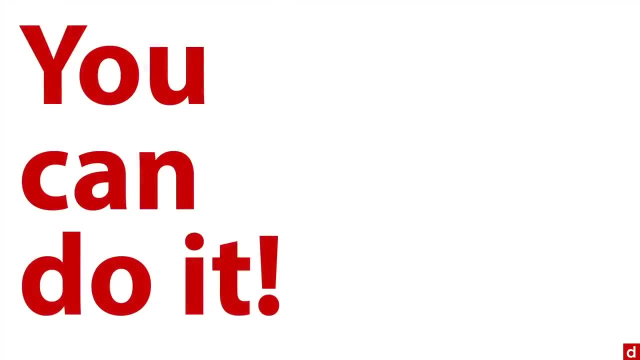 Remember: data is democratic. It's there for everyone. Everybody has data. Everybody works with data, either explicitly or implicitly. Data is democratic, so is data science Really. my overall message is: you can do it. A lot of people think you have to be at this totally. 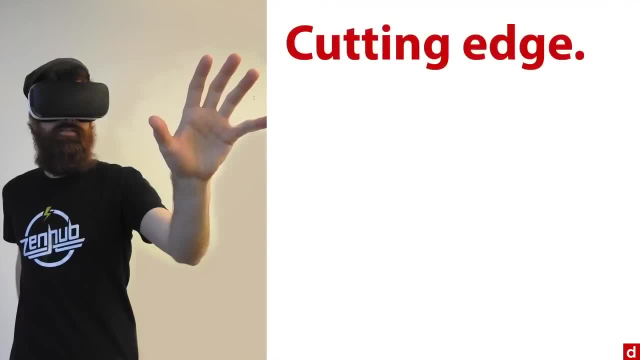 cutting edge virtual reality sort of thing, And it's true there's a lot of active development going on in data science. there's always new stuff. The trick, however, is the software that you can use to implement those things often lags. It'll show up first in programs like R and Python, But as far 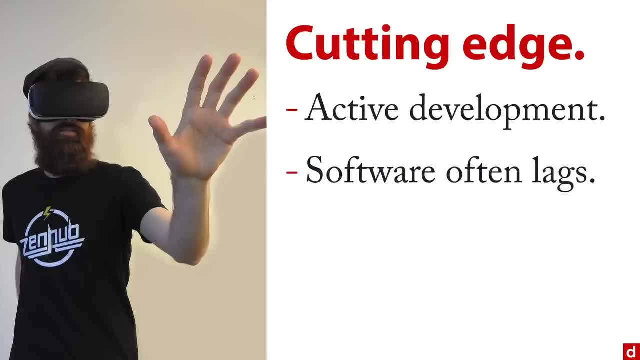 as it's showing up in a point and click program. that could be years. What's funny, though, is often these cutting edge developments don't really make much of a difference in the results of the interpretation. They may in certain edge cases, but usually not a huge difference, And so I'm just 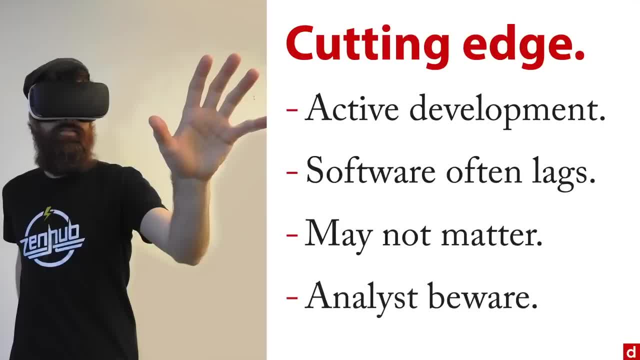 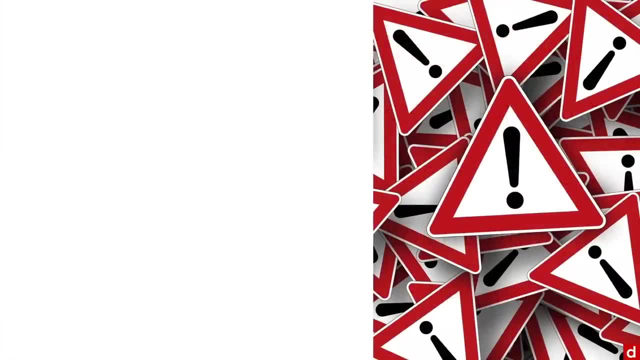 going to say: analyst, beware, you don't necessarily have to do it. it's pretty easy to do them wrong, And so you don't have to wait for the cutting edge. Now, that being said, and do want you to pay attention to what you're doing- A couple of things I've said repeatedly- is know your goal. 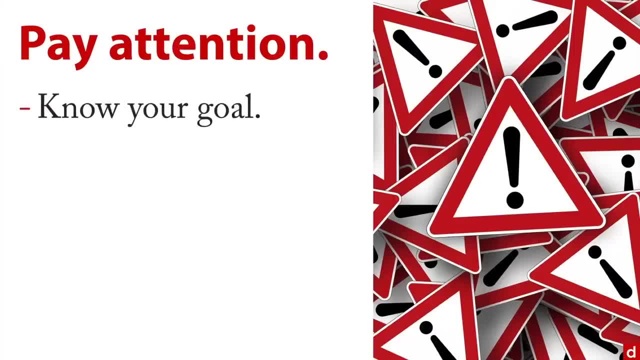 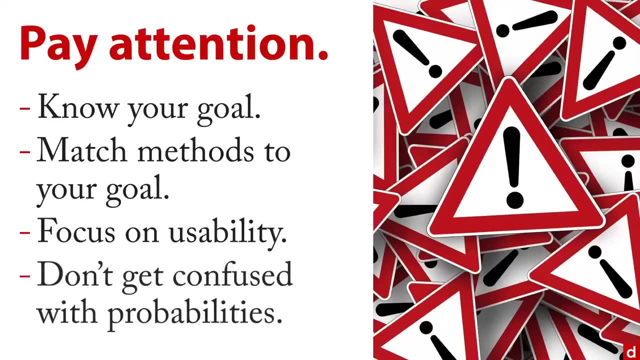 Why are you doing this study? Why are you analyzing data? What are you hoping to get out of it? Try to match your methods to your goal. be goal directed. focus on the usability. will you get something out of this that people can actually do something with? And then, as I've mentioned several times, 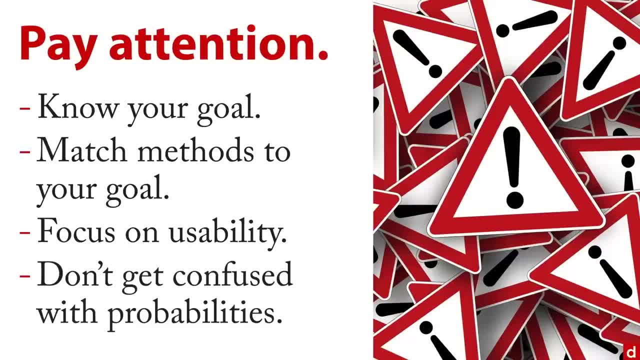 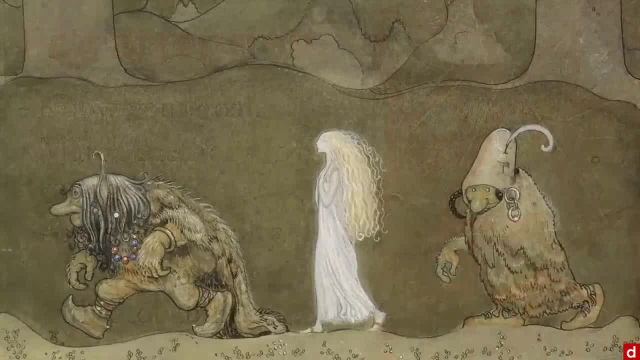 with the Bayesian thing. don't get confused with probabilities. Remember that priors and posteriors are different things, just so you can interpret things accurately. Now I want to mention something that's really important to me personally, And that is: beware the trolls. 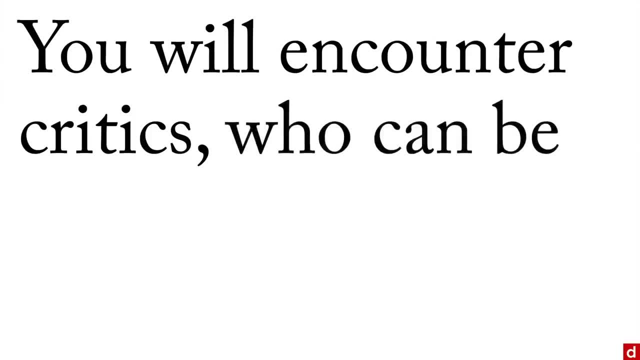 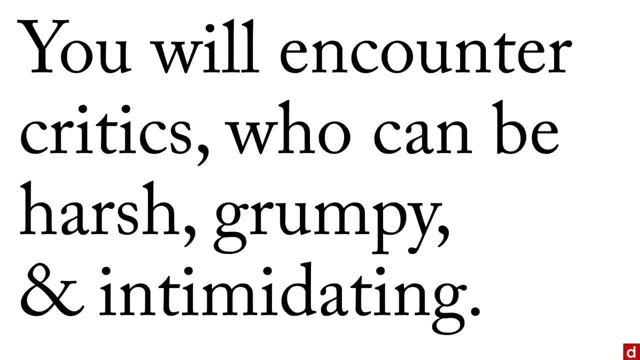 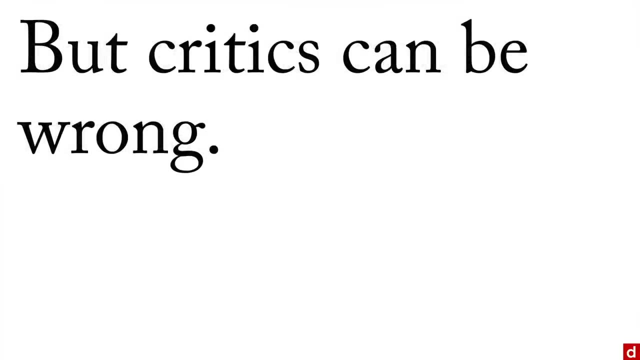 You will encounter critics, people who are very vocal and who can be harsh and grumpy and really just intimidating, And they can really make you feel like you shouldn't do stuff because you're going to do it wrong. But the important thing to remember is the critics can be wrong. Yes, 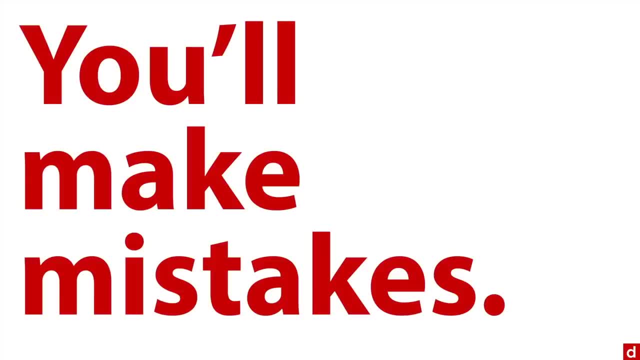 you'll make mistakes. Everybody does, You know. I can't tell you how many times I have to write my code more than once to get it to do what I want it to do, But in analysis, everything is completely wasted if you pay close attention. I've mentioned this before. 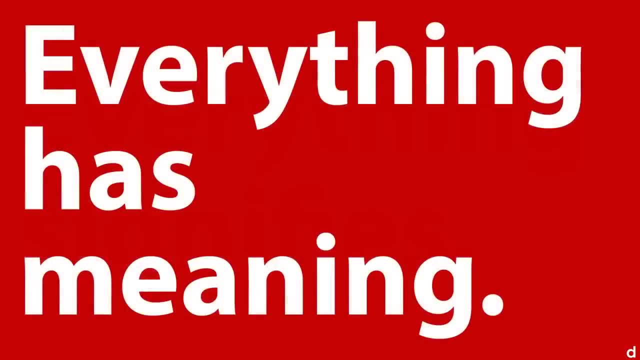 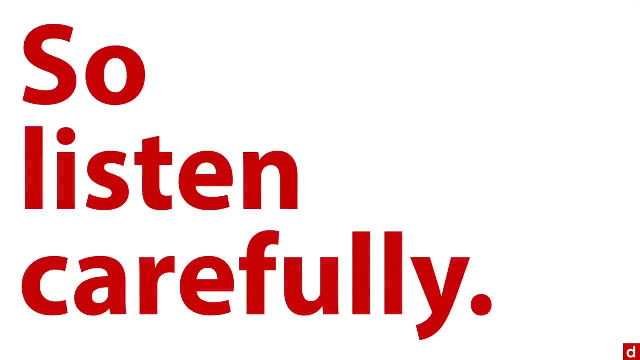 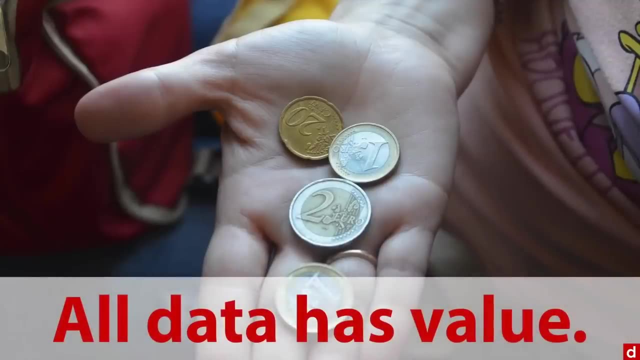 everything signifies, or, in other words, everything has meaning. The trick is that the meaning might not be what you expected it to be, So you're going to have to listen carefully, And I just want to reemphasize: all data has value, So make sure you're listening carefully. In sum, let's say: 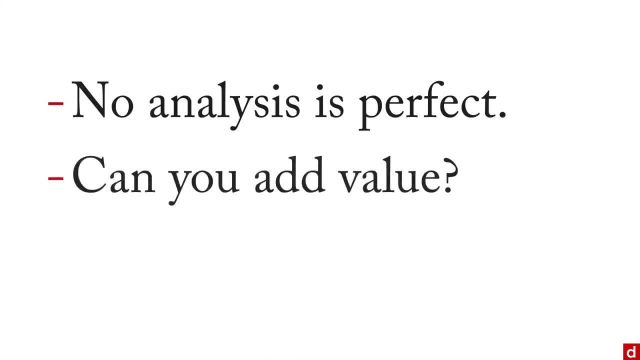 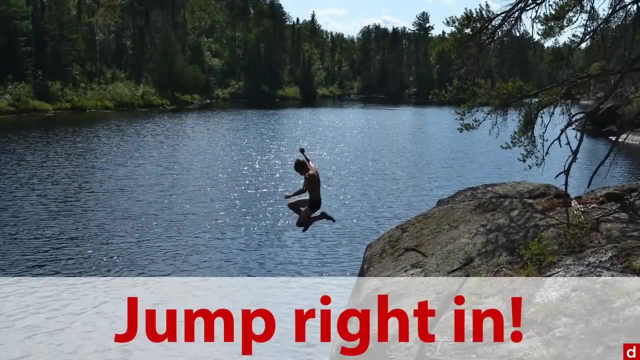 this: no analysis is perfect. The real question is not: is your analysis perfect? But can you add value? And I'm sure that you can, And fundamentally, data is democratic. So I'm going to finish with one more picture here, And that is: just jump right in and get started. You'll. 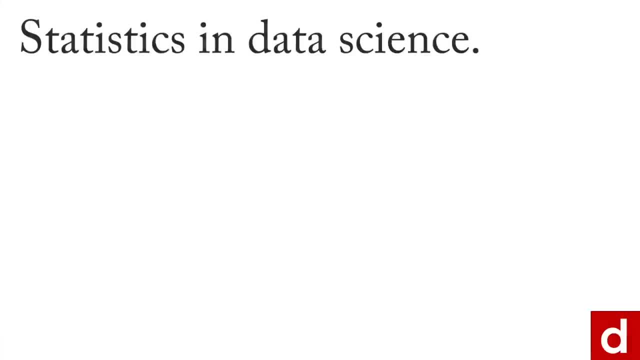 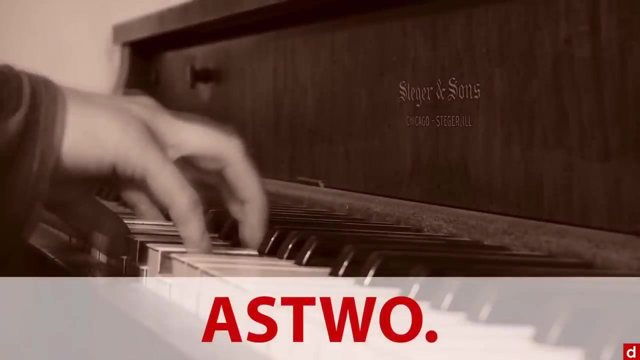 be glad you did To wrap up our course, statistics and data science. I want to give you a short conclusion and some next steps. Mostly, I want to take a little piece of advice. I learned from a professional saxophonist, Kirk Whalum, And he says there's always something to do, And I'm 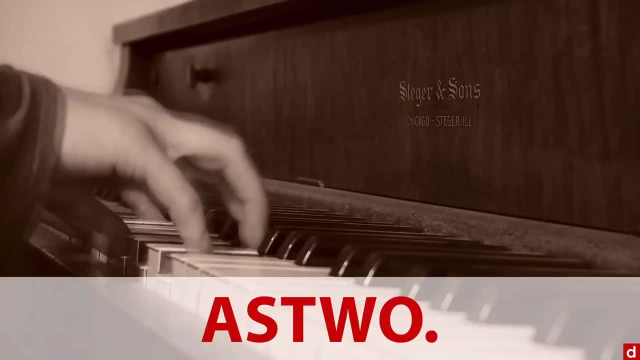 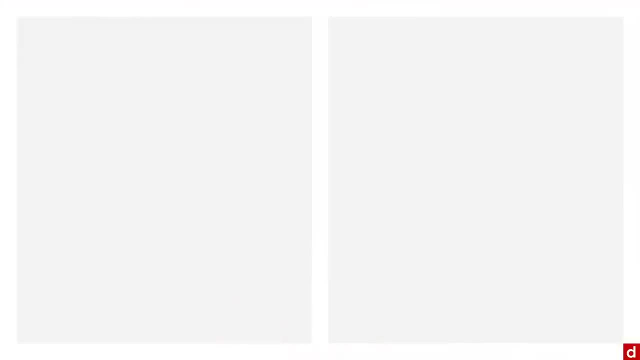 going to tell you there's always something to work on. There's always something you can do to try things differently to get better. It works when practicing music. It also works when you're dealing with data. Now there are additional courses here at datalabcc that you might want.